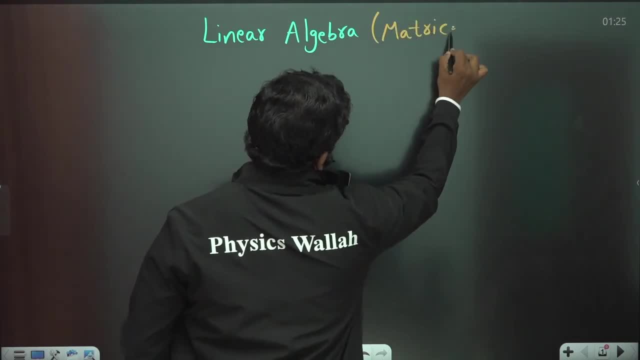 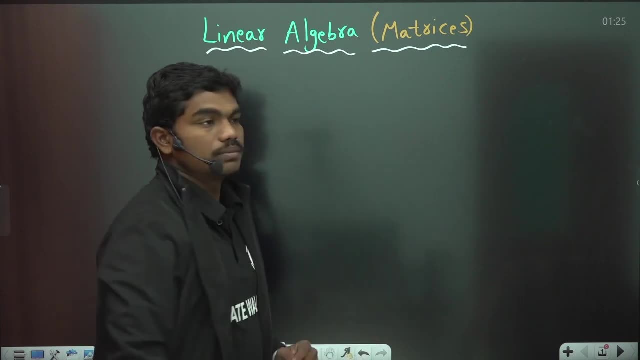 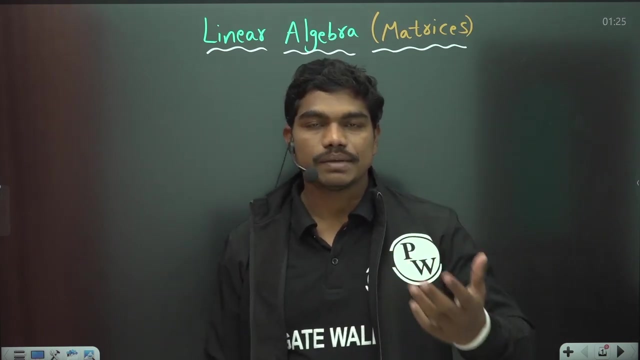 called Mathesis, So many of you might have studied a bit of this with the name of this subject, as the name of this particular module, as linear algebra. Now, this medium of teaching will be in English and nowadays, you know, English is basically the language of the education and 80%. 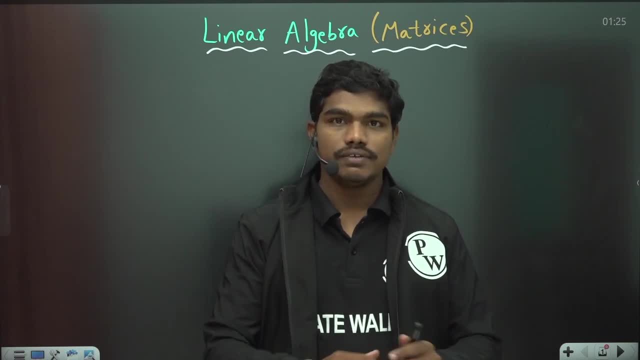 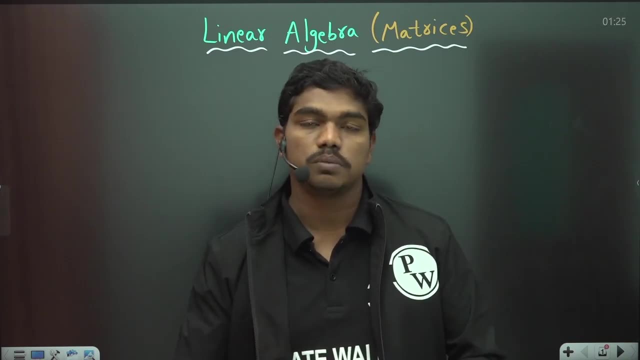 of the books across the world are written in English. And I'm telling you one thing: even if you secure a good admission in some IITs or IIC, Bangalore, in India at least you will experience, all of your professors almost will teach you in English. So I 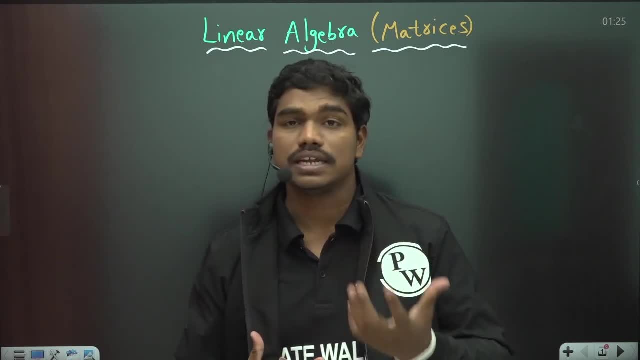 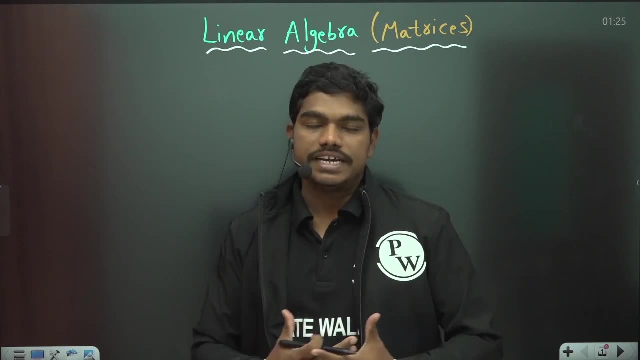 you know, I suggest you basically to have the understanding of the things in things in English and definitely this will definitely, you know, help you out. Okay, so straight away going to this chapter where you use this linear algebra. if you ask this question to yourself many instances, you 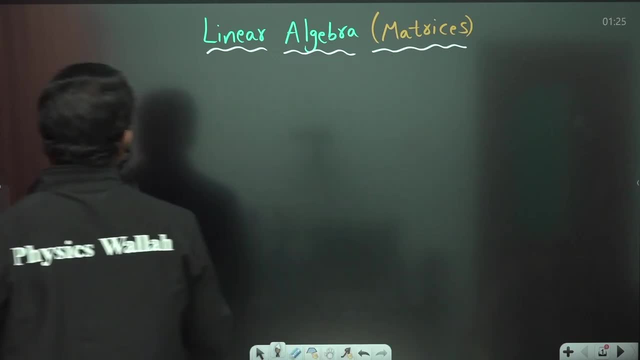 will be solving simultaneous equations, correct? Let us suppose if I give you this equation like: a11x plus b11y is equal to c1 and a21x plus b21y is equal to c2, for example. let us suppose, if I ask you to solve, 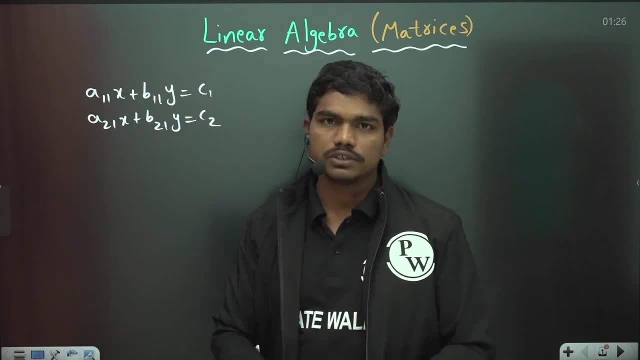 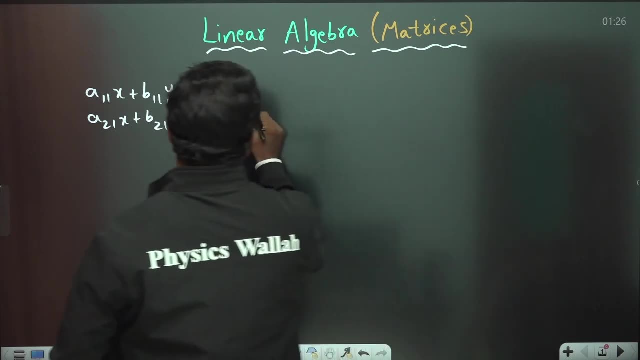 these two equations. It's very simple for you, right? you have a lot of techniques for you, like elimination, substitution. You have a lot of techniques. But let us suppose if I try to increase the complexity, For example, instead of giving this 2D system, let us suppose I have given you a system like this: a12x, or you can say y. 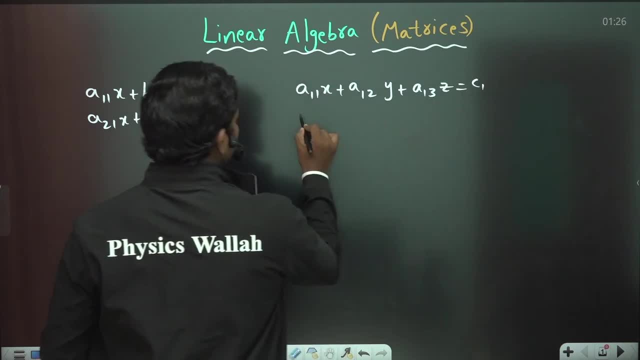 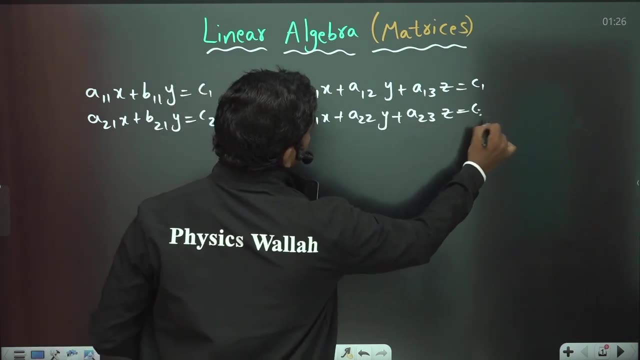 plus a13, z is equal to c1, a21, x plus a22, y plus a23, z is equal to c2, and a31, x plus a32, y plus a33, you can say z is equal to c3. so let us suppose, if i give you this particular system, 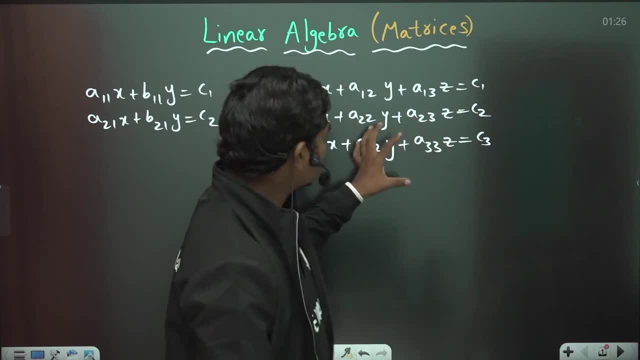 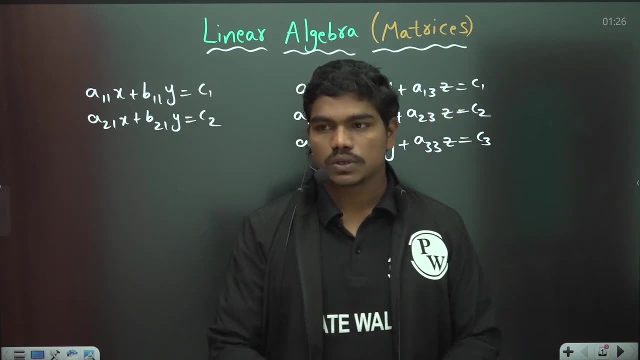 it's a three equations with three unknowns, then you know you can still solve this system using such kind of techniques. but it's not very simple, correct? now let us suppose if you get 4 by 4, then it's much difficult case. so basically, matrices is. the main application of this is you can solve. 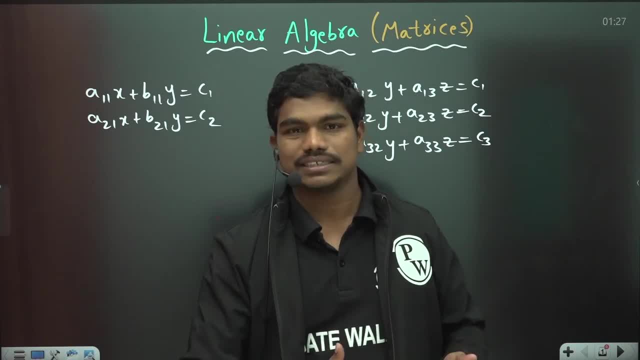 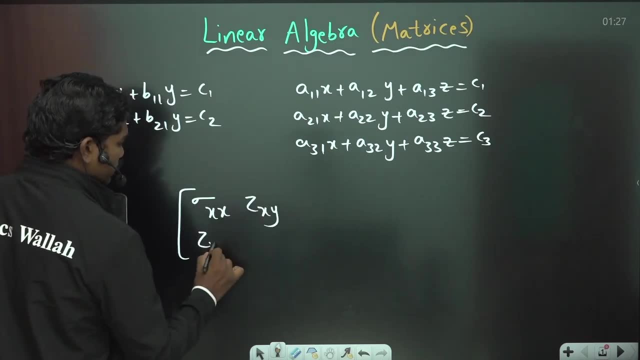 simultaneous systems and there are n number of applications in technical subjects, for example. many of you might have seen this matrix, like i was talking: tau x y, tau y x and sigma y y. this is basically a 2d stress tensor. if you see, in strength of details of fluid mechanics you get 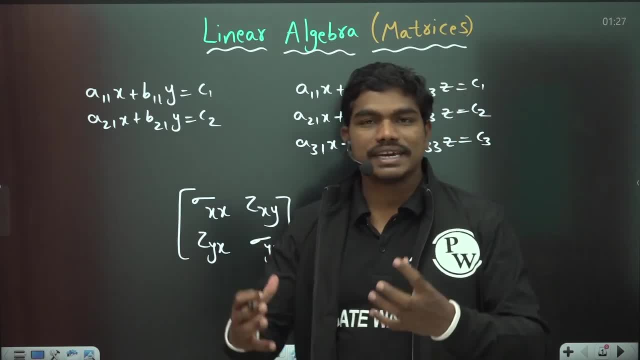 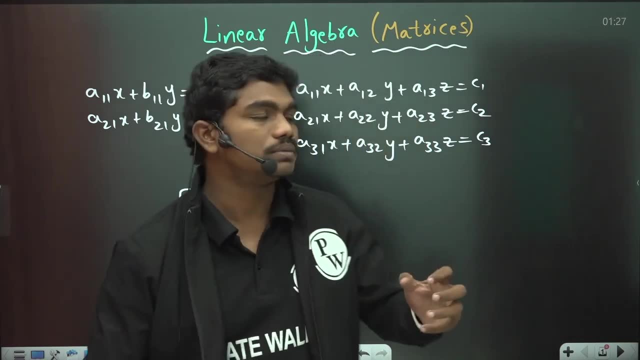 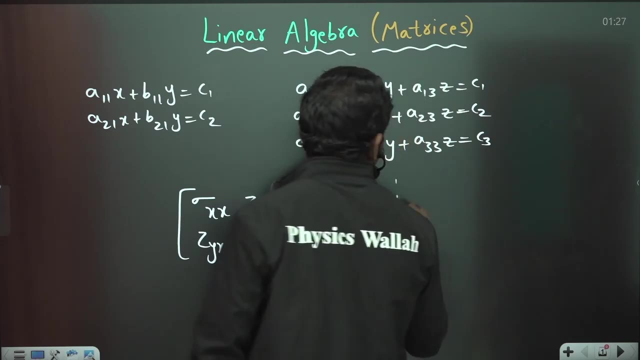 such systems. similarly, if you are dealing with finite element analysis, you will be getting stiffness matrices, all these things. okay, so it has large number of applications and linear algebra is definitely one very good subject to deal with all such things. in mathematics and myself, when i was doing some research earlier, i have dealt with a system of 101 unknowns and 101 equations also. 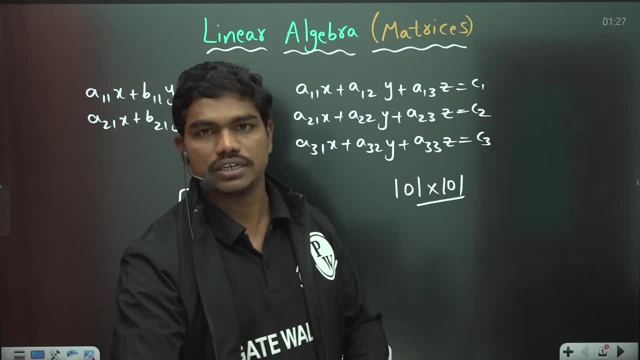 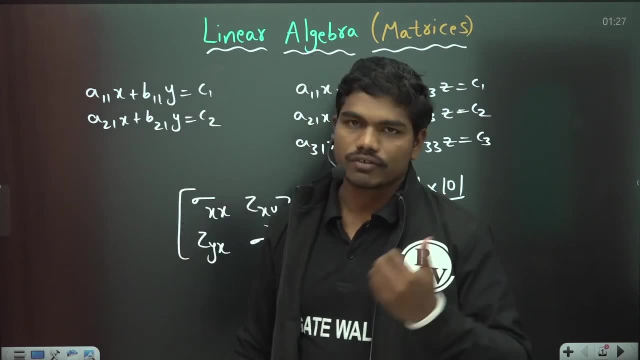 because, you see, generally many things change with respect to time, location, temperature, there are certain things. so i was able to solve 101 by 101 system, using matrices again and, of course, with the help of some coding. but right now my aim is to tell you that least linear algebra is one very 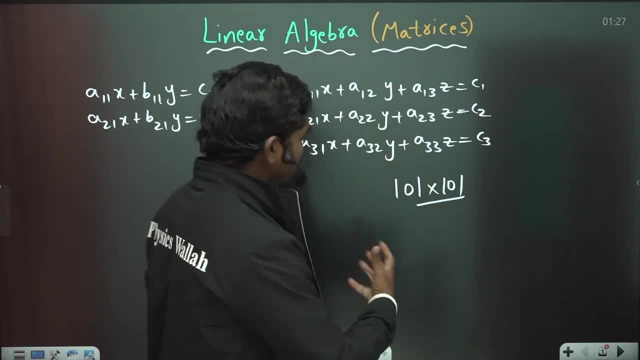 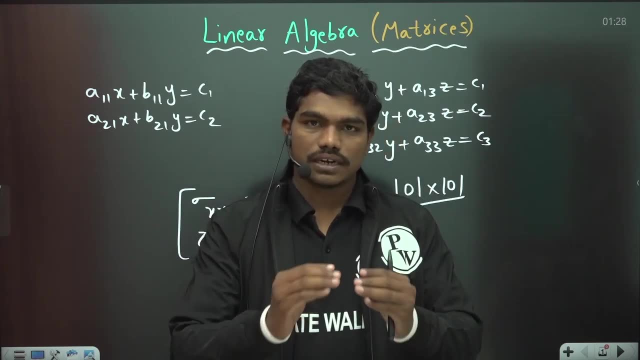 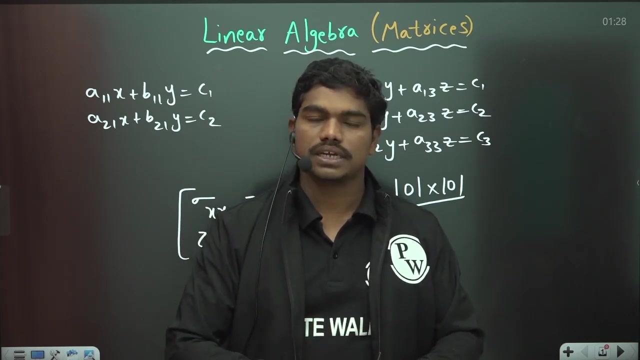 important tool to crack all the you know such simultaneous systems in engineering. okay, so let us straight away start from this basics, and this video will definitely help you out in understanding from the definition of a matrix, then slowly progressing to the advanced levels such that you can clear your all the exams, basically, and also a 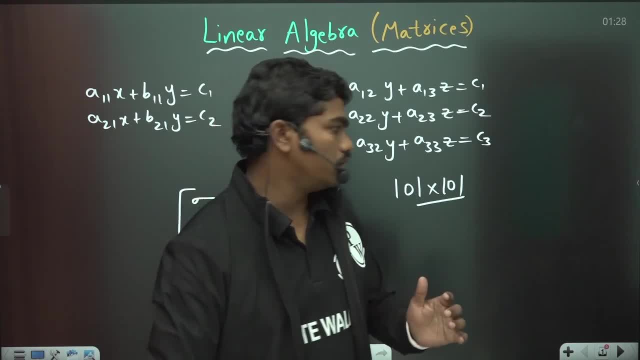 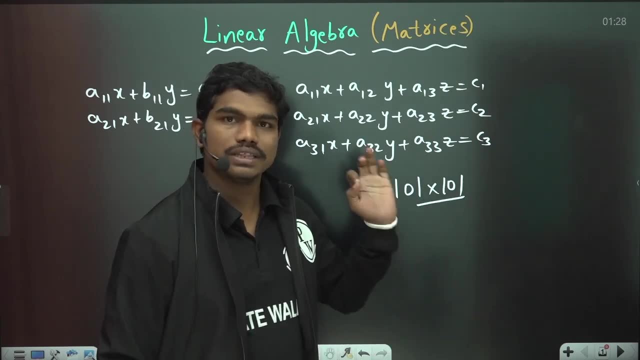 very good knowledge in matrices clear, so this video is helpful even for some je aspirants as well. if you try to go for the first two hours of this video, it's a single shot video on this complete linear algebra and i'm very privileged to give you this information in this video. so if you 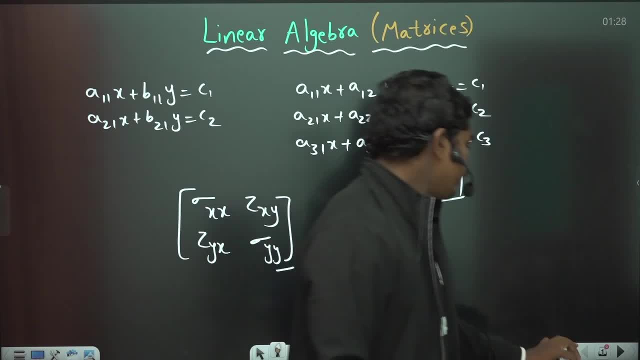 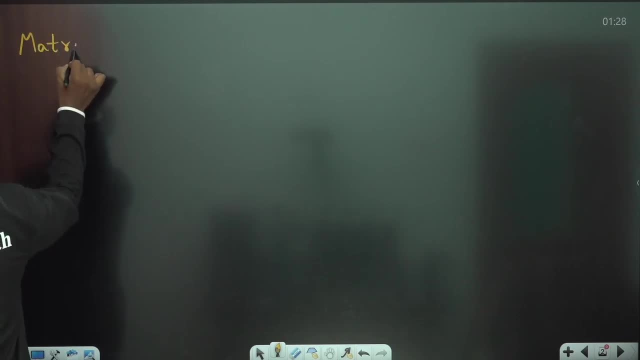 want to learn more about this topic, then please do subscribe to my channel and hit the bell icon. okay, so now let us straight away start with the definition of a matrix. so what is a matrix? what is a matrix, for example? for example, if you see, many of you feel that any rectangular area of elements 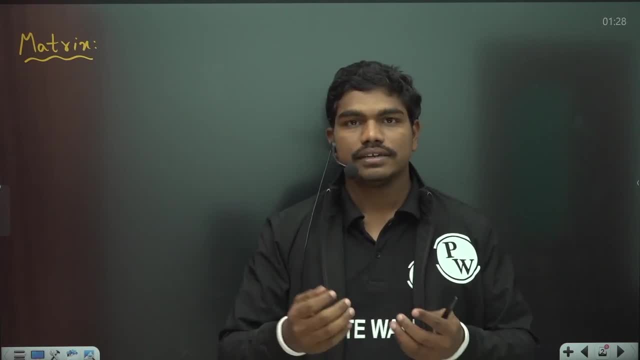 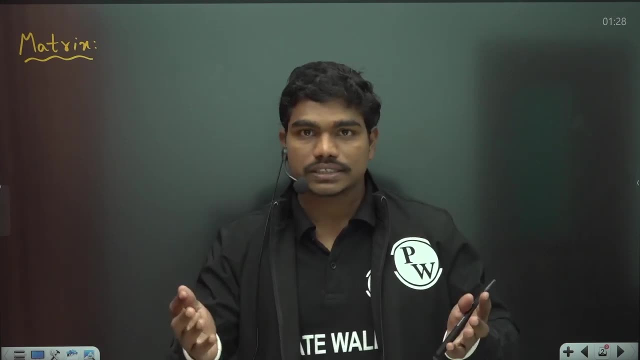 is called a matrix. correct you. in some books you find this definition: a rectangular arrangement of elements in rows and columns is called a matrix, but you have seen square matrices also. then square matrix is not a rectangular arrangement. it's basically a square arrangement of elements, and so 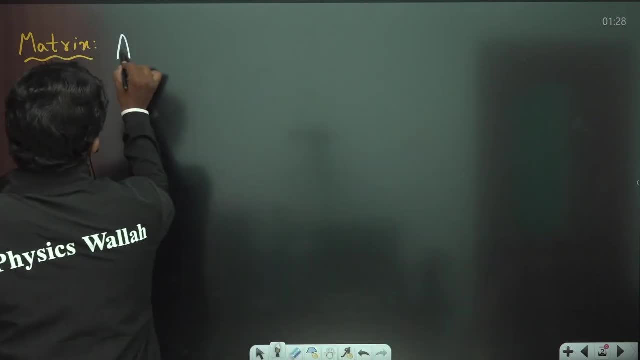 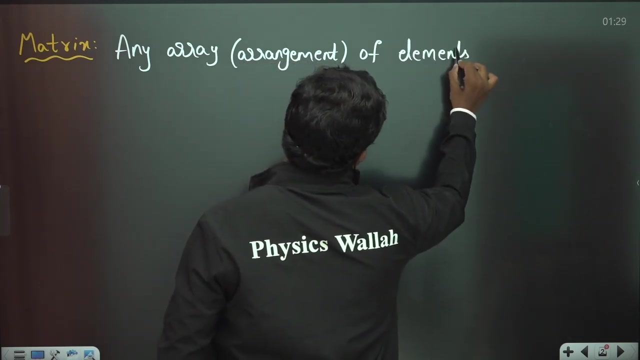 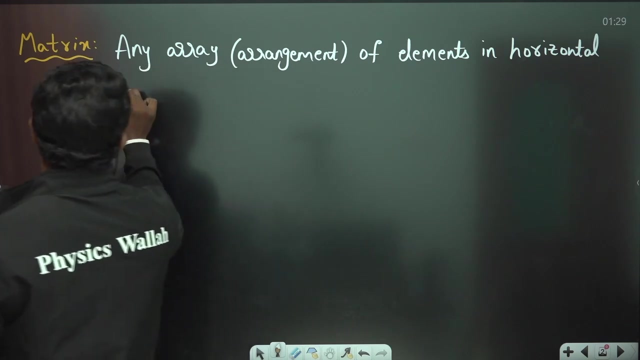 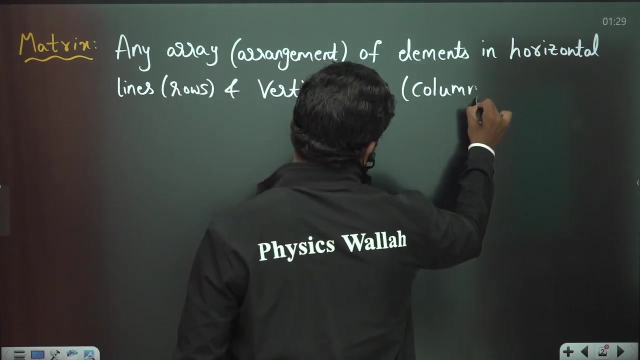 here. i generally define this as any arrangement. you can write any array or you can say arrangement of elements, of elements in horizontal lines, in horizontal lines, and you call this horizontal lines as rows and vertical lines, you call this vertical lines, basically as columns is called, is called a matrix. 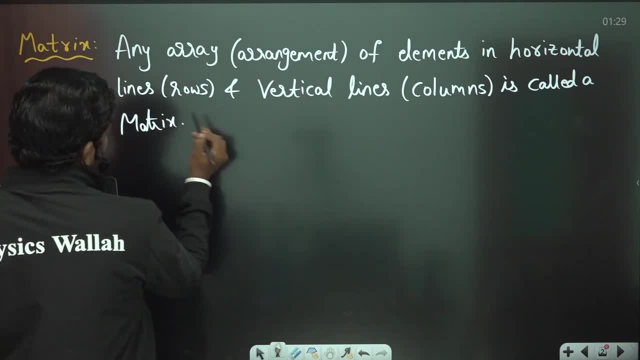 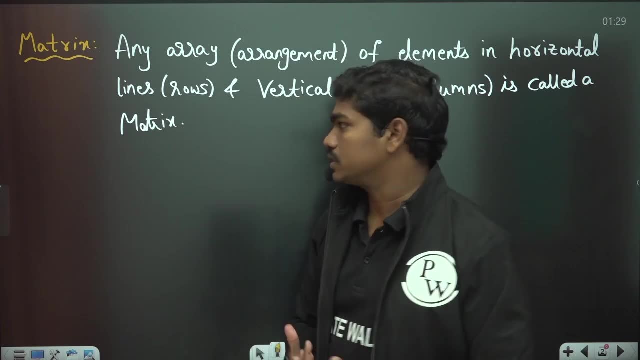 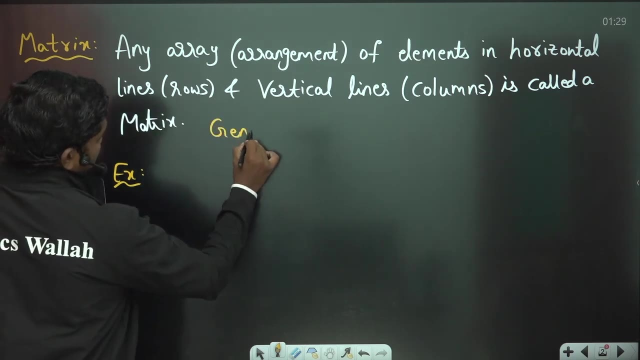 is called a matrix. now, for example, if i'll definitely give one examples for each of the cases, what to discuss so that it will, you know, make you better in understanding the things. so examples, if i take, for example, i can take normally these matrices are generally, you can write generally. matrices are defined by or denoted by, you can say generally. 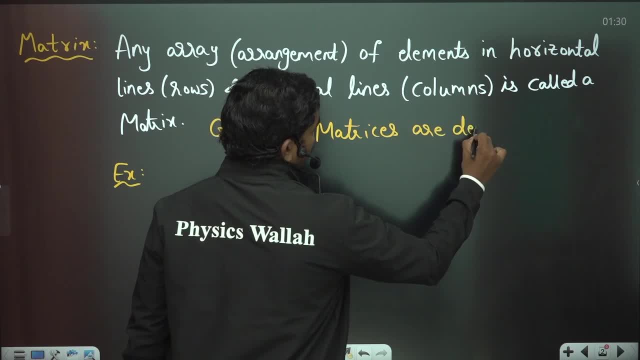 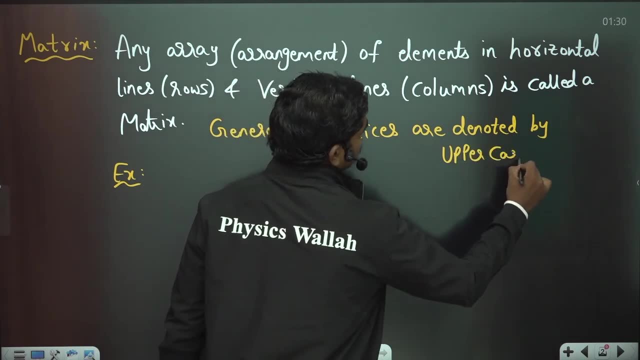 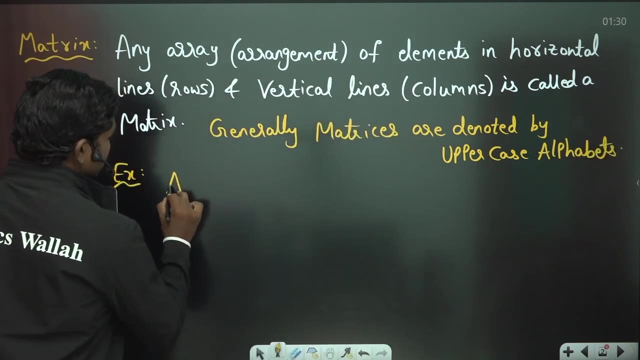 matrices are denoted by. are denoted by uppercase letters: okay, are denoted by. uppercase letters means basically capital letters. okay, so uppercase alphabets, you can say generally uppercase alphabets. okay. so, for example, if i say a is equal to, if i write these elements, india, you can write: 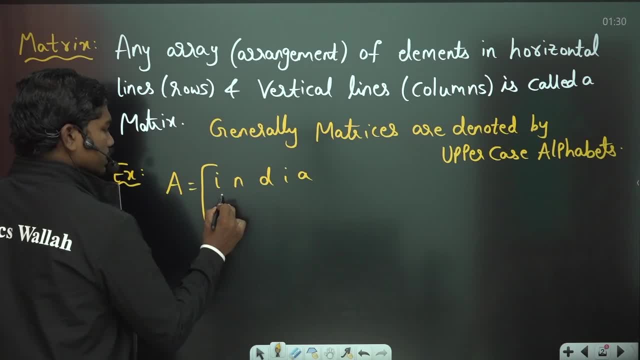 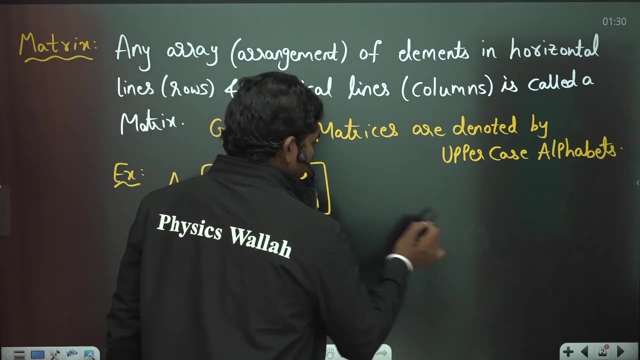 then what is the other five letter country? okay, you can say japan, for example. so if you see this, this matrix, then here all these elements, i n, d, i, a, again j a, p, a, and all these elements are arranged in some horizontal and also in vertical rows, so basically this row is called the first row. 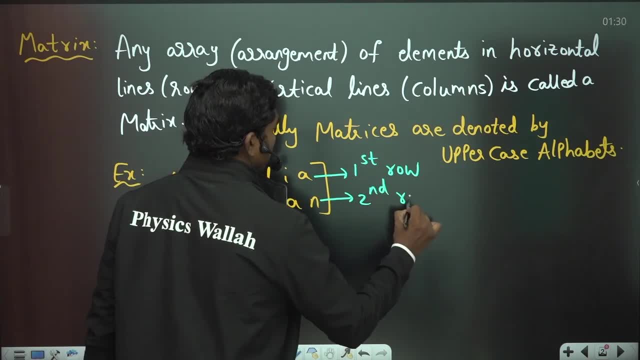 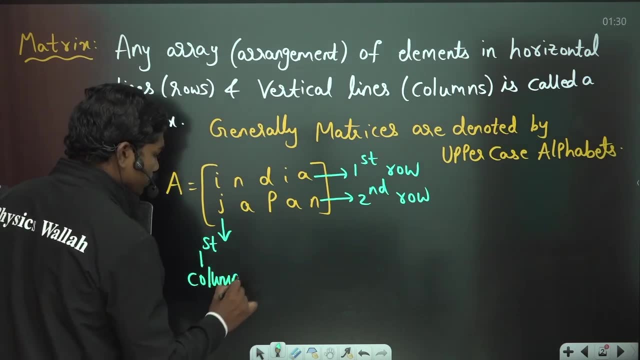 and this row is called the second row and similarly, if you see, this column is called the first column. similarly, this column is the second column. second column: this is the third, similarly followed by this fourth and finally, we have this fifth column. so this is your fifth column. 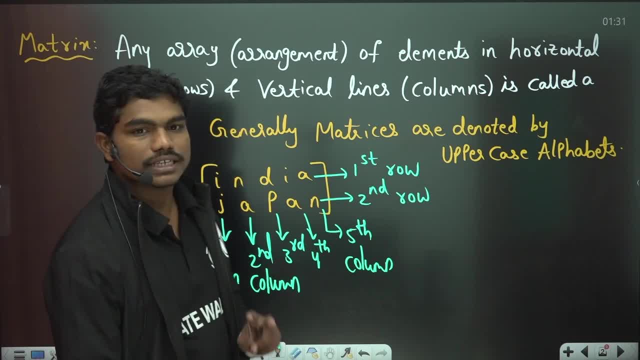 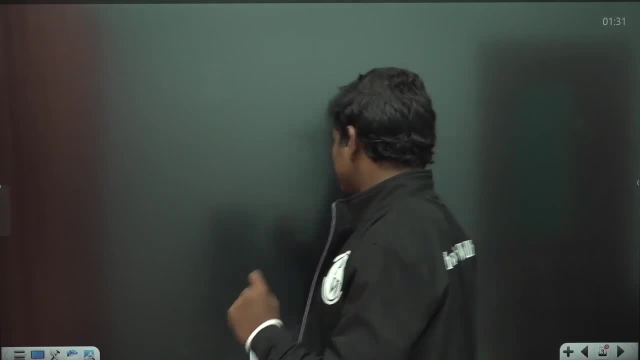 so if you see this example, this matrix, capital a has two rows and five columns in it. so what we say? there is something called size or order of the matrix. okay, so next we are going to for that definition: size or order of the matrix. okay, so next we are going to for that definition size. 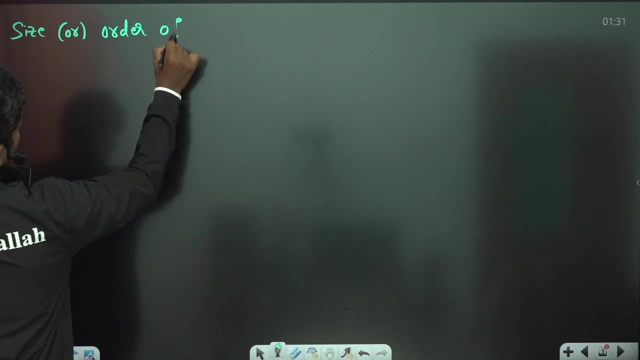 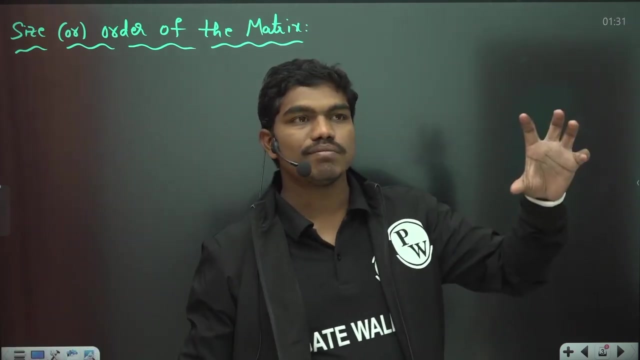 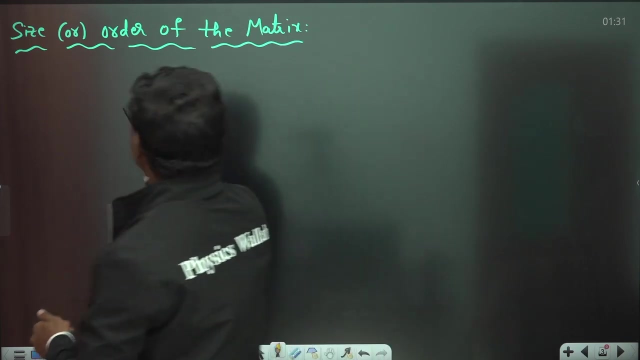 order of the matrix. size or order of the matrix. now, basically, if you want to see the size of a matrix, then the size is defined by number of horizontal rows you have and also number of vertical rows. i mean basically the vertical lines, basically the columns you have. okay, so if a matrix has 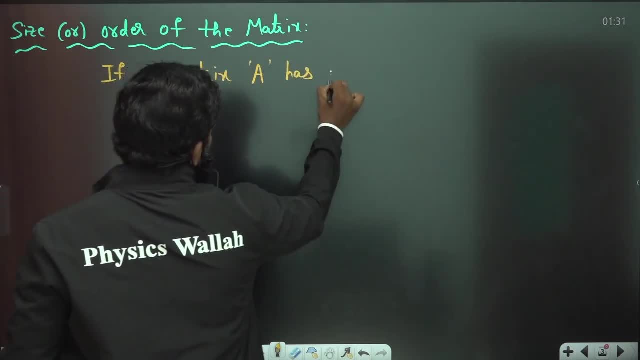 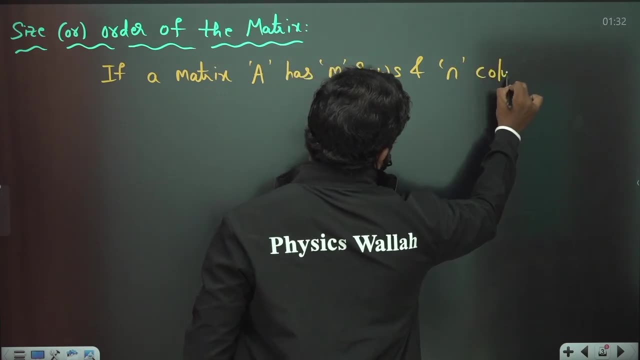 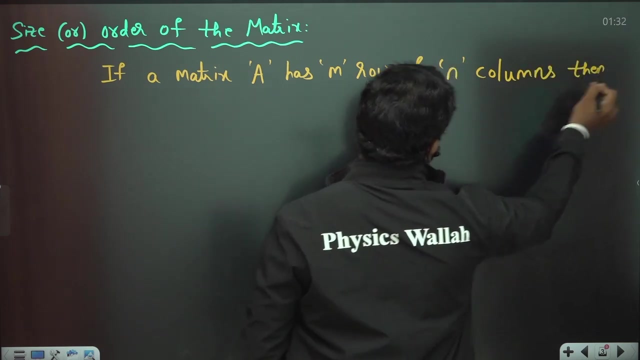 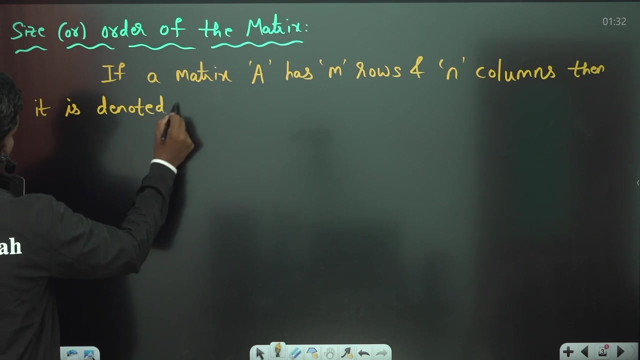 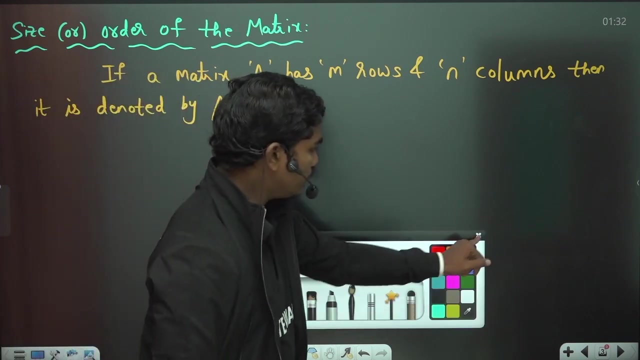 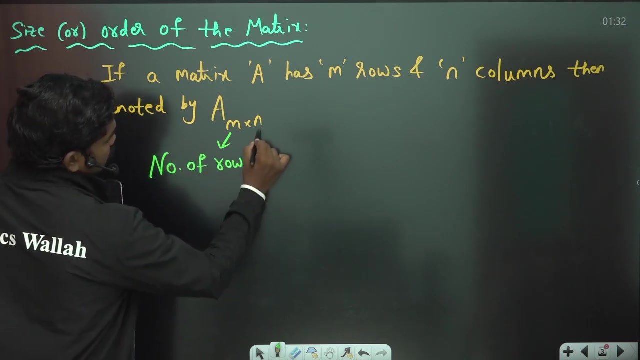 if a matrix capital a, has m rows and n columns, n columns, then it is denoted by. it is denoted by a m by n. so basically, this is as a m by n and, if you see, this m is basically number of rows that you have and this n is. 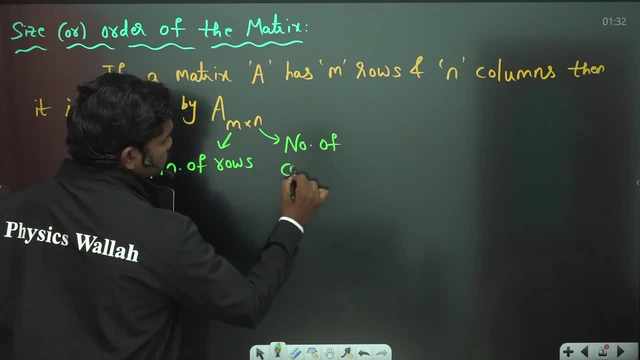 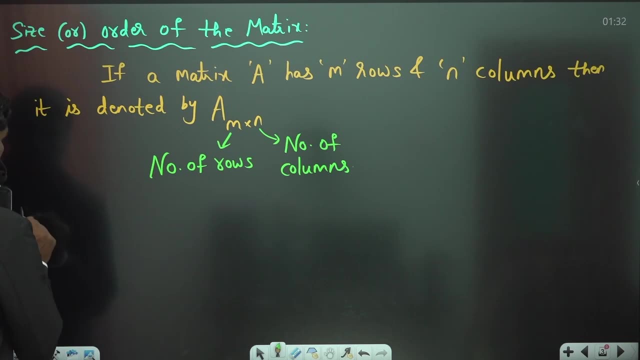 basically number of columns that you have here. okay, now how we define matrices. let us suppose i write a matrix, for example. okay, so general notation of matrix. for example, if i write this, matrix a is equal to 2, 3, 4, for example, 3, 4, 5 and 4, 5, 6, for example. let us suppose there is some. 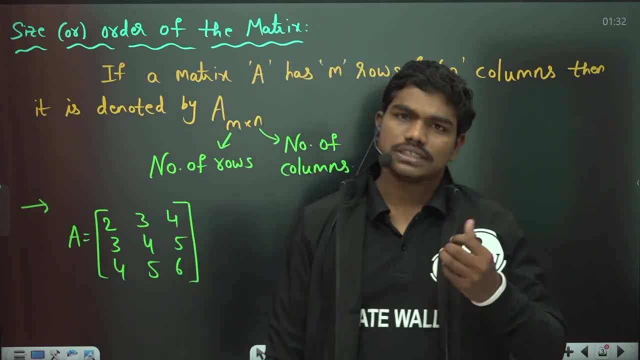 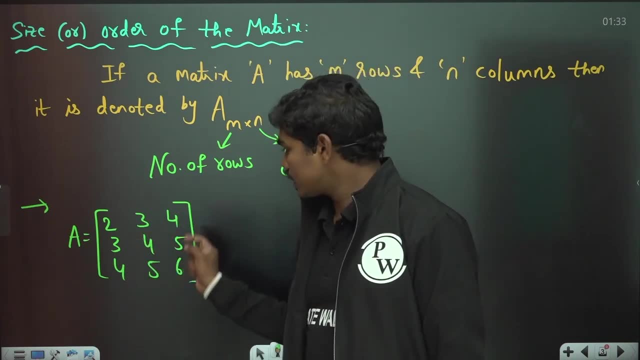 matrix like this now many times in gator examinations or in general, in some standard textbooks or advanced textbooks, you find the notation of this matrix in a different way, means they tell about the same matrix but in a different sense. how look? i'll tell you basically what they. 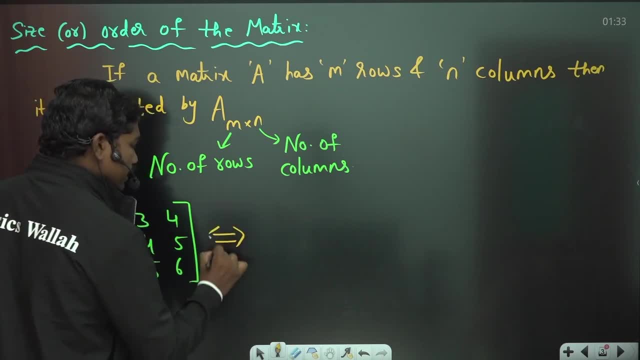 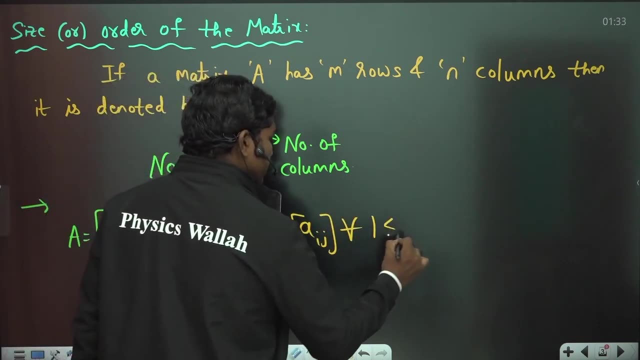 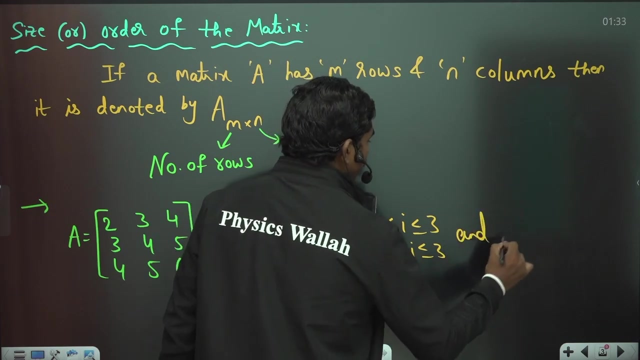 give you is, for example, if you take this matrix, this matrix is equivalent to a, is equal to a, ij for all, one less than or equal to i, less than or equal to three, one less than or equal to j, less than or equal to three, and a ij is equal to i plus j. so what? 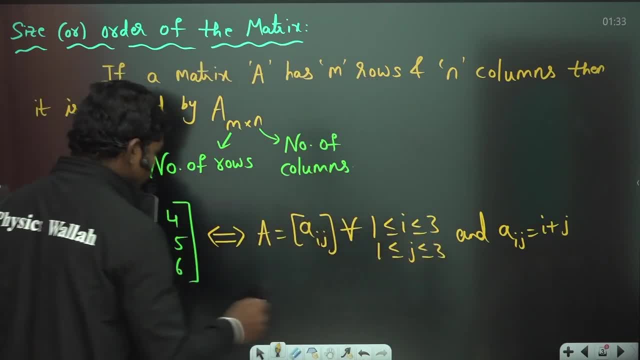 is the meaning of this sentence, how this matrix and this matrix both are same basically here. so if you see, normally if they denote a ij, this first subscript, so let us suppose they write a matrix, say: let us just write a strip, so let us obtain a Hm and 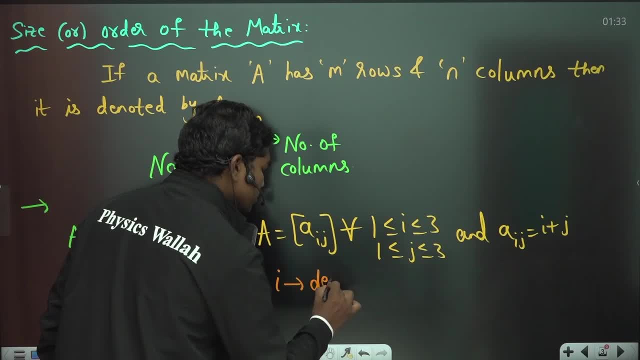 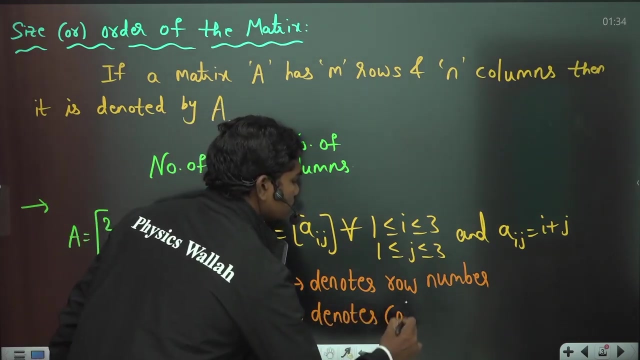 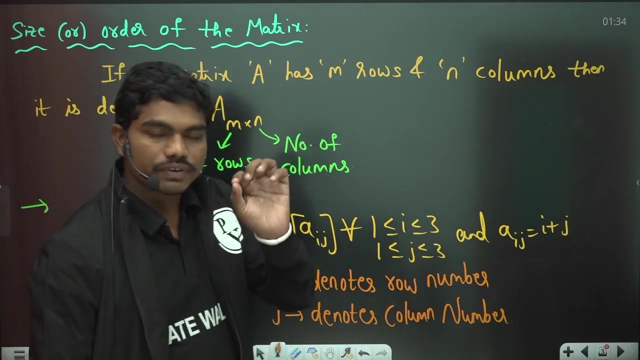 means basically, i denotes row number. okay, so this i denotes row number and j denotes this. j denotes column number. okay, so this j denotes column number. so once, if you want to specify location of any element in a matrix, let us suppose, if i want to specify this element, 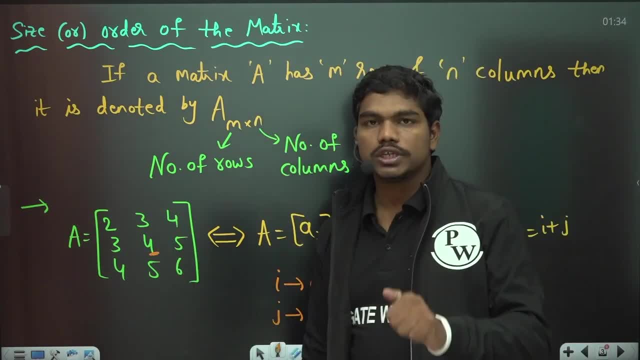 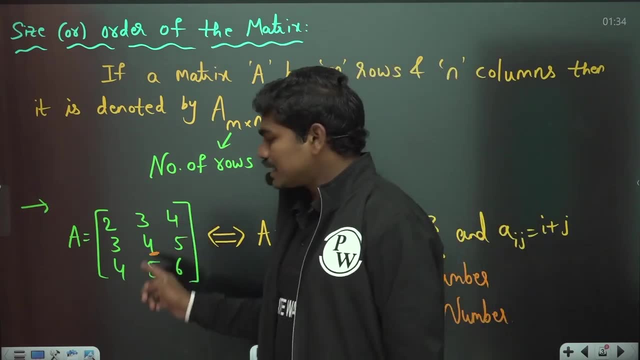 then you know this element is in the second row and it's also in the second column. so basically, if i denotes the row number and j denotes the column number, then i can say this element 4, which i have highlighted here, is nothing but a 2: 2, which means it belongs to the second row, second column. 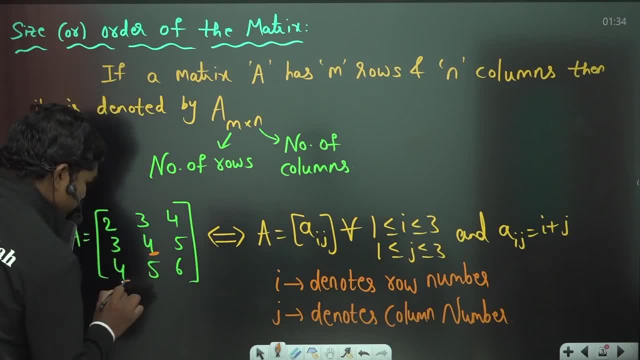 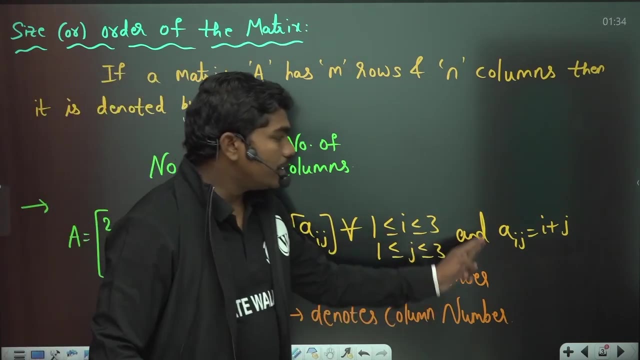 element: okay. so similarly, if i want to spot about this 4, for example here, then this 4 is in the third row and first column, so we call this as a 3, 1. okay, similarly any other. for example, if you take this 5, this is in the second or third column, so we take as a 2 3 and this element is given by. 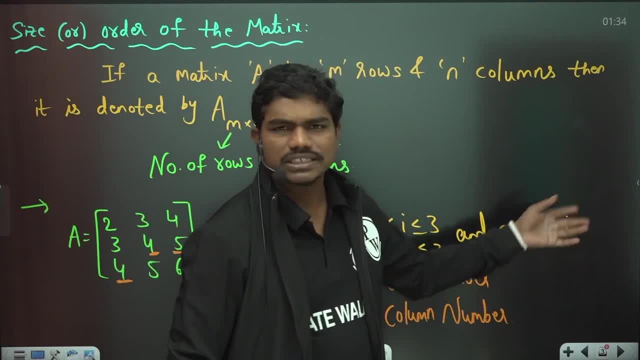 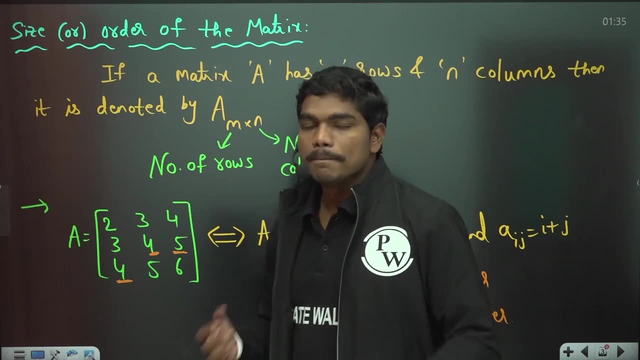 some function of i comma j in general. okay, it can be i plus j, i into j, whatever any algebraic expression they can put, sign i: whatever they want they can put. but if they want to generate a matrix, my intention is to tell you that they need not completely specify the matrix in this form. 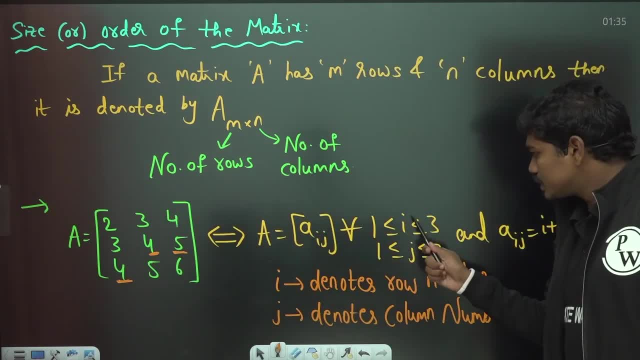 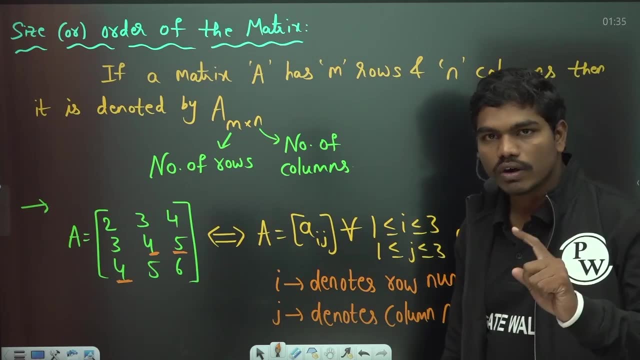 but rather they can specify you in this form. and here, if you see, i value is less than 1, i mean i is greater than 1 and less than 3. so basically, if you see, i can take the values of 1, 2 and 3, which means this matrix a, which you are talking about, has 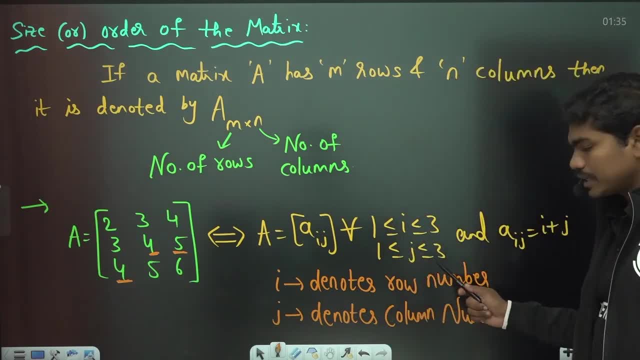 3, 0s and at the same time, 1 less than or equal to j, less than or equal to 3. that means this matrix can have 3 columns. so basically it's a 3 by 3 matrix. how do i know it's a 3 by 3? because row numbers. 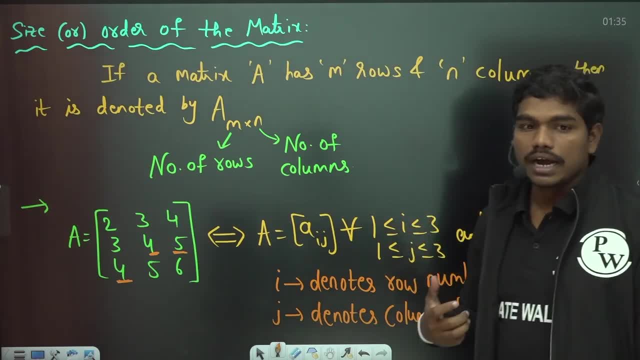 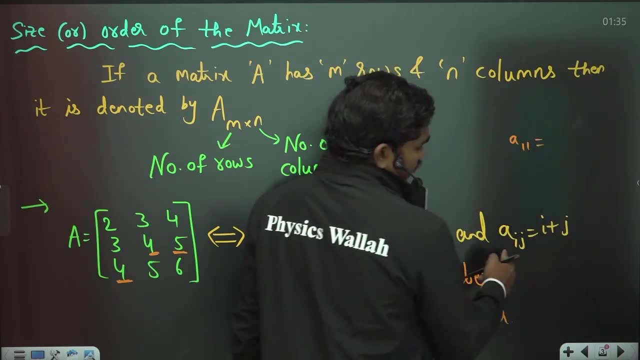 are from 1 to 3 and also column numbers are from 1 to 3, and how do i know what are the elements inside this matrix that is given by this? for example, if i want the element a 1, 1, then a, i, j. 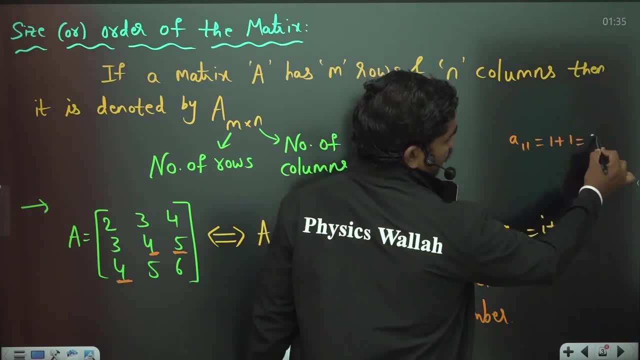 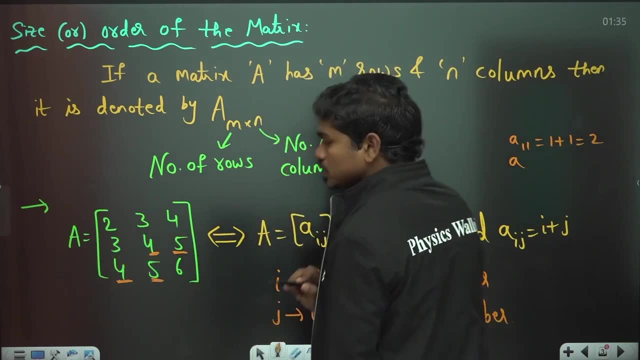 value is 1, j value is also 1, so this 1 plus 1 is equal to 2. similarly, if i want and if you see, the first element is 2 in the first row, for example, if you want this element, it's a third. 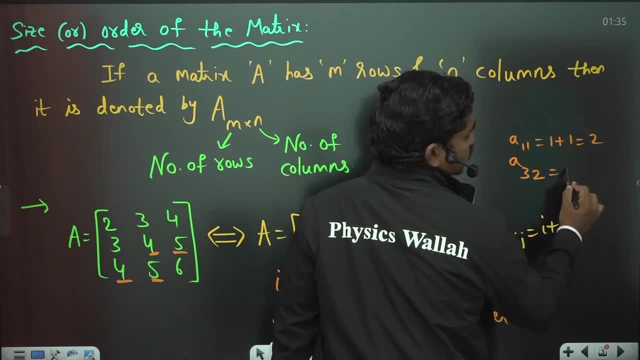 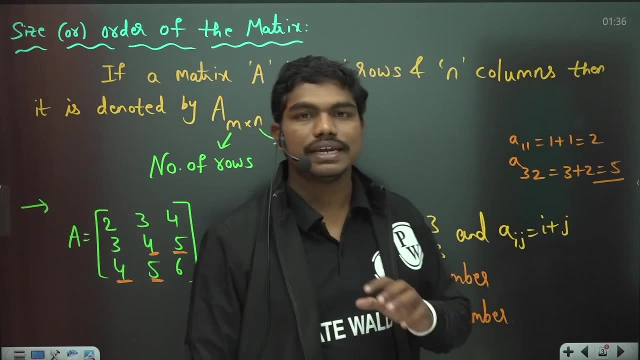 or second column element. so third or second column element. so this is 3 plus 2 and this value has to be 5. so if you see, this element is 5 actually here. so that's how you actually need not completely specify the matrix, okay. so this is one very important way which you know they ask you. 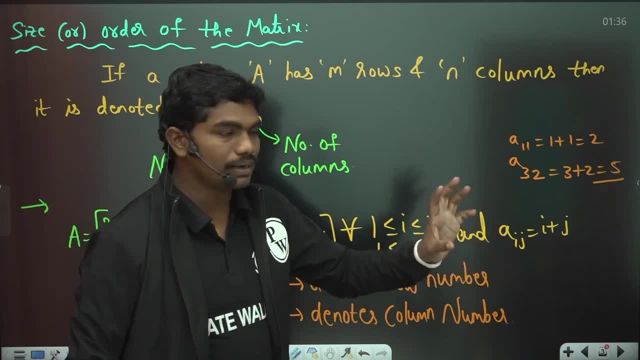 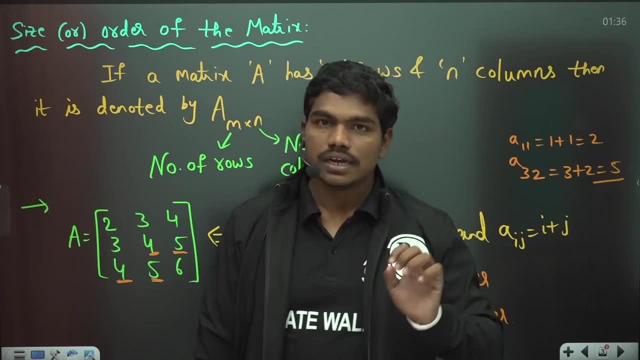 this size, with the help of this, inequalities, and they define the elements using some function in terms of i and j. so that's how this is one very important notation- of matrices clear and because i'm going to use this from no one words. so that's how i am, you know, going basically. now i would like 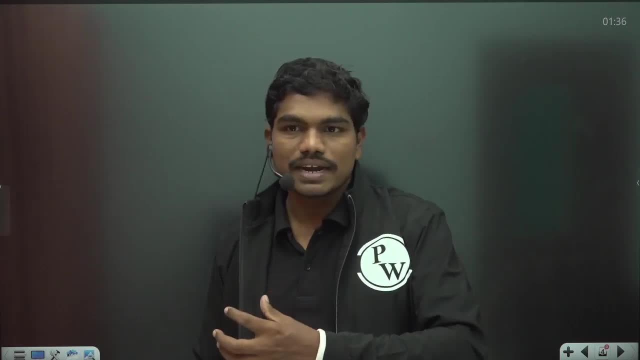 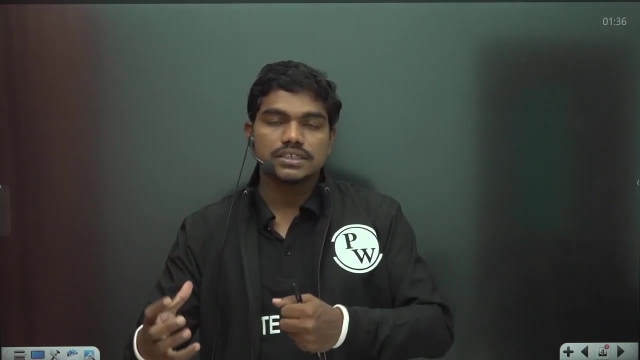 to give you some basic types of matrices, because these types of matrices means there are certain types of matrices like upper triangular, lower triangular, diagonal matrix, all these things. and these type of matrices they have certain special properties in determinates, in inverse, in eigenvalues, all these things. okay, so we will see slowly in this video how we progress. 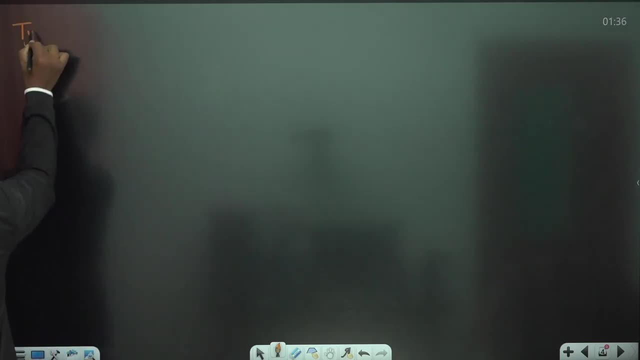 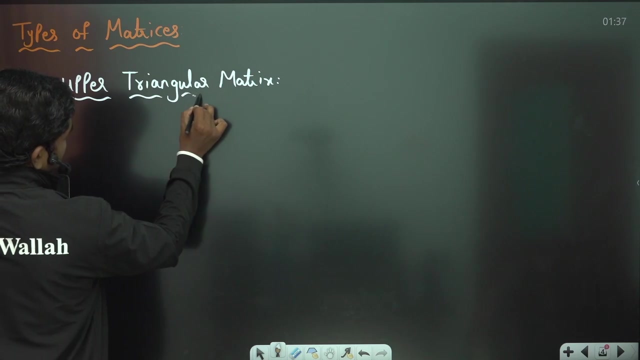 okay, so types of matrices. i'll quickly put a heading: types of matrices. types of matrices: now, the first type of matrix that i'm going to give you is upper triangular matrix. upper triangular matrix, upper triangular matrix. so what is this upper triangular matrix? so, basically, if you take 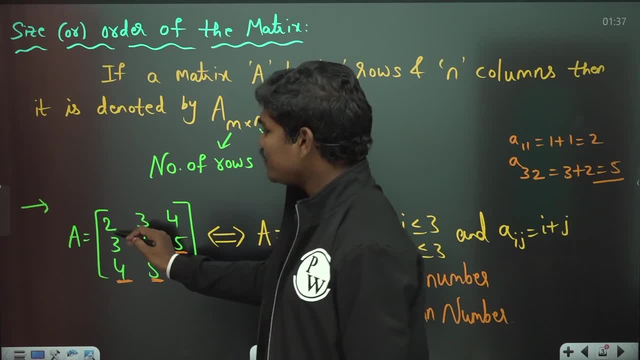 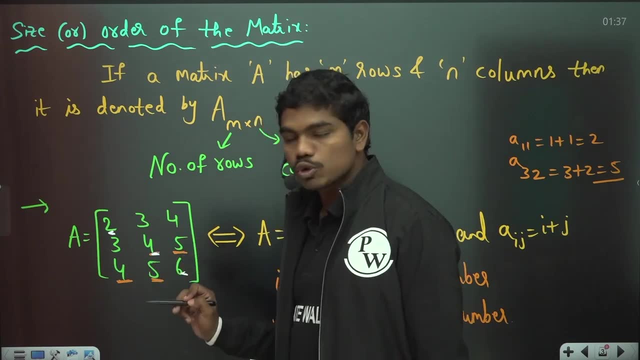 any square matrix, then these elements for which i value is equal to j, so 2, 4, 6, because if you take this first element, this is a 1, 1, then this element is a 2, 2, this element is a 3, 3. so basically, if you, 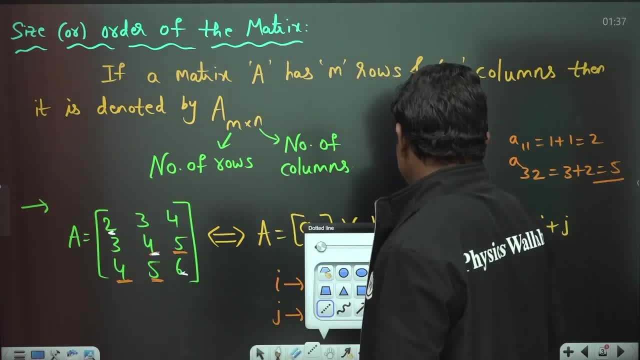 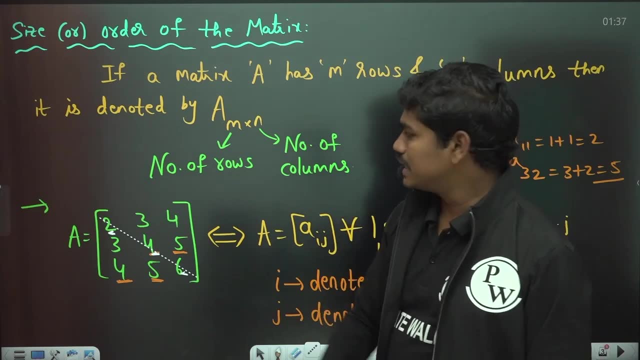 take this diagonal, for example. let me show using a dotted line. if you take this diagonal, then all these elements on this diagonal have same number of i comma j. so that's why we say, since it looks like a diagonal, we say those elements are called a principal diagonal element. okay, this is the main. 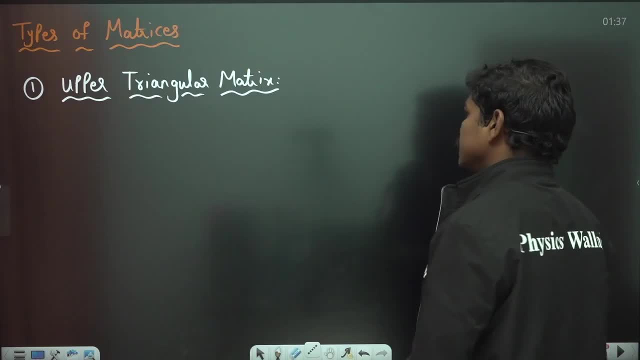 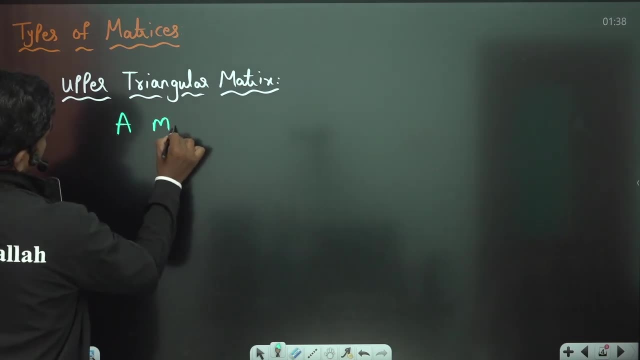 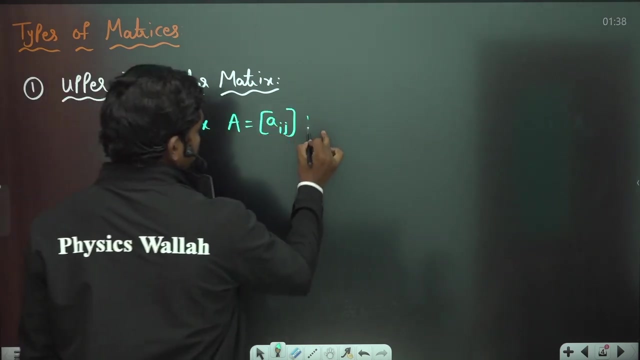 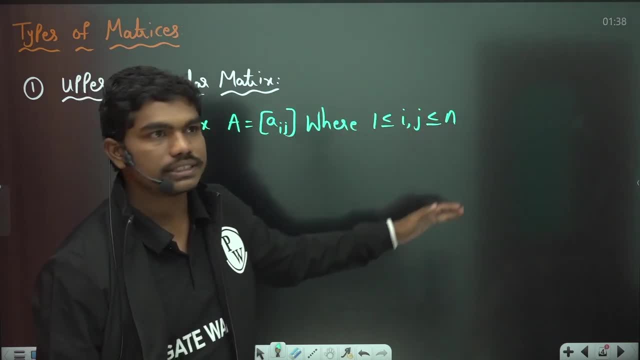 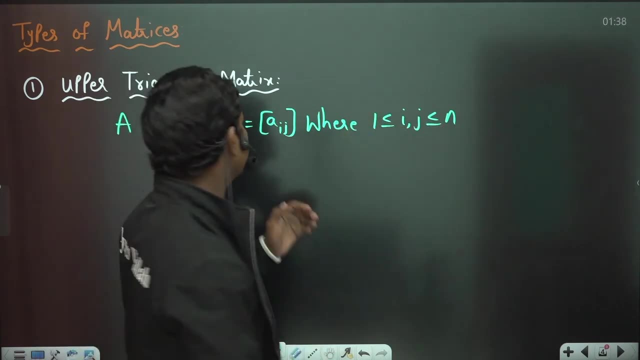 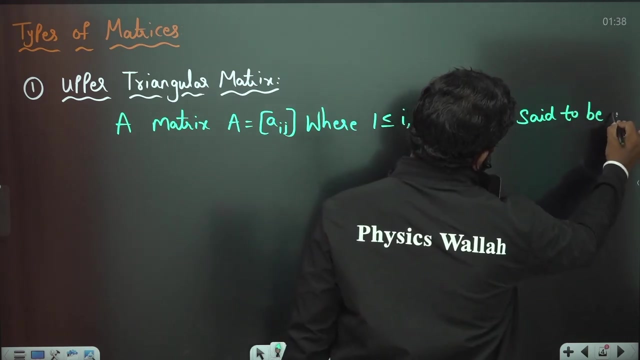 different inequalities, like one less than or equal to i, less than or equal to three, then one less than or equal to j, less than or equal to three. but it need not be like that. once it's a square matrix, you can directly denote it. okay, so this matrix is said to be- is said to be- an upper. 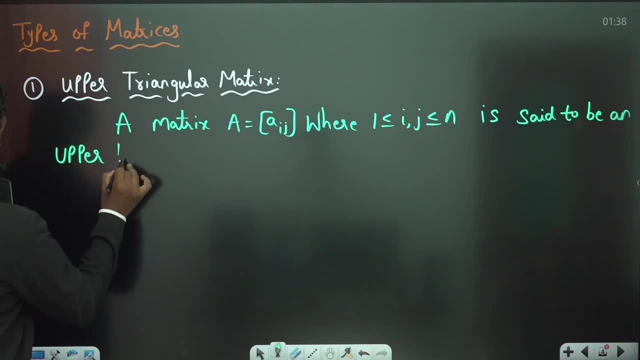 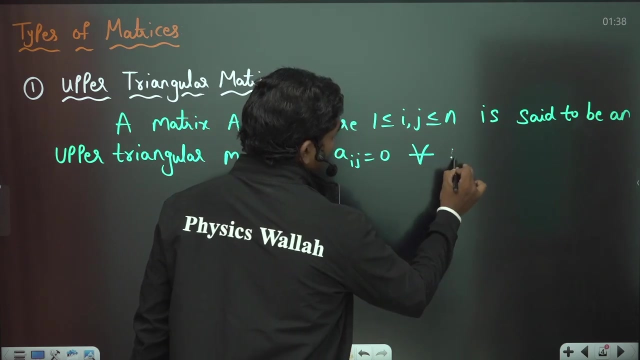 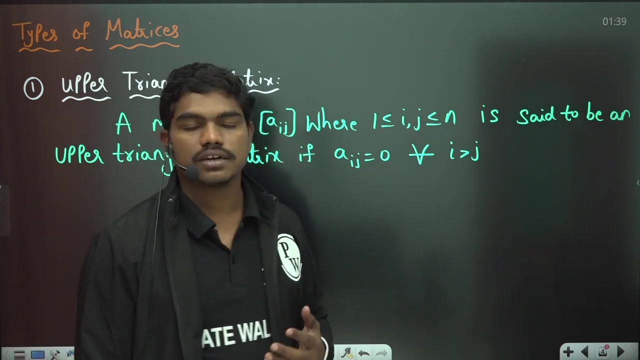 triangular matrix is said to be an upper triangular matrix is said to be an upper triangular matrix if a, i, j is equal to zero for all i greater than j. so what is the meaning of this equation? okay, i have written. this element will become zero whenever i is greater than equal. 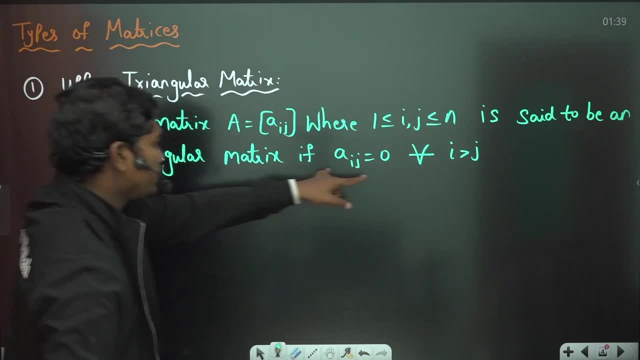 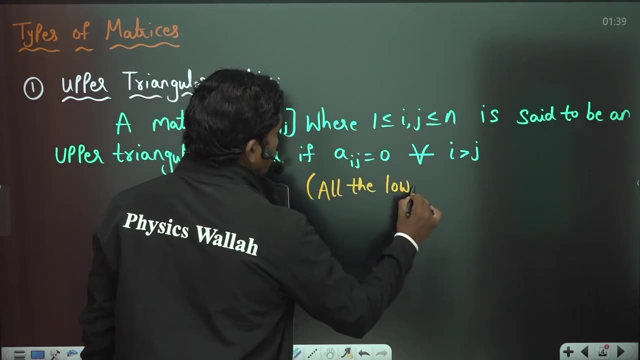 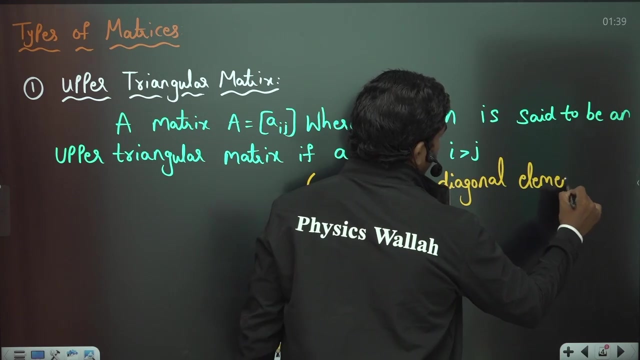 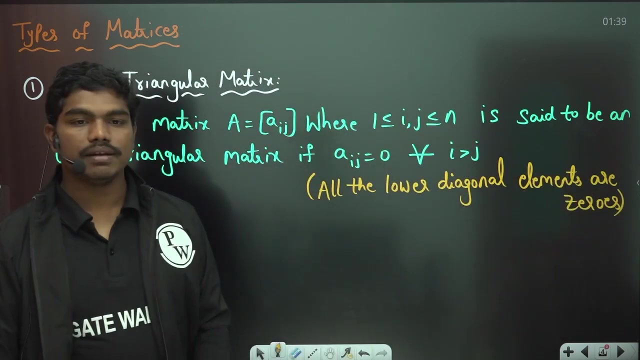 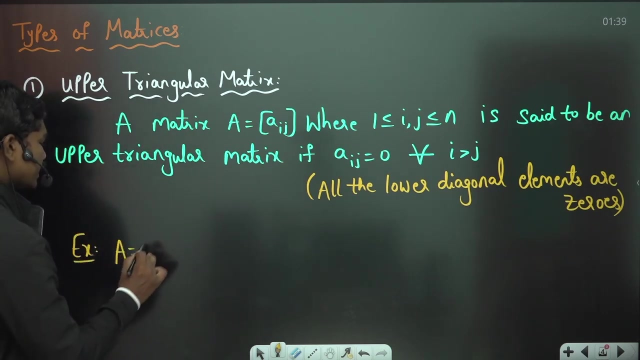 is greater than j. basically here. now, what does this equation tells you? this tells you you that all the lower diagonal elements, all the lower diagonal elements, are zeros. all the lower diagonal elements are zeros. now, how do you know this? look, for example: let us suppose if i take this matrix, let us suppose if i take this matrix a three by three. 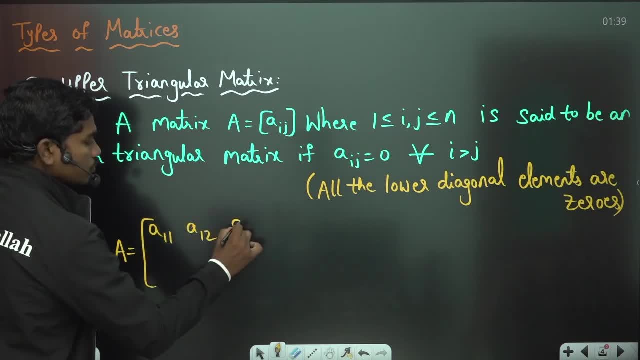 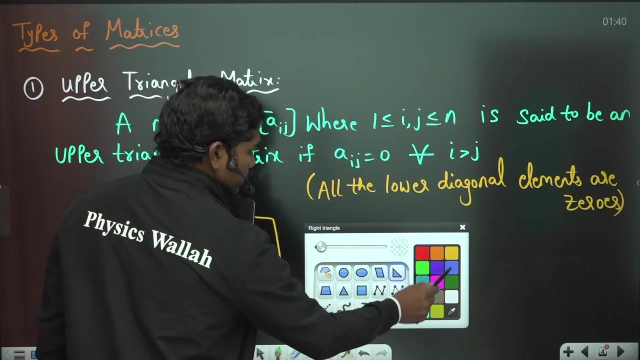 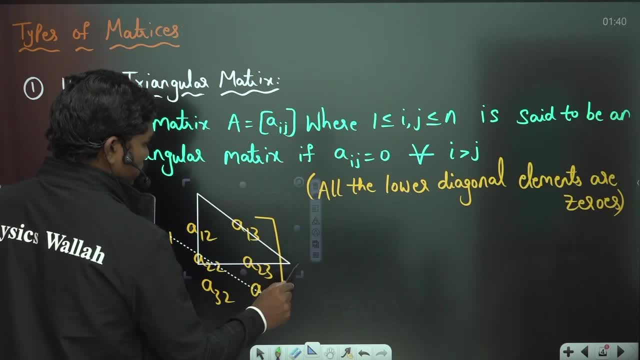 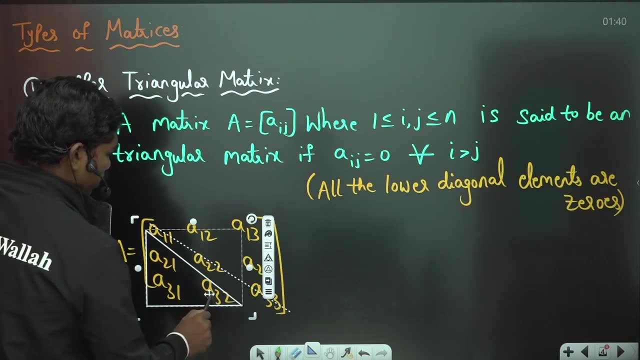 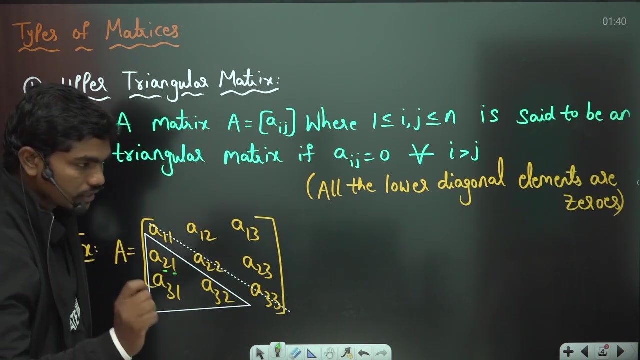 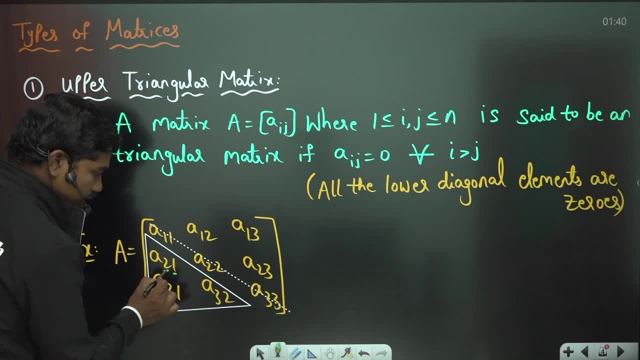 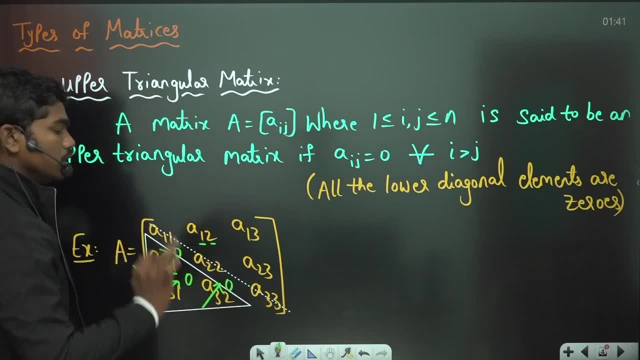 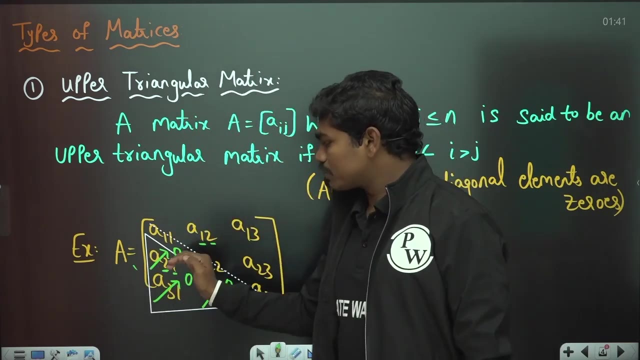 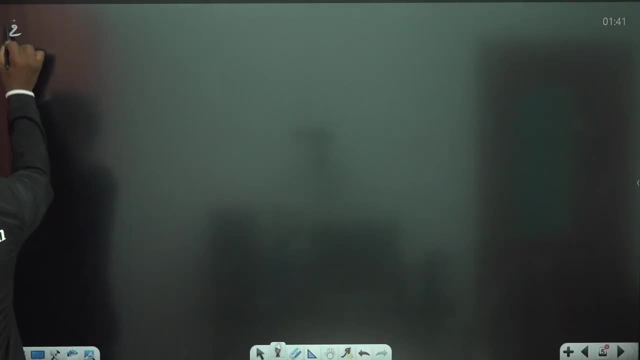 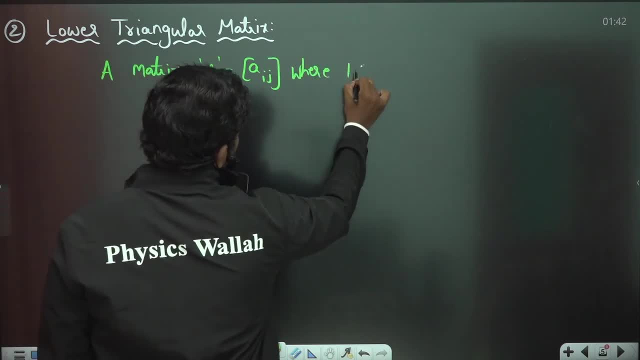 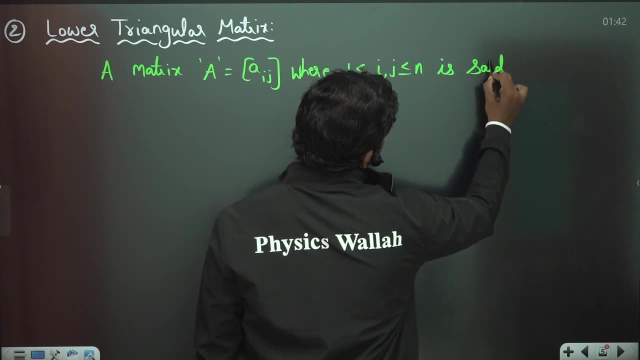 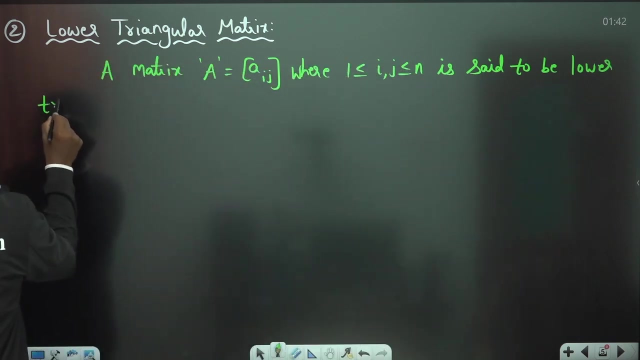 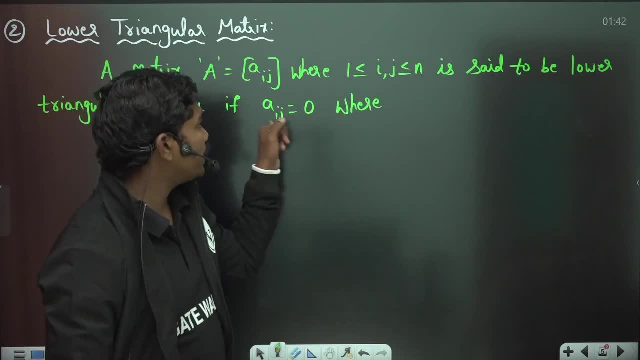 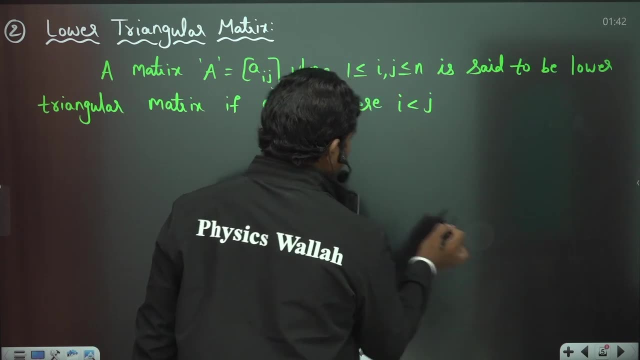 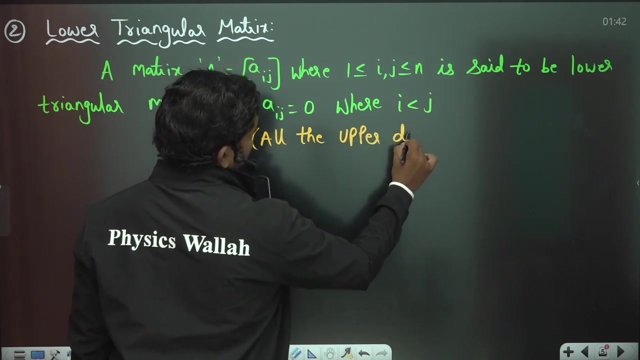 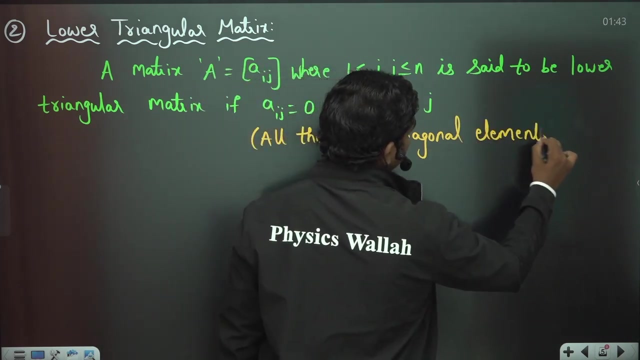 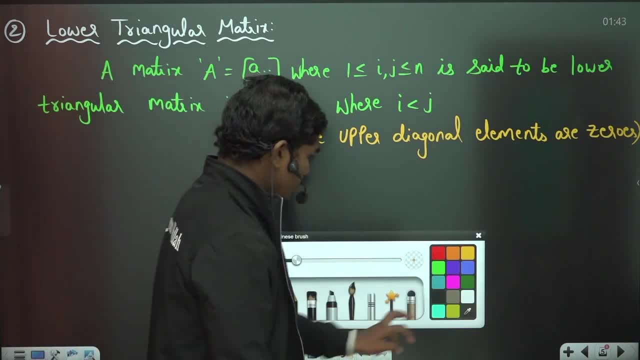 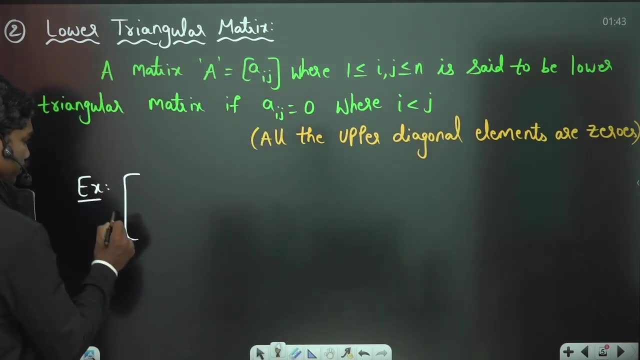 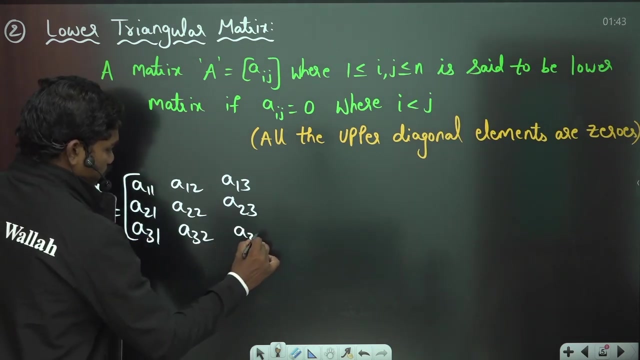 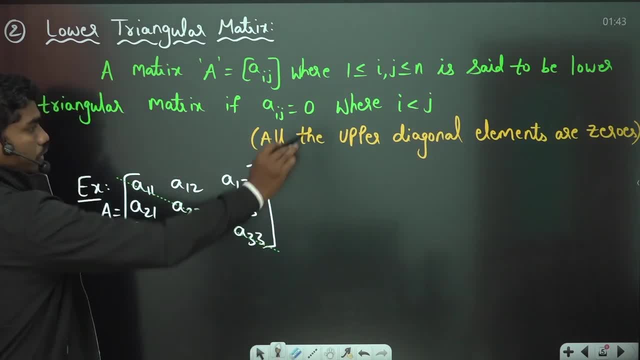 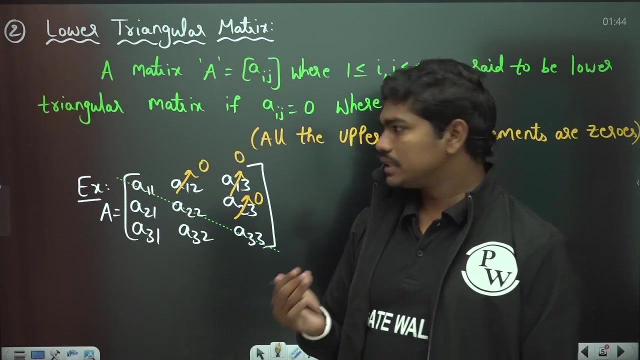 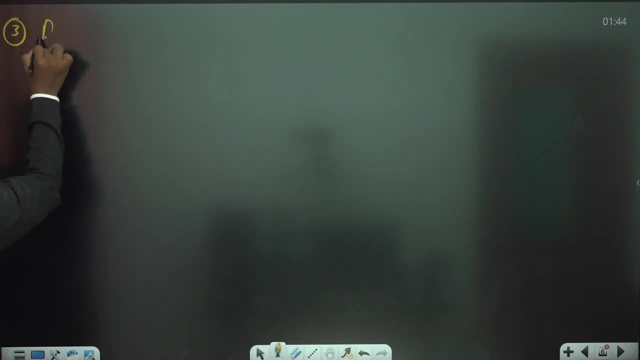 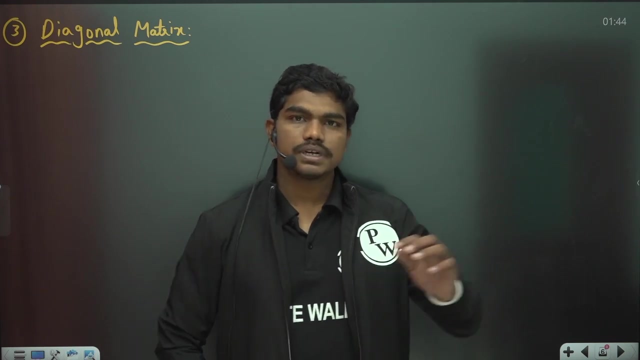 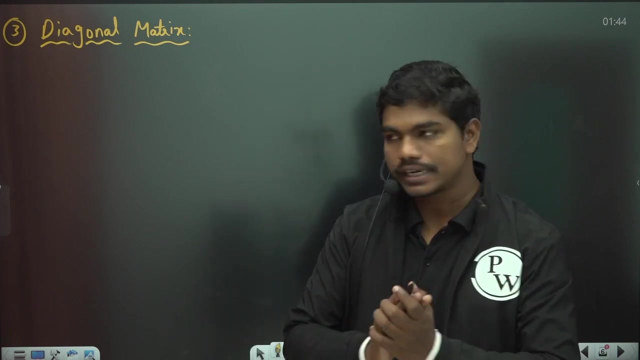 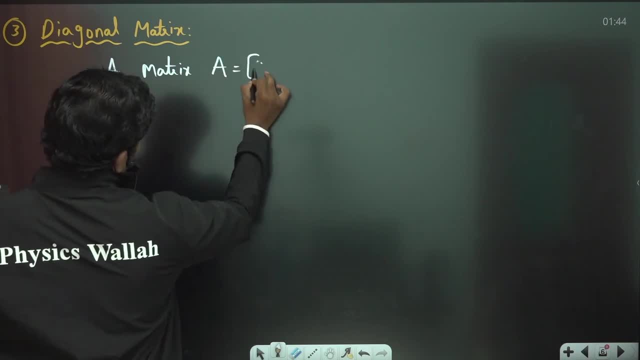 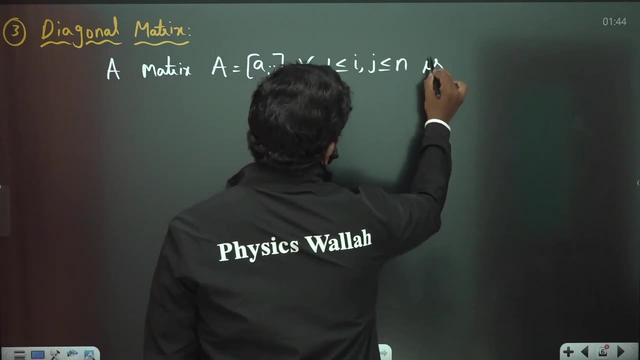 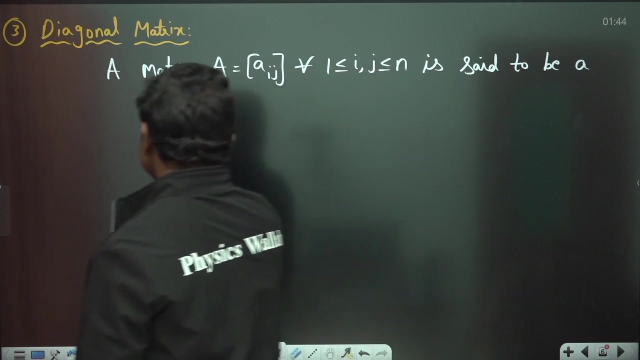 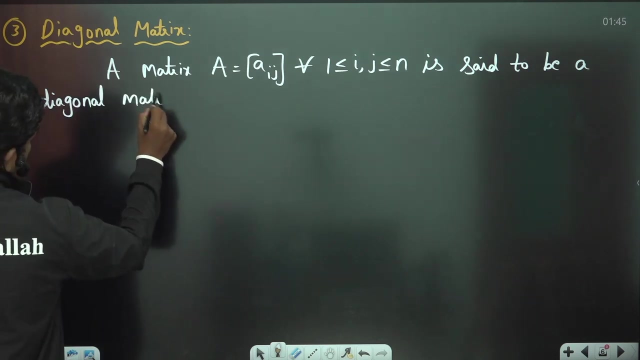 matrix A is equal to Aij for all, 1 less than or equal to i, j less than or equal to n, is said to be. is said to be a diagonal matrix, is said to be a diagonal matrix, is said to be a diagonal matrix. if, now you know one thing: if the elements are above the principal diagonal, 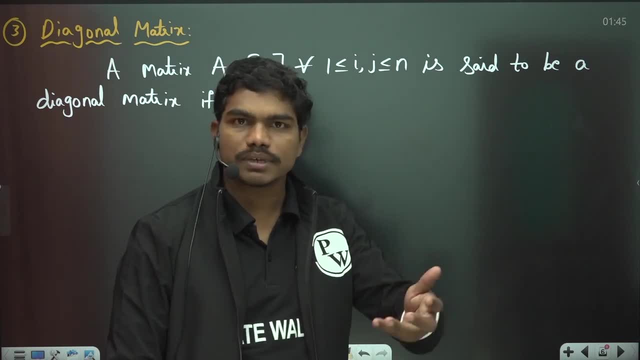 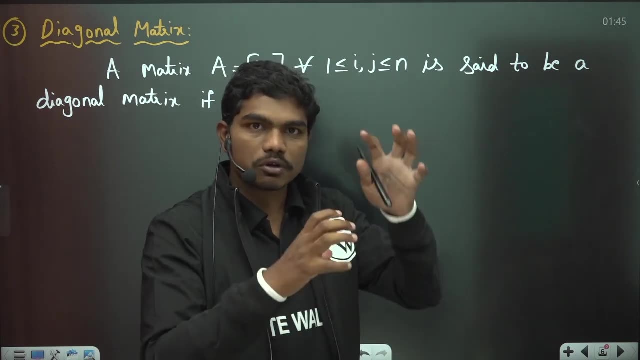 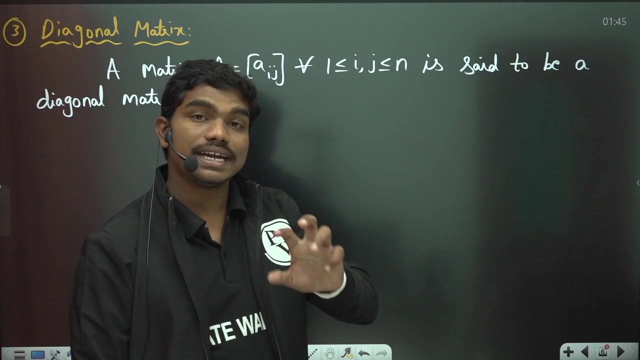 they must be definitely zeros. if the elements are below the principal diagonal also they must be definitely zeros. so which means, except the principal means, of course, even principal diagonal elements can be zero, but you are very much sure about the upper diagonal and lower diagonal elements being zero. so if the elements are lying either on upper diagonal or lower diagonal, then 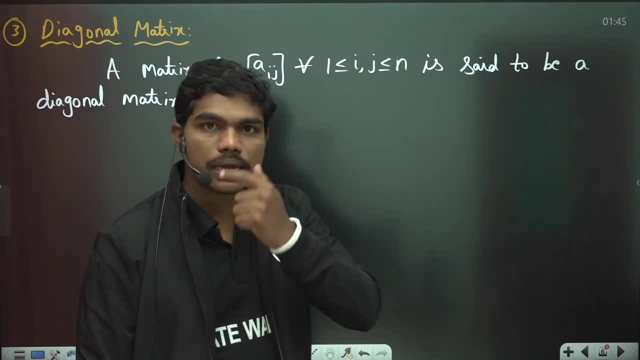 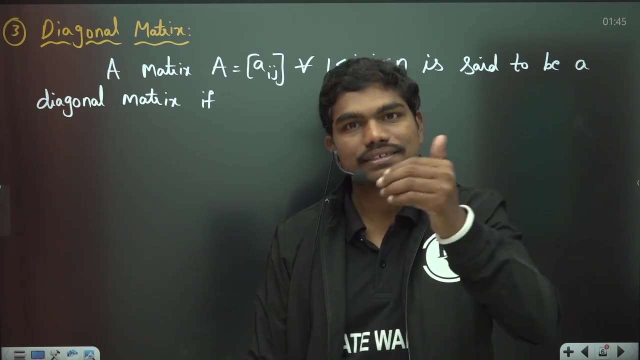 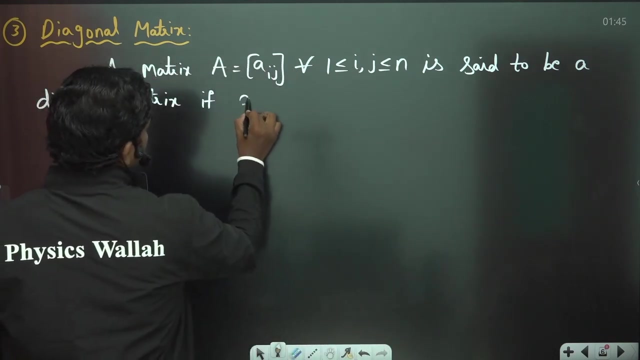 definitely. you know one thing: i is not equal to j, correct? because in case of upper, upper diagonal elements, if you see, i is less than j. in case of lower diagonal elements, i is greater than j, which means in both the cases i is actually not equal to j, correct? so is said to be a diagonal matrix, if Aij. 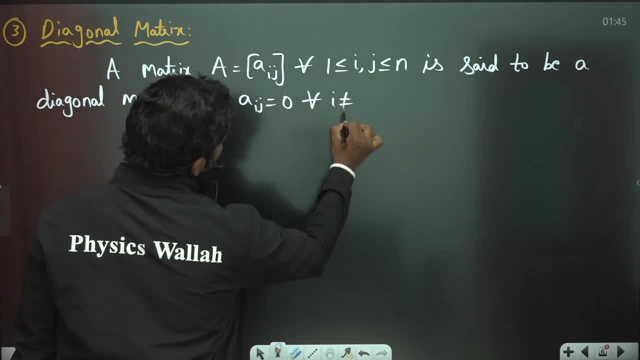 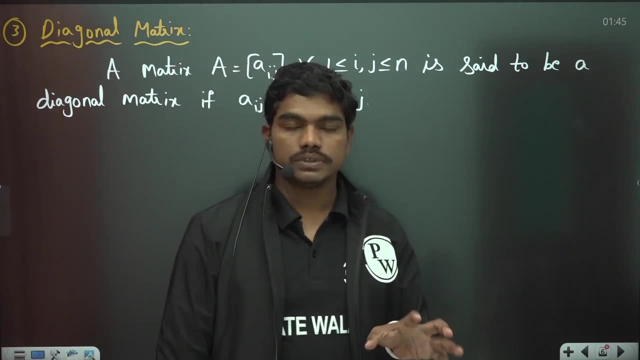 is equal to zero for all i, not equal to j. so this is one very, very important matrix. why i will tell? because there comes one very important concept in matrices which is called diagonalization, which we will see at the end, hopefully. so, if you see, this is the matrix. 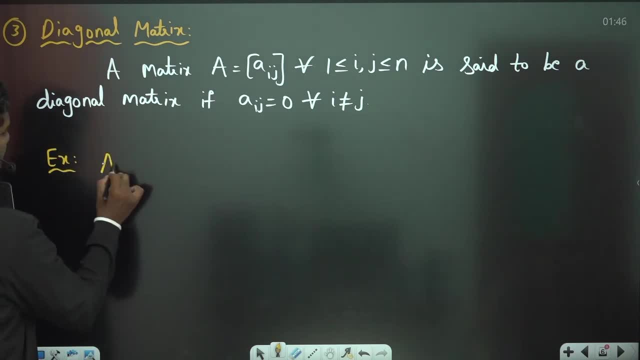 so example: Aij is less than j. in case of lower diagonal elements, i is greater than j, which means in both the cases i is actually not equal to j. correct, so is said to be a diagonal matrix if case of aij is with j, which means in both the cases of Aij is equal to j. correct, so is. 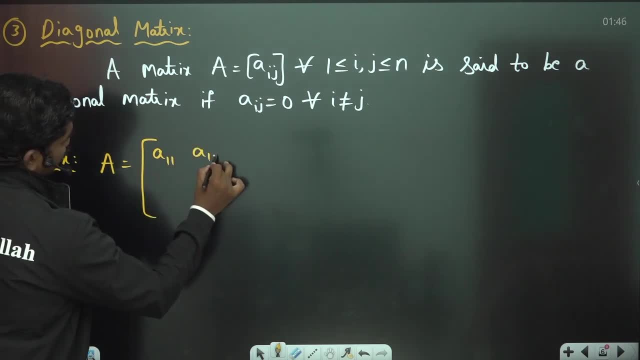 said to be a diagonal matrix, if i take this matrix example. so let us suppose so. if this is the case, then you can understand one thing: this is the principal diagonal here again. so this is the principal diagonal. so now if you check whenever the elements are not on the principal diagonal, then you can answer it correctly and this would be equal. 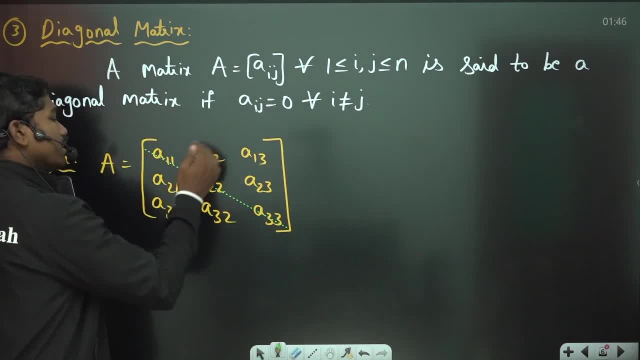 back now, because if the elements are not on the principal diagonal then you could probably find all those elements at a couple of times from one single mat experimental matrix, because those elements should be zeros. and if elements lie away from the principal diagonal means if they are not on the principal diagonal, then this i and j will not be equal to any of these elements. 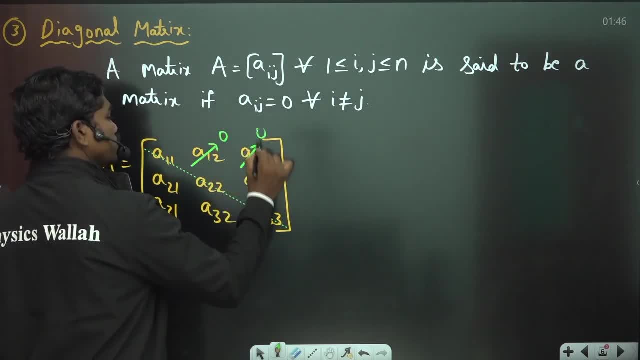 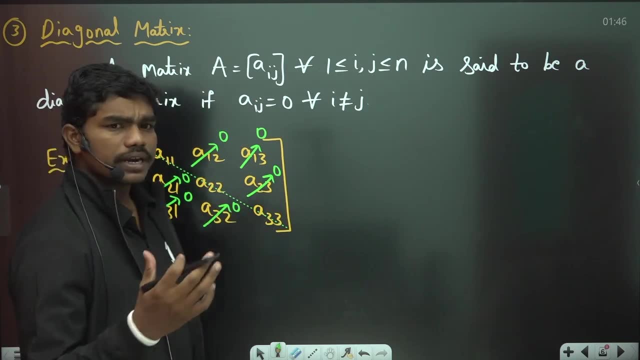 so that's why this element should be zero, this should be zero, this element should also be zero, and obviously, all these elements, they should be zeros, clear so, and even the principal diagonal elements can also be zeros. but one thing that we need to make sure is all the non-principal. 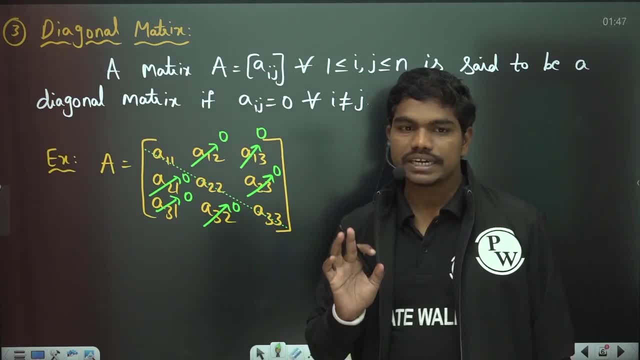 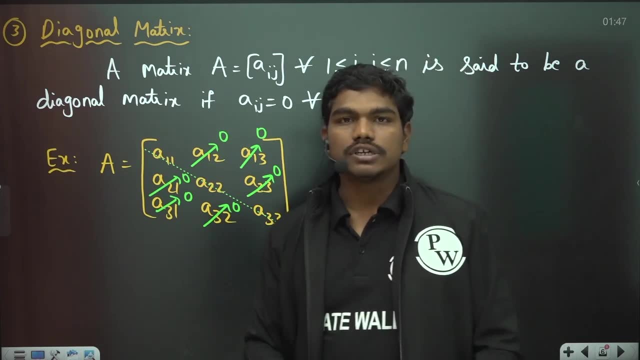 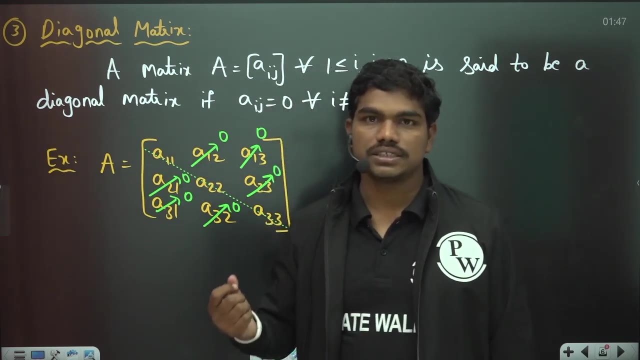 diagonal elements. they must be definitely zeros, clear. so this is a diagonal matrix. and there's one very, really important concept: when you talk about this: diagonal matrices, basically okay, and of course you know how to add two matrices or subtract two matrices, basically. so, straight away, i'm going to talk about multiplication of matrices in the next part. okay, so i we have a lot of more. 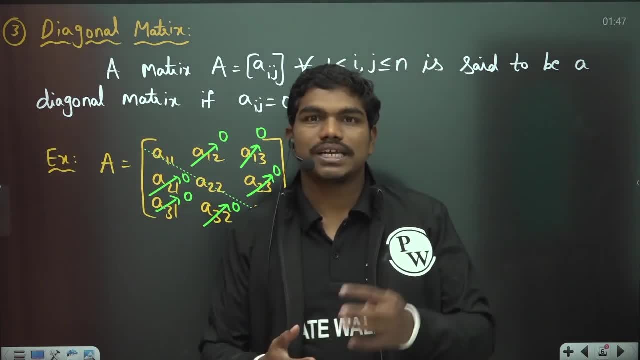 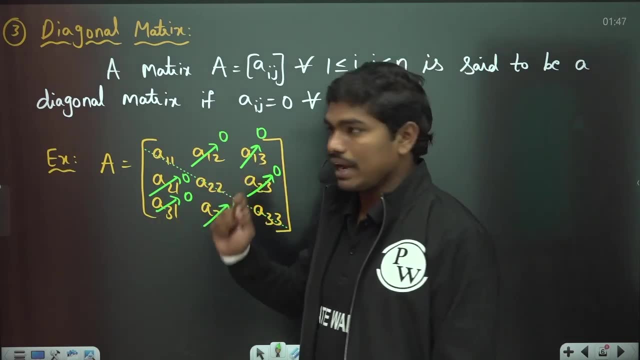 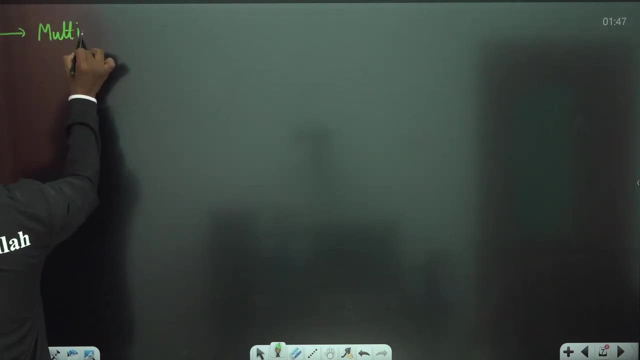 many more types of matrices, but for that you need to understand certain concepts like transpose, multiplication of matrices, those kind of things. so that's why we are talking about multiplication of matrices for a while. okay, so we will go for one thing, which is multiplication of matrices. multiplication of matrices, multiplication of matrices, matrix addition and matrix subtraction. 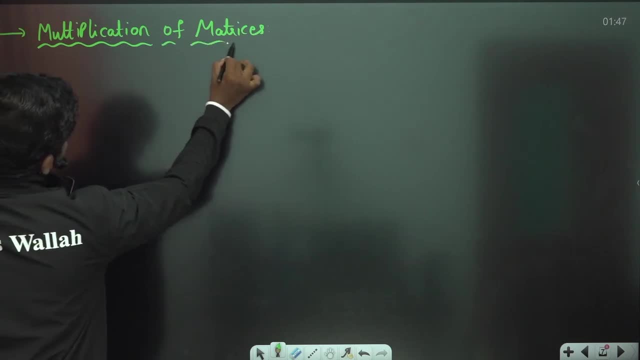 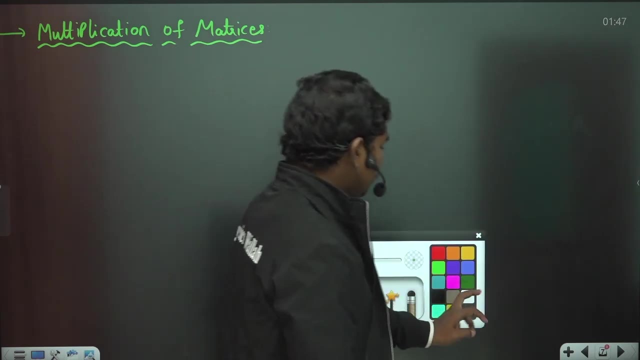 since many of you are very familiar at this level. So I am not, you know, going again to that, but multiplication of matrices is something which is very important. So we will see here. So, multiplication of matrices. So the first property that I would like to give you is 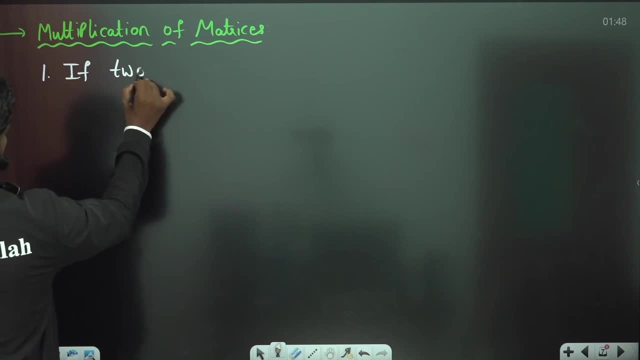 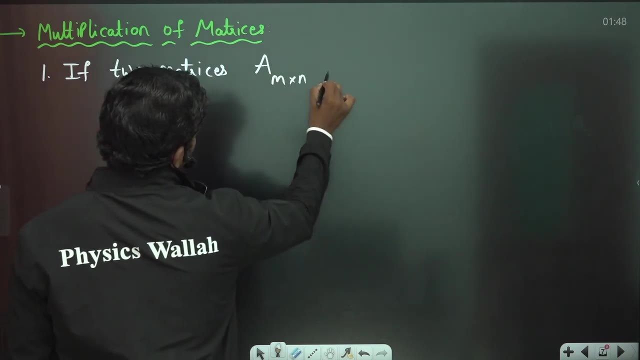 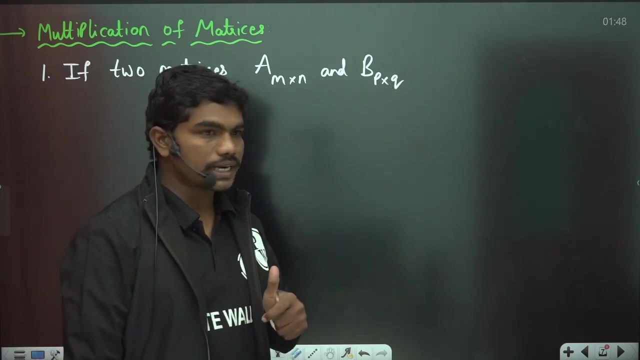 if two matrices, if two matrices- A, m by n and B, p by q- What is the meaning of this? A is the matrix of size m by n means it has m, o's and n columns. B is the matrix of size p by q. means it: 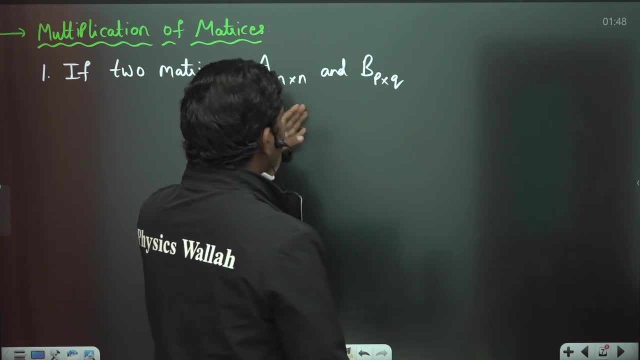 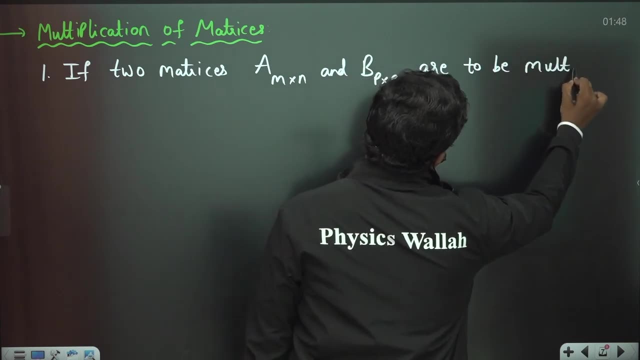 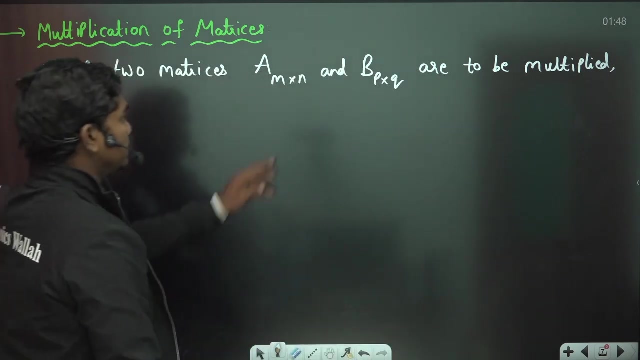 has p, o's and q columns. So if two matrices, A, m by n, and B- p by q, are to be multiplied, are to be multiplied, Then then definitely, if you see, this number of columns in the first matrix should be same as number of o's in the second matrix. So this n should be definitely equal to p. So why this? 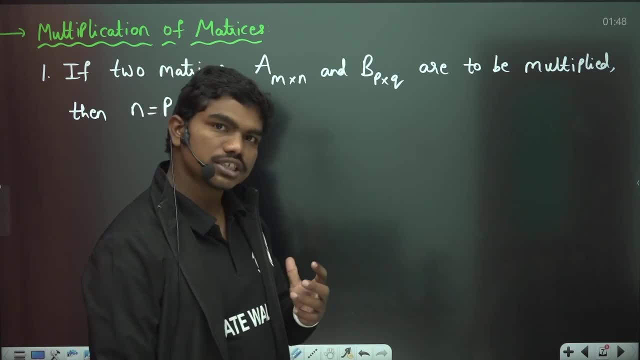 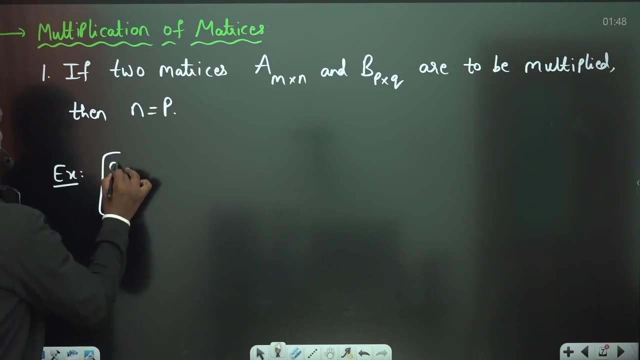 happens? because if you have a quick remembrance of how we do the matrix multiplication, you can easily understand this, because and how we multiply these two matrices. look, I will tell you. Let us suppose you have A, B, C, D, E, F, And so this is a matrix basically of size two by three. then definitely you should have. 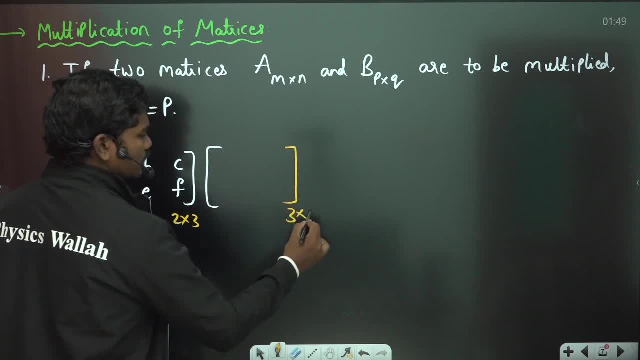 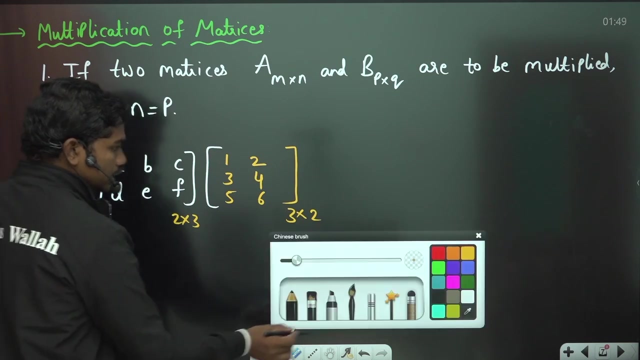 a matrix starting with three o's and any columns you can have. For example, say two columns, If you design this, then three by two, So three o's and two columns So F. So let us say one, two, three, four, five, six, for example. okay, So if you see, these two are 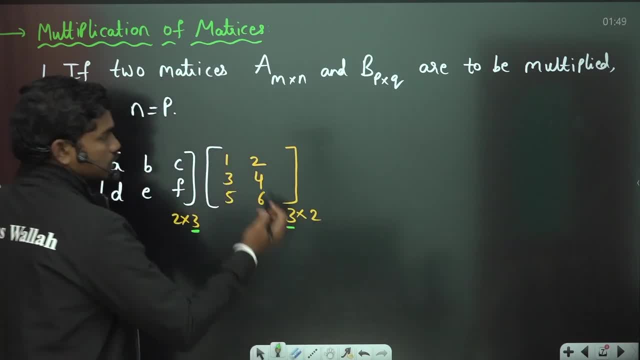 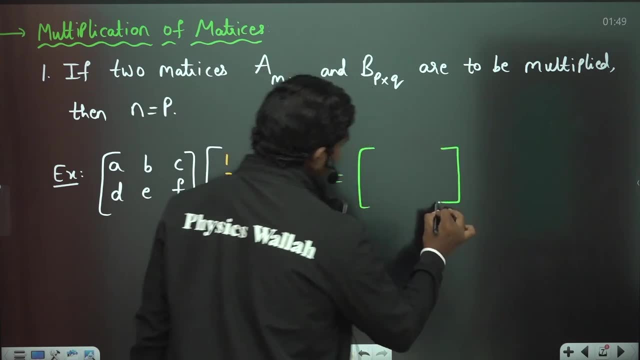 equal number of columns here and number of o's here, which I have stated. So how do you do this multiplication basically? So if you see, the final output matrix is going to be half this size. okay, So the final matrix, if you see, is going to be half this size. 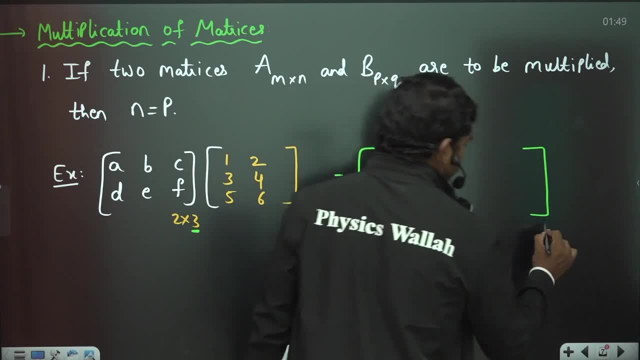 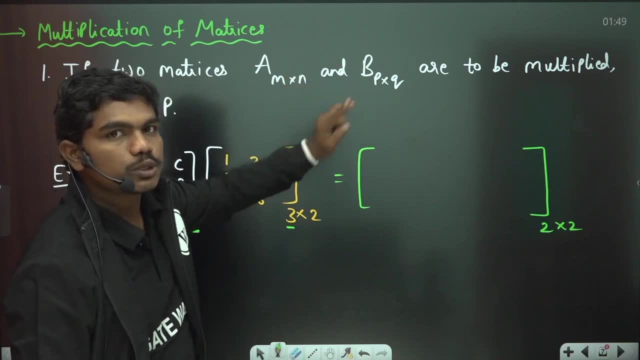 This is of the form m by q, So two by two. okay, So if you see, if you multiply these two matrices- for example, let us suppose if n is equal to p, and if you multiply these two matrices, the product matrix is going to have this order of m by q. okay, So that? 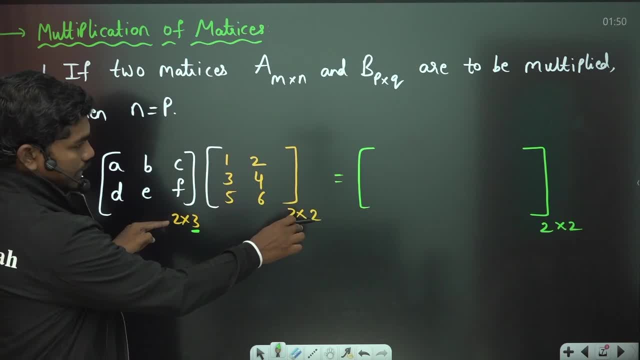 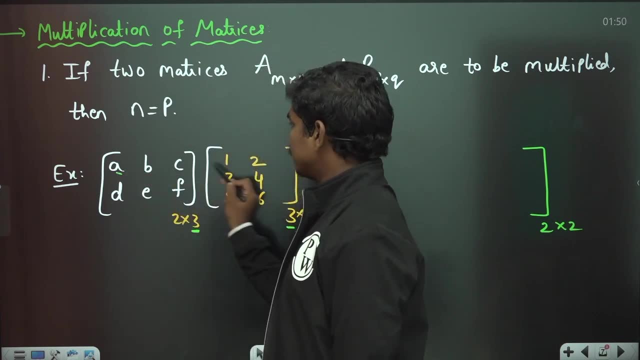 is how? here it is starting with two, These two are equal, and finally it is ending with two. So you have two by two here clear. Now let us see how we will multiply. So you multiply this first element with this first element means basically to get the first. 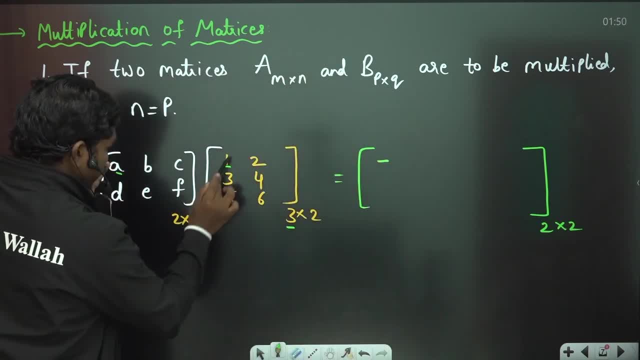 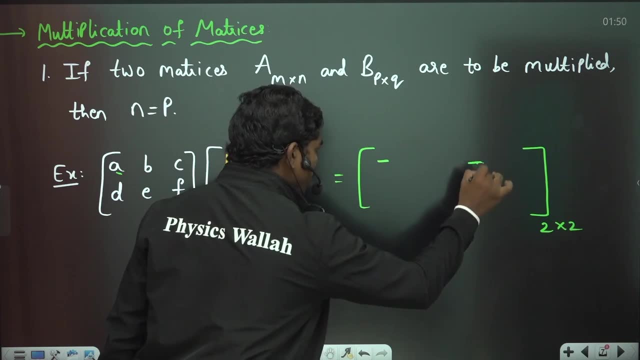 element here, then you should multiply the first o with the first column. Similarly, you will be having one more element here, So to get this element, since it is two, one a two one- So that is why you need to multiply this second o with the first column. That 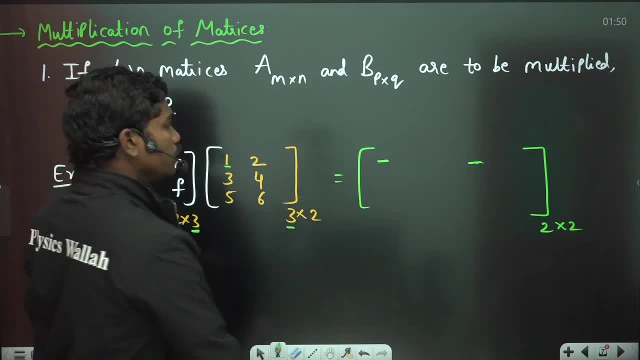 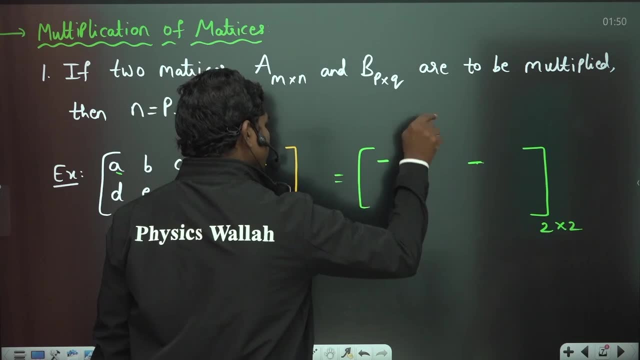 is how you get the first o of this matrix. I am repeating, if you want this element, for you know this is the element in the first or second column. So if you want the first or second column element in the product matrix, you need to multiply the first o with the. 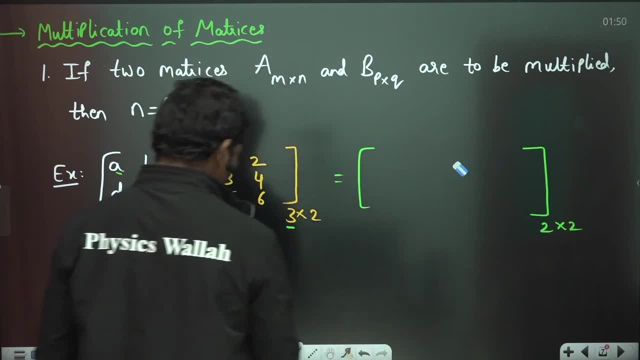 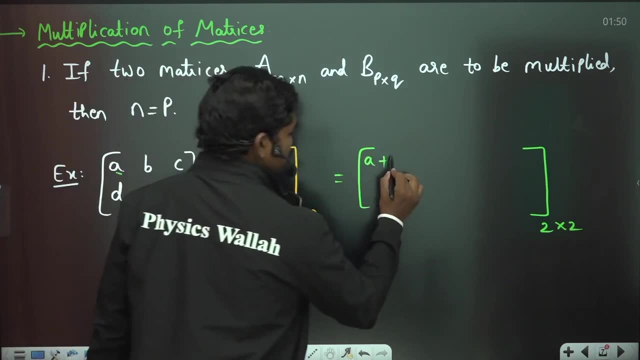 second column. okay, So anyhow, let us do the multiplication quickly. So if you do the multiplication a into 1. So a plus b into 3. So 3 b plus c into 5. So 5, c. So. 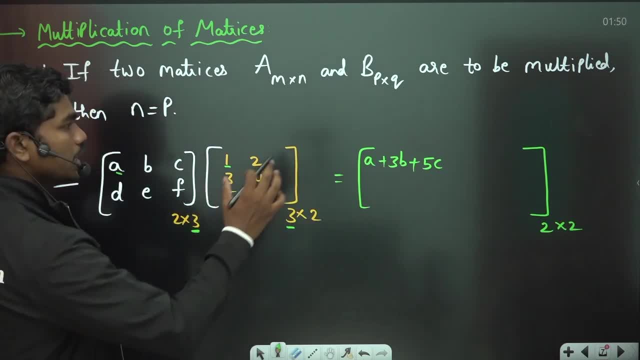 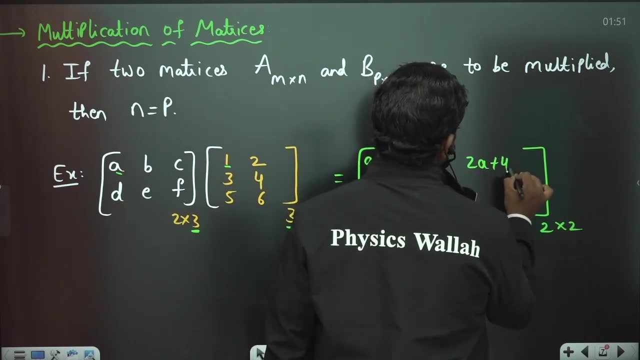 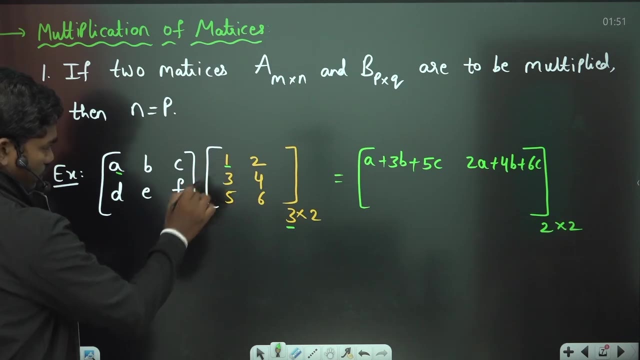 this is the first o first column element of this matrix. Now, what about the first o second column? you want first or second column, a into 2, so basically 2, a plus 4, b plus 6. this is going to be the first or second column. okay, next coming here, second or first column. so 2: 1. here is 2, 1. 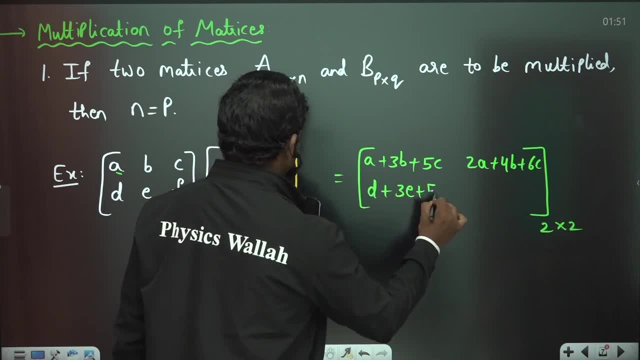 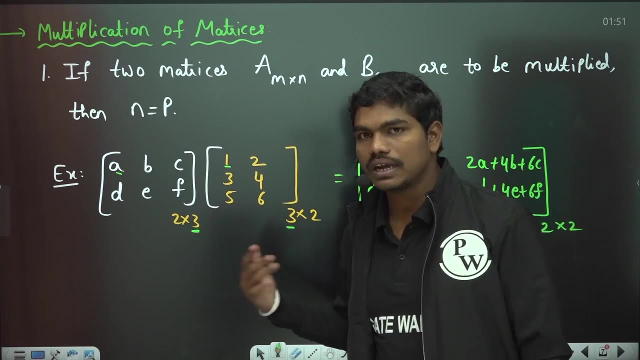 so d plus 3 times of e plus 5 times of f. similarly, here you can write easily: 2 d plus 4 e plus 6 f. okay, many of you may feel that this is all basic stuff, but uh, i'm repeating. understanding this matrices in this ij format is really important, so that's why i'm, you know, going for this, okay. 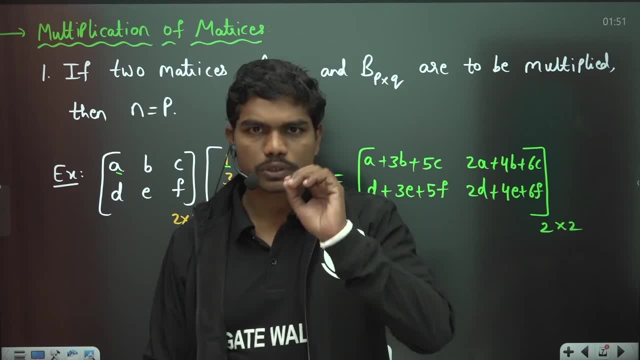 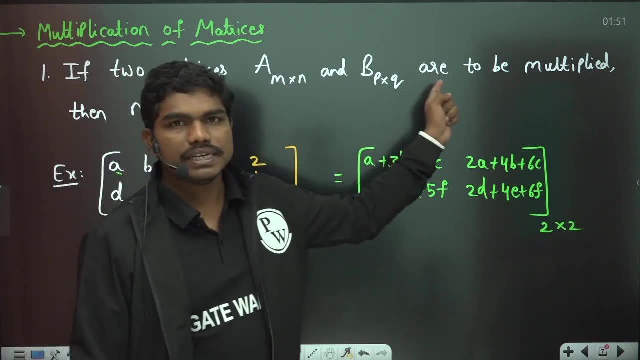 now i'll ask you one very important question. i'll give you time for 5 seconds. you can pause the video here and you can try to answer. let us suppose, if i want to multiply these two matrices, a is of size m by n and b is of size. let's say n by q, p and m p and sorry, p and n. both are equal. 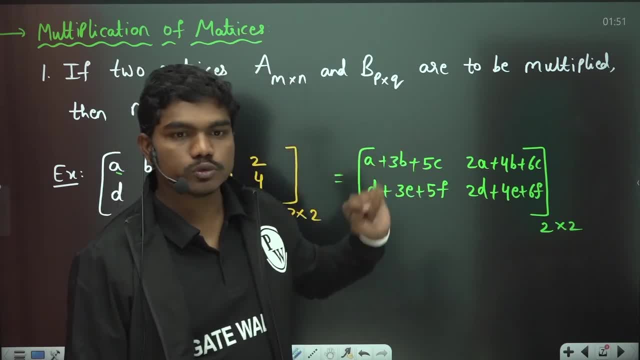 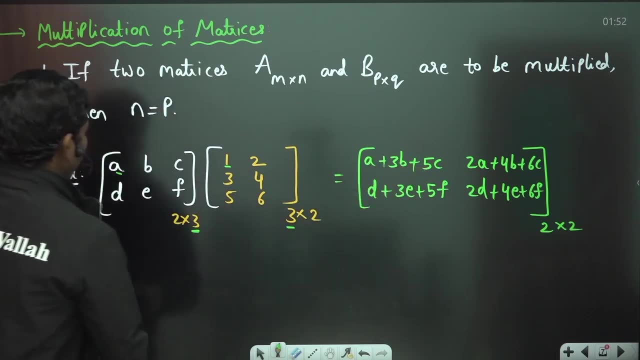 so let us suppose if these two are same, then if you want to multiply these two matrices, what are the total number of multiplications you need to do? look, for example, to get this first element, what i'm doing, i'm multiplying the number of multiplications you need to do. 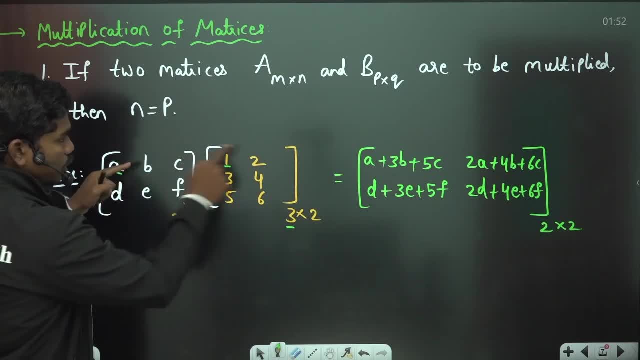 so i'm multiplying this a with this one. so first multiplication i'm doing again to get this 3b. i'm multiplying this b with 3. so i'm doing one more multiplication. c with 5, i'm doing one more multiplication. so basically, how many multiplications i need to do if you have this matrix of n and p? 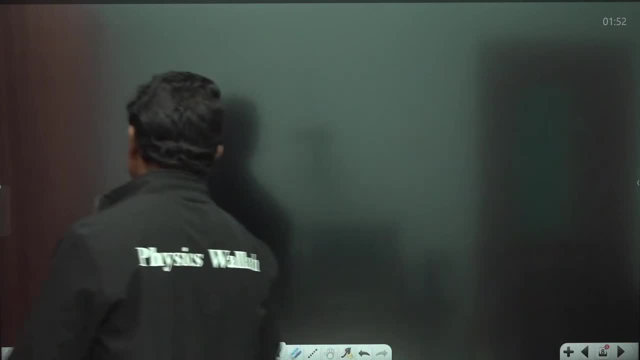 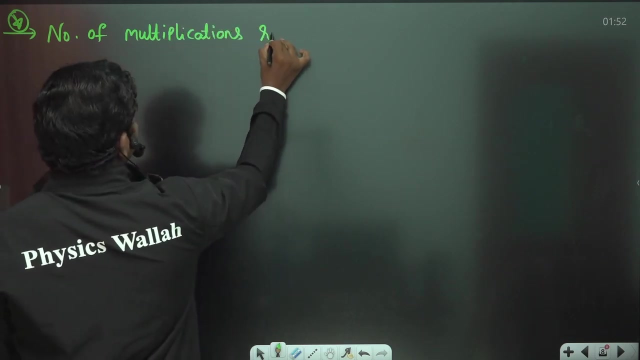 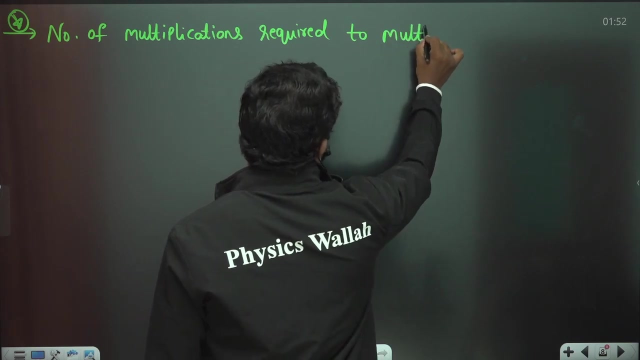 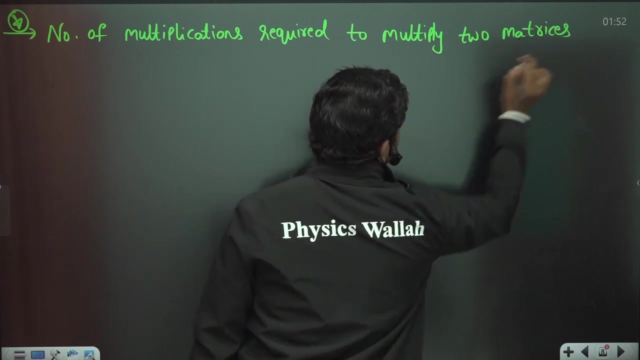 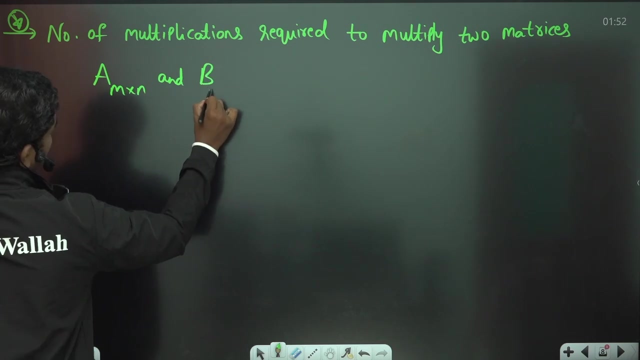 basically here. okay, the answer is number of multiplications required. number of multiplications: number of multiplications required required to multiply two matrices. to multiply two matrices, to multiply two matrices- a, m by n and b? n by p- is: do you know how many? the answer is going to be: 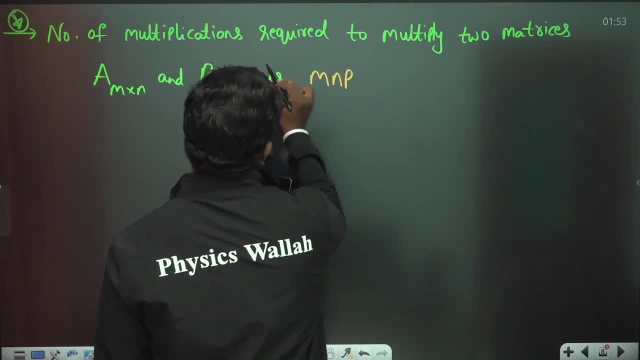 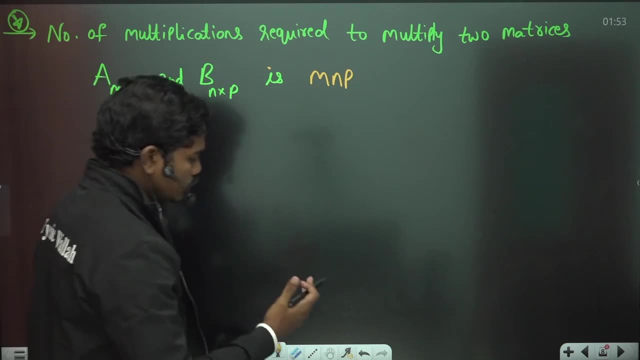 m by n and b and b 0 and b by m into n, into p. so these many multiplications actually you need to do to get these elements okay, and this is- i can show you this- results very easily. okay, but before showing the result, i would like to give you one more important point: number of additions. 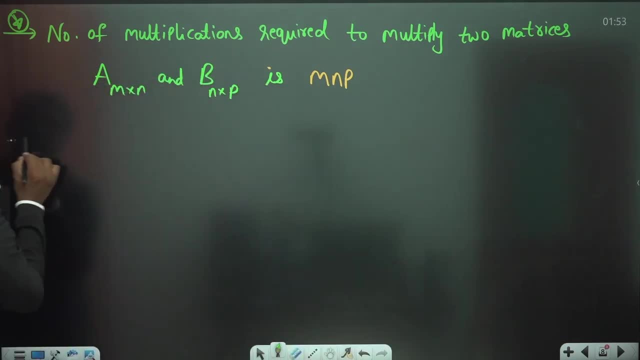 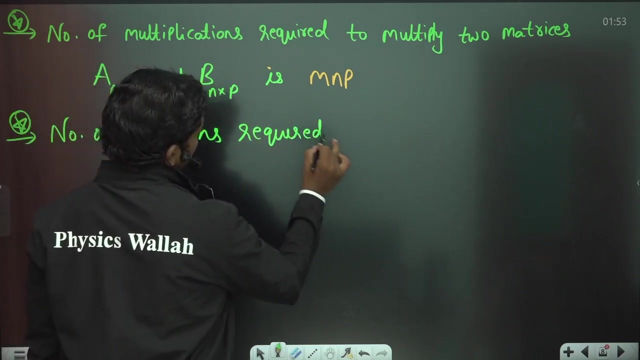 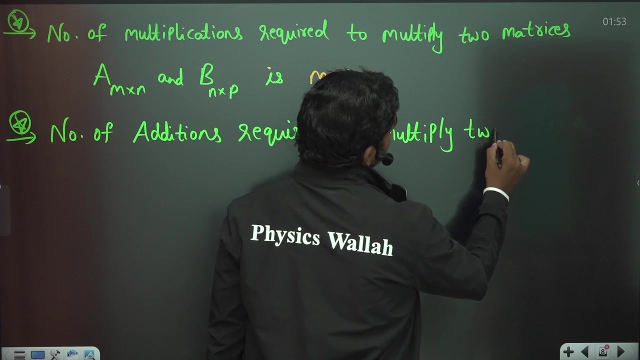 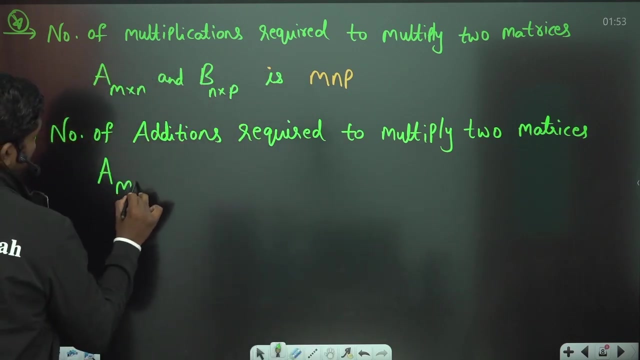 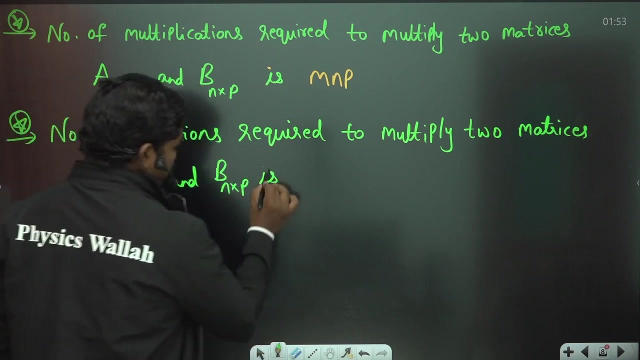 m by n and b? n by 3s. number of additions: m by n and b? n by 2. m by and b? n by 2. number of additions: number of additions: number of additions: qualities. number of additions required. multiply: to multiply two matrices: to multiply two matrices, a? m by n and b? n by p, is is you: 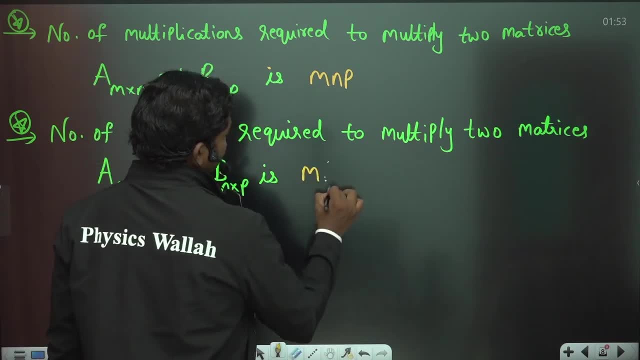 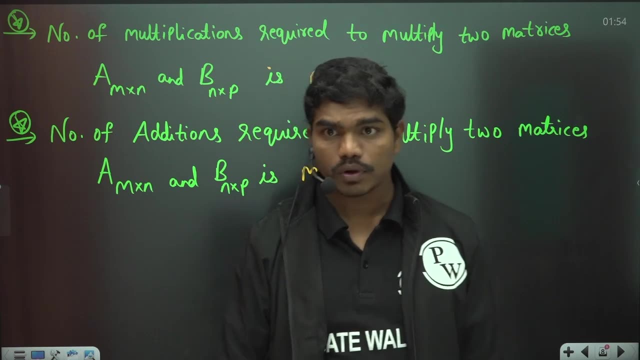 can see, is m times of n minus 1 into p. so basically, how did i get this expressions? it is very simple. and first of all, you may have one doubt with the second point: if i am multiplying two matrices, how come additions are coming into the picture correct? this may be common intuition. 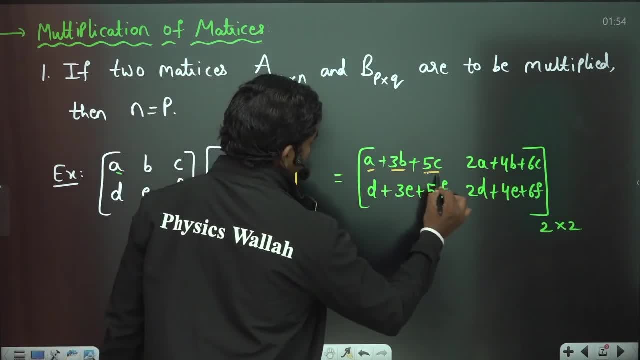 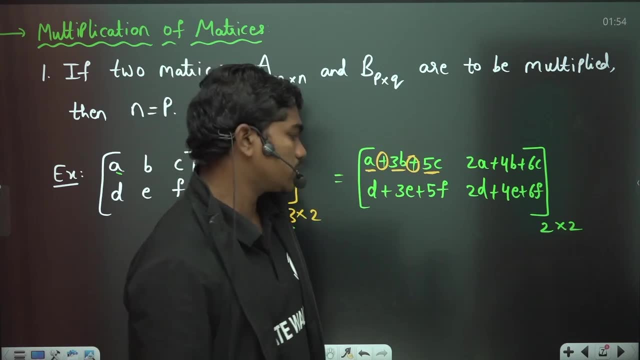 but here, if you see to add these three numbers, three multiplied values, you have. but to add these three multiplied values you are doing two additions, correct. if you have three numbers, you will do two additions, right to get the total sum. that's how. so let us quickly see how we are. 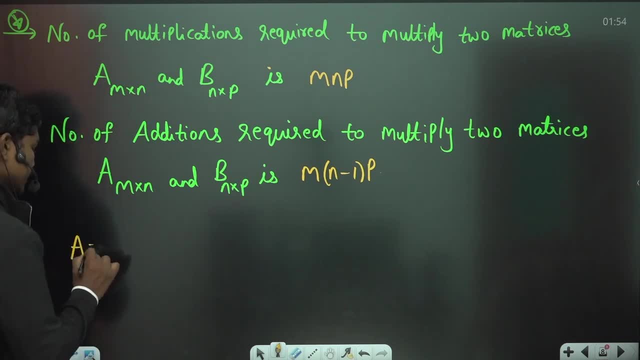 getting these formulas. for example, let us suppose a is equal to m by n matrix, so a 1, 1 a, 1 2, a 1 3, and so on. a 1 n because it has n columns, so there should be n numbers in the first row. similarly, a: 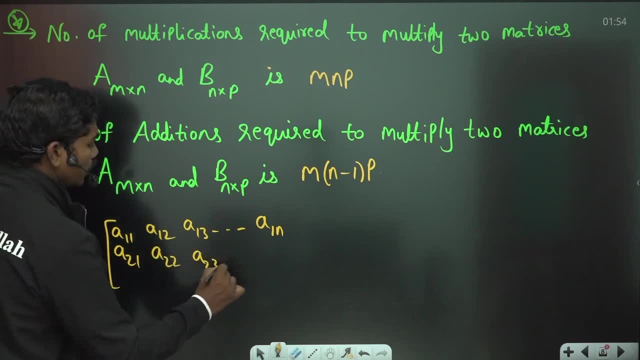 2, 1, a 2, 2 a 2, 3, and so on. a 2, n, and this goes on. finally, you know that there are m rows in this matrix. so a m 1, so you can see that this is a m 1, a m 2, a m 3, and so on. finally, you have. 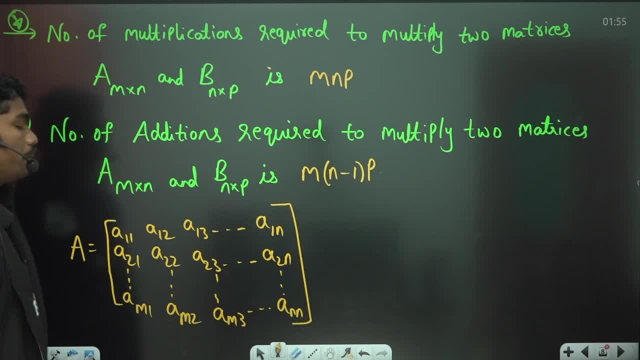 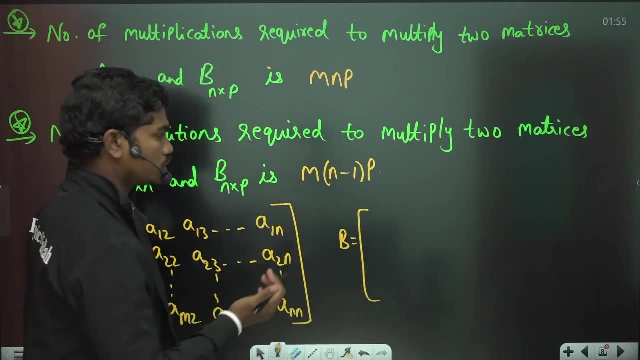 a, n, n. this is the matrix that's going to come here. and what about this? uh, you know b matrix, b, b is. it has again n rows. so let us suppose you write b 1, 1, b, 1, 2, b 1, 3, and so on. 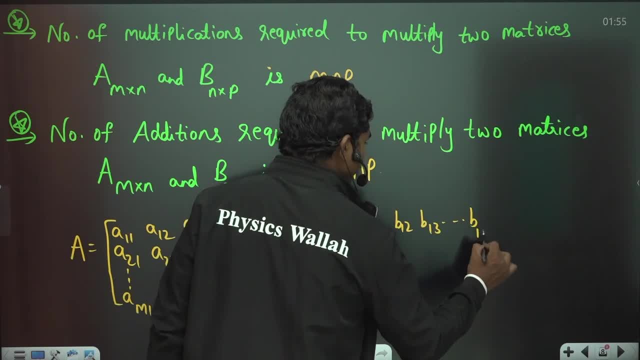 it has p columns, so we have written n by p, so this is b 1 p, similarly b 2 1, b 2 2, b 2 3 and so on b 2 p. so this goes on and finally we have this n rows here. so 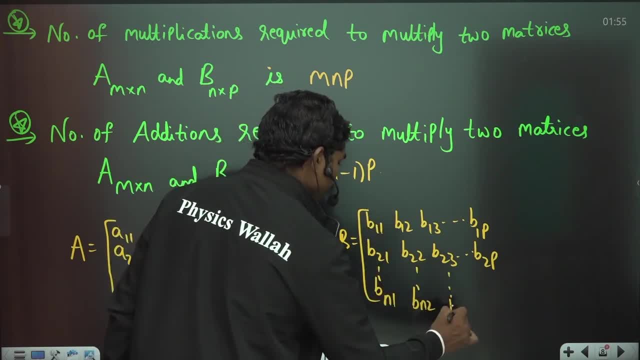 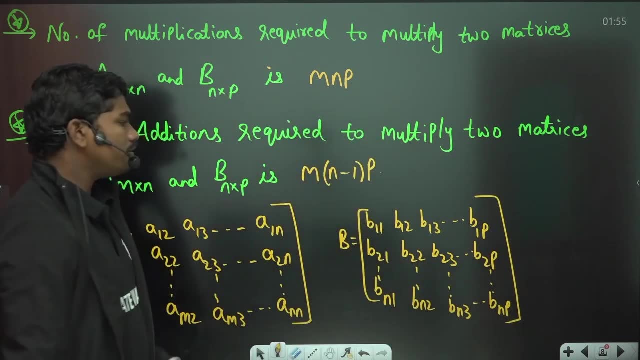 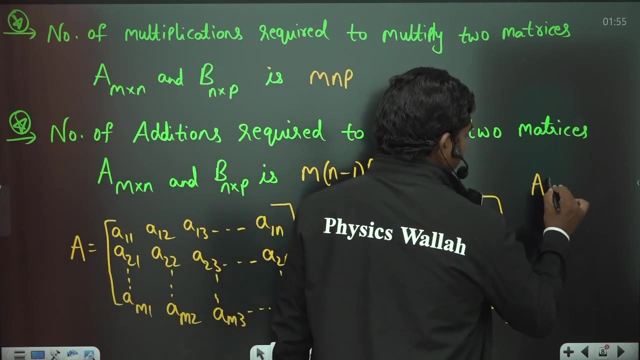 that's why n, 2, n, 3 and so on, b, n, p. so these are the two matrices. now let us suppose if i ask you, if you want to multiply these two matrices, how many multiplications you need? first of all, tell me one thing: if you multiply this matrices a and b, the order of this matrix is going to be: 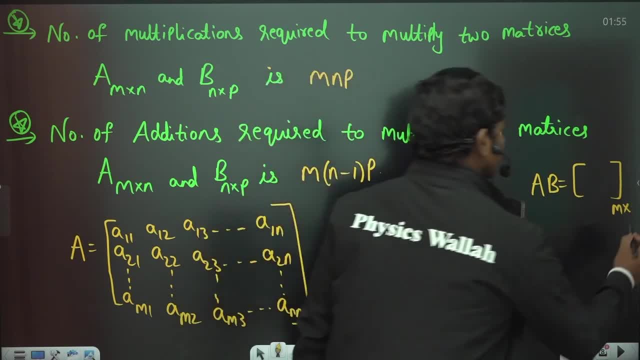 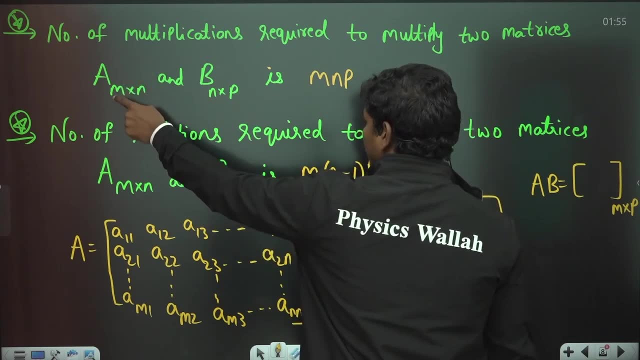 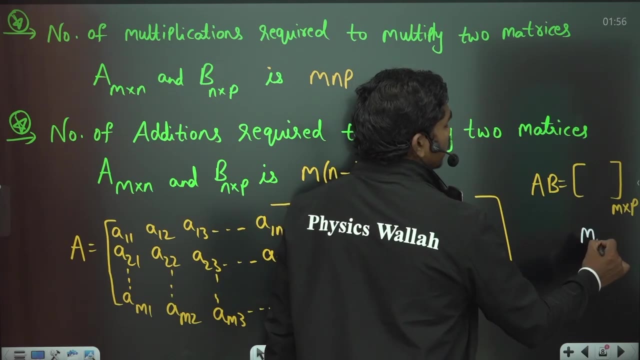 m by p, correct? so, because, if you see, this is of order m by n and this is of order n by p, and if you multiply these two, the resultant is going to be having of order m into p. now try to understand one thing: so total number of elements in this matrix will be m into p. you know this, correct? 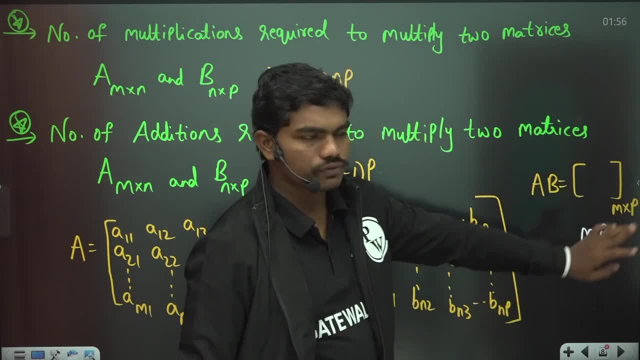 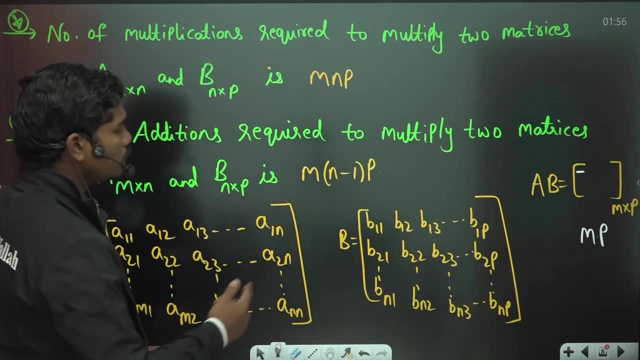 so total number of elements in this matrix is nothing but number of hours into number of columns. now tell me one thing: if you want to get the first or first column element, if you want to get the first or first column element, what you will do? you will multiply this first row with this first column. 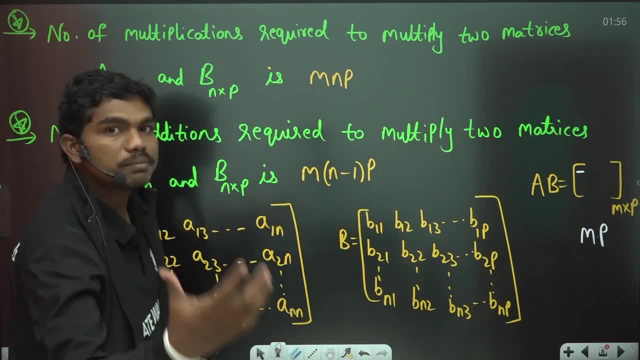 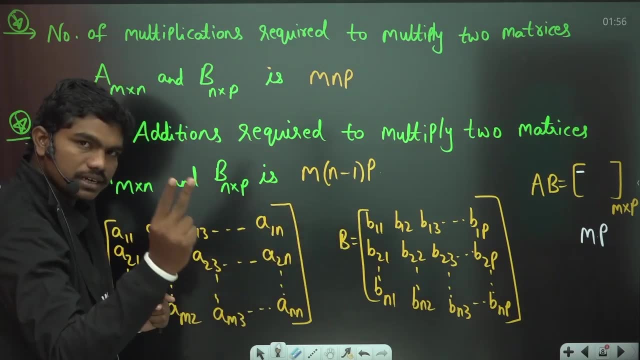 correct. so for multiplying this first row, with this first column, how many multiplications you will do? a 1, 1 into b 1: 1. one first multiplication you will do. next: a 1, 2 into b 2: 1 second multiplication you will do. 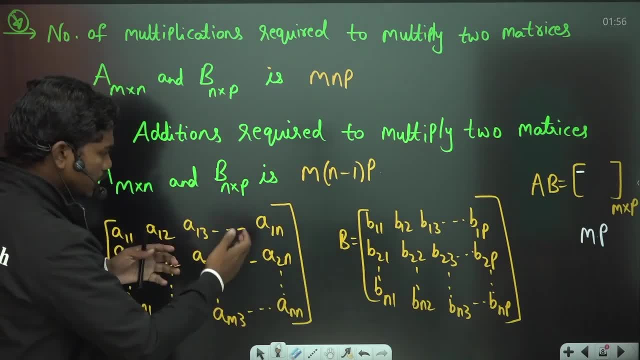 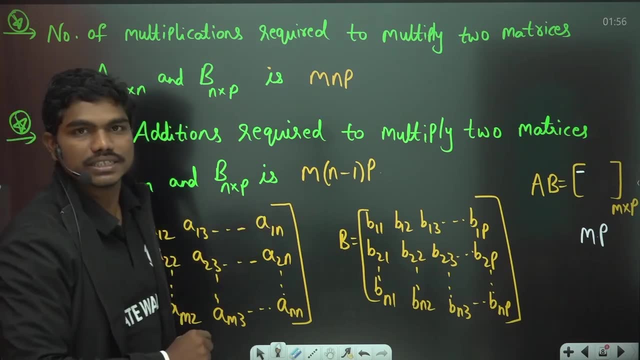 a 1, 3 into b 3, 1. so third multiplication you will do, and so on. if you keep on doing five, by the time you reach a 1 n into b n, 1, you are total doing n multiplications because the n elements in the first okay, which means for getting the first, first column element, you are 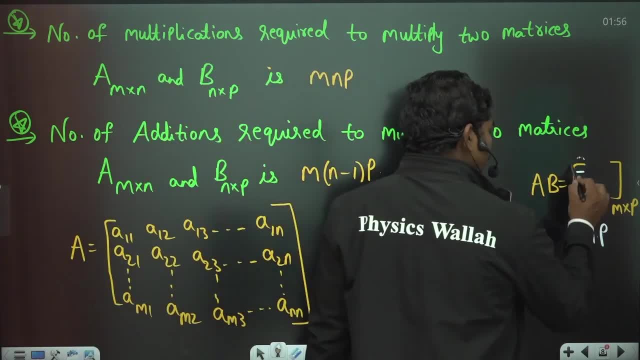 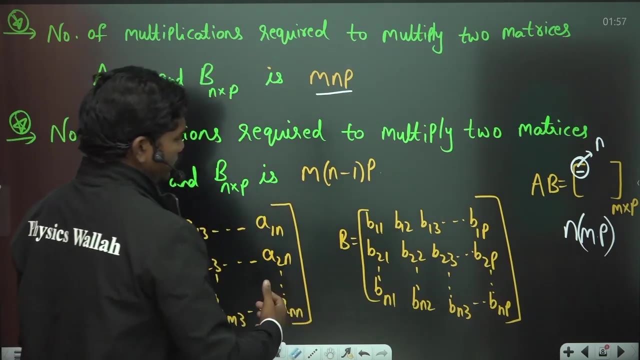 actually doing n multiplications, right? so for getting one element you are doing n multiplications. so to calculate this m into p elements, how many multiplications you will do n into this m, p, which is nothing but this m and p. clear, now you can understand the same thing: if you are doing n multiplications to get this first number, then how many additions? 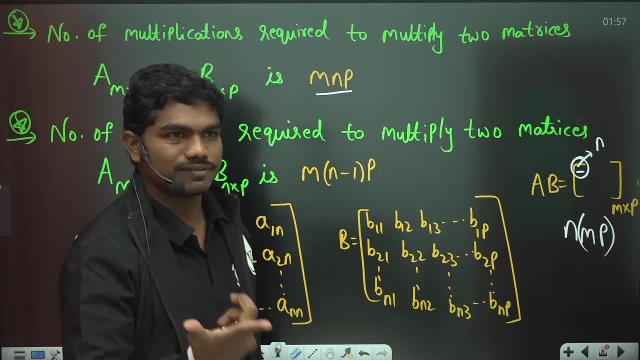 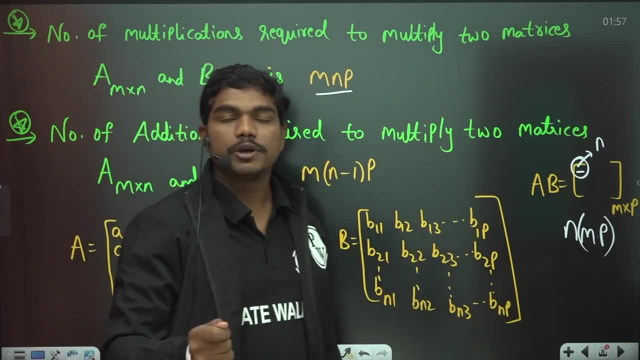 you will be doing. obviously, number of additions are one less than the number of multiplications. so that's why, if you are doing the n multiplications to get this first or first column element, that means you will definitely do n minus 1 additions to add them up. so for one. 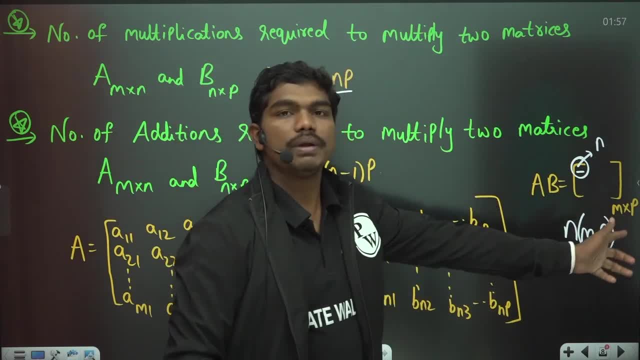 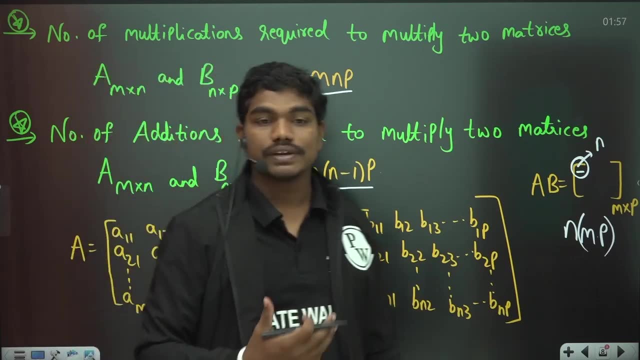 element, you are doing n minus 1 additions. so for m into p elements, how many multiplications, how many additions, you will do n minus 1 into m p. so this m into n minus 1 into p, otherwise you see, is the number of additions required to multiply the two matrices. that's all you know, basically, in 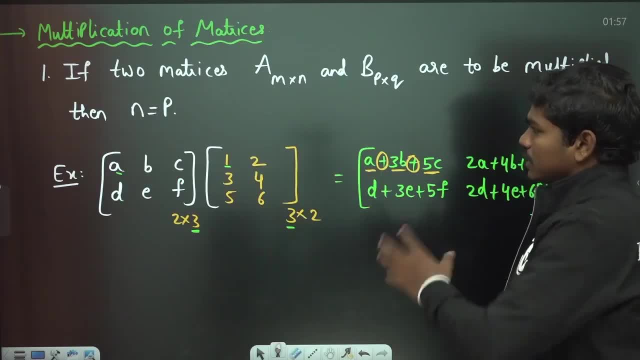 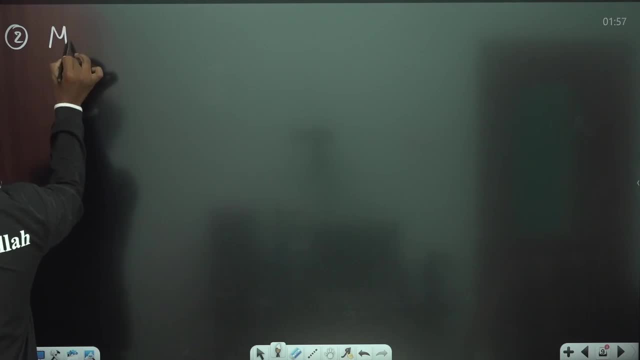 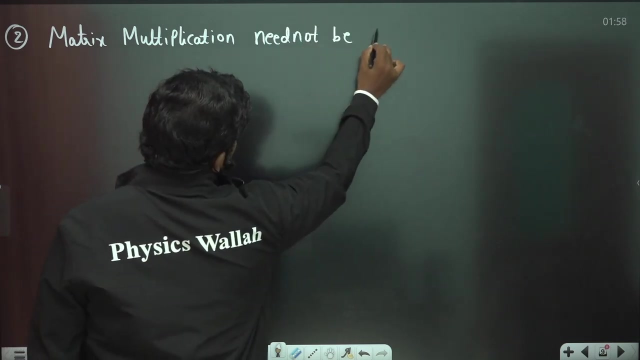 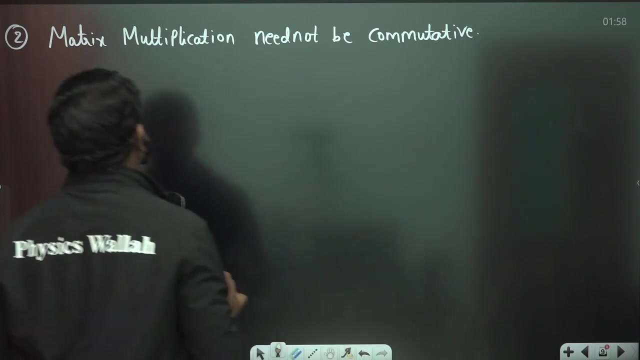 the multiplication. okay, so this is one very important. uh, you know understanding from here. now, the second point that i would like to talk about, matrix multiplication, is matrix multiplication, matrix multiplication. matrix multiplication need not be commutative, need not be commutative, need not be commutative. so what is the meaning of this? you know the commutative law. 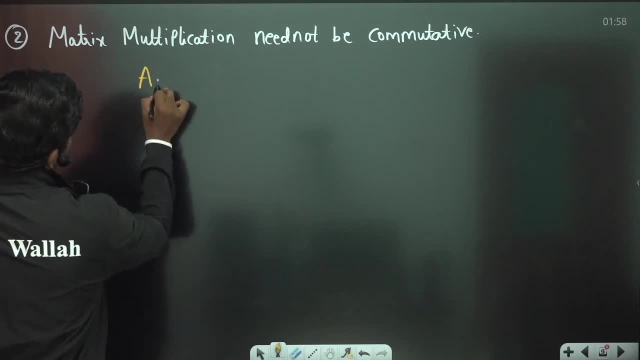 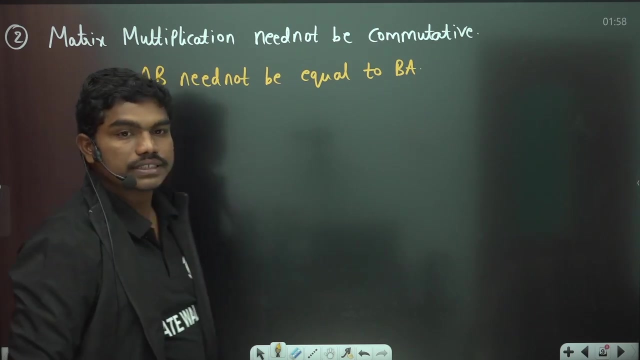 in mathematics. so basically means a into b, a b, you can say: need not be equal to b, a, a b need not be equal to b, a equal to b a. now how i can show this, for example, because i have told some- uh, you know order just now. 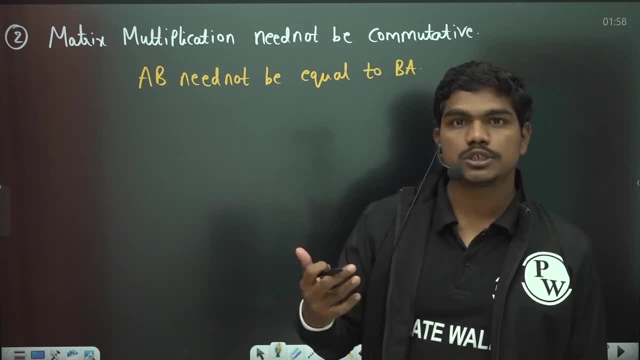 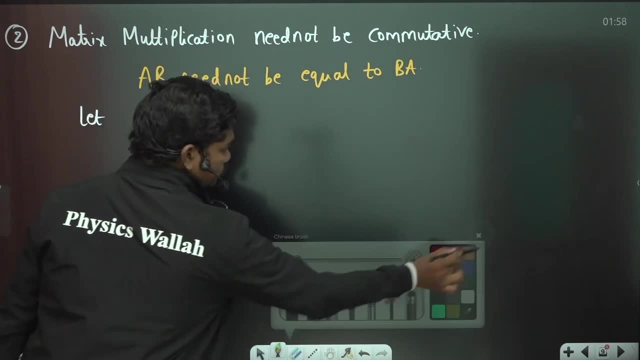 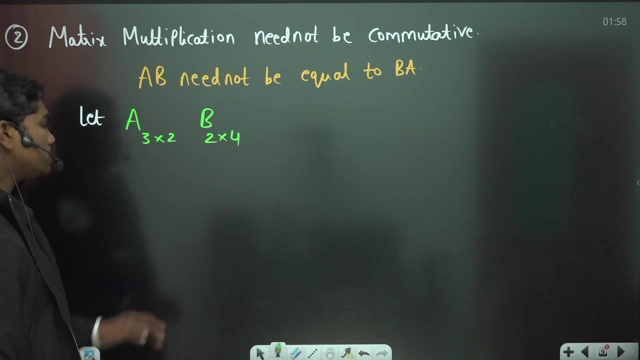 that matrix multiplication need not be commutative. but how do i prove this to you? look, i can prove you. for example, let us suppose you have taken this matrix: let a is equal to let a is of size 3 by 2 and b is of size 2 by 4, for example. then if you see, then if you see, 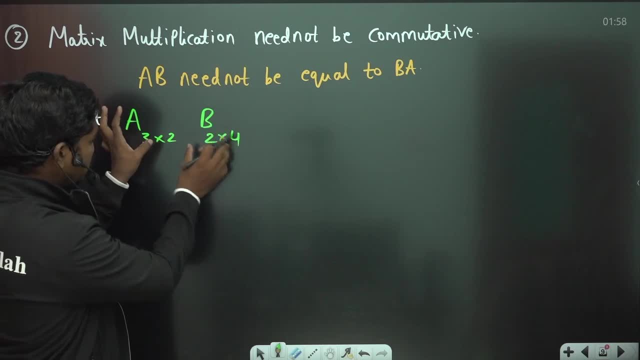 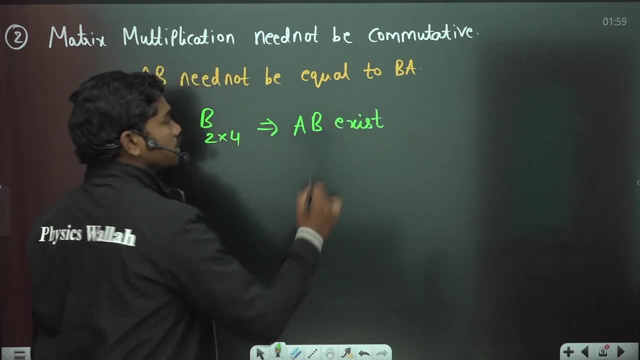 this two matrices, a into b, is possible. correct means: if you multiply this b with this a, this a is possible. means: if you multiply this b with this a, this means this implies AB exists. Yes or no AB will exist. Why? Because if you multiply, in this order, this number of 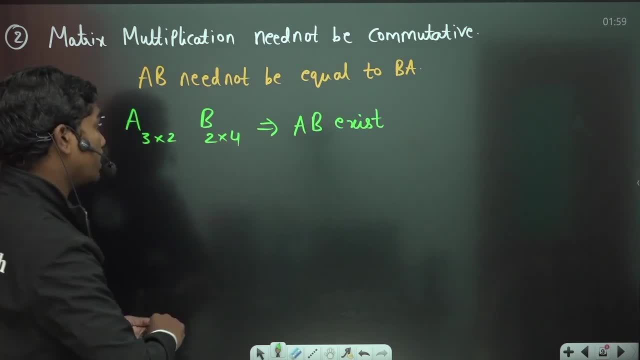 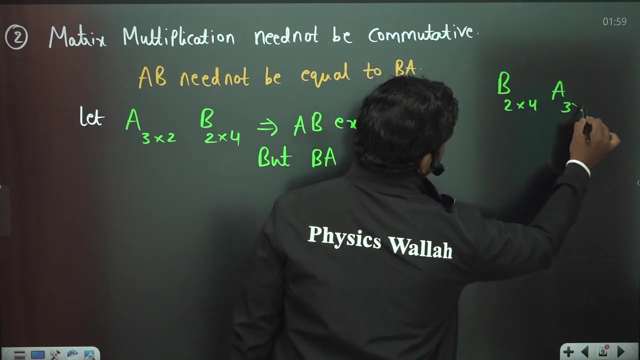 columns in the first matrix is same as number of rows in the second matrix, But B into A. if you try multiplying B into A, then 2 by 4 and 3 by 2 matrix, correct. So basically BA is something like this: B is 2 by 4 matrix and A is 3 by 2 matrix. So here clearly you can understand. 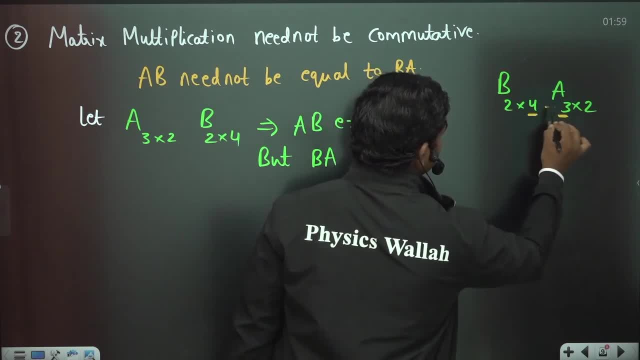 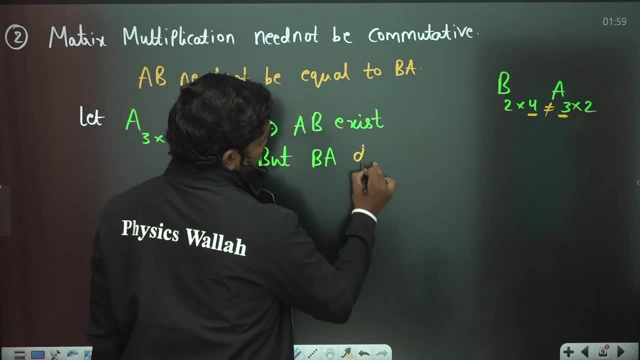 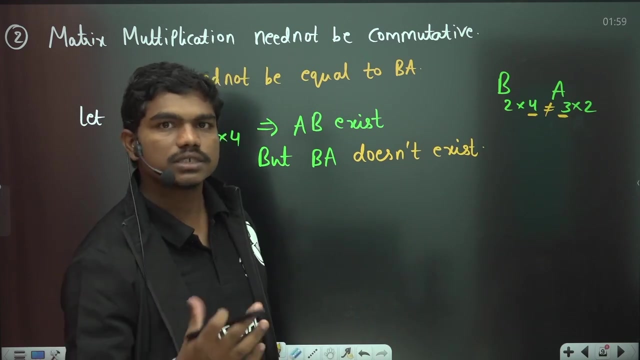 one thing, that here the number of columns and number of rows are not equal. okay, So that's why this kind of multiplication is not possible for the same two matrices. So, but BA doesn't exist, This doesn't exist, So forget about equating them or not equating them Sometimes, even if AB exists. 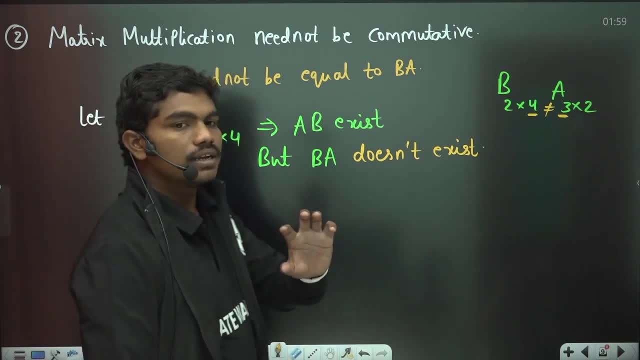 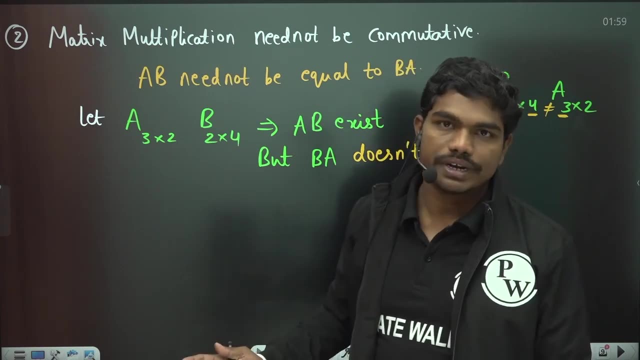 BA may not even exist, okay. So that's why you can never conformally say that matrix multiplication is commutative. This, you know, this result is actually one good thing that shows that matrix multiplication cannot be commutative clear. So this is one very important thing. 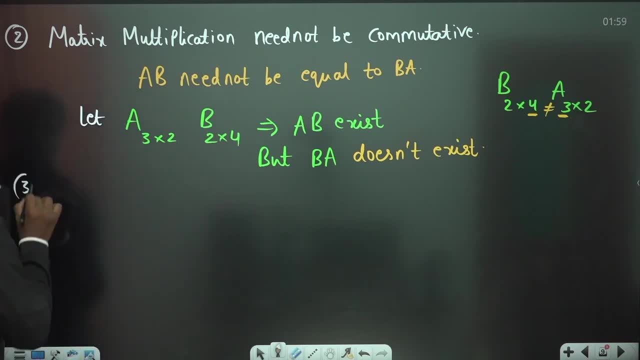 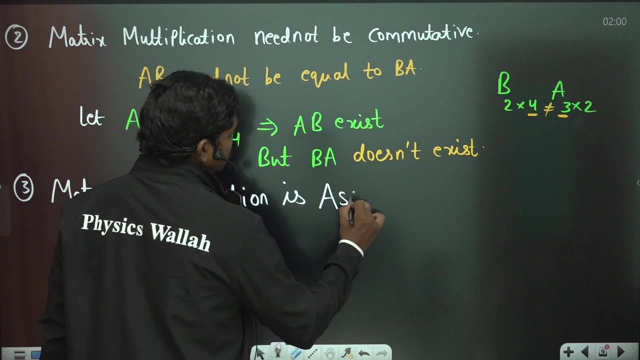 And property again Now third property: matrix multiplication is associative. Matrix multiplication is associative, is associative. So, basically, what's the meaning of this If you have three matrices, for example? let us say then, if you first, of course, all these, 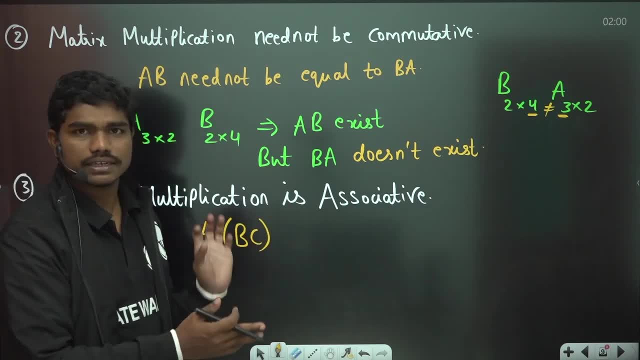 three matrices are facilitating matrix multiplication. So if you have three matrices, for example, multiplication means number of columns in the first matrix should be same as number of, you know, rows in the second matrix. All these things are holding good. So, whenever in such cases, if you 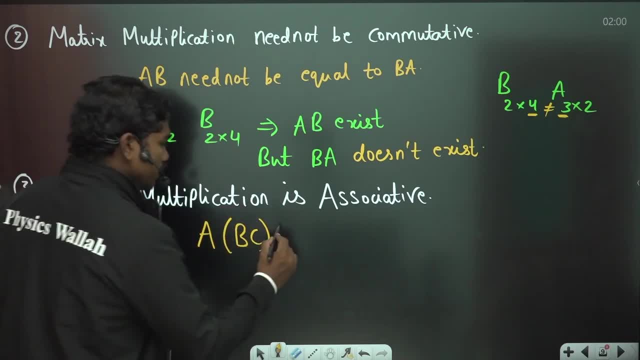 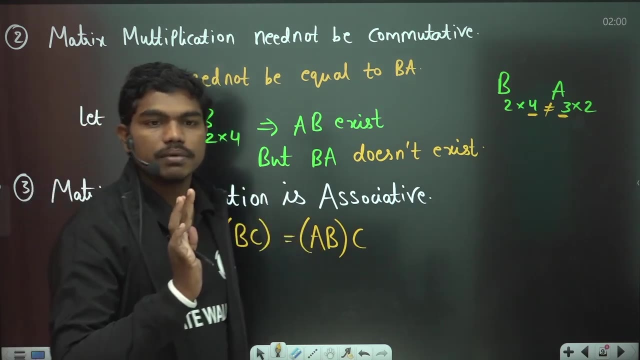 have three matrices, for example, then A of this BC will be same as AB of C. Means first of all, when you have three matrices now, if first you multiply BC and then you multiply A to the result, or if you multiply AB and then if you multiply C, the result remains same. Why this property is. 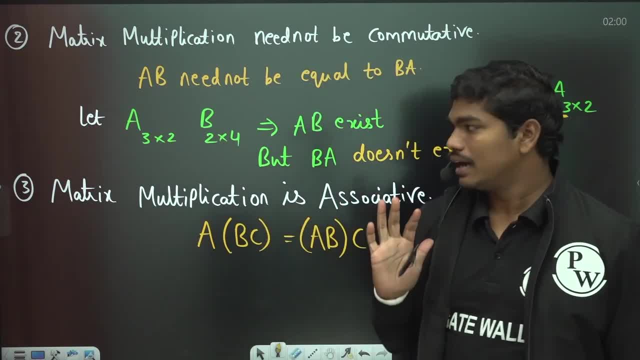 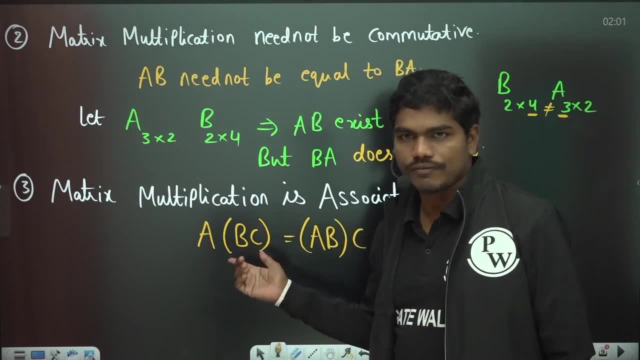 very, very important. Actually, frankly speaking, this property is very important. Why? I'll tell you. Let us suppose you had some big matrices, some 50 by 50, 100, or 50 by 100 and some 100 by you know 50 again, some matrices like this. Now, many of you might be doing this: C plus plus. 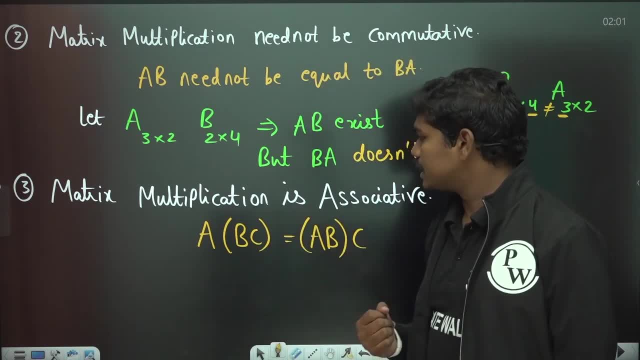 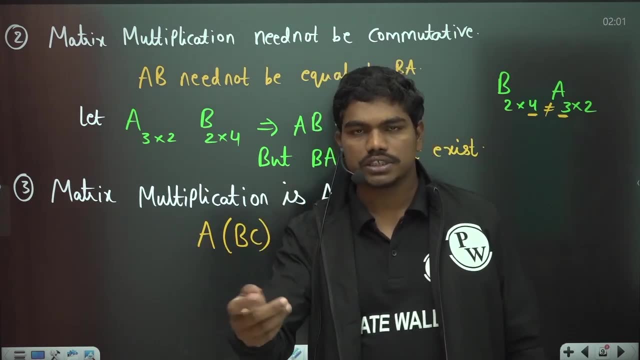 or C coding in general in labs. So what happens is normally you write a code. If you want to multiply three matrices, you will write a code, and the time of execution of this code depend upon the number of calculations- number of automatic calculations, the computer perform. Now let me give 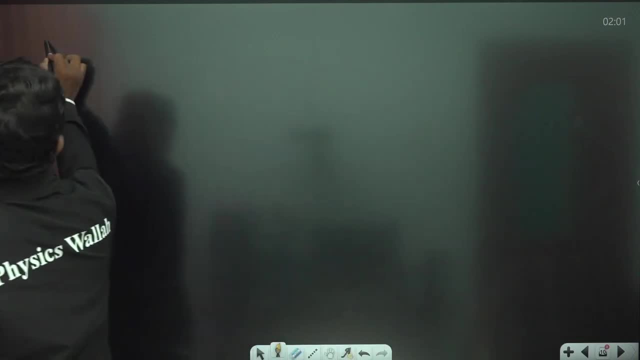 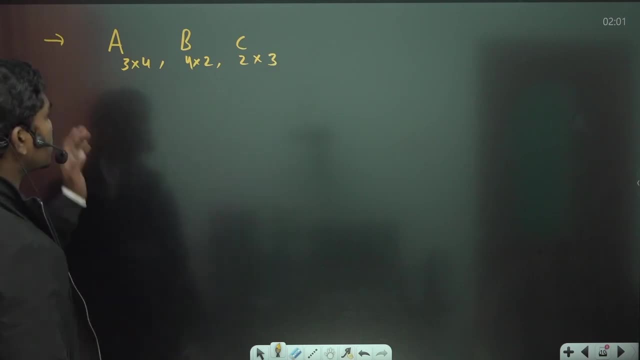 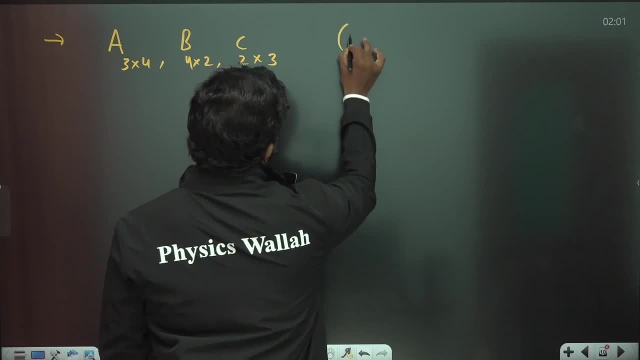 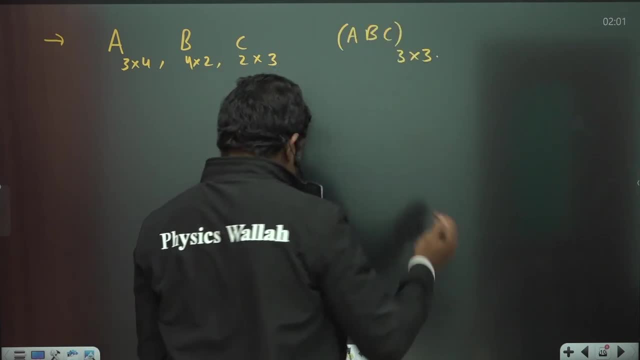 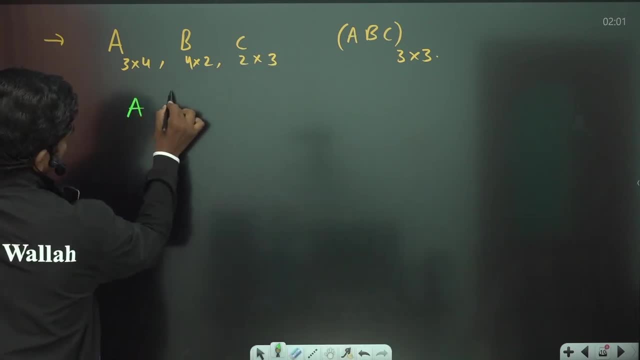 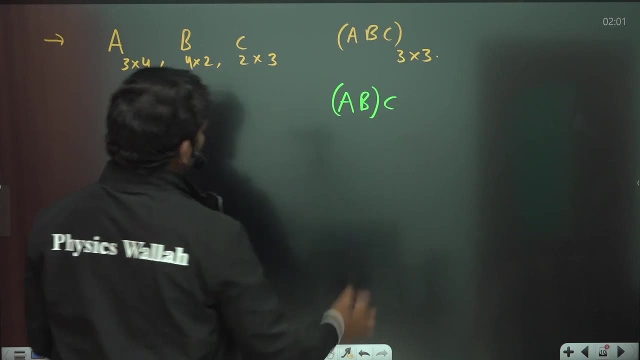 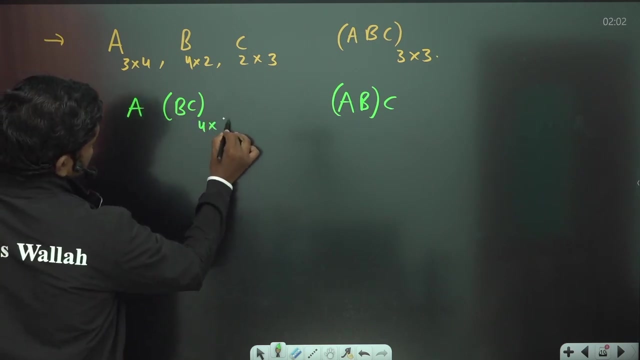 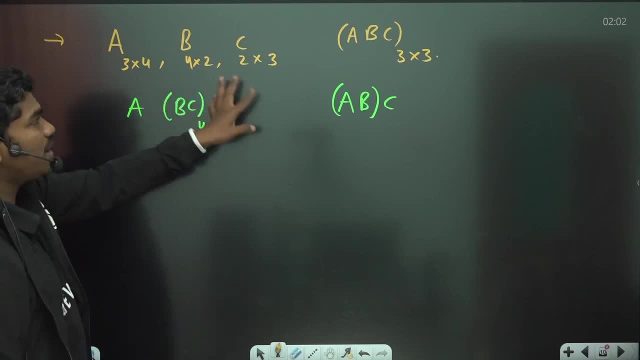 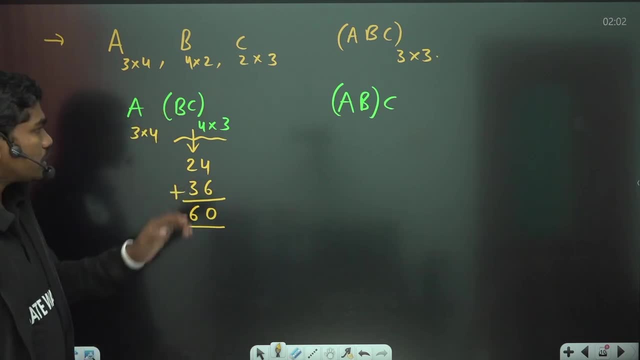 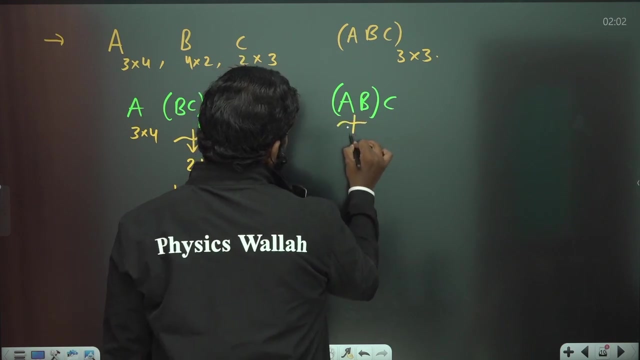 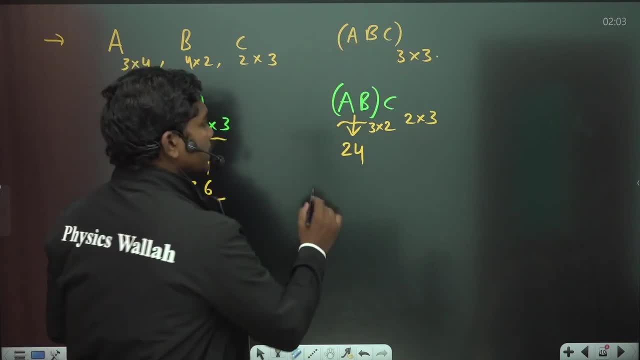 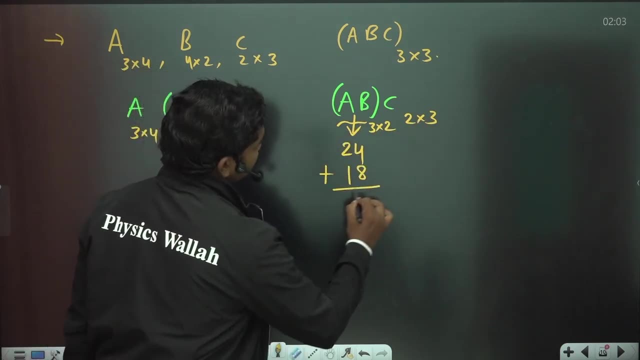 if you see the multiplication of this a, b with c, how many excess multiplications you need? this is a, 3 by 2 and this is a, 2 by 3. so 3, 2's are 6, 6, 3's are 18. so if you see, this is 18, so total: 42. so here: 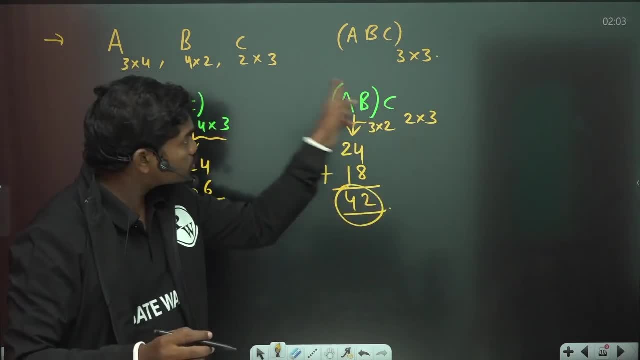 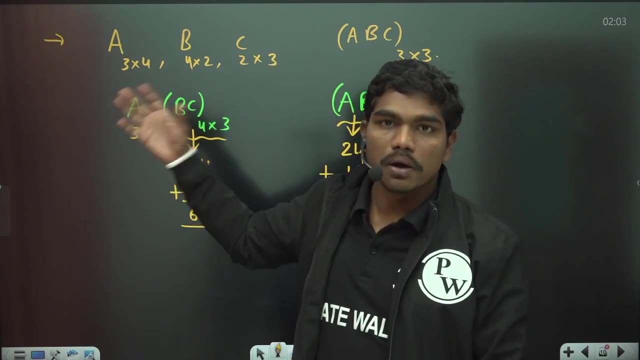 in this case you need only 42 multiplications. of course these are small numbers, so that's why 42 and 60. of course, still there is much variation. but imagine when you are dealing with 100 by 50 of that size. when you are in some research or some work, you will definitely write the programming in. 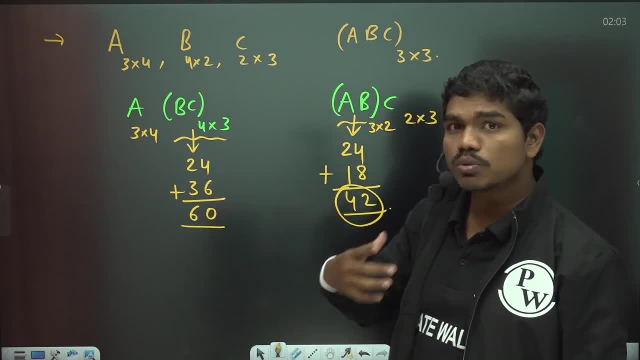 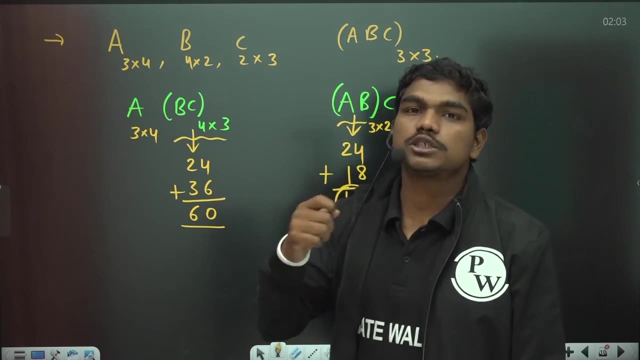 such a way because, you see, the result is same in both the cases. so in such cases, what you write, you will definitely write the code in such a way that the minimum number of operations will be done by the computer, so that your execution time will be faster. so, using this simple manual analysis, 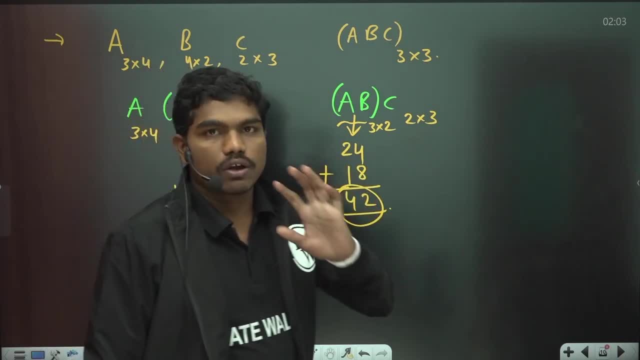 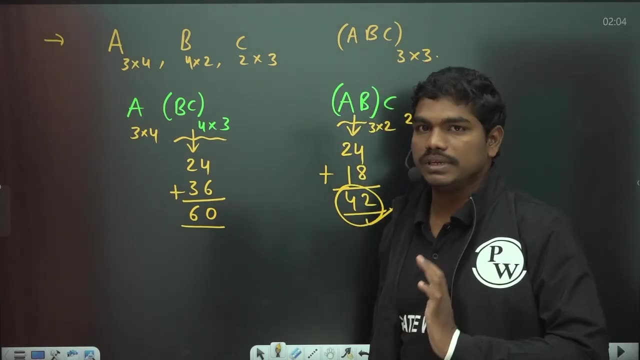 you will come to know which order to multiply and you will write the code accordingly for reducing your execution time. clear. so that's how. in this case, the number of multiplications required is less and it's minimum, basically, okay. so that's how this mnp is very important here and, of course, 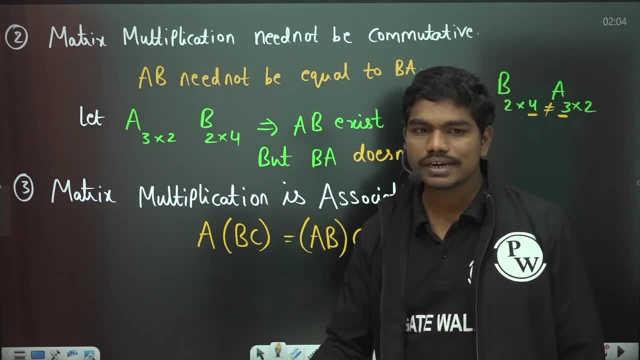 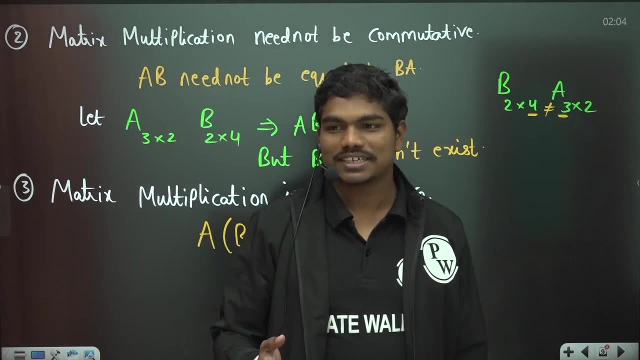 this law. you will definitely write the code in such a way that the minimum number of operations will be done and that x multiplication is associative is also very important. clear. i hope i've, uh, you know, cleared your questions and uh, previously, when i was taking some youtube class, people were asking: 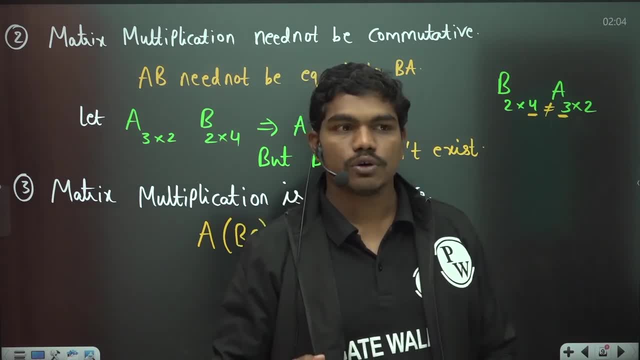 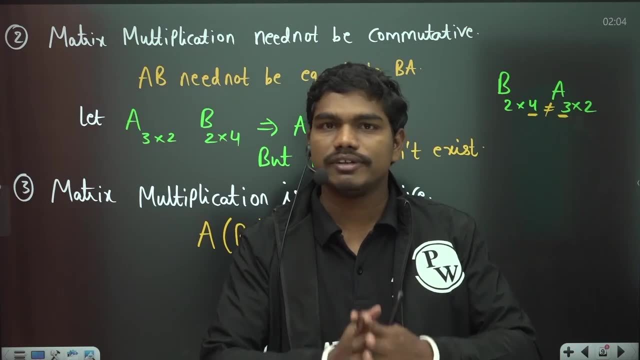 me, uh, when you're going to give the content and all. definitely, i know there's very less time for gate 2023, so, uh, you know we have actually planned that if it's a single short video, so it would be very helpful for you so that a single go some four to five hours. if you spend, you will definitely get. 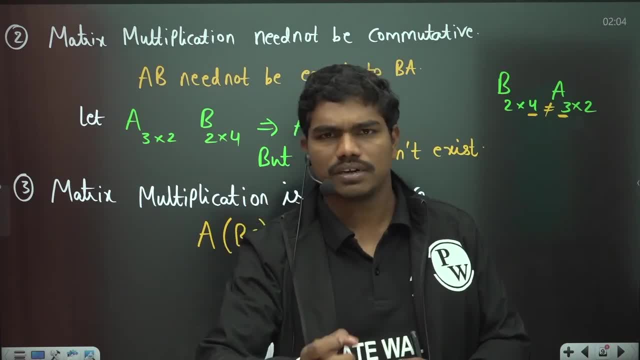 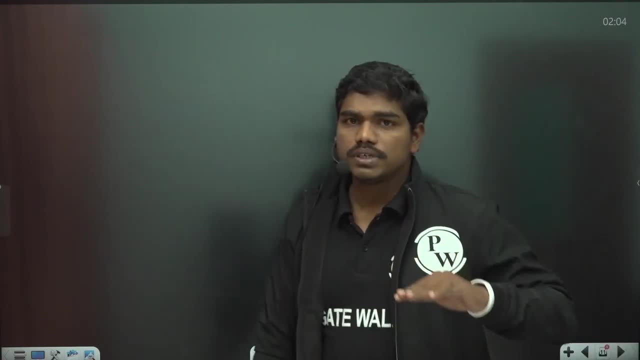 one complete, uh, you know module, some linear algebra, numerical methods, whatever. completely okay, so let's continue now i would like to give you one very important property in real numbers. let us suppose, if you get some expression x into y is equal to 0. you write x is equal to 0 or y is equal. 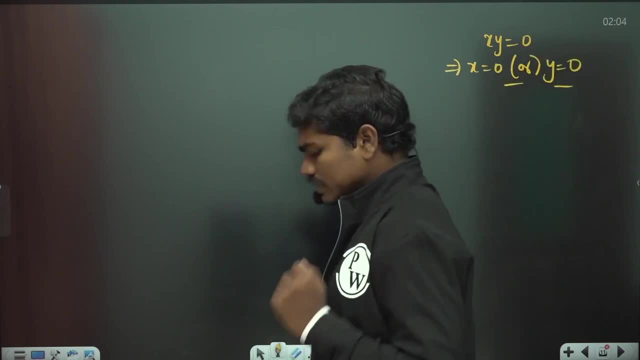 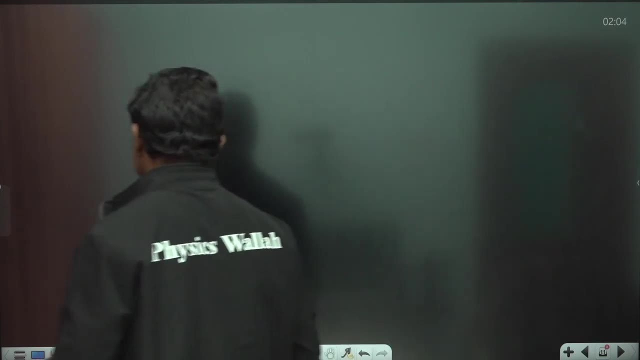 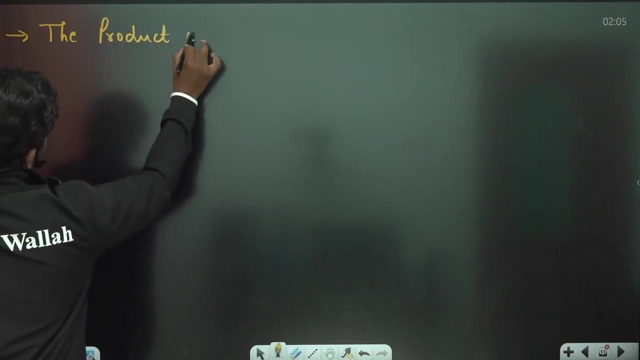 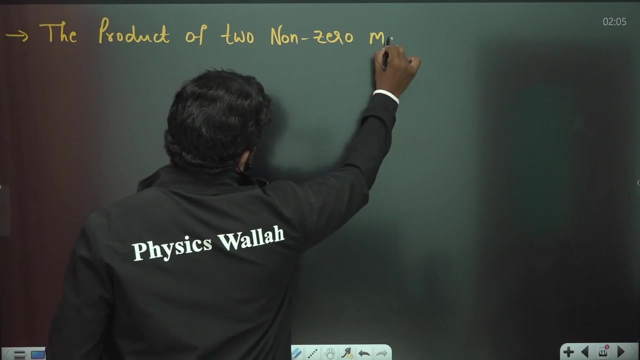 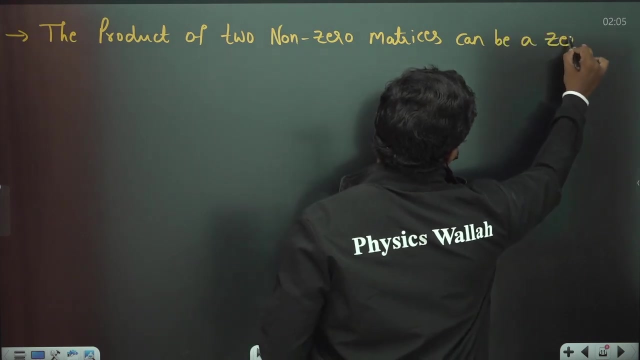 to 0. right, because in numbers you know that for the product to be 0, at least one of them, or maybe both, can be 0, but in case of matrices you can see the product of the product of two non-zero matrices. the product of two non-zero matrices can be a zeomatics. 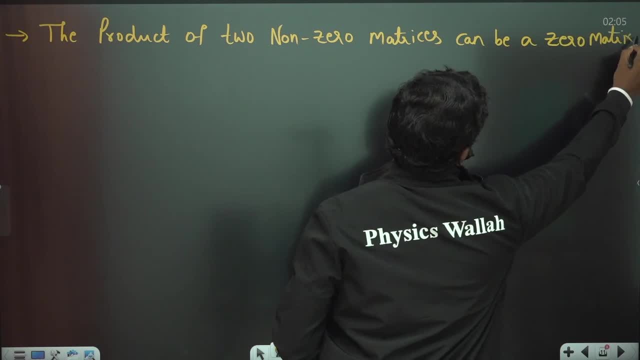 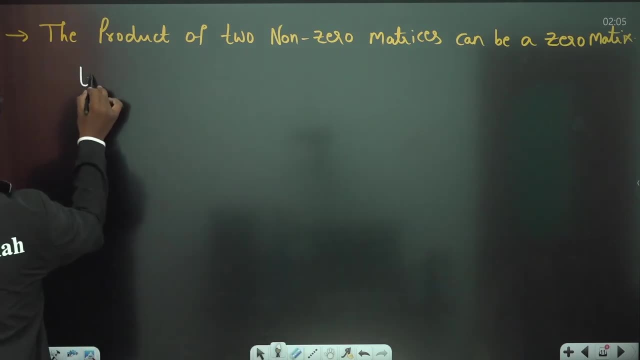 can be a zeomatics. look, this is very strange, correct? i will show you with the help of an example again. you can and understand this. so let: a is equal to some value: a zero, zero, zero. so this matrix is not a zeomatics, because this a small a, what i am taking here. 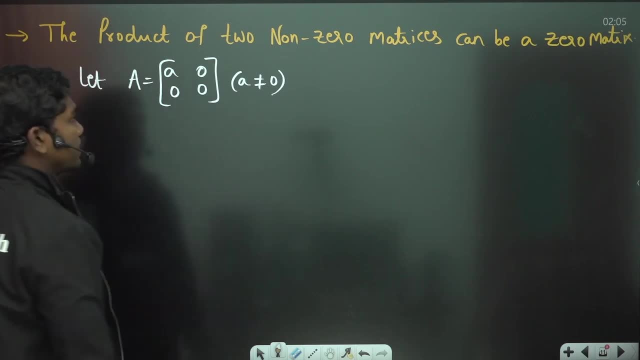 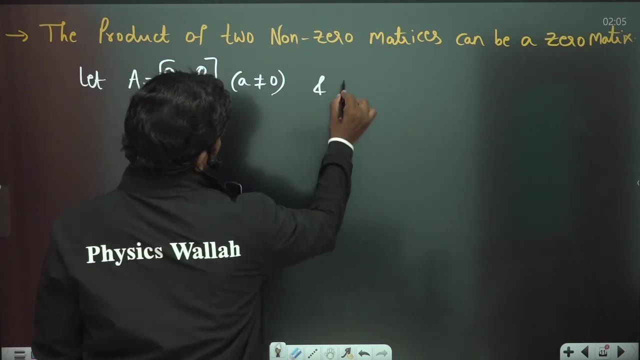 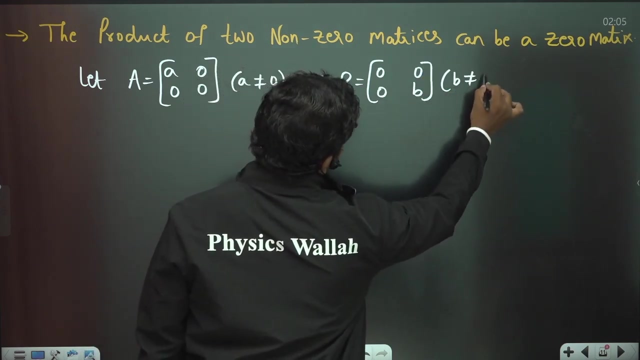 is non-zero, okay, so small a not equal to zero, so definitely this matrix. you cannot call this a zeomatics. basically you cannot call this a null matrix, because this is non-zero and b is equal to zero, zero, zero b and here also b not equal to zero. so here this is also non-zero matrix, correct? 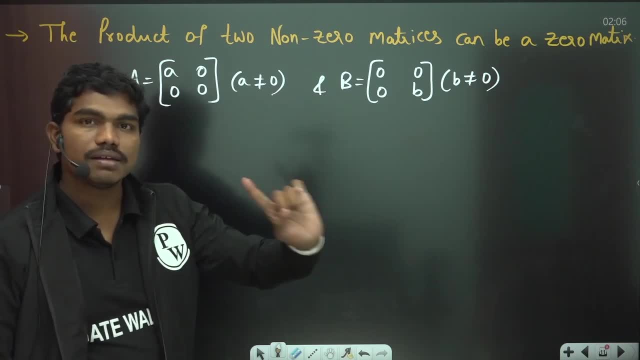 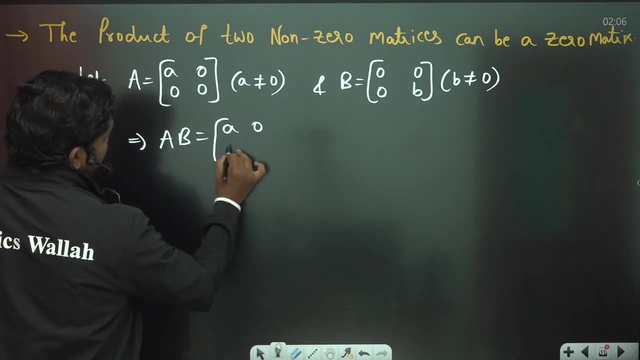 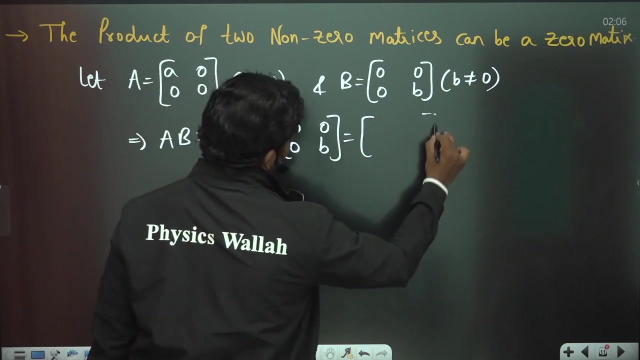 so these two are non-zero matrices because they have at least one element as non-zero. but if you calculate this- a, b, let us see what it turns out: a zero, zero, zero into zero, zero, zero b. so now, if you calculate this, the outcome is going to be: 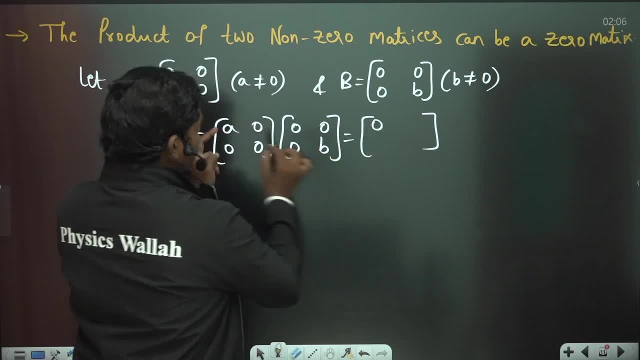 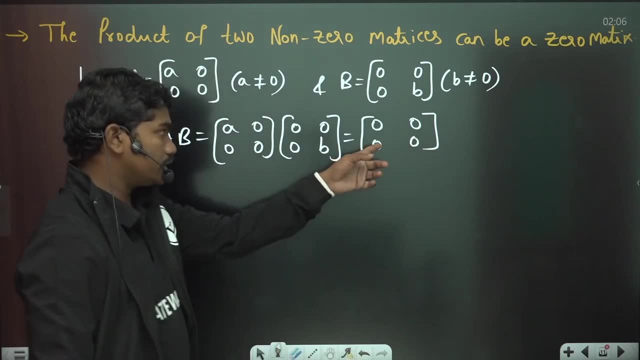 two by two: a into zero plus zero into zero. this is zero. a into zero plus zero into b. this is zero. since these two elements are zeros, definitely these two elements will also be zeros. so, if you see, this is a null matrix. okay, so this is null matrix. so this is a null matrix, so this is null. 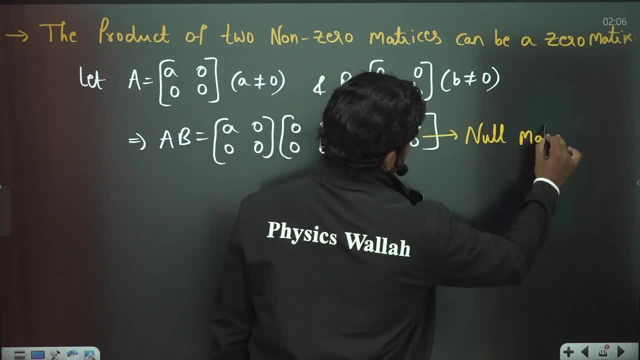 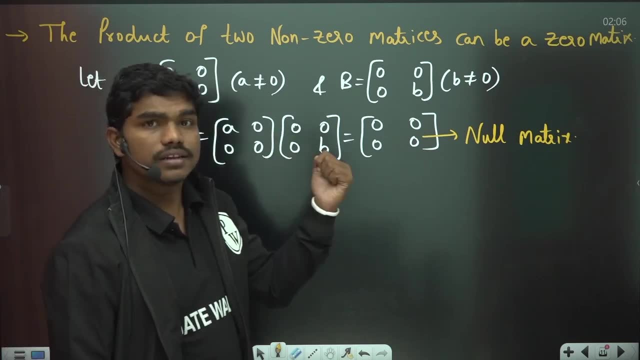 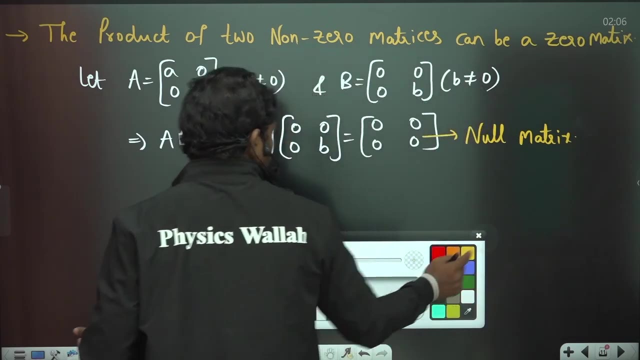 matrix. this is null matrix. so that's how you have seen. clearly these are two non-zero matrices, but still the result is a zero matrix, which generally don't happens in real numbers. so that's why this law, or you can see this, what do you say? this? uh, you know result. you can say: this result is also: 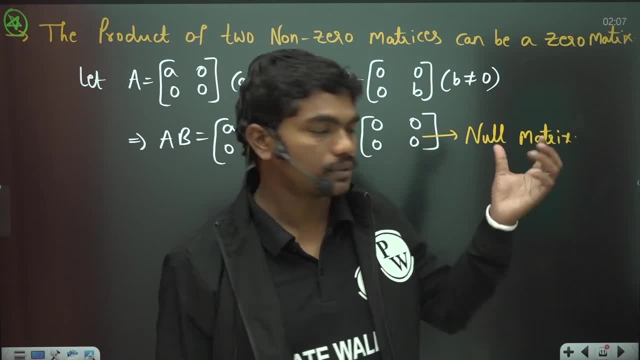 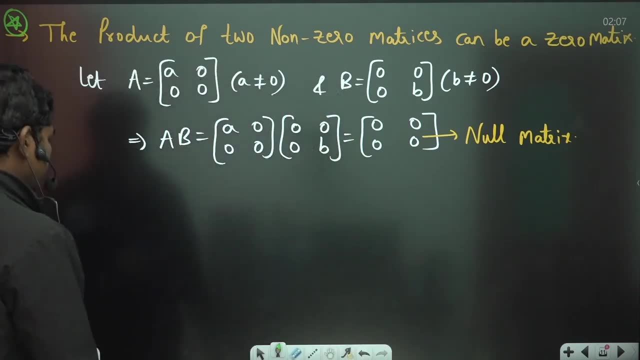 one very important result, because generally you have this intuition that for the product to be zero, at least one of them should be zero. but in matrices you did not have that clear. now let us continue the types of matrices. or, before continuing, i would like to give you: 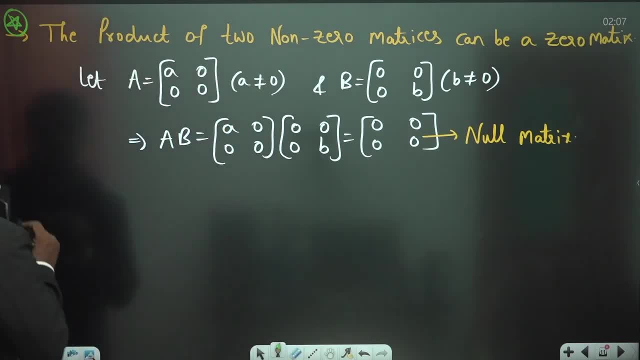 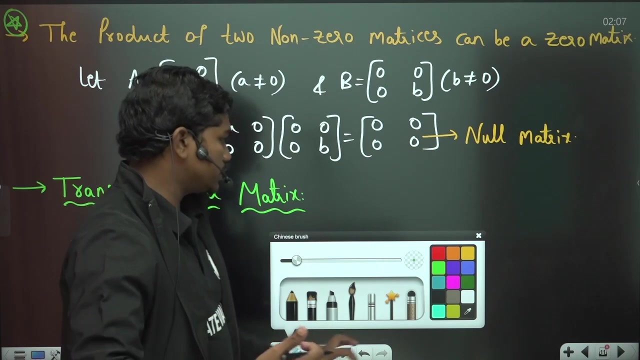 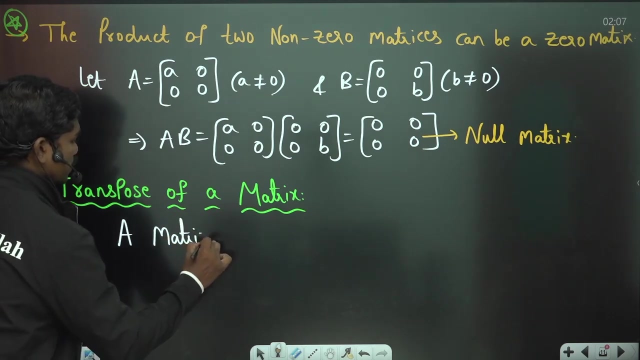 one more point: okay, so transpose of a matrix. this is one very important thing: transpose of a matrix, so transpose of a matrix. so what is transpose of a matrix, so transpose? what's the meaning of this? basically, reflection. okay, so if you interchange, you need to actually interchange them. So a matrix b is equal to bij, for all. 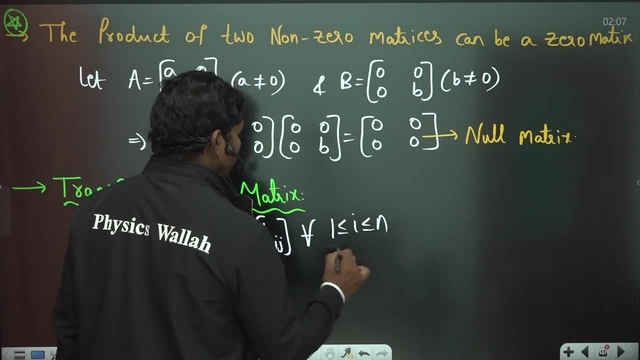 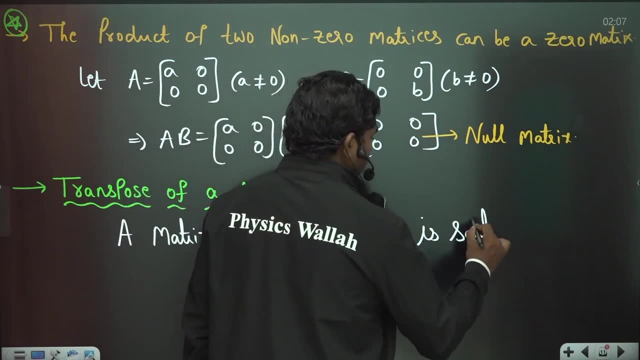 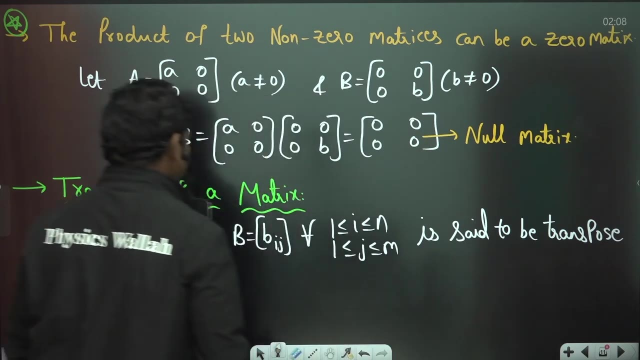 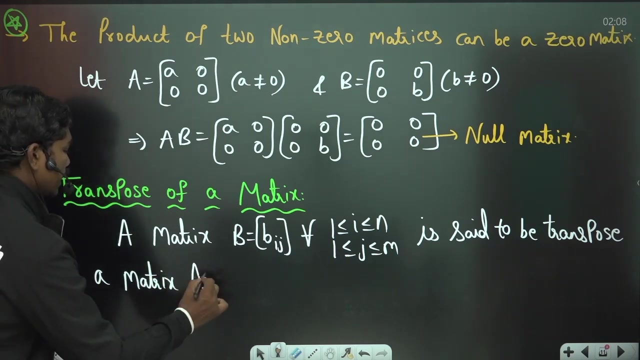 1 less than or equal to i, less than or equal to n, and 1 less than or equal to j, less than or equal to m, is said to be. is said to be. transpose of a matrix. is said to be: transpose of a matrix, transpose of a matrix. capital A is equal to aij, for all. 1 less than or equal to i, less than or. 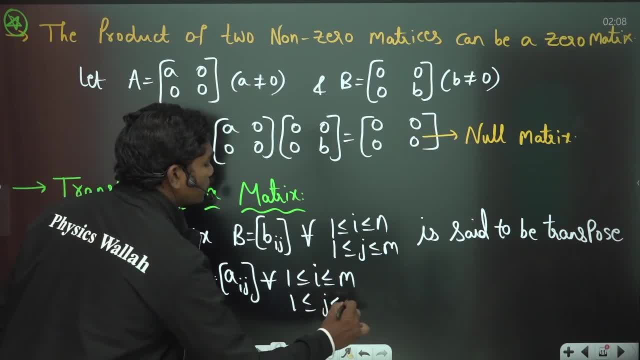 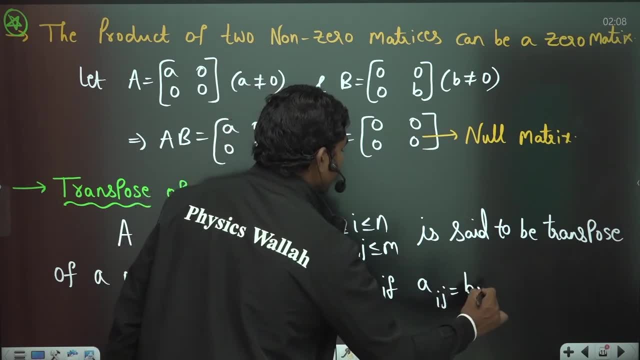 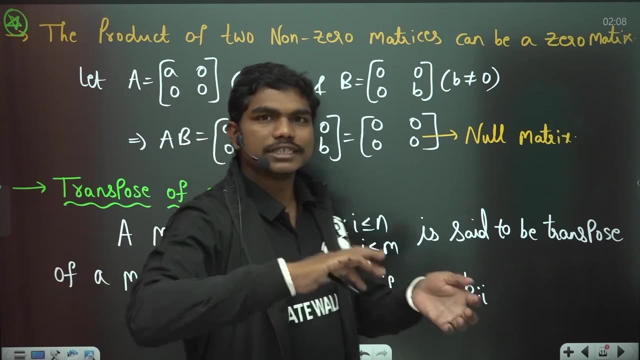 equal to m and 1 less than or equal to j, less than or equal to n, If aij is equal to bji, bji. So this is how you define transpose of a matrix and normally in simple terms. you know, if you interchange rows and columns, then definitely you will get the 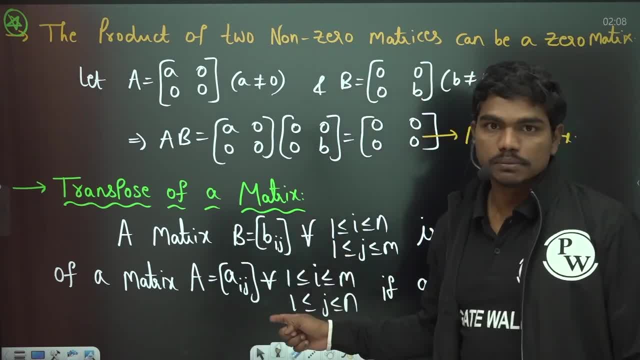 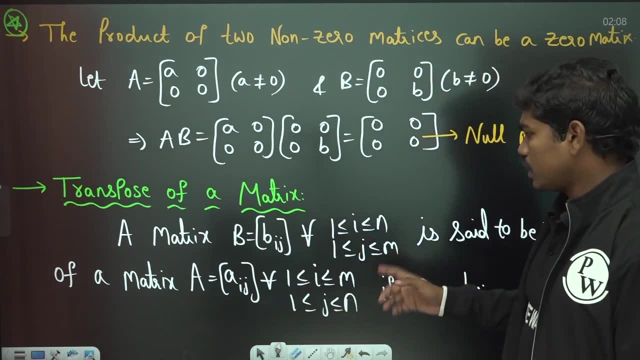 transpose of the given matrix correct. Now why this definition is very important? because, if you see, very soon after the single shot videos will come up with a problem solving. you know series basically. So now, if you see why this, definitely in that, in that, basically in that. 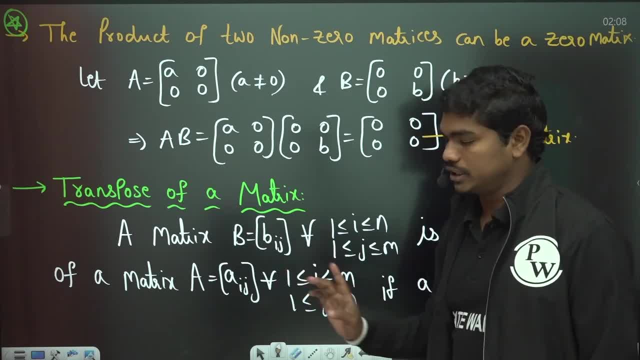 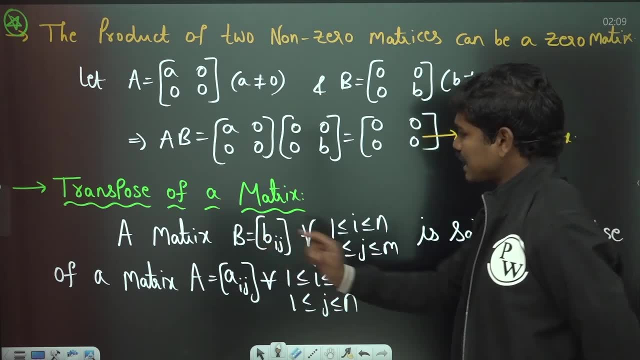 you'll see a lot of questions. that transpose is given in these notations, Okay. So now, if you see what is the meaning of this, let us try to understand. First of all, you need to understand one thing: This matrix, capital B is of size n by m. It's not m by n, It's n by m because row numbers: 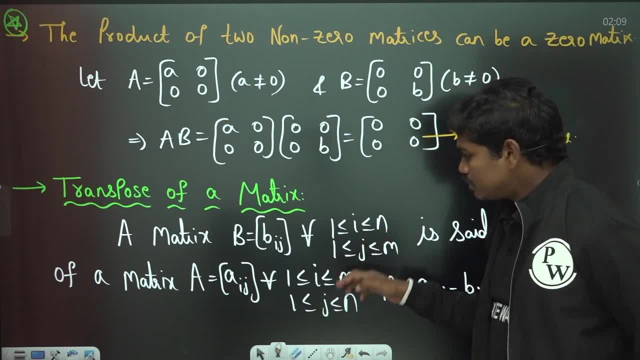 can go from 1 to n and column numbers can go from 1 to m. Similarly, this matrix here, which is the initial matrix, it has m by n order. So definitely you know one thing when you have a matrix of order. 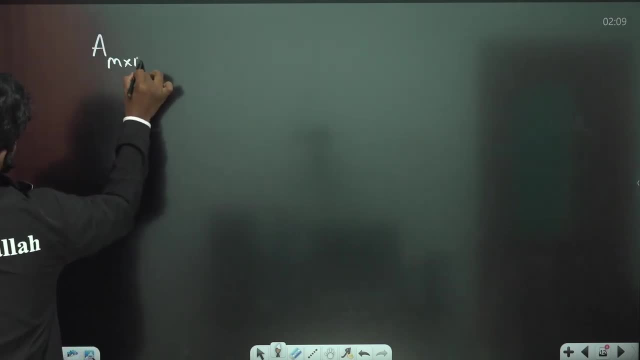 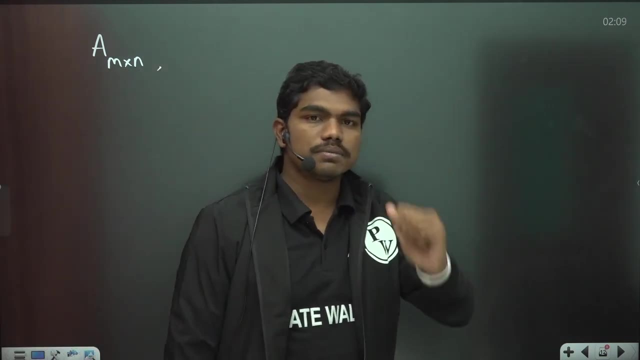 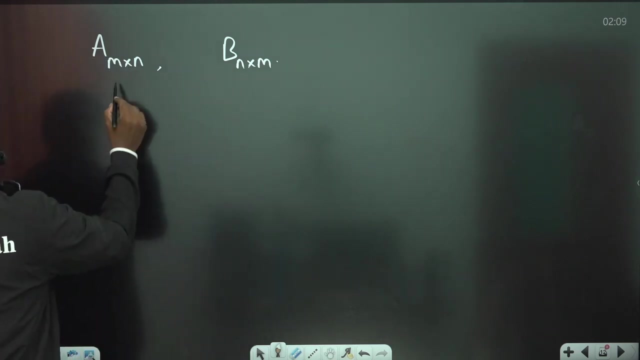 m by n. when you have a matrix of order m by n, then if you interchange rows and columns, then the number of rows will become number of columns and the number of columns becomes number of rows. So this matrix B will be of this size, n by m, correct? For example? let us take some simple values: 2 and. 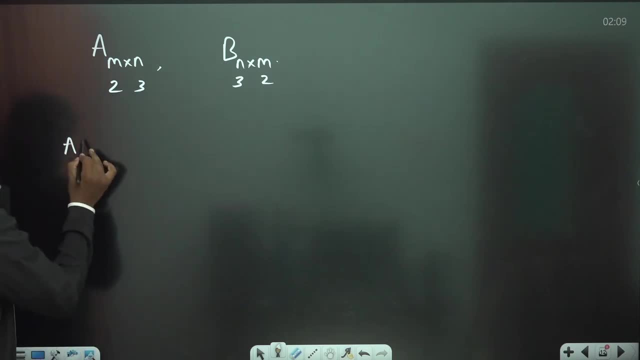 3. Let us take, then this becomes 3 by 2.. For example, let me take one matrix. If I take this matrix, 2 by 3. So 1, 2,, 3,, 4, 5,, 6. Then you know, if you want to call this B matrix, then you. 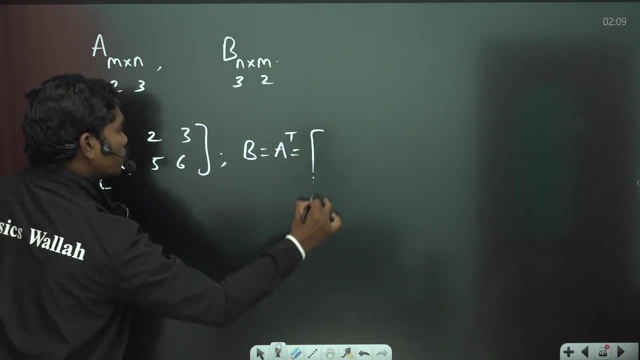 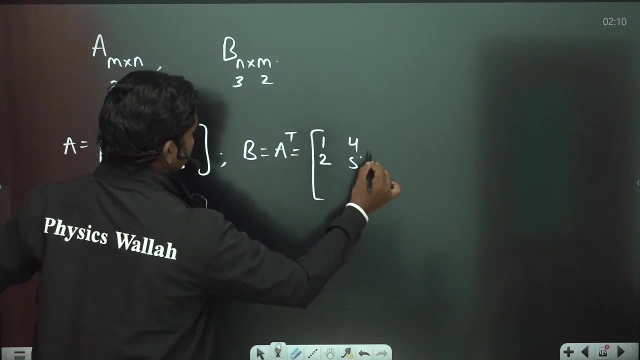 can call B as A transpose which is generated by this. So then you know you need to interchange rows and columns, So this first column can be interchanged as the first row, then second row and third row. So now, if you see, this is of size 3 by 2, because this is of size 2 by 3.. It's quite. 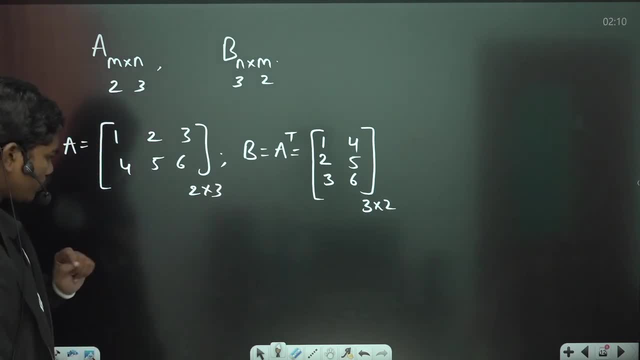 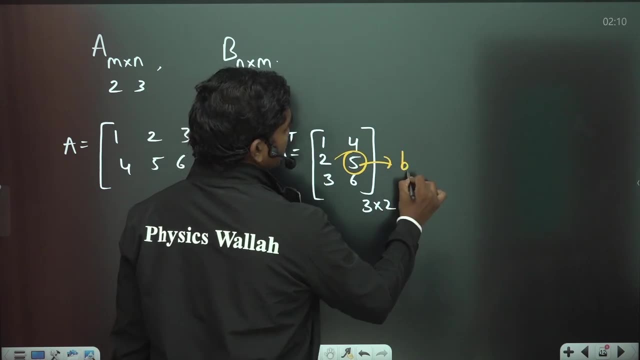 off. Yes, correct. Now what is the meaning of this matrix? Look, if I take B ij means if I take, for example, B 2 3 or B 2 2, element B 2 2, then definitely this is going to be of size 2 by 3.. 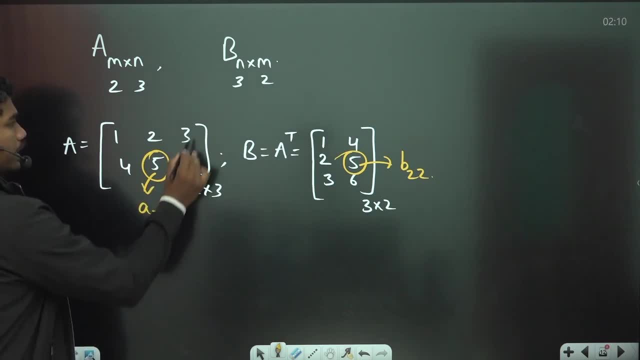 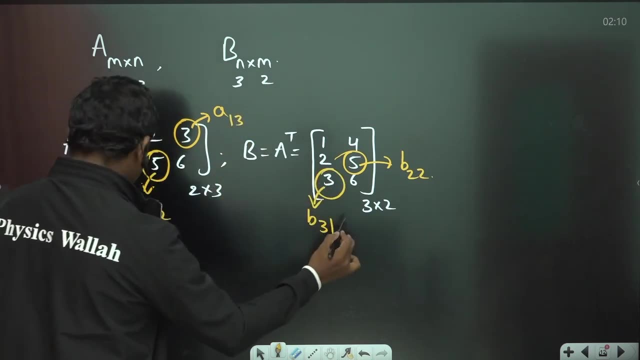 It's going to be same as A 2- 2.. Or if I take A 1- 3, then definitely it is going to be B 3- 1.. So that's why I told you that A ij is equal to B ji. Means, if you are taking 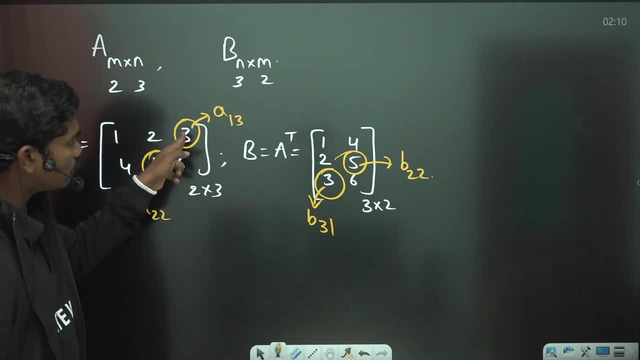 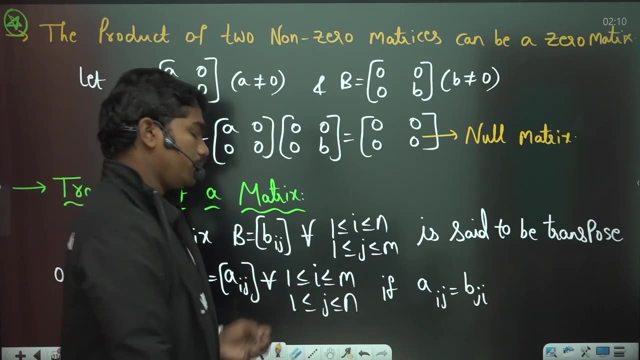 second row. second, or you can say first or third column element. in B you should take third or first column element, Okay, So these two will be equal. That's what I have defined in slightly complex terms, because this is generally important for get examination. Okay, And you can write one. 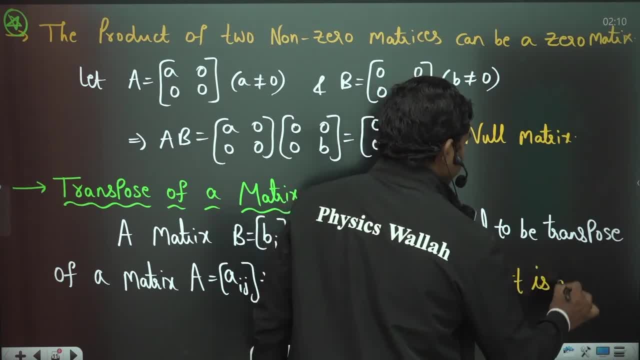 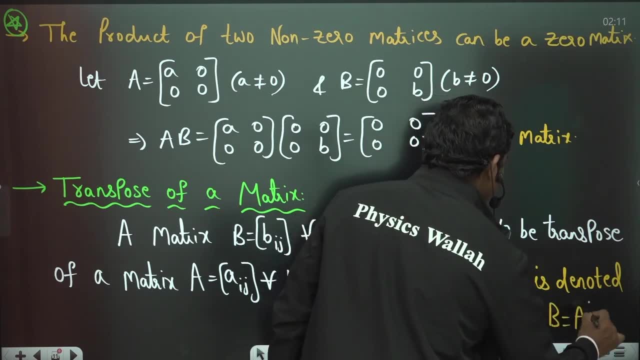 more statement. It is denoted as it is denoted as it is denoted. as B is equal to A, transpose T on the superscript of T of A, basically here. Okay, So that's why I hope you understood this. 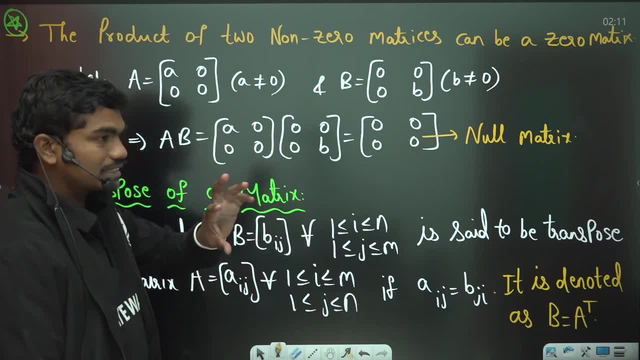 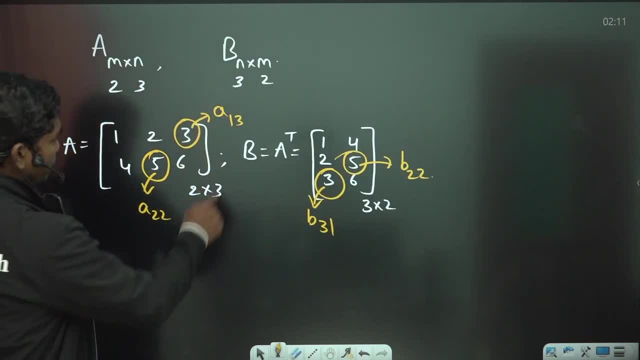 I am repeating: Whenever you are making a transpose, the order of the matrix gets interchanged Means. basically, if this is of size m by n, then this becomes of size n by m. as you have seen, And obviously, if you find out element A, ij, this element will be same as 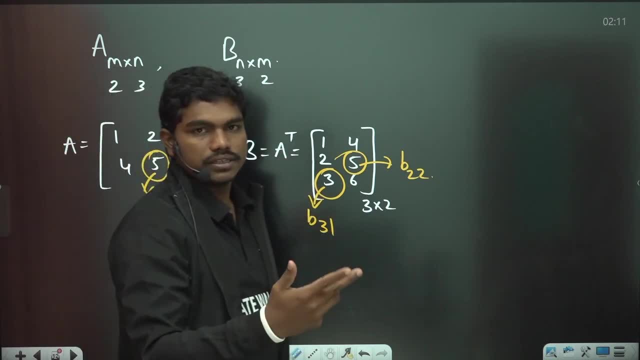 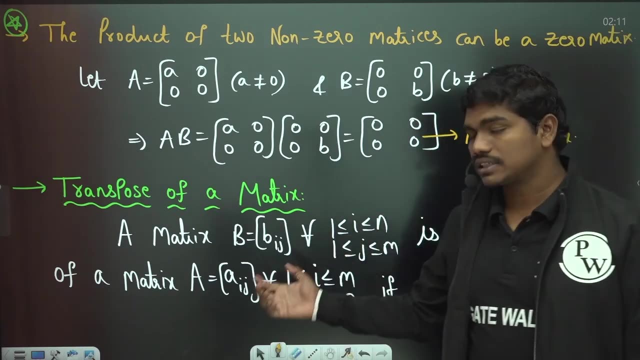 B ji, with the order and row number reversed because you have interchanged the matrices. That's the reason And this is how you actually define the transpose of a matrix. And this is very, you know, interesting thing, because transpose means basically rows become columns. 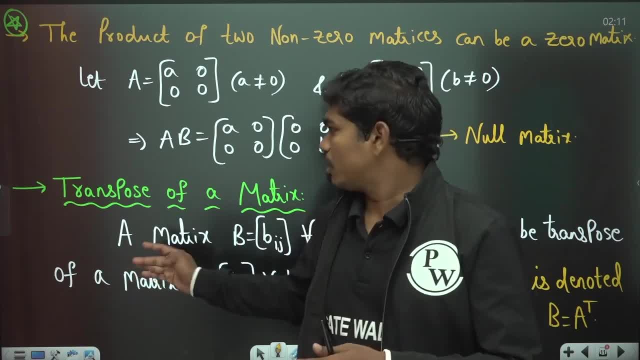 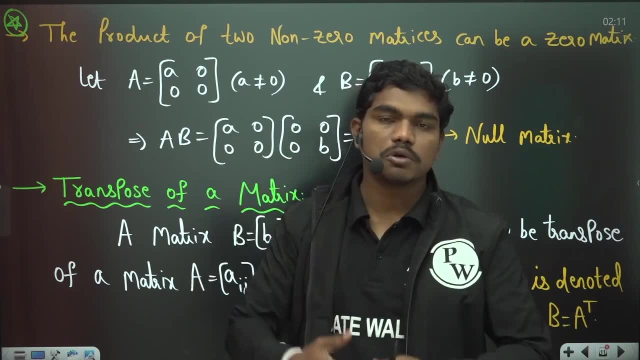 and columns become rows. Normally, if you see the meaning of transpose this, if you have any matrix and if you do transpose of it, the points will actually come as a reflection about the line y equal to x, basically Okay. So, for example, if you have one, two matrix, then if you transpose. 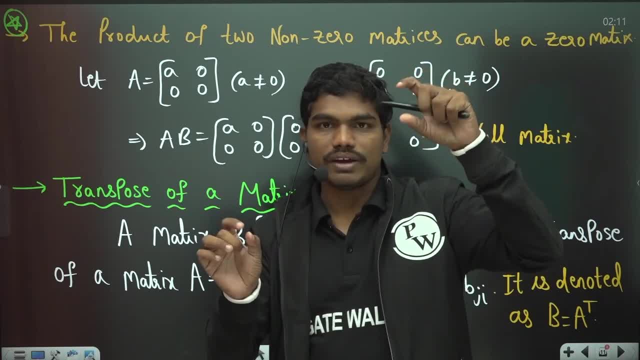 it becomes 2, 1.. And that point- 1 comma 2 and 2 comma 1, if you take these two points, they are nothing but the reflection of each other. about the line: y is equal to x generally, Okay, So. 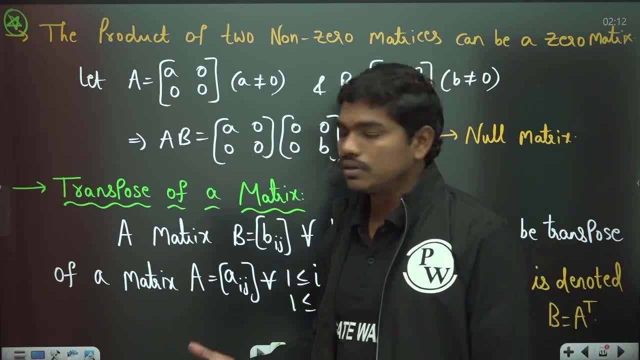 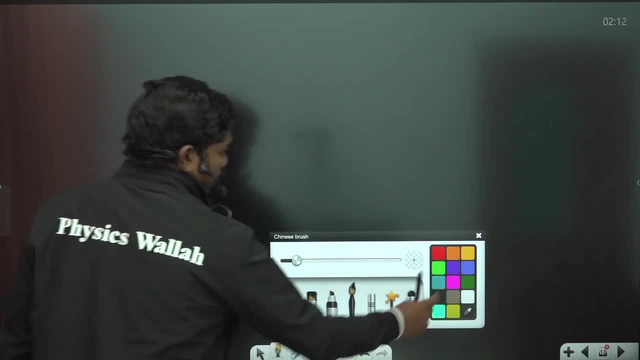 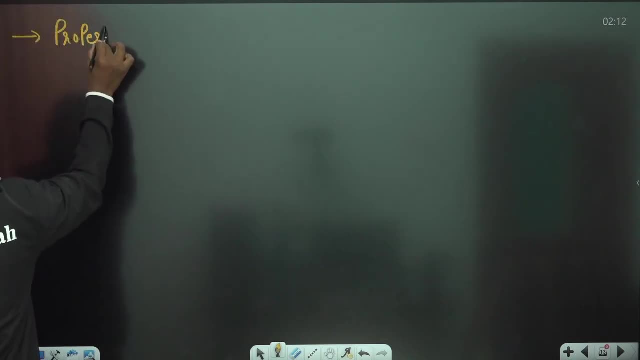 that's why you know this transpose is one very important. you know operation in matrices. Now, if you see properties of transpose, I would like to give some properties of transpose, Properties of transpose, Properties of transpose. Okay, So now the first property. Let us suppose if you transpose any matrix, even 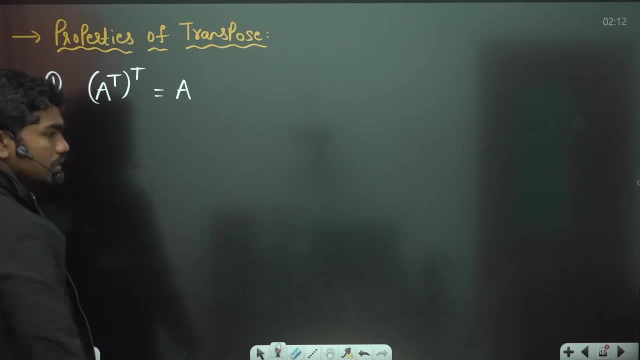 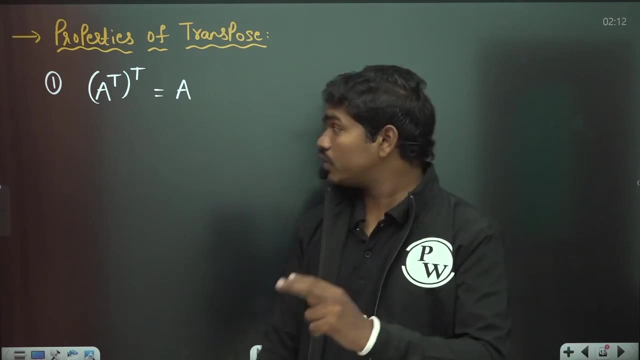 number of times, for example, then you will get the same matrix Correct. Let us suppose if you transpose once, Okay, Then you will get the transpose of that matrix. Now let us suppose if you transpose it again means if you apply the transpose two times, then what happens First time? 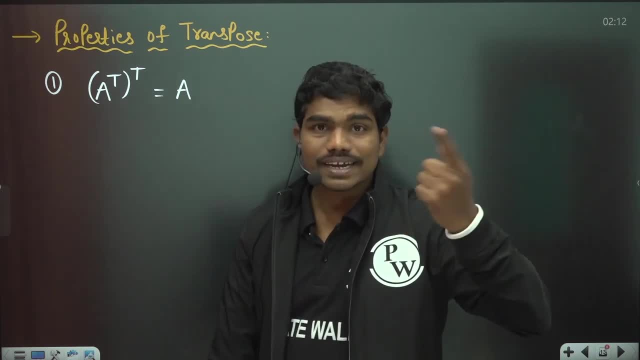 when you do the transpose, you will get the interchanged matrix. So you will get the transpose of the rows and columns, But second time, when you are interchanging again, you will again get the original matrix. Okay, So even number of transformations give you the same matrix. Odd. 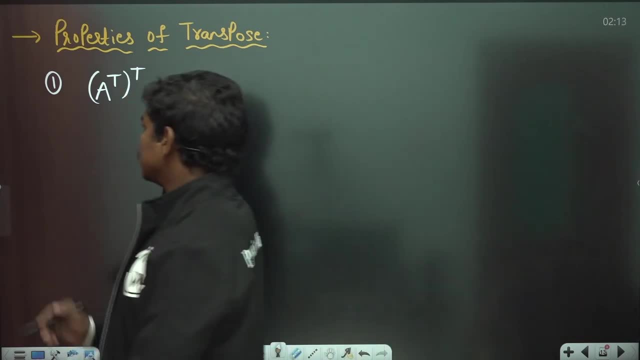 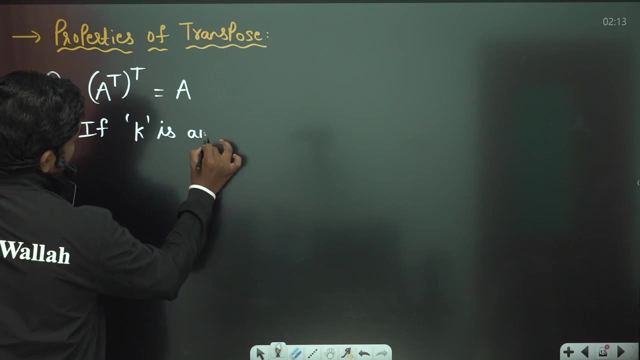 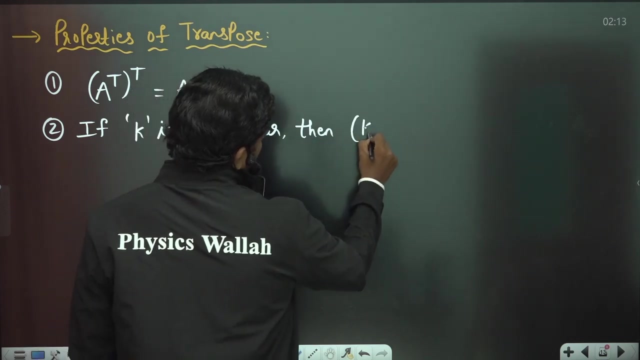 number of transformations. give you the, you know the transpose matrix, Okay. So second, if k is any scalar, if k is any scalar, scalar means some number, Okay, Some constant. If k is any scalar, then k a whole transpose is actually equal to k times of a times. 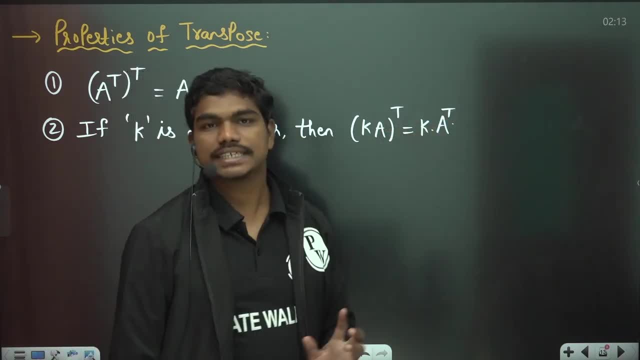 So this result is again very important, because you can never transpose any scalar, Okay. So, for example, if you see 2a, for example, if I take this matrix, a is equal to 1,, 2,, 3, 4.. Simply, I am. 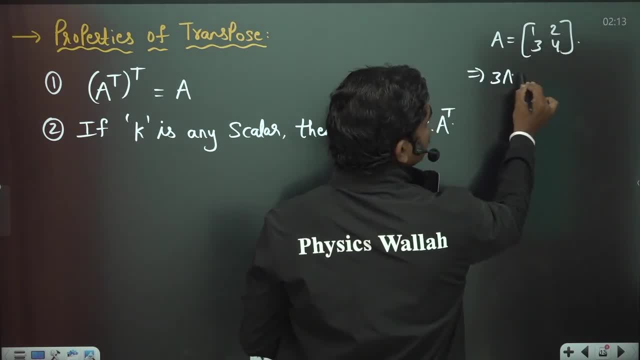 just denoting it. So this implies if I calculate 3 times of a, I need to multiply 3 to all the elements. So if I do the 3a whole transpose, 3a whole transpose, this gives me 3,, 9,, 6,, 12.. 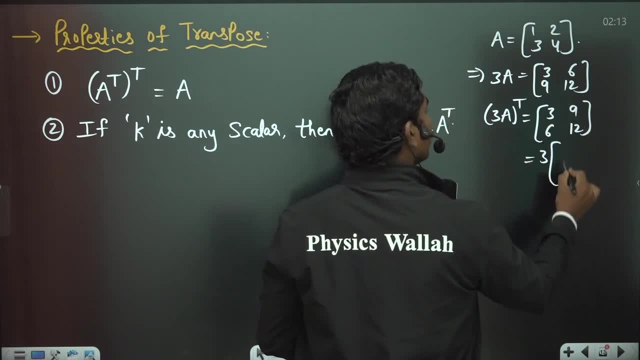 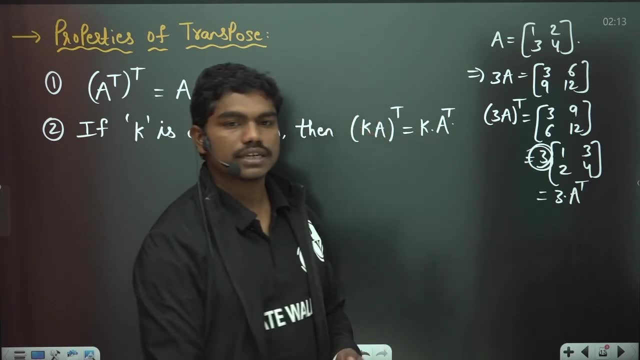 Correct. So this matrix is nothing but 3 times of 1,, 3,, 2,, 4.. And this is 3 into this is a transpose. But scalars, these scalars, they never undergo any transformation, basically Okay, So that is what we have here. Then, third, you can see some a plus. 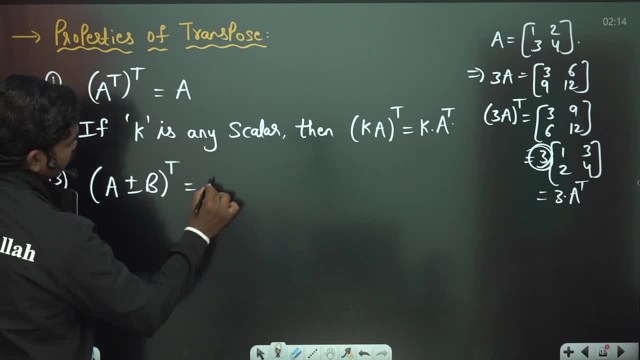 or minus b whole transpose. If we have this, then this is equal to a transpose plus or minus b transpose Means. basically, if you take plus here, here also it is plus. If you take minus here this is also minus. You can check all this with simple examples And one very important property. 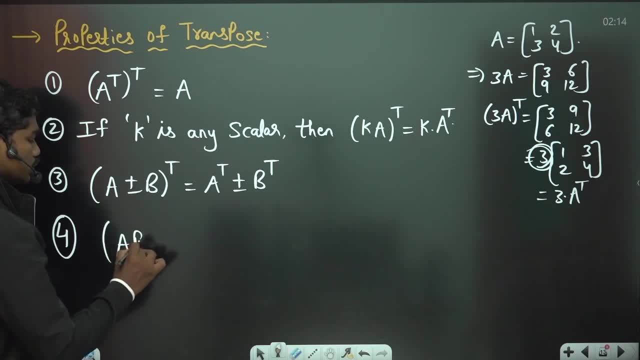 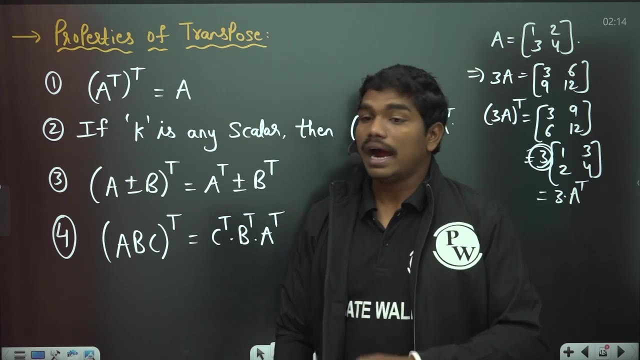 that I am going to give you now is a, b, b, whole transpose, or you can write c also whole transpose is equal to c transpose, b transpose into a transpose. So all these are basically some nice results of addition, multiplication of transposes of matrices, Okay, And this result is very important For the resultLS. 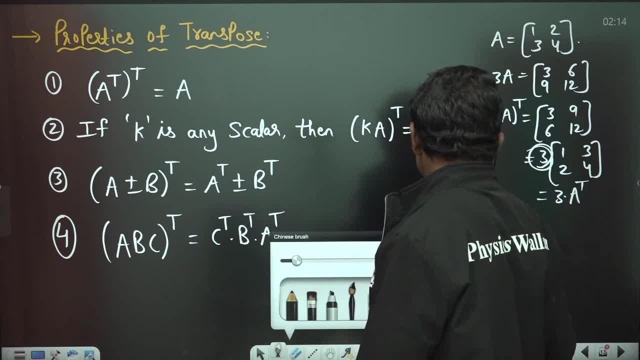 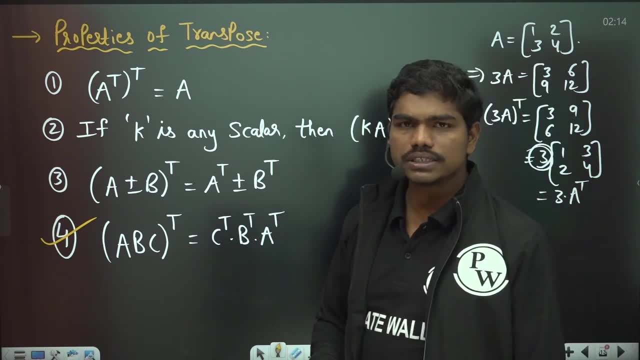 specially we will use after some time in this lecture. So now, if you see, this fourth one is a very much good property of matrices actually. and anyhow, these are the four important properties that generally sometimes they ask you in examination. 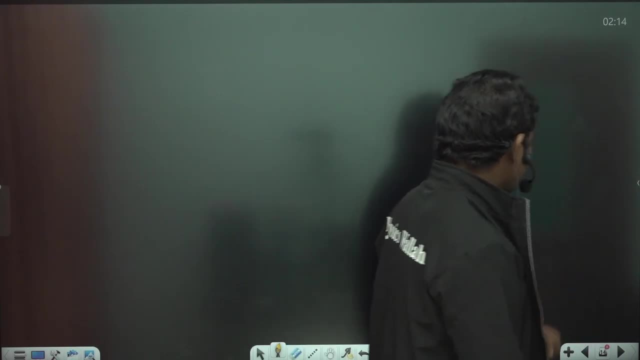 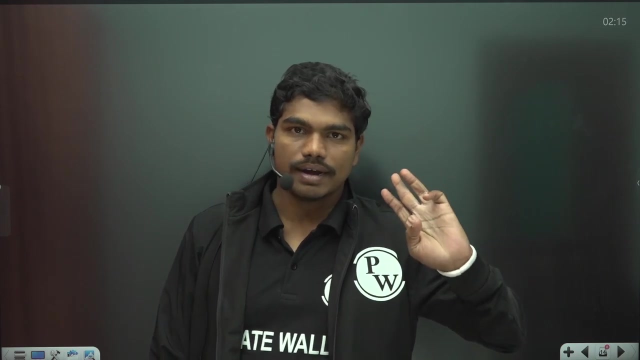 and also in, you know, general university exams. Now, coming to the continuing to the types of matrices, we have defined three types of matrices. What are they? Lower triangular, upper triangular and also diagonal matrix, correct, So let us continue. 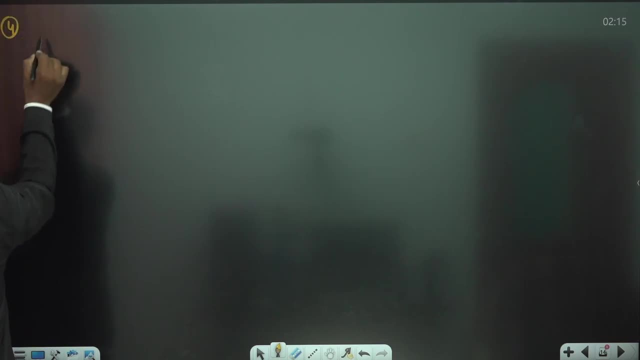 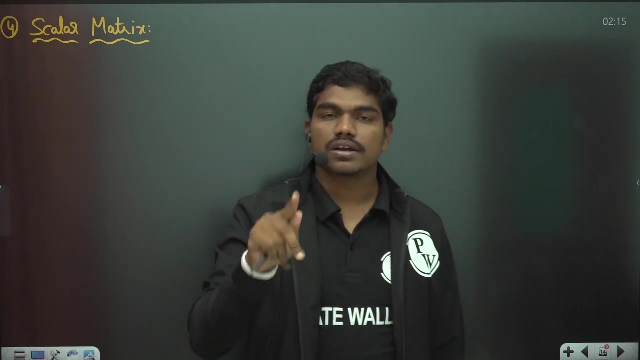 So again, fourth, if you see, we'll define something called scalar matrix, Scalar matrix. So, in simple terms, if I want to explain you what is a scalar matrix, It's basically a diagonal matrix, but this time all the diagonal elements are equal. 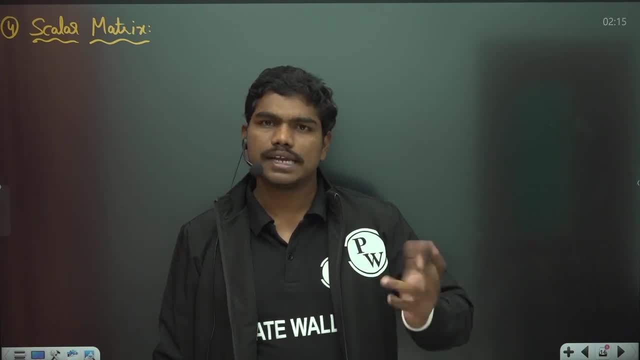 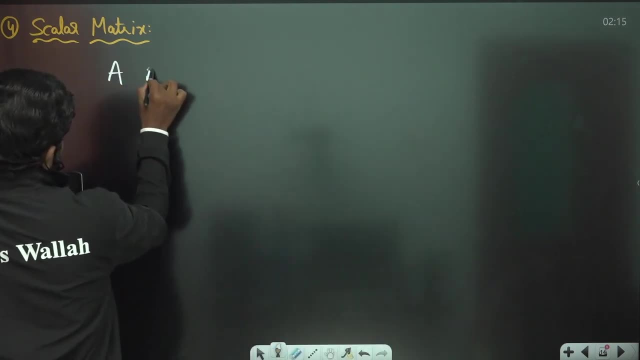 Like, for example- you see the case of identity matrix- all the diagonal elements are equal. okay, So that's how this scalar matrix is basically done. So a matrix A is equal to a matrix A is equal to Aij, for all one less than or equal to. 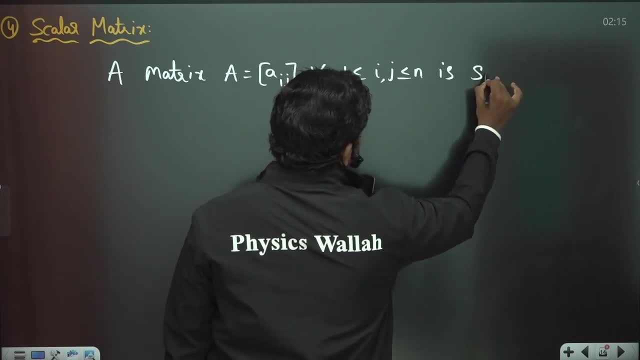 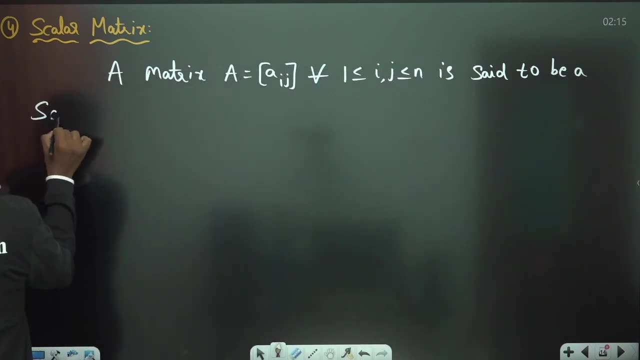 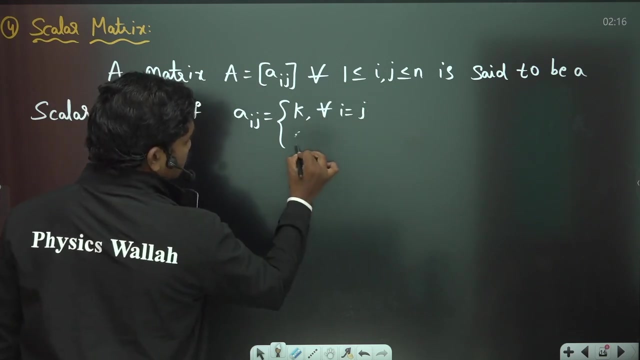 i comma, j less than or equal to n and the matrix A is said to be a scalar matrix is said to be a scalar matrix if Aij is equal to some constant. k for all i is equal to j and a zero for all i not equal to j. 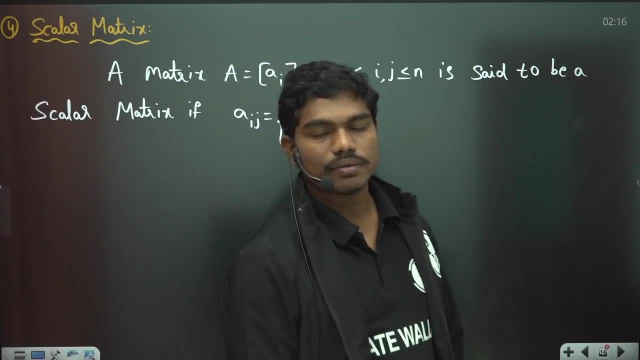 So you can see, this time this Aij is given as some function of i comma j, but Aij is given as some function of i comma j whenever i is equal to j means if element is lying on the principal diagonal then it should have some. 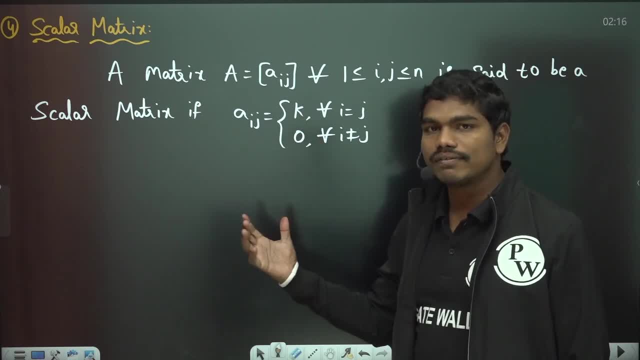 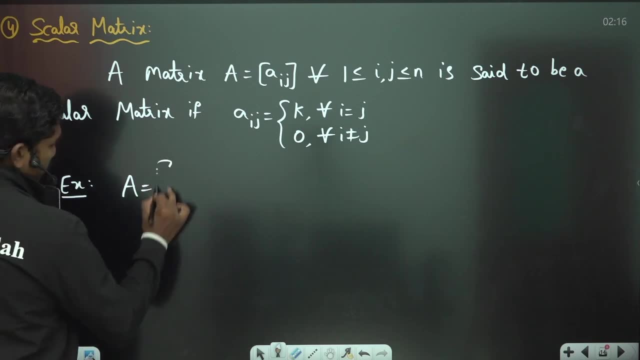 fixed value. but when elements are non-diagonal elements, then definitely they are zeros and you can see. this is something like this example: if i take 3 by 3, then you can see k 0, 0, 0, k 0 and 0, 0 k. so this is how you can get a scalar matrix, basically all the principal diagonal. 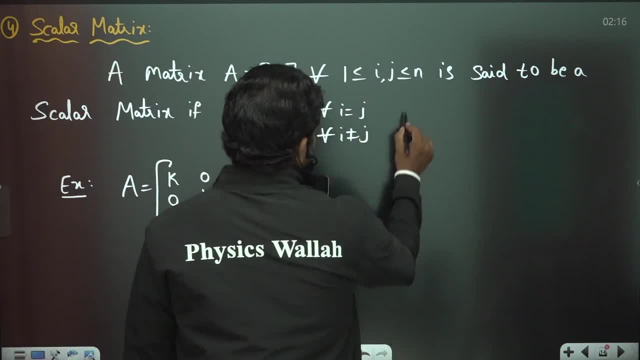 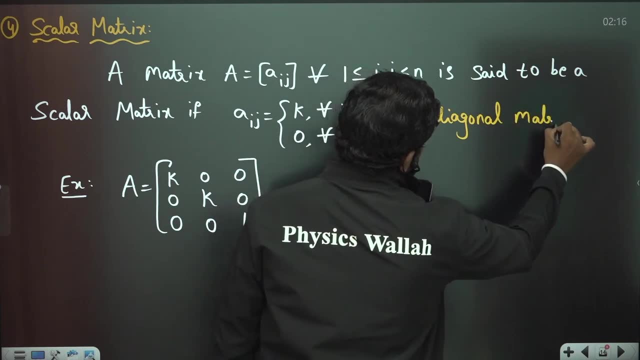 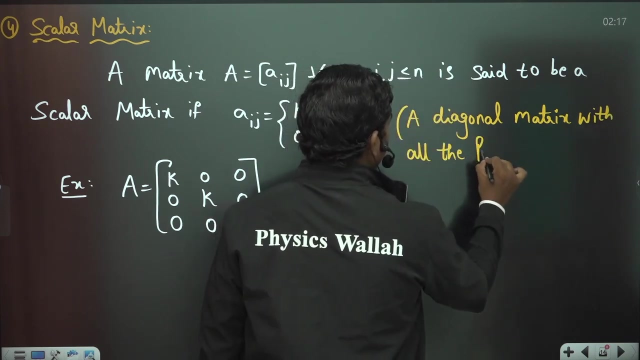 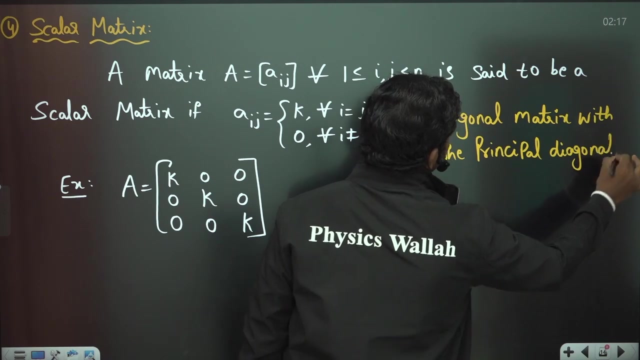 elements are same. you can write here a diagonal matrix, a diagonal matrix, a diagonal matrix with all the principal diagonal elements, with all the principal diagonal elements, with all the principal diagonal elements being same, with all the principal diagonal elements being same actually here. okay, so now, if you see, 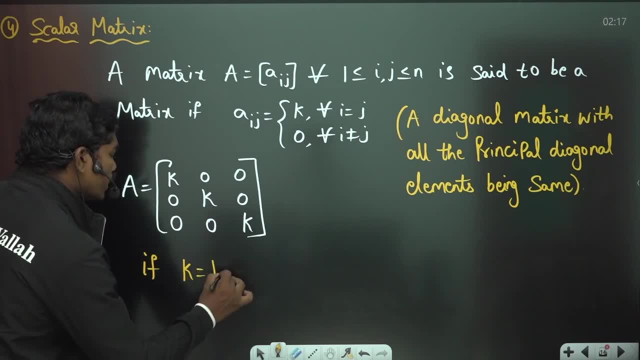 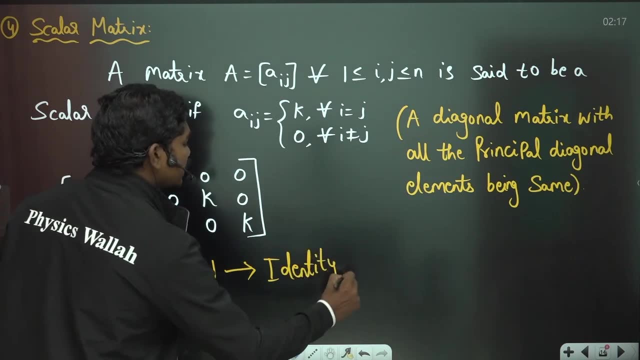 if you can understand one thing carefully: if k is equal to 1, then this matrix is called identity matrix. okay, because you know in identity matrix you have the principal diagonal elements 1 and all other elements zeros. so when k is equal to 1- because this can be any constant- 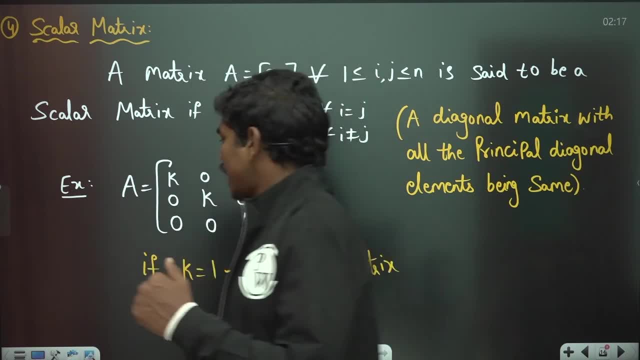 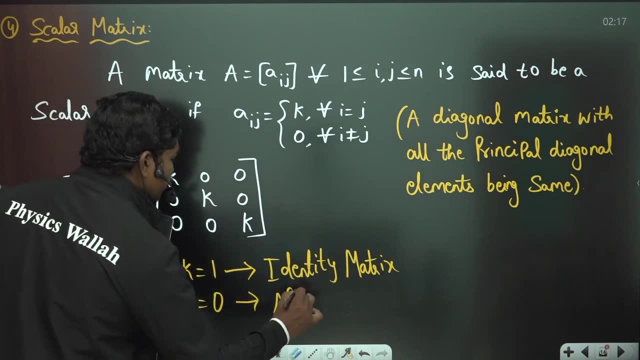 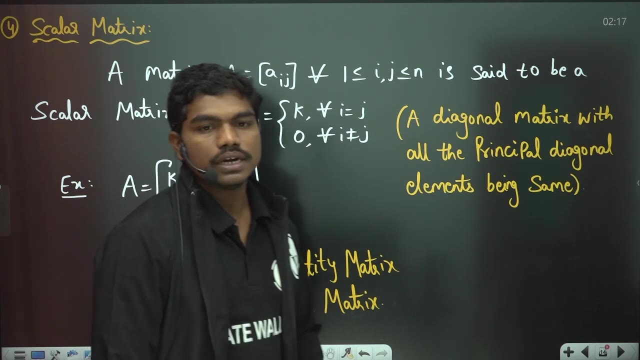 so when k is equal to 1, this matrix is called identity matrix, and if k is equal to 0, if k is equal to 0, this is called null matrix. null matrix, okay, so this k is equal to 0, this gives you null matrix actually here. okay, so these are two special cases of this scalar matrix. so 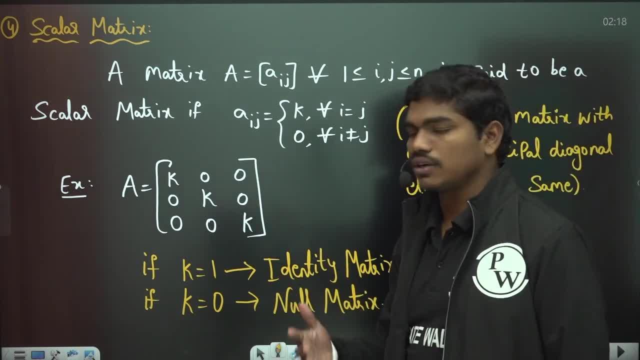 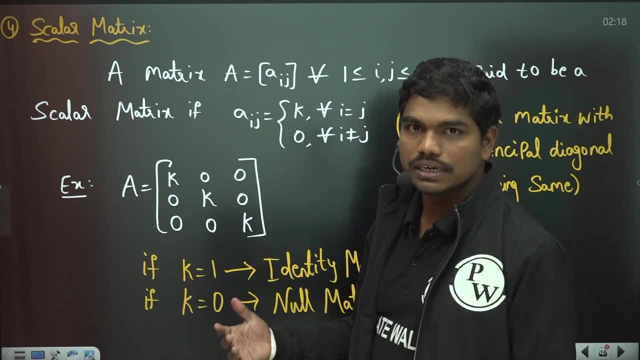 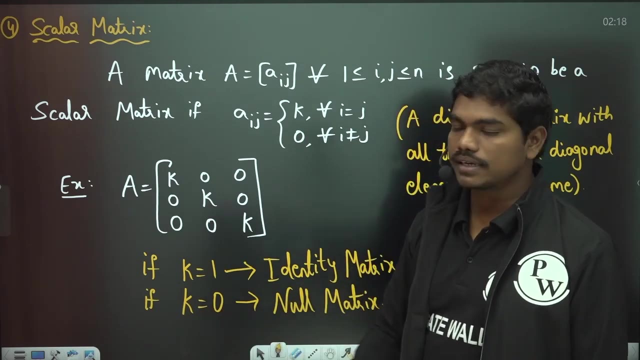 basically, you deal with identity matrix everywhere. when you talk about inverse of the matrix, orthogonal, all these cases, and null matrix is again the common. you know what do you say? additive law means basically, if you see, additive identity matrix is basically this: k means if you add any matrix to this matrix, null matrix, you'll again get the same matrix. okay, so this. 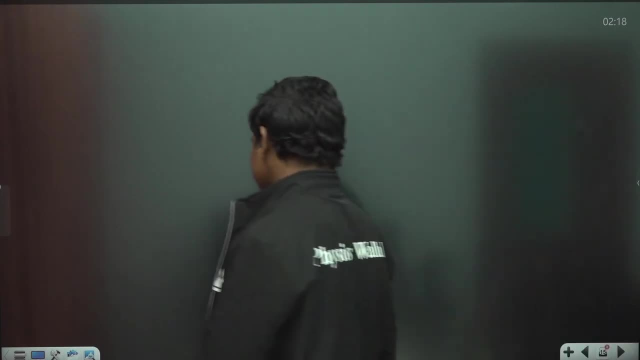 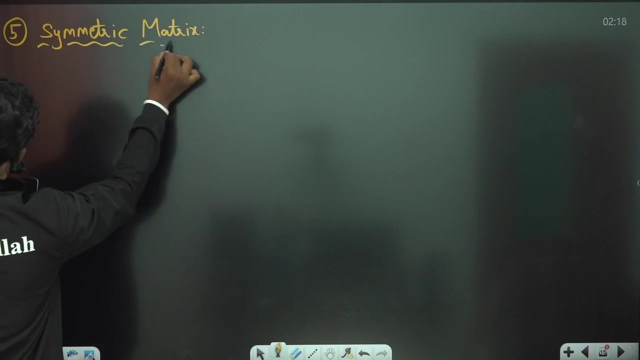 is scalar matrix. now i'll go for one very important matrix, which is called symmetric matrix. symmetric matrix: you can tell by the name itself. the matrix is symmetric about its principle diagonal. so now you see what is a symmetric matrix. okay, so in simple terms, you know a is. 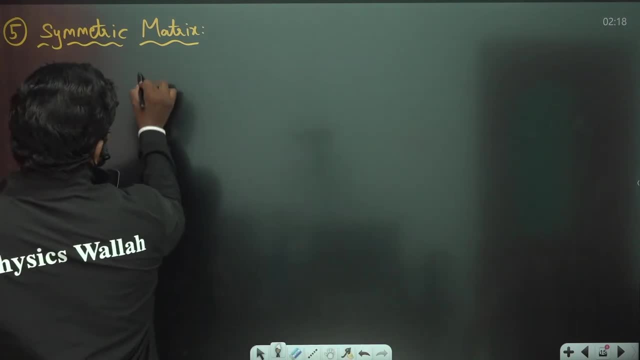 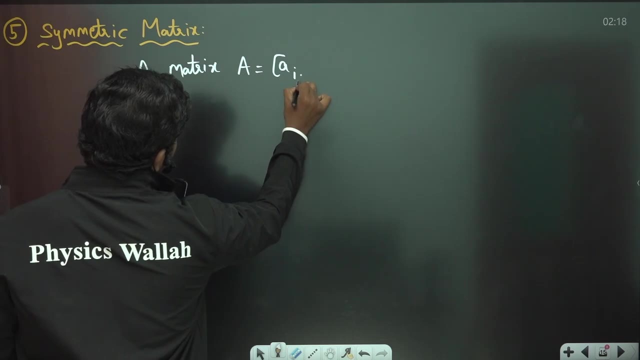 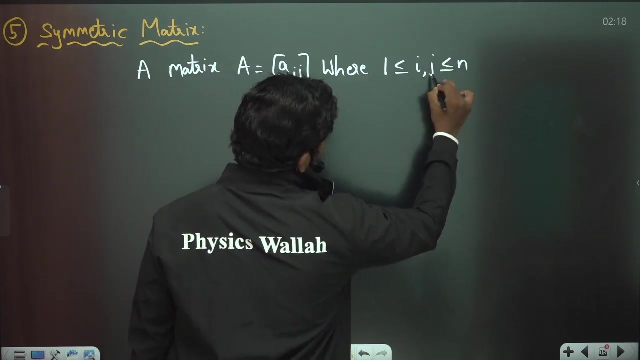 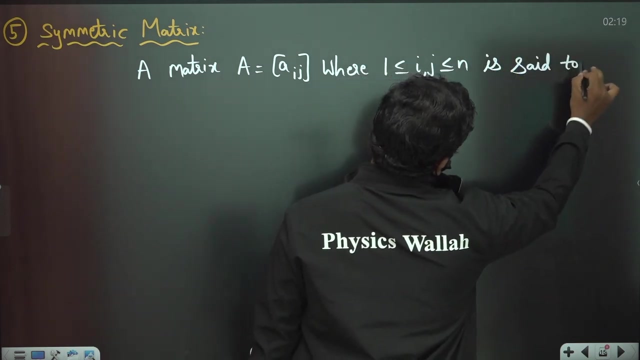 equal to a. transpose. let us write it in terms of ij notations: a matrix. a matrix a is equal to a ij, where 1 less than or equal to i comma j less than or equal to n. i comma j less than or equal to n is said to be symmetric. 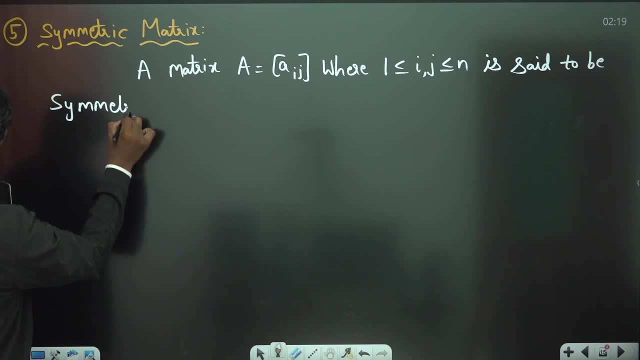 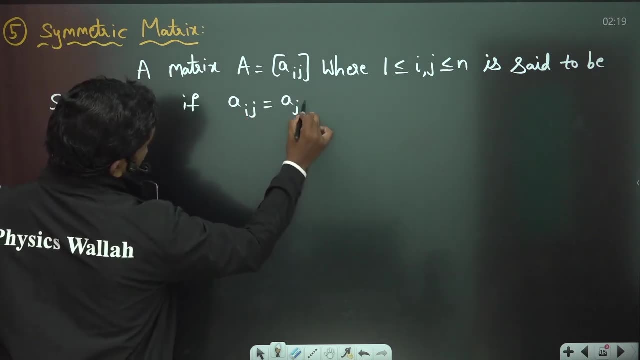 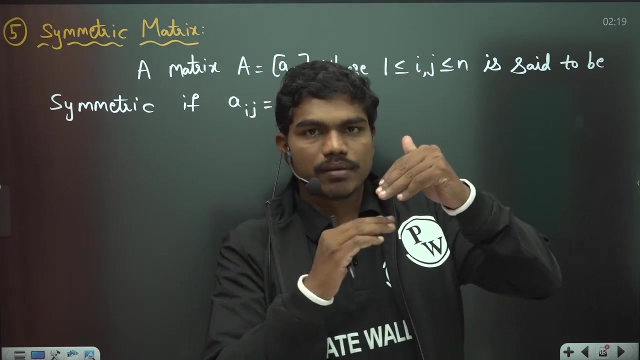 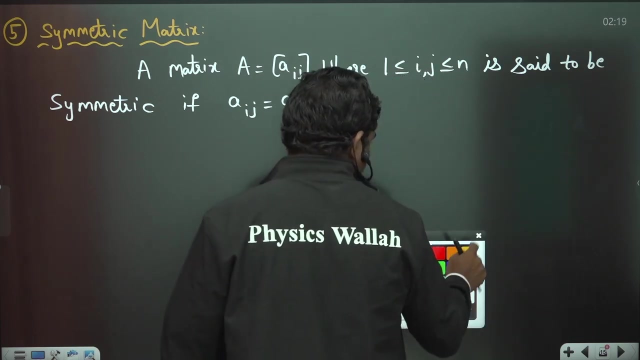 is said to be symmetric if aij is equal to aji means. what does this mean actually here? if you see this, aij is equal to aji means if you take any element symmetric about the- you know, basically symmetric about the principle diagonal, then the elements values are same, okay. so example i would 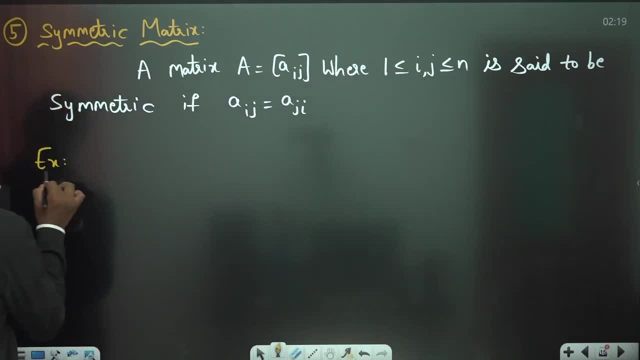 like to give you example. a is equal to, for example, you can write two, three, four, then this is also three, four, five, six, then this is also six, seven. let us suppose, if you take this, then what happens here? if you see carefully, this is the principal diagonal. so this is the. 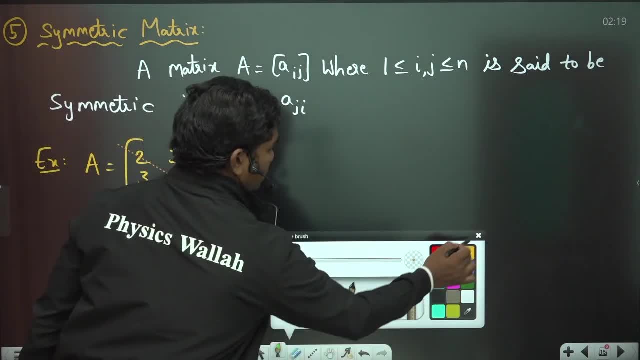 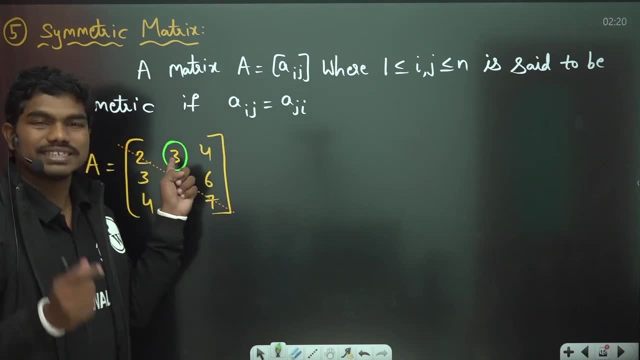 principal diagonal. so if you see this element, for example, if you see this element, this element is on the second o, i mean sorry, the first row, second column. so that element 3, which i have heard of, is a1, 2. so now this a12 will be same as, for example, if i read this a12. now, if you interchange, 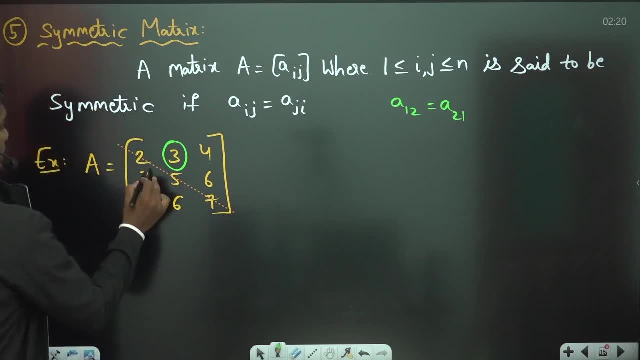 these ji values. this should be equal to the warded column. so now this a12. what happened to the warded movies is that This not only matches, but it makes sense that they are intrinsic and this is alsogreg values. this should be equal to a to one, correct? so if you see, this is also same here. so these two. 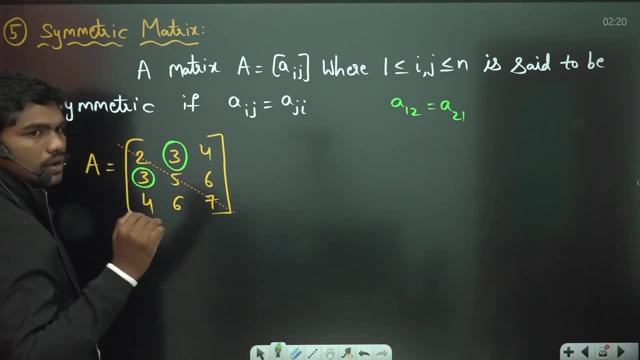 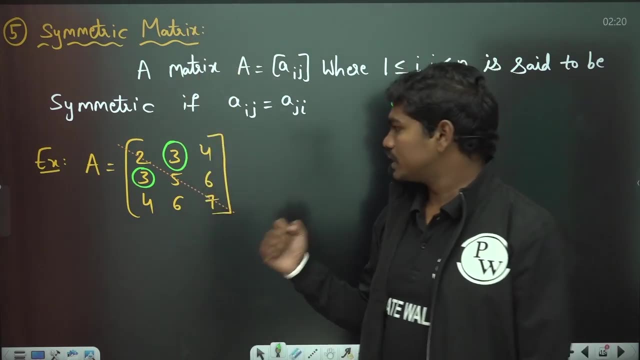 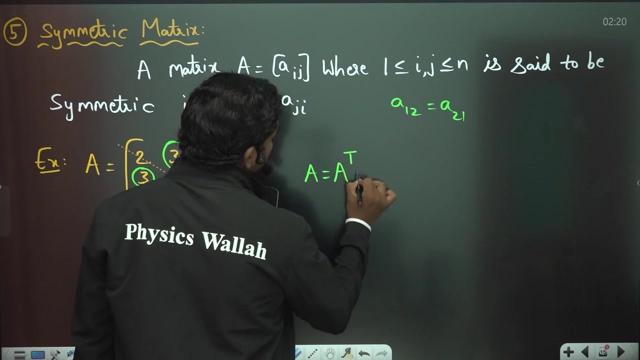 elements will be same generally. similarly these two elements, similarly these two elements. so about the principal diagonal? if you take the corresponding reflection, then the reflection value and the actual value, both will be same, actually. okay, so this is how you define a symmetric matrix and in general, you can write basically this: a is equal to a. transpose clear. 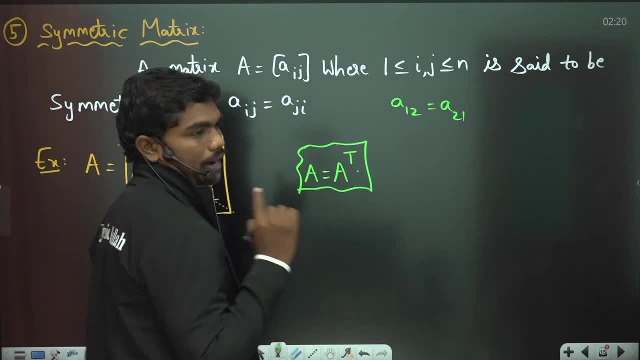 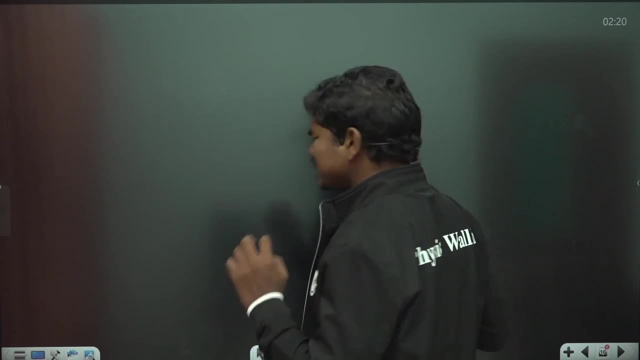 so that's how. this is one very important you know thing in matrices. now i would like to give you one again, one very important type of matrix: skew, symmetric matrix. okay, this matrix is very, very much important. okay why? i'll talk about it when i come to the eigenvalues. okay, so see here six. 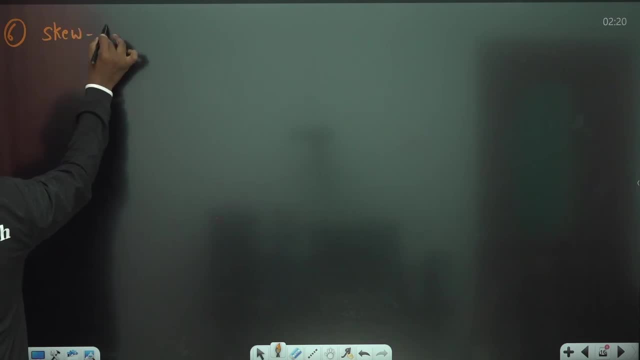 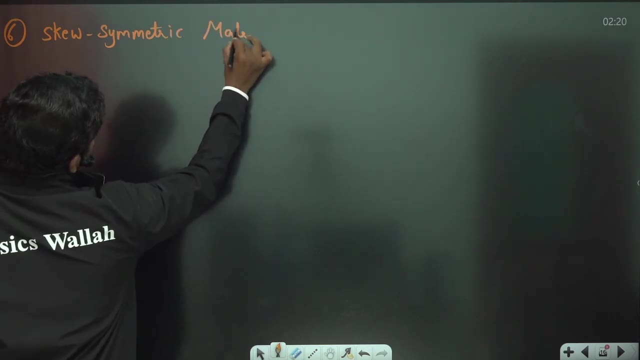 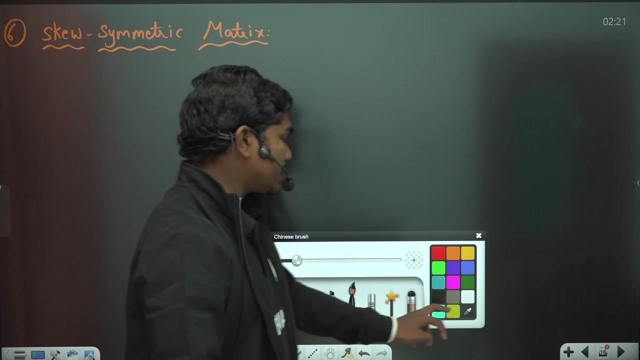 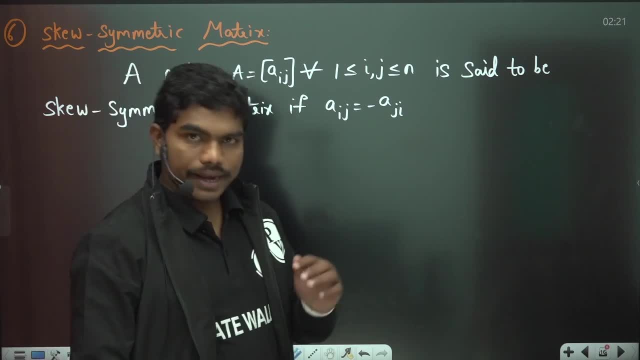 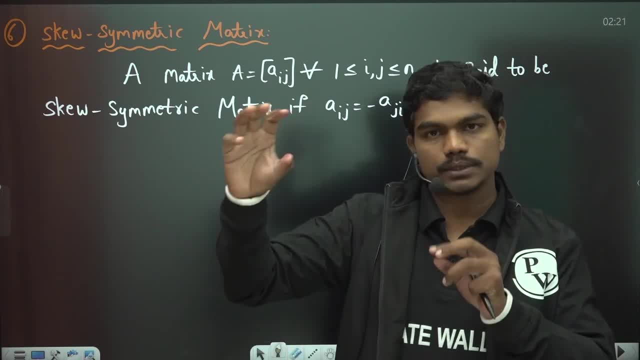 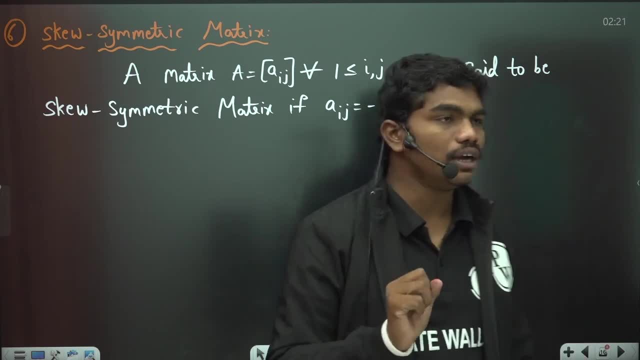 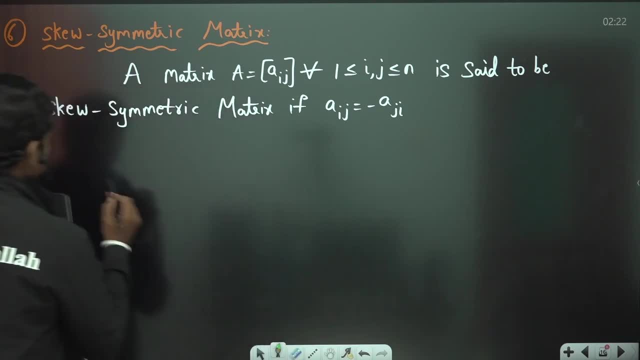 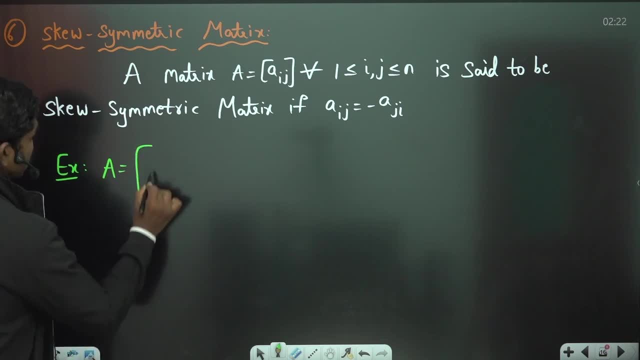 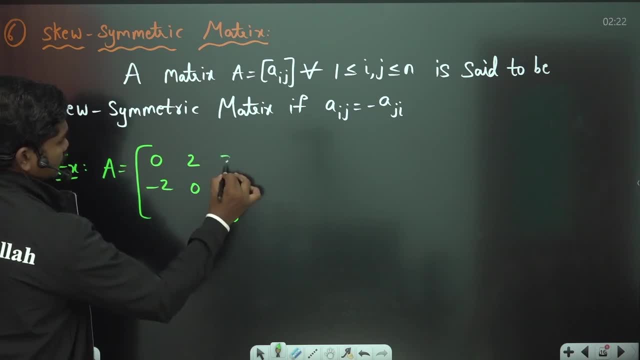 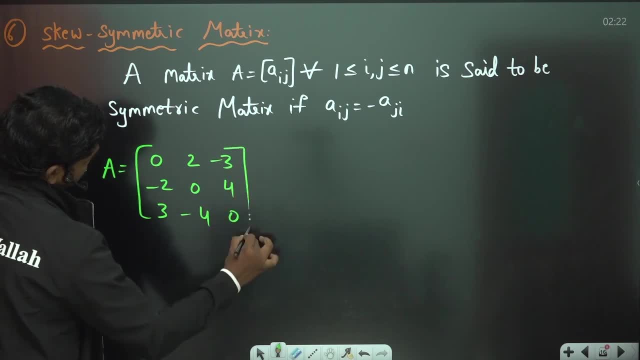 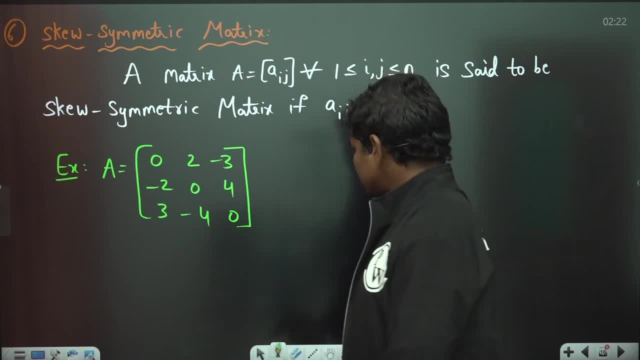 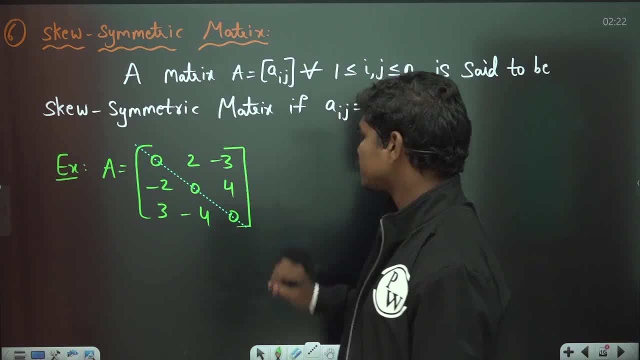 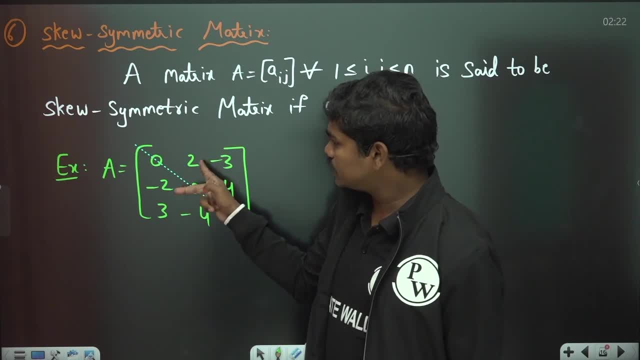 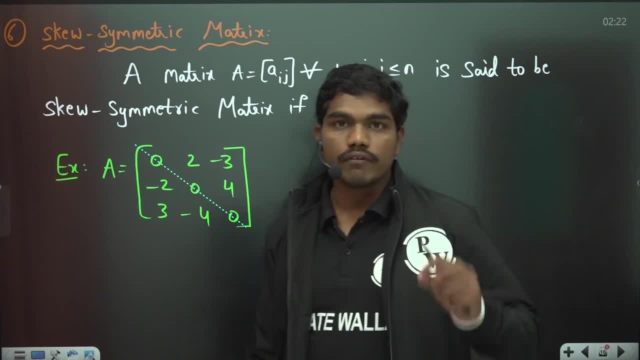 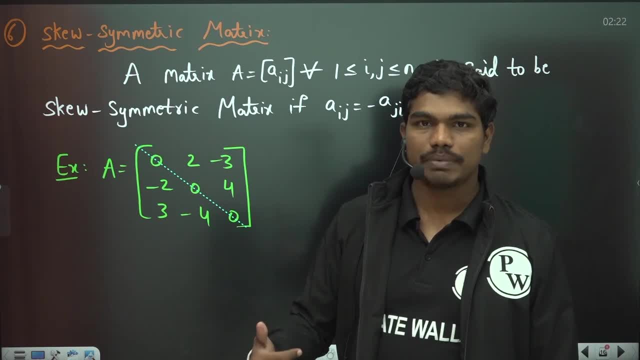 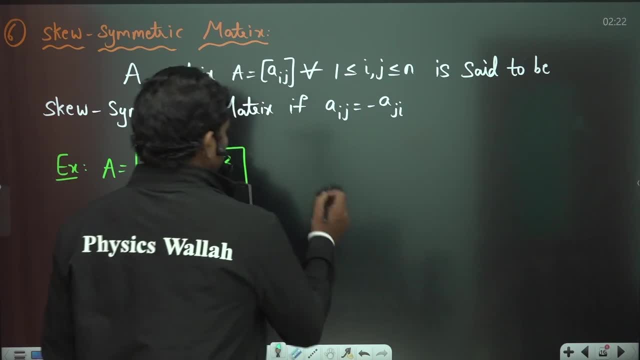 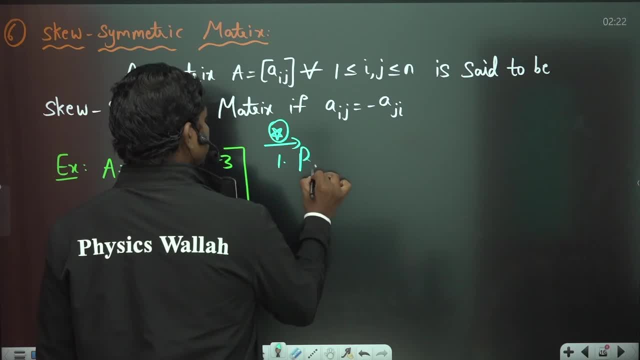 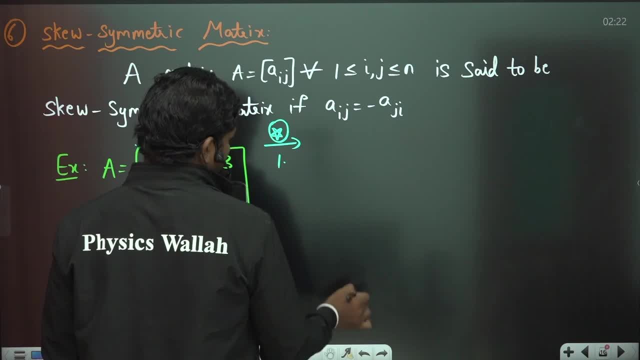 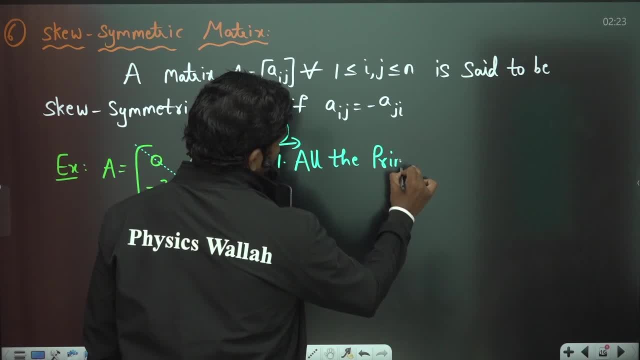 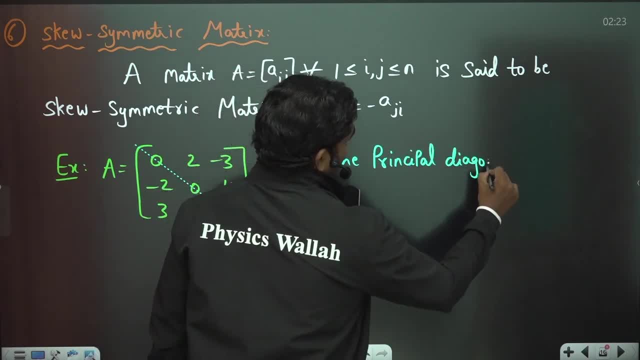 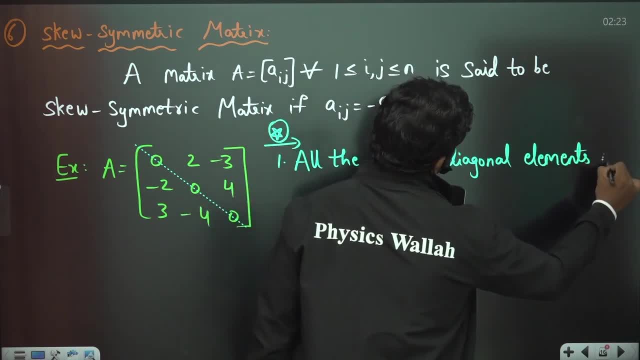 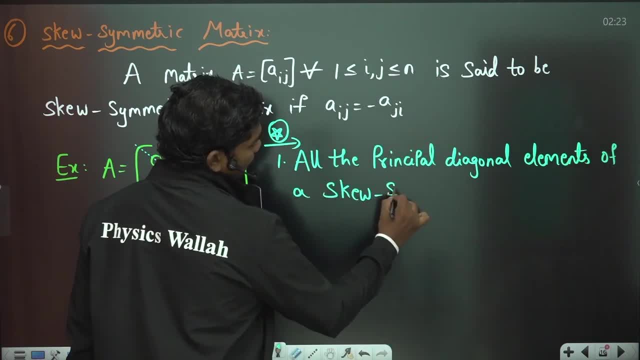 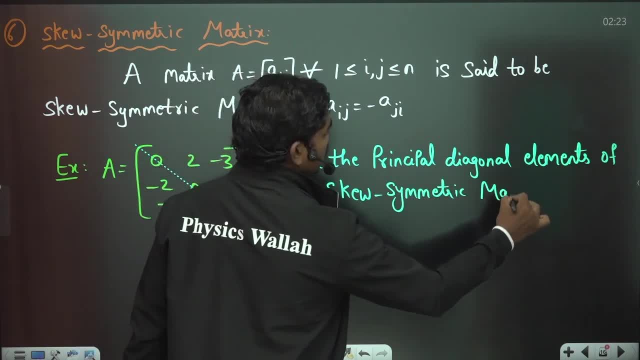 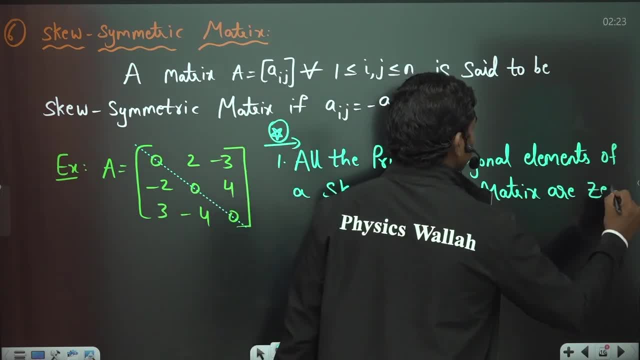 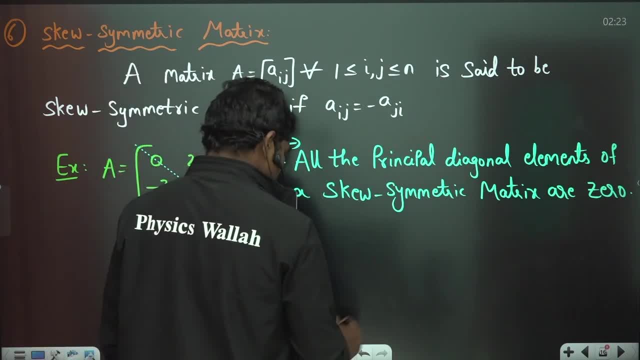 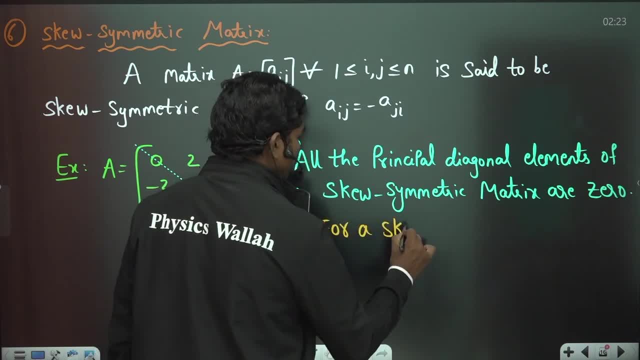 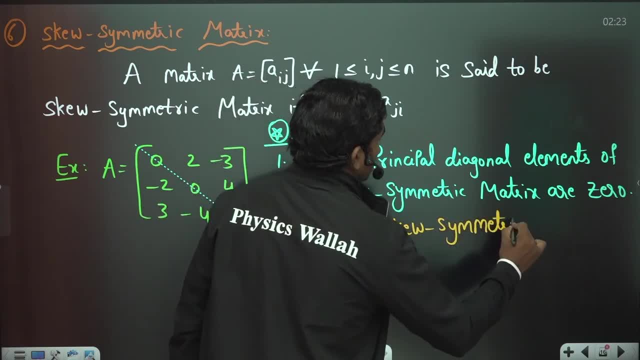 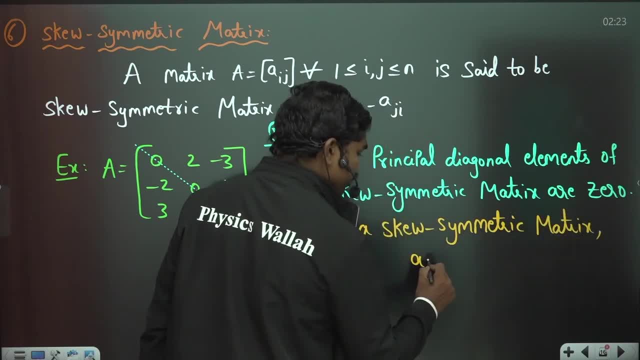 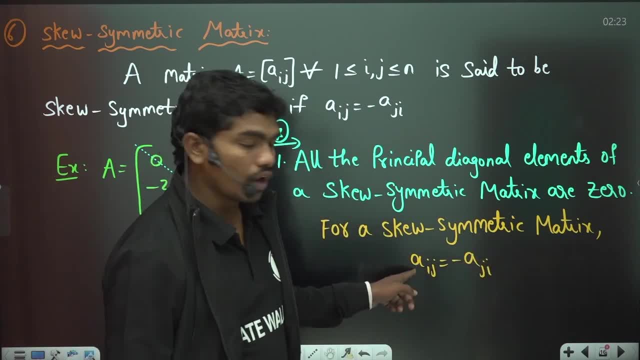 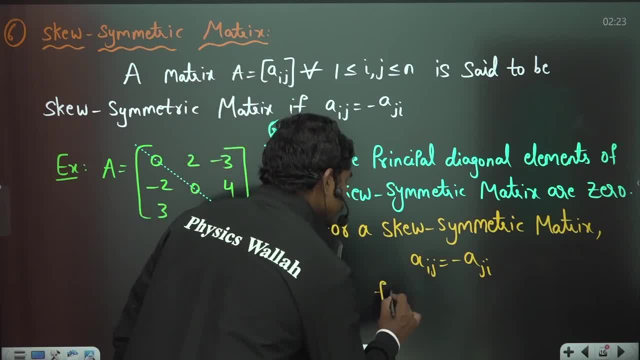 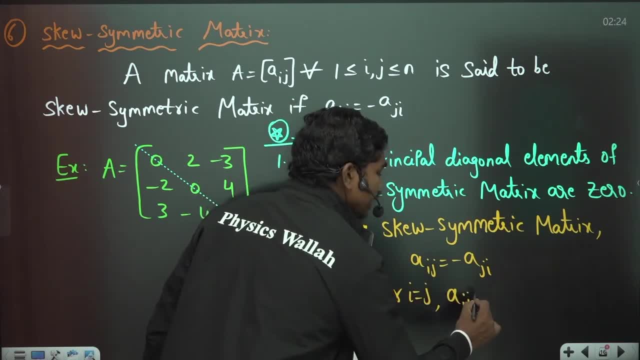 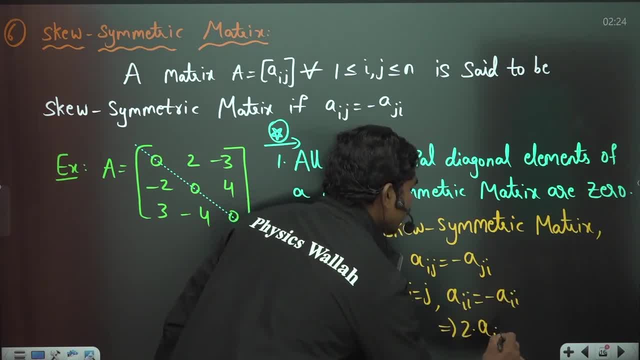 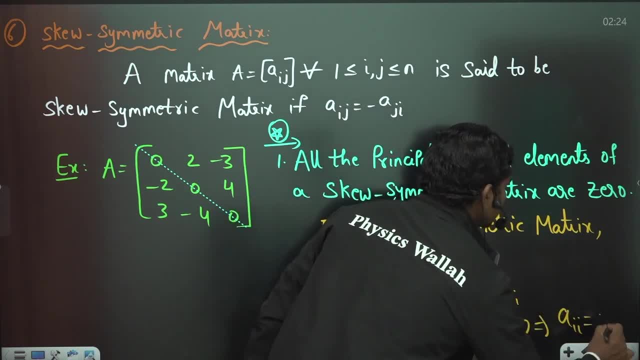 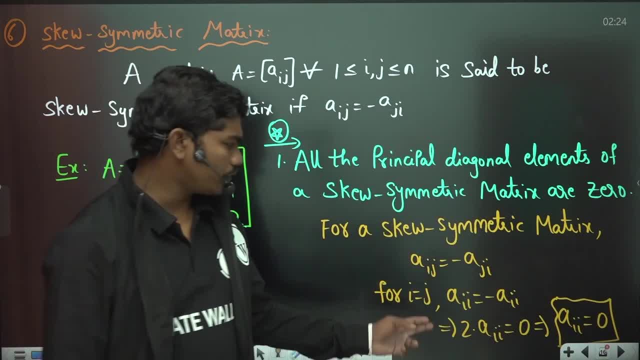 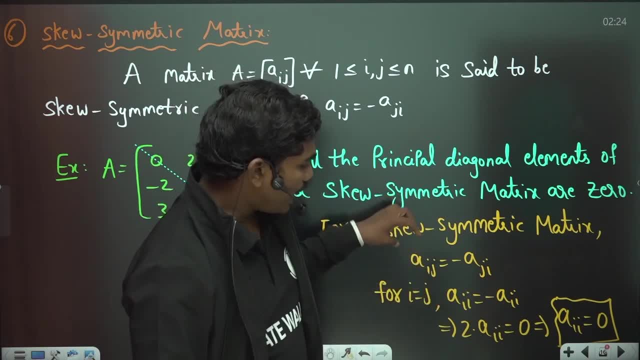 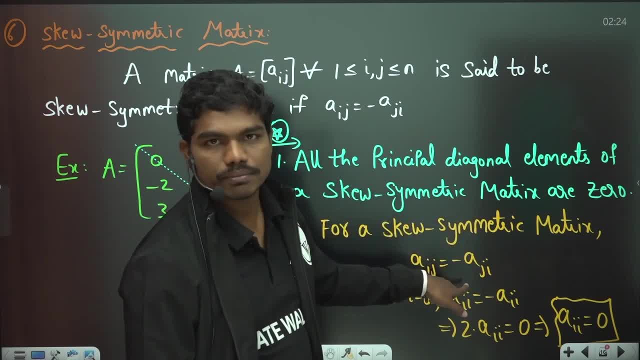 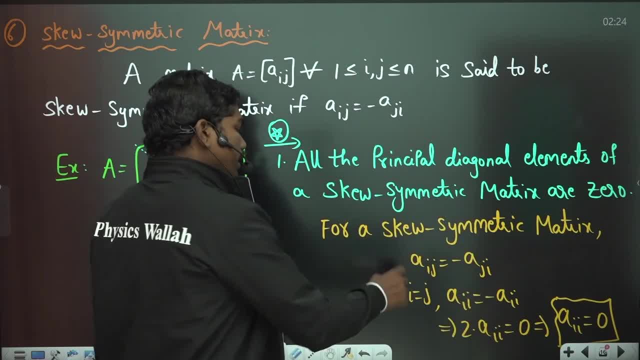 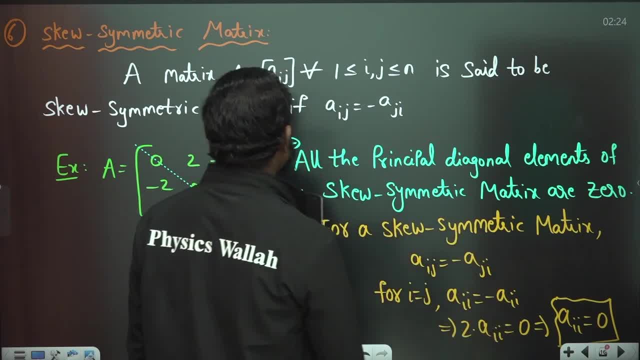 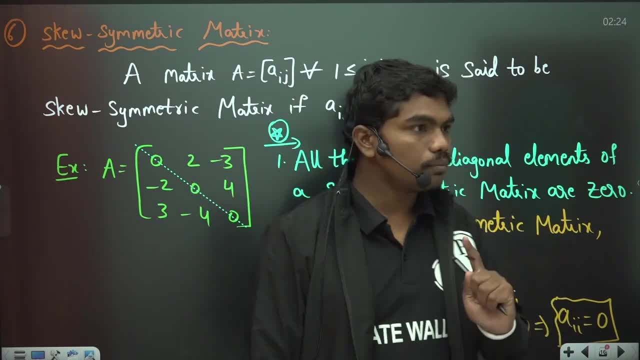 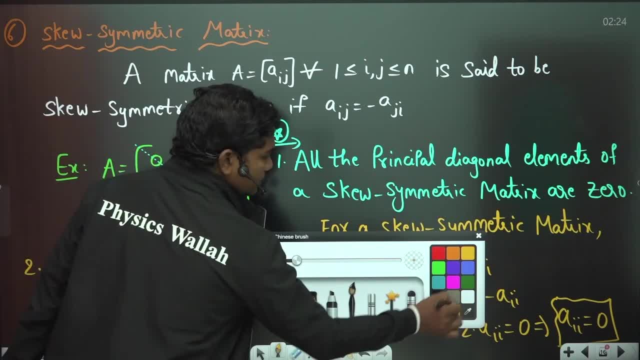 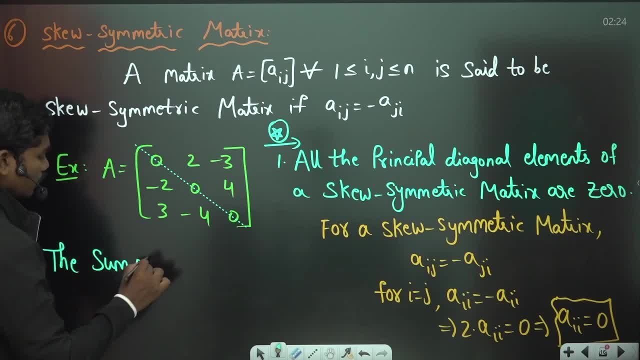 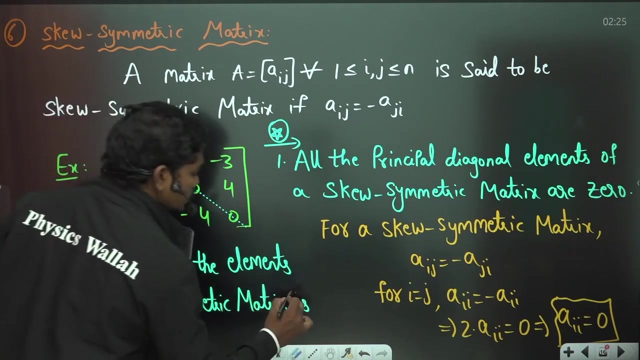 a transpose. but let us say a is equal to minus. So the sum of all the elements, the sum of all the elements of a skew symmetric matrix, the sum of all the elements of a skew symmetric matrix, of a skew symmetric matrix, is 0. basically. 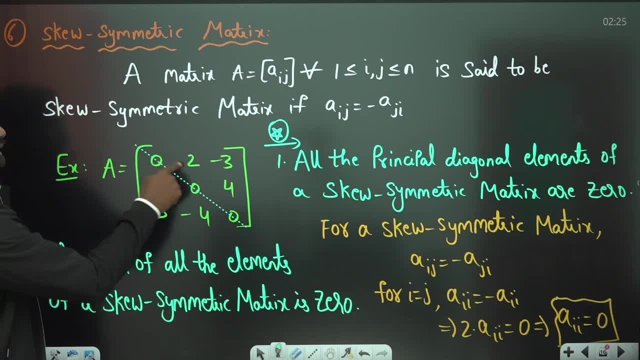 This is 0.. Clear, If you see, because for every element that you find, there is definitely an element with an opposite sign, Correct? So when you add these two, you will get 0.. Similarly, when you add these two, you will get 0. 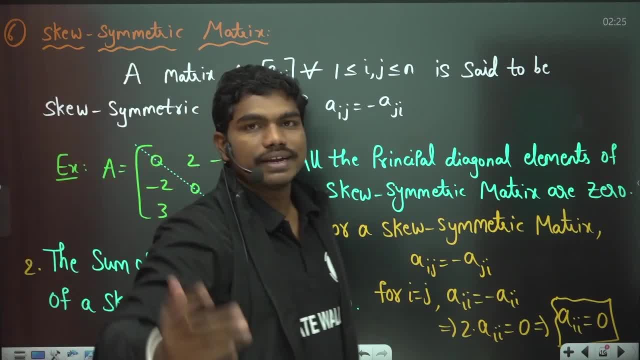 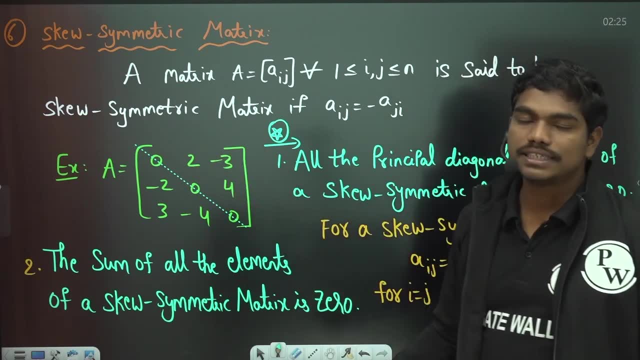 When you add these two, you will get 0.. For every element that you find, you will definitely find a reflection with an opposite sign. So when you add these two elements, you will get 0.. So, similarly, every total sum of these elements in this matrix turns out to be 0. here, 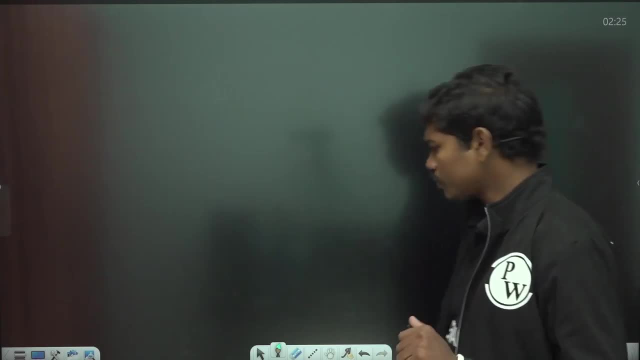 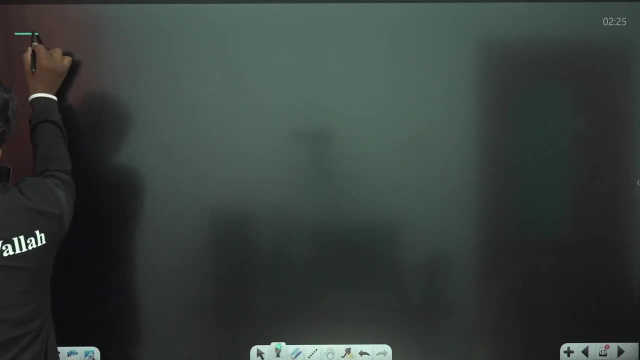 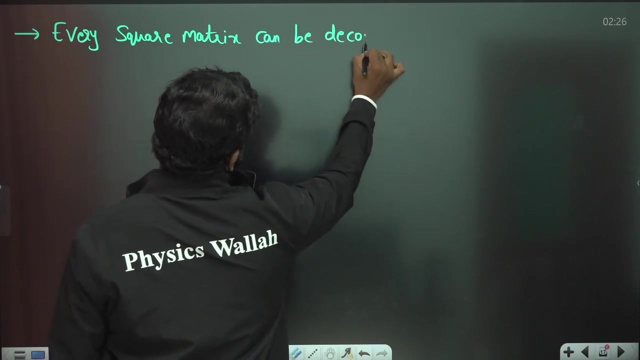 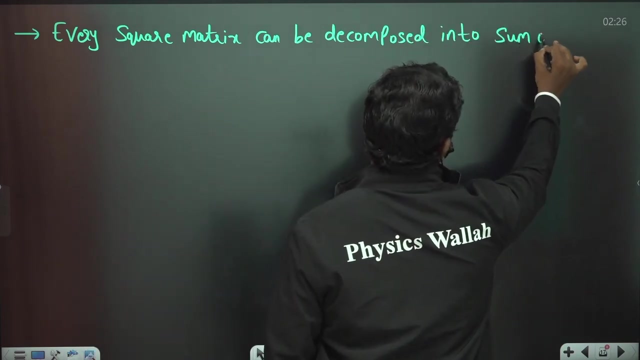 Clear. Now I would like to give you one very important result coming up to this symmetric and skew symmetric matrix. Look what I will tell you: every square matrix, every square matrix, can be decomposed. can be decomposed means splitting up. can be decomposed into sum of a symmetric sum. 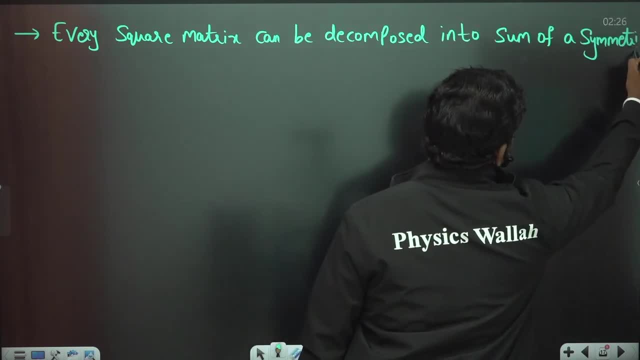 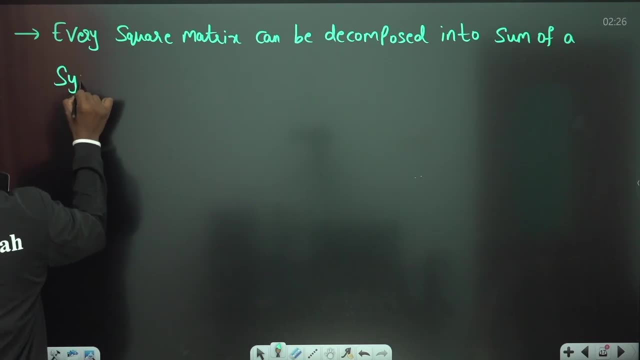 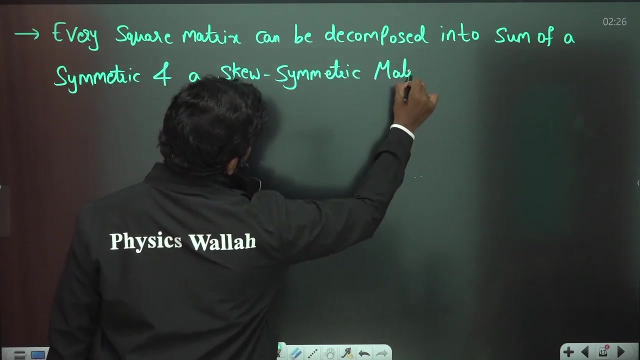 of a symmetric symmetric- oh, I am sorry, I think it is. space limitation is sum of a symmetric and a skew symmetric matrix, a symmetric and a skew symmetric matrix. Now you see how it happens. Look, I will tell you. 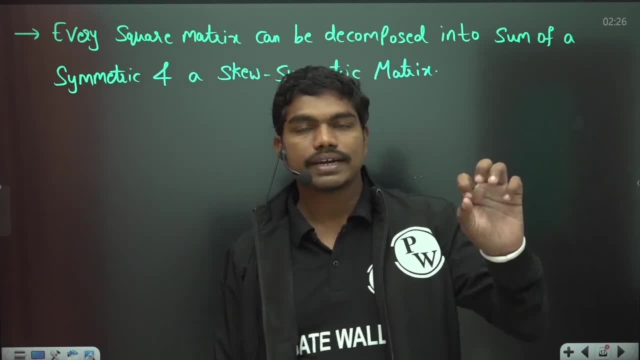 So if you take a look at this matrix, you will see that it is a skew symmetric matrix. So if you take any- basically what I am telling you- if you take any square matrix, then this square matrix can be written as sum of a symmetric matrix and a skew symmetric. 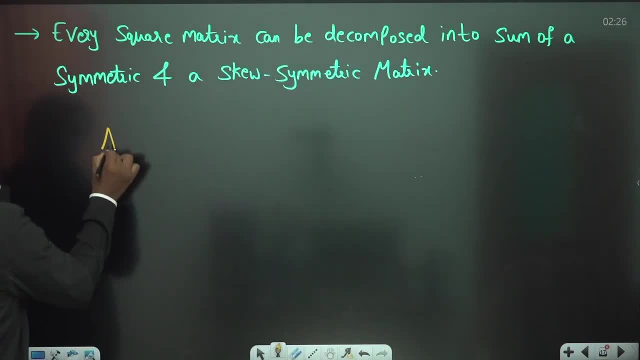 matrix. Look how it happens. Can I write: if I take a square, matrix A, this can be written as half times of A plus A transpose and half times of A minus A transpose. can I write this? because I can write this? 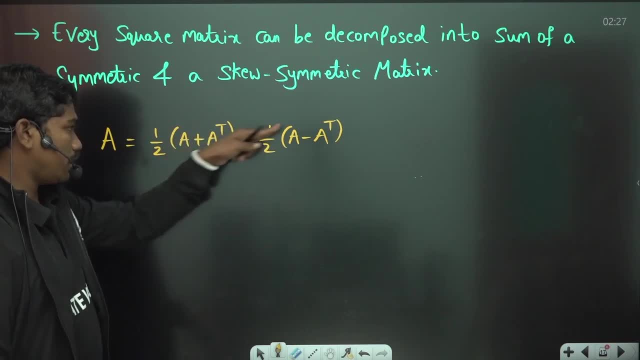 because if you simplify the things, this plus A transpose by 2 and this minus A transpose by 2 and plus A transpose by 2, they cancel each other. So A by 2 plus A by 2 will again give you A. 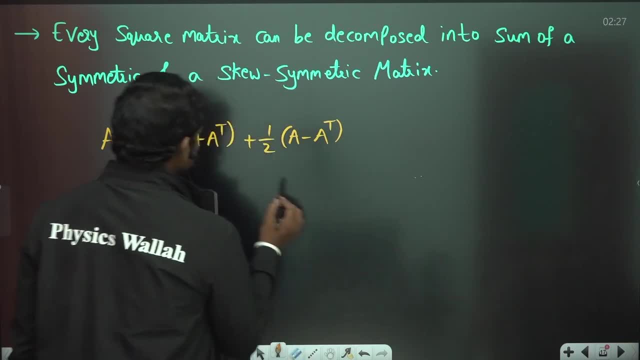 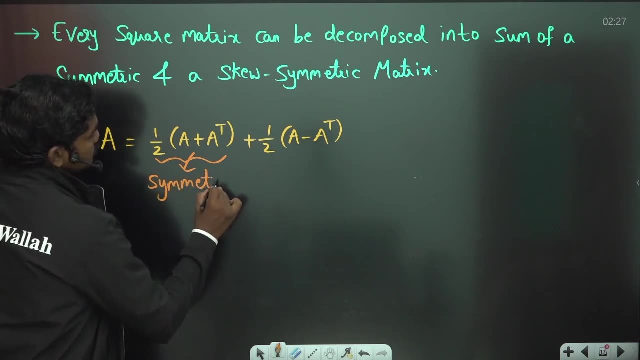 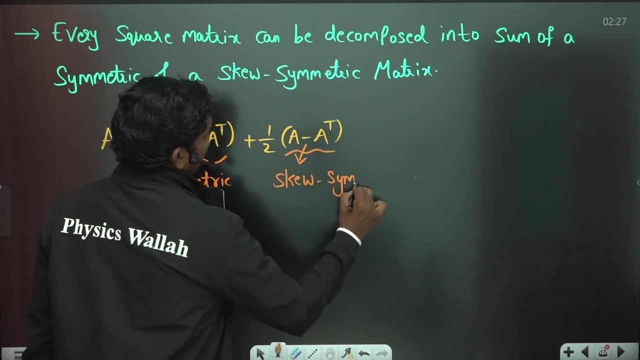 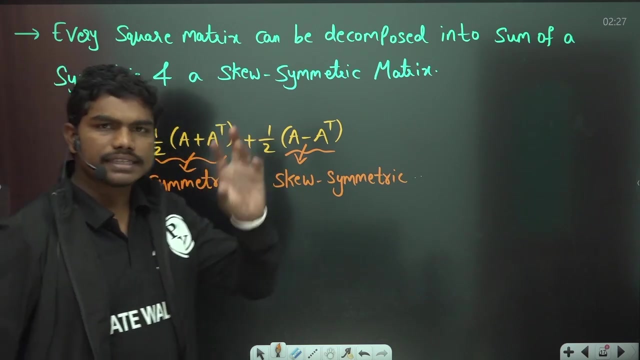 So now, if you see this, if you see this matrix, if you see this matrix, this matrix is always symmetric, symmetric, and this matrix is always skew, symmetric, skew, symmetric. Now, how come you know this? because, look, tell me one thing. let us suppose: if a matrix 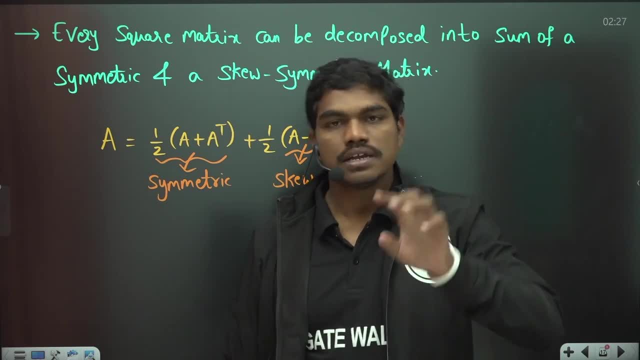 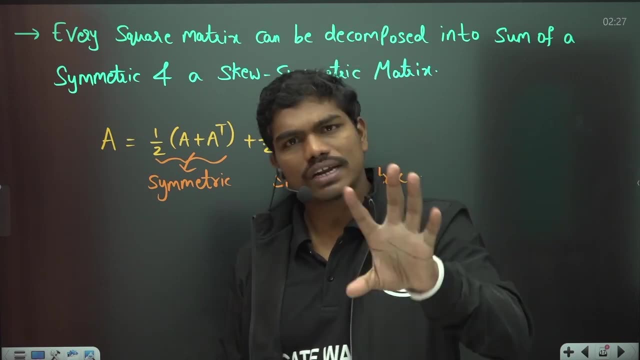 A is symmetric, for example. Okay, Okay, Let us take some matrix: B is symmetric. If B is symmetric, then any multiplication of B is also symmetric. means basically, if I take 3 times of B, 5 times of B, 10 times of B, whatever, I take 10B, 5B, 3B, whatever. 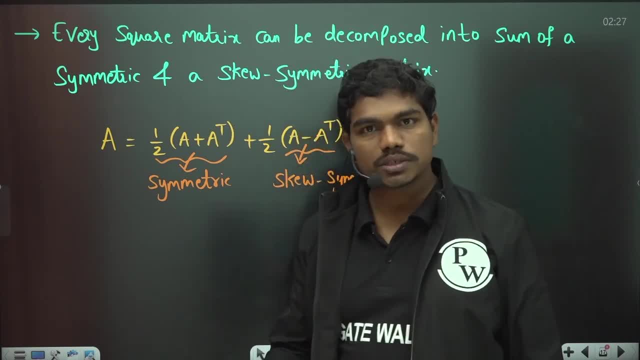 you take, all these are also symmetric matrices. Similarly, if B is skew symmetric, then again this 3B, 5B, 7B, all these things are, or 2B, 4B, anything, all these things are skew symmetric. 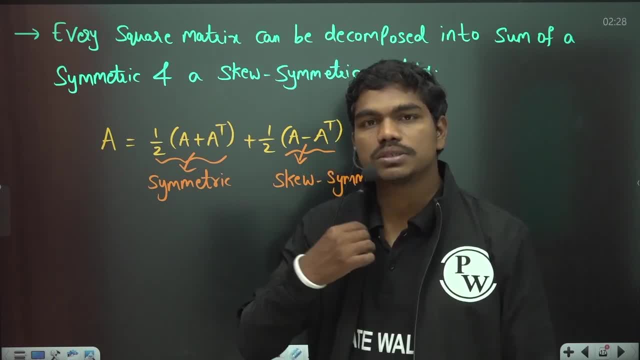 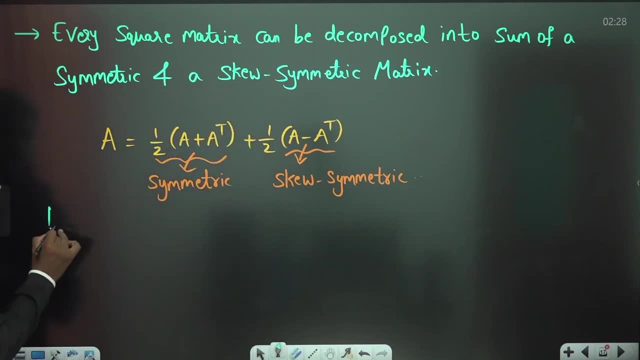 So how to identify whether a given matrix is symmetric or a skew symmetric matrix? Look, I will tell you: Let C is equal to Let C is equal to A plus A transpose. Okay, So what does this imply? If you take C transpose, this gives you A plus A transpose, whole transpose. 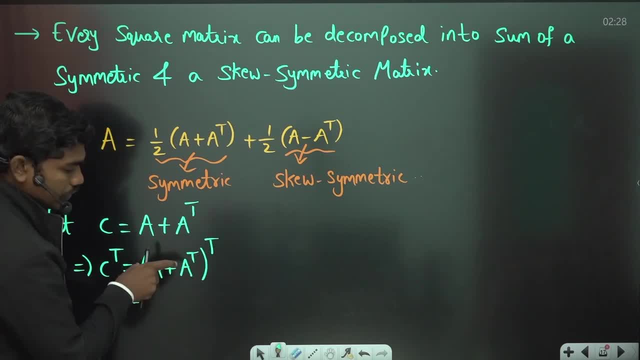 So this is equal to, in properties of transpose I have given you, if you have sum of two matrices, whole transpose, you can write the sum of individual transposes. So this is equal to A transpose plus A transpose, whole transpose. So this is A transpose plus, this is A. 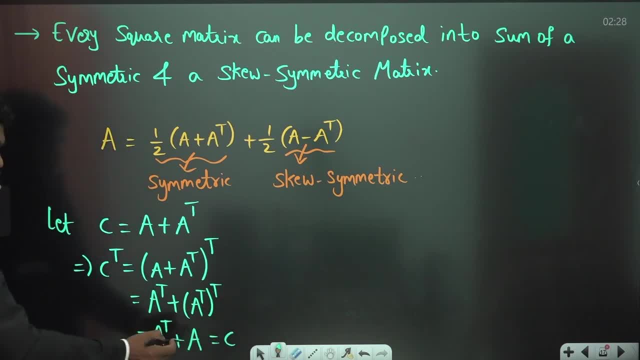 And this is again same as C, because C is same as A plus A transpose, or A transpose plus A. both are same, So C transpose is finally ending up with C. So that's why this matrix C is actually symmetric, Okay. 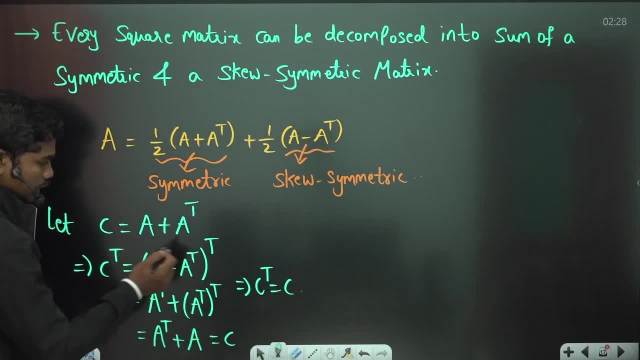 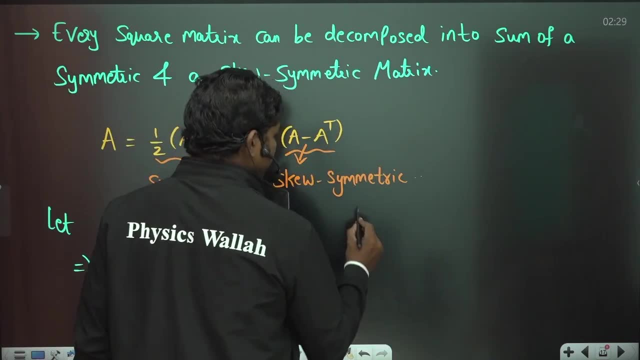 So this implies C transpose is equal to C. So this C matrix, what you assumed- A plus A transpose- is always symmetric. Similarly, if you take this D, if you take this D, let D is equal to A minus A transpose. 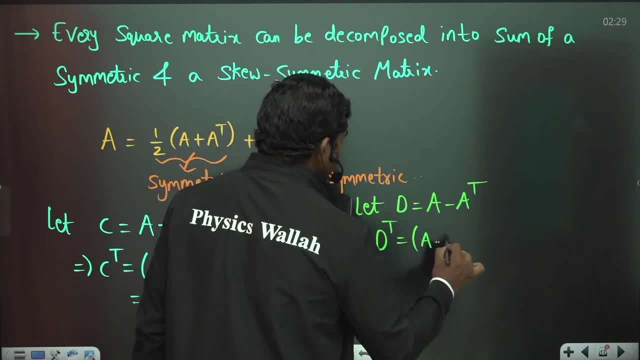 So this implies your D transpose is equal to A minus A transpose, whole transpose. So A transpose minus this, A transpose, whole transpose. If you write, then this is going to be A transpose minus A And if you take a minus sign this: 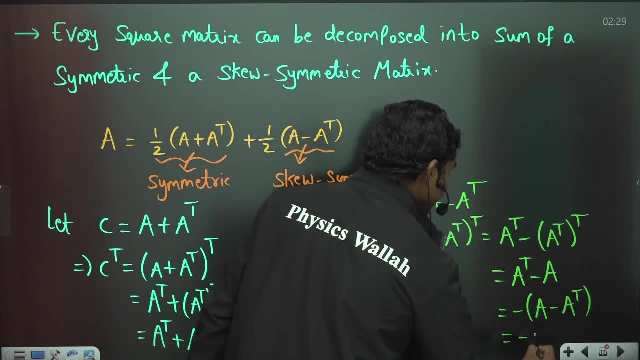 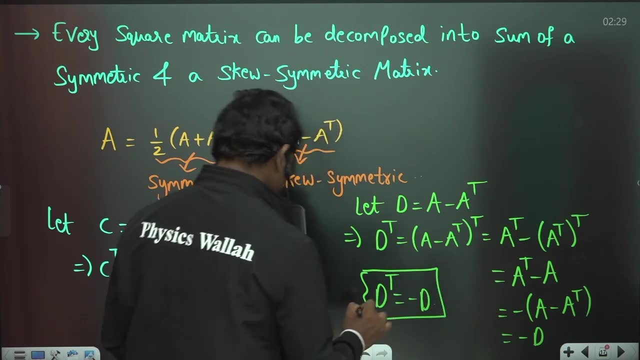 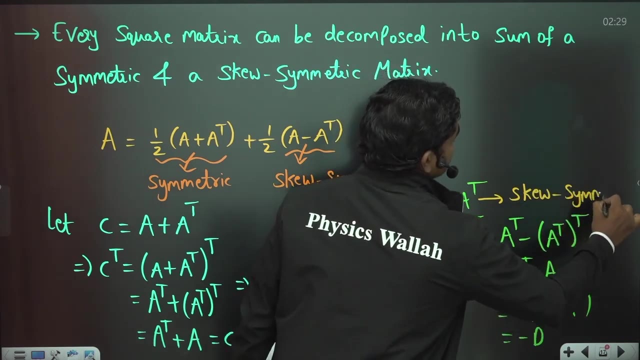 is coming out as A minus A transpose, which is nothing but minus D. So your D transpose is equal to minus D. So which means this implies that this matrix is skew symmetric, Skew symmetric. okay, So this is symmetric matrix. 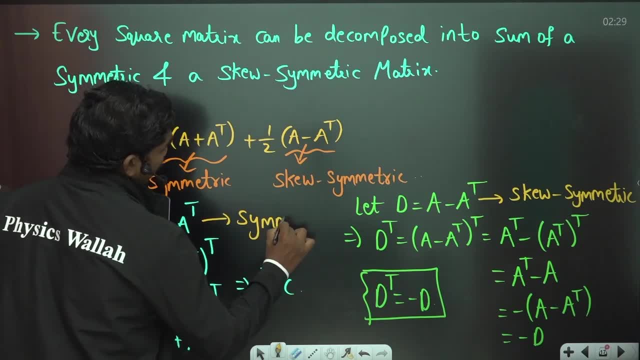 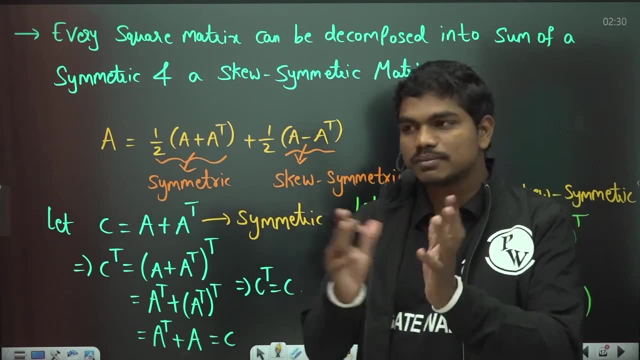 So this is basically symmetric And this A minus A transpose is always skew symmetric. Okay, So if you take any square matrix, you can definitely split this into some of two matrices, out of that, One is symmetric and the other being skew symmetric. 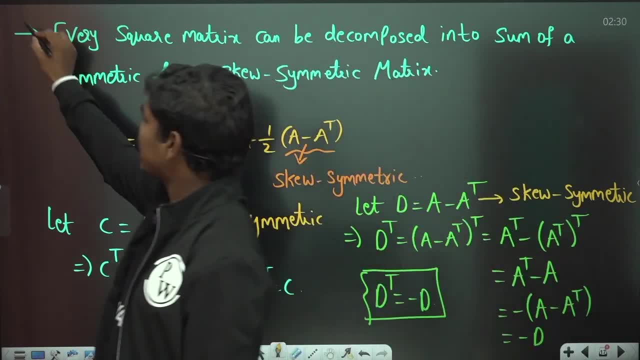 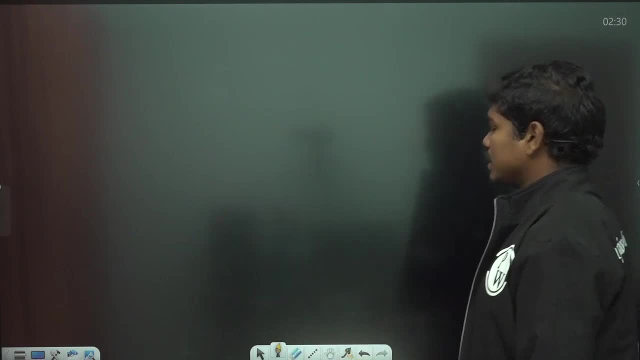 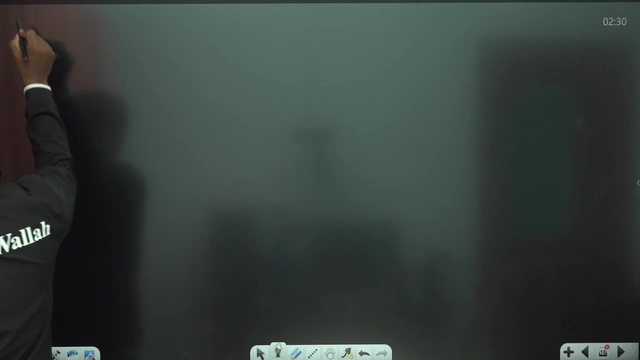 Okay. So I hope we are clear with this result that every square matrix can be split into sum of a symmetric and a skew symmetric matrix. Okay, Now let us go for one way. next important result: that normally these statements, when they ask you in examinations, people get very afraid, but they are simple. 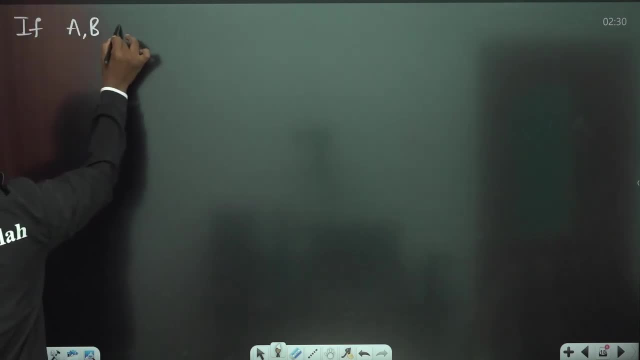 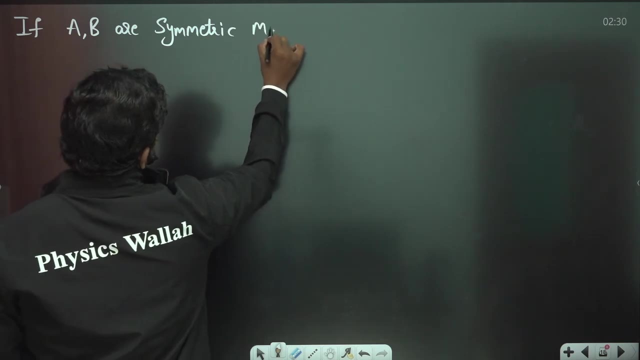 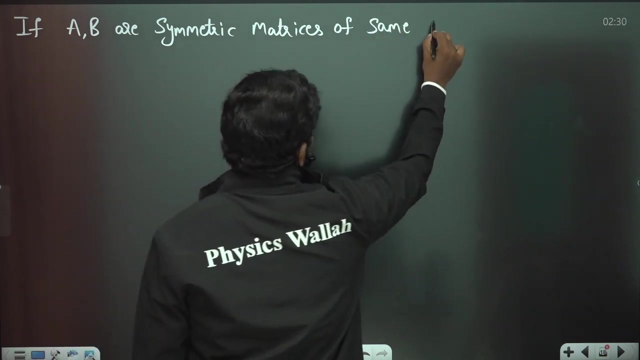 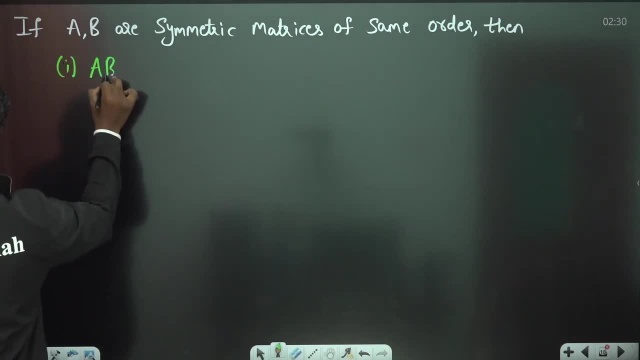 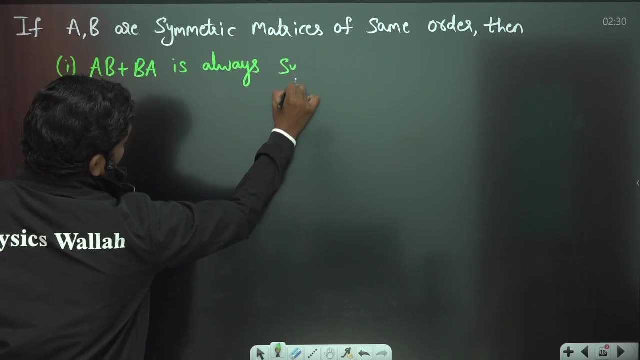 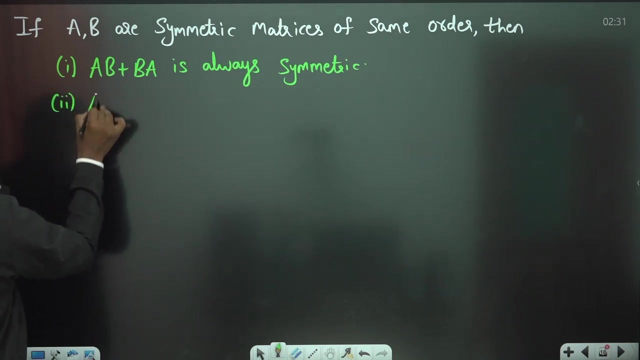 show you how it is happening. First, is A, B plus B. A is always symmetric, is always symmetric. A, B minus B A is always skew symmetric, Symmetric, Symmetric, Symmetric, even. but provided these are symmetric matrices individually, okay, so it's always skew symmetric. 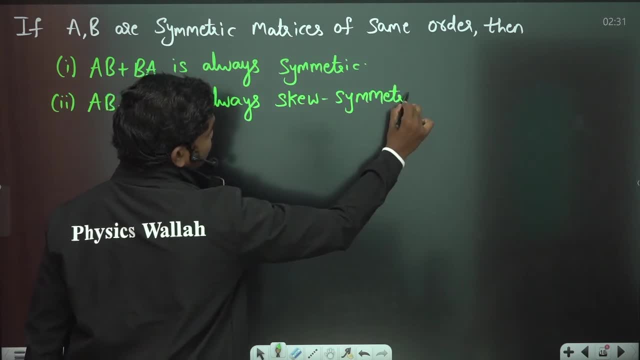 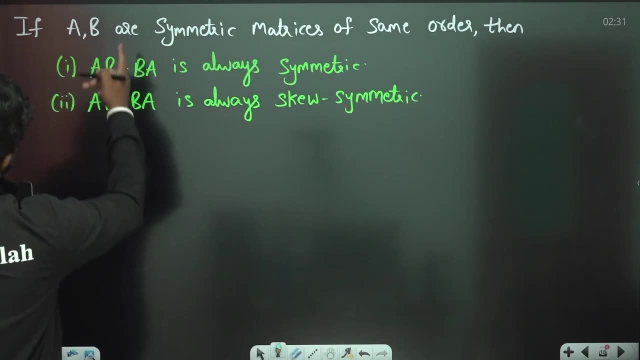 skew symmetric. now how come this is possible? look, i'll tell you. you need not actually remember these results, but you can actually show them. so firstly they are: given a and b are symmetric matrices. so, given a transpose is equal to a and b transpose is equal to b. now let us consider the. 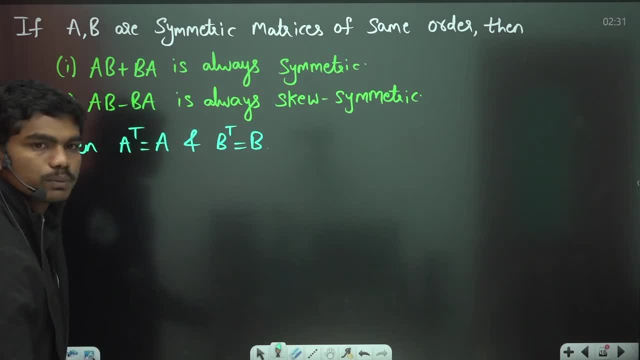 first case: a b plus b a. okay, so when you consider the first case, let us see what's happening here. so the first case is: let c is equal to a, b plus b a. so whenever you want to check whether matrix is symmetric or skew symmetric, just simply consider the transpose of it. c transpose is: 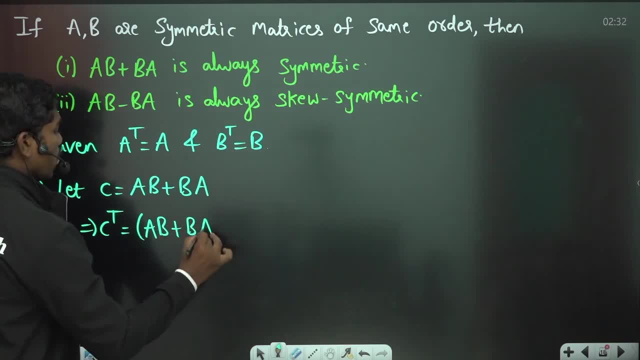 equal to a, b plus b, a whole transpose. so this is nothing but a b transpose plus b a transpose. now i have told you the multiplication of matrices, basically. so if you apply transpose of any multiplication, then the result is going to be like this: b transpose into a transpose. 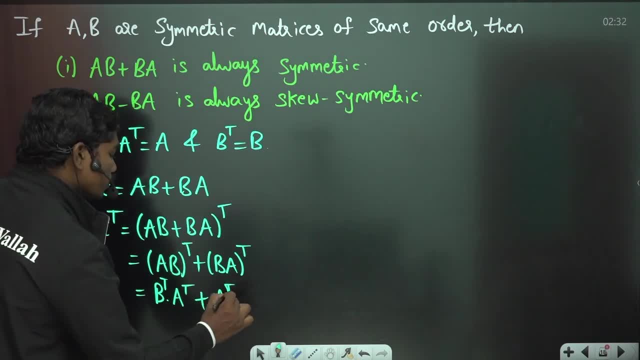 plus a transpose into into b transpose. so this is equal to. since these two are individually symmetric matrices, i can replace this b transpose with b and a transpose with a similarly here. so this is going out to be b, a plus a v. okay, so this result i can write as: b transpose into a. transpose into b. 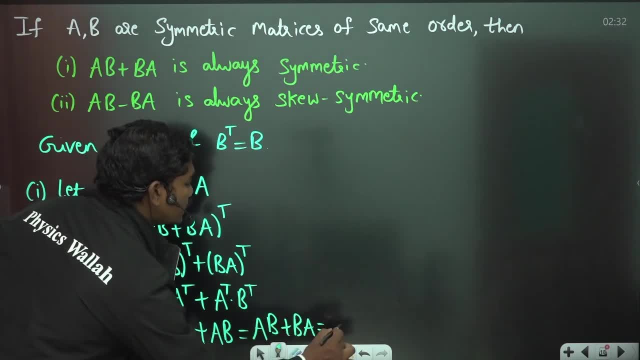 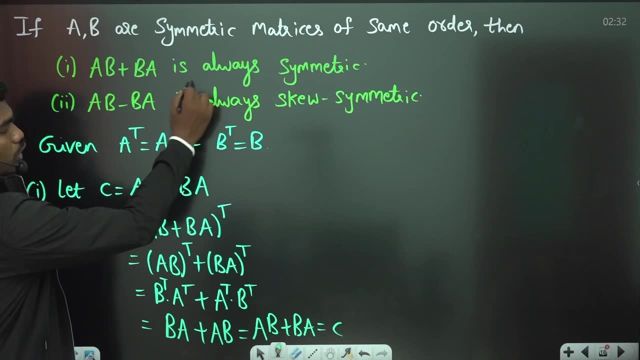 a, b plus a, b plus b a, which is again equal to c. so you have started by considering c transpose and finally you ended up that c transpose is same as c. so this matrix a b plus b a is always symmetric here. one caution: i have written b a plus a b as a b plus b a, not because that b? a should be equal. 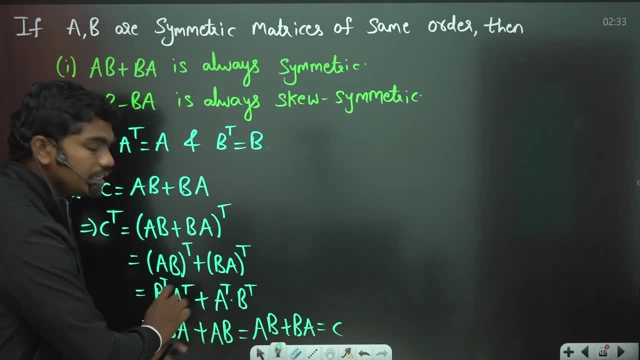 to a b. no, that's not the case, but since the summation is commutative in any way, so this is b a plus a b or a b plus b a. both give you same answer, but not this. b a should be equal to this a b. this is the same answer, so this is the same answer. so this is the same answer. so this is the. 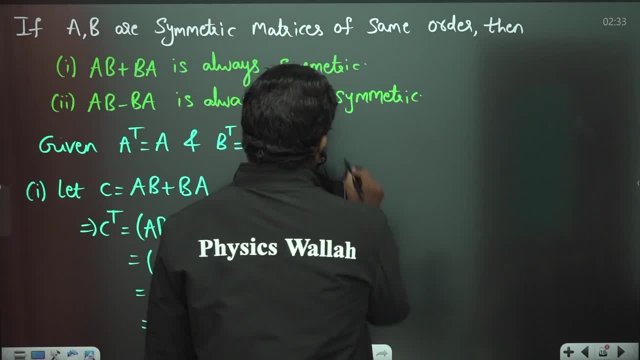 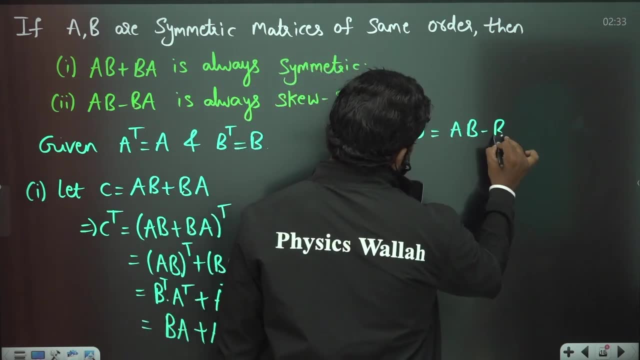 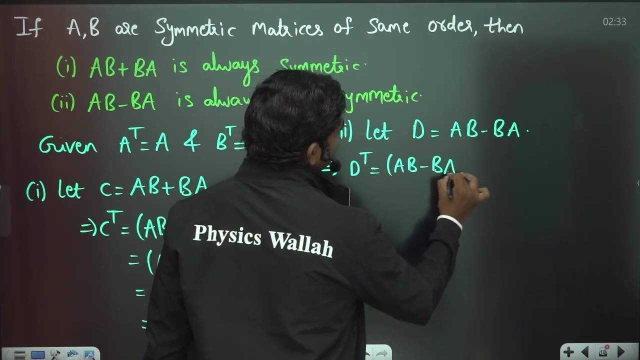 need not happen, okay. so please be sure with this now. second, let c is equal to or d. you can say a b minus b a, then what this tells you: d transpose. if you take a b minus b, a whole transpose. so this is a b transpose minus. 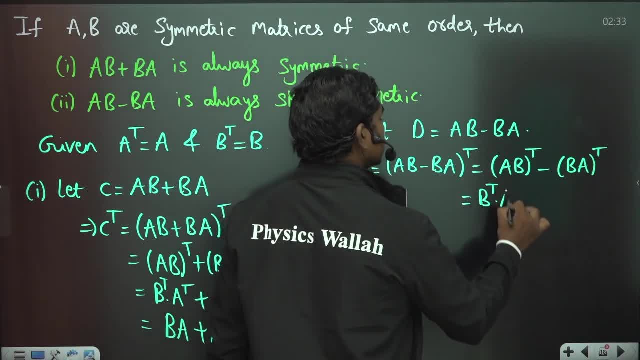 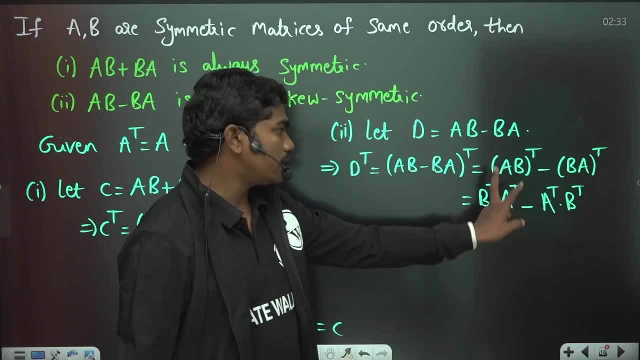 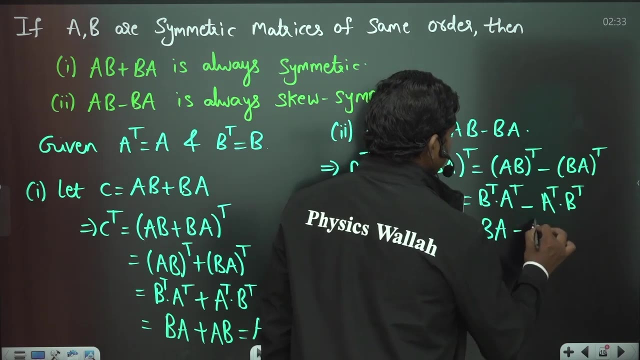 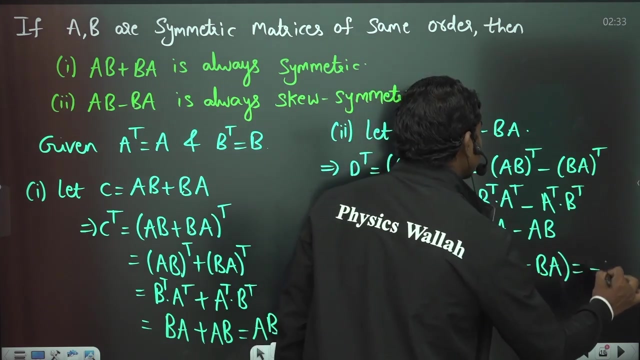 b a transpose which is equal to b transpose, a transpose minus A transpose into B transpose, because you have seen AB whole transpose is, you know, the transpose individual, transpose, multiplication, but taken in a reverse order. so this is equal to BA minus AB. so if you take a minus sign here you will get AB minus BA, which is nothing but minus D actually. 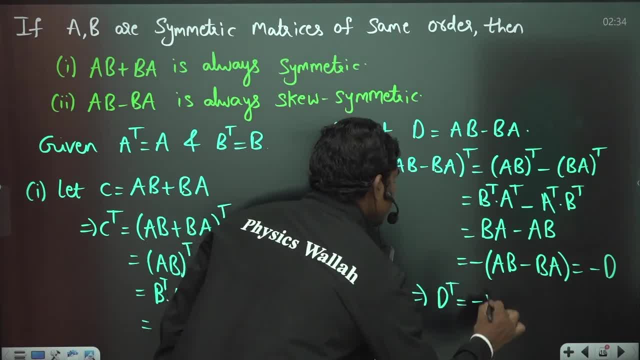 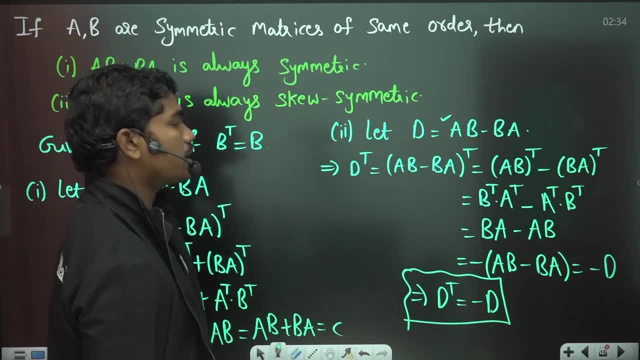 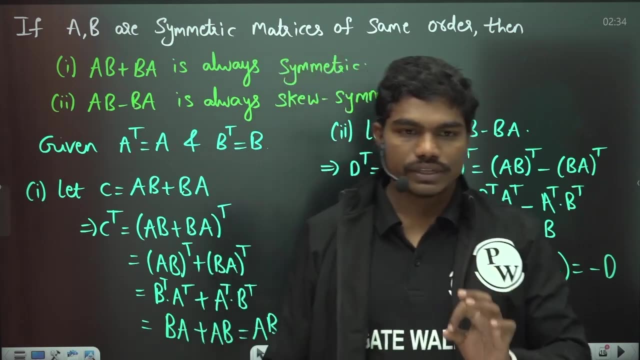 so this ends with D. transpose is equal to minus D. so definitely, D is a skew semantic matrix. and what is D? we have taken this AB minus BA. okay, but this transposes we are able to replace in this form because it's individually, given that both these are symmetric matrices. clear, if this. 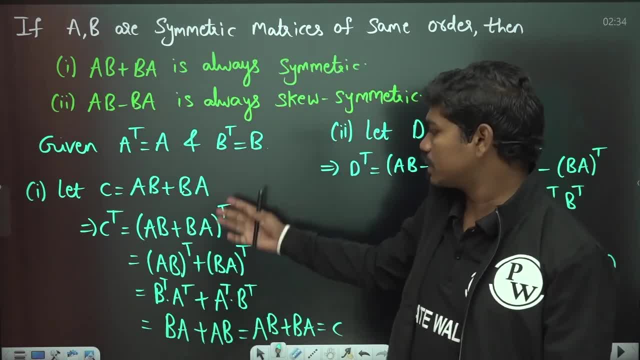 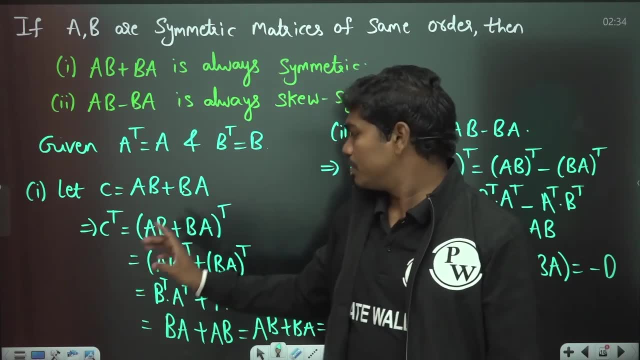 individual symmetricity is not given, then definitely you need to. you cannot substitute this: B transpose as B, A transpose as A. sometimes they'll give skew symmetric. here. then again, the process needs to be same, but in place of B transpose, let us suppose if they give A and B. 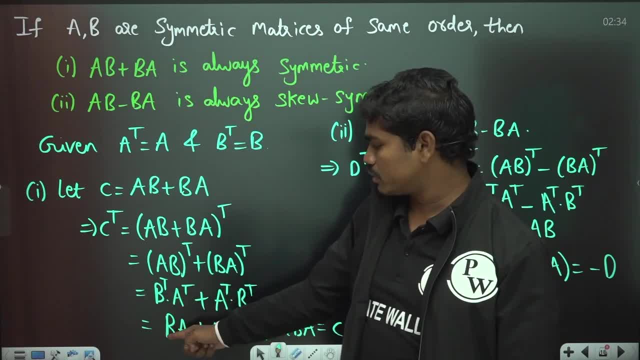 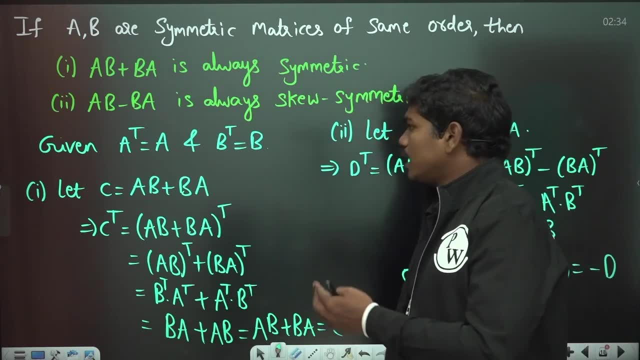 are skew symmetric matrices, then here you will put B transpose equal to minus B and A transpose is equal to A transpose minus A. okay, so that's how we actually, you know, generate the results, and these two results are very much easy now. you need not remember them. actually they are very easy to you know to show. 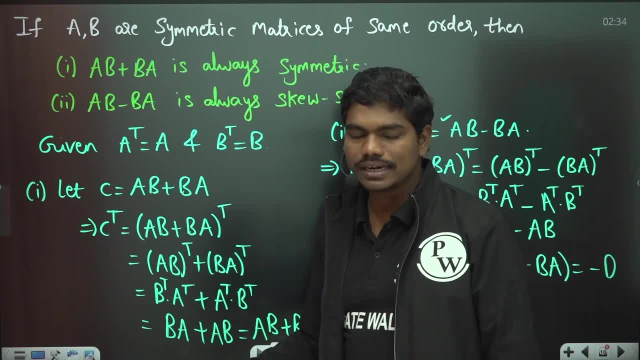 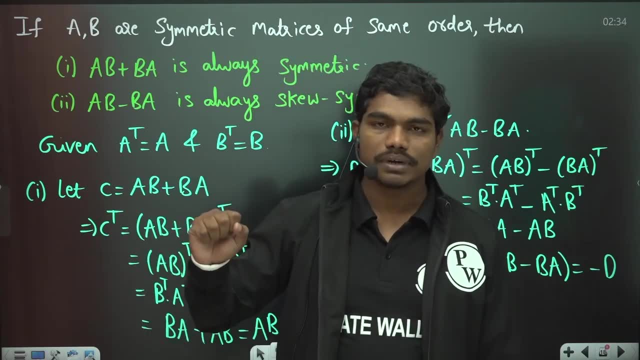 them. it's just some two, three basic properties. if you apply, you will get the answers clear. I hope I am clear till this point. so this is a single short video. so by the completion of this video you will be able to get complete knowledge on this linear algebra, which is very, you know, very. 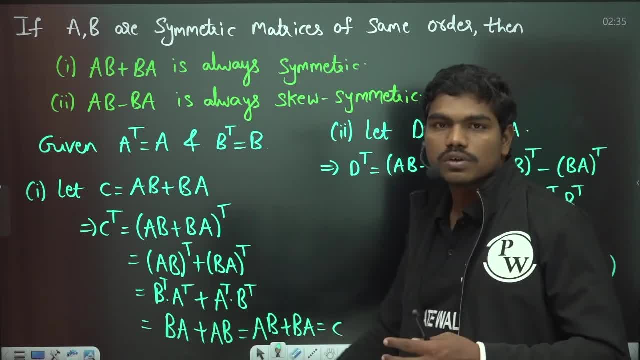 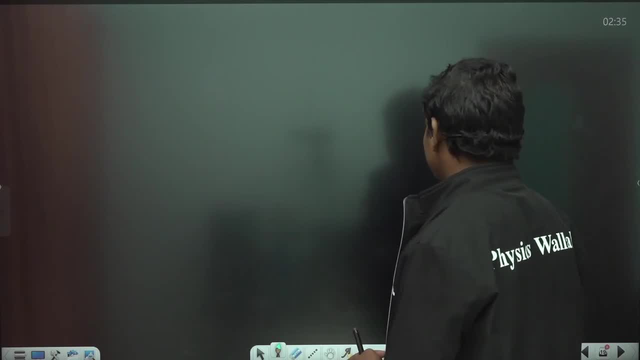 good for gate examination. okay so, and of course, this video, I am inclined to share it with you and, of course, if you have any questions, please feel free to ask in the comment section below and I will try to answer your questions as well. so that's why I am dealing with this. okay, now once. 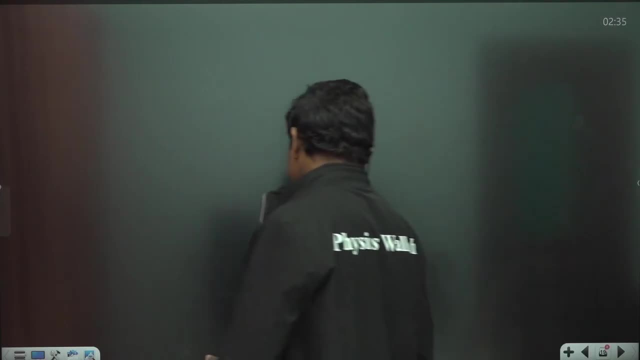 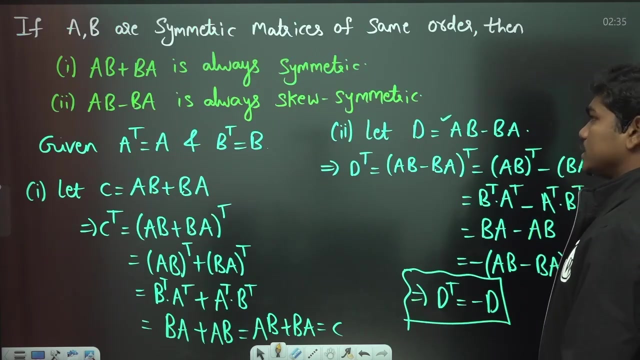 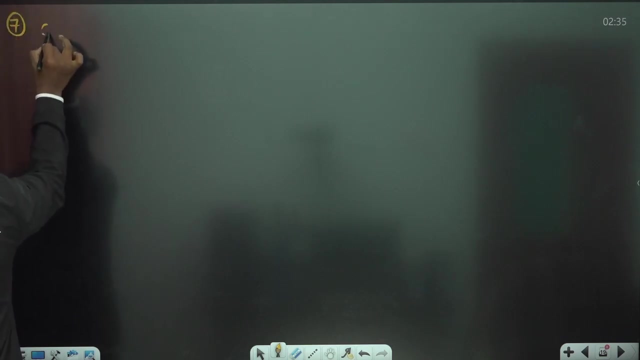 you have with this. now I would like to give you some more properties. okay, so now some more types of matrices let us give. so how many types I have given you till now? so all these are properties. six types I have given you. so let us go for the seventh type. so seventh, orthogonal matrix. 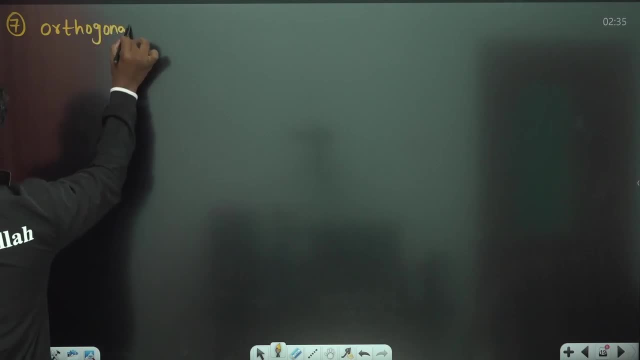 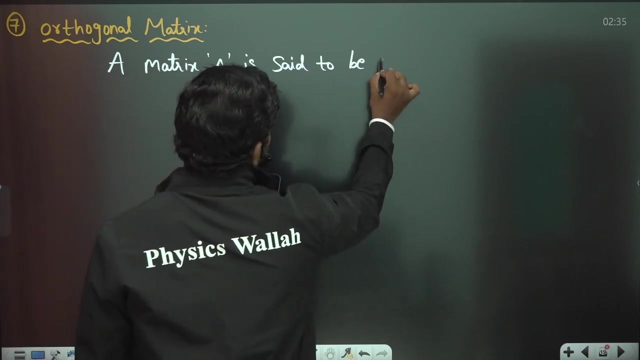 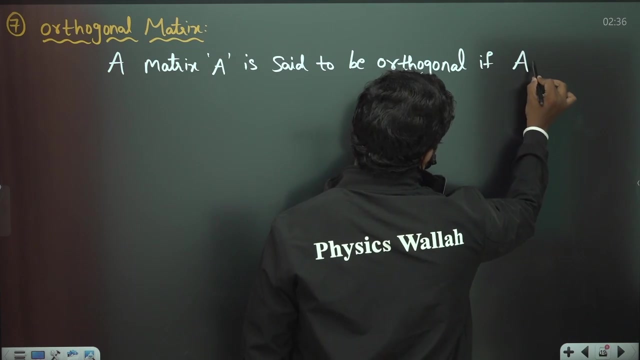 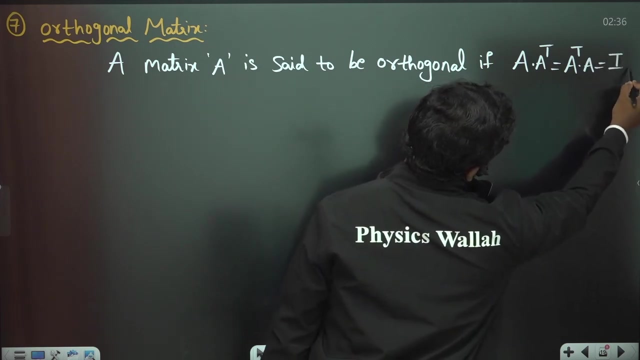 so orthogonal matrix. so what is an orthogonal matrix? so let us see a matrix, a matrix. capital A is said to be orthogonal, is said to be orthogonal, is said to be orthogonal if A times A transpose is equal to A transpose times A, which is equal to identity matrix- okay, of same size of course. so A into A transpose. 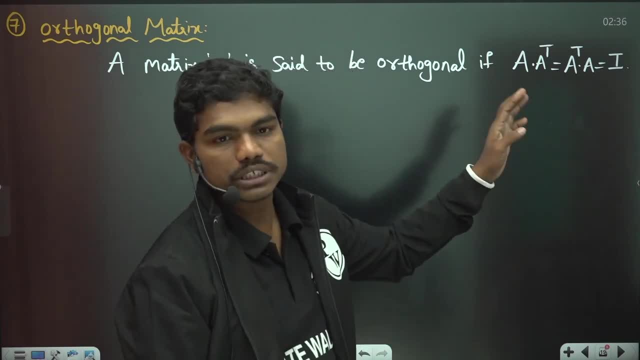 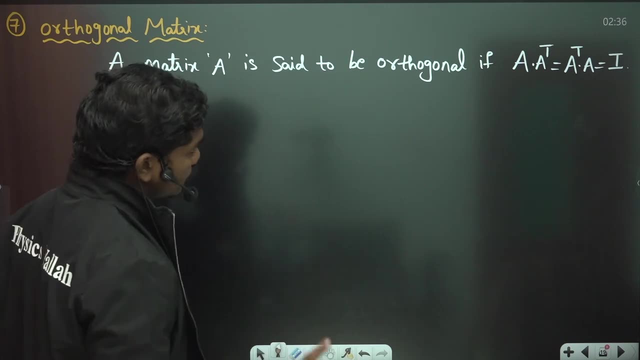 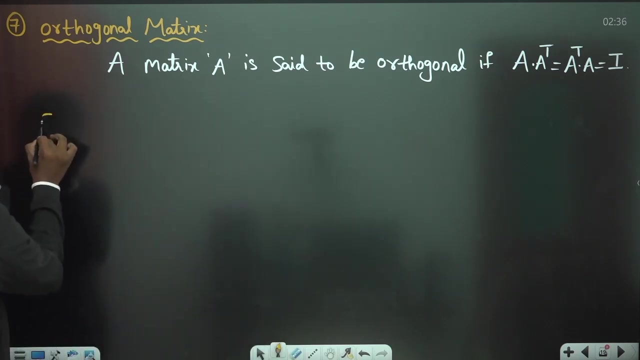 this: A into A transpose is equal to A. transpose into A is equal to I. now let us see here: okay, I hope mic is good, yeah, mic is good, so no issue. so A into A transpose is equal to A. transpose into A is equal to I. so let us take one example and let us see example. A is equal. 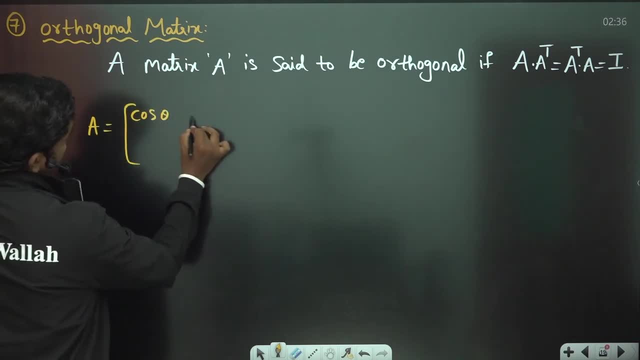 to, for example, say cos theta A is equal to cos theta A is equal to cos theta Minus sine theta, Minus sine theta, zero sine theta, cos theta zero zero one. so let us suppose this is some matrix. now, if you multiply this mechanics with its transpose, so A into A transpose is equal to a into A transpose is equal to cos theta minus sine theta. 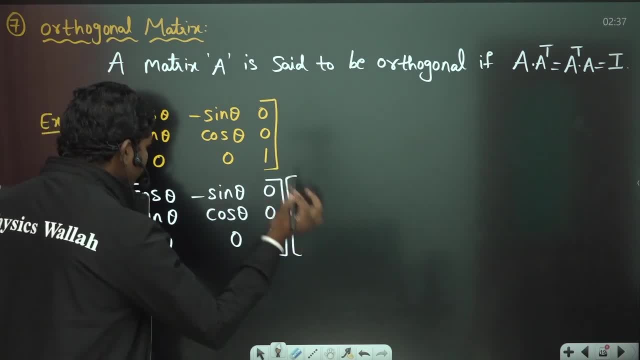 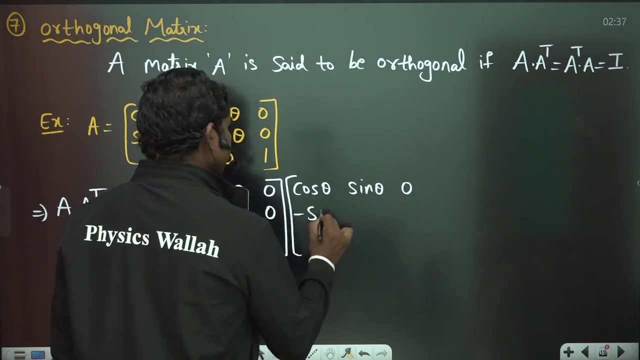 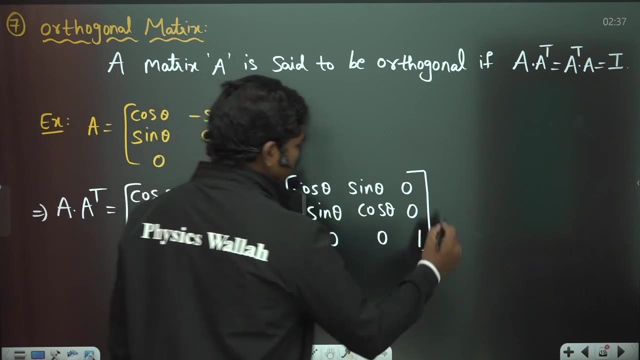 0, 1. now multiply the transpose of this matrix. so if you do the transpose it's like cos theta sine theta 0 minus sine theta. cos theta 0, 0, 0, 1. now if you multiply these two matrices you can easily understand that first row, first column element. if you multiply this first row with this: 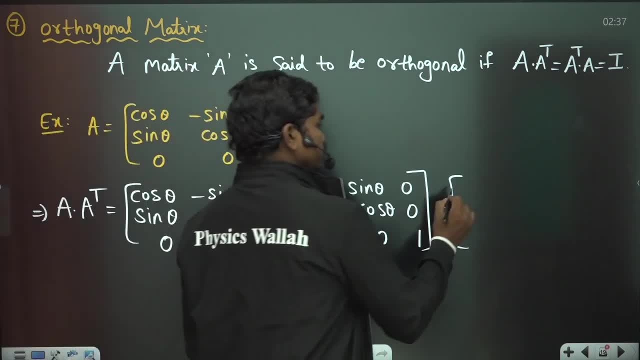 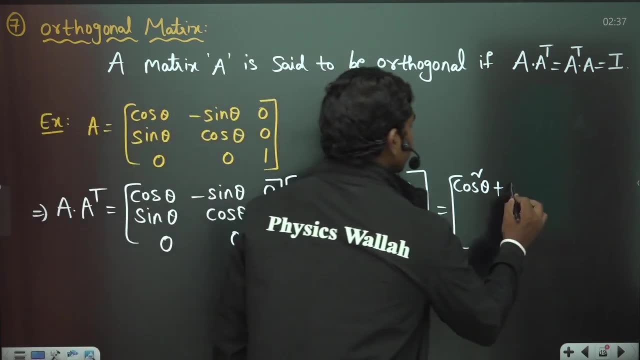 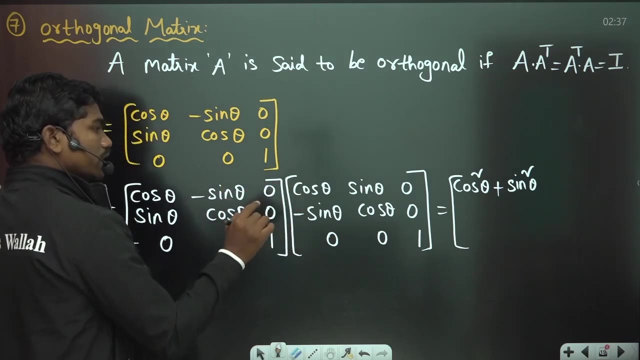 first column: cos theta into cos theta. cos square theta plus minus sine theta into minus sine theta. sine square theta plus this 0 into 0: 0. so the first row, first column element, is going to be cos square theta plus sine square theta. that's it okay. now first row, second column element. 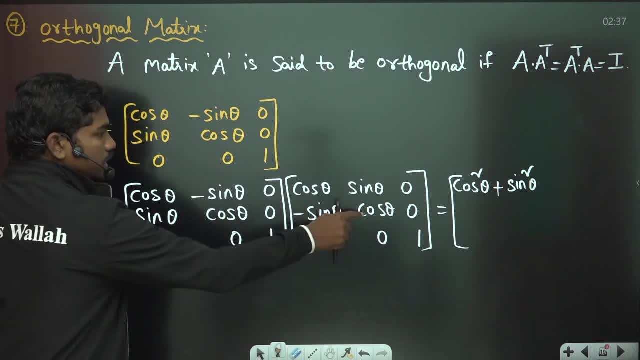 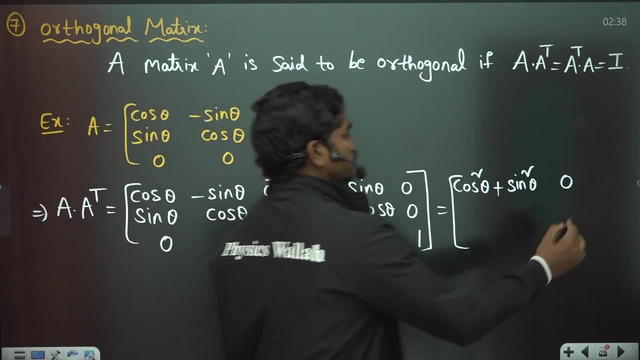 cos theta into sine theta plus minus sine theta into cos theta. so this is cos theta sine theta minus sine theta, cos theta, which is 0. next third row, so the first row with the third column, cos theta into 0, minus sine theta into 0, 0 into 1, so total 0. so this is how we have this next second row, first column, sine theta into cos. 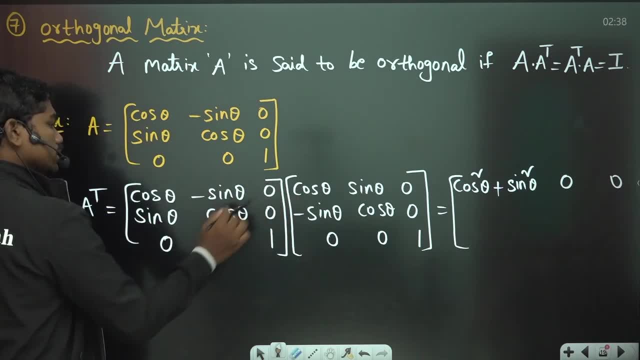 theta plus cos theta into minus sine theta. so this is sine theta cos theta minus cos theta sine theta, and that gives you 0 directly. now second row, second column: sine theta, into sine theta, sine square theta plus cos theta into cos theta cos square theta. so again you got here. 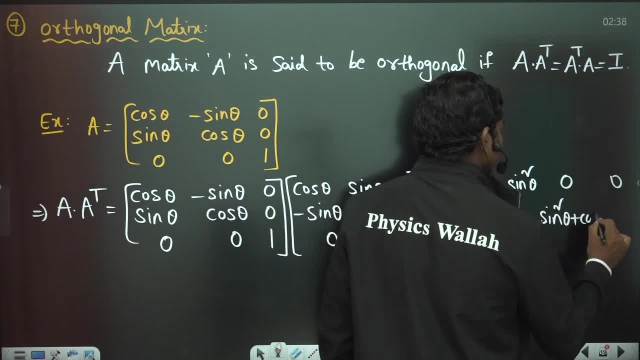 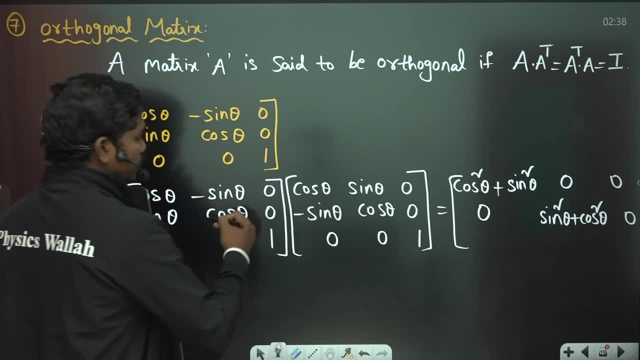 sine theta into sine theta, sine square theta plus cos theta, into cos theta, cos square theta. so going to have, as you see, if it is 0 here and just here, 0 here, sin square theta plus cos square theta. okay, next second row, third column: again, it is 0 directly. now, third row, first column, those 2. 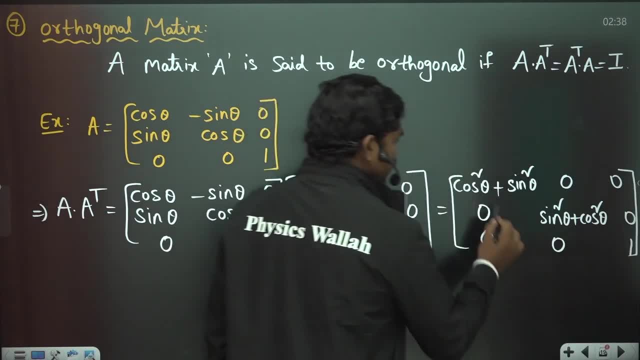 inner zero's 1 into 0, 0 for the term zero, and finally here we have 1 to 1. this is 1, so sine square theta plus cosه d theta is always 1, irrespective of the theta value. so zero, 1 and 0ê 1. 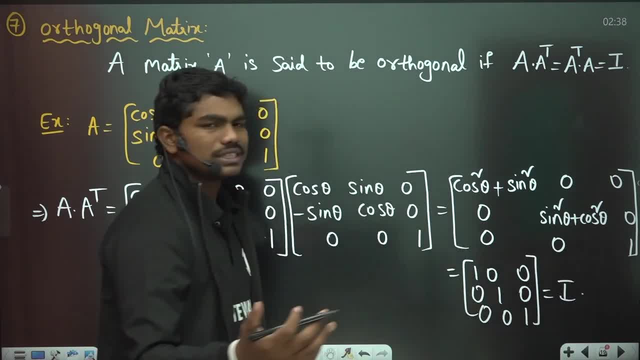 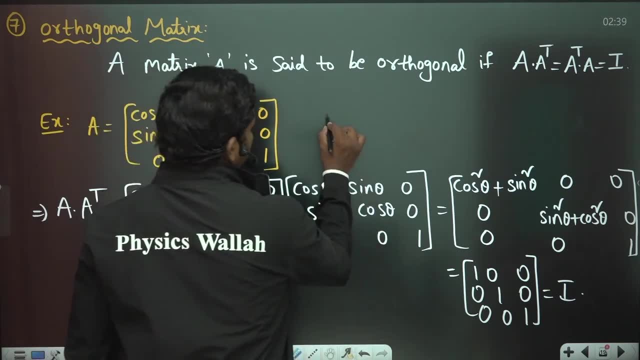 4 00 1, which is actually an identity matrix. now, if you want more examples which can change the, you can do one thing: whatever you can put, you can generate a matrix by putting different values of theta. let us suppose, if i put theta equal to zero, let theta is equal to zero, then i'll get one. 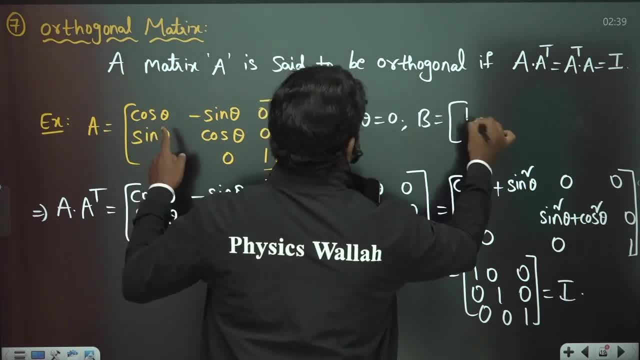 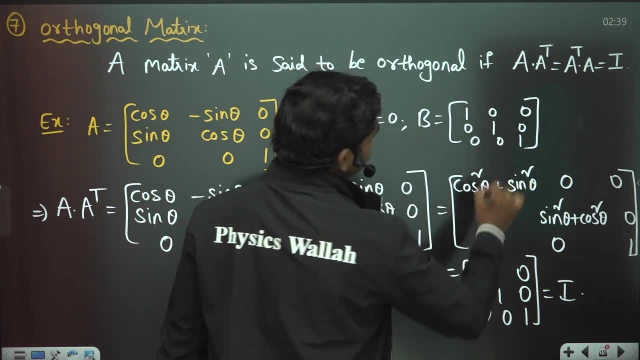 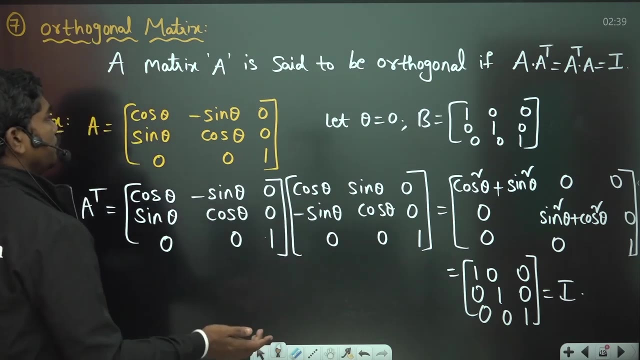 matrix that b is equal to cos zero. one sine zero, zero, zero. this is zero, then this is one. this is zero, zero, zero one. so i'll get identity matrix, and identity matrix is again one. uh, you know one of the orthogonal matrix. if i put theta is equal to some 90 degrees, for example, then you'll get. 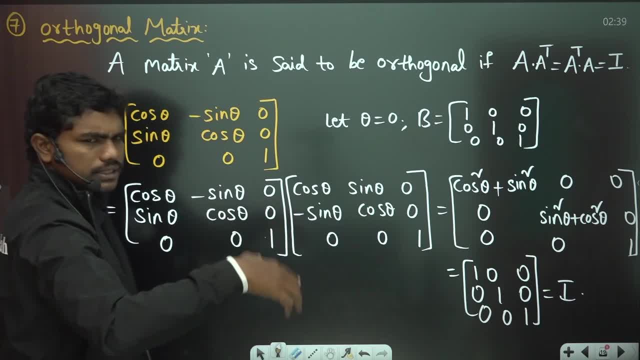 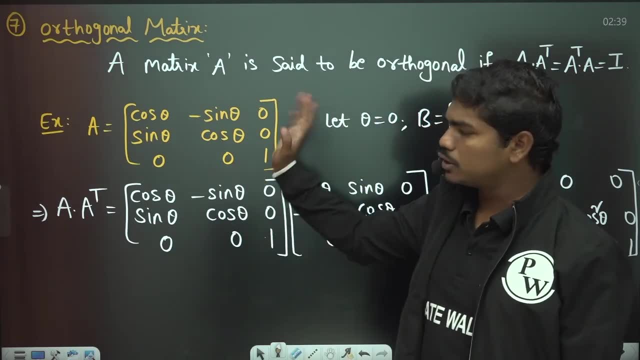 a zero minus one, zero one, zero, zero, zero, zero one. that's again one more orthogonal matrix. so you can. if you want to generate n number of orthogonal matrices, you can just go for some n values of theta. whatever the value of theta you put for this particular configuration, you always. 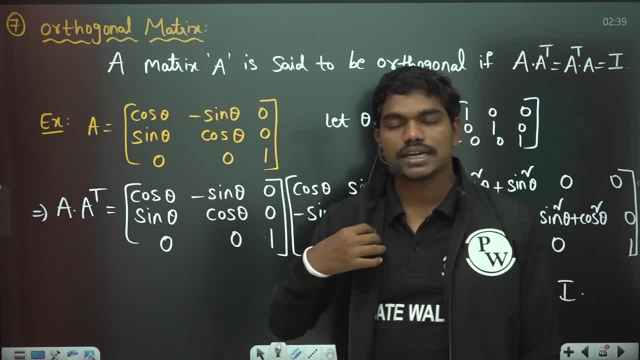 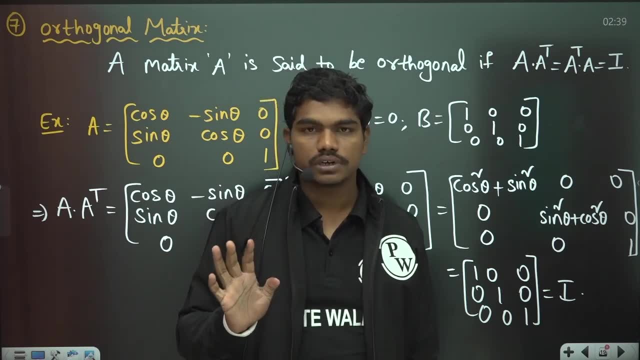 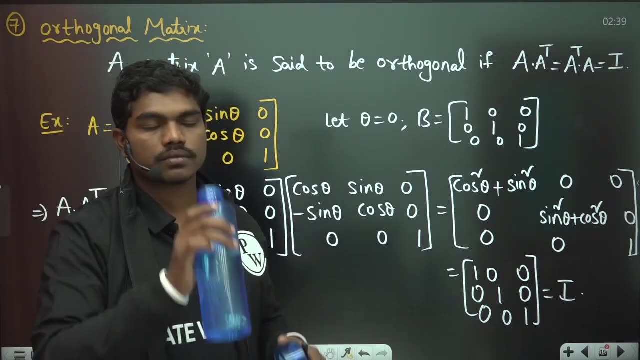 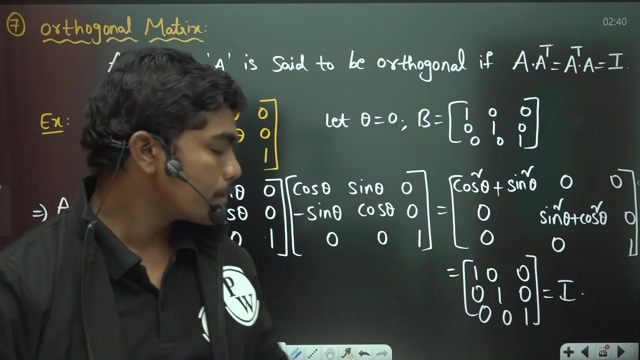 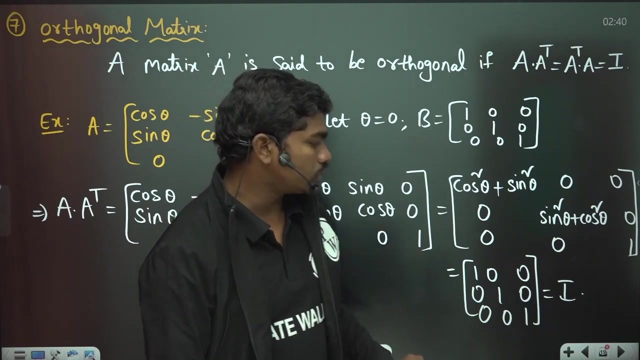 end up with an orthogonal matrix- clear. so orthogonal matrix is that matrix which, when you multiply with its transpose, you always get an identity matrix. okay, and this example, i hope it's clear to you. let me have some water, you okay? so let's continue. so this is orthogonal matrix. now i would like to give you one more. 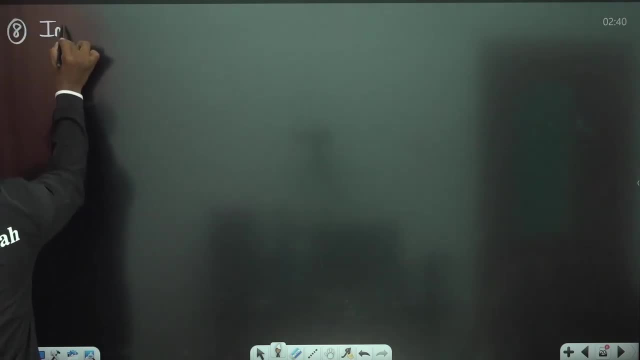 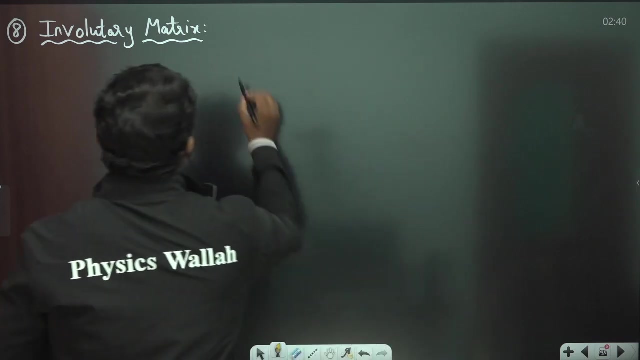 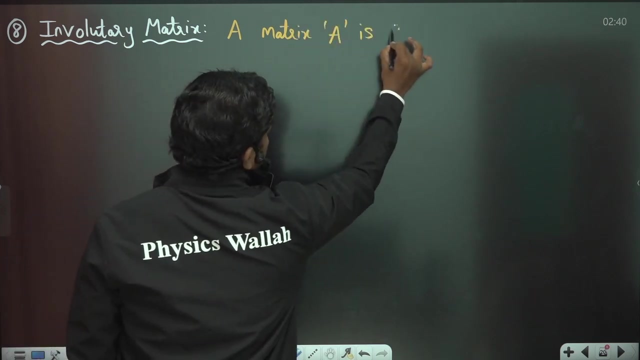 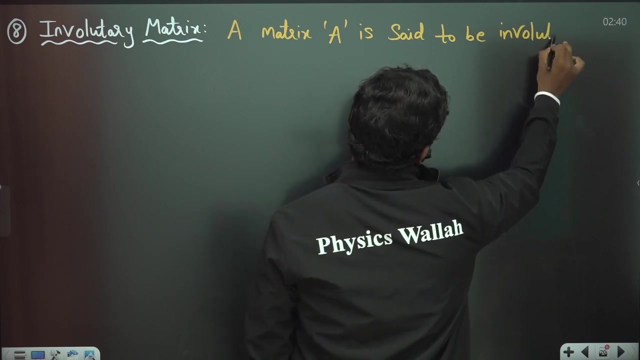 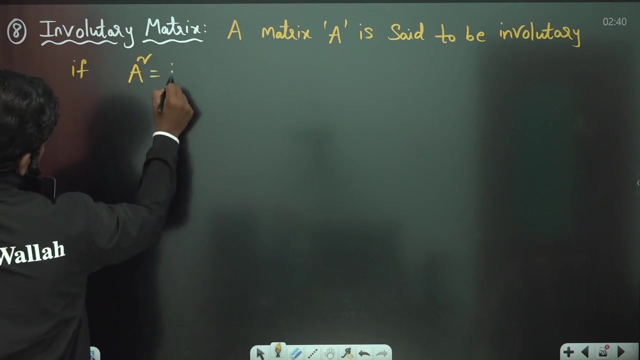 important matrix which is invalutimatics, invalutimatics, invalutimatics. so in this, if you see invalutimatics, a matrix, capital a is said to be invalutary. invalutary if a square is equal to i, which means if you. 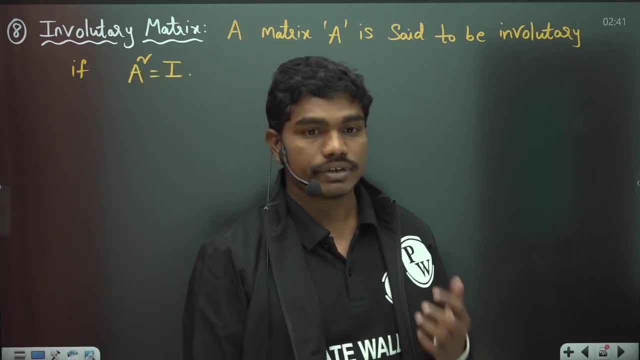 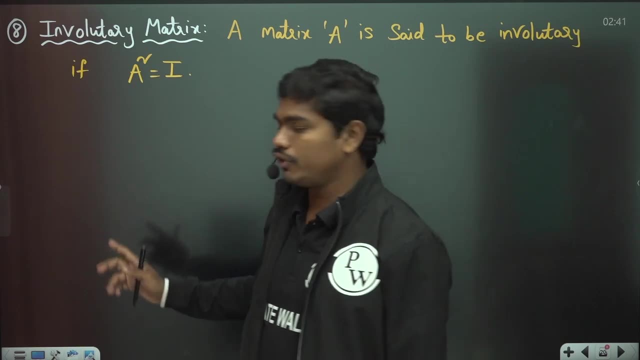 square any matrix, you will get the identity matrix of same order. and for getting this, this here need not be an identity matrix. there can be some different matrices okay where if you do a square, you will get i value. let us see how you get this. you know, many times i'll be looking. 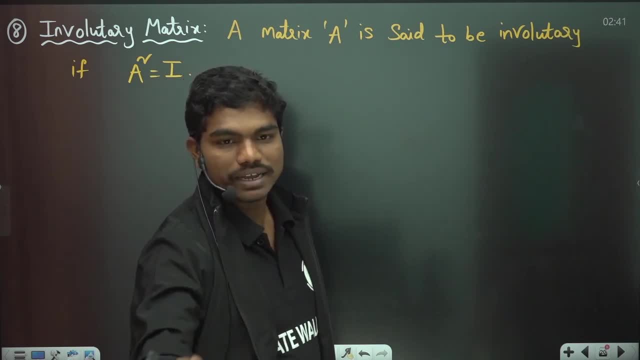 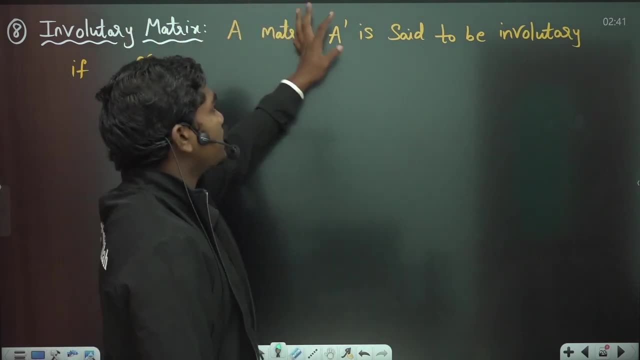 downwards because i have the system here. so if there is some issue with the mic i'll get to know. okay, otherwise, this recording you know there is, it's not a live class, so i don't know what's happening. so, anyhow, look here a matrix capital. a is said to be invalutary if a square is equal to i. 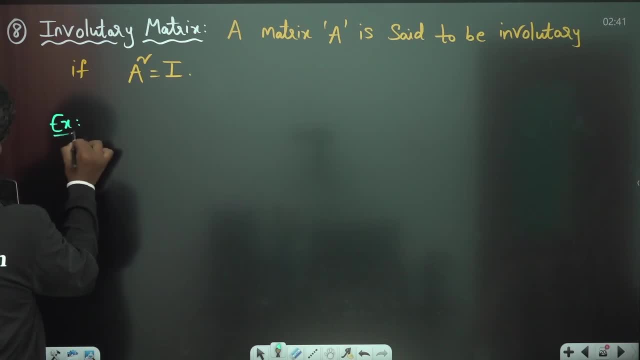 let us see how we'll get this. i'll give you one simple example. a is equal to 4 minus 1. let us keep so. if you keep 4 minus 1, then this is 15, and this is, you know, two times of this, so minus 4. so let us suppose, if you take this example- it's a simple example. 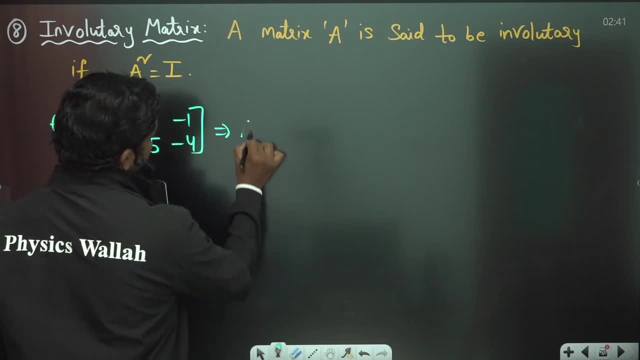 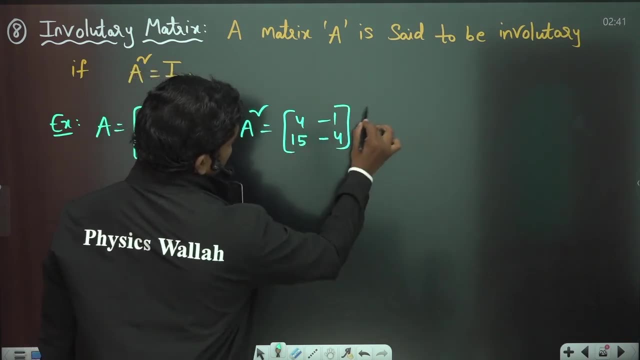 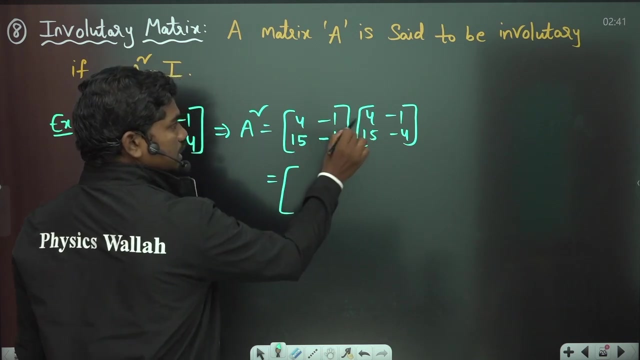 for example: okay, now if you calculate this square, if you calculate the square 4 minus 1, 15 minus 4, and this you know, 4 minus 1, 15 minus 4. so if you calculate this product, you can see: 4, 4s are 16 minus 1 into 5, 15 is 16 minus 15, which is 1. so 4 into minus 1 is minus 4 plus. 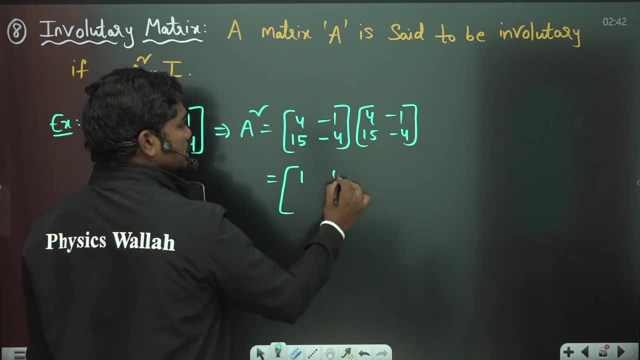 minus 1 into minus 4 is plus 4. so minus 4 plus 4, this is 0, 15. 4s are 60 plus minus 4 into 15 is minus 60. so 60 minus 60. again, this is 0. 15 into minus 1 is minus 15 plus minus 4 into minus 4 is. 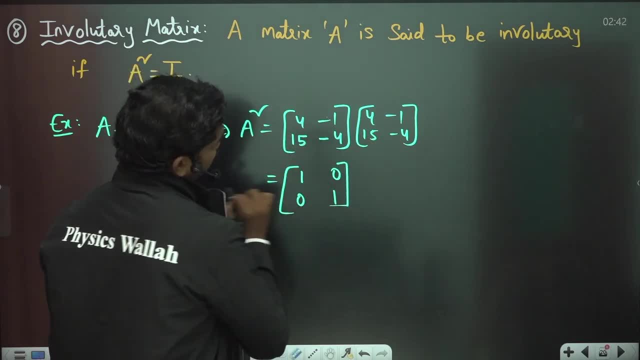 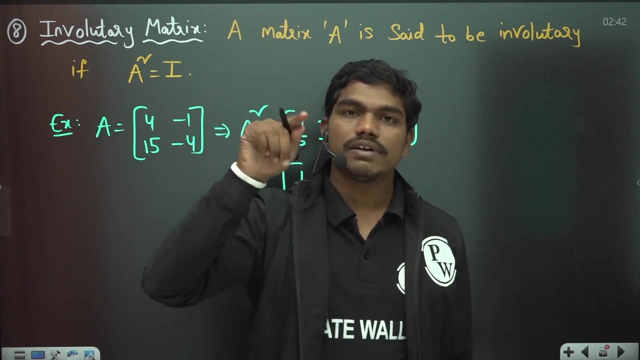 plus 16, so 16 minus 15, this is again 1. so if you see this matrix, if you see this matrix, if you see this matrix is an- uh, you know, basically involute matrix. so i would like to give you one very good property here. sometimes they give you that let a is equal, let a is an involute matrix, and they 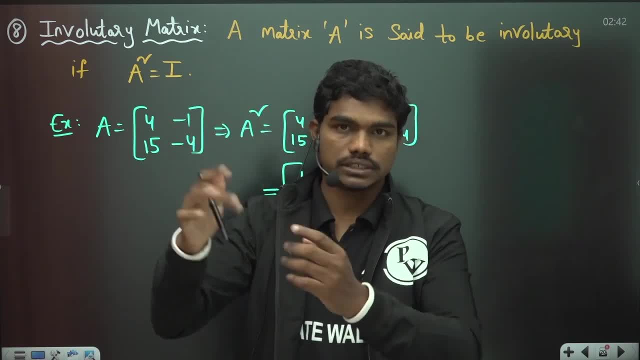 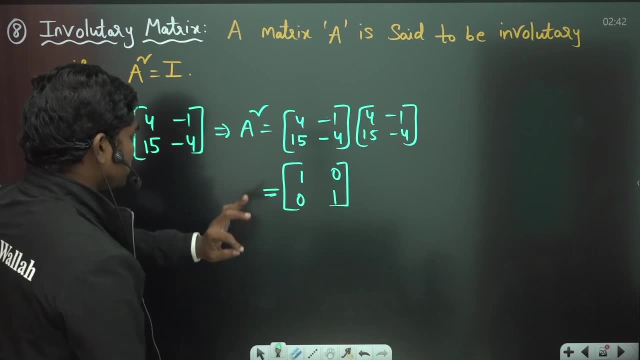 give you some complicated elements inside, but and they'll ask you for a inverse, okay, so we'll talk about how to do in a inverse, simply and all. but right now, if you see, in this matrix there is one very special property that a inverse is basically- again, sorry, a inverse. 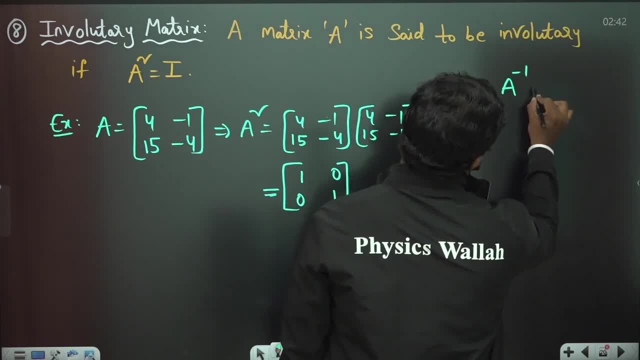 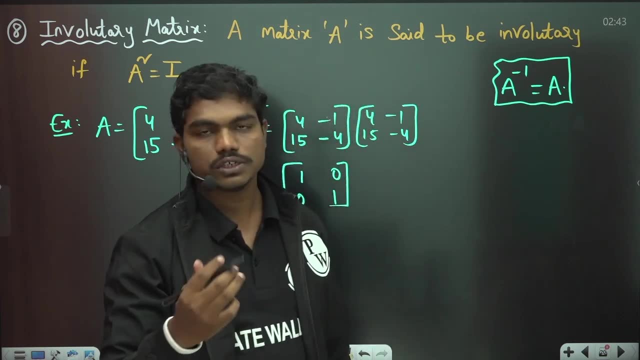 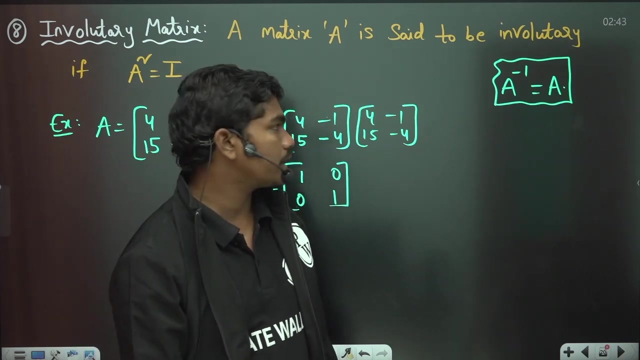 a inverse is basically equal to a. okay, so what happens in that case is whenever you- uh, you know, whenever you, with all the difficulty, when you try to calculate a inverse, finally you try to get the same- uh, you know- matrix as the inverse matrix. okay, and even after getting the same matrix, many of you will 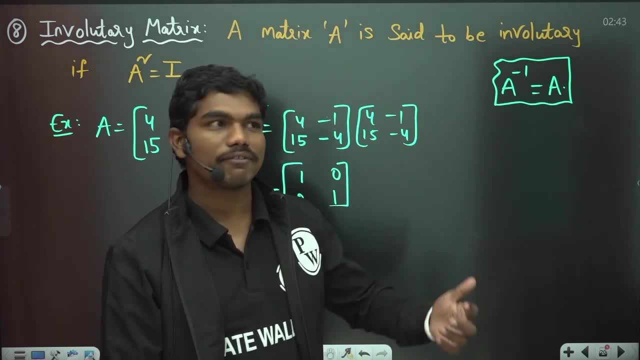 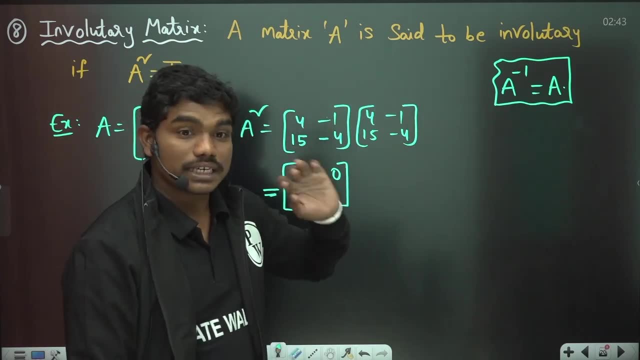 have this doubt that, uh, have i done some wrong calculation or what? i have got the same question matrix. but this is actually the case with this matrix: the inverse of this matrix will be same as the matrix itself. okay, that's why, if you, if you observe, you can tell clearly that you have. 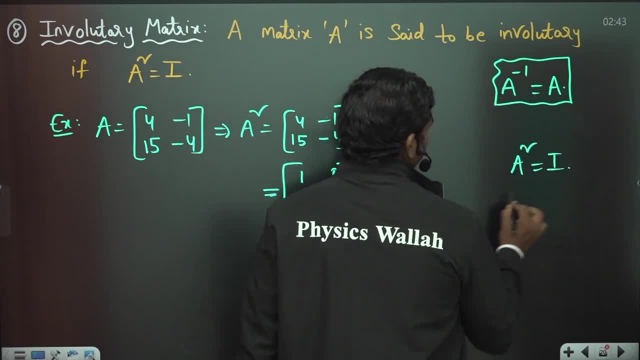 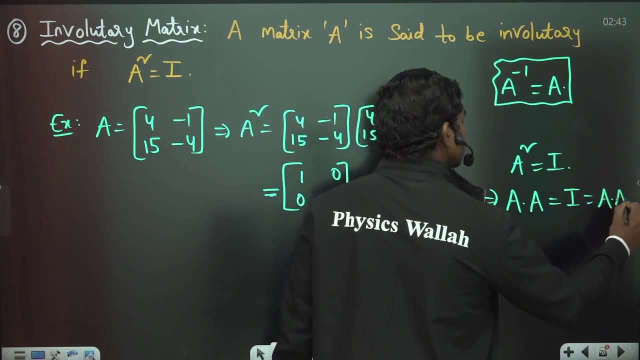 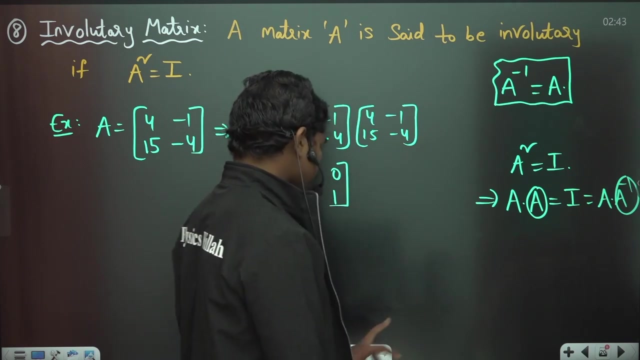 clearly, you know, a square is equal to i, is what you got correct. so a into a is equal to i, but generally, you know this, i can also be written as a into a inverse, right? so that's why, if you compare generally these two matrices, they will be uh, same, of course, okay, so that's why this a inverse is. 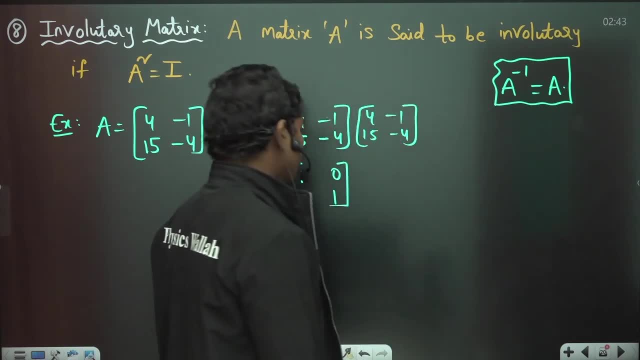 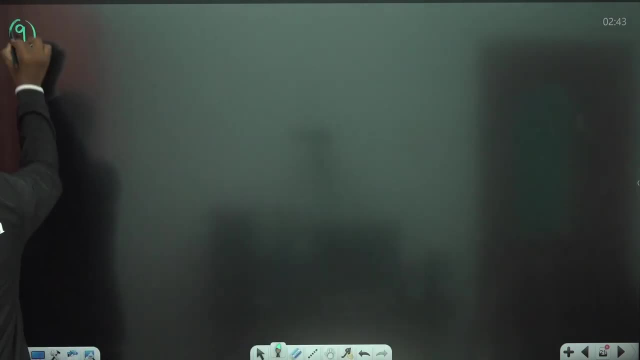 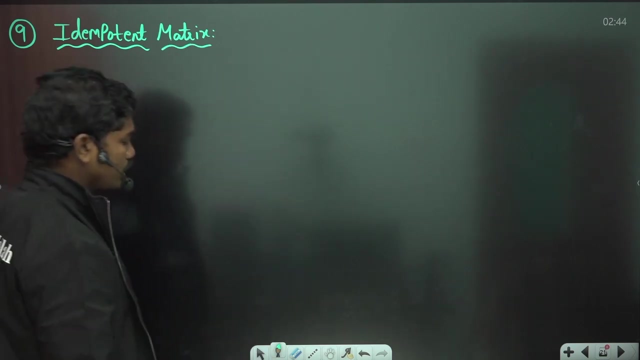 equal to a, in this case clear. so let us go for the next things. so this is involute matrix. now i will give you one again, some good matrix, which is idempotent matrix, idempotent matrix, okay, so what is this idempotent matrix look. 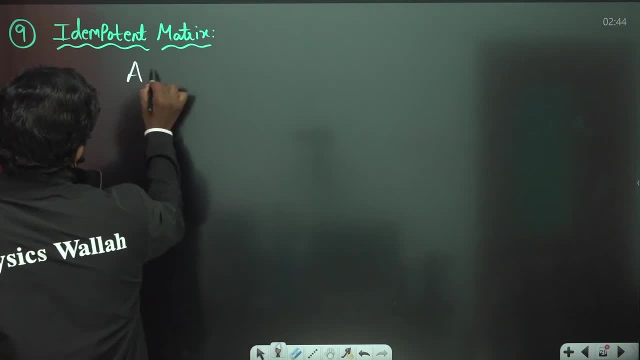 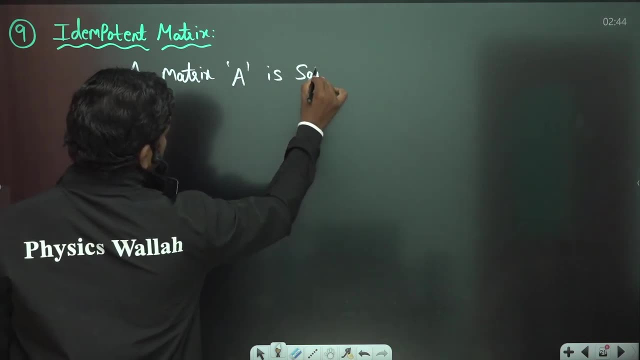 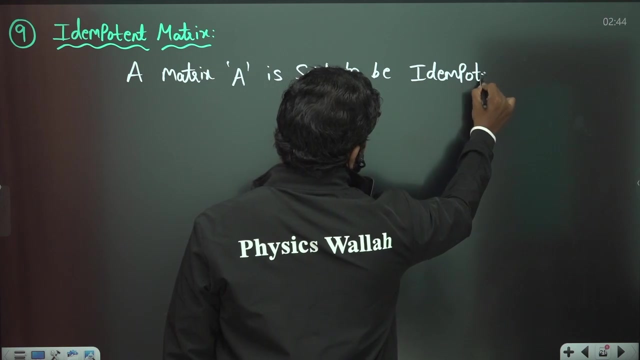 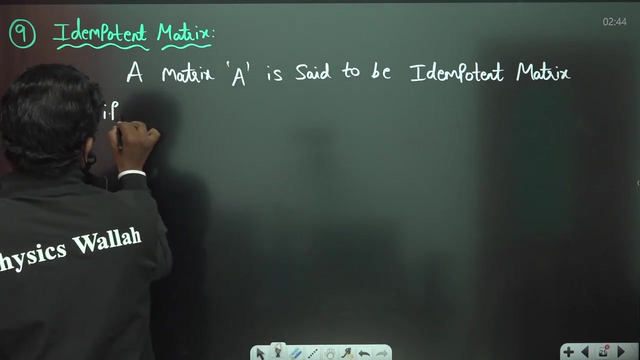 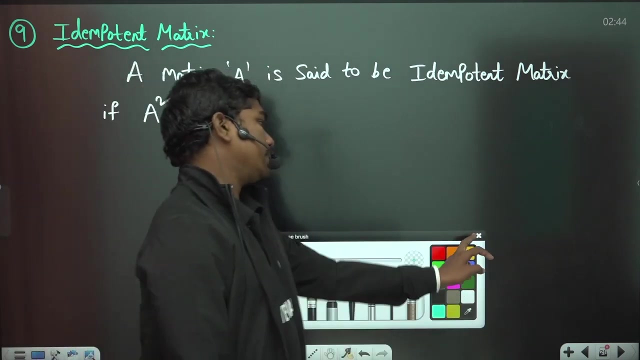 i'll give you a matrix capital: a is said to be idempotent. matrix is said to be idempotent matrix, idempotent matrix. if a square is equal to a, if a square is equal to a here, okay. so look if a square is equal to a. now try to understand. uh. so basically, if you try to square any matrix, you'll 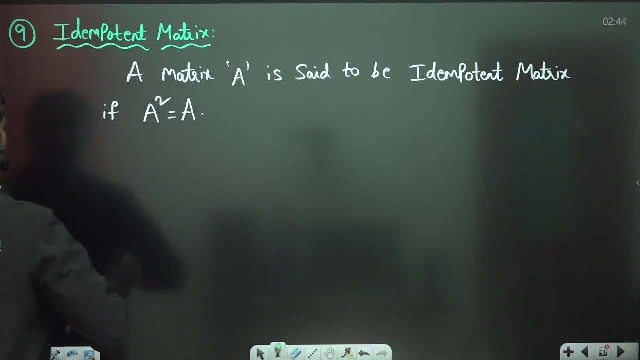 get the same matrix. let us see we can write any example here. example a is equal to. again let us take 4 minus 1 here. 4 minus 1 is this one. can you give me the same example right again? say that this is the cell. 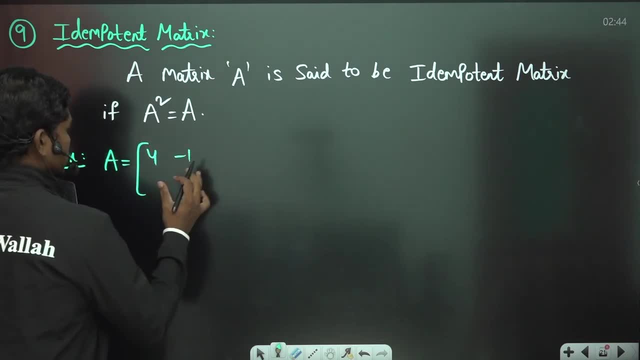 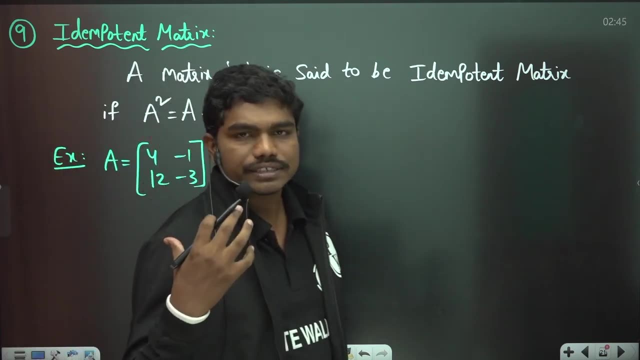 minus 1 here, for example. so if you take 4 minus 1, this any multiplication, for example, 3 times, you write so 12 minus 3, for example. so if you take this matrix, okay, all these matrices, why i am talking? because they have certain properties in determinants. okay, so in determinants, if i say the 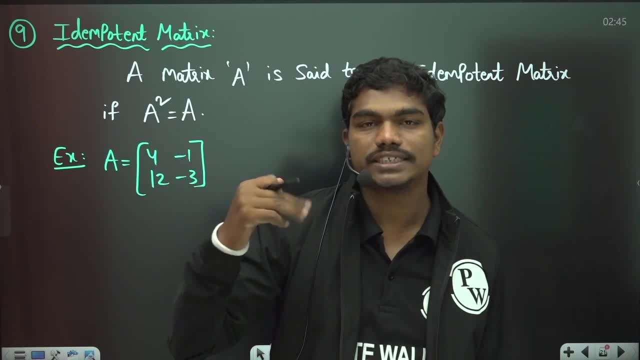 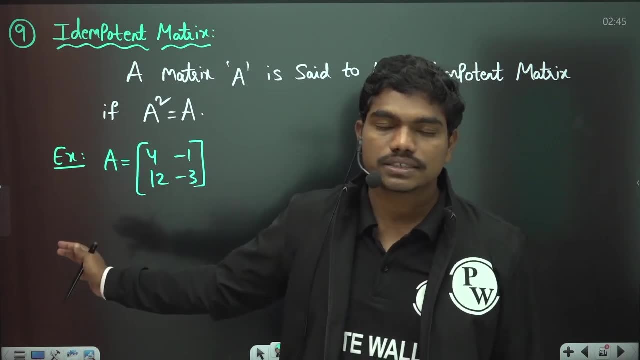 determinant of an orthogonal matrix is plus or minus 1, you should know what is orthogonal matrix by that time, okay, similarly, if i talk something about determinant of an idempotent matrix, you should know what is idempotent matrix. so that's why these matrices i'm discussing now, and of 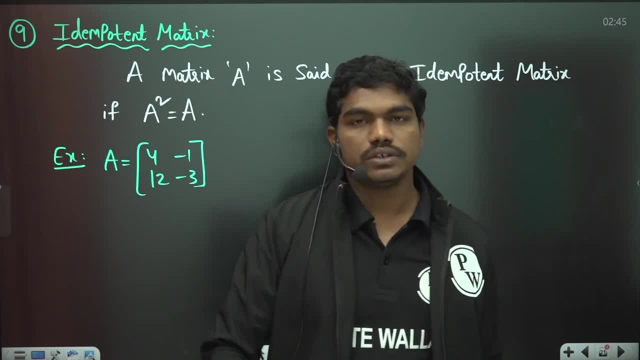 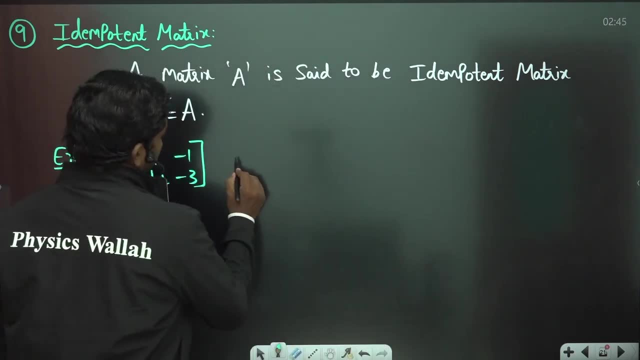 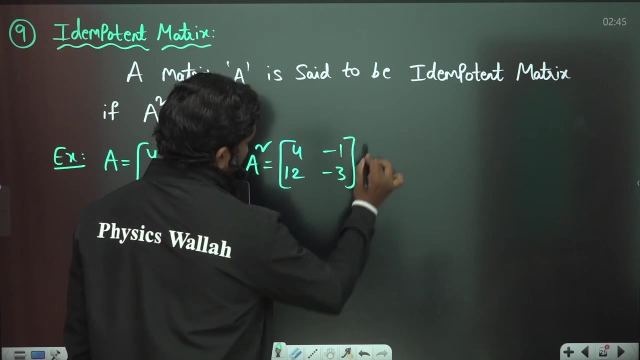 course, there are many gate questions on this types of matrices, okay, which you will come to know later in the pyqs solving sessions. so, anyhow, let us come here. so 4 minus 1, 12 minus 3. so this implies, if you calculate a square, for example, 4 minus 1, 12 minus 3 and 4 minus 1, 12 minus 3. 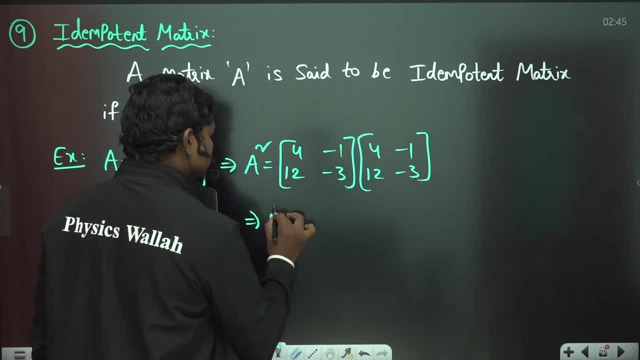 so if you multiply this, a square is going to be equal to 4: 4, so 16 plus minus 1, into 12 minus 12. so 16 minus 12 is 4: 4, so 16 plus minus 1 into 12 minus 12. so 16 minus 12 is. 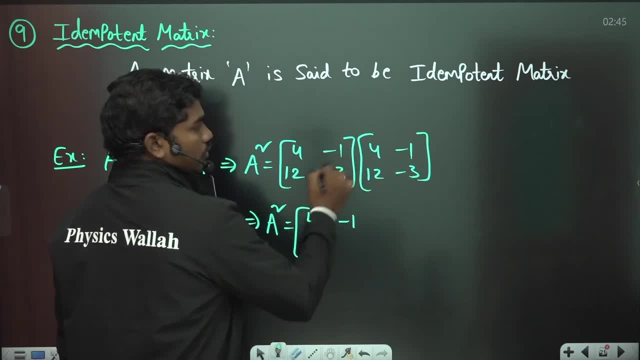 4: 4, so 16 plus minus 1, into 12 minus 12. so 16 minus 12 is 4 again. so minus 4 plus 3, it's minus 1, 48 minus 36, 12 minus 12 plus 9 minus 3, so this is again. 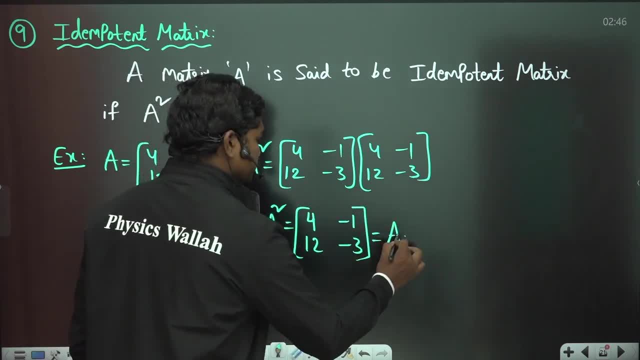 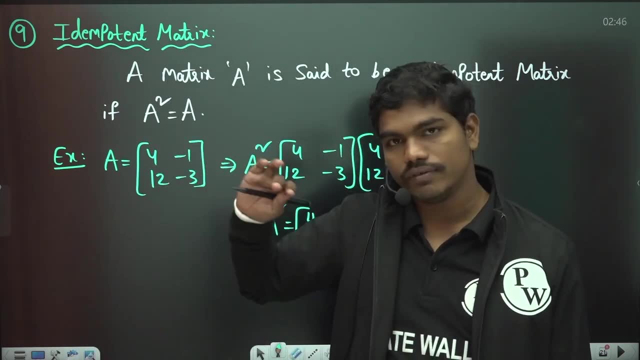 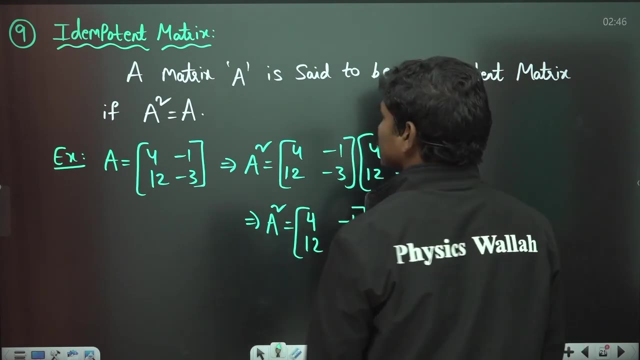 equal to a. okay, so this is how you get this matrix, which is this idempotent matrix, actually here. okay, because i will talk about some properties of this matrix again when i come to the, you know, determinants. actually, okay, so now let us go ahead, and i would like to discuss my last type of matrix before i go. 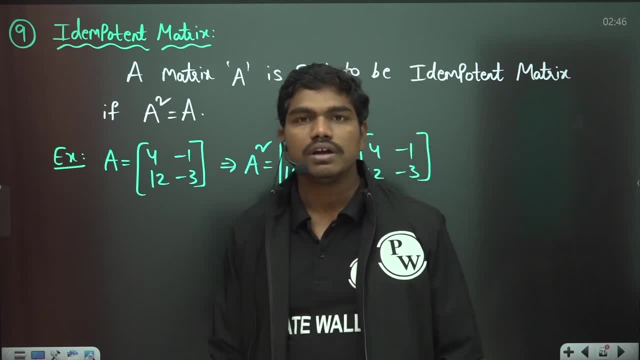 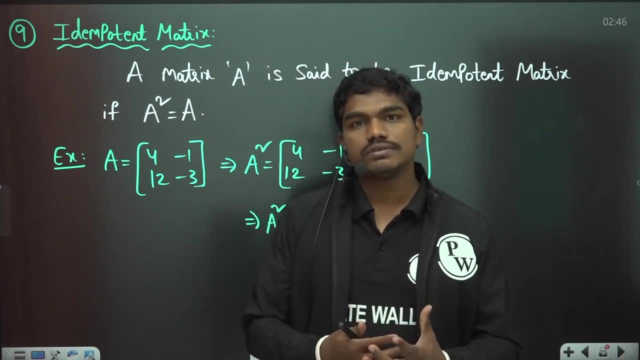 for the determinants. actually, okay, you have seen transpose of the matrix, how we need to identify whether the given matrices are symmetric matrices, geosymmetric matrices. we have seen all these things. okay, now we'll go for one important topic, which is determinant. but before going for the determinant, 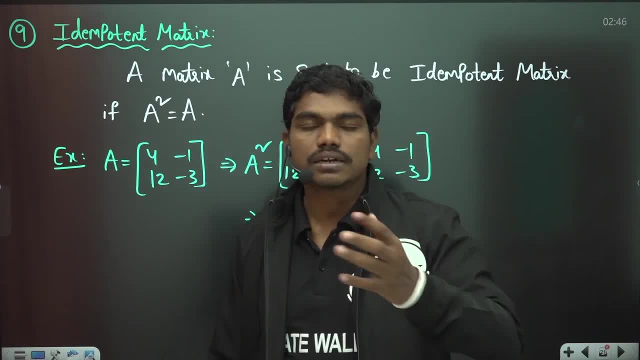 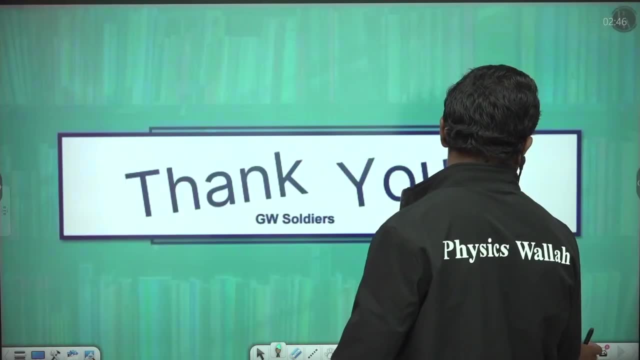 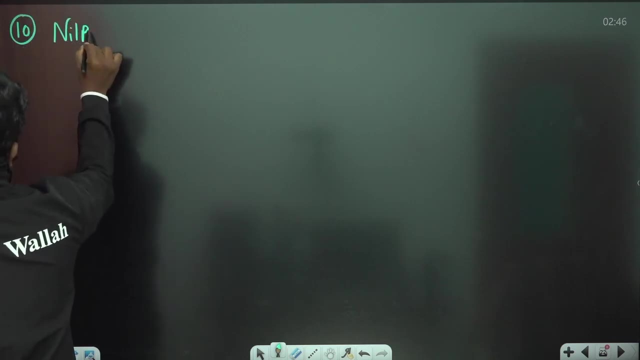 we have one last type of matrix, that of course we have many types, but in gate point of view, i would like to discuss one particular matrix at this point which is actually a, oh, which is actually a new important matrix. you can say nilpotent matrix. so what is this nilpotent matrix? let us see here a non-geomatics. 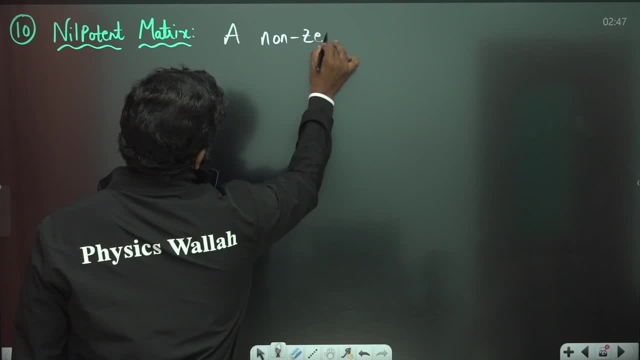 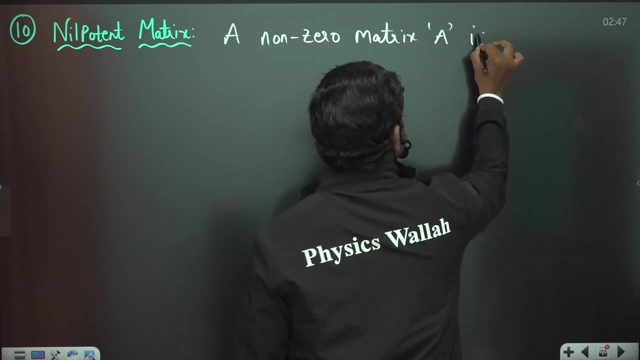 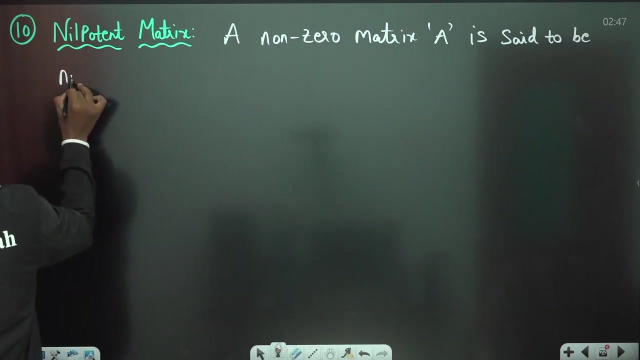 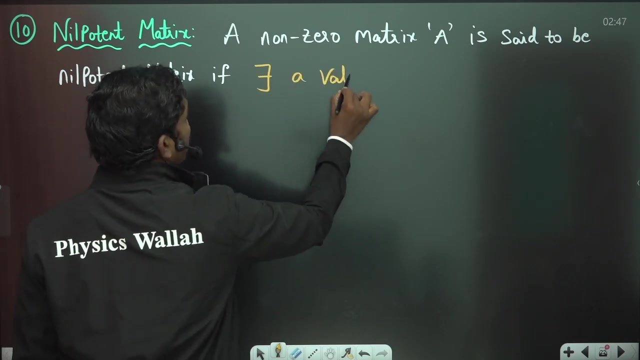 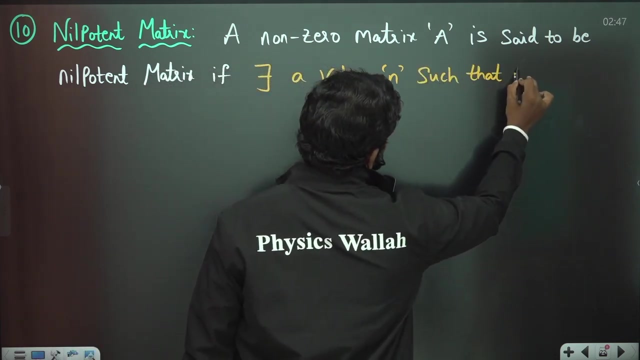 a non-geomatics capital, a is said to be nilpotent. matrix is said to be nilpotent matrix is said to be nilpotent matrix if there exist a value n, a value n such that, such that n belongs to z. plus means, basically, what's the meaning of this? n is a positive. 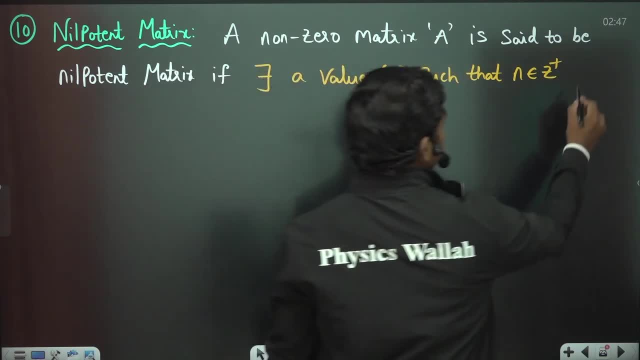 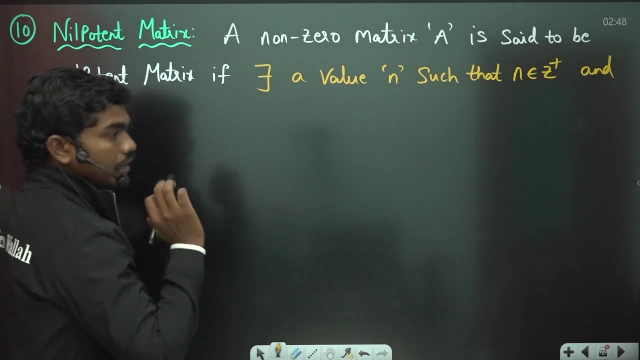 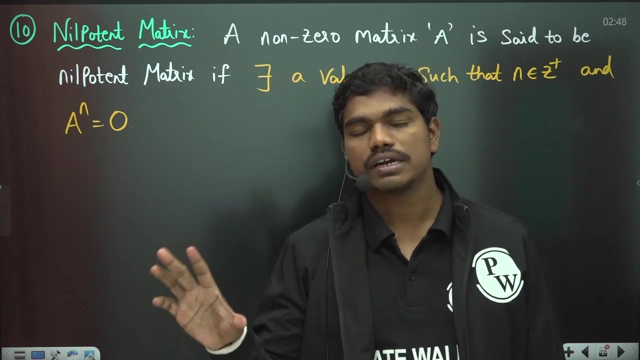 integer. okay, so n is a positive integer and a power n is equal to a null matrix. basically here: okay, so means whenever you take any non-geomatics but some value or some higher power of that matrix is a nilpotent matrix, then you call that matrix as a nilpotent. 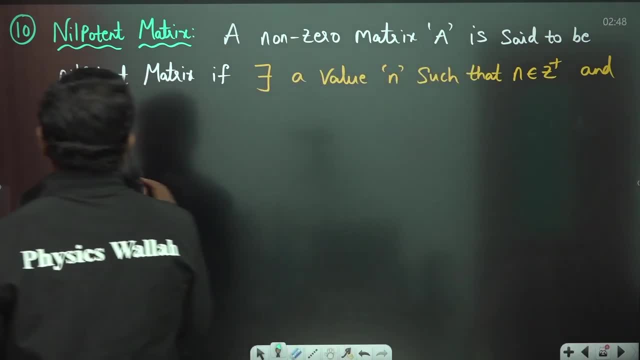 matrix. now let me see what is the case. example a is equal to. so let us take two minus one, and four plus two is zero. power n is a zero matrix and nilpotent matrix at n. this value here isnt equal to zero matrix. so a power n is naprawdę ripens. take nilpotent matrix, then you make it nilpotent matrix, and so on. everywhere you call that matrix, then you call that there space matrix. ok, now let me the fram. 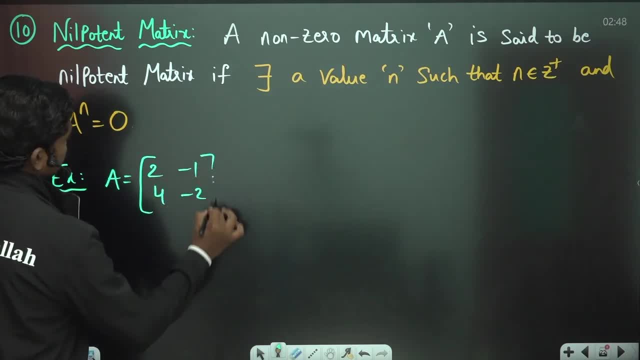 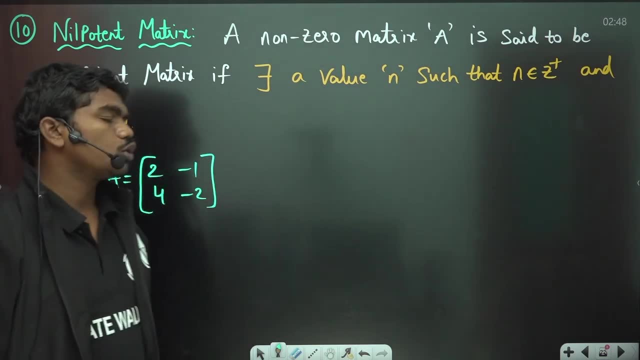 take 2 minus 1 and 4 minus 2, for example. let us say, okay, fine, good enough, so 2 minus 1 and 4 minus 2, for example, if you take this: uh, just in check, so 2 times of this. okay, fine, yeah, 2 minus. 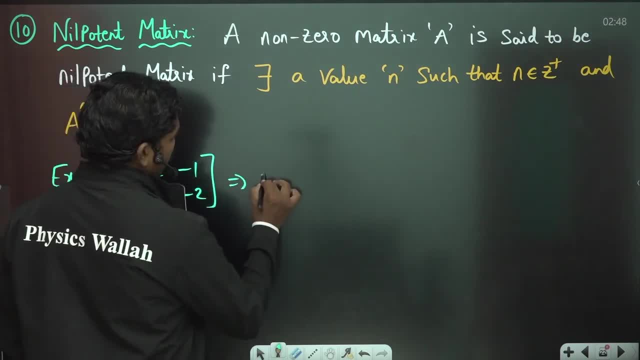 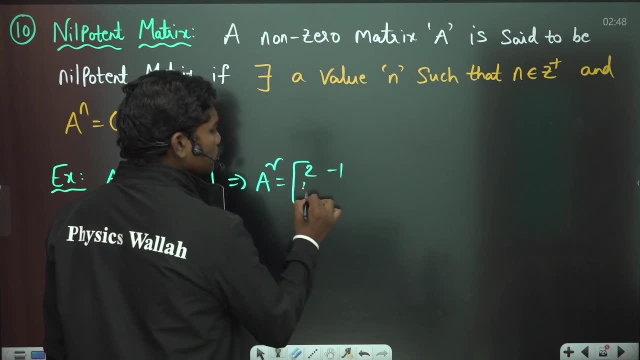 1 and 4 minus 2. now if you calculate this a square, you see this is a non-zero matrix. but if you multiply this matrix to itself- 2 minus 1- i'm dealing in 2 by 2, so that calculations will be easy. the same can hold good for 3 by 3s, also 4 minus 2. so a square is equal to now, if you. 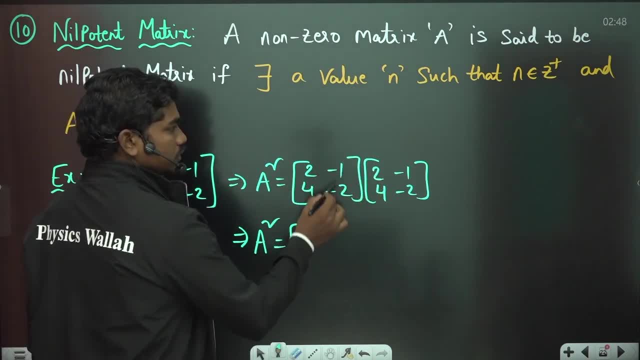 multiply 2. twos are 4 plus minus 1 into 4 is minus 4. so 4 minus 4, 0, 2 into minus 1 minus 2 plus minus 1 into minus 2 is plus 2. so minus 2 plus 2, 0, 4 twos are 8 plus minus 2 into 4 is minus 8, 0, 4 into. 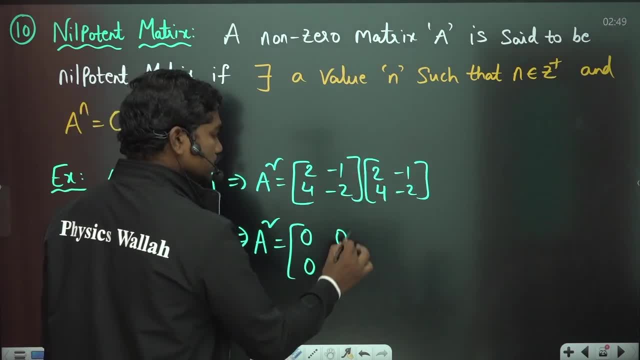 minus 1 minus 4 plus minus 2 into minus 2 plus 4, which is again 0 here. so if you see, this is a non-zero matrix. so if we see, this is a non-zero matrix. so if you see, this is a non-zero. 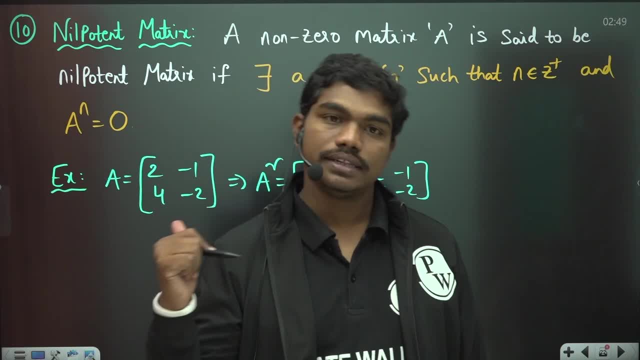 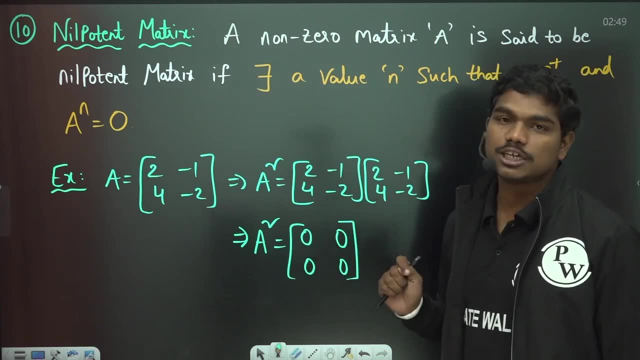 this: a square is a null matrix, but actually a is not a null matrix. okay, this is again in evidence to that result, what i have given there- that product of two non-zero matrices can be still a zero matrix. okay, so that's why you can see this is the case. and here i would like to add one more. 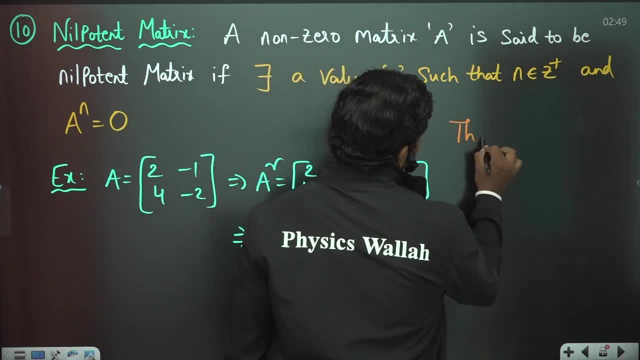 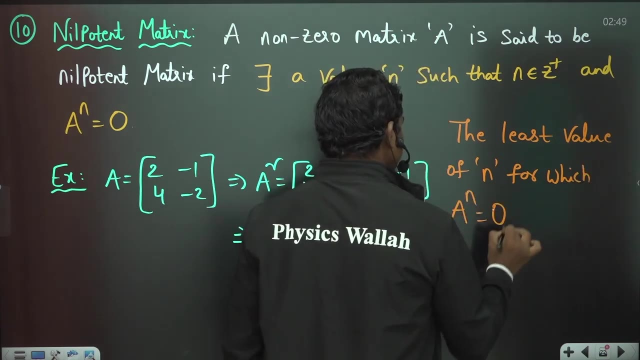 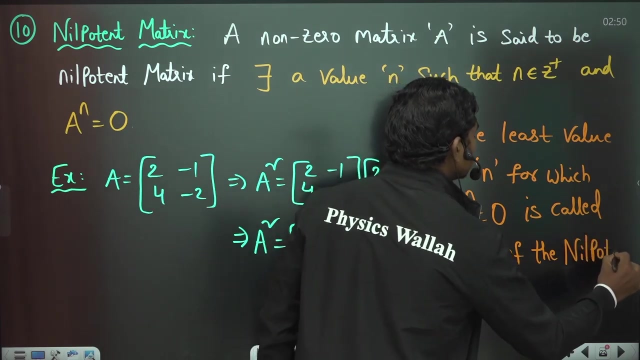 point, because you know it's a good point- the least value of n, the least value of n for which, for which this a power n is equal to this null matrix, is called, is called index of the nilpotent matrix. index of the nilpotent matrix. okay, so this is called nilpotent matrix. 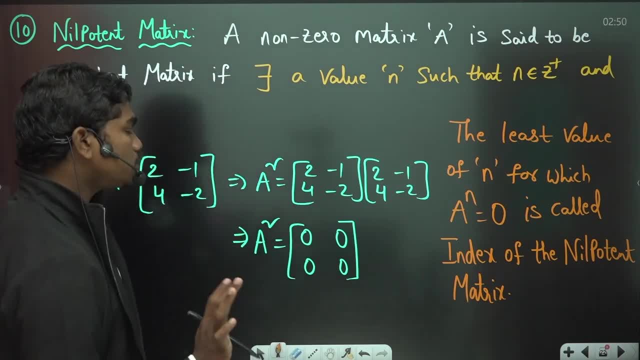 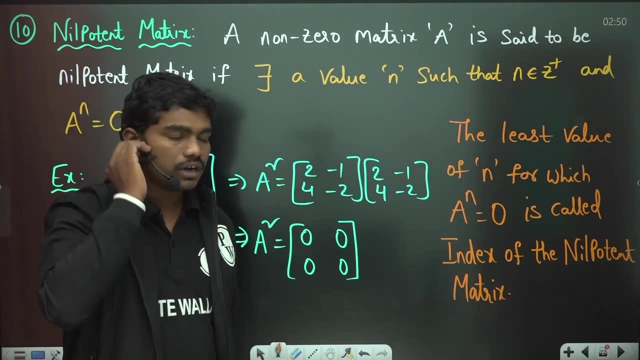 is called index of the nilpotent matrix. now try to understand one thing, because if a square is zero, then definitely from next onwards every power will go to zero. a cube, a power four, a power five, all these things will be zeros, because a cube can written as a square into a, so a square is zero. 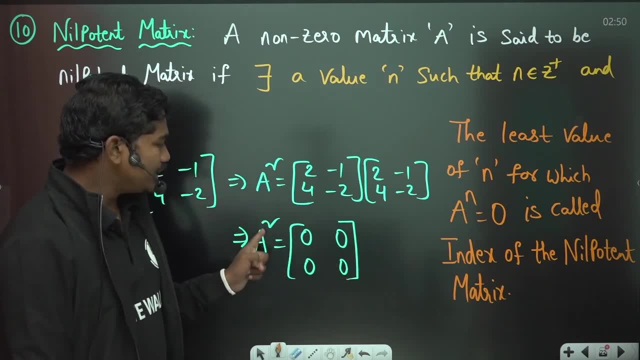 a cube is also zero. so all this goes on, but two is the first time. this, whenever this n is equal to two, this is the first time when a power n becomes zero. so index of this matrix is actually two. clear for some matrices you can have the four. what can be the? 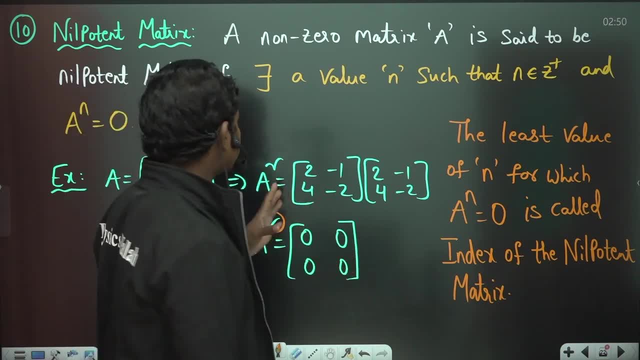 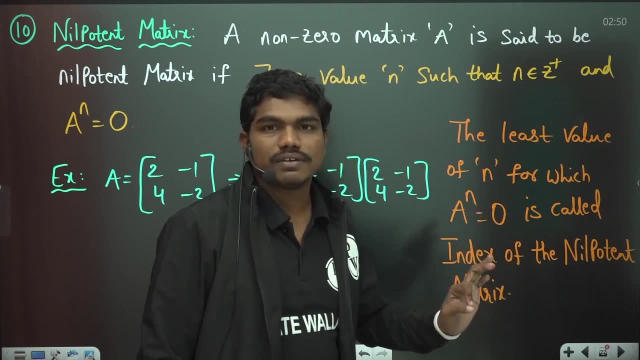 uh, depending on the type of matrix, but here the right now, this is called this, uh, you know, nilpotent matrix basically, and this value, the least value of n, for which this a power n turns out to be a null matrix for the first time, is called index of this nilpotent matrix. 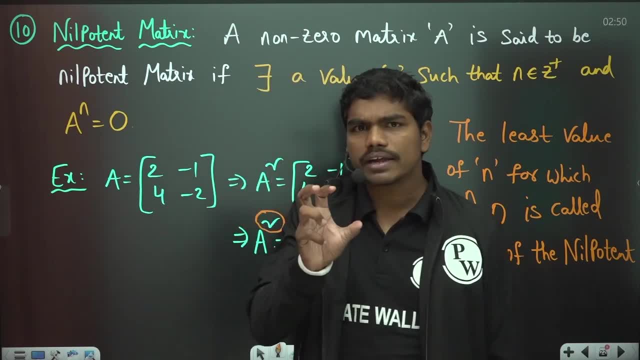 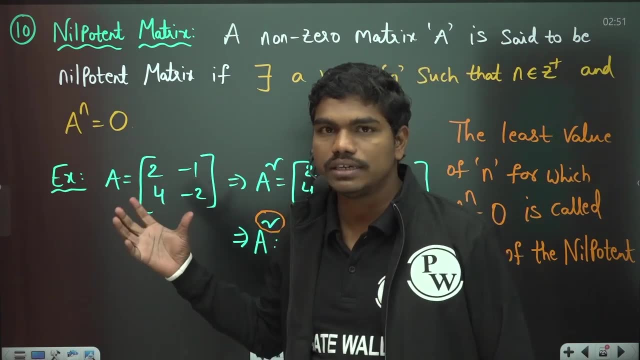 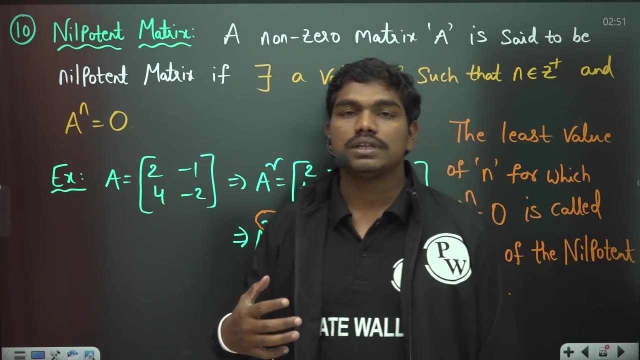 okay. so with this we finish this first part of this video. like, uh, types of matrices and basic matrix, algebra, multiplications, additions, or you can see some types of mad, a symmetric matrices, or nilpotent, orthogonal, all these things, okay, check, theo, Okay. so now, next, we'll move on to the second part of this video, which is the talk about determinants. 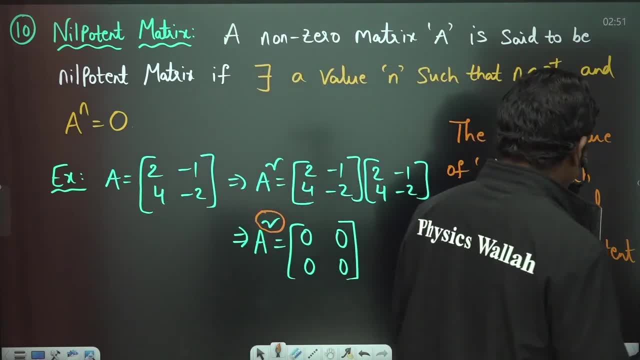 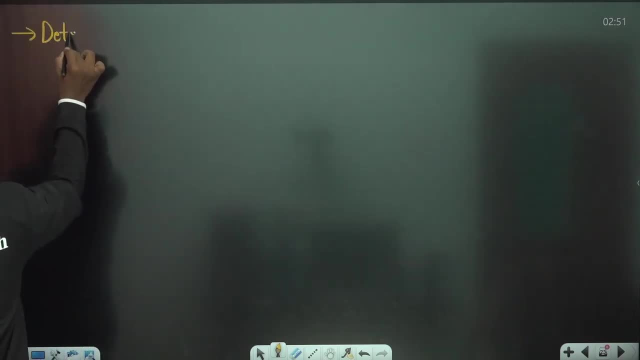 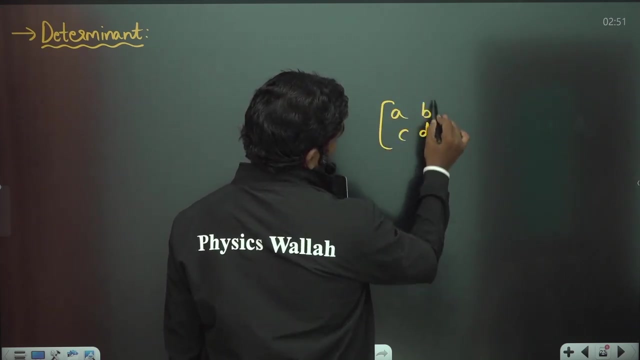 Okay, so let us go ahead and let us discuss the concept of determinants, determinants, determinants, determinants or determinant. You can say now, if I ask you, for example, if I ask you if this is a matrix and if I ask you, what is the determinant of this matrix? 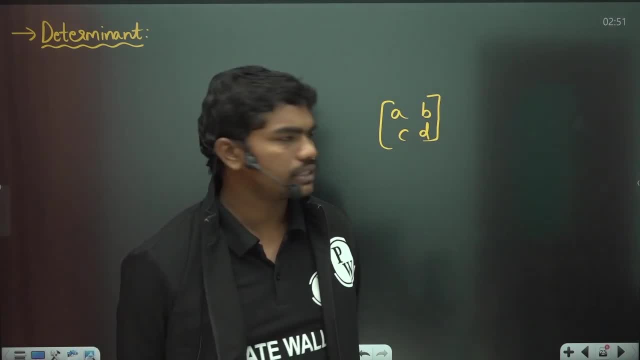 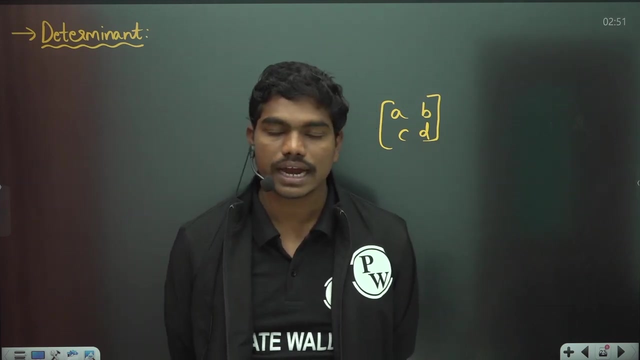 Okay. so immediately you start telling ad minus bc, cut a into d, minus b into c. But if you observe the question carefully, I didn't ask you what is the value of the determinant, I asked you what is determinant. Okay, so you should definitely know, because even this question, I'll tell you one of the experiences that I had recently. have you know. 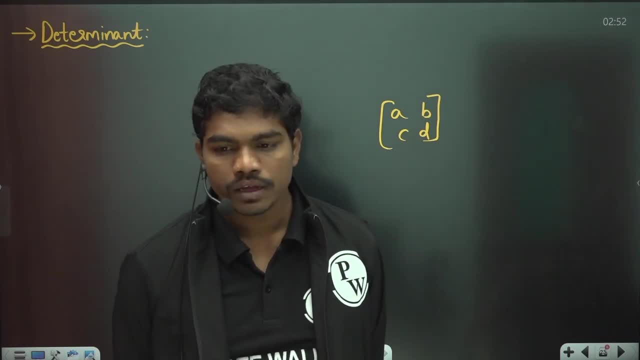 appeared For BRC interview also. so now I'll tell you one thing: in every interviews, generally in technical interviews, there will be one faculty from one, you know, interviewer from maths, actually from mathematical background, and they'll try to ask you some. 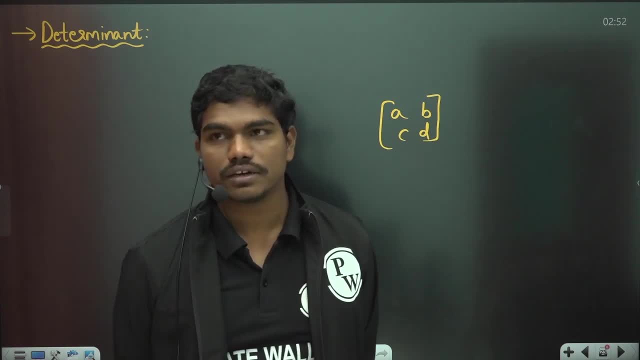 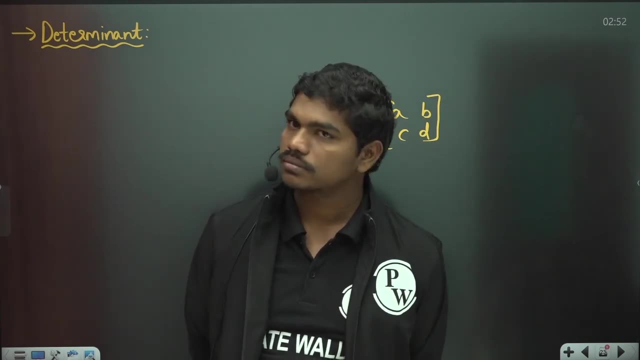 questions. So you prepare a lot of things in mathematics and you go for the interview, but finally they ask you what is determinant and you'll end up with telling the value of the determinant Okay. so that's why this understanding of the concept of determinant is actually very important. 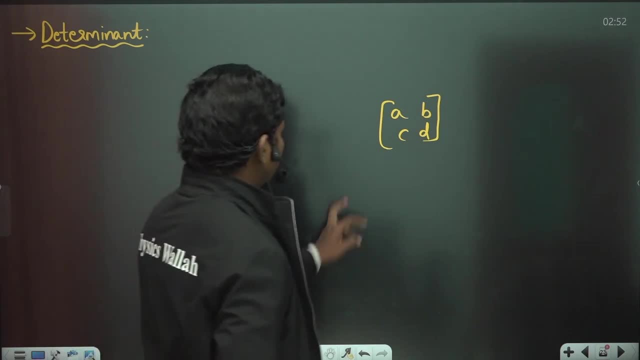 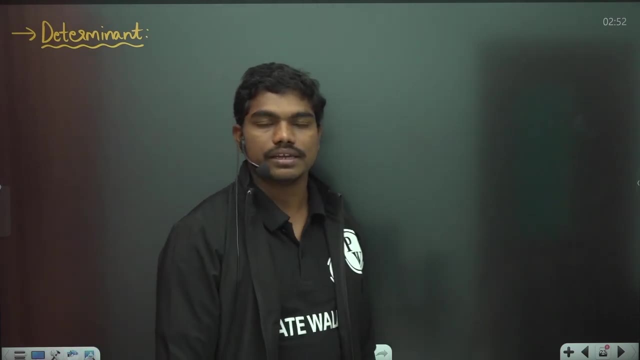 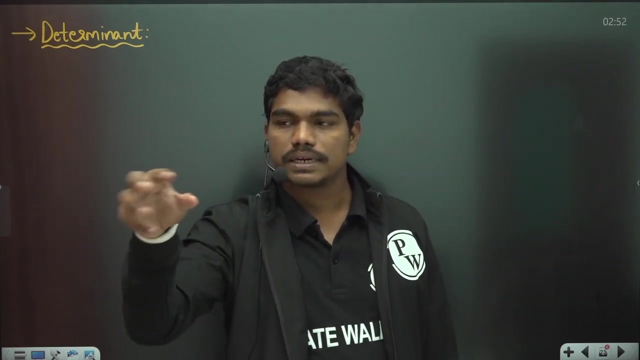 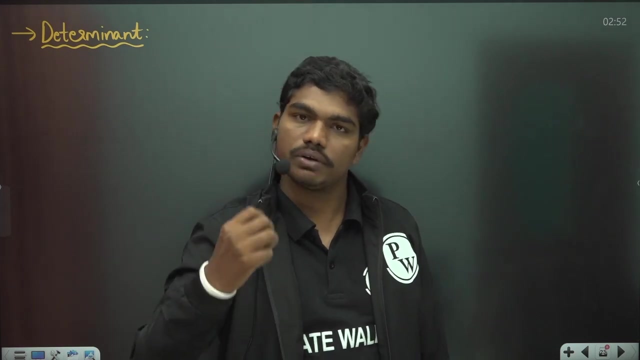 Okay, so now let us see. what is this determinant Actually? look, I'll define the definition formally and then we'll see what's happening here. Okay, and you know, whenever you're trying to calculate a three by three determinant, you let first term minus second term plus third term means between every terms you're you're actually alternating the plus minus sign. why you are alternating this plus minus sign. okay, we'll see all these things in this. you know part, look so determinant: the sum of 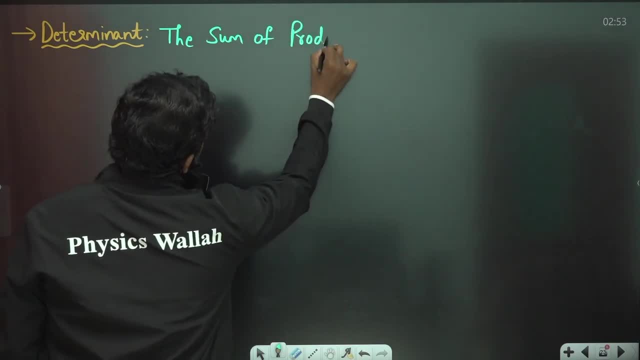 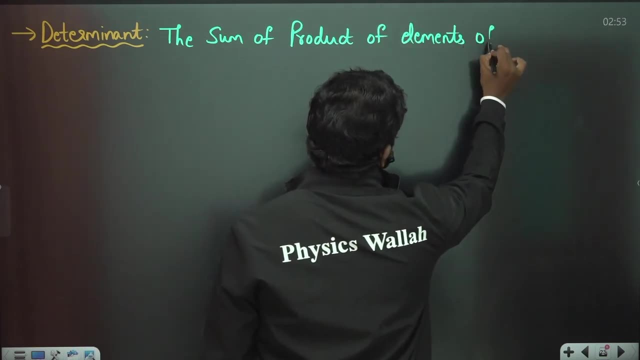 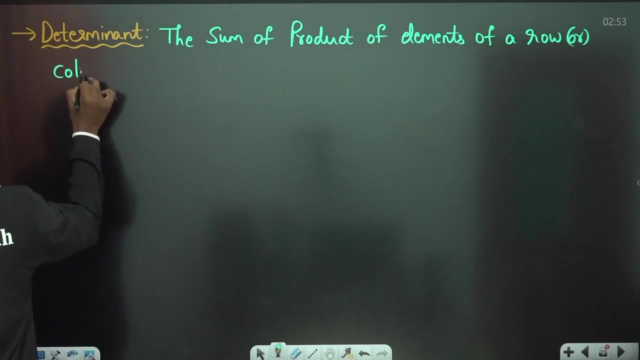 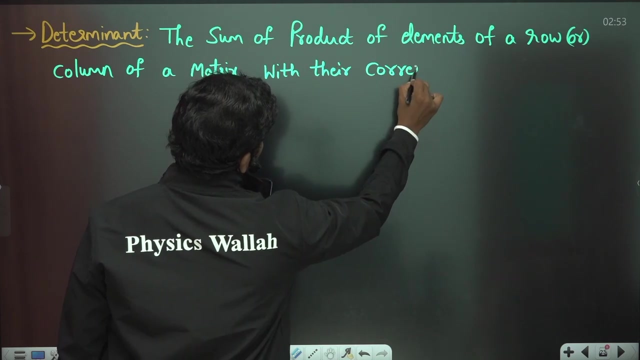 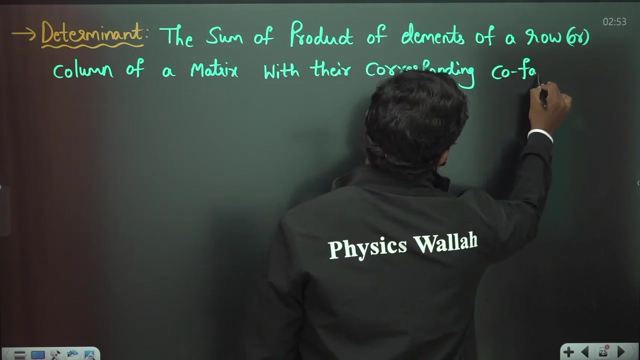 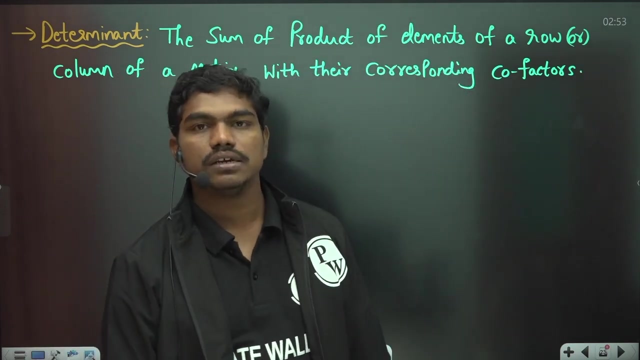 the sum of product of elements, product of elements of a row or column of a matrix, of a matrix with the, with the corresponding, with the corresponding cofactors, with their corresponding cofactors. So what are these cofactors And what is this definition? basically, product of some of the different things kept. 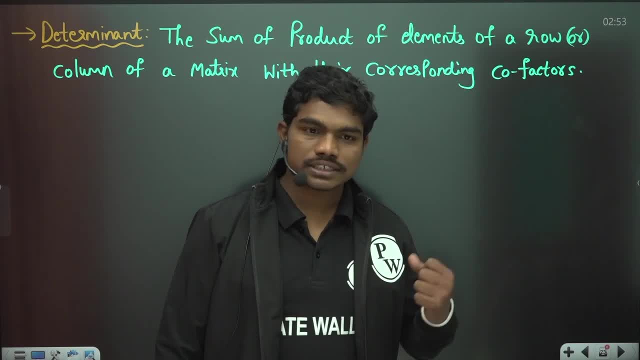 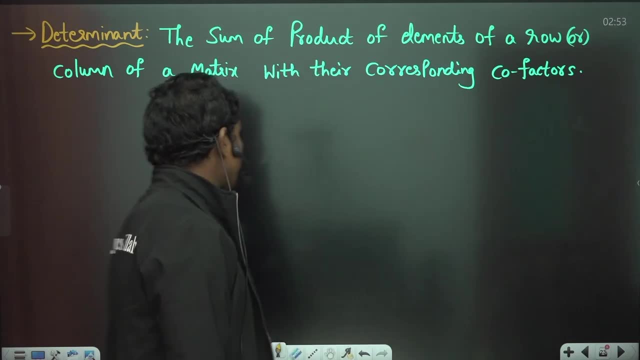 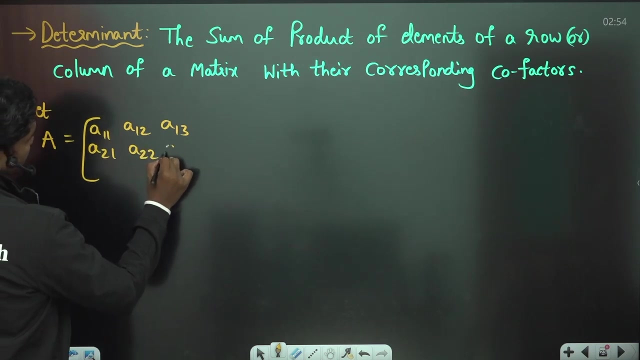 So let us see what we are actually talking about. Okay, but to make you understand this, I'll go with the help of a three by three matrix so that you'll understand. Okay, so look here, Let us suppose I have taken this matrix. let a is equal to A one. one A one. two. A one, three A two. one A two. two A two, three. 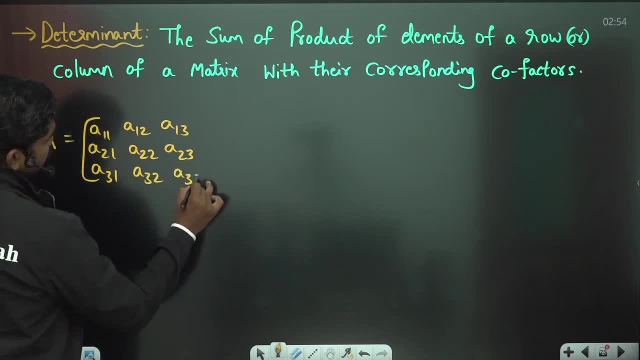 A three one, A three two and A three three. actually, if I have explained it with the help of two by two, you'll actually got what is the definition of a minor or something. but anyhow, let me show you with this. 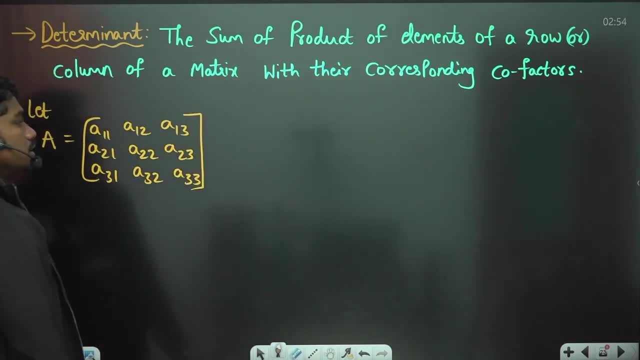 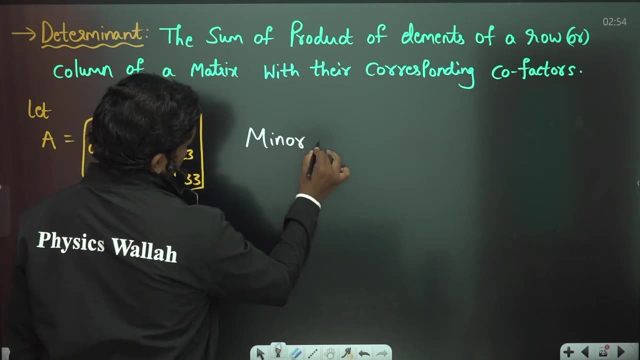 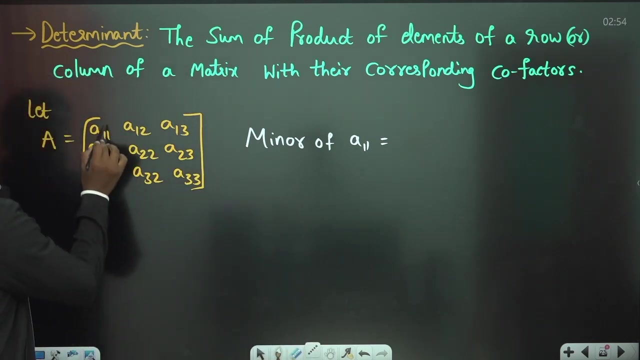 Now here's one. Let me show you how. Let me show you how. Now, if I see this matrix, then there are total 9 elements. so now we write something called minor of a11, for example. okay, So if I ask you about this minor of a11, then see, this is the element containing a11. so 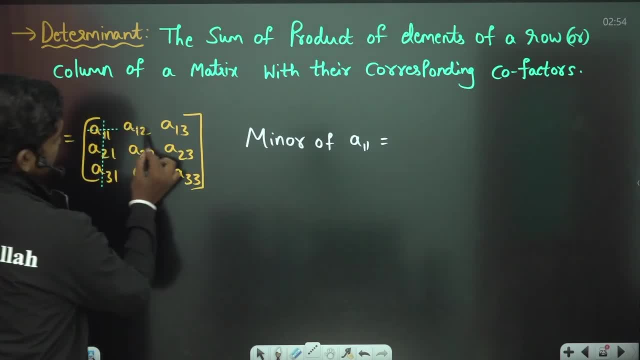 this is the column which is containing a11 and this is the row which is containing a11.. So if you delete this row and column from this matrix, you will get some sub matrix. sub matrix is basically some small part of the matrix. okay, So from this matrix, if you delete this column and this row, then what happens here? you will. 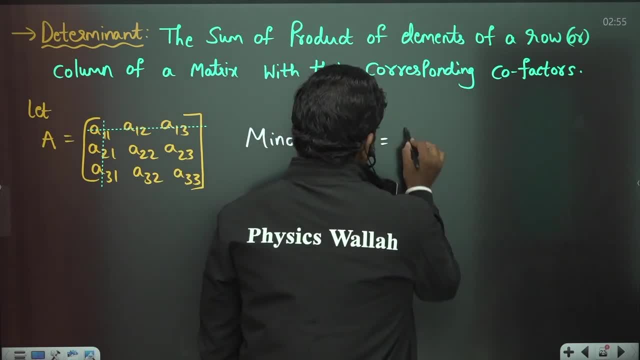 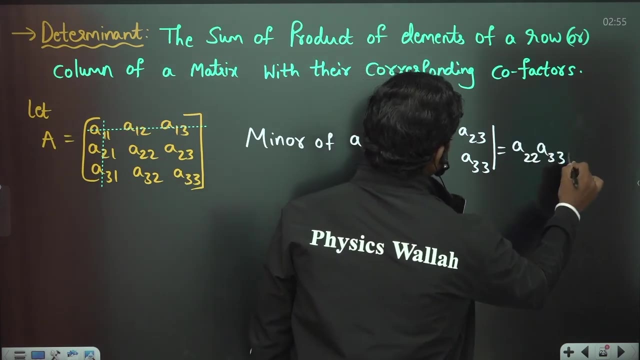 end up with this. you know value that a22, a23, a32 and a33.. So if you see, this value is nothing But a22, a33 minus a23, a32. you need to, you know, understand one thing here. I am directly. 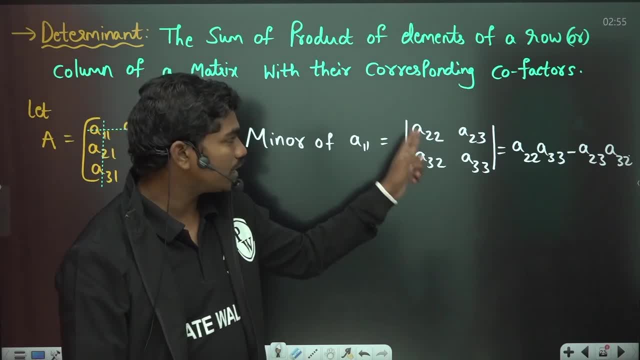 going with the guess of 3 by 3. that's why I am not explaining you, why you need to multiply these two and then, with a minus sign, these two. okay, If I have started with the example of 2 by 2, you might have easily understood. but again, 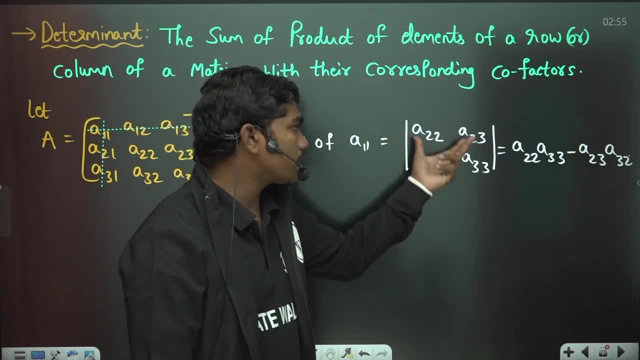 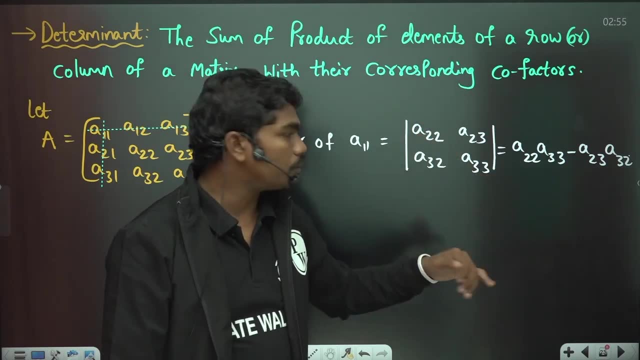 I know that at this level you will be knowing how to calculate the determinant of this. I am just writing directly, okay, But actually I should start the discussion with the 2 by 2 matrices. then you will come to know why I am multiplying this. 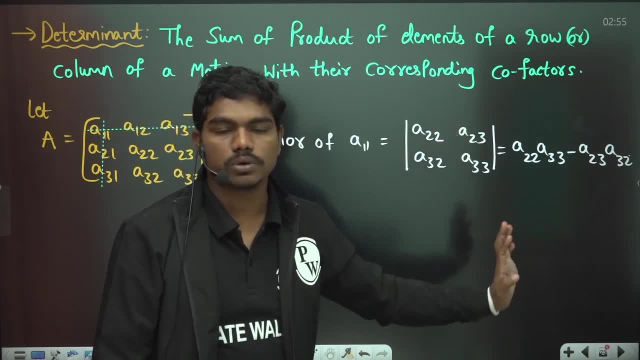 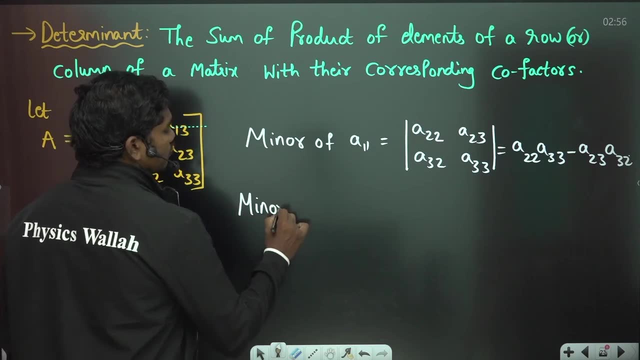 Cross minus this. okay, but right now I am assuming you know how to do this, So I am doing it evidently Now. similarly, if I want to write minor of some other element, for example minor of, you know, a12, let us suppose I am writing minor of a12. 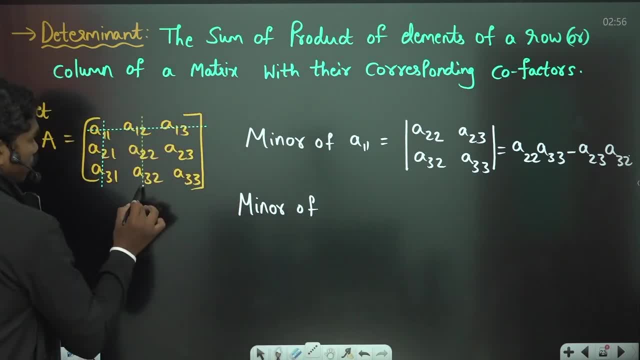 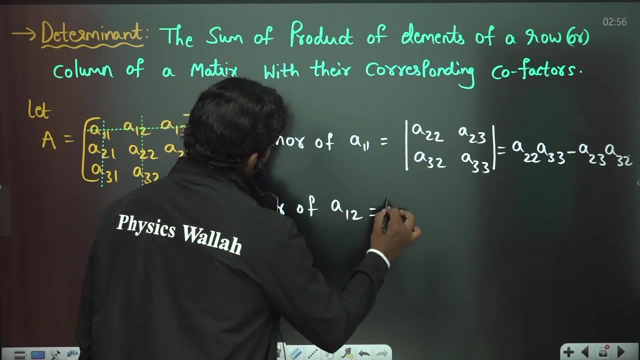 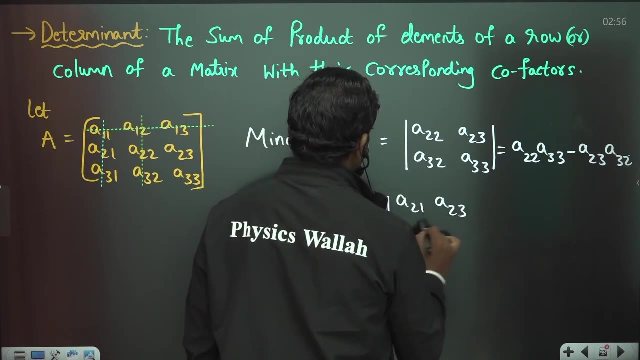 So if I want to write minor of a12, then this is the column and again, this is the row that is containing a12.. So this is left with. If I delete this column and this row, I have a21, a23, a31 and a33.. 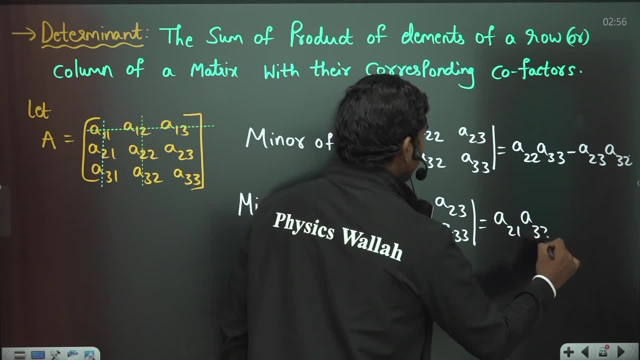 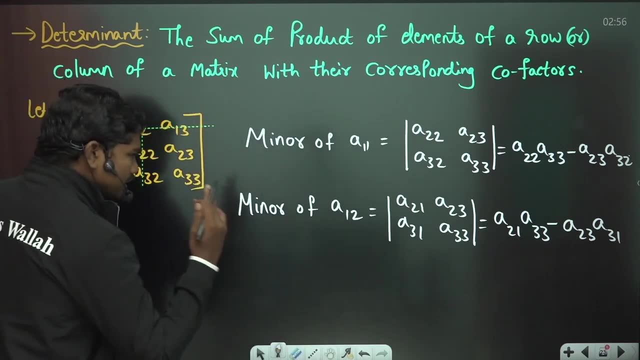 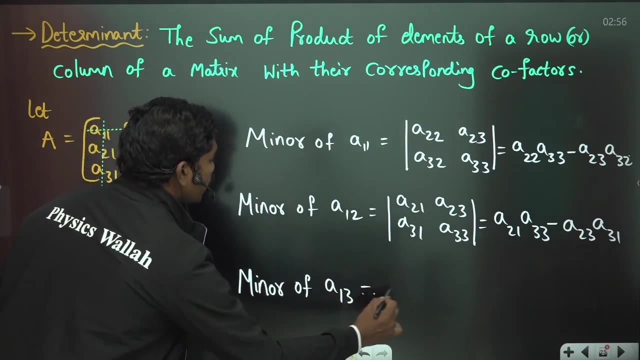 So, if you simplify this, a21, a33 minus a23, a31, okay. Next, why I am doing: I want to write for three elements: minor of a13 also I will write, okay. So minor of a13 also I will write. So now you see here: minor of a13. 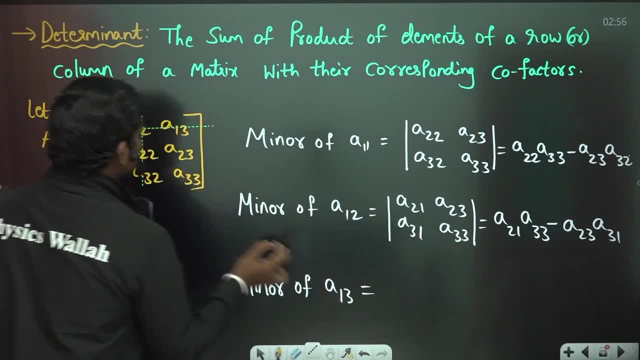 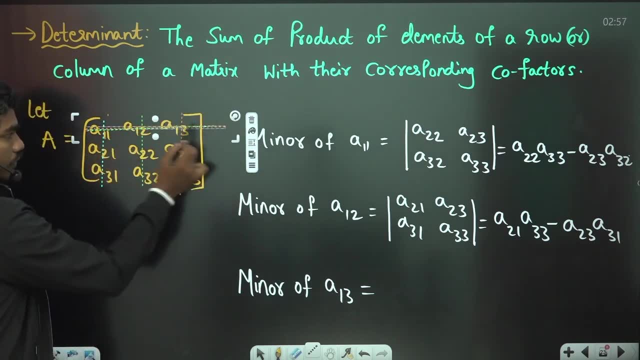 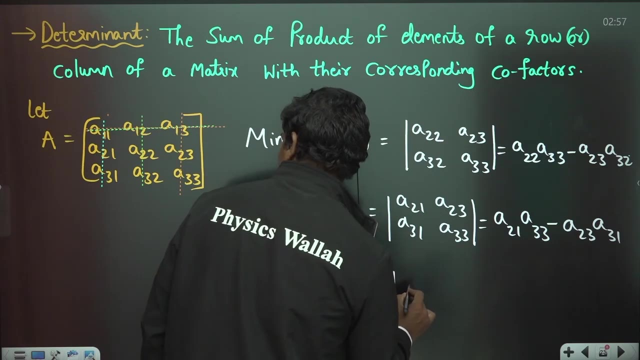 If I Take this, you know elements, This is the column containing a13 and this is the row containing a13.. So if you delete this column and the first row, you will end up with thing like this: So determinant of a21, a22, a31, a32.. 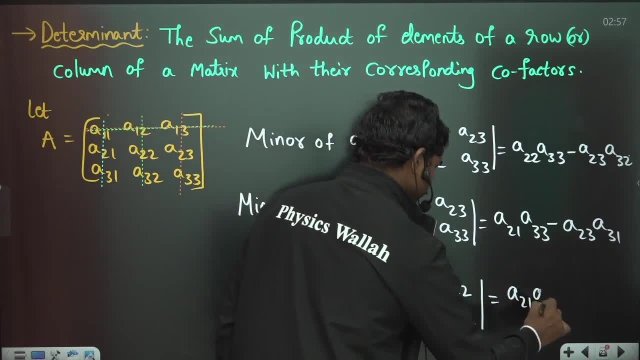 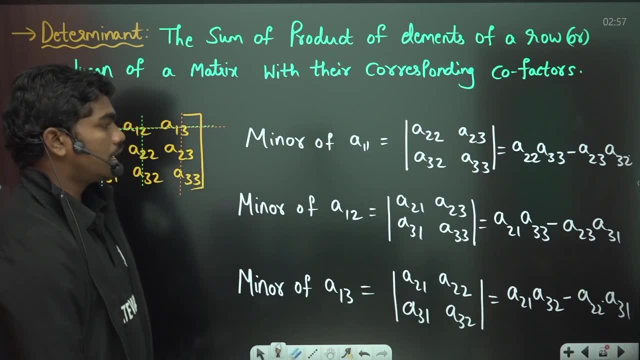 So this is equal to, If you do this again, a21, a32, a33.. So this is equal to, If you do this again, A32 minus a22 times a31. okay, So this is how you have this. Now, these are the three elements which I have written intentionally. 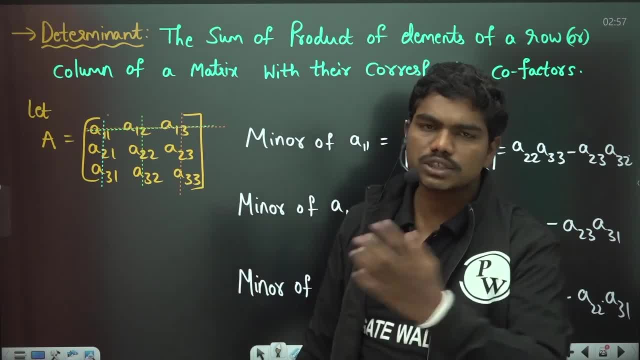 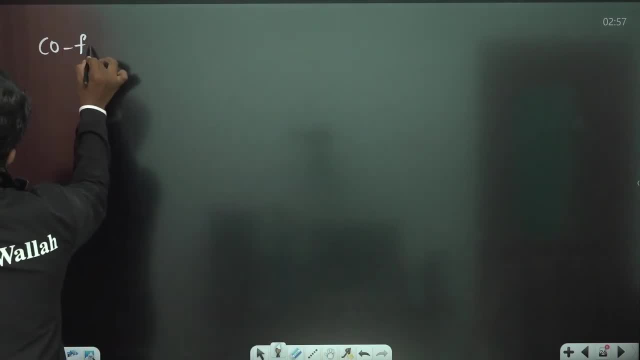 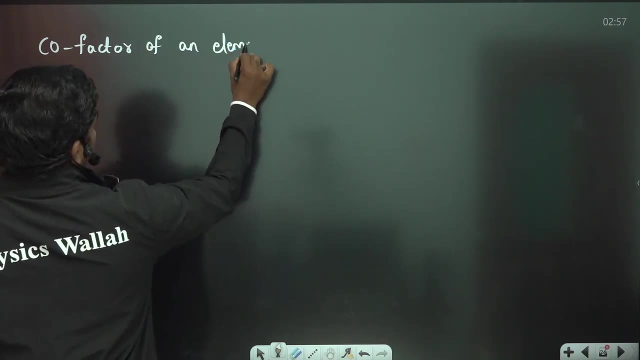 But if you want, you can write for all the nine elements. So if you write for all the nine elements, you will get nine different minors. okay, So now let us see what I define by a cofactor. So cofactor of cofactor of an element, an element aij. 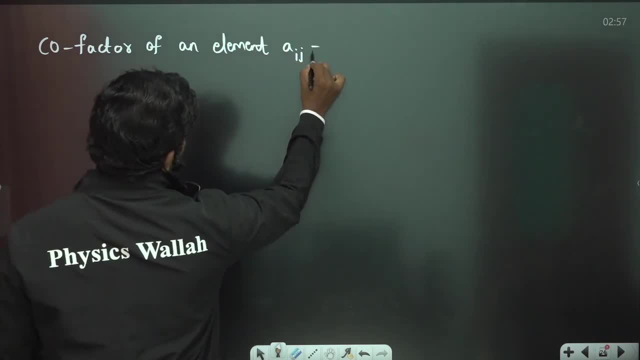 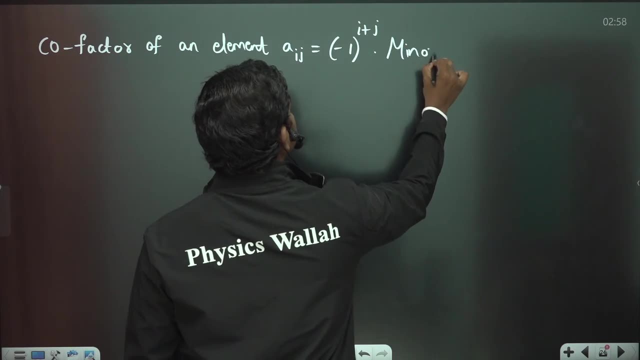 This Is Equal to Minus one whole power, i plus j Times, Minor of Aij, Minor of Aij. Now, If you See the cofactor of a11, a12, all these things You will get. 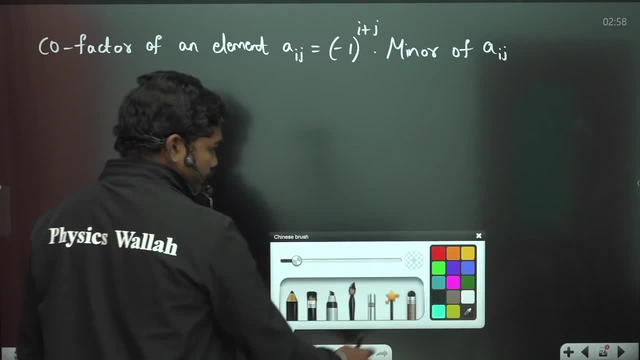 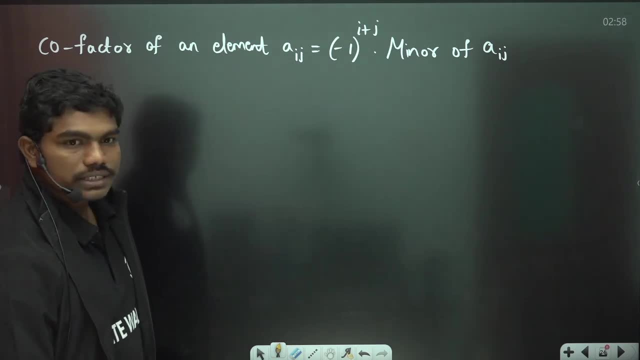 A different Elements with a plus sign, minus sign, change. Now Try to understand the definition now, If you see I can get. Look, This is the first row. For example, I have calculated the minus of the first row, a11, a12, a33.. 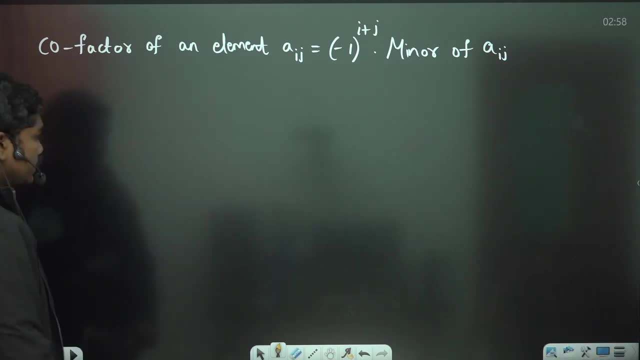 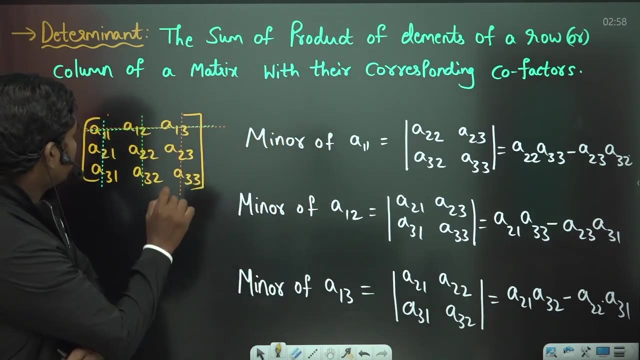 Now Try to understand the definition. now, If you see I can get. look, This is the first row. For example, I have calculated the minus of the first row, A11.. A13. So Now Try to understand one thing. 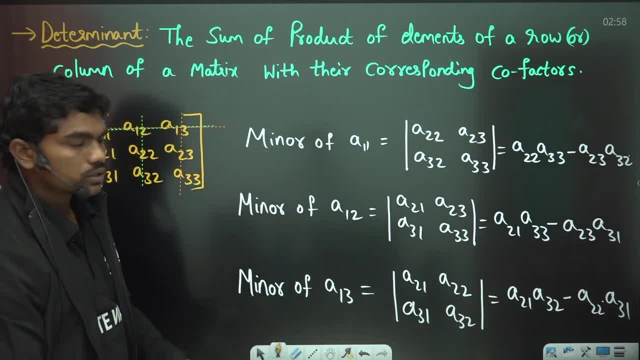 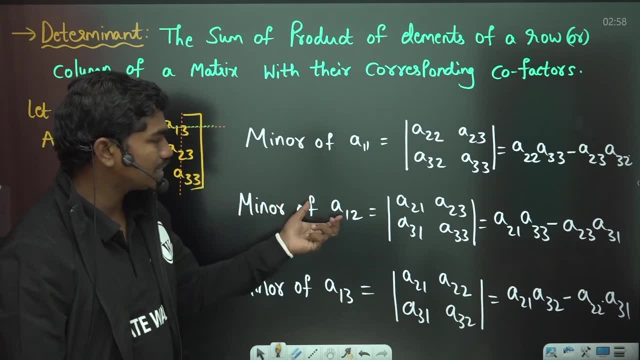 If I calculate the minus, Then Definitely I can calculate the cofactors of these elements also Correct. So What will be the cofactor of this, This Minor of a11.. Into Minus one whole power, one plus one. 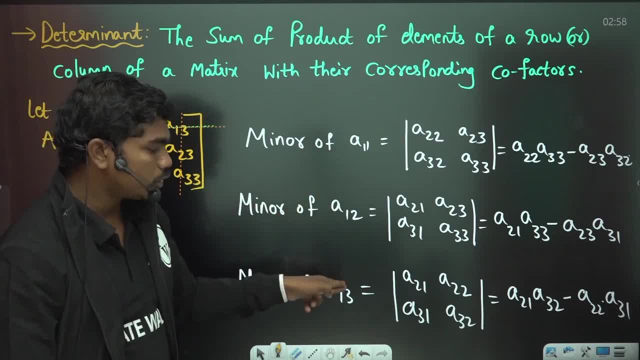 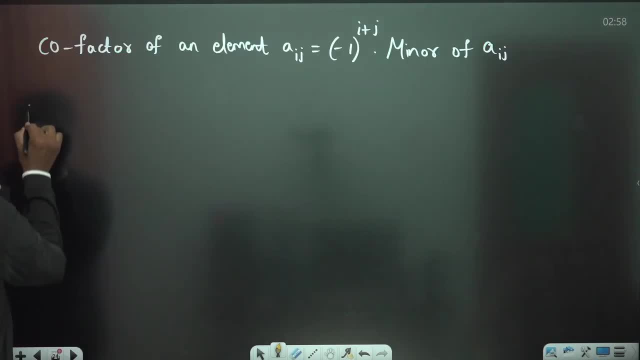 Similarly, Cofactor of a12. Is equal to A12. I mean This Minor of a12.. Into Minus one whole power: one plus two. Into Minus one whole power, one plus three. Similarly Here: 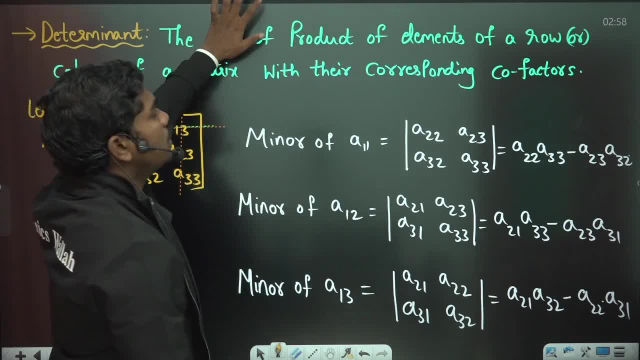 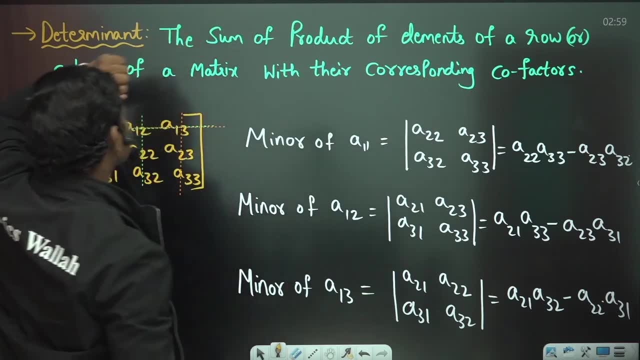 Now Look at this definition: The sum of, Forget this sum of, First of all, Product of Elements of a row Or column With their corresponding cofactors. Look, Let us suppose, If I take the first row, Then 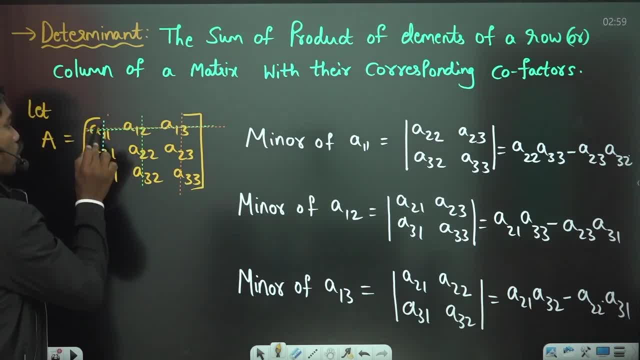 What I should do is I should multiply this A11. With the cofactor Of this a11. Then I need to sum this To The product of This a12. With The cofactor of a12.. 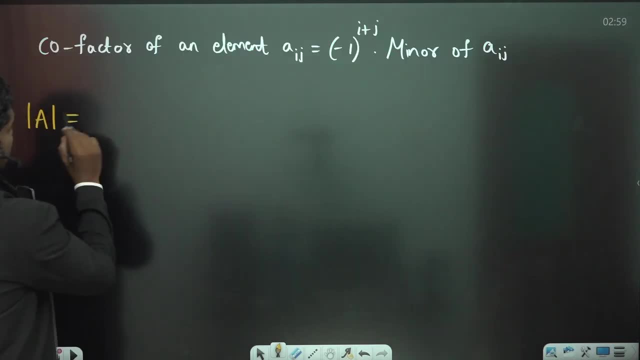 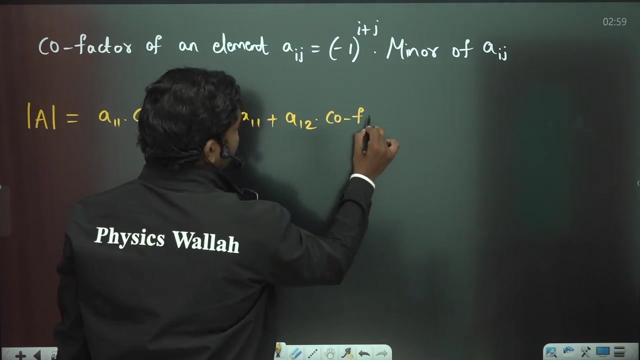 Plus A13.. Into Cofactor of a13. Means, Basically, I have A12.. Into Cofactor Of A11. Plus A12.. Into Cofactor Of A12.. 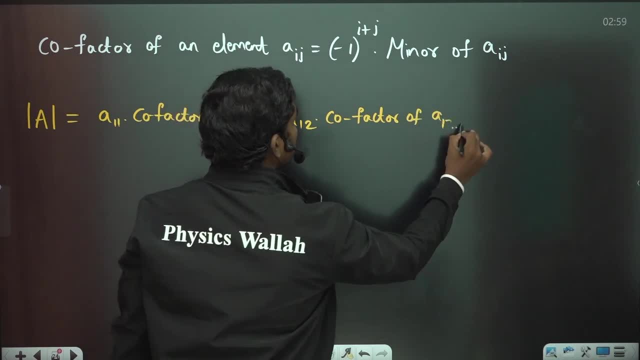 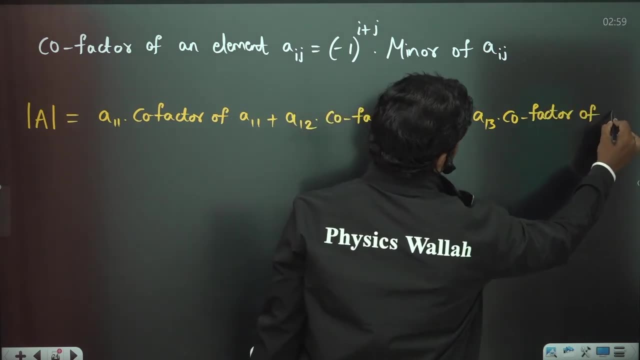 Plus A13.. Into Cofactor Of A13.. Look Here I have taken the first row, But It is not mandatory That you need to take Always the first row. You can take second row. 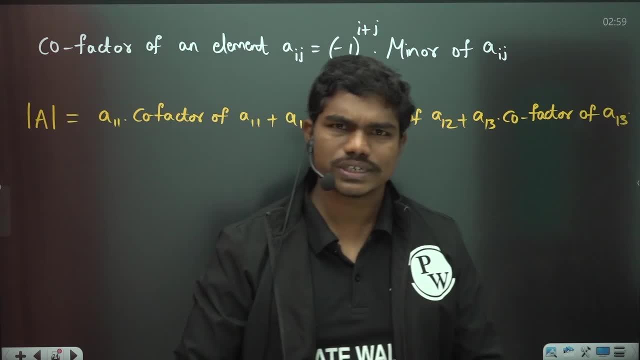 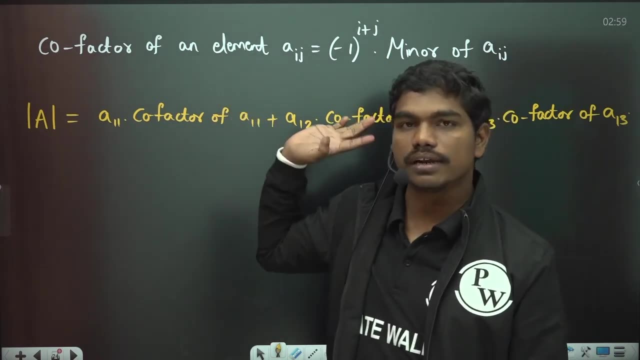 Third row, Anything. But You can also take First column, Second column, Third column, Anything, But You need to Multiply The same cofactor Corresponding to that element. This must be done Carefully, Okay. 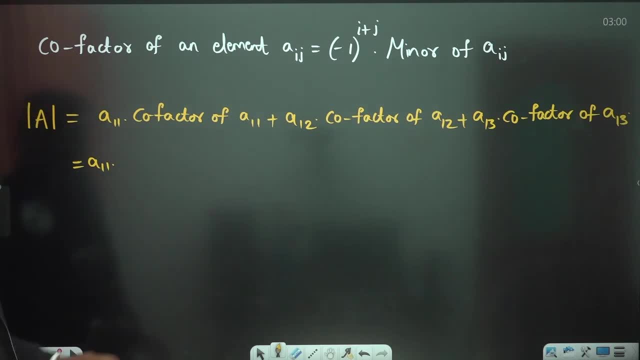 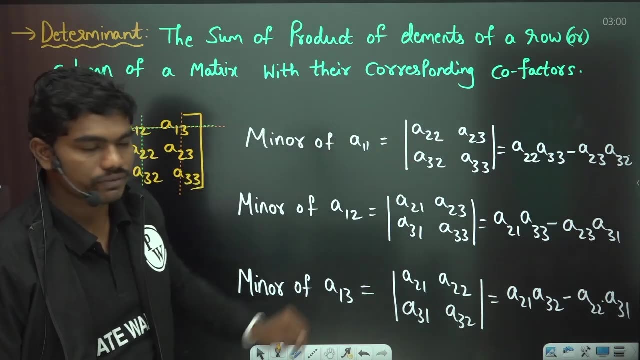 So Now Let us check here. This is equal to A11.. Into Now, Cofactor Of this A11. Will be nothing but Minus 1.. Whole power: 1. Plus 1.. 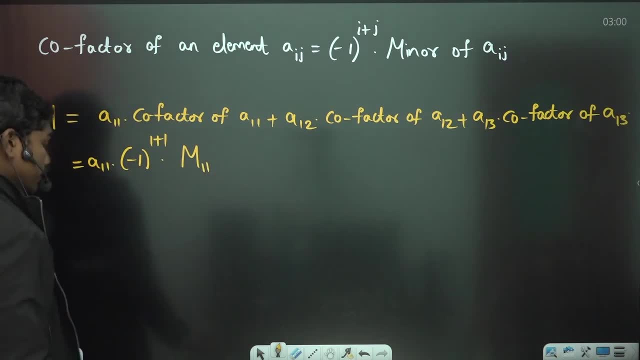 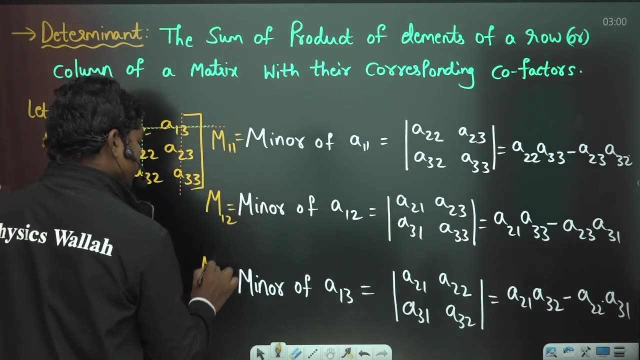 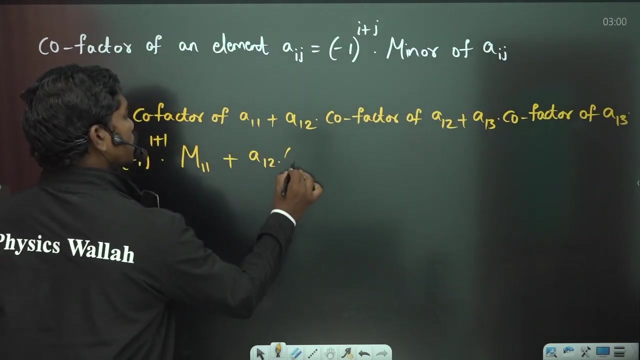 Into Minor Of A11.. Let us suppose If I write this as M11.. This is M12.. This is M13. Minus, Basically Okay. So Now You try to understand One thing. 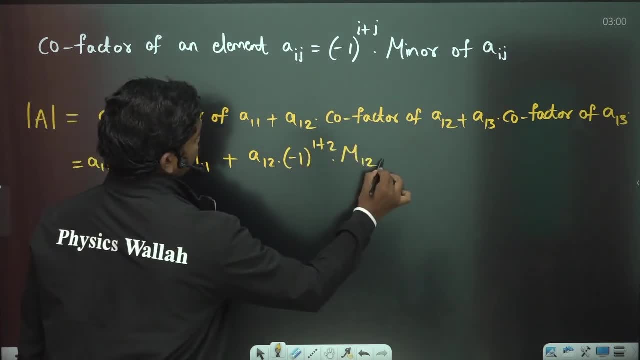 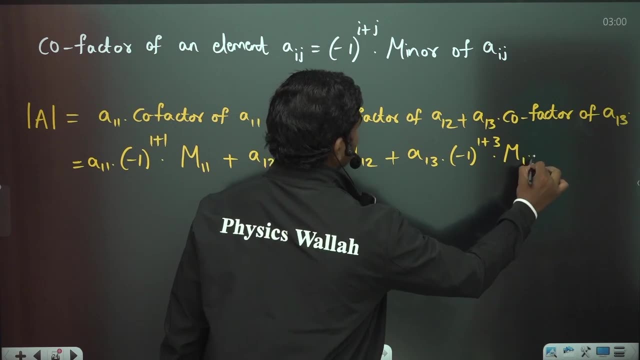 Plus A12.. Into Minus 1. Whole power: 1. Plus 2. Into M12.. Plus A13.. Into M12.. If you substitute the values, What you will get A11 times of. 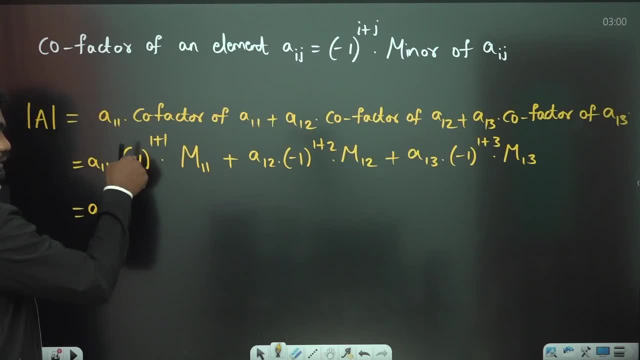 This: Minus 1. Whole power 1.. Plus 1. Is nothing but Plus 1.. So First of all, I want you Make you understand that, Why you are Putting a plus- minus sign. Alternatively, 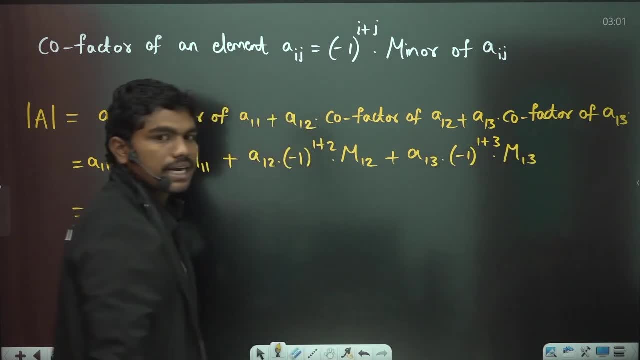 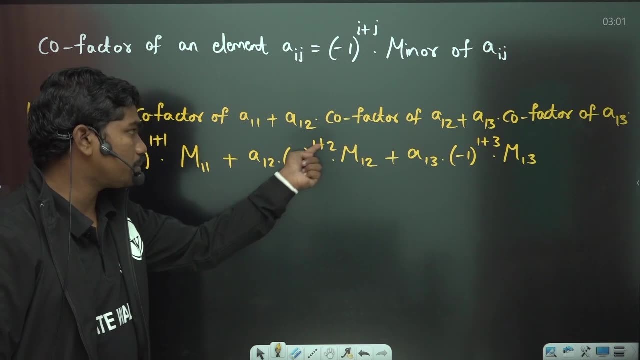 Because This gives you plus sign. This gives you Minus sign. Again, This gives you Plus sign If you have 4. By 4. sum basically here: okay, so if you see, depending on this summation, here you have a plus sign. 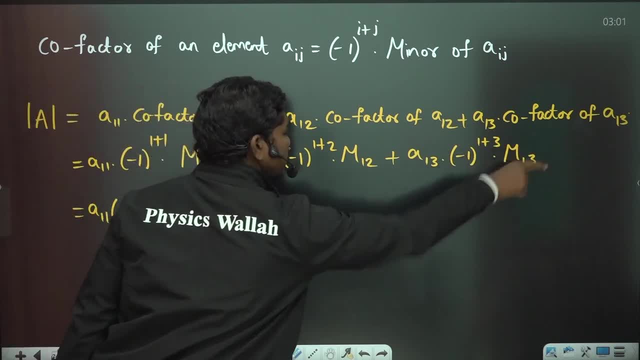 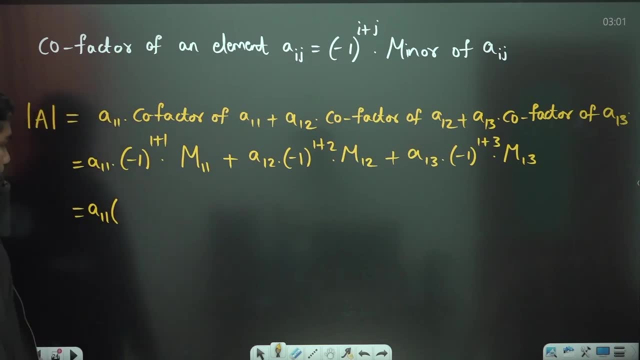 and here you will get a minus sign. again, here you will get a plus sign, here you will get some minus sign. that is the reason of writing alternative plus and minus in case of determinants. okay, so this: if you write this, that term, a22, a33, a22, a33 minus a23, a32, then there is a. 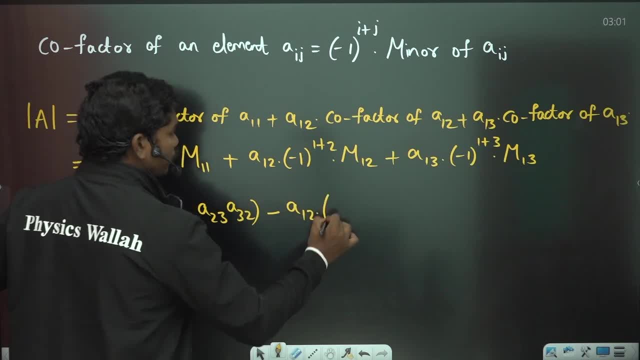 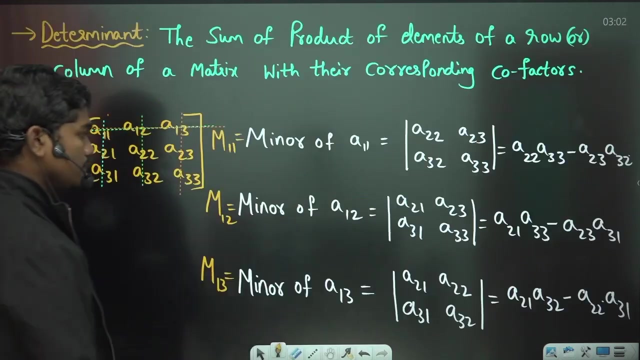 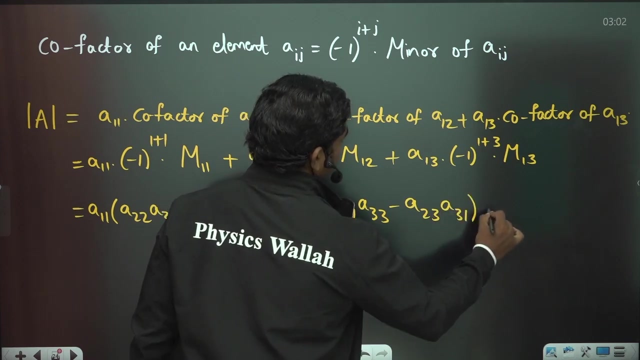 minus sign here, so minus a12 times of this m12 which is, you know, which is basically a21, a31, a33, a21, a33, minus minus a2, a31. then again here you have a plus, so plus a13 times of there you can write a21a33. so it get some numbers for the product regulations, your 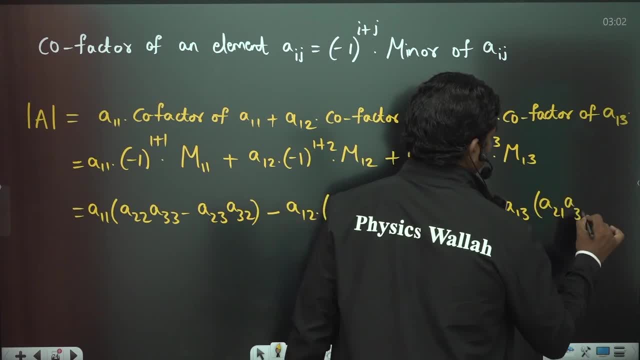 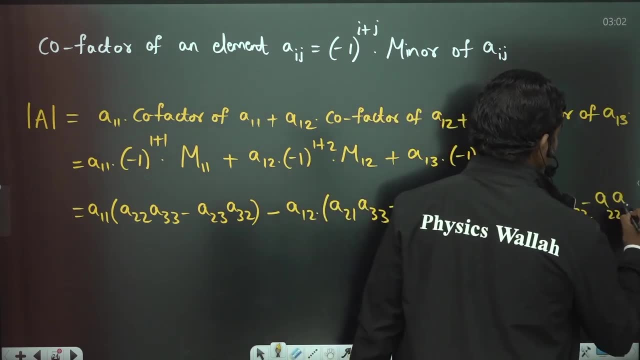 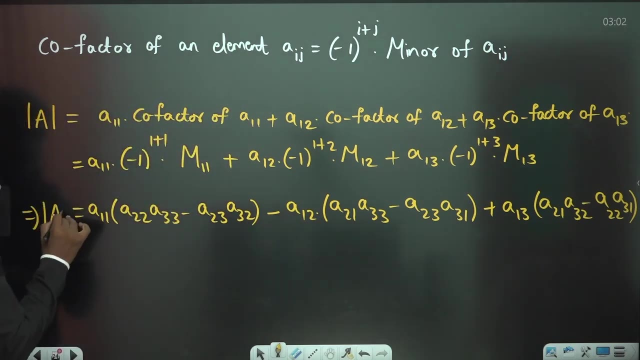 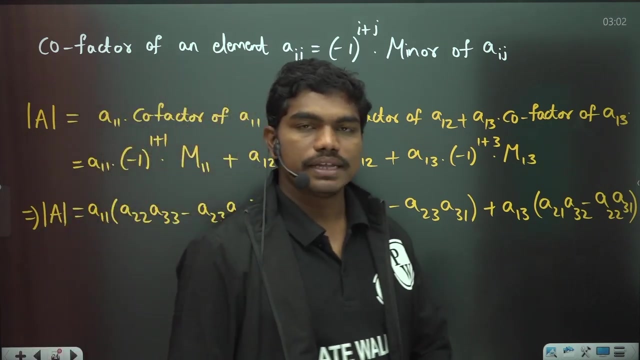 A32 minus A2 to A31.. So, basically, this is how you actually write the determinant value when they ask you for the determinant of the given matrix. So, anyhow, this is the determinant value. Now I would like to tell you one thing: If you multiply the cofactors of the same elements with the corresponding cofactors, 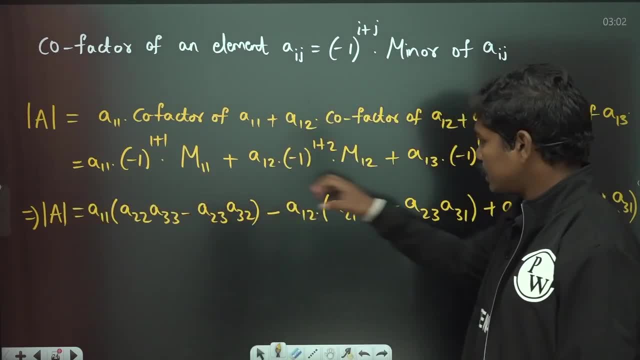 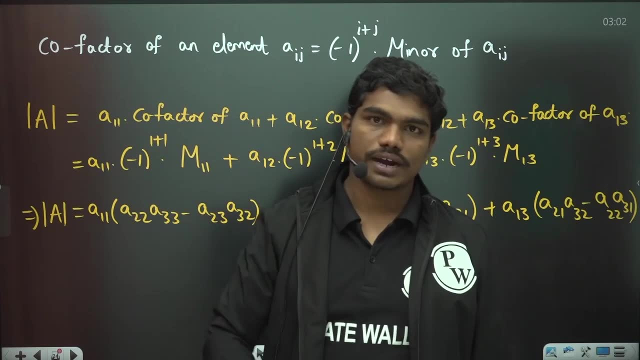 you will get the determinant value. Means, if you multiply this row elements with the corresponding cofactors, you will get determinant. Now let us suppose if you multiply the elements of a row with other row cofactors- Means, basically, you are taking elements of one row and you are multiplying this row elements. 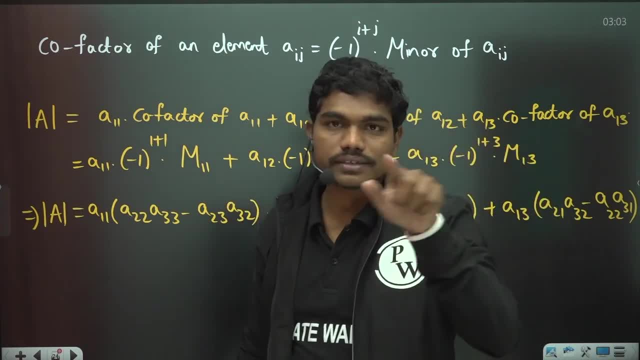 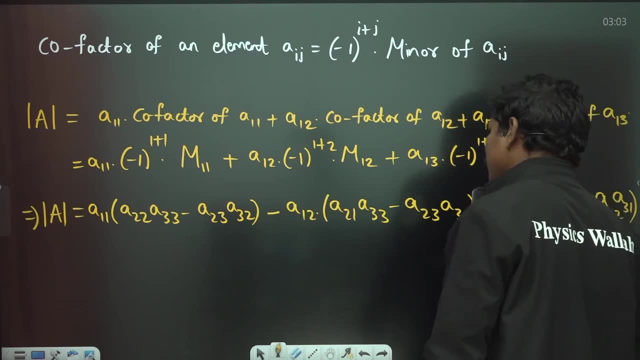 with cofactors of some other row, Then what you will get the result? The answer is going to be 0.. Look, I will show you how it is coming, Basically how it is coming. I will show you with the help of a 2x2.. 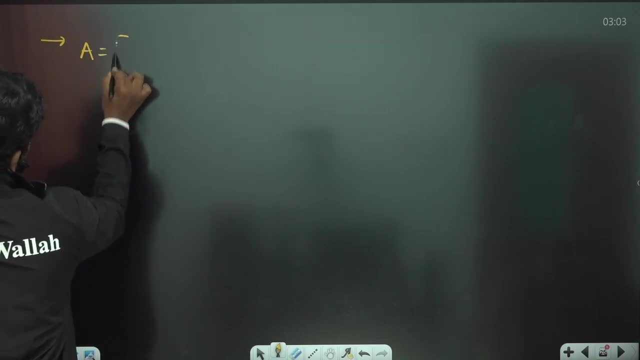 Look, Let us suppose you have taken some 2x2 matrix, which is ABCD. Now, if you write the minus in how? I would like to directly write the inverse of this. If you want to write the inverse, you should always write this: 1 by determinant AD, minus. 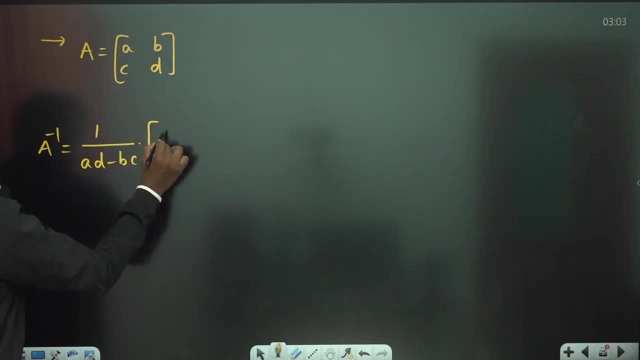 BC and now interchange these two terms. So D and A comes here, and of course these two has to be replaced with a minus sign: Minus B, minus C. You will see shortly how this is coming. and all So A inverse. the simplest form to write A inverse is this: 1 by AD minus BC. you write directly. 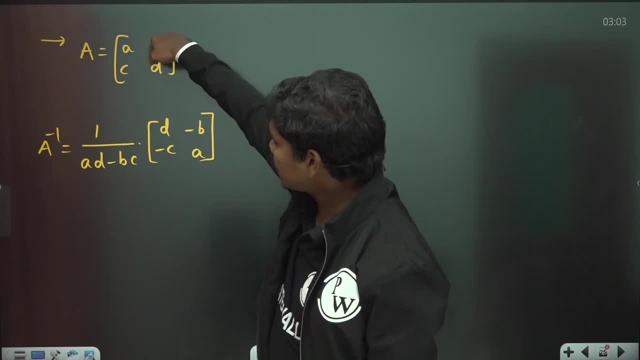 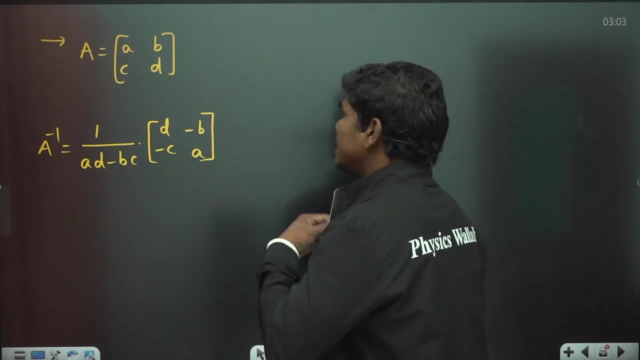 then you swap these two means basically you interchange these two diagonal terms. So D and A comes here, then you replace these two with a minus sign. Okay, So anyhow, if you see, look I will show you- If you take the first row means M11. minor of first row, first column element. 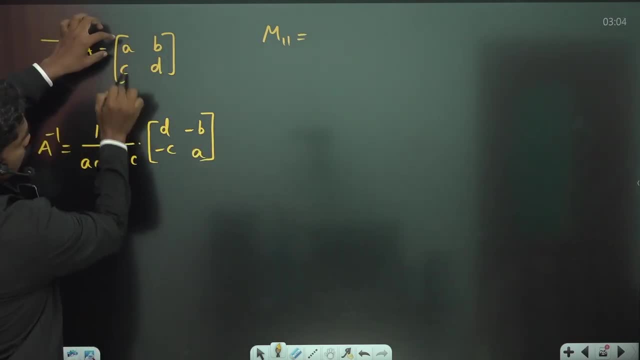 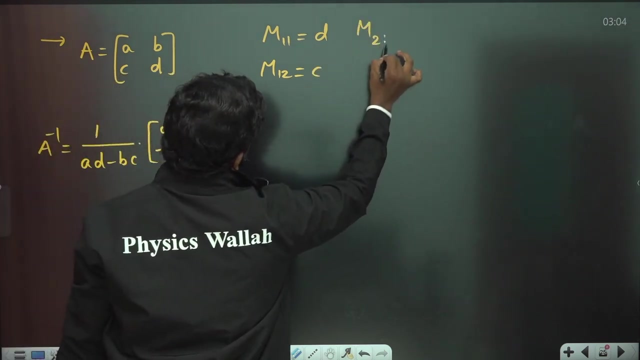 If you take this element, then if you delete this row and this column, then D is the thing which is left over. So D- M12.. So if you take this element B, Now This row and this column, you are left with this C. So this is C. Next M21.. 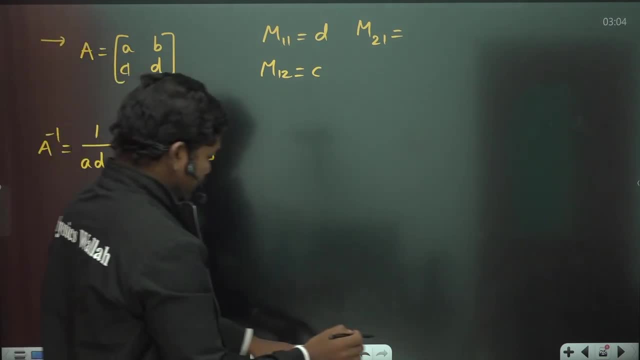 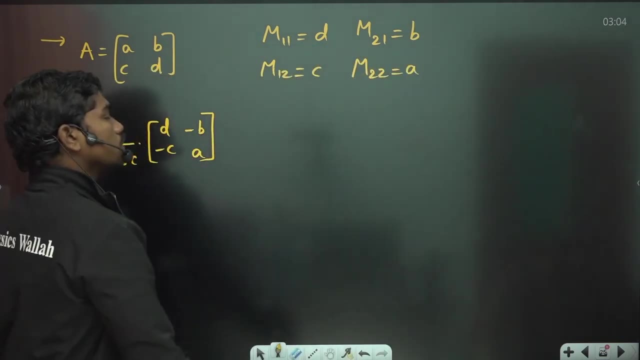 So if you take this C, for example, if you delete these two, you have a B and M22 will be A, Correct. So what are the cofactors? So if you want to talk about cofactors, then cofactor of 11. you can write capital A11, cofactor. 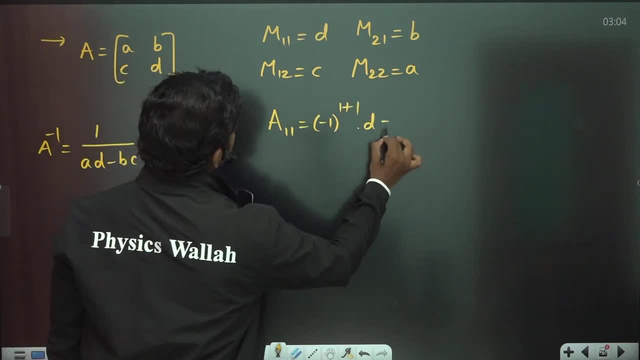 of 11 is equal to 1 plus 1. into D, which is equal to D, Cofactor of 11.. Cofactor of 12.. Into this C, which is minus C, Cofactor of 13, or okay, this is a 2 by 2.. 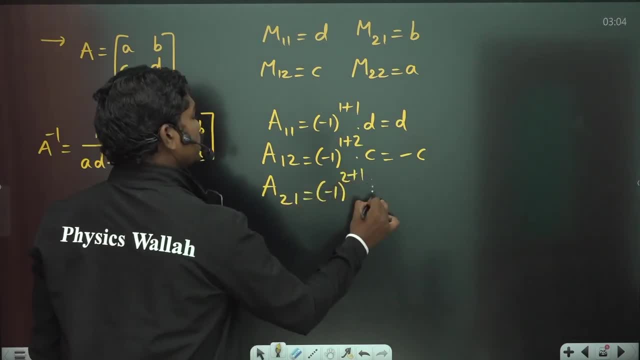 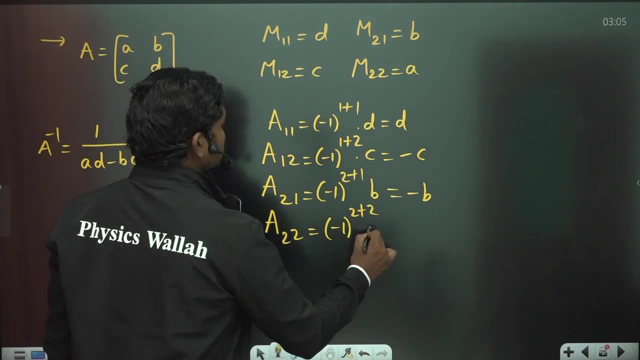 So 21 is equal to minus 1 whole power, 2 plus 1 into B, which is minus B. A22 is equal to minus 1 whole power, 2 plus 2 into A, which is equal to A. Okay, So these are the cofactors. 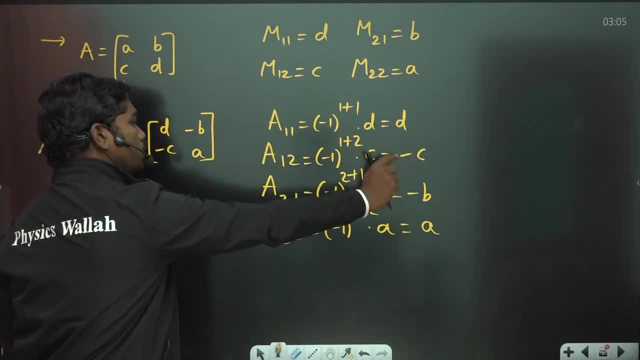 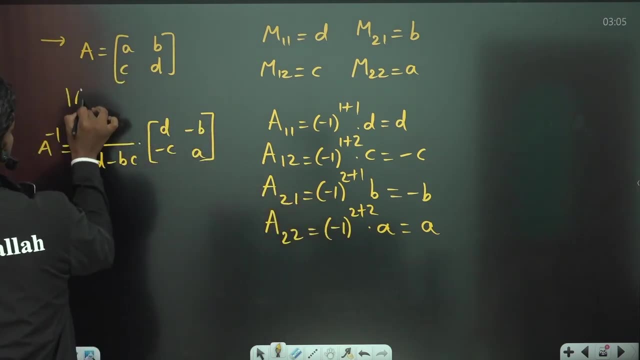 Now, this is the cofactor of 111.. This is the cofactor of 12.. This is cofactor of second or first column. This is cofactor of second or second column. Now, as I told you, you all know that, that A, if I ask you this, you will directly tell me. 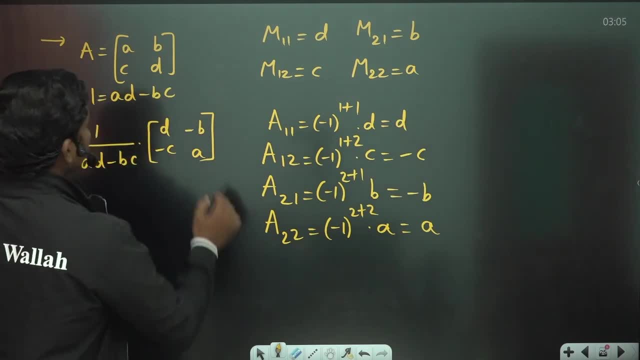 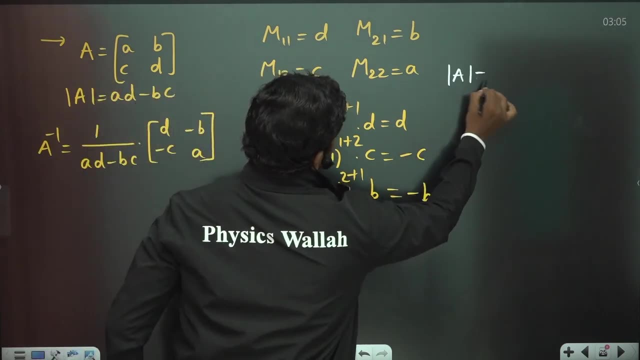 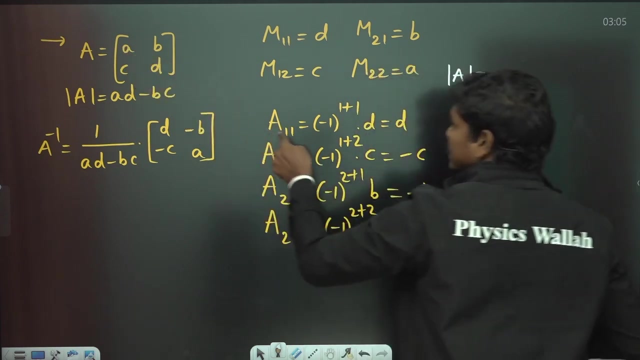 AD minus BC. But how this AD minus BC is coming? If you multiply first row with the corresponding cofactors you will get correct So that A can be written as first row elements multiplied with the first row cofactors. So first row, element A. What is the cofactor of A? You can see cofactor of first row first. 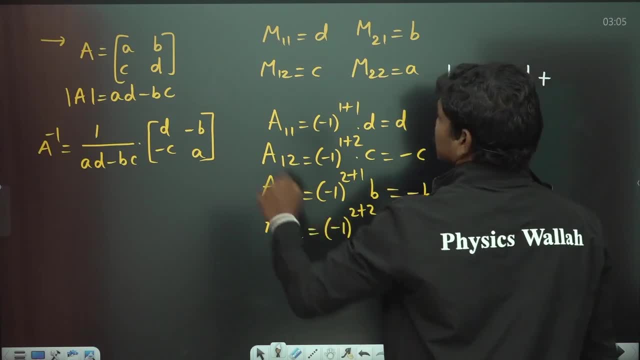 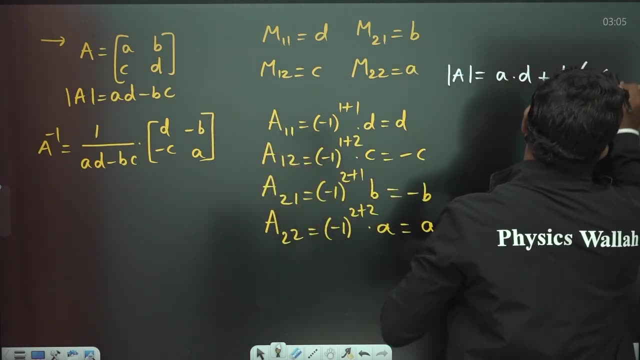 column element is D, Then Okay, Then plus second element B into what is the cofactor of this first or second column element minus C. So you can see this is nothing but AD minus BC, which is the determinant of this matrix. Next, 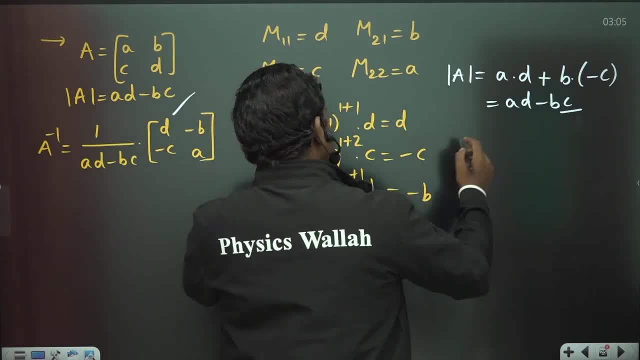 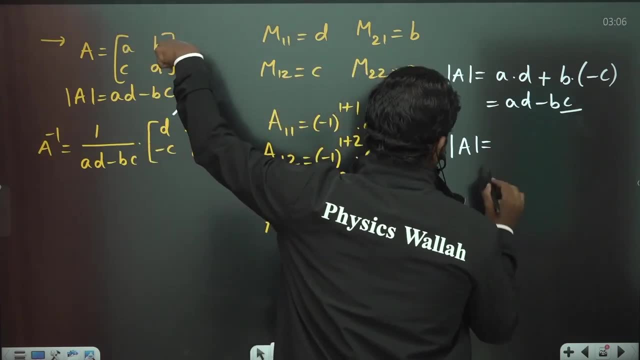 You can calculate that A using another method also, by taking some other also. for example: let us suppose, if I take using this column BD, any column you can take BD, let us take So first B, B into, Then what is the cofactor corresponding to this B? 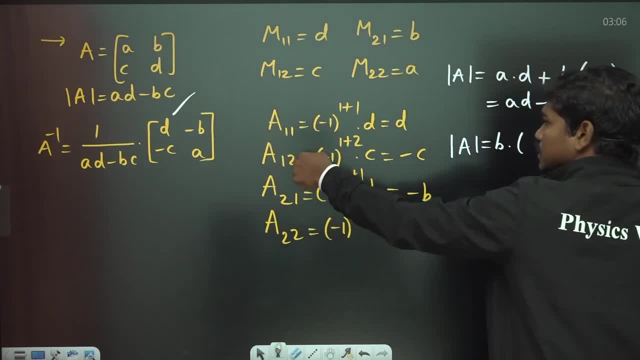 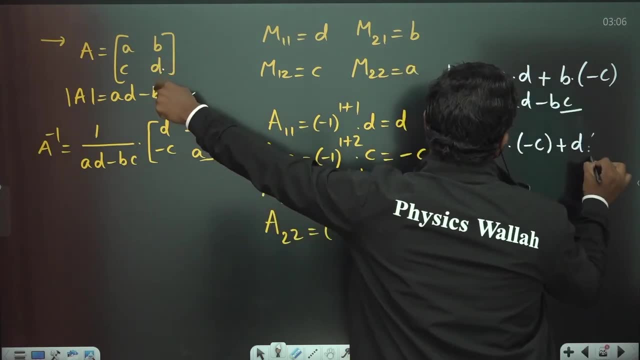 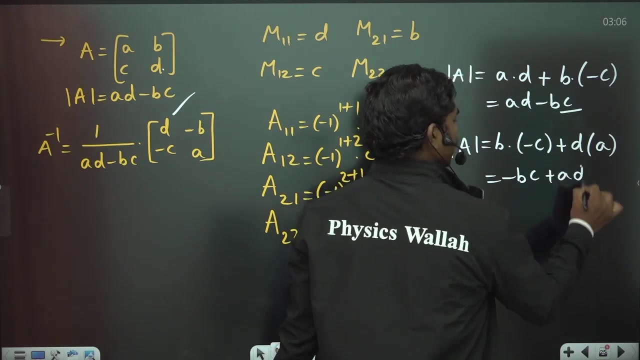 Cofactor corresponding to this B. This is first or second column element. So first or second column is minus C plus this element is D. And what is the cofactor corresponding to D? Last element is A. So you can see, this is nothing, but minus BC plus AD, which is nothing. 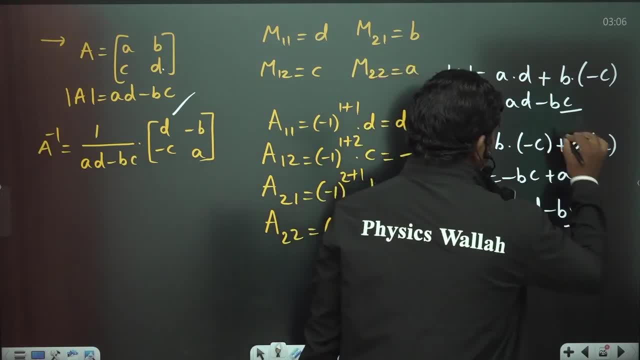 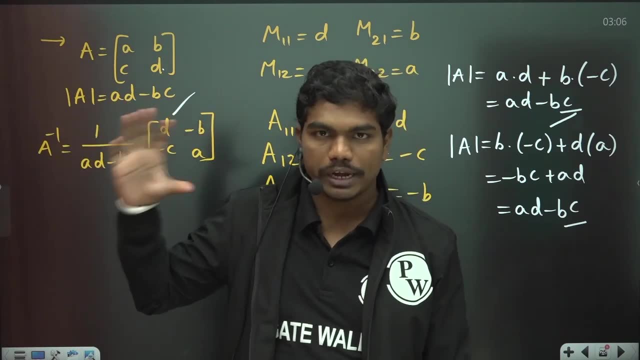 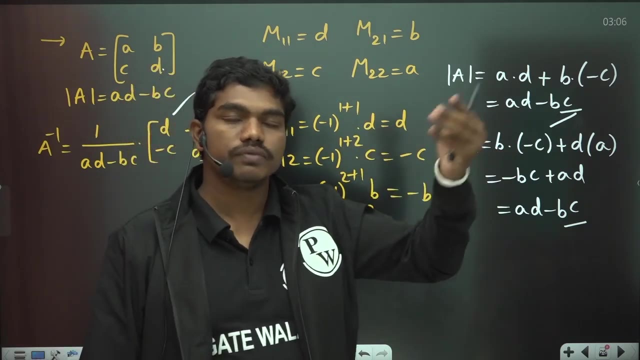 but AD minus BC, Again, you will get the determinant. So my intention is basically to tell you that if you multiply elements of a row with their corresponding cofactors, or maybe column with their corresponding cofactors, you will get determinant value. Okay, Now what happens if you multiply the cofactors of some other row with the actual some other? 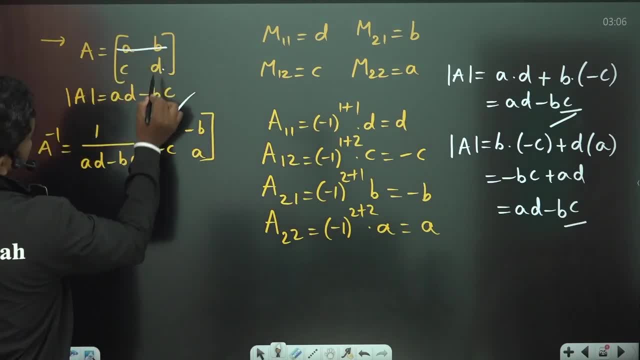 elements. Okay, For example, let us try to multiply this row with these cofactors. If you try to multiply, let us see what happen. A into: So cofactor of C is how much minus B plus B into what is the cofactor of D Cofactor? 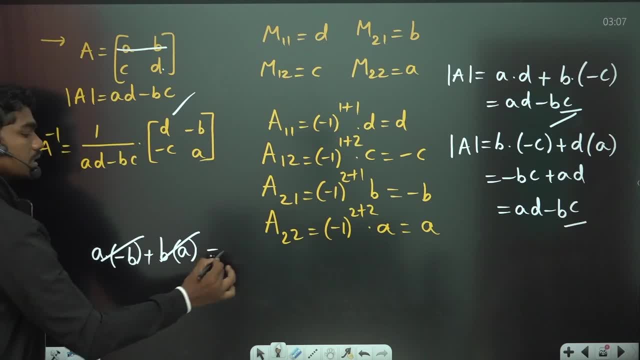 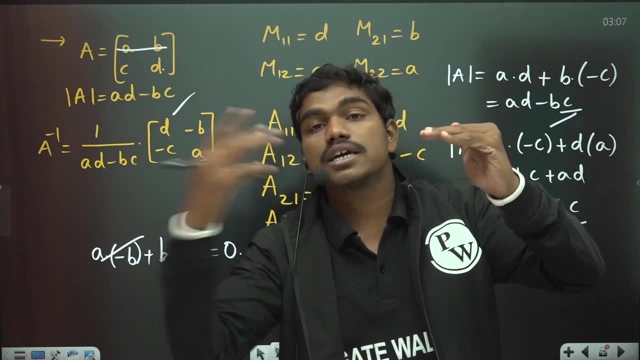 of D is A. So if you see AB and minus AB, the answer is got to be zero. Okay, So if you multiply elements, means if you multiply elements of a row with other row cofactors, you end up with having a zero. This is a two by two case. 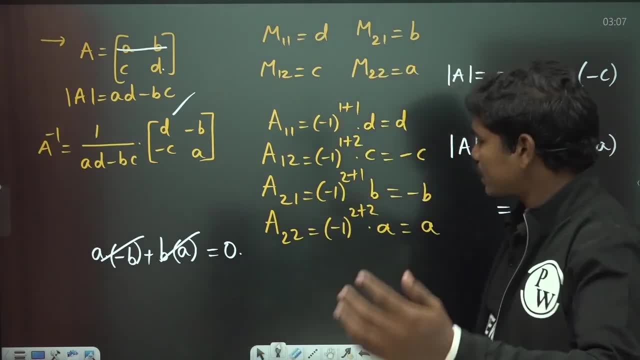 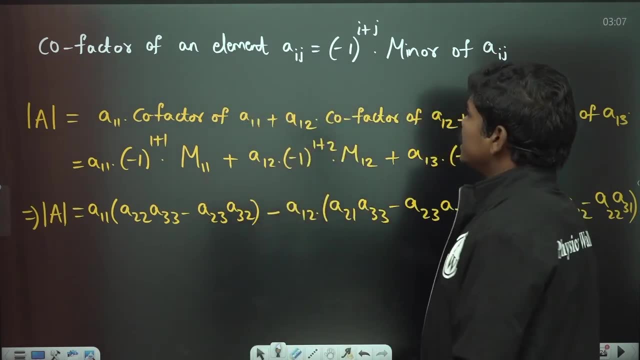 It is very simple. So I have shown you using this two by two case, But actually you can show for three by three also. So basically, my intention is to tell you that if you multiply elements means basically, if you take the sum of product of elements with their corresponding cofactors, you will get 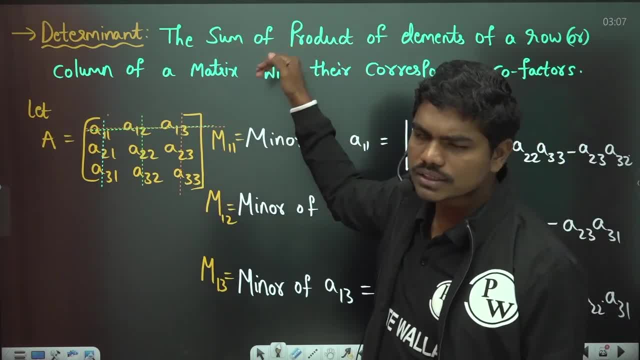 the determinant. And if you multiply some other elements- cofactors- you will get this zero. Now I want to show you that if you multiply elements of a row with other row cofactors, you will get the determinant. And I want to tell you one thing here: 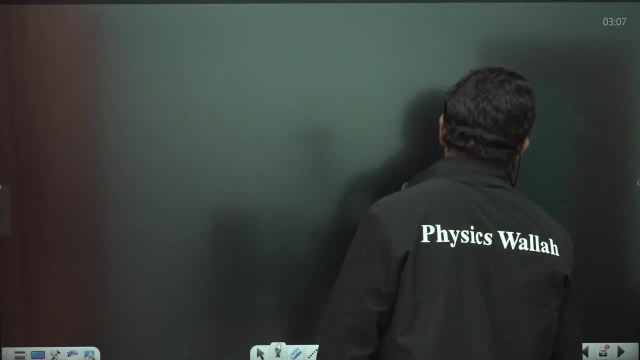 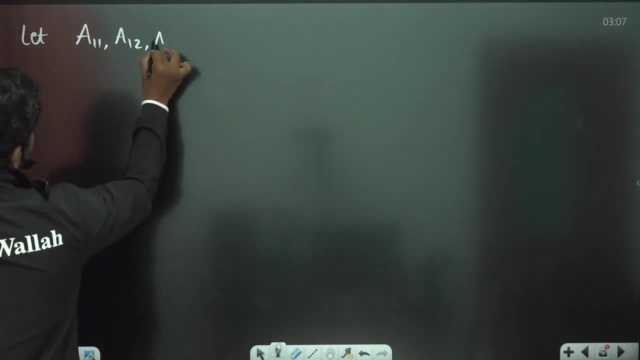 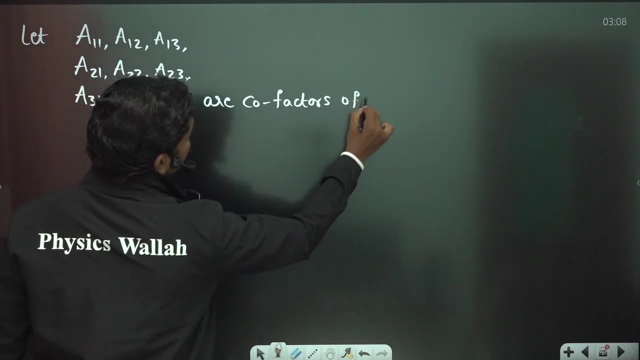 Look, look, let a11, a12, a13, a21, a22, a23, a31, a32, a33 are cofactors of A, Are cofactors, are cofactors of A. then what can I write? I can form some cofactor matrix, correct? so cofactor. 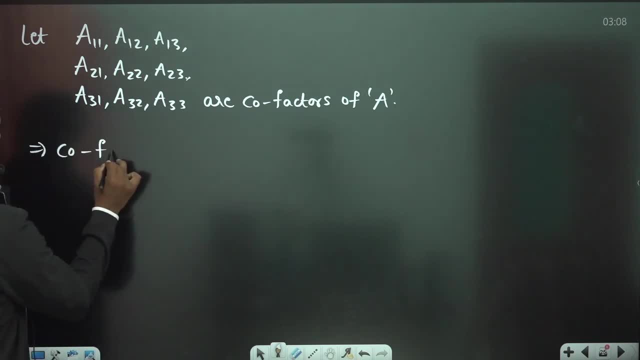 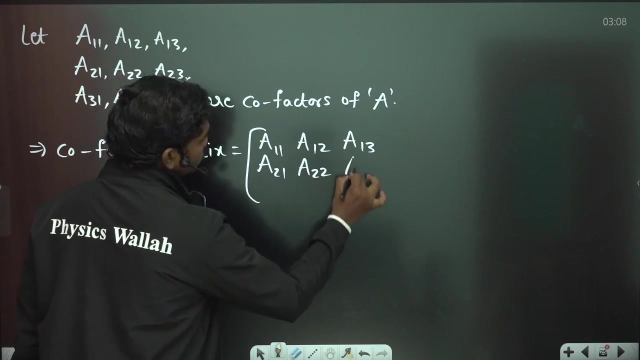 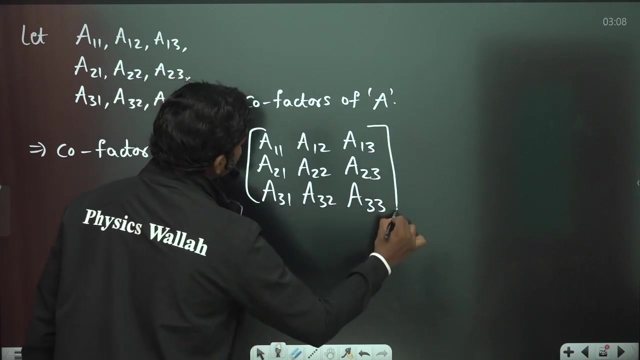 matrix, cofactor matrix. cofactor matrix is going to be something like this: cofactor of the first or first column element. first or second column element, first or third column. we are occupy A21, A22, A23, A31,, A32, A33. ok, so let us suppose this is the cofactor. 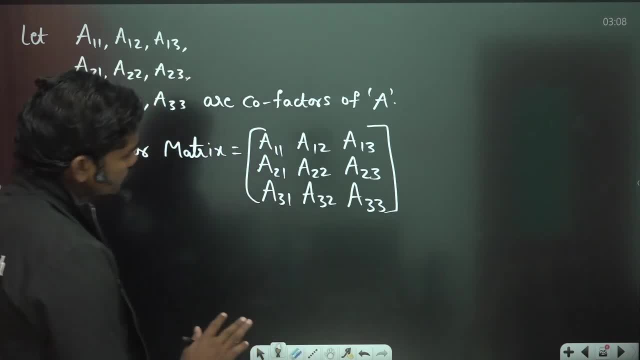 matrix means basically calculated cofactors of all the 9 elements. now let us suppose if we take transpose of this. why I am taking transpose you will come to know when I multiply. ok, so let us suppose I am taking transpose. so, transpose of cofactors, matrix, transpose. 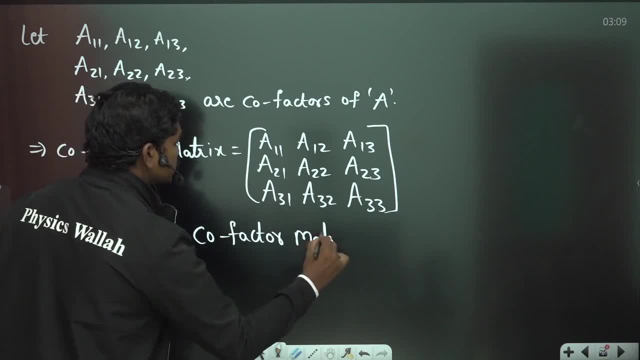 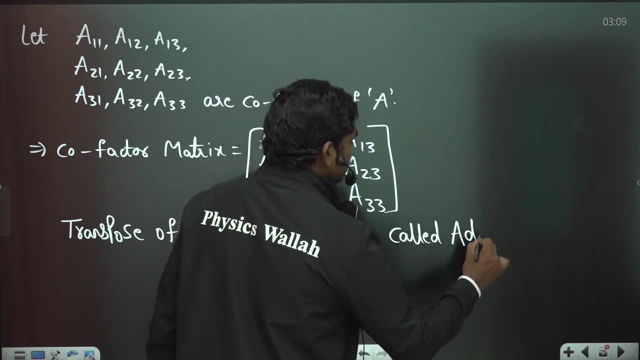 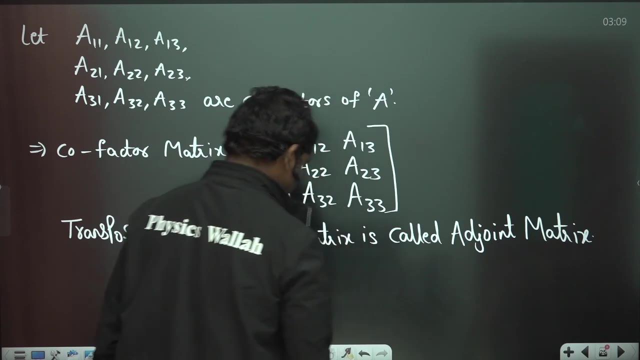 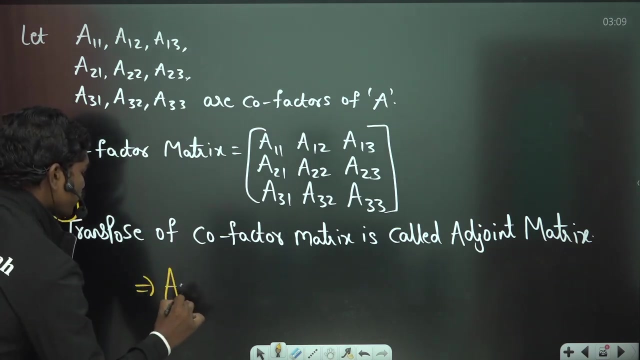 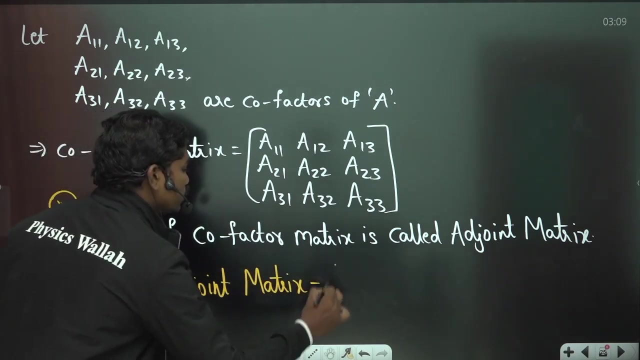 of A и A现 AC. transpose of this cofactor matrix is called is called adjoint matrix. transpose of this cofactor matrix is called adjoint matrix. now let us see means basically: if you want adjoint matrix, adjoint matrix, this is equal to cofactor matrix, cofactor. 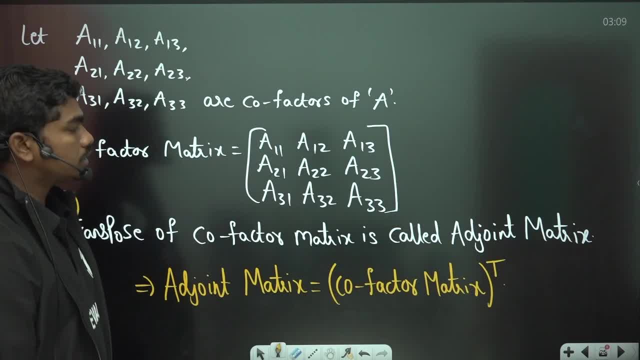 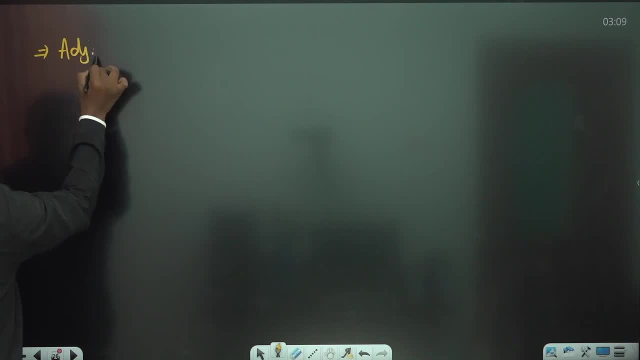 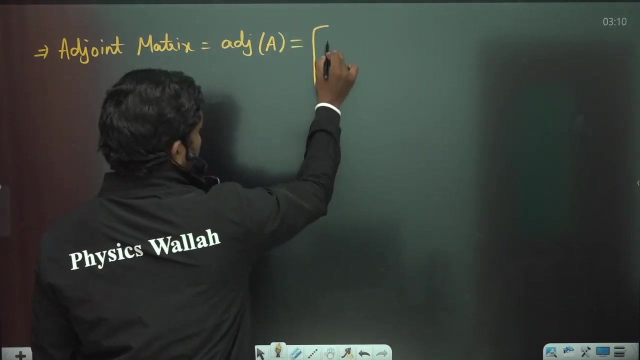 matrix full transpose. Now let us see what is this adjacent adjoint matrix basically? so this implies adjoint matrix, adjoint matrix matrix, or generally write this as adj of a, adjoint of a. so adjoint matrix of a is nothing but this transpose of the cofactor matrix, which means a11, a12, a13, similarly a21, a22. 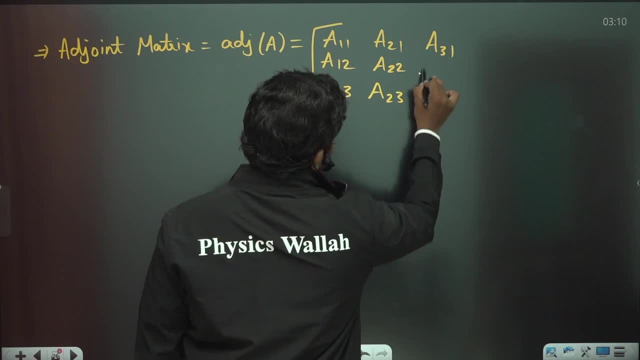 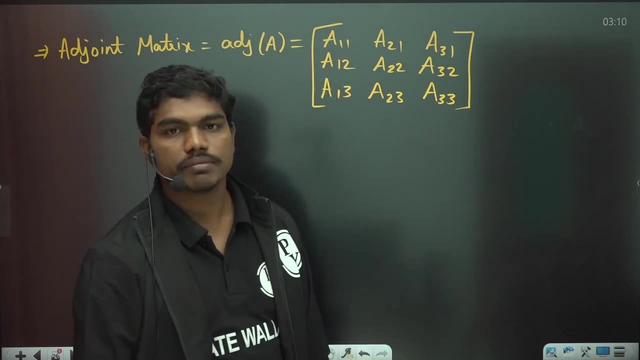 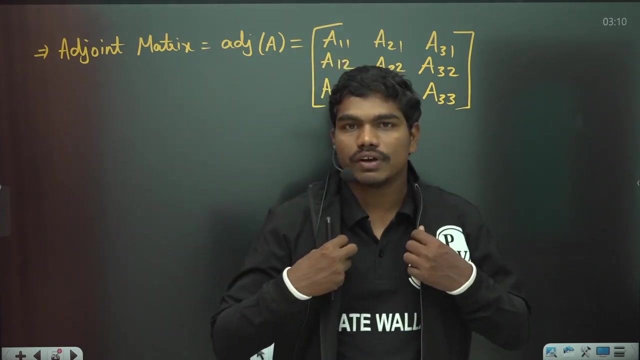 a23, a31, a32, a33. okay, so let us suppose this is the cofactor, i mean this adjoint matrix. now let us see what happens. i want to show you one very important result at this moment, because that result is the main basic for, or the concept of, you know, adjoint and inverse of the matrix. 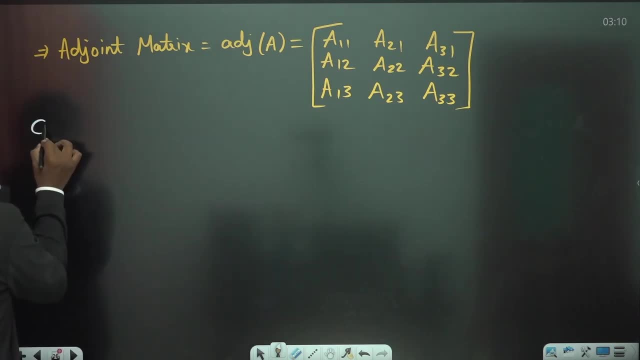 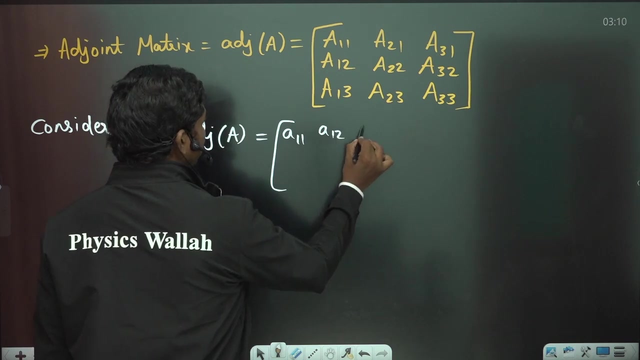 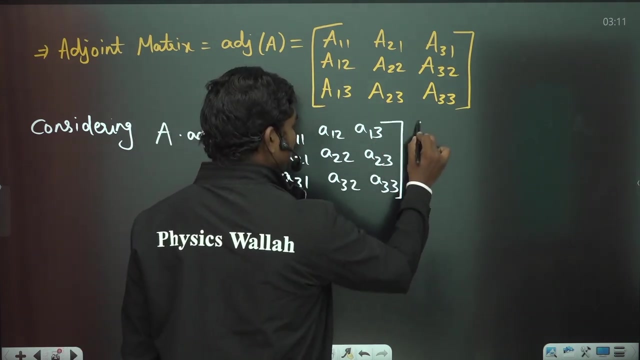 actually okay. so let us see here. so considering considering a in to joint of a, for example, if you consider this a into adjoint of a. look, i am considering this: a11, a12, a13, these are normal elements. so matrix a, elements a31, a32 and a33. now let us suppose, if you multiply this with this adjoint matrix, which is a11, a21. 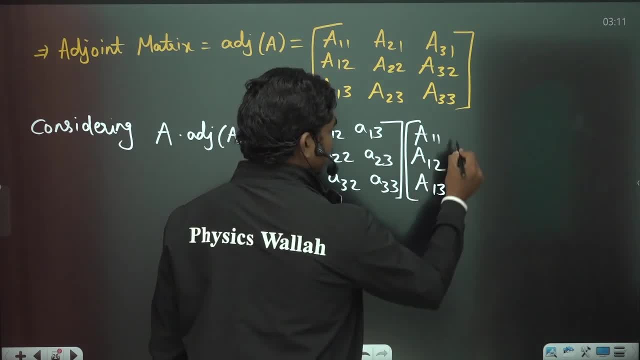 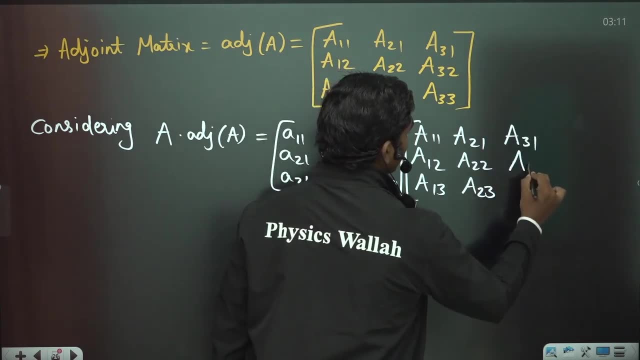 a32 and a13, because we have transposed it- a21, a2, a23, a31, a32 and a33, for example. so let us suppose: if you have this, okay, so once you have this, for example. so let us suppose: if you have this, okay, so once you have this, then see what's happening. 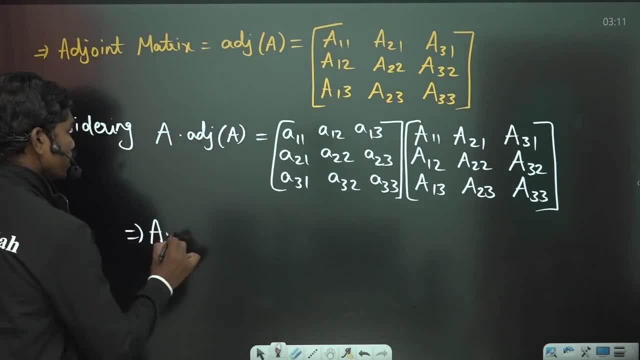 here, if you multiply these two, a into adjoint of a, a into adjoint of a, is equal to look, try to observe carefully now for getting the for today we have one more example, which is a, and this is, for example, the first row, first column element. you need to multiply the first row with the first column and. 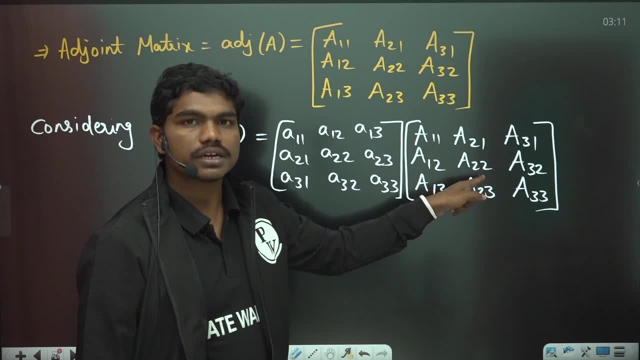 all this means. if i write a 2 2, that means this capital a 2 2 is nothing but cofactor of this element small a 2 2. if i write capital a 3 2, this capital a 3 2 is nothing but cofactor of the. 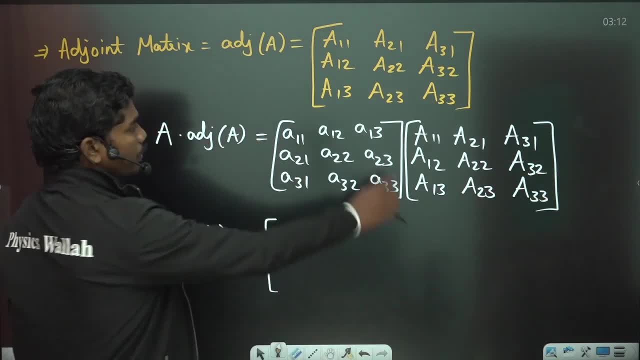 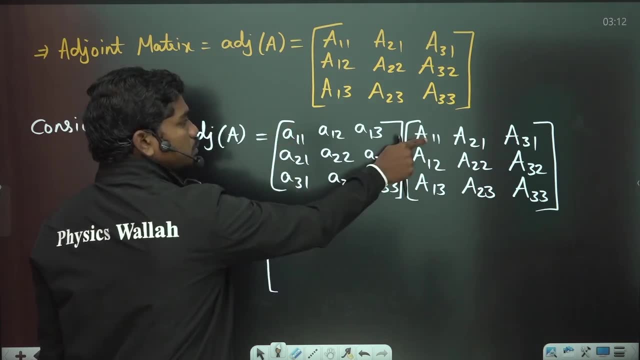 element small: a 3- 2. correct. now let us see if you multiply. if you multiply this first row with the first column, a 1- 1 into capital a 1 1 means you are multiplying the element with its corresponding cofactor plus a 1- 2 into capital a 1- 2. plus a 1: 3 into capital a 1- 3. so if you see the first, 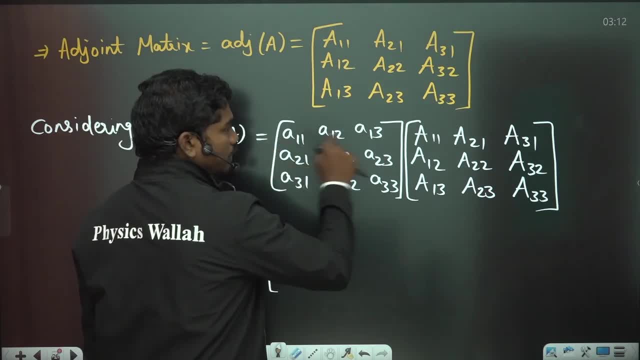 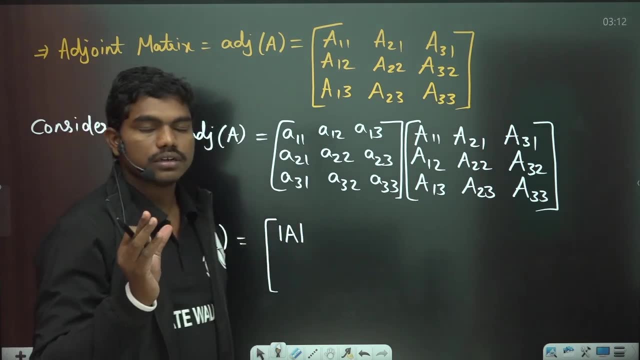 row, first column element is nothing but the sum of product of elements of this row with its corresponding cofactors. so, which means you are going to get determinant of a here, correct? so the first element that you are going to get is actually the dot a next, if you see first row. 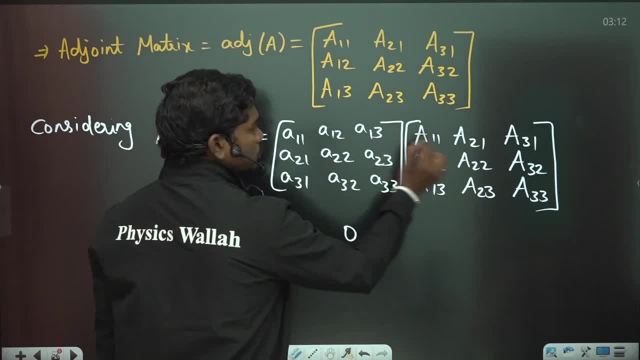 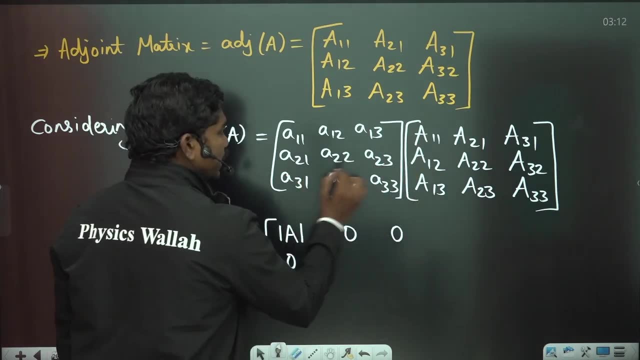 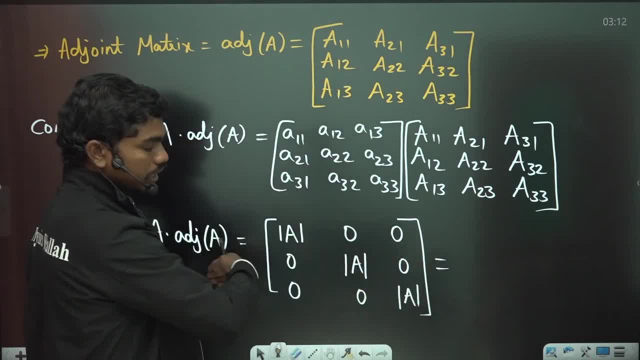 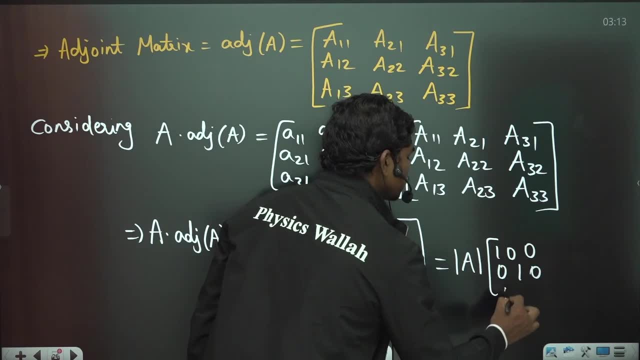 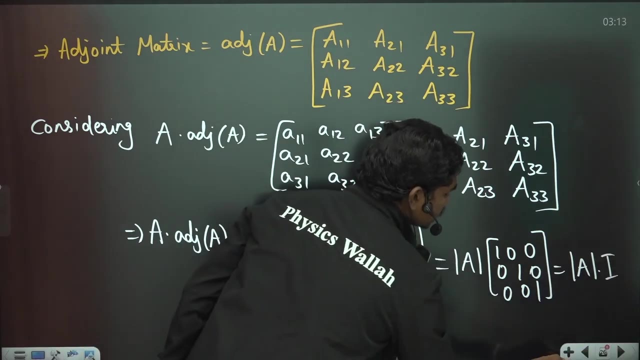 important thing and from this matrix, if you take this debt a constant as multiplication, you will have debt a times of one, zero, zero, zero, one, zero, zero, zero one, so which is nothing but debt a into identity matrix. so if you take any square matrix, this result is very much. 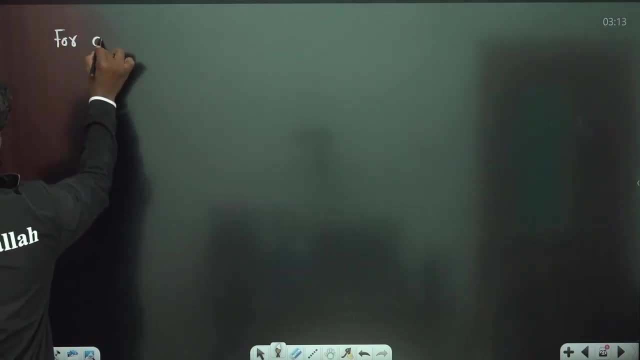 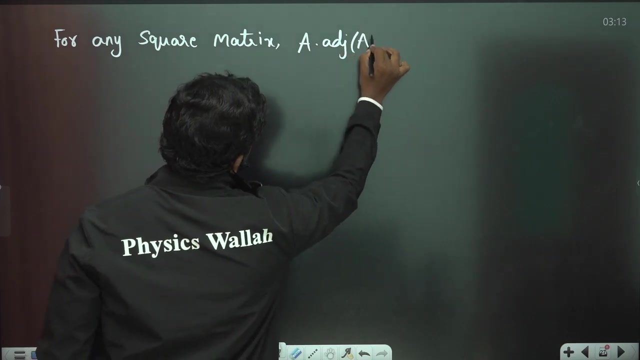 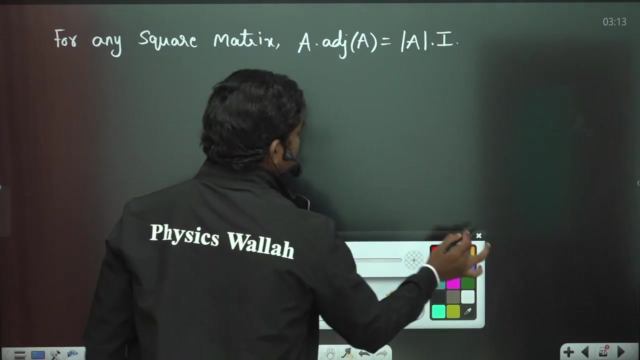 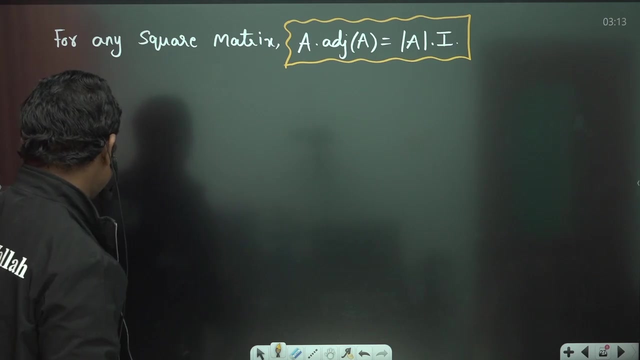 important that for any square matrix, for any square matrix, a into adjoint of a, a into adjoint of a is equal to debt a times of that matrix. okay, so this, This is one very, very important equation. and this equation is coming here from the definition of determinant, because if you see, here you are supposed to write that here only if you 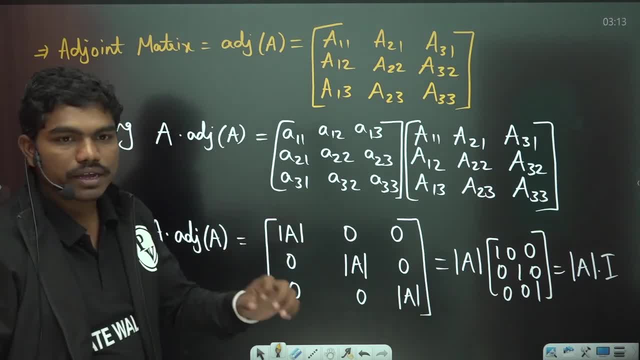 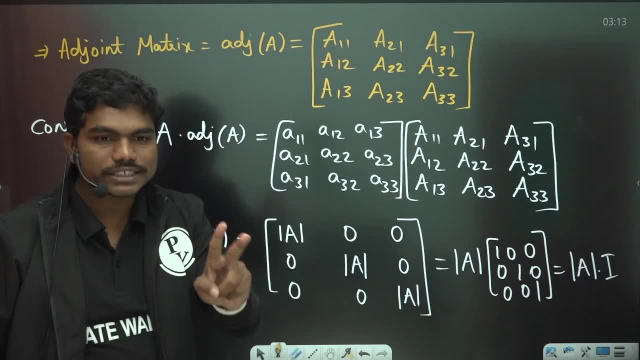 know the definition of that incorrect, because you are actually summing up the product of this elements with its corresponding cofactors, correct? So for writing this matrix here, you should know two conditions: that if you multiply elements of a row or column with its corresponding cofactors you will get determinant, and if 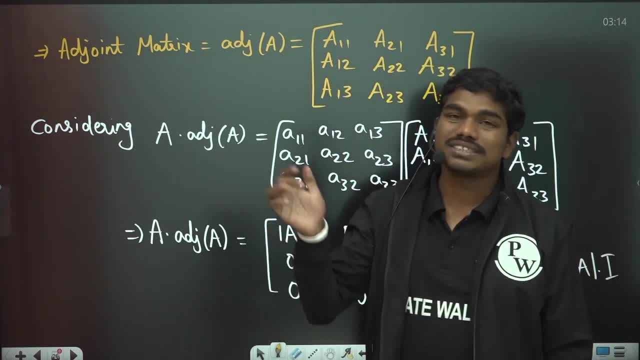 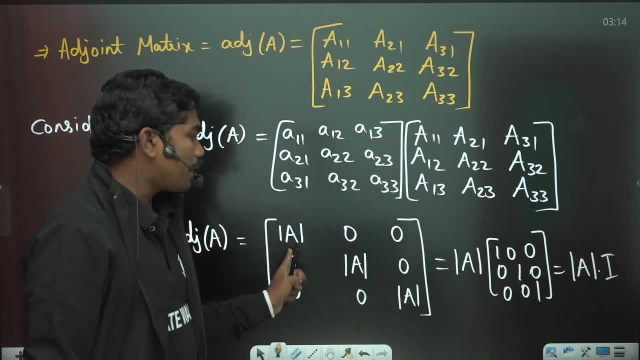 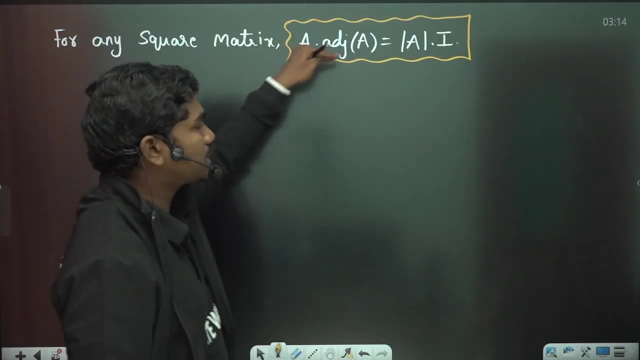 you get. if you multiply elements of a row or column with some other cofactors, you will get zero. So that's how these two rules will help you out. in writing this matrix, I mean this determinant of A- 0, 0, 0.A, 0 and 0- 0.A, and you were able to form this equation. 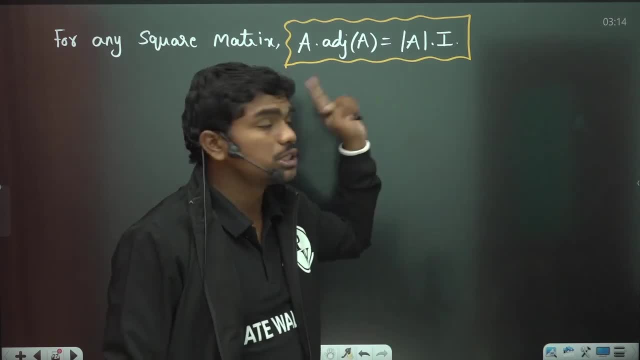 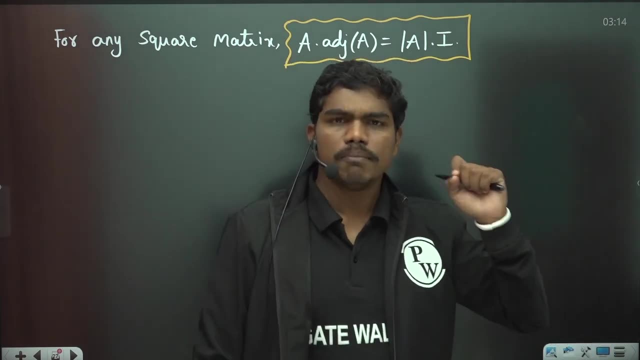 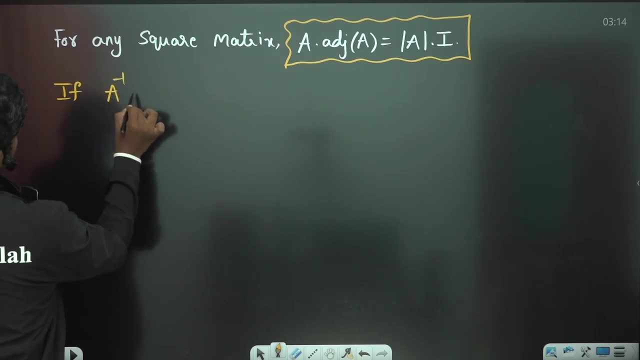 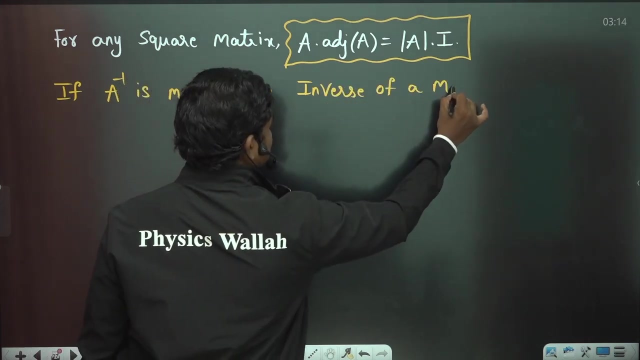 with the knowledge of definition of determinant. okay, and why this equation is very, very important, because this is the equation that gives you a fundamental for the concept of inverse of a matrix. okay, multiplicative inverse, If you see, Look, if A inverse is multiplicative, multiplicative inverse of a matrix, then definitely, you know. 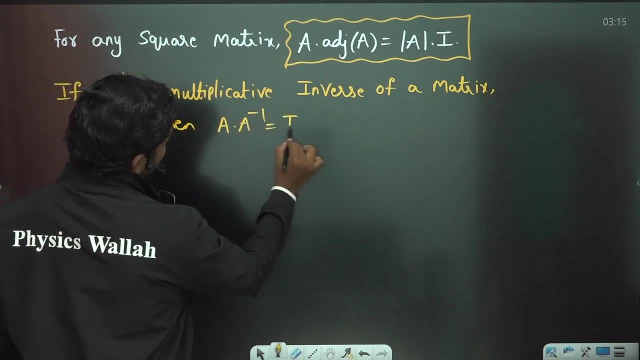 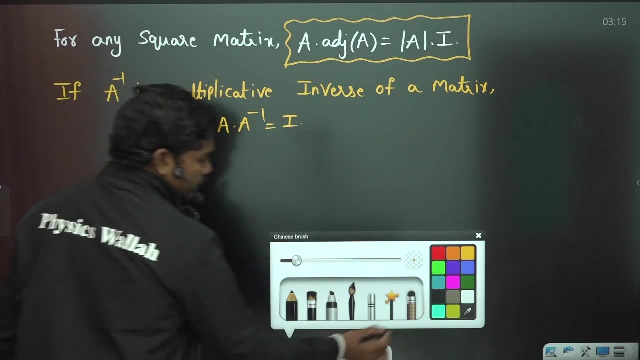 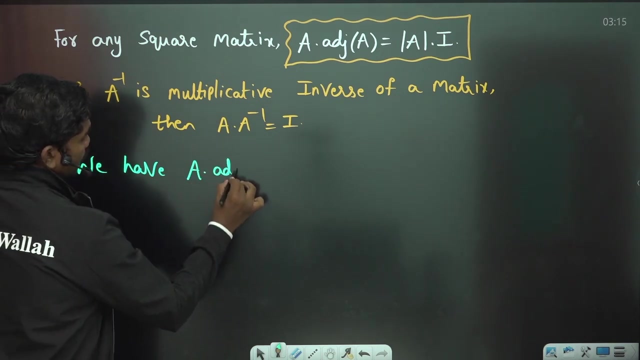 that A into A inverse gives you identity matrix, correct? Now let us see How to calculate the inverse of this matrix. look, I'll tell you for this equation we have. look, we have: A into adjoint of A is equal to det A into I. 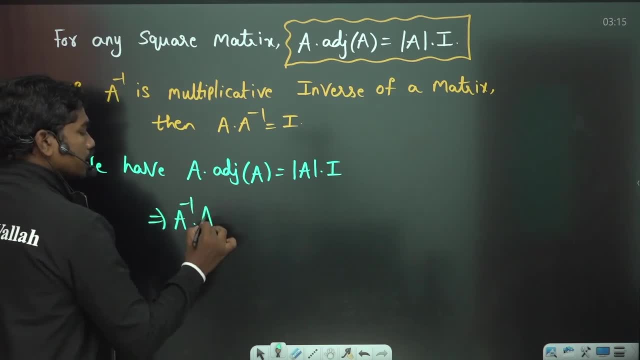 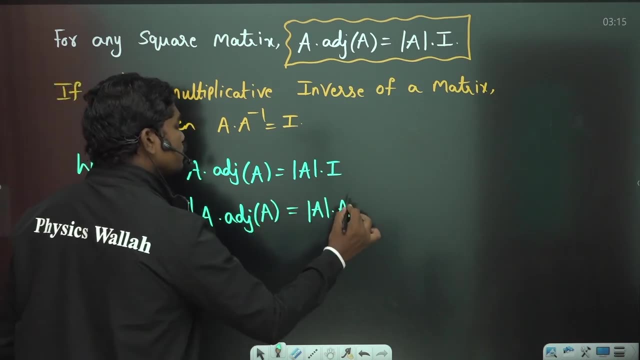 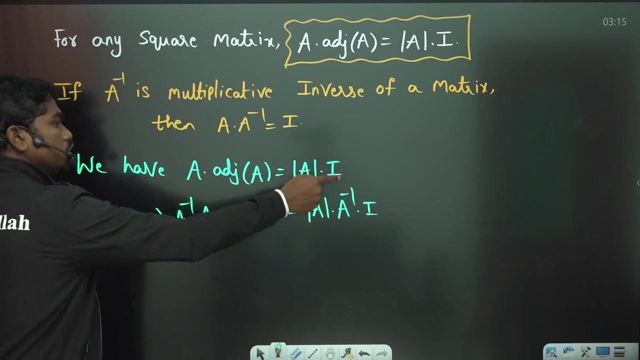 So if you multiply this, A inverse on both sides, A inverse into A into adjoint A is equal to det, A is anyhow constant. A into A inverse into- I look in matrices it is very, very important: if you are multiplying A inverse before this, here also you should multiply before this. okay, this is one because 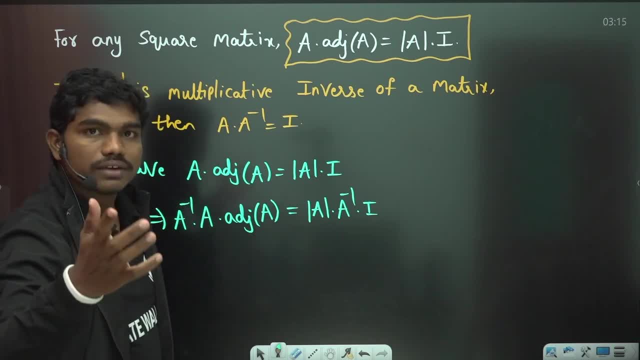 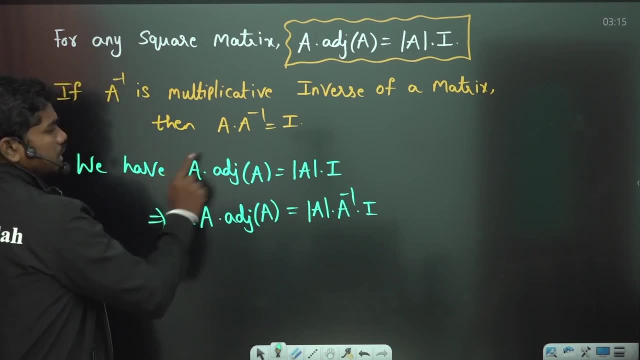 in numbers. we don't follow this generally, but in matrices, you have seen, the order of multiplication is of very much importance. So that's why if you see, if you are multiplying this A inverse here, then definitely you should multiply A inverse before this. I okay. 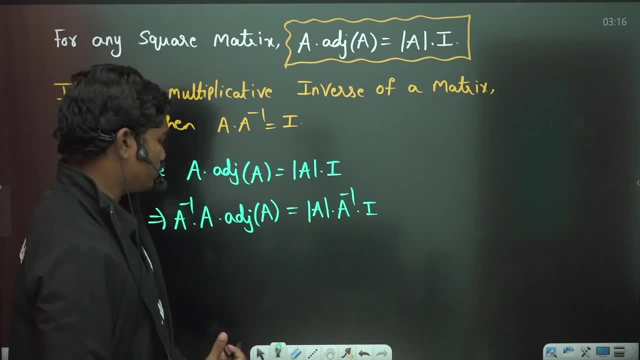 So now we have seen matrix multiplication is, you know, associate to basically cut. So I can take multiplication of these two first and then this two. Now, if you see, A inverse into A is nothing but I into adjoint A is equal to det, A into 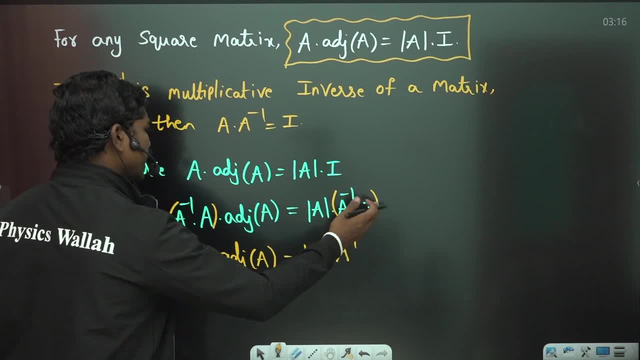 A inverse, because A inverse into I is again a inverse. identity matrix is just an identity. So if you multiply any matrix with identity, you'll get the same matrix. So this gives you adjoint of A and this is equal to det A into I. 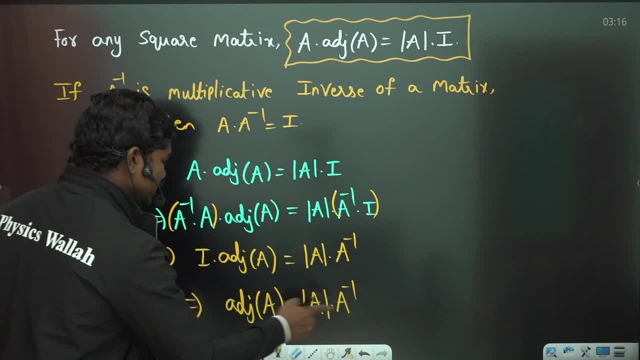 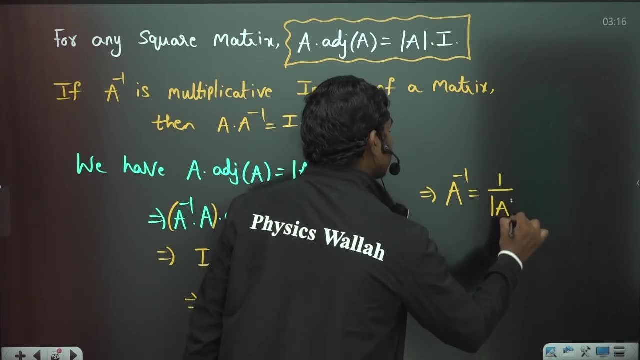 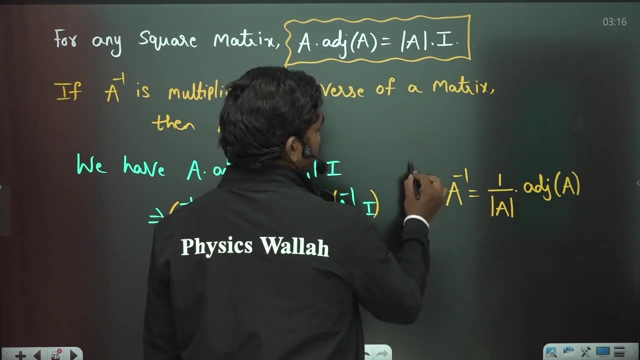 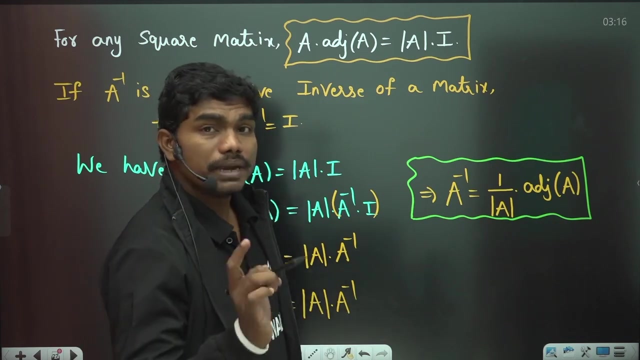 Okay, So this Yes into a inverse. so from this equation you will end up with one formula: that a inverse is equal to 1 by debt a into a joint of a, and this is the fundamental equation which is known to you from your basic schooling. but you never know what is why this equation is coming, and many times. 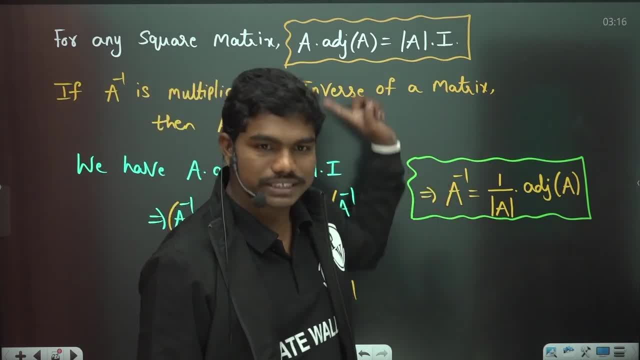 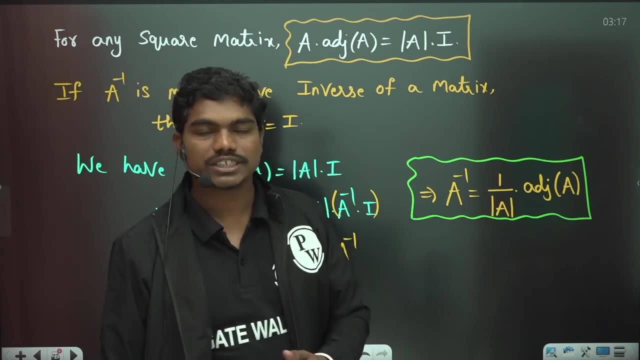 they tell you, for a inverse to exist, this debt a should not be equal to 0. this is the reason, this is how this is coming. and if this inverse has to exist, then definitely this debt a should not be 0 because, you know, definition by 0 is not defined. so that's why this, you know this. 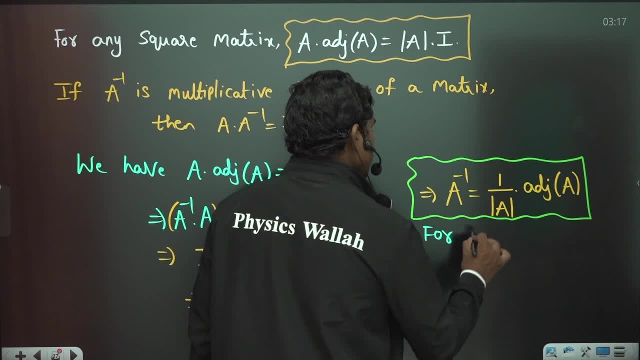 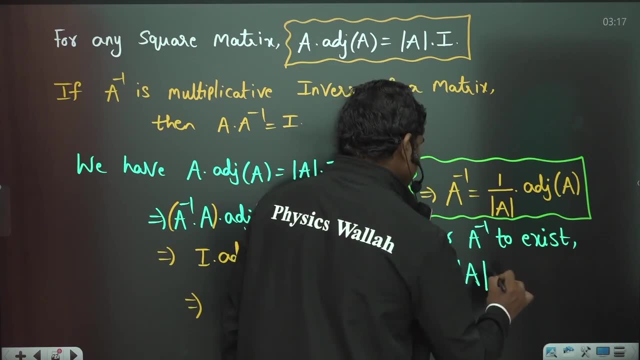 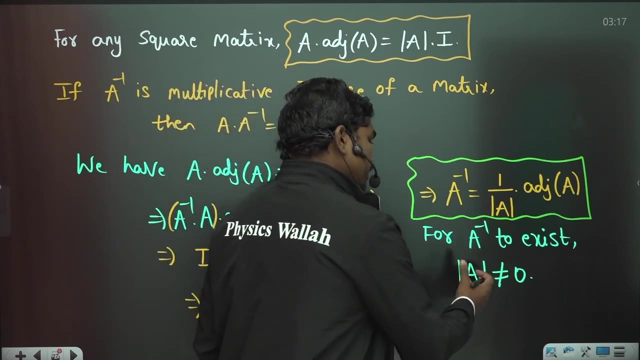 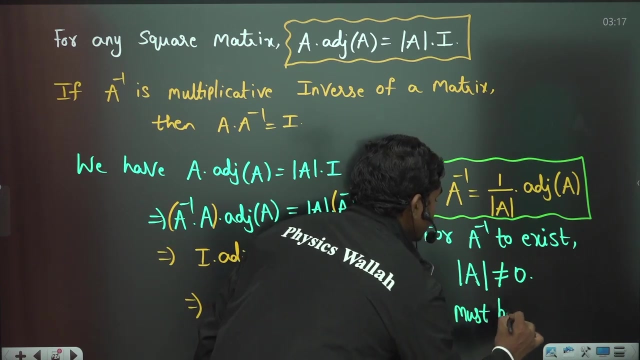 for a inverse to exist. you can say: for a inverse to exist, this debt, a should not be equal to 0, clear. so this means- if you see, we generally name this with some technical term- a is a should be a must be non-singular, non-singular matrix. you can say a must be non-singular matrix. okay, so this capital a. 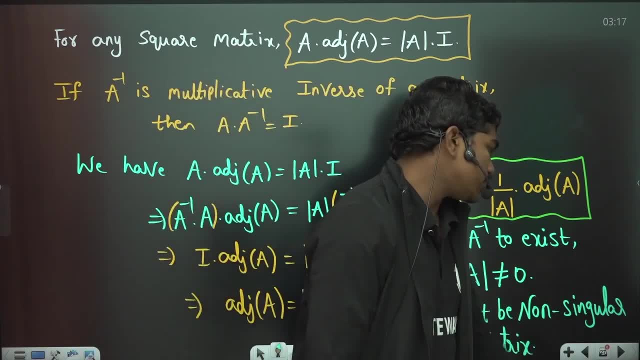 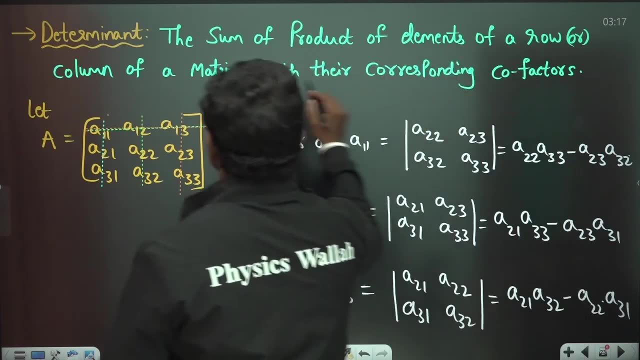 must be non-singular matrix. okay, and what's the meaning of singularity? basically, singularity means determinant is equal to 0, anyhow, okay, and here i would like to add one more point. it is denoted as. it is denoted as you can write here. it is denoted as: 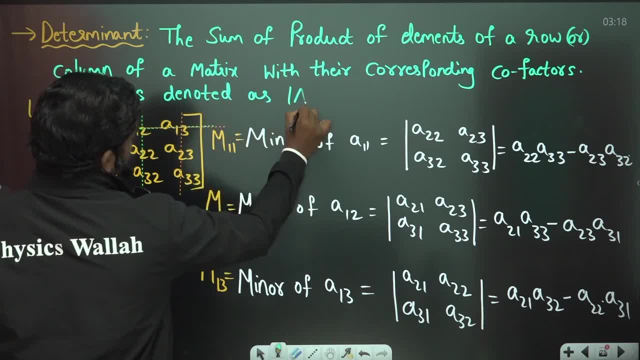 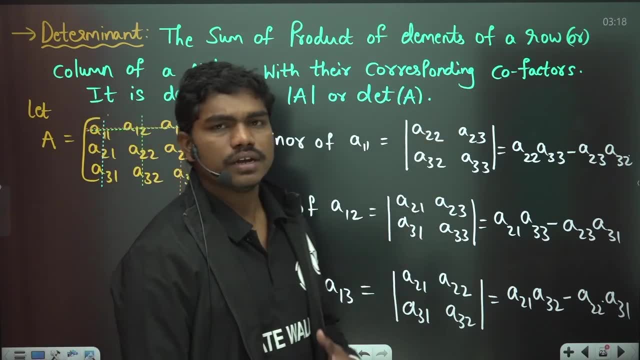 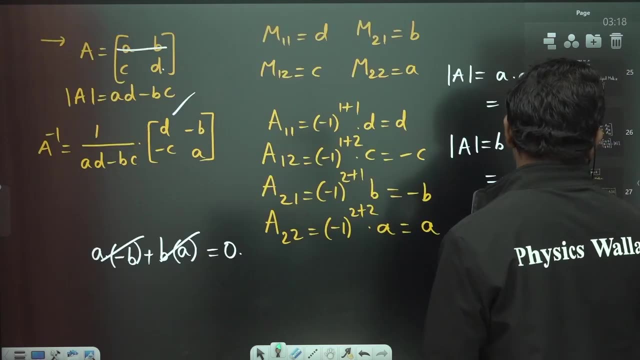 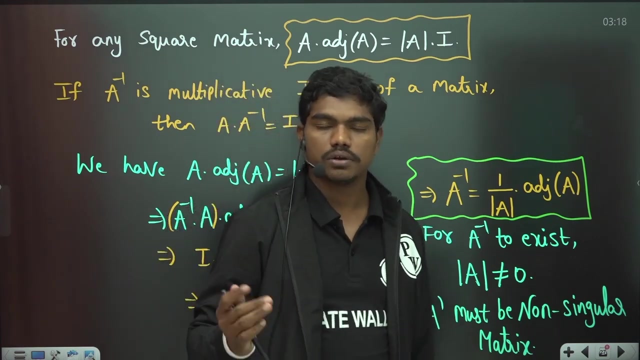 a debt, a, or sometimes you write this det of a: both are same, both they mean determinant, is the actual thing that they are asking you for. okay, so now if you see, uh, fine, so this is the fundamental equation, that a inverse is equal to 1 by the t a times of a joint a is one very important, uh you. 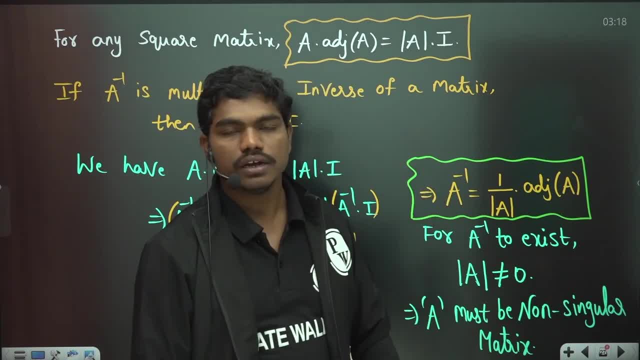 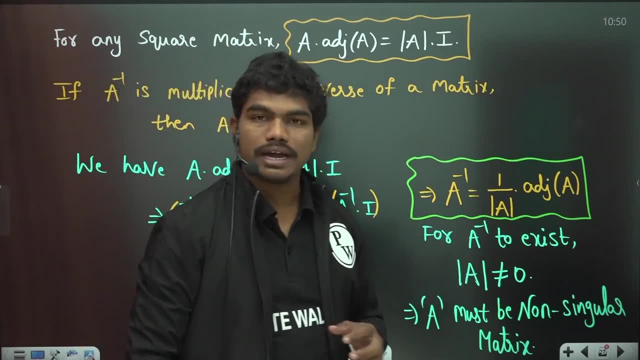 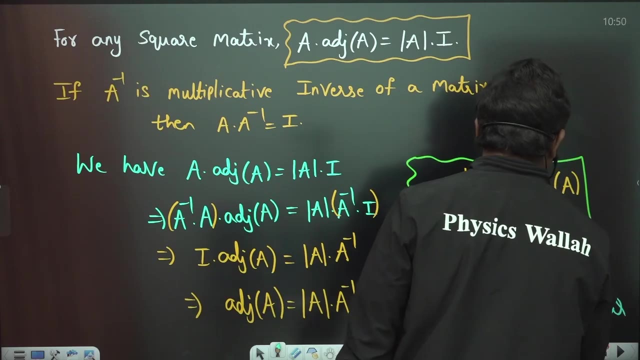 know, uh, fundamental equation for calculating inverse of the matrices. okay, so, so we have seen that this fundamental equation- a into a joint of a is equal to t, a into i is the most fundamental equation that gives rise for this a inverse matrix. now let us try to look at some properties of this. 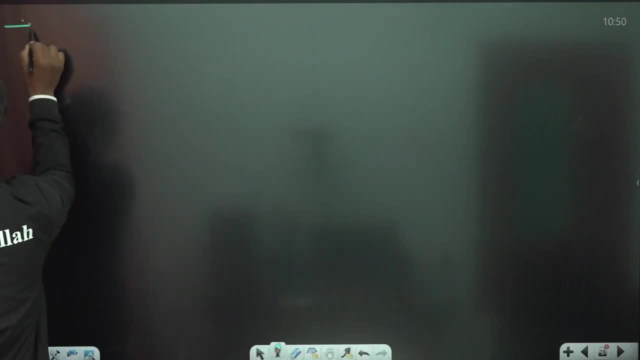 determinants. okay, so if you see properties of determinants. properties of determinants, because this is one of the very important part where general equations turn over in data examination. so properties of determinants. properties of determinants. now let us see certain properties. okay, so if straight away, first property, you can write the determinant of: 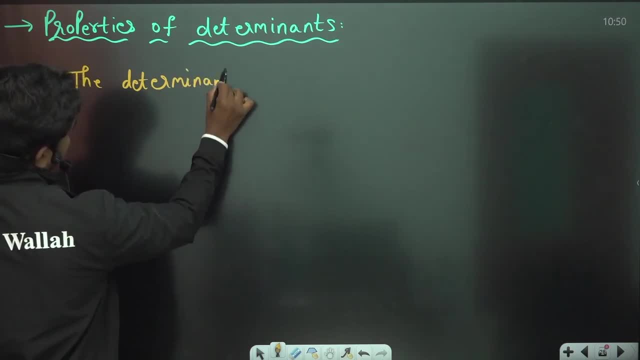 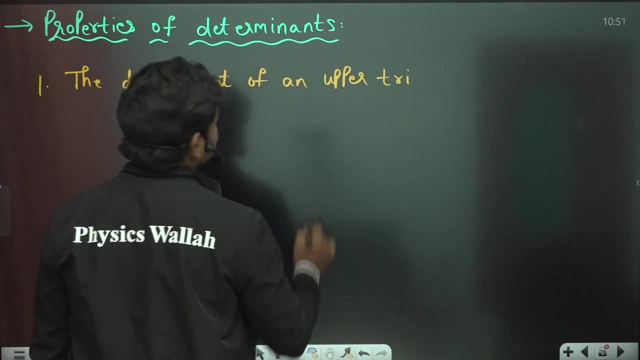 the determinant of the determinant of an upper triangular, the determinant of a. you can write a here and that's not the oh, i think there is some issue with the determinant of a. you can write a here and that's not the. oh, i think there is some issue. 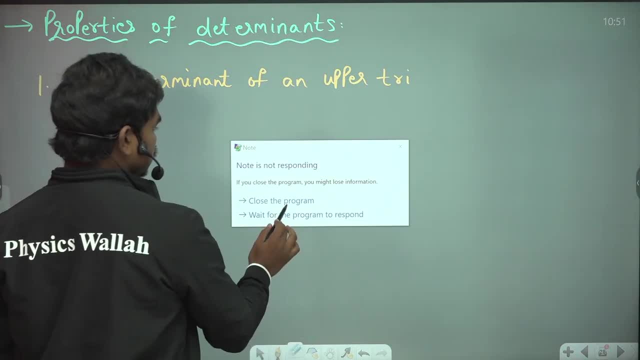 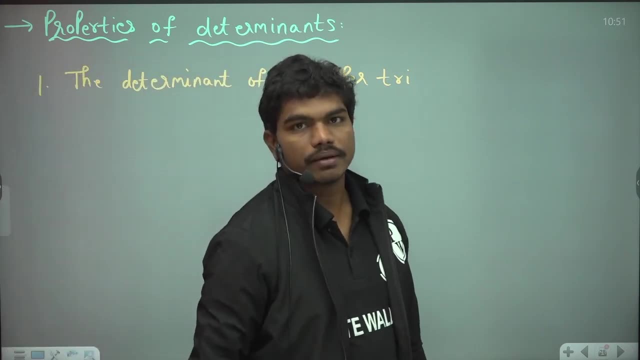 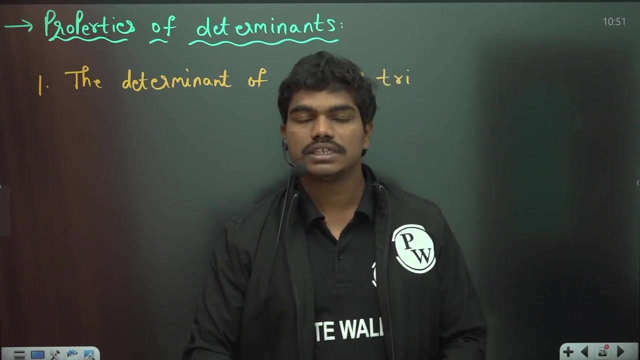 just a minute. oh, uh, just a minute, so wait for the program to respond. so, uh, yeah. so i hope things are going fine. you are getting enough time to make your notes. i'm not coming up with a ppt, because you know when i write, you'll also have some time to make your own notes. okay, and this video series. 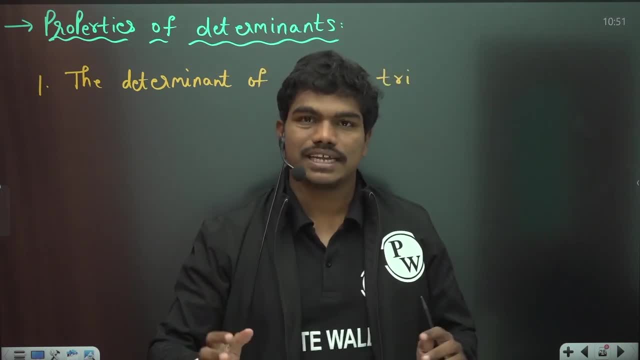 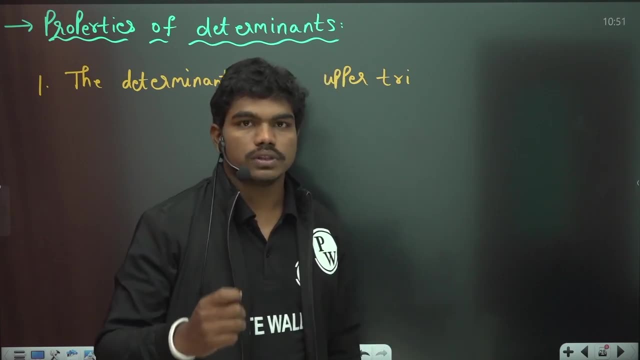 definitely is going to get all the concepts of your maths in very less time. so hardly. if you spend some four to five hours every day for some seven to eight days, let us say you will be very clear through the mathematics portion. okay, so that helps you in getting very good marks in the math. 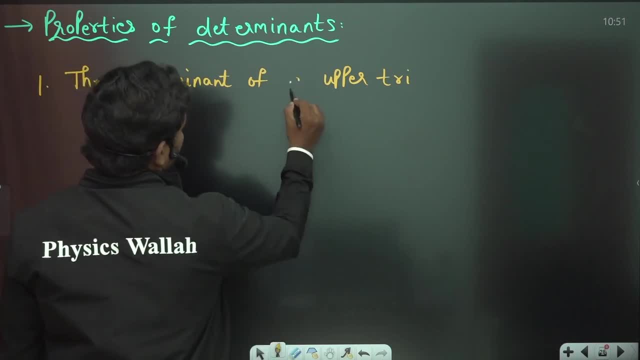 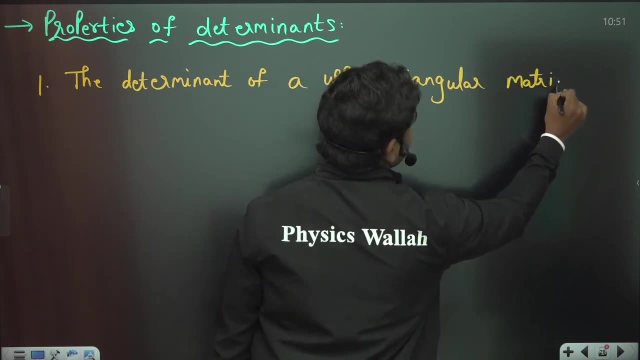 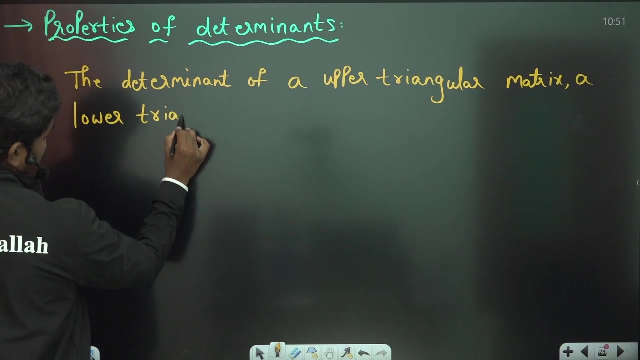 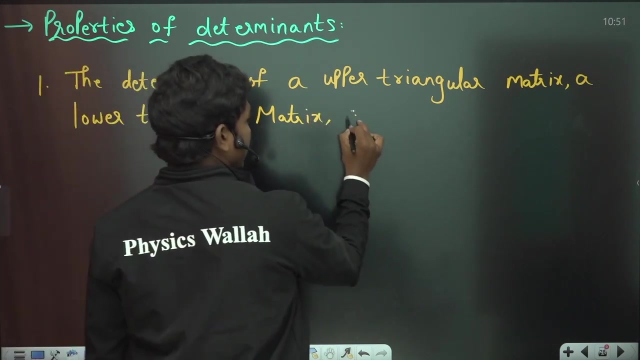 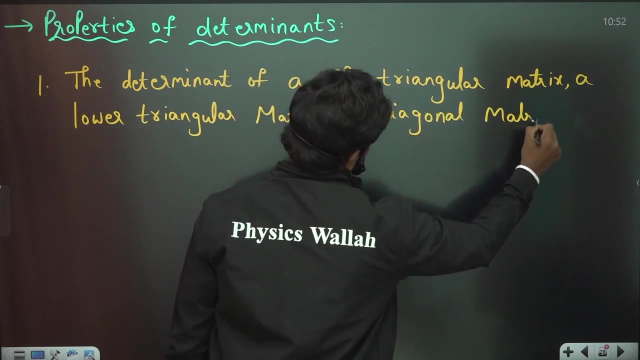 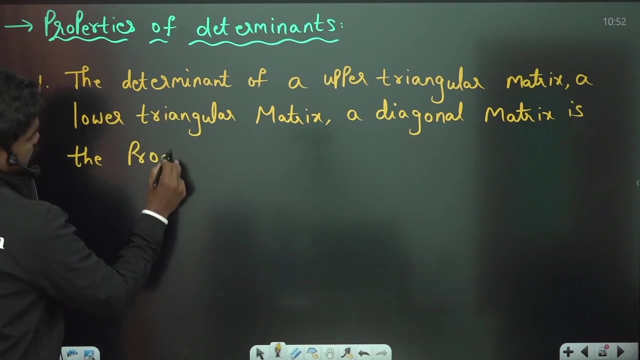 gate, obviously. so anyhow, let us try to continue here. so of a upper triangular matrix, of a upper triangular matrix or a lower triangular matrix, a lower triangular matrix, a lower triangular matrix or a diagonal matrix, a diagonal matrix, a diagonal matrix is the product of, is the product of principal diagonal elements of the matrix. so this is one very, very important. 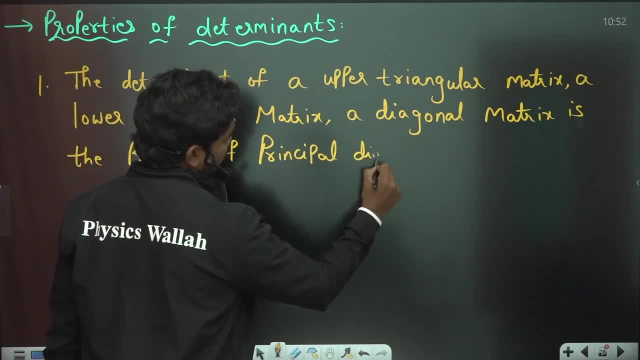 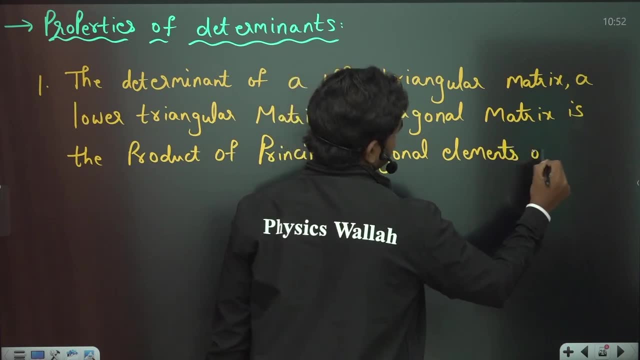 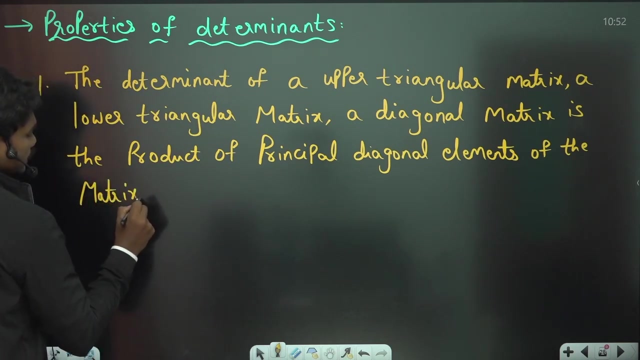 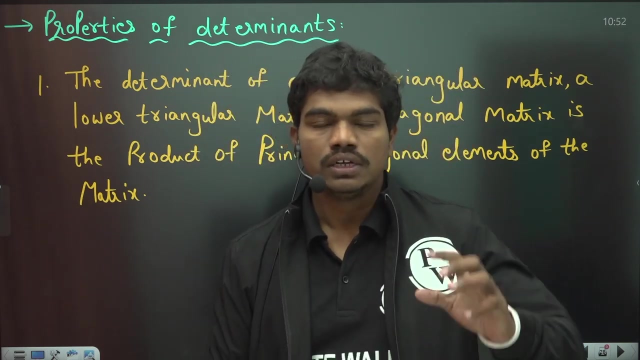 property. so principal diagonal elements of the matrix, principal diagonal elements of the matrix, okay, of the matrix. so this is one really very important property because many times what they give you, they'll give you matrices of high orders, four by four, five by five and all. so when they give you such orders, 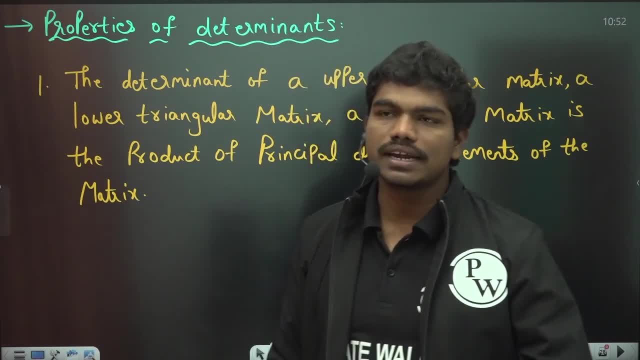 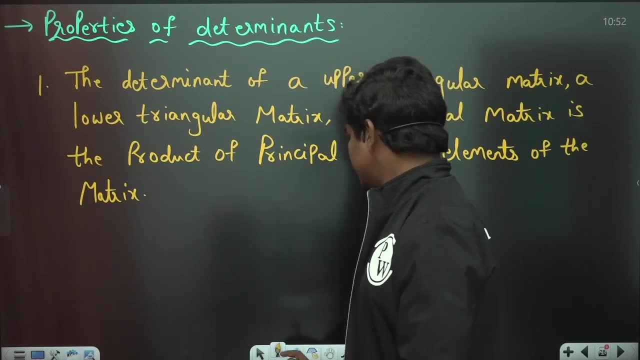 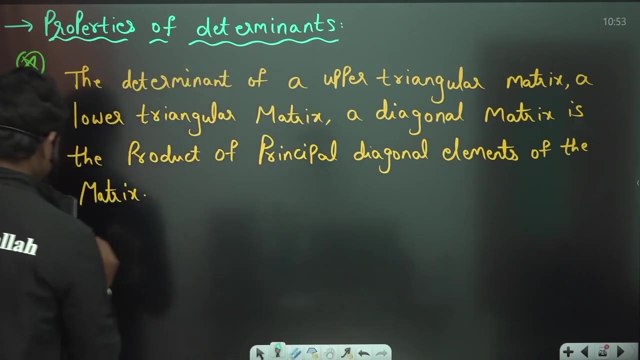 this normal procedure for writing the determinant will not work, you know that effective. so in such cases you can use this property so directly. if you multiply the product of the principal diagonal elements, you will get the determinant value. so this first property is really some very good, you know, property in matrices. and second, i would like to give you the if. 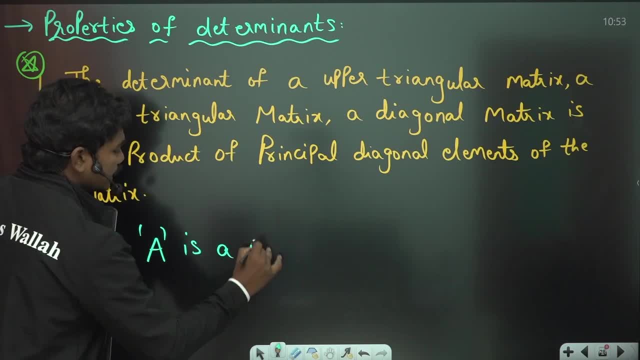 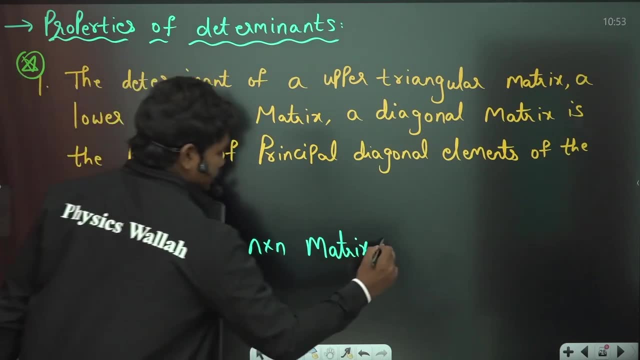 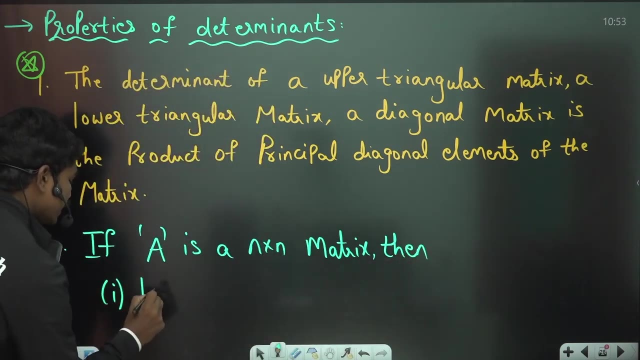 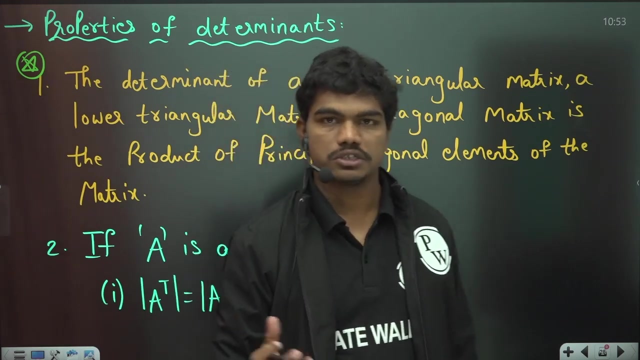 a is an n by n matrix. if a is a n by n matrix, then then you can write: then first, then, first, debt of a transpose will be same as determinant of a. so basically, if you calculate the determinant of a matrix or its transpose, both the values turns out to be the same thing. okay. and second, 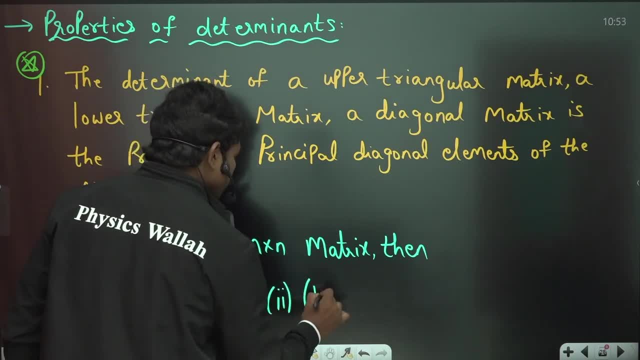 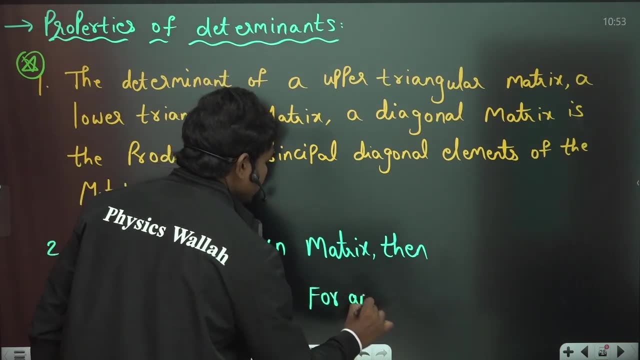 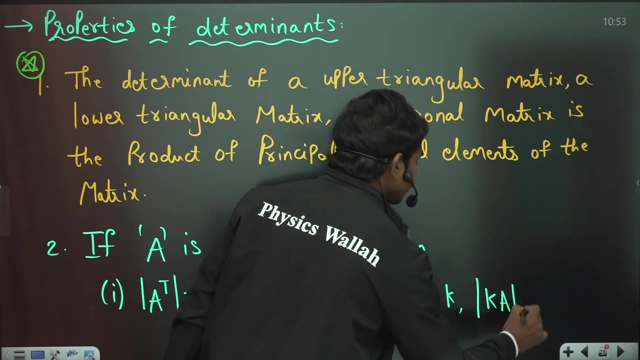 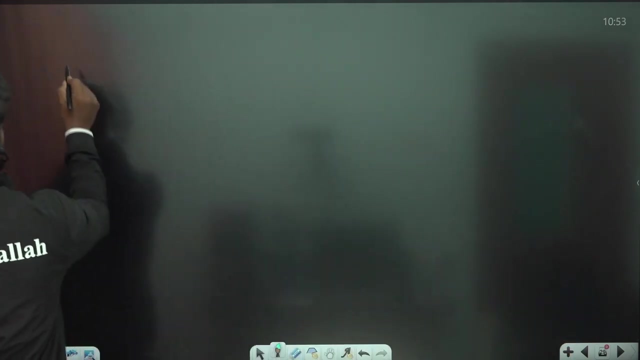 a, a k into a whole power. and or you can say debt of k a for any scalar k, for any scalar k, debt of k? a is equal to k power n times of this debt a. look, basically, you might have known this property. let us suppose, if i have this determinant, a 1, 1 a, 1, 2 b, 1, 1 b. or you can say a 2, 1, basically. 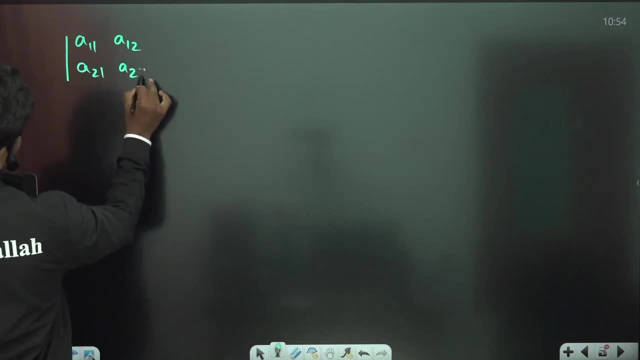 a 2: 1 and a 2: 2. let us suppose if this is equal to determinant of a. now let us suppose if i want to calculate determinant of one particular matrix, like, for example, debt of k 1 a 1 1. k 1 a 1, 2 means. 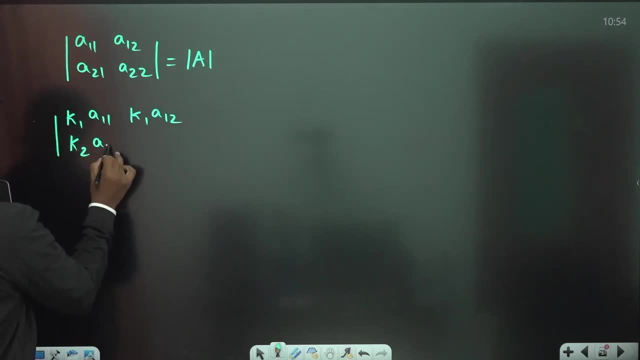 the first row elements are multiplied by a constant k 1 and second row elements are multiplied by a constant k 2. so in such case, if i want to calculate the determinant of this matrix, you can see this: k 1 can be taken out from this first row, so k 1 can be taken out from this first row, so k 1 can be. 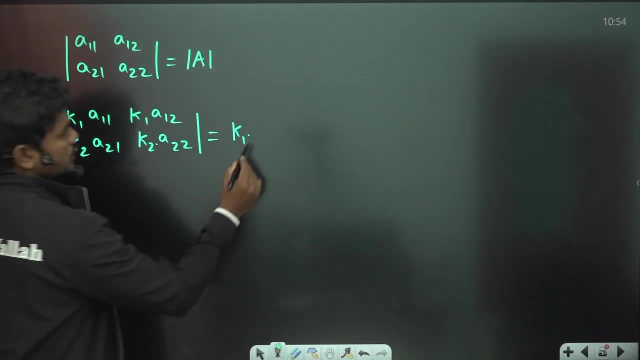 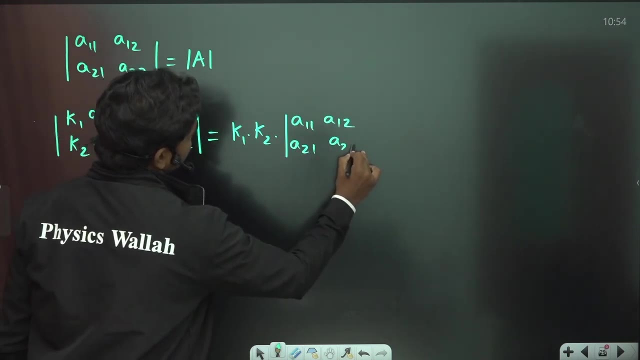 taken out from this first row. similarly, from this second row you can take a k 2 out, so k 1 into k 2 times of this debt. a 1 1 a 1, 2 a 2, 1 a 2, 2, basically here. okay. so now this: a 1 1 a 1 to this. 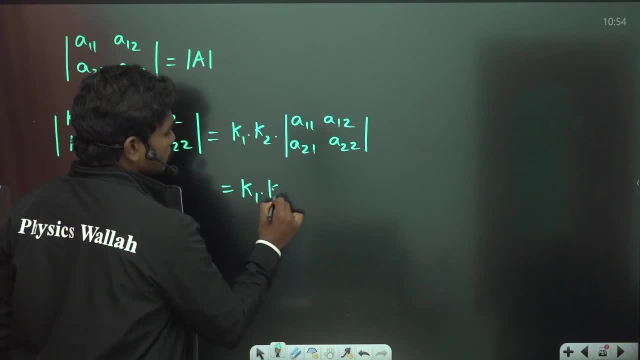 determinant of 2 by 2 is again nothing but k 1 into k 2 times of that a here. okay. now if you see carefully, when a matrix is multiplied by a constant, what happens? this k 1, k 2 values will be same. okay, because every element of the matrix is multiplied by some constant. so let us suppose 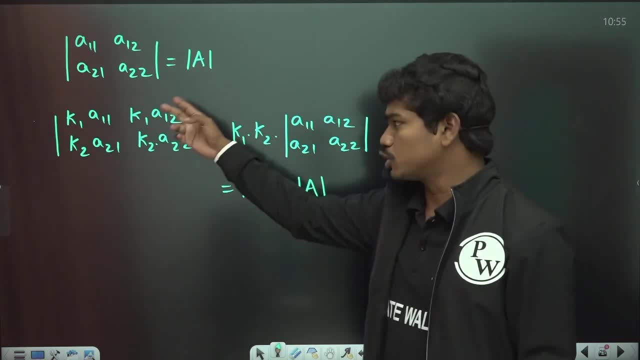 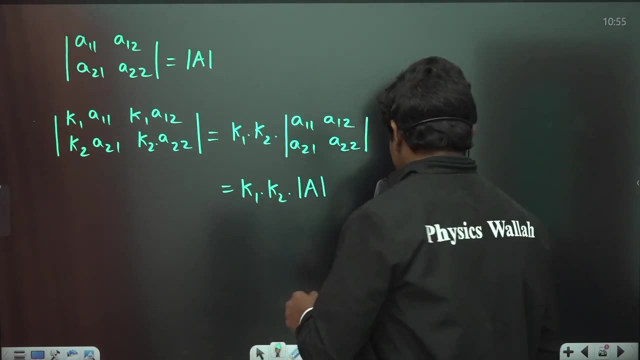 k 1 is equal to k 2. this becomes k square times that here, because it's a 2 by 2. so if the matrix is of order n by n, then definitely you will have k power n times of determinant of it. okay, now we. 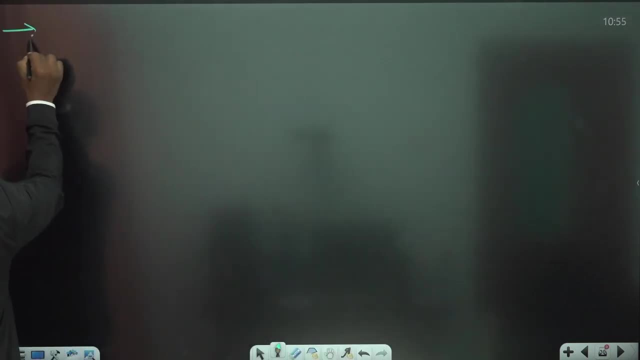 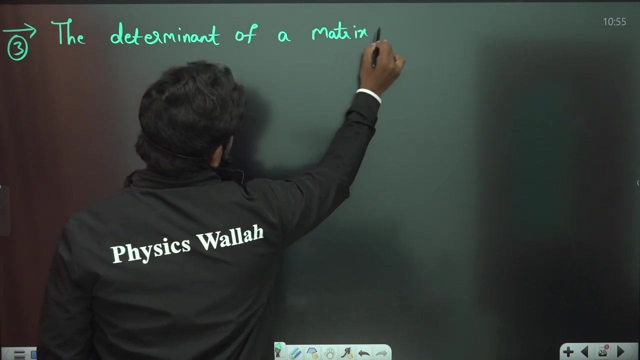 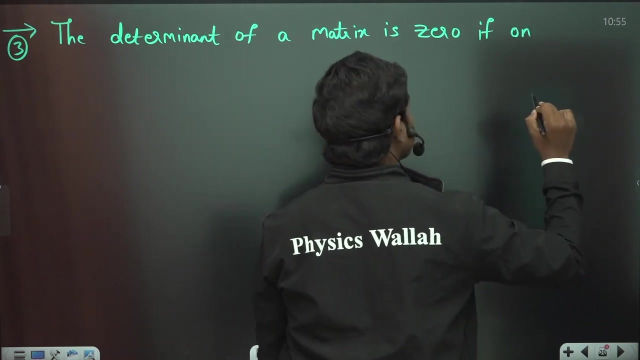 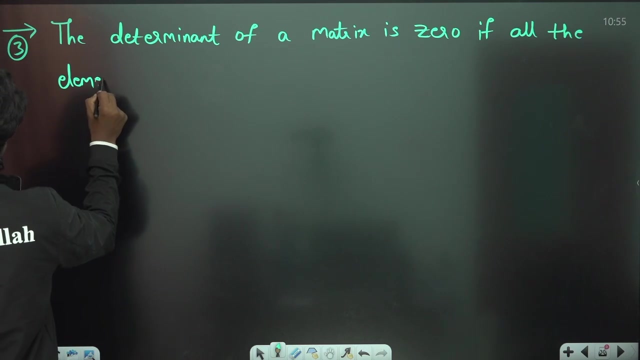 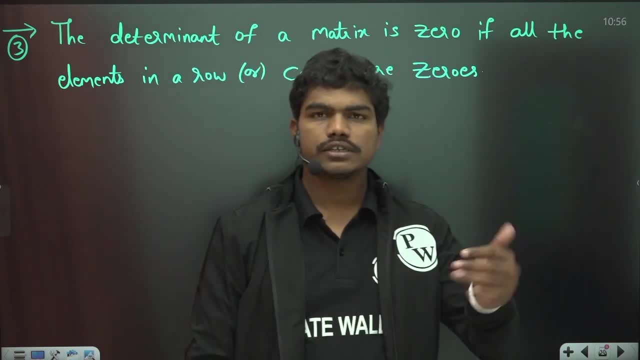 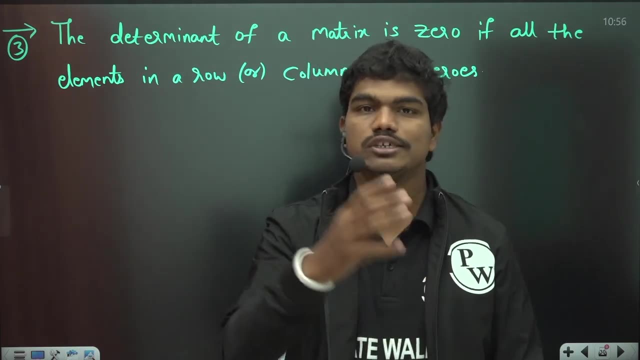 us suppose, if you have a particular determinant in which one complete row is zero, or maybe one complete column is zero, then definitely, if you take the product of cofactors with respect to that, then you know, obviously zero into some cofactor of that element, plus again zero into something, plus again zero into something. so 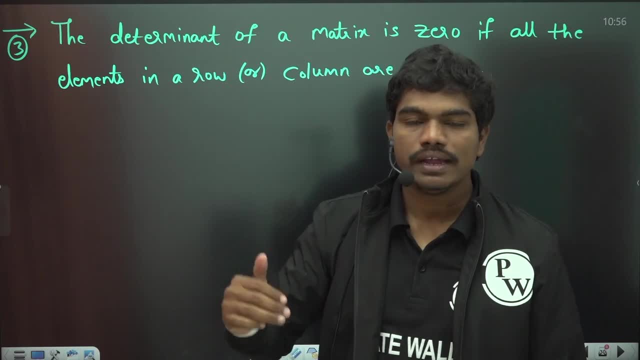 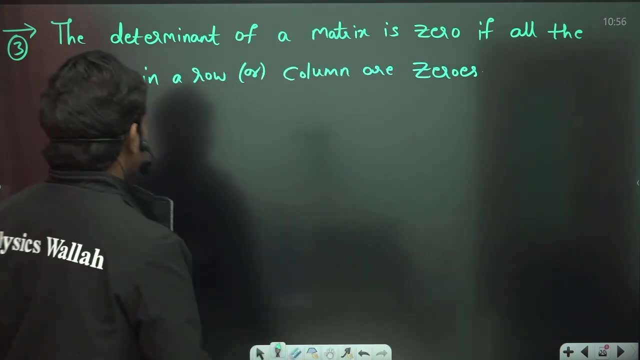 this total will give you a zero value. that's the reason why in determinants, if one row or one column is completely zero, then the determinant value is going to be zero here. okay, now example. you can see. I'll give you one example also better. so if you see, determinant of this root, 3 by 2. 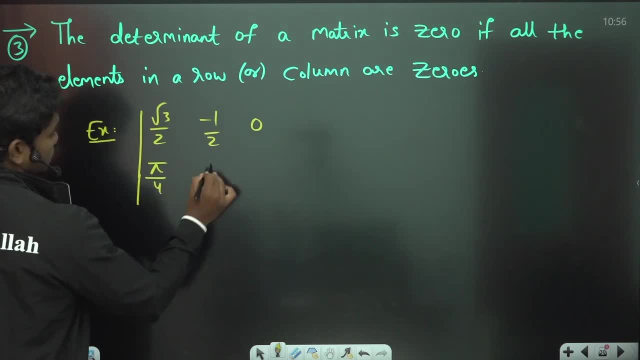 okay. so again pi by 4, 2 by 8 or 2 by lon 2, 0. then again, if you see for example some values, some random values: minus 1 by 2, okay, e power 4: 0. so let us suppose, if I give you some determinant like: 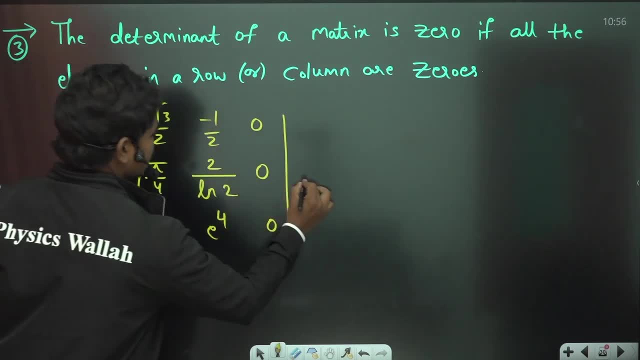 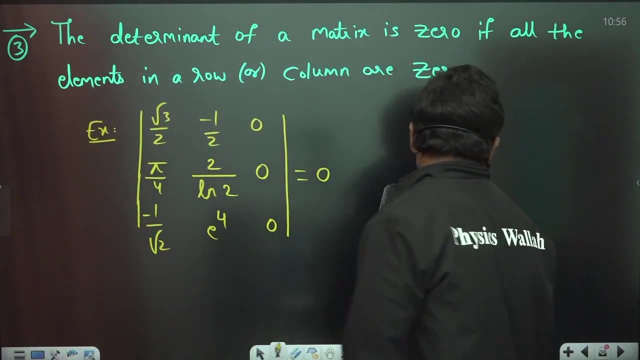 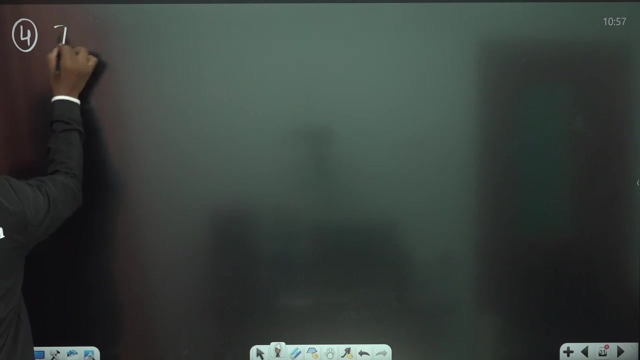 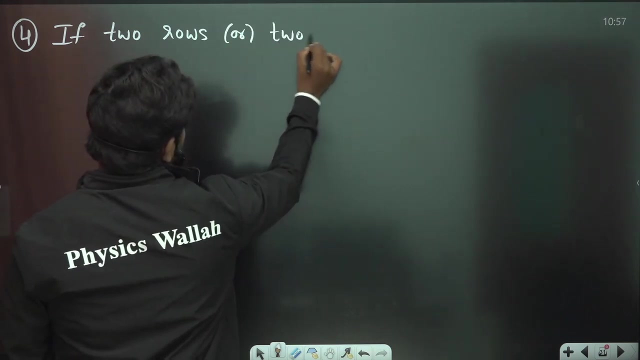 this, since this one complete column is zero, this determinant value is definitely 0, irrespective of these elements. so sometimes they can ask you these kind of things. okay, so you should be little careful. and fourth property: you know, fourth property if two rows, if two rows or two columns, if two rows or two columns of a. 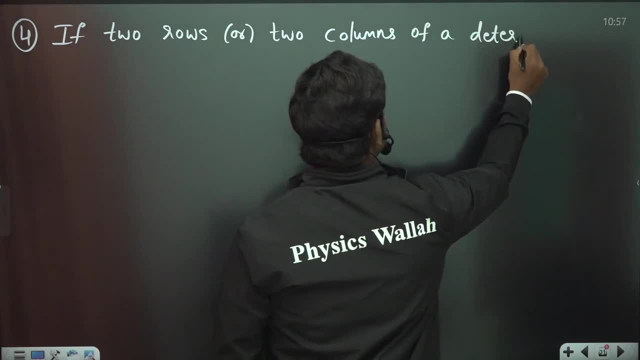 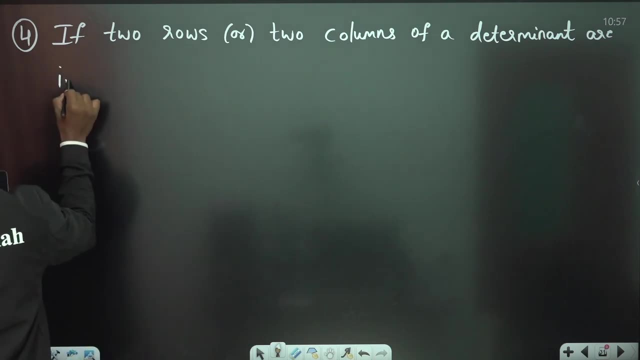 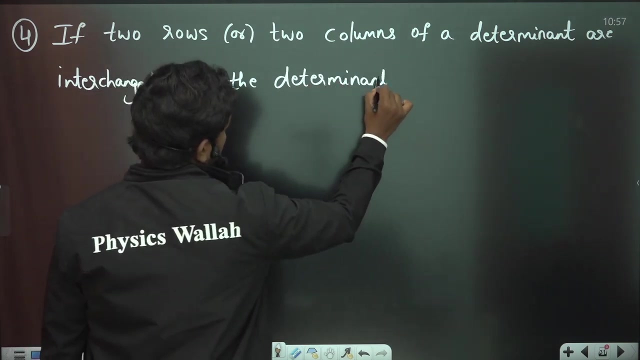 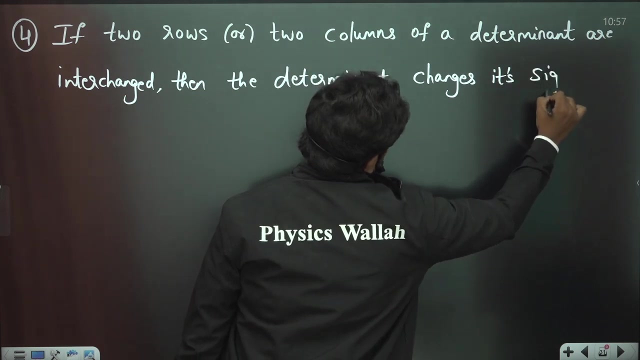 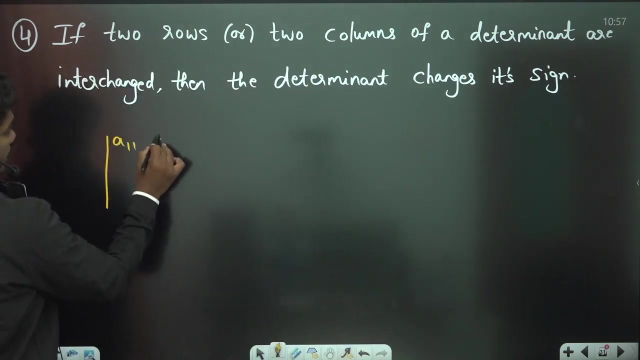 determinant are interchanged, of a determinant, of a determinant are interchanged. if these are interchanged, interchanged, then the determinant changes its sign, then the determinant changes its sign, changes its sign. so basically, what I'm telling here is: let us suppose you have this determinant: a 1, 1 a 1, 2 a 1, 3 a 2, 1 a 2, 2 a 2, 3. similarly, a 3, 1 a 2, 3 a 2, 3 a 2, 1 a 2, 2 a 2, 3 a 2, 1 a 2, 2 a 2, 2. 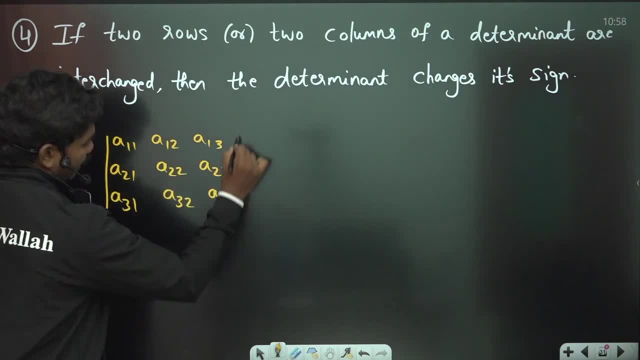 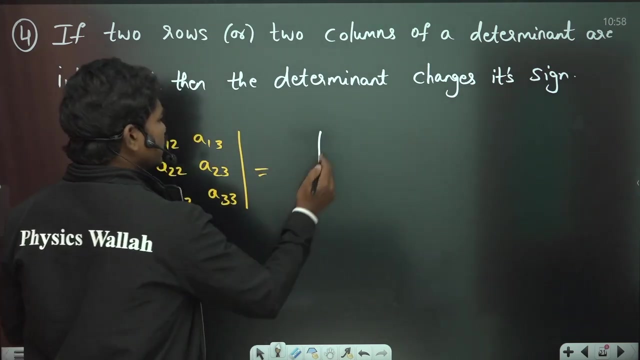 a 32 and a 33. so let us suppose if you have this determinant now, this determinant will be equal to the same determinant value when you swap two rows or two columns. they come say minus sign means. let us suppose if i swap second and third row, for example, or second and third column, anything, i'm 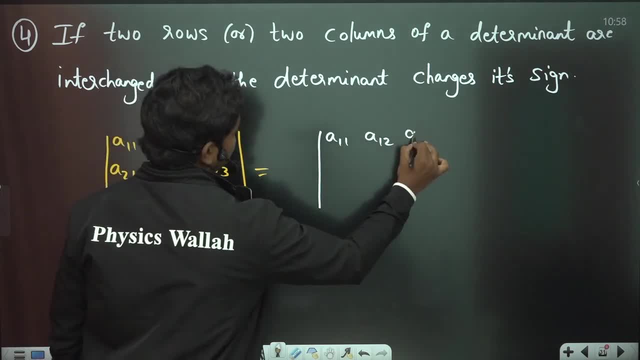 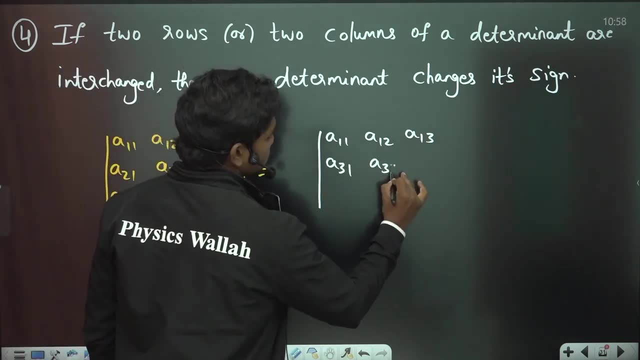 swapping second and third row, so a 11 a 12, a 13, now this a 21, a 22, a 23. instead of that, i need to give the third row, so a 31, a 32, a 33 and a 21, a 22 and a 23. so if you take this determinant, 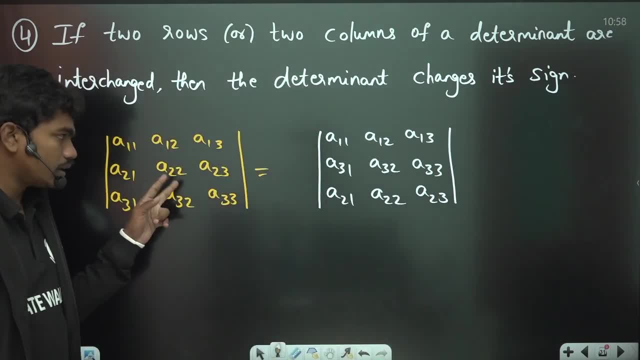 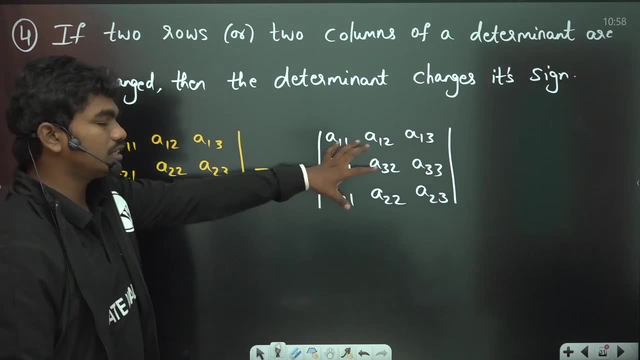 the difference between these two determinants is nothing, but we have swapped second and third rows, so in such cases the result changes with a minus sign, actually. okay, so this determinant value will be same as negative of this determinant value, clear. so when you interchange two rows or two, 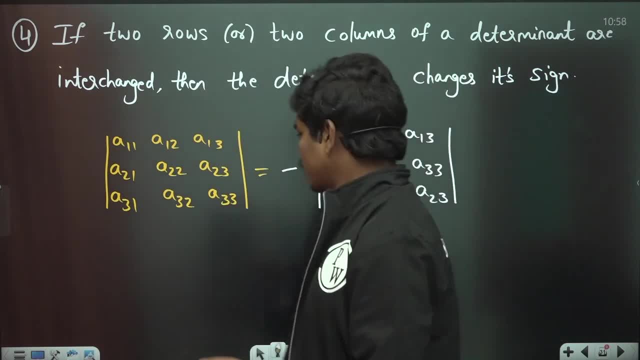 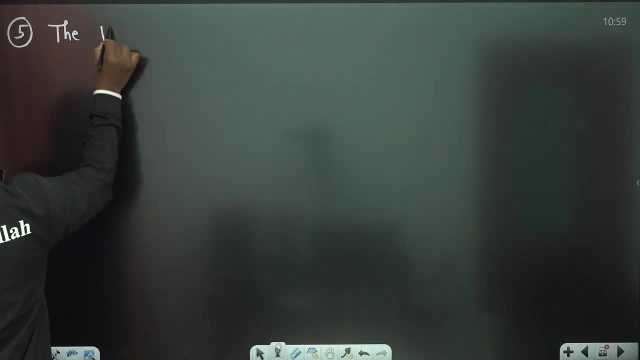 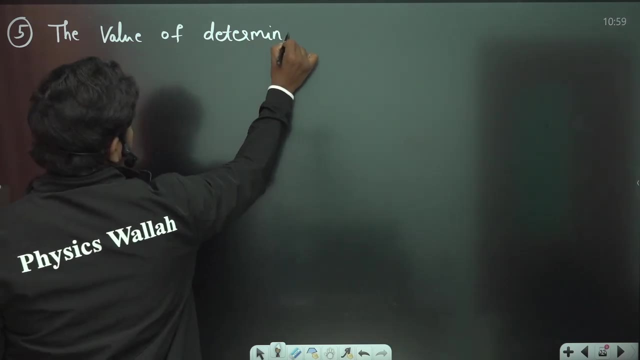 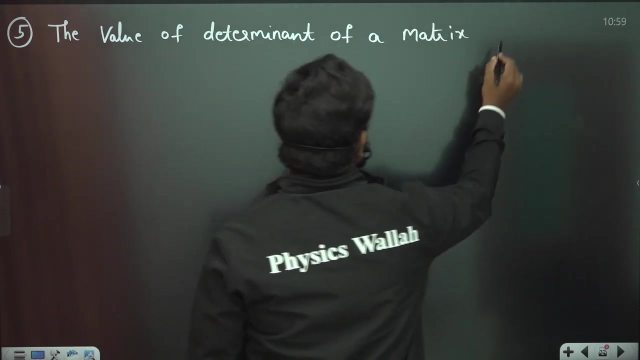 columns, the determinant changes its sign. this is again one very, you know, important property here. now, coming to the fifth you: the value of a determinant of a matrix. the value of determinant of a matrix. the value of determinant of a matrix, uh, you know, basically the value of determinant of a. 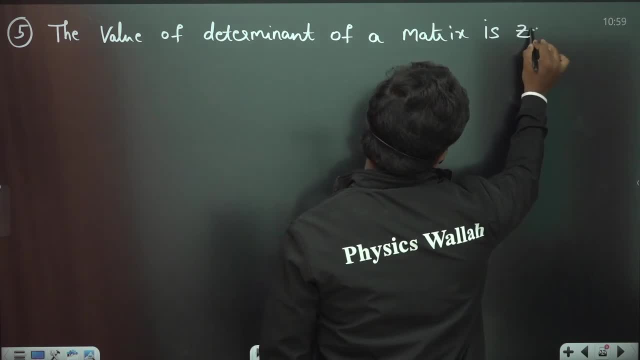 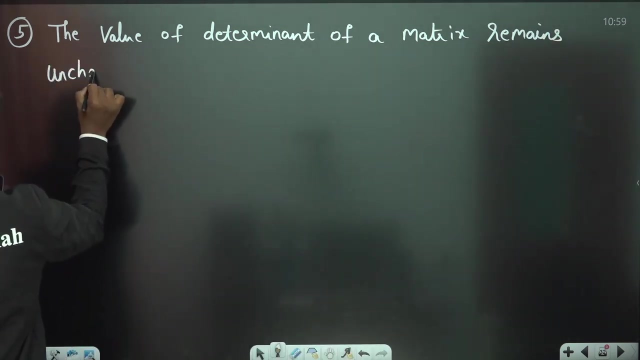 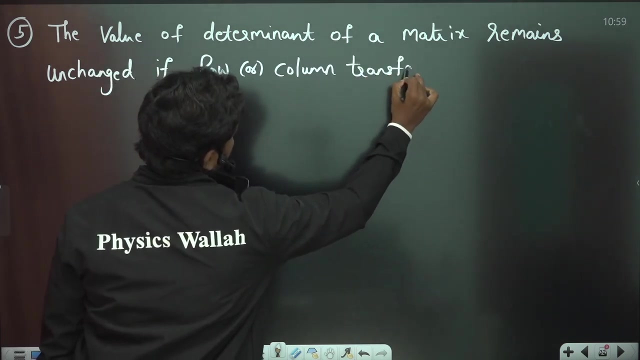 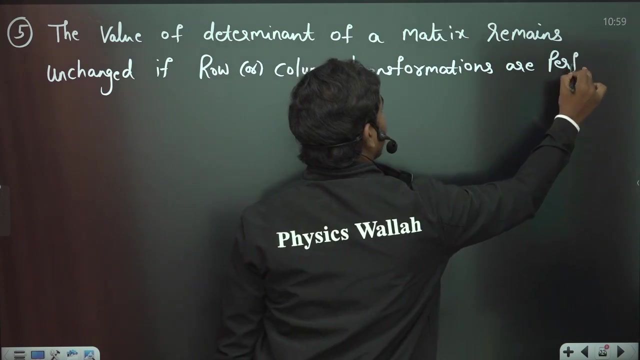 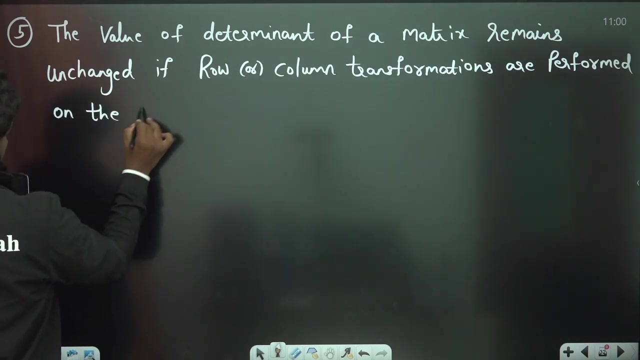 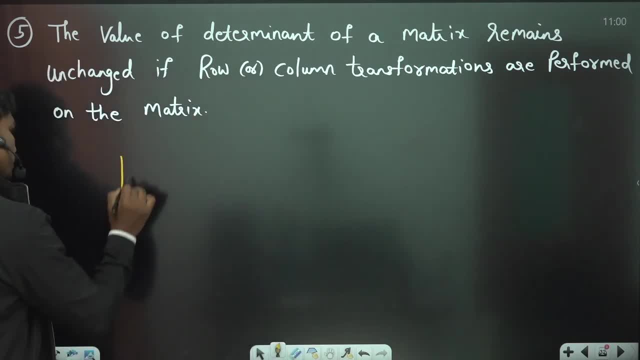 i have this matrix or this determinant, for example. look, let us suppose, if i take this determinant a 1, 1, a 1, 2, a 1, 3, a 2, 1 a 2, 2, a 2, 3, a 3, 1 a 3, 2 and a 3, 3, so this determinant- 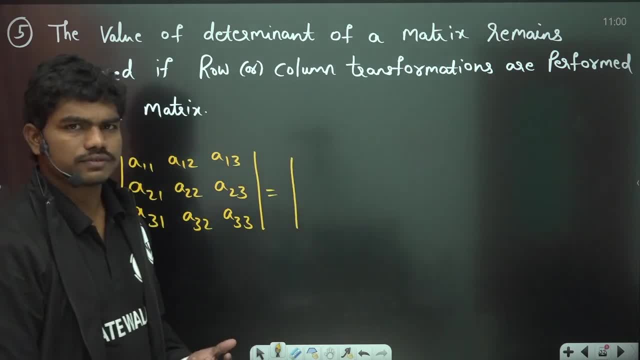 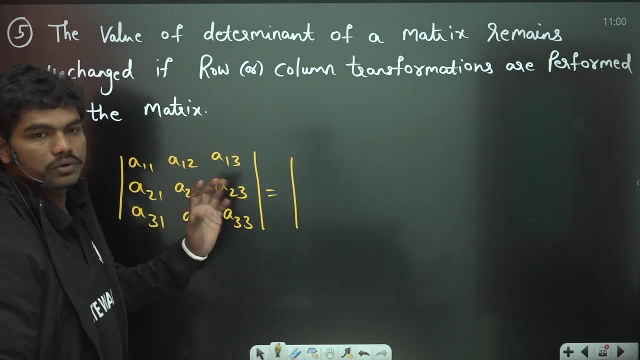 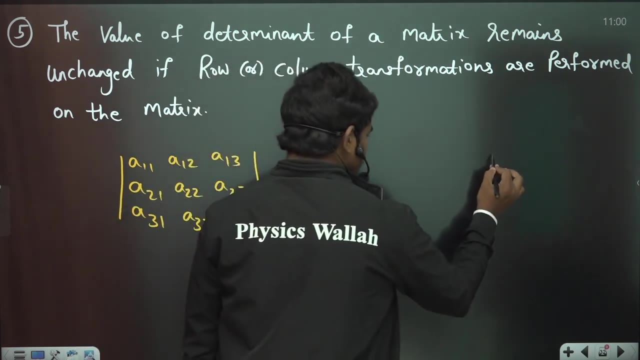 value will be same as. let us suppose if you perform some row transformations- for example, you have subtracted second row from first and added the third row- let us suppose if you do any transformations, this determinant value doesn't change. okay, so, for example, example what i'm doing. for example what i'm doing here, example: transformation, what i'm doing. 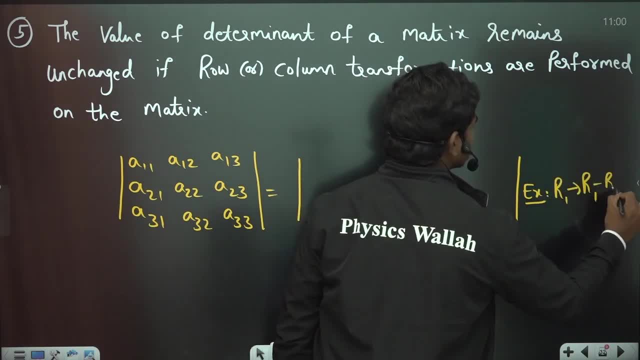 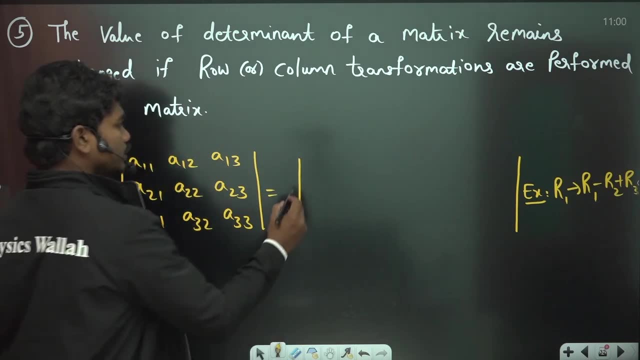 is r 1 changes to r 1 minus r 2 plus r 3. let us say, for example: okay, so we have done some row transformation, so this first row changes as first row minus second plus third. okay, so which means first element is here is going to be a 1 1 minus a 1 2. 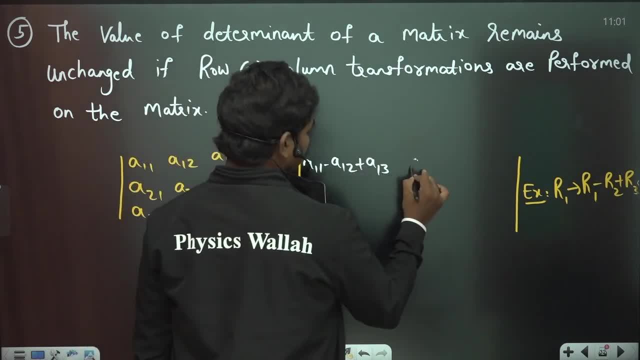 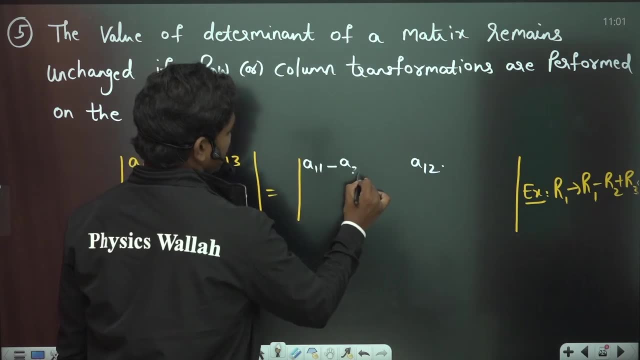 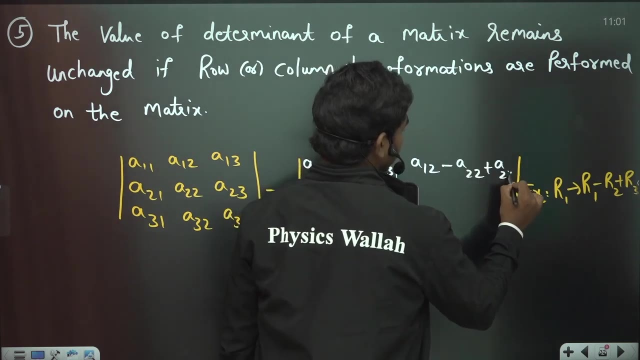 plus a 1: 3. next, this element is going to be a 1: 2. sorry, i think here we have done some error. so a 1: 1 minus a 2, 1 plus a 3: 1. okay. similarly here: a 1, 2 minus a 2, 2 plus a 2, 3 plus a 2- 3. okay, and next? 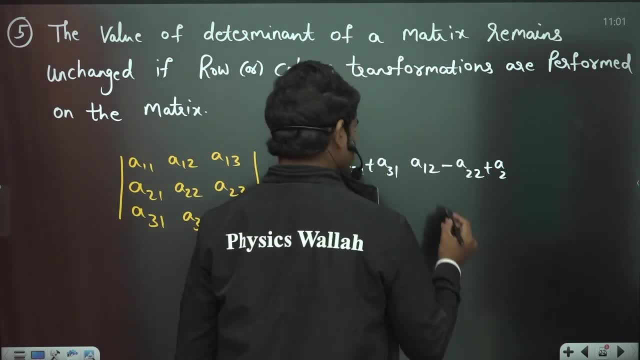 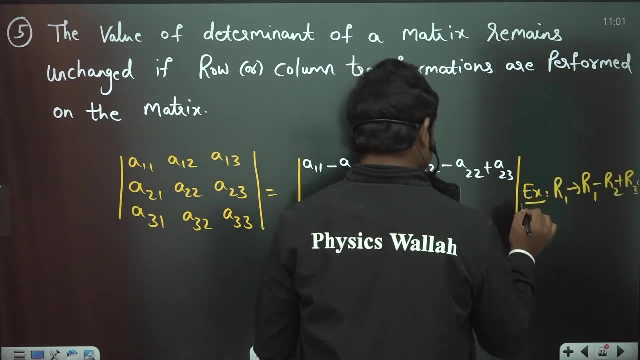 anyhow, i'm writing this on the other side. so a 2, 3 or a, you know, basically this is 3, 2, so this is a just a minute, yeah. so now let us continue, plus a 3, 2 and third, third element, first or third column. 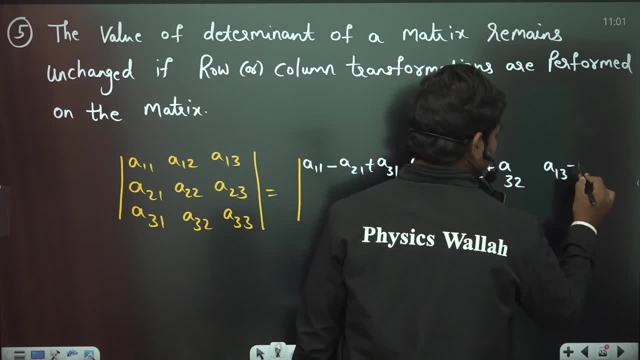 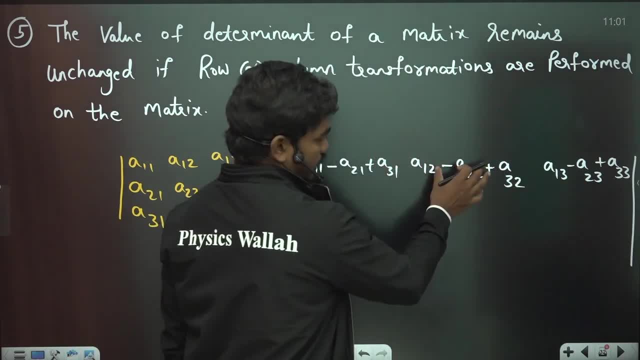 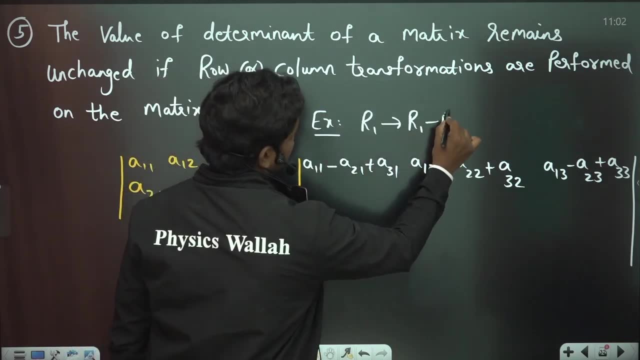 element here. okay, so this is the first or first column element, first or second column and first or third column, and the transformation we have applied here is r1 changes to r1 minus r2 plus r3. so this is the transformation we have applied, so we are not applying any transformations on. 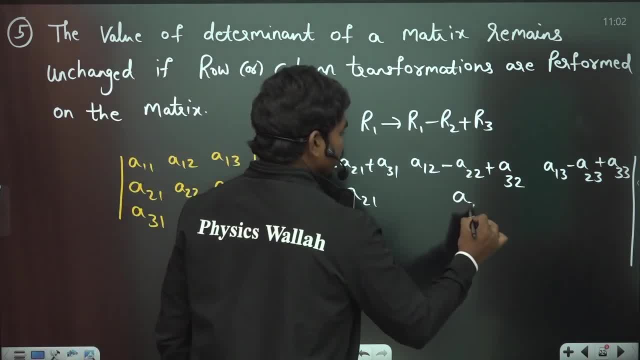 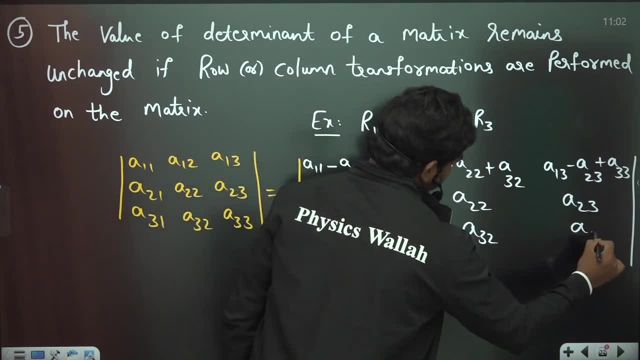 second and third rows, so they remain as it is: a 2, 1 a 2, 2 a 2 3, a 3 1 a 3, 2 and a 3: 3. so this is how we get this determinant and if you see, both the and a 3: 3. so this is how we get this determinant, and if you see both the this determinant and if you see both, the determinant values will remain the same. determinant values will remain the same. determinant values will remain the same. not only this, even if you apply some more. 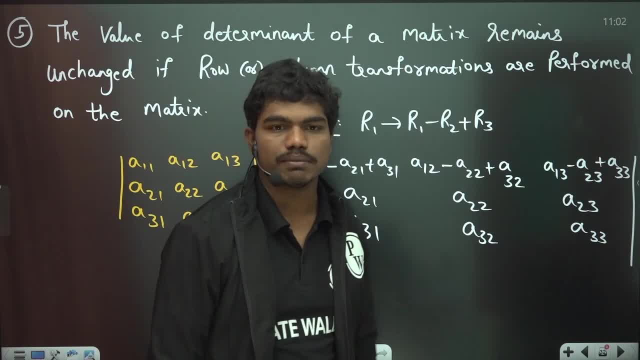 not only this, even if you apply some more. not only this, even if you apply some more. transformation c2 changes to c2 plus c3. transformation c2: changes to c2 plus c3. transformation c2 changes to c2 plus c3. you can apply any number of. 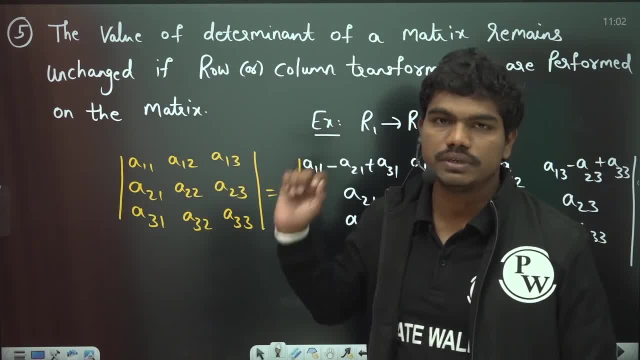 you can apply any number of, you can apply any number of transformations. so these row transformations, transformations, so these row transformations, transformations. so these row transformations or column transformations cannot impact or column transformations cannot impact or column transformations cannot impact the value of the determinant. okay and i. the value of the determinant: okay and i. 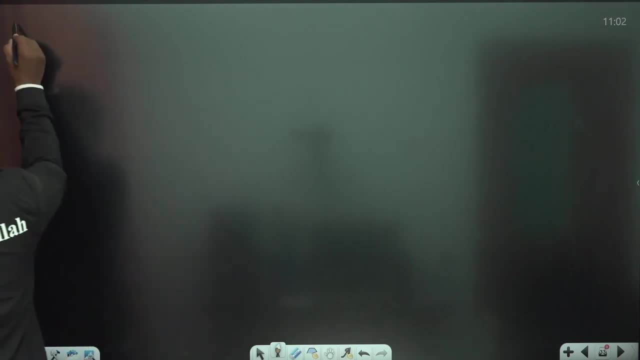 the value of the determinant. okay, and i would like to give one more point again. would like to give one more point again. would like to give one more point again: six, six, six if two rows or two columns, if two rows, or if two rows, or if two rows or two columns. 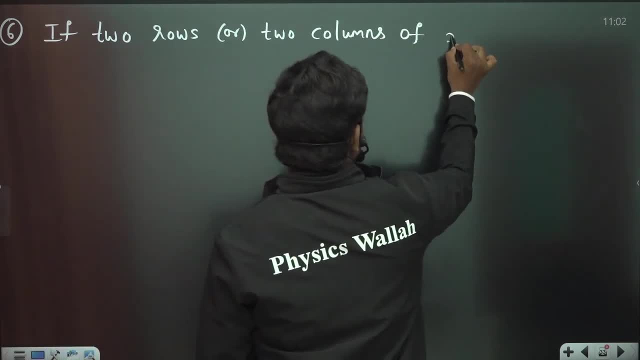 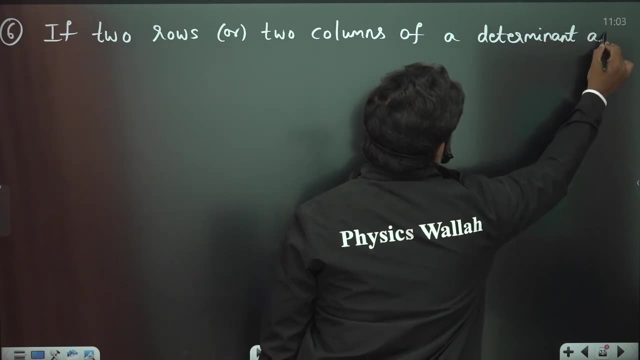 two columns, two columns, or two columns of, or two columns of, or two columns of a matrix of a determinant, or you can say a matrix of a determinant, or you can say a matrix of a determinant, or you can say of a determinant of a determinant, are equal. 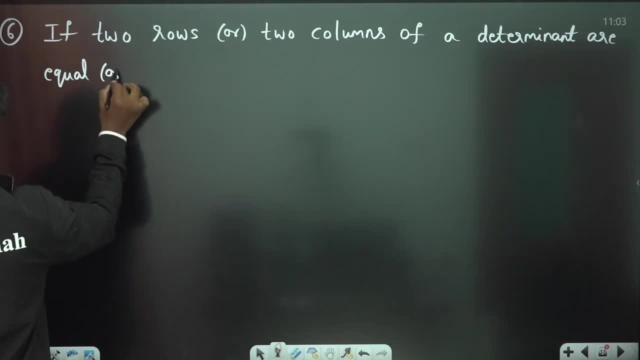 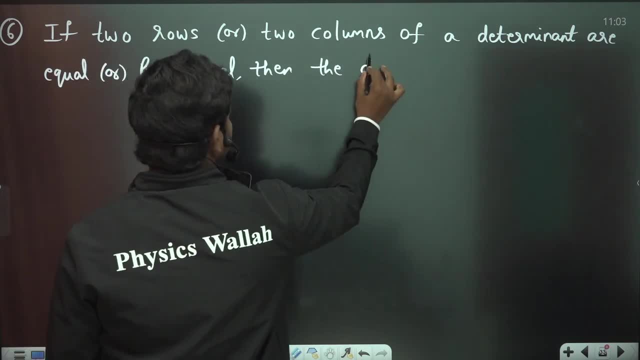 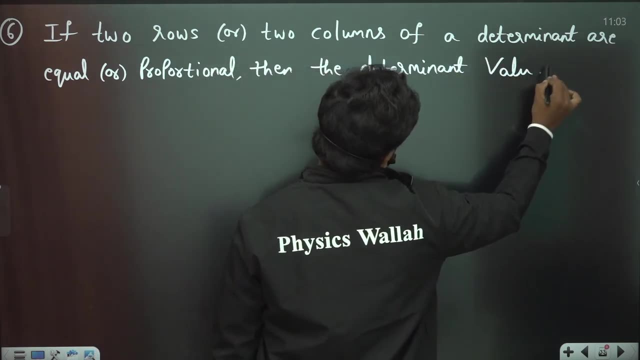 or proportional. or proportional, then the determinant value is zero, then the determinant value is: then the determinant value is, then the determinant value is zero. okay, so then the determinant value is zero. okay, so then the determinant value is zero. okay, so then the determinant value is zero means, let us suppose, if you have 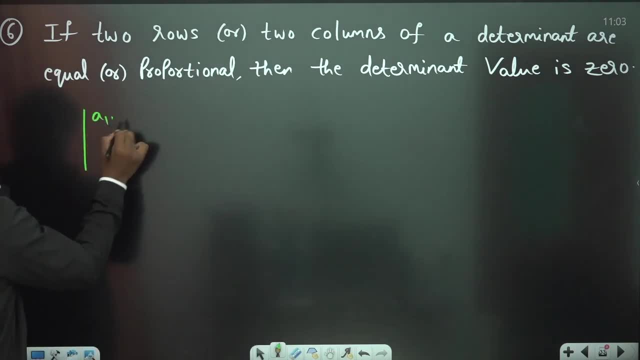 zero means. let us suppose if you have zero means. let us suppose, if you have something like this, something like this, something like this: a11, a12, a13, a11, a12, a13, a11, a12, a13, a21, a22, a23, a21, a22, a23. 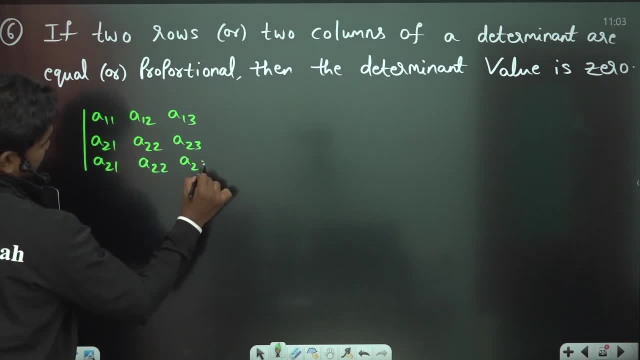 a21, a22, a23, a23, a21, a22, a23, a23, for example, then in such case, if you try, for example, then in such case, if you try, for example, then in such case, if you try to calculate the determinant value, you to calculate the determinant value, you, 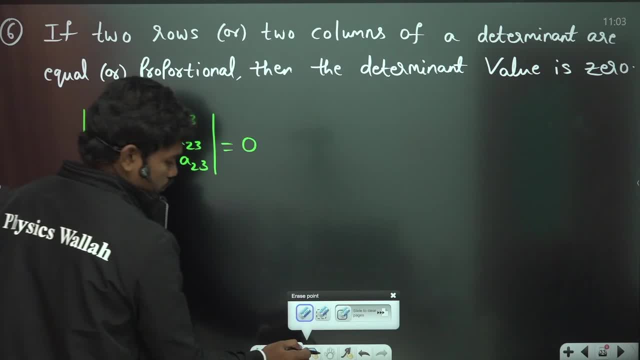 to calculate the determinant value, you will definitely end up with a zero sign, will definitely end up with a zero sign. will definitely end up with a zero sign. the reason being these two, the reason being these two, the reason being these two: these two rows are identical actually, here. 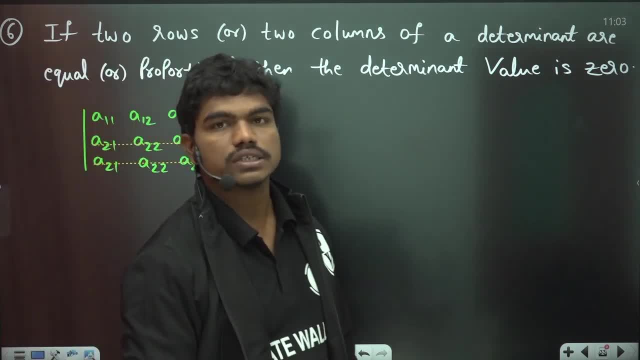 these two rows are identical, actually here. these two rows are identical, actually here, correct. similarly, if two columns are correct, similarly, if two columns are correct, similarly, if two columns are identical also, then also your determinant. identical also, then also your determinant identical also, then also your determinant is here, or sometimes what happened they. 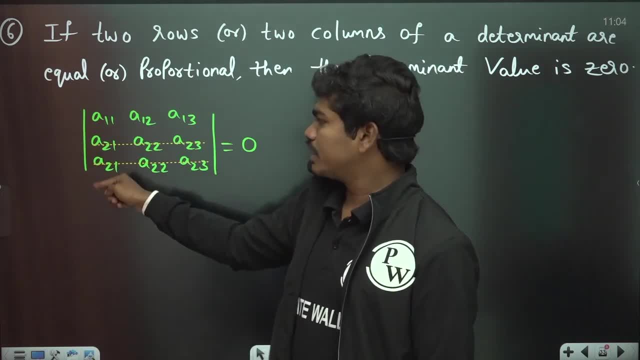 is here, or sometimes what happened. they is here, or sometimes what happened. they can be proportional means. let us suppose can be proportional means. let us suppose can be proportional means. let us suppose here i have some constant k1 into a21 k2. here i have some constant k1 into a21 k2. 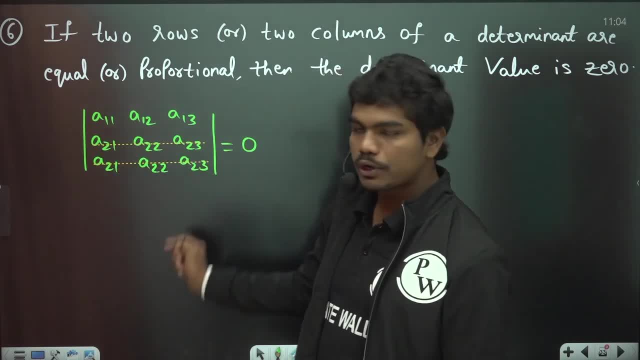 here i have some constant k1 into a21, k2 into a22 or k1 into a21, k1 into a22, k1 into a22, or k1 into a22, k1 into a22, k1 into a22 or k1 into a22, k1 into a22, k1 into a23. in such cases, what you will do, into a23. in such cases, what you will do, into a23. in such cases, what you will do: you will take out the k1 constant and you will take out the k1 constant and you will take out the k1 constant and again, these two rows will become: 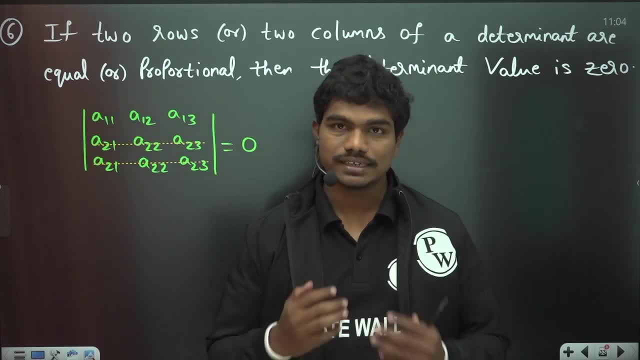 again. these two rows will become again. these two rows will become same. okay, so that's how. if two rows or two same, okay, so that's how. if two rows or two same, okay, so that's how. if two rows or two columns of a matrix are either equal, 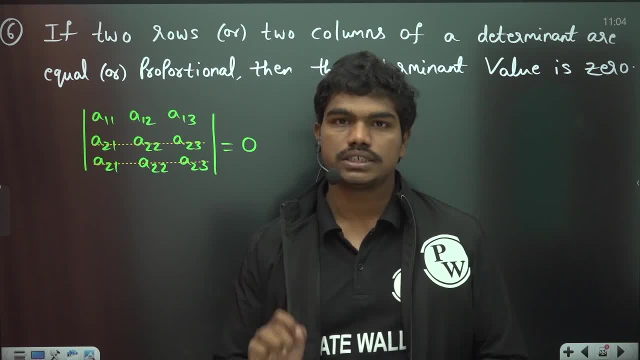 columns of a matrix are either equal. columns of a matrix are either equal or proportional, then definitely their. or proportional, then definitely their. or proportional, then definitely their determinant value is going to be determinant value is going to be determinant value is going to be zero. okay. so this is again one of the very 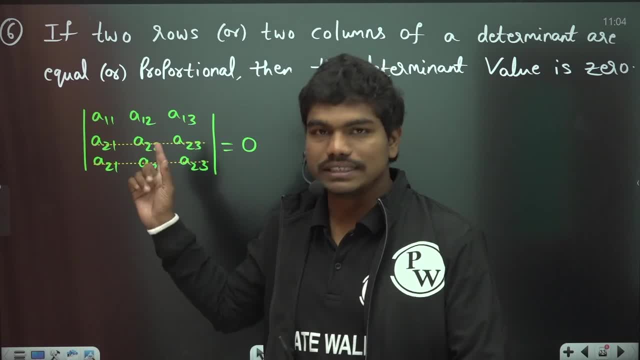 zero. okay, so this is again one of the very zero okay, so this is again one of the very nice properties, because many times nice properties, because many times nice properties, because many times we try to, we try to, we try to bring determinants in such form so that 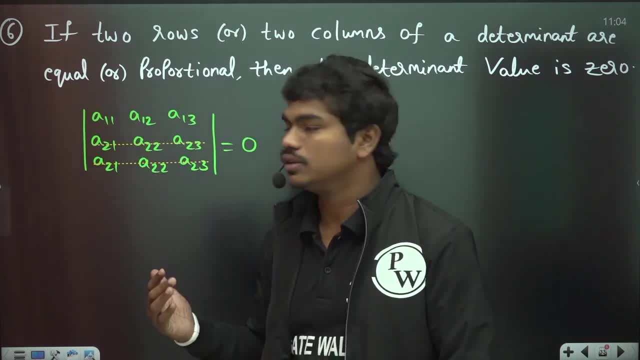 bring determinants in such form so that. bring determinants in such form so that, to make them, uh, you know, to show that, to make them, uh, you know, to show that, to make them, uh, you know, to show that the value of the determinant is zero, okay. 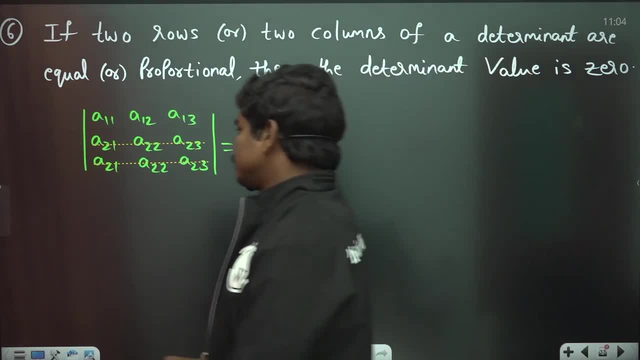 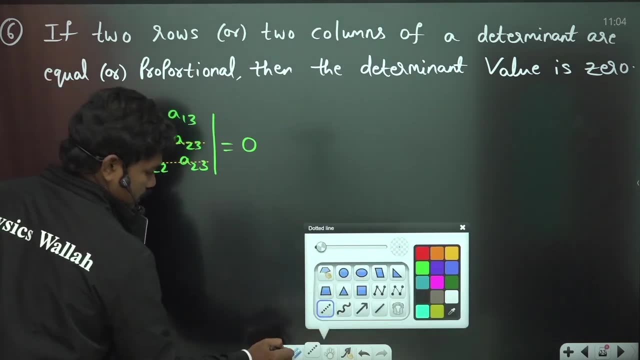 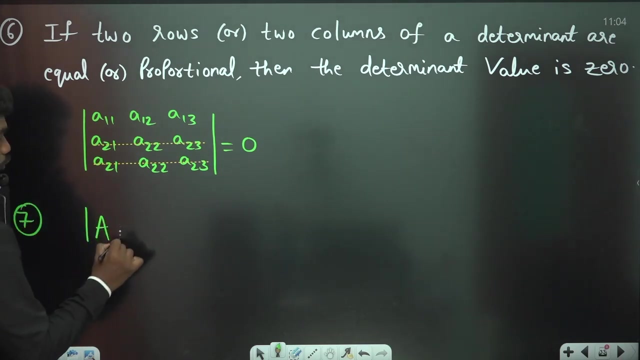 the value of the determinant is zero. okay, the value of the determinant is zero, okay. determinant of a into b. determinant of a into b. determinant of a into b is basically equal to product of the is basically equal to product of the is basically equal to product of the individual determinants. 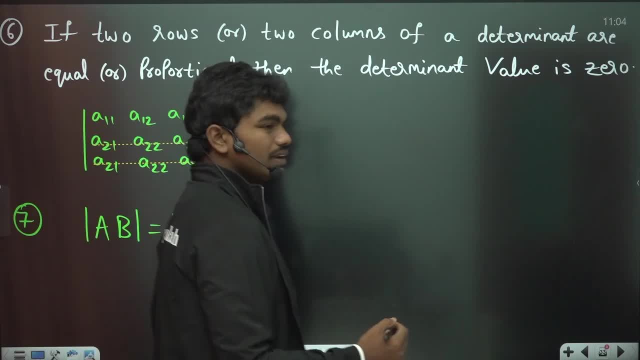 individual determinants. individual determinants: that a into that b. okay, now i'd like that a into that b. okay, now i'd like that a into that b. okay, now i'd like to give. we have talked about a lot of to give. we have talked about a lot of. 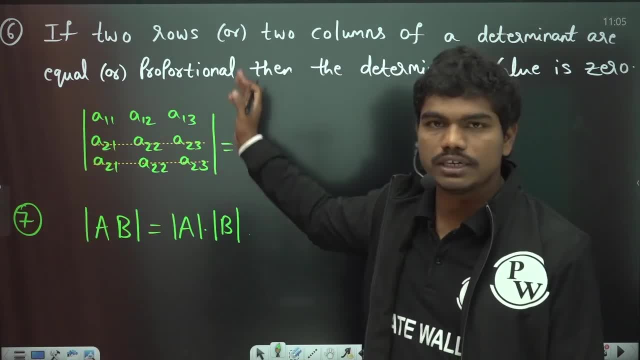 to give. we have talked about a lot of special type of matrices, orthogonal special type of matrices. orthogonal special type of matrices. orthogonal matrix. you know we have talked about matrix. you know we have talked about matrix. you know we have talked about determinants of lower triangular upper. 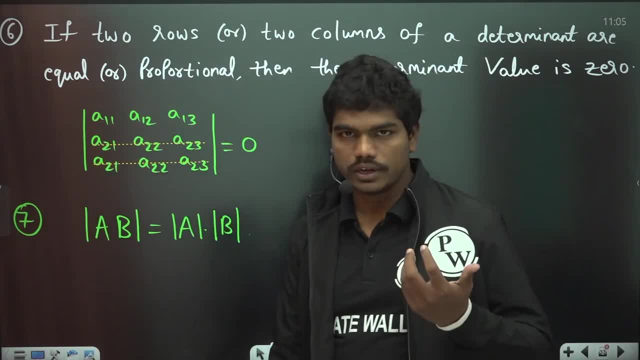 determinants of lower triangular upper determinants of lower triangular upper triangular diagonal matrix. so now, let us triangular diagonal matrix. so now let us triangular diagonal matrix. so now, let us try to talk about this. uh, you know, uh, try to talk about this. uh, you know, uh. 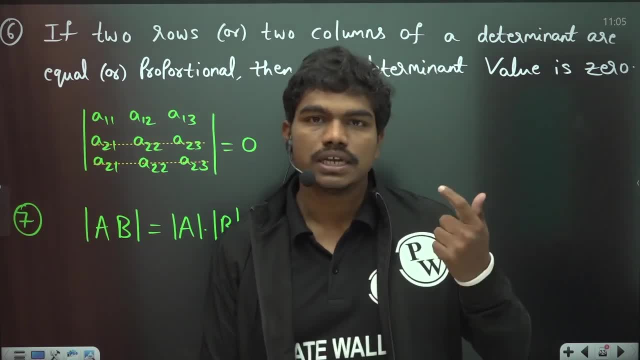 try to talk about this. uh, you know, uh, determinants of this special matrices, determinants of this special matrices, determinants of this special matrices that i told you orthogonal matrix, that i told you orthogonal matrix, that i told you orthogonal matrix, involute idempotent, all these cases. 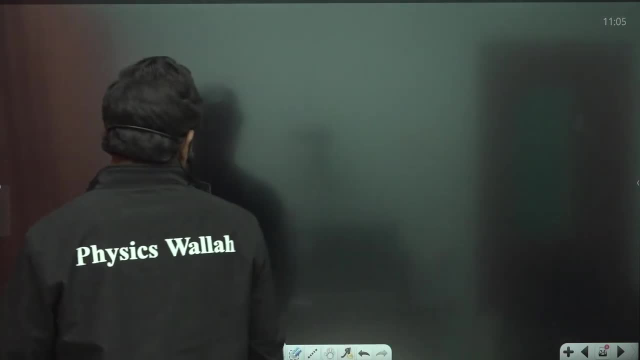 involute, idempotent, all these cases, involute, idempotent, all these cases basically okay. so let us see what are basically okay. so let us see what are basically okay. so let us see what are the cases, the cases, the cases, eight, eight, eight, the determinant of 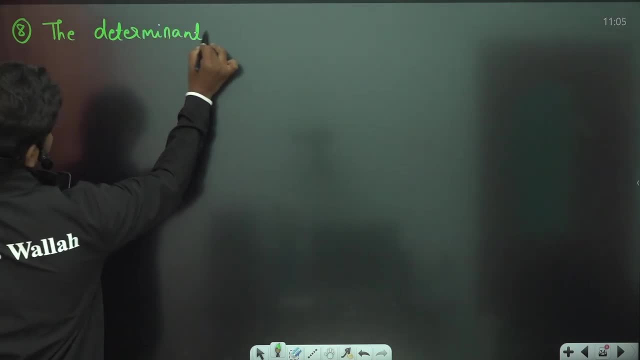 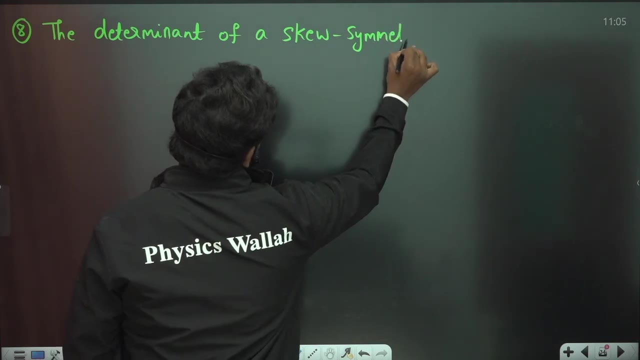 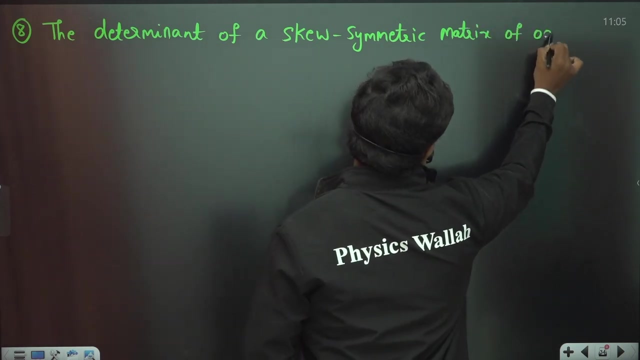 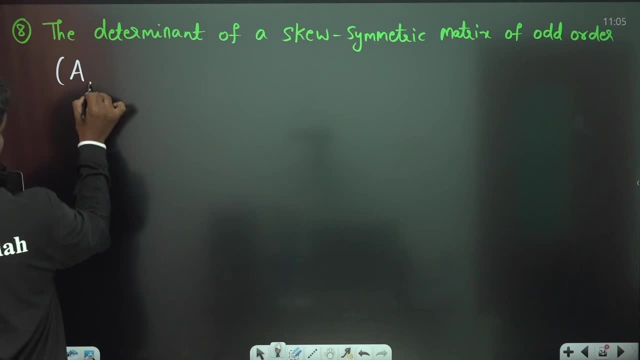 of odd order. what is the meaning of odd order? you know if you have a matrix of order. you know if you have a matrix of order. you know if you have a matrix of this size n by n because it's a skew, this size n by n because it's a skew. 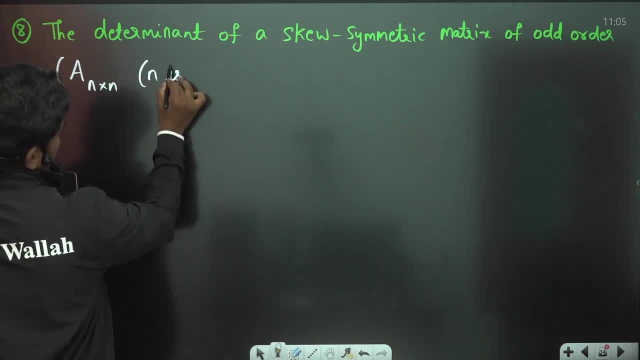 this size n by n, because it's a skew: symmetric, so it has to be square matrix. symmetric, so it has to be square matrix, symmetric, so it has to be square matrix. n is odd, okay, n is odd. basically so this: n is odd, okay, n is odd, basically so this: 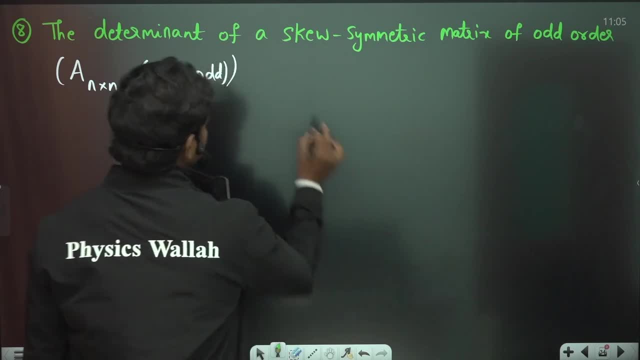 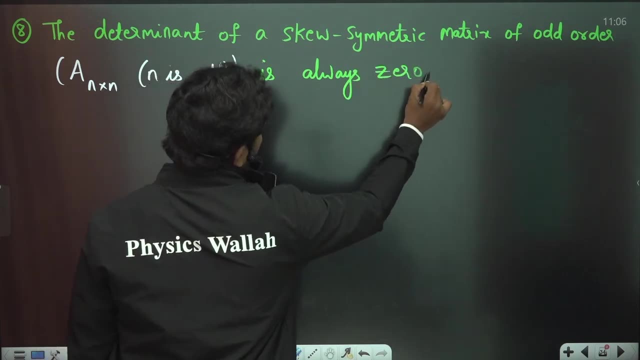 n is odd. okay, n is odd, basically. so this is a skew symmetric matrix of odd order. is a skew symmetric matrix of odd order. is a skew symmetric matrix of odd order. is always zero, is always zero, is always zero, is, is always zero, always, always, always zero. how this property is one, really very. 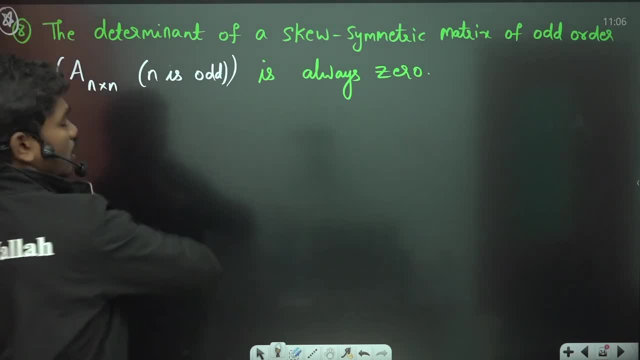 zero. how this property is one really very zero. how this property is one really very important property, important property, important property. that determinant of a skew symmetric, that determinant of a skew symmetric, that determinant of a skew symmetric matrix of odd order is also zero. matrix of odd order is also zero. 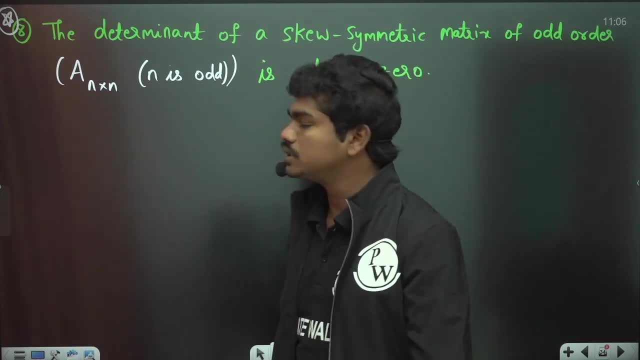 matrix of odd order is also zero, essentially in je advanced also. you have essentially in je advanced also. you have essentially in je advanced also. you have a question on this basically in this year. a question on this basically in this year, a question on this basically in this year. so, anyhow, let us see how this is. 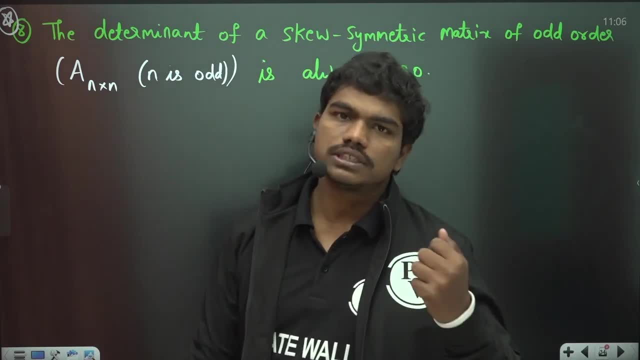 so anyhow, let us see how this is so anyhow, let us see how this is happening. means if you take any skew. happening means if you take any skew. happening means if you take any skew. symmetric matrix of odd order. third. symmetric matrix of odd order: third. symmetric matrix of odd order, third order. fifth order. seventh order, ninth: any. 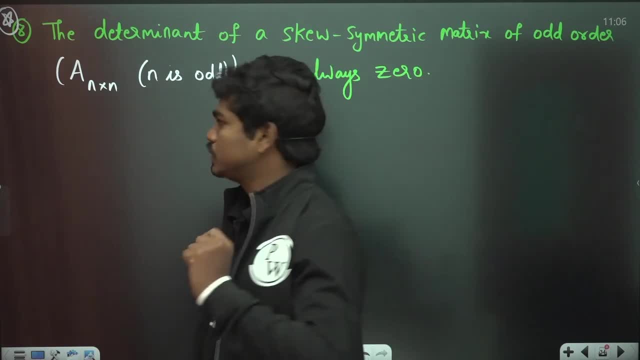 order. fifth order. seventh order. ninth: any order. fifth order. seventh order. ninth: any any order so that value is always equal. any any order so that value is always equal. any any order so that value is always equal to zero. how come see here, so i would to zero. how come see here, so i would. 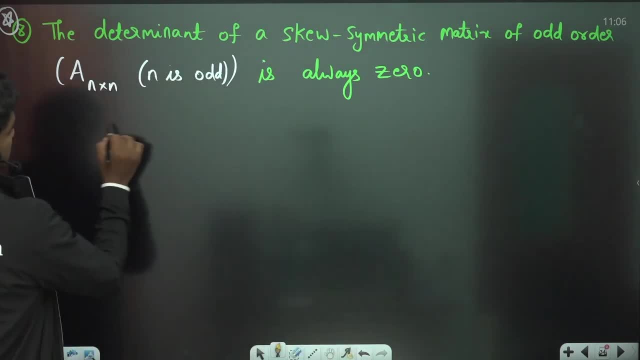 to zero. how come see here? so i would like to give you this analysis here, like to give you this analysis here, like to give you this analysis here. you can see a is skew symmetric, correct. you can see a is skew symmetric, correct. you can see a is skew symmetric, correct. so here this a is a skew. 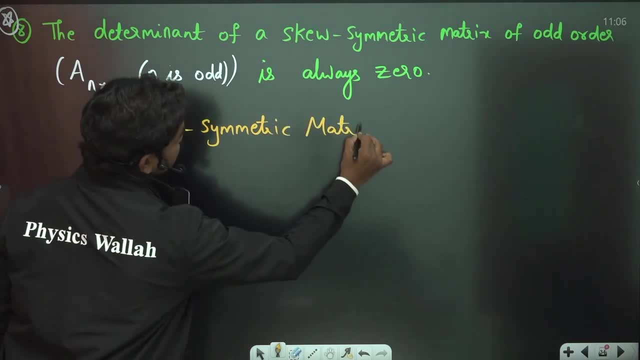 symmetric, symmetric, symmetric matrix. so a is a skew symmetric matrix. so a is a skew symmetric matrix. so a is a skew symmetric matrix here, correct? so if a is skew symmetric matrix here, correct? so if a is skew symmetric matrix, then a is equal to minus matrix, then a is equal to minus. 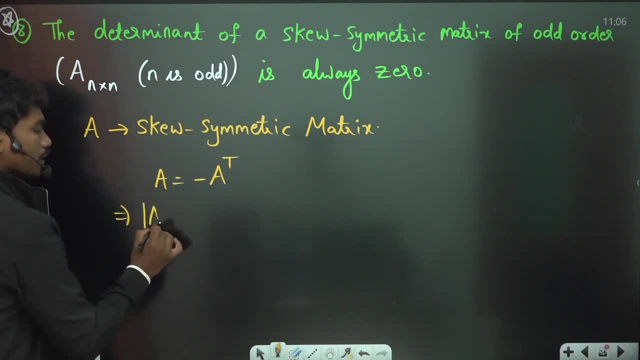 matrix, then a is equal to minus a transpose which you know now. if you a transpose which you know now, if you a transpose which you know now, if you apply determinant on both matrices, apply determinant on both matrices. apply determinant on both matrices because both these matrices are same. 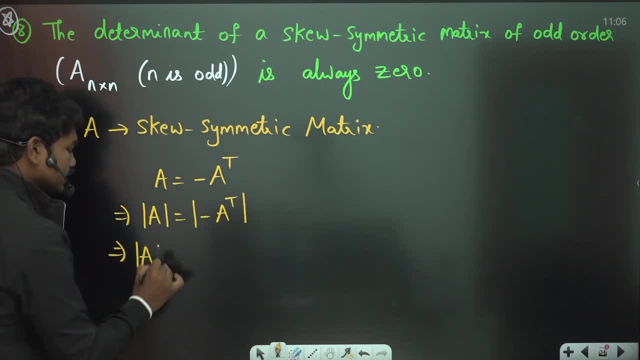 because both these matrices are same. because both these matrices are same, minus a transpose. so this implies minus a transpose. so this implies minus a transpose. so this implies that a is equal to look to this a, that a is equal to look to this a, that a is equal to look to this a transpose. can i take this minus one as? 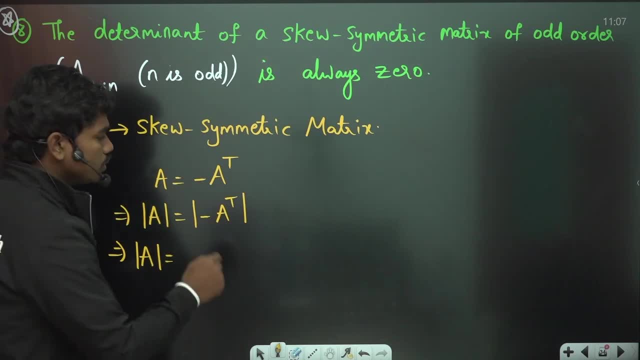 transpose. can i take this minus one as transpose? can i take this minus one as some scalar multiplication, because k value some scalar multiplication because k value some scalar multiplication, because k value can be minus one also. so if you take can be minus one also. so if you take, 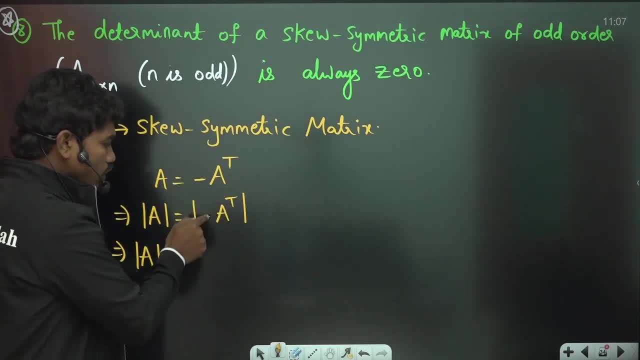 can be minus one also. so if you take this minus one as multiplication to this a, this minus one as multiplication to this a, this minus one as multiplication to this a transpose, so if i want to take this transpose, so if i want to take this transpose, so if i want to take this minus one out of this determinant, i know. 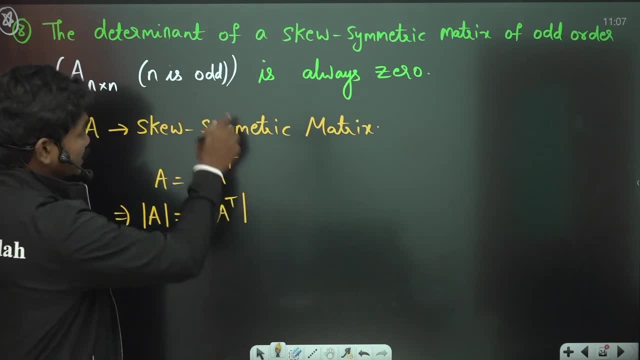 minus one out of this determinant. i know minus one out of this determinant. i know i need to take out this k. i need to take out this k. i need to take out this k as k power n times, so let us suppose if. as k power n times, so let us suppose if. 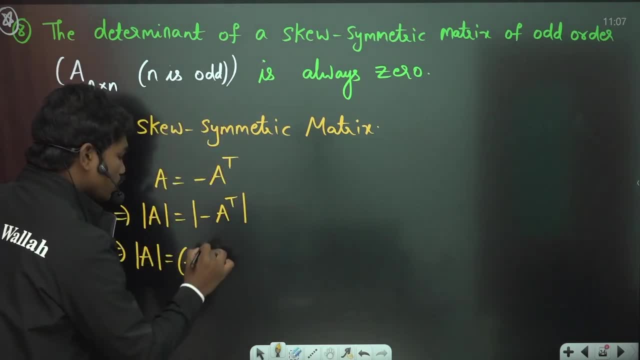 as k power n times. so let us suppose: if the matrix order is of n by n, the matrix order is of n by n. the matrix order is of n by n. i can write this as minus one whole power. i can write this as minus one whole power. 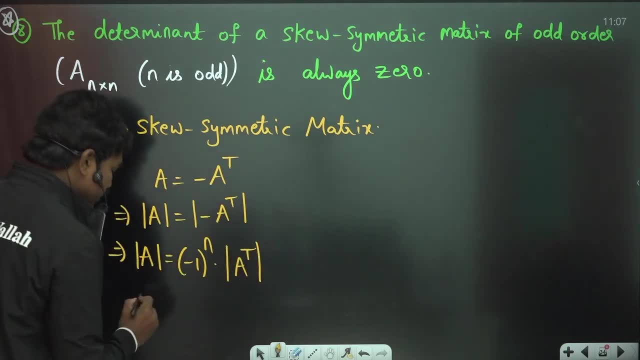 i can write this as minus one whole power n into that of a. transpose, so from n into that of a. transpose, so from n into that of a. transpose, so from this equation. what can we write that a, this equation. what can we write that a, this equation. what can we write? that a is equal to minus one whole power n. 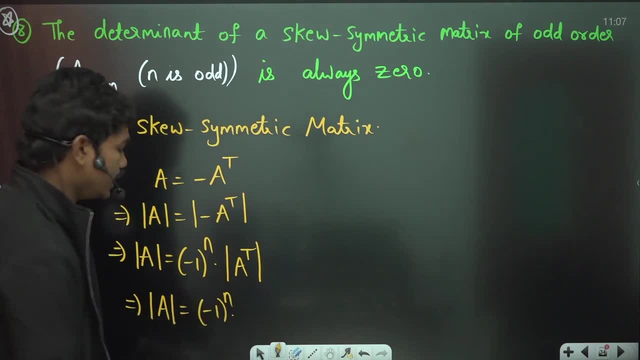 is equal to minus one whole power. n is equal to minus one whole power n into. you know this property determinant into. you know this property determinant into. you know this property determinant of a transpose is same as that a of a transpose is same as that a of a transpose is same as that a. so this is again equal to that a. so 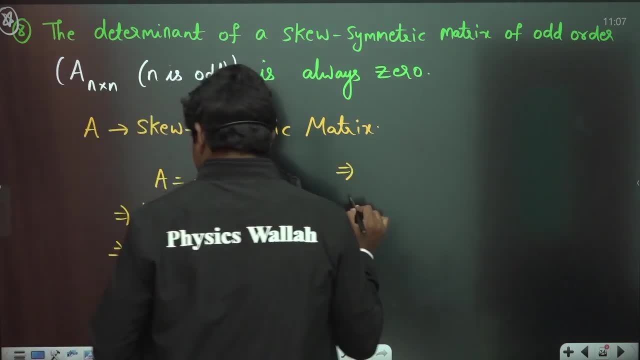 so this is again equal to that a. so. so this is again equal to that a. so, from these two equations, you can, from these two equations, you can, from these two equations, you can understand one thing. understand one thing, understand one thing: this implies that a minus. this implies that a minus. 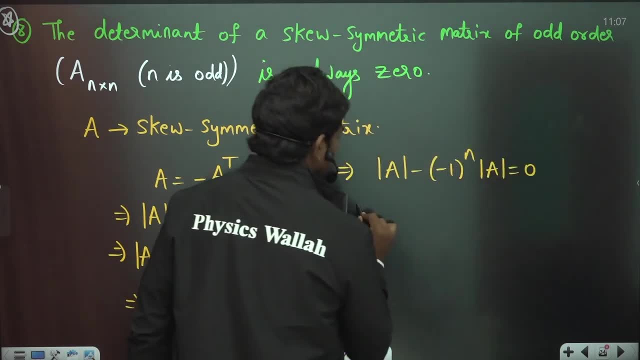 this implies that a minus one whole power n times of that a is one whole power n times of that a is one whole power n times of that a is equal to zero. and this, if you take that, equal to zero, and this, if you take that equal to zero, and this, if you take that a common, you have one minus minus one. 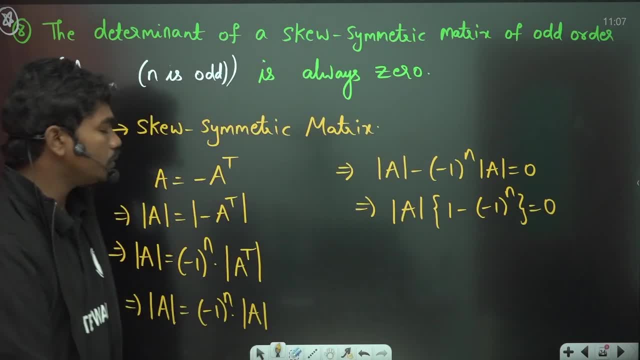 a common: you have one minus minus one. a common: you have one minus minus one. whole power. n is equal to zero. this is whole power. n is equal to zero. this is whole power. n is equal to zero. this is the equation that you attend with, but the equation that you attend with, but. 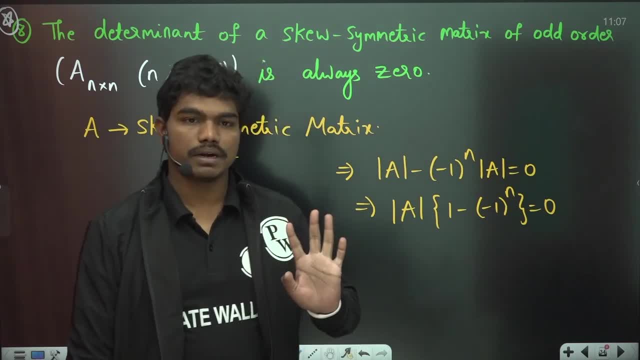 the equation that you attend with. but now try to observe one thing. let us now try to observe one thing. let us now try to observe one thing. let us suppose if n is even, for example, okay. suppose if n is even for example, okay. suppose if n is even, for example, okay, if n is even, then what happens? this minus. 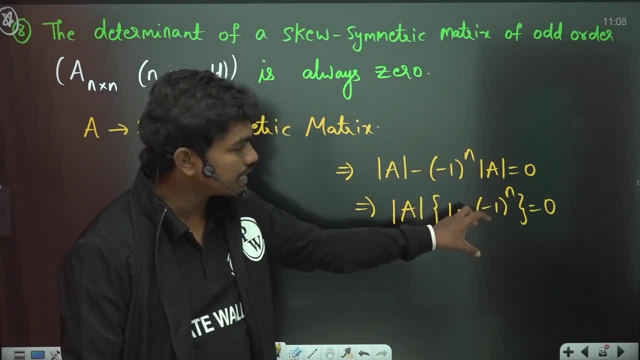 if n is even, then what happens this minus? if n is even, then what happens this minus one whole power? n gives you an even one whole power. n gives you an even one whole power. n gives you an even number, correct? so if n is an even number, 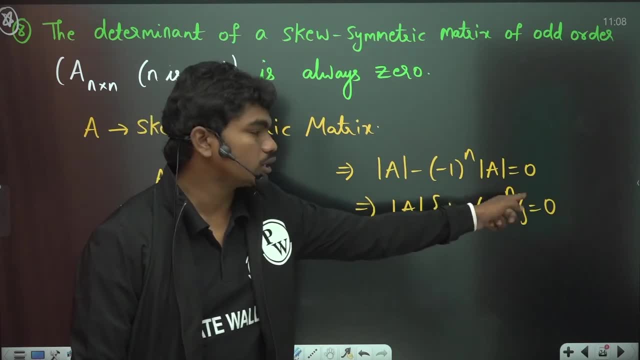 number correct. so if n is an even number number correct. so if n is an even number minus one, whole power n gives you plus one, minus one. whole power n gives you plus one, minus one. whole power n gives you plus one, and one minus one is always zero. and 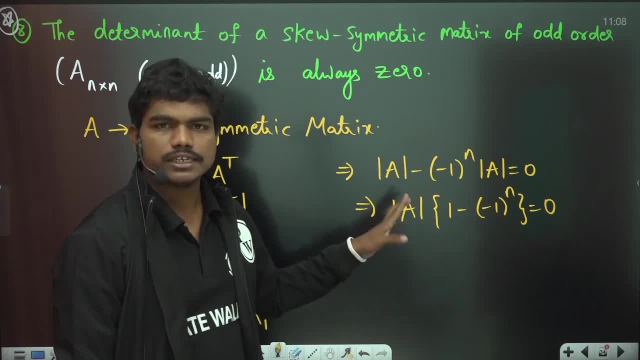 and one minus one is always zero, and and one minus one is always zero, and this equation gets satisfied, irrespective this equation gets satisfied, irrespective this equation gets satisfied, irrespective of this data being zero or not correct, of this data being zero or not correct, of this data being zero or not correct. i'm repeating: if this n value is even 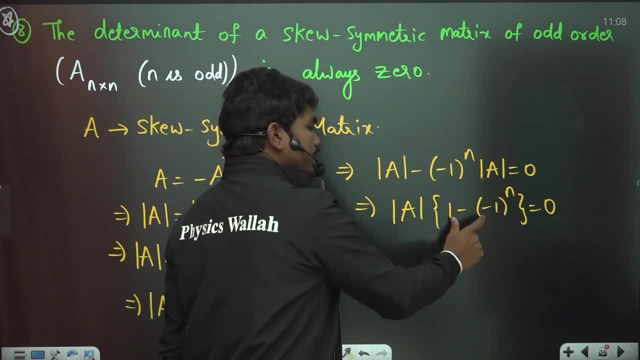 i'm repeating: if this n value is even, i'm repeating, if this n value is even, then this minus one whole power n will then this minus one whole power n will, then this minus one whole power n will become one and this one minus one product become one, and this one minus one product. 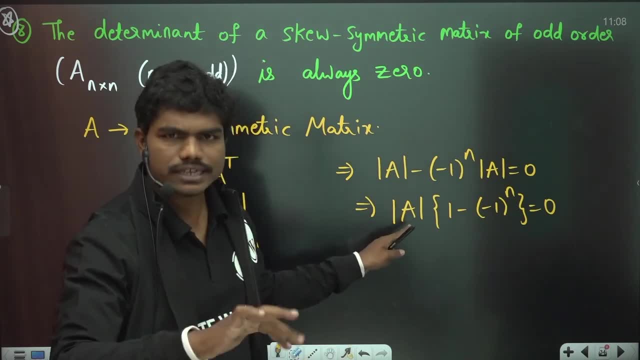 become one, and this one minus one product will definitely come out to zero correct will definitely come out to zero correct will definitely come out to zero correct. so even if that is zero or non-zero, so even if that is zero or non-zero, so even if that is zero or non-zero, doesn't matter, 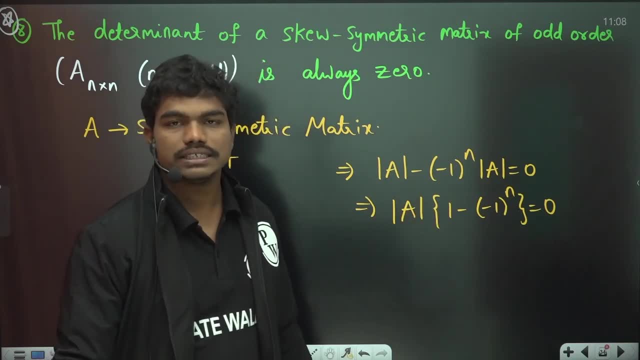 doesn't matter. doesn't matter. this equation always holds good when n. this equation always holds good when n. this equation always holds good when n is even so. that's the reason when n is is even so. that's the reason when n is is even so. that's the reason when n is even. you can't comment anything. 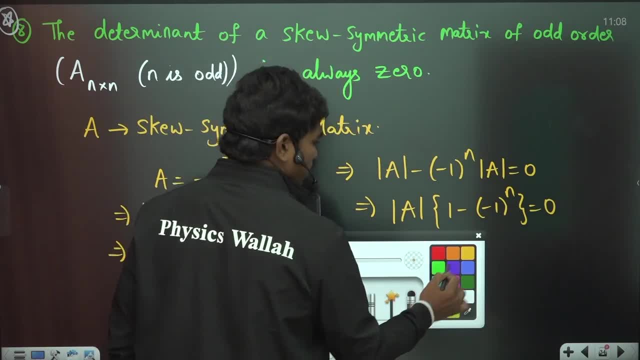 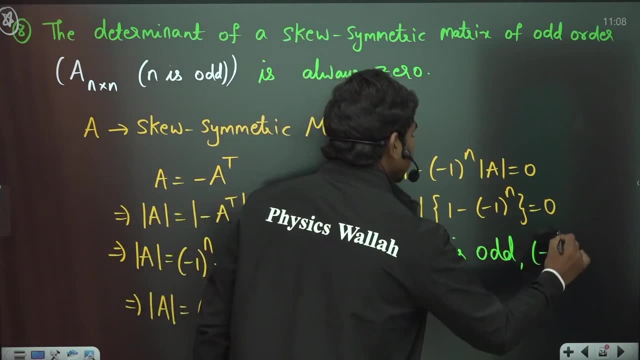 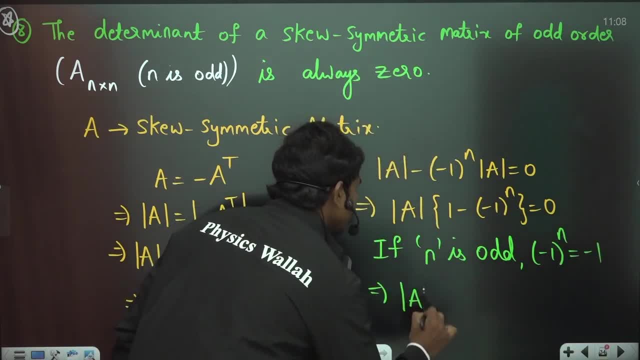 then you know, minus one whole power n is, then you know, minus one whole power n is equal to minus one correct. equal to minus one correct. equal to minus one correct. so this implies that a times of so this implies that a times of so this implies that a times of one minus of minus one, which is equal to. 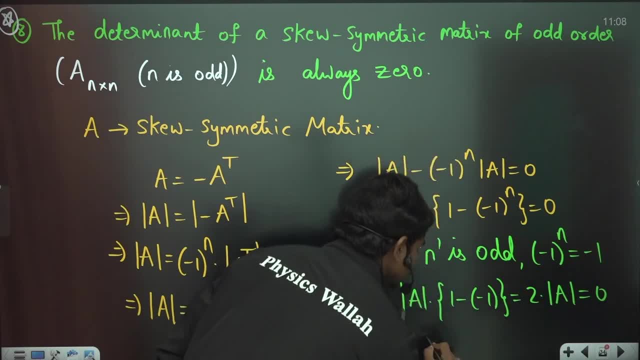 one minus of minus one, which is equal to one minus of minus one, which is equal to two times of that a, is equal to zero, and two times of that a is equal to zero, and two times of that a is equal to zero. and this gives you. 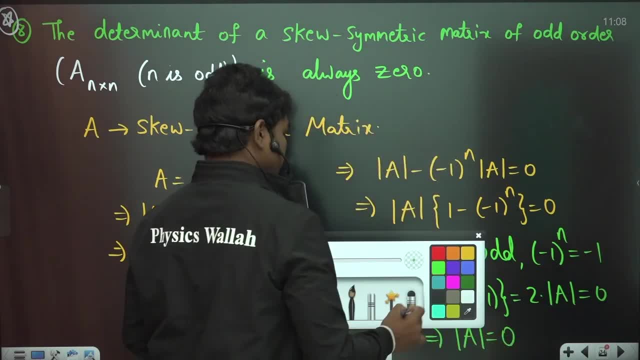 this gives you. this gives you: debt of a is equal to zero. okay, so, this debt of a is equal to zero. okay, so, this debt of a is equal to zero. okay, so this: that a is equal to zero under two. that a is equal to zero under two. 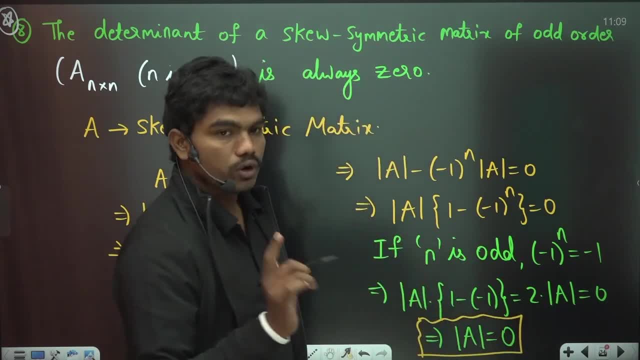 that a is equal to zero under two conditions. first thing conditions. first thing conditions. first thing: a is is cosmetic matrix, and more more a is is cosmetic matrix and more more a is is cosmetic matrix. and more, more importantly, this n is odd number correct. importantly, this n is odd number correct. 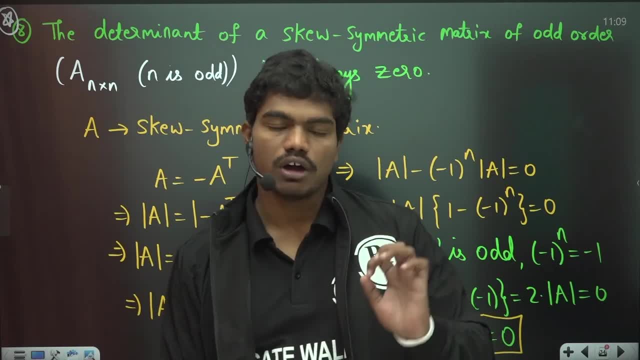 importantly, this n is odd number, correct. so that's why, if you take any, so that's why, if you take any, so that's why, if you take any determinant of skew symmetric matrix of determinant of skew symmetric matrix of determinant of skew symmetric matrix of odd order, definitely the answer turns. 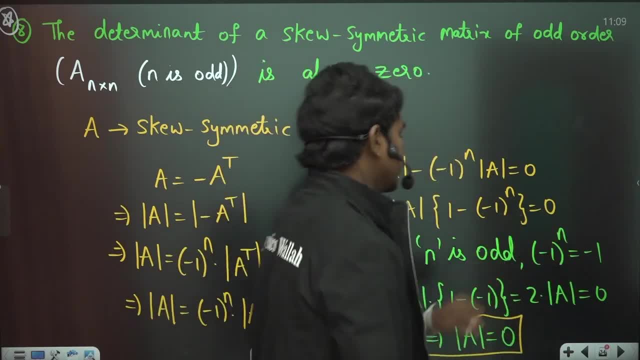 odd order. definitely the answer turns odd order. definitely the answer turns out to be out to be out to be zero clear. so many times they ask you zero clear. so many times they ask you zero clear. so many times they ask you, they give you questions like this in: 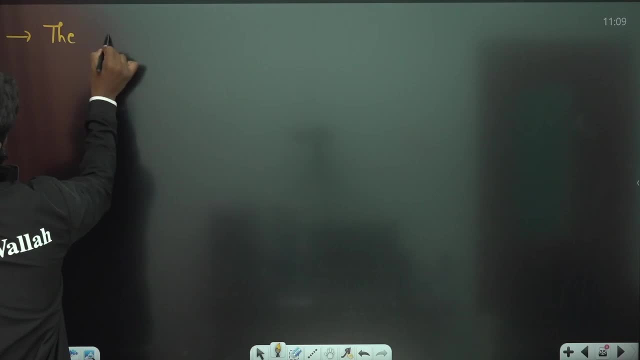 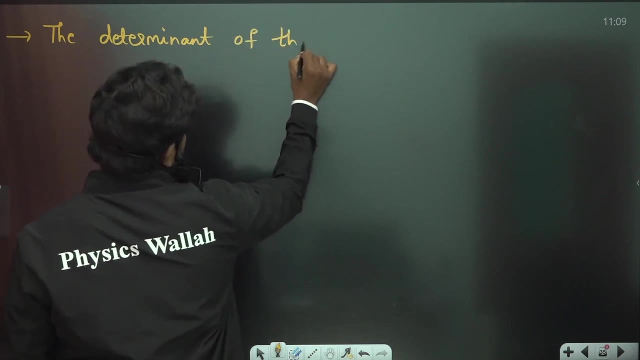 they give you questions like this in. they give you questions like this in exams, exams, exams. the determinant of the value, the. the determinant of the value, the. the determinant of the value. the determinant of the matrix. determinant of the matrix. determinant of the matrix. the determinant of the matrix. 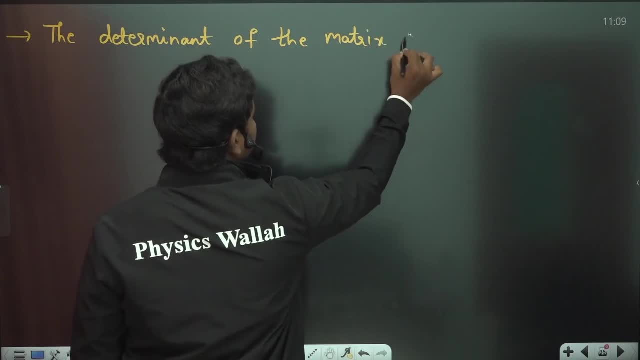 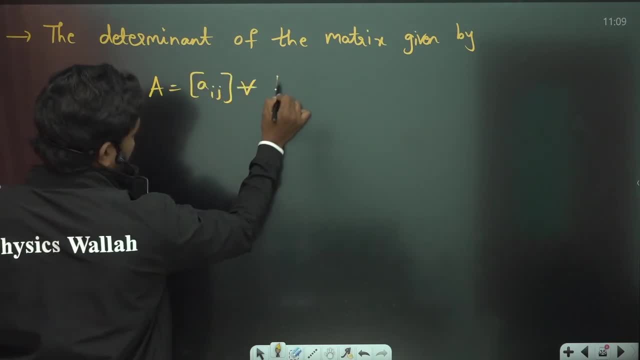 a is equal to. a is equal to a. i, j, a, i, j a. i. j. for all one less than or equal to i comma. for all one less than or equal to i comma. for all one less than or equal to i comma. j less than or equal to five, it's a five. 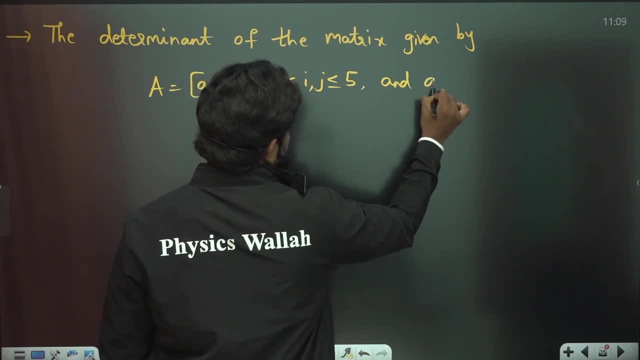 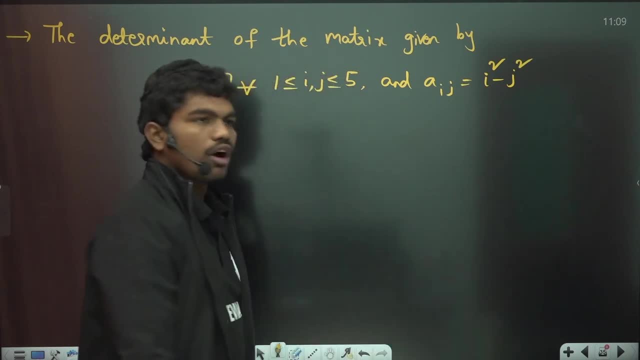 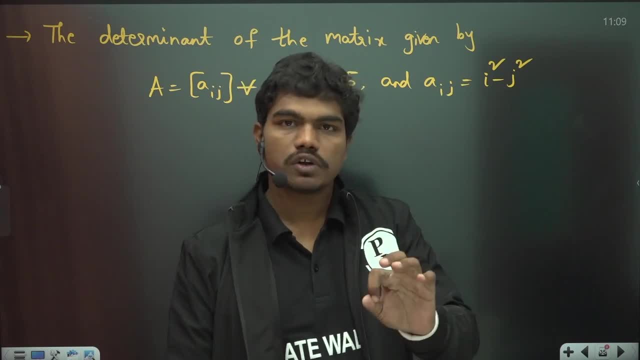 function, i mean it's not very complicated. function, i mean it's not very complicated, but again slightly complicated, so i. but again slightly complicated, so i, but again slightly complicated. so i square minus j, square means, if you want, but again slightly complicated. so i square minus j, square means, if you want. 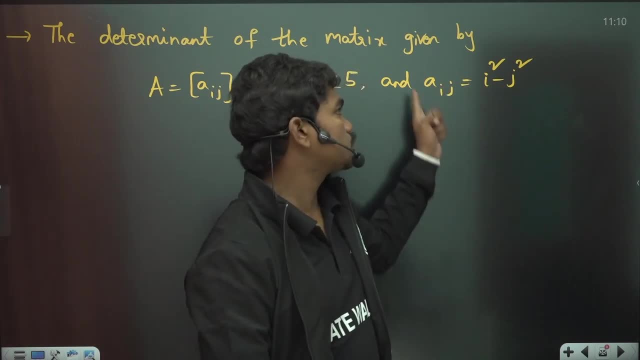 but again slightly complicated. so i square minus j. square means, if you want to calculate third or fourth, to calculate third or fourth, to calculate third or fourth column element three square minus four. column element three square minus four. column element three square minus four. square is going to be a34, correct? so? square is going to be a34, correct. so square is going to be a34 correct. so, like this, if you try to frame a matrix like this, if you try to frame a matrix like this, if you try to frame a matrix, it takes a lot of time to form the. 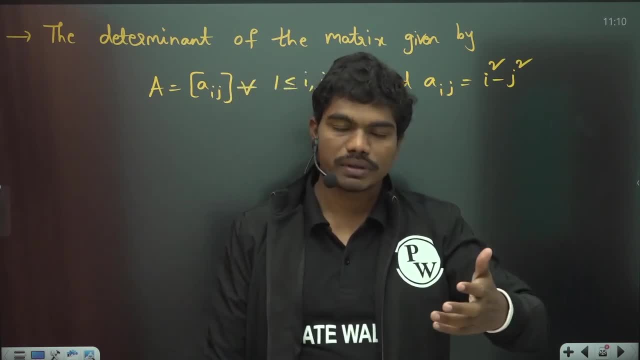 it takes a lot of time to form the. it takes a lot of time to form the matrix. second thing: it's a five by five matrix. second thing: it's a five by five matrix. second thing: it's a five by five matrix. so even after forming the matrix, 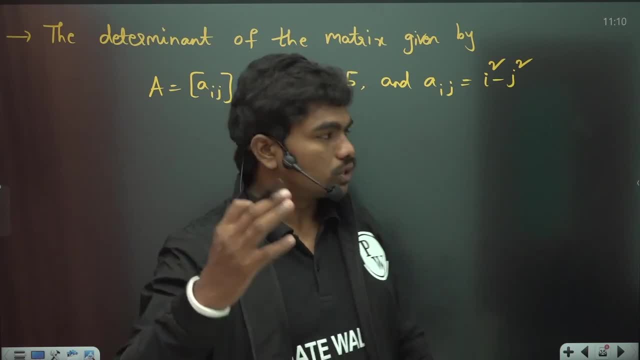 matrix. so even after forming the matrix matrix. so even after forming the matrix, the time taken by you to calculate the, the time taken by you to calculate the, the time taken by you to calculate the determinant, will be very large. so that's determinant will be very large, so that's. 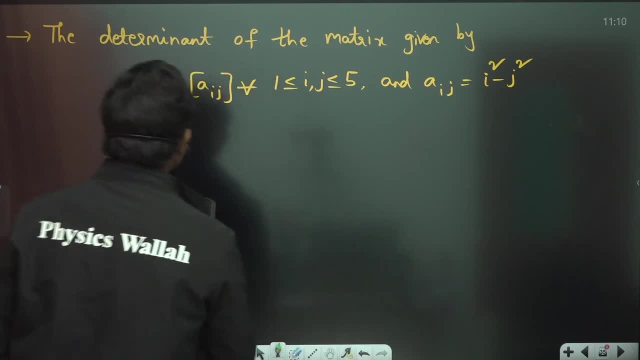 determinant will be very large. so that's why, if you observe one thing carefully, why, if you observe one thing carefully, why, if you observe one thing carefully, in such cases, aij, in such cases, aij, in such cases aij is equal to i square minus j square. 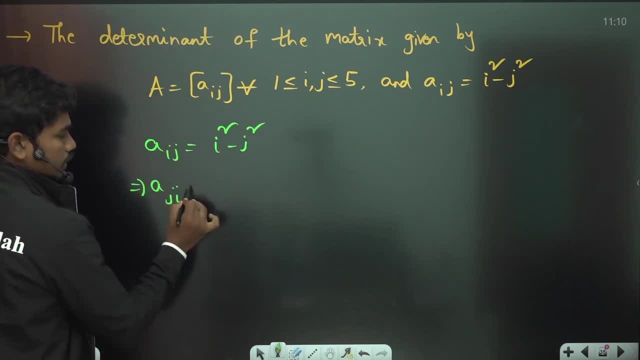 is equal to i square minus j square is equal to i square minus j square, correct? so if i calculate aji, correct? so if i calculate aji, correct. so if i calculate aji, what is this? j square minus i square. what is this? j square minus i square. 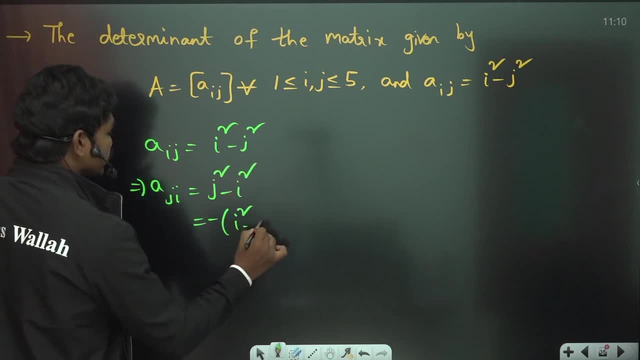 what is this? j square minus i square, obviously correct. so if i pull out a: obviously correct. so if i pull out a, obviously correct. so if i pull out a minus sign, this is i square minus j minus sign: this is i square minus j minus sign: this is i square minus j square, which is nothing but minus this i. 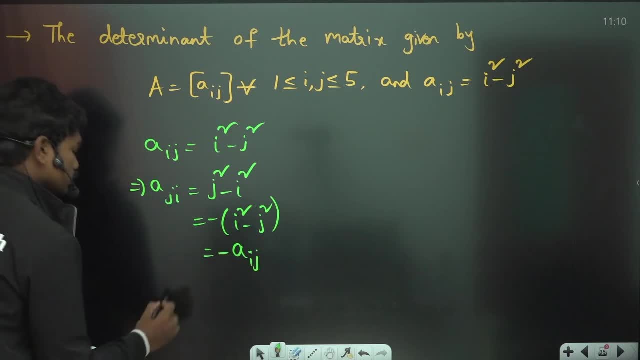 square, which is nothing but minus this. i square which is nothing but minus this. i square minus j square, i can replace with square minus j square. i can replace with square minus j square. i can replace with aij. so that's why, if you see this matrix, 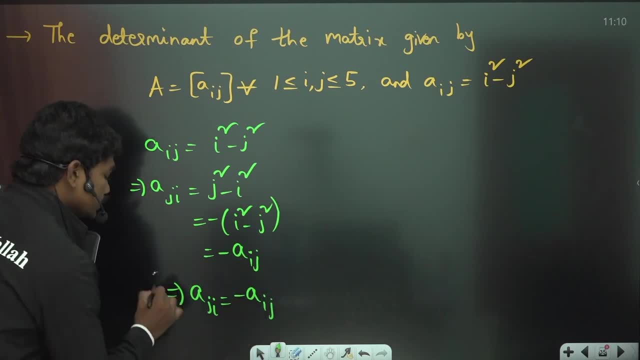 aij. so that's why, if you see this matrix, aij, so that's why, if you see this matrix, aji is equal to minus aij. this is the aji is equal to minus aij. this is the aji is equal to minus aij. this is the notation for this skew symmetric matrix. 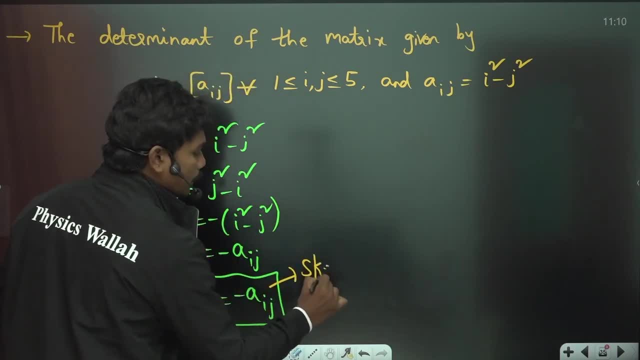 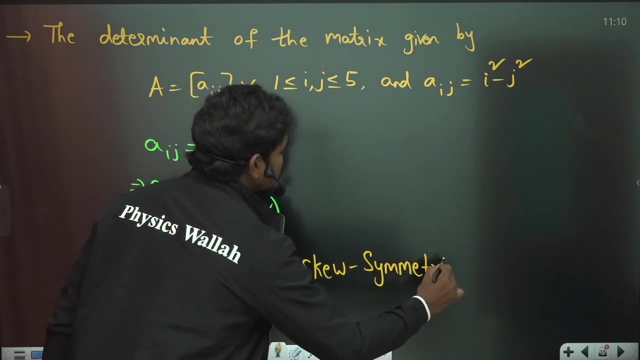 notation for this skew: symmetric matrix. notation for this skew: symmetric matrix. okay, so, if this is the condition, then okay. so, if this is the condition, then okay. so, if this is the condition, then this matrix is skew, this matrix is skew. this matrix is skew. symmetric, symmetric, symmetric skew, symmetric matrix. 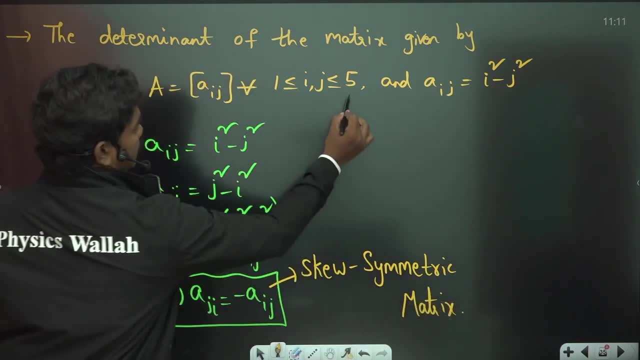 skew symmetric matrix. skew symmetric matrix. so obviously you know that this matrix. so obviously you know that this matrix. so obviously you know that this matrix is a skew symmetric matrix and n value is a skew symmetric matrix and n value is a skew symmetric matrix and n value is odd. so definitely this determinant is: 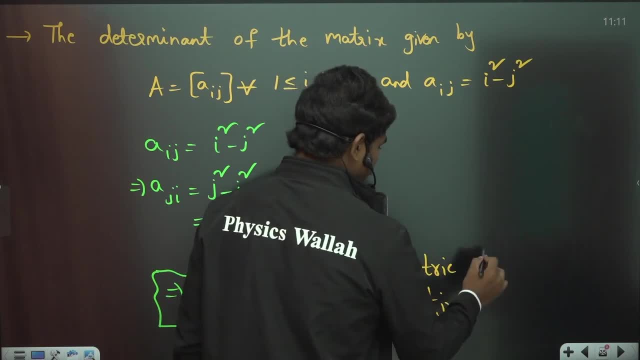 is odd. so definitely this determinant is is odd, so definitely this determinant is going to be zero. okay, so n is equal to going to be zero. okay, so n is equal to going to be zero. okay, so n is equal to five, five, five. n is equal to five, which is odd. 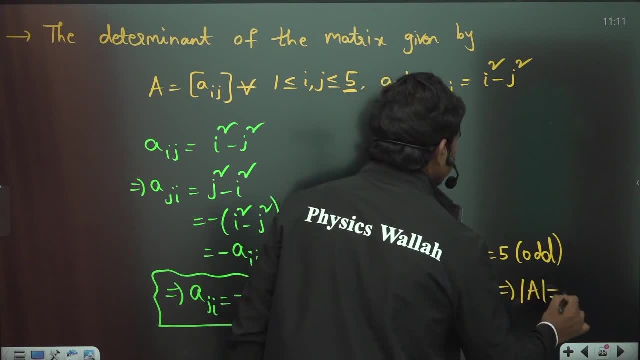 n is equal to five, which is odd. n is equal to five, which is odd. so therefore, you can decide directly that. so, therefore, you can decide directly that. so therefore, you can decide directly that that a is equal to zero. okay, so i'm. that a is equal to zero. okay, so i'm. 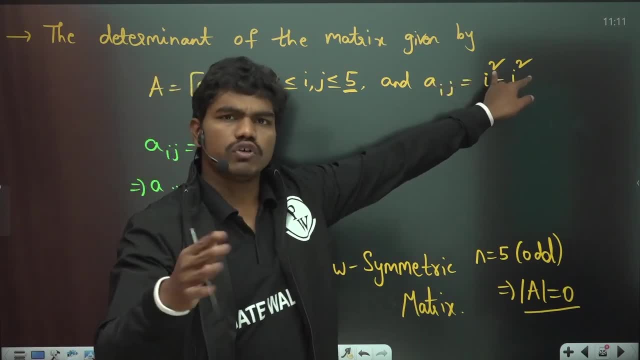 that a is equal to zero. okay, so i'm telling you in general, telling you in general, telling you in general: here, it's need not be two, it can be. here, it's need not be two, it can be. here, it's need not be two, it can be three, four, five, anything, any number as. 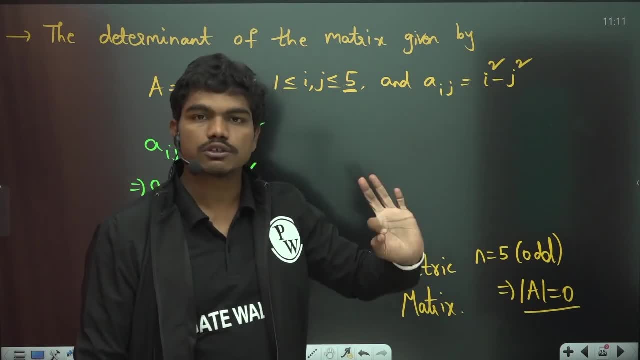 three, four, five, anything any number as three, four, five, anything any number, as long as it is of the format i power k, long as it is of the format i power k. long as it is of the format i power k minus j power k. definitely it's going to. 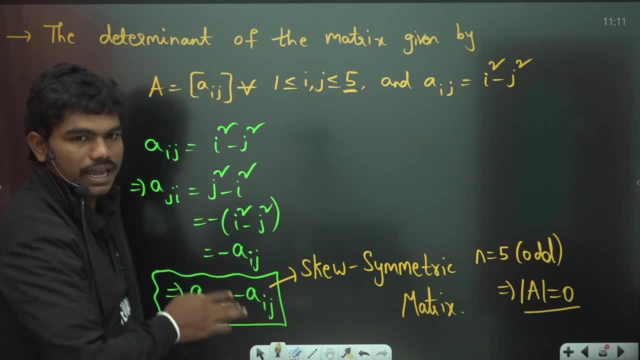 minus j power k. definitely it's going to minus j power k. definitely it's going to be a skew symmetric matrix because of be a skew symmetric matrix because of be a skew symmetric matrix because of this: two, three steps. what i have written: this two, three steps, what i have written. 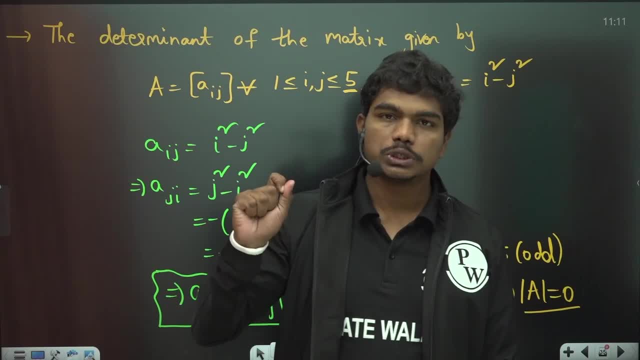 this two, three steps, what i have written here clear. so that's how the determinant here clear. so that's how the determinant here clear. so that's how the determinant of every odd order skew- symmetric matrix of every odd order skew, symmetric matrix of every odd order skew, symmetric matrix is basically zero clear. i hope i am. 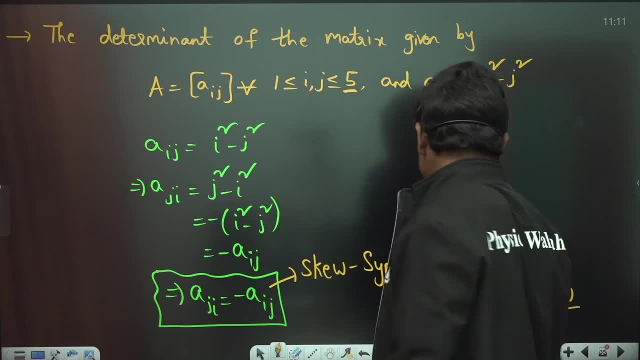 is basically zero clear. i hope i am is basically zero clear. i hope i am clear till this point. so let's go to the clear till this point. so let's go to the clear till this point. so let's go to the next property, next important property. so 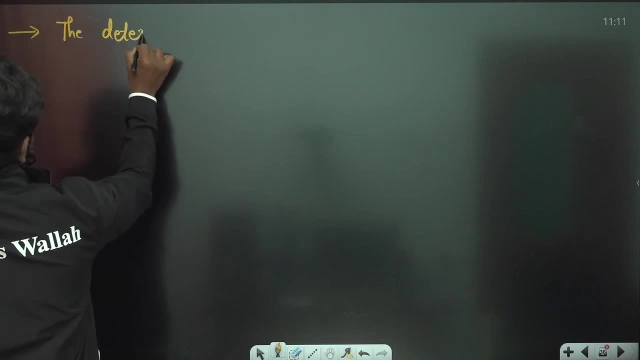 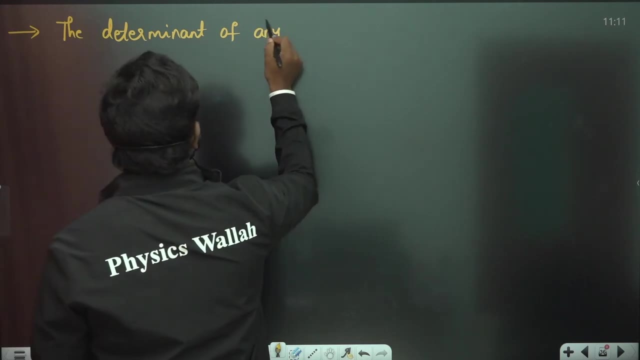 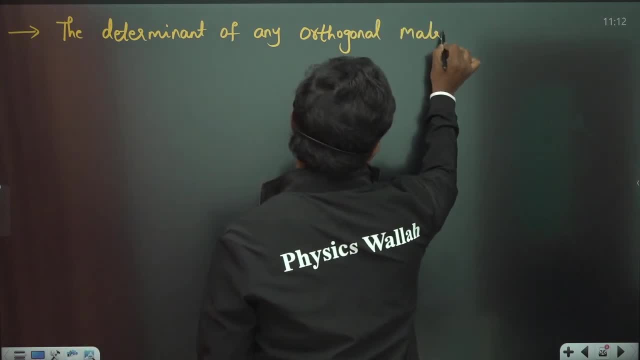 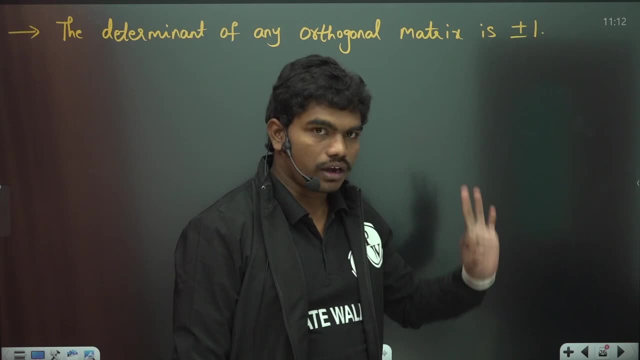 can say. can say the determinant of any orthogonal matrix. the determinant of any orthogonal matrix, the determinant of any orthogonal matrix is is is plus or minus one, that's it okay. you can plus or minus one, that's it okay. you can plus or minus one, that's it okay. you can never find a orthogonal matrix being. 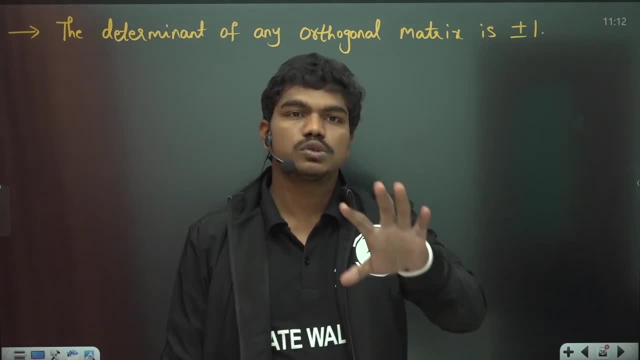 never find a orthogonal matrix being never find a orthogonal matrix being singular, which means singular, which means singular, which means you can never find any orthogonal matrix. you can never find any orthogonal matrix. you can never find any orthogonal matrix whose determinant is zero, basically, whose determinant is zero, basically. 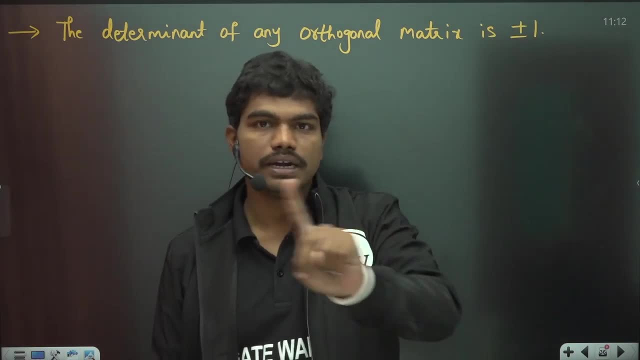 whose determinant is zero. basically clear, because orthogonal matrix can take. clear. because orthogonal matrix can take clear, because orthogonal matrix can take only two values for its determinant one, only two values for its determinant one, only two values for its determinant. one is plus one, another is minus one. okay, 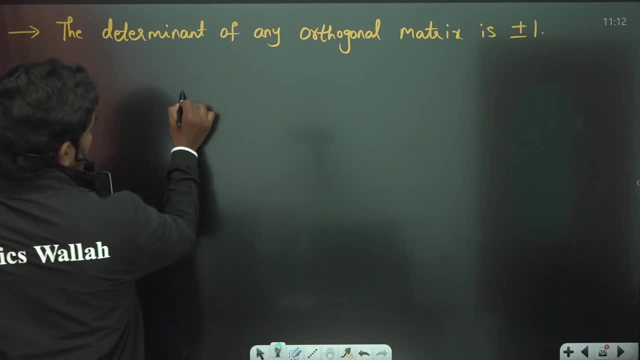 is plus one, another is minus one. okay, is plus one, another is minus one, another is minus one, another is minus one. okay, let's see how this happens. look, let's see how this happens. look, let's see how this happens. look, you have a times a transpose is equal to. 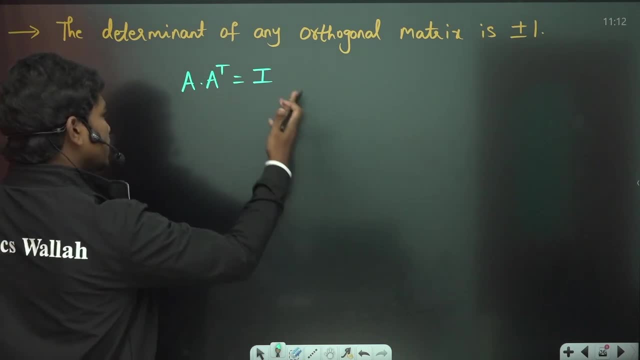 you have a times a transpose is equal to. you have a times a transpose is equal to i. correct so? or a transpose into a: is i correct so? or a transpose into a: is i correct so? or a transpose into a is also equal to i. that's one very. 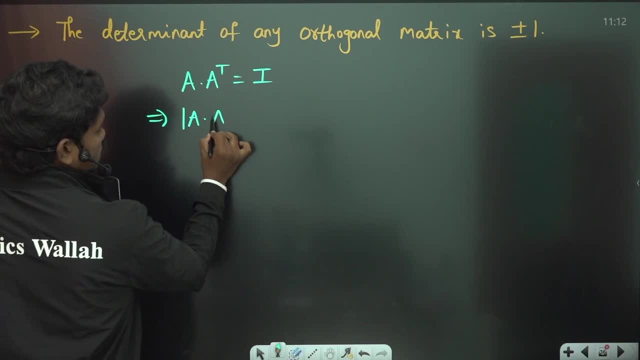 also equal to i. that's one very also equal to i. that's one very important thing. so now, if you see, if you important thing, so now, if you see, if you important thing, so now, if you see, if you apply transpose to both sides of this, apply transpose to both sides of this. 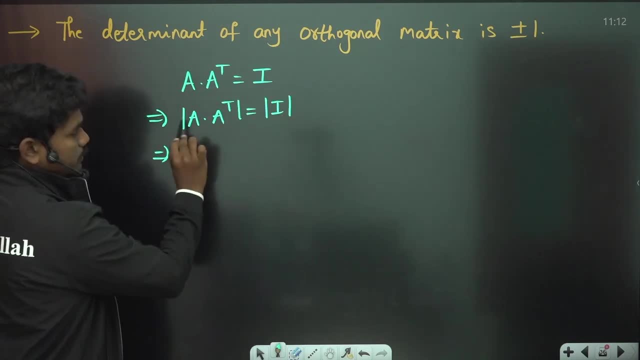 apply transpose to both sides of this. i mean so if you apply determinant to both. i mean so if you apply determinant to both. i mean so if you apply determinant to both sides of this equation: sides of this equation, sides of this equation. this is product of two matrices, so i can. 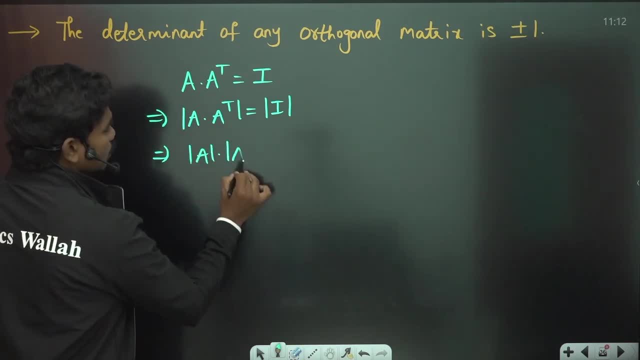 this is product of two matrices, so i can. this is product of two matrices, so i can. write them as individual products. write them as individual products. write them as individual products. that a into that of a transpose is equal. that a into that of a transpose is equal. 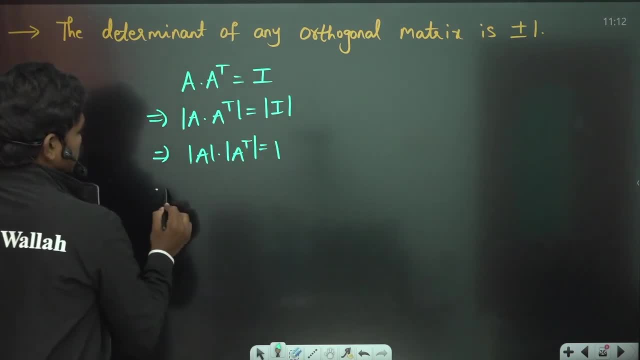 that a into that of a transpose is equal to. we all know the determinant of to. we all know the determinant of to. we all know the determinant of identity matrix is identity matrix is. identity matrix is one, so this implies that a into now one, so this implies that a into now. 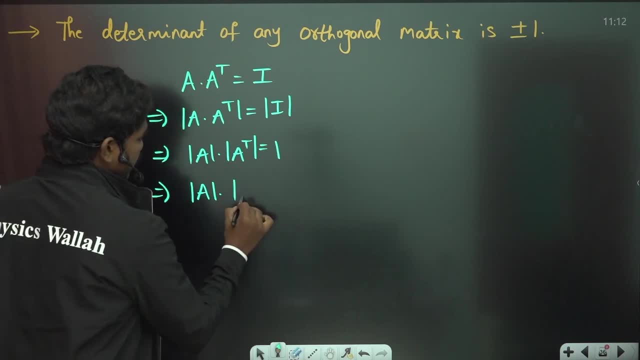 one. so this implies that a into now. determinant of a transpose is same as determinant of a transpose is same as determinant of a transpose is same as that a. so this is again that a and this that a. so this is again that a and this that a. so this is again that a and this is equal to one, so that a whole square is. 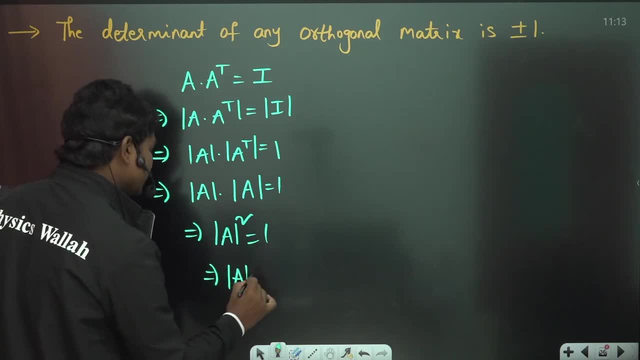 is equal to one, so that a whole square is is equal to one, so that a whole square is equal to one. so this determinant of a is equal to one. so this determinant of a is equal to one. so this determinant of a is basically equal to plus or minus one. so 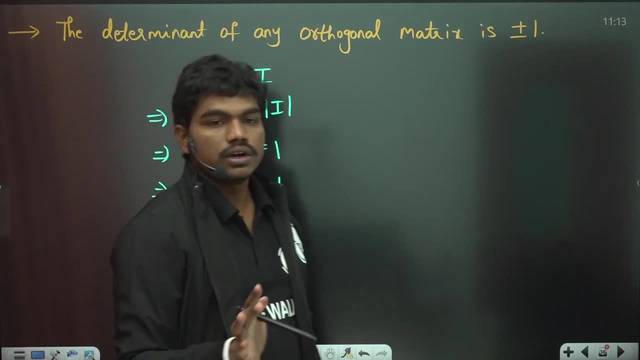 basically equal to plus or minus one. so basically equal to plus or minus one. so if you find one thing I have told you in, if you find one thing I have told you in, if you find one thing I have told you in a studies class also, normally, since you 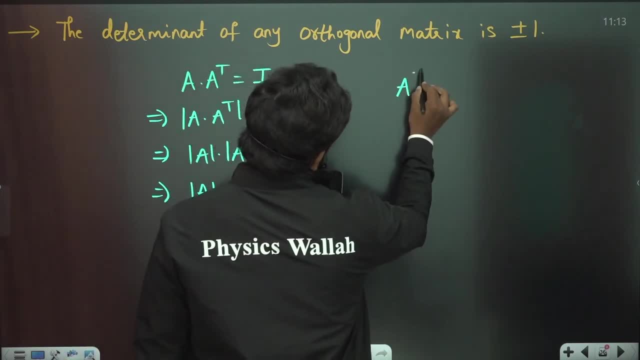 a studies class also normally, since you a studies class also normally, since you know what is inverse and all I'll tell know what is inverse and all I'll tell know what is inverse and all I'll tell you one thing: I told you a inverse is you one thing I told you a inverse is. 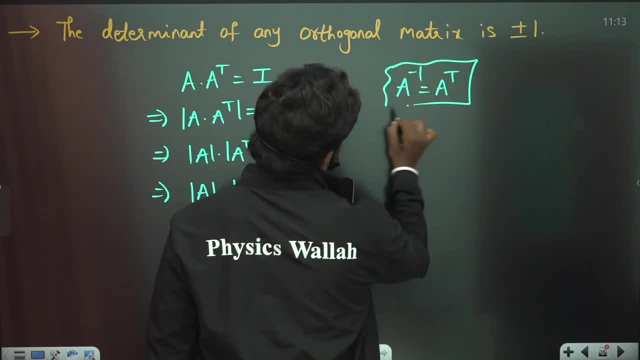 you one thing. I told you: a inverse is equal to a transpose for this matrix. equal to a transpose for this matrix, equal to a transpose for this matrix. correct, if you remember for this, correct, if you remember for this, correct, if you remember, for this orthogonal matrix, a inverse is equal to a. 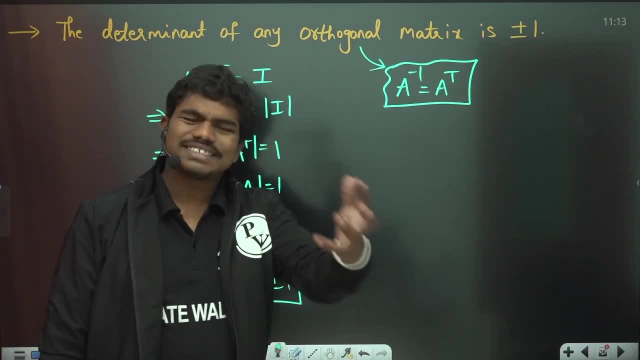 orthogonal matrix. a inverse is equal to a orthogonal matrix. a inverse is equal to a transpose. now for the given orthogonal transpose. now for the given orthogonal transpose. now for the given orthogonal matrix. you can always have transpose matrix. you can always have transpose matrix. you can always have transpose, because transpose is nothing but just. 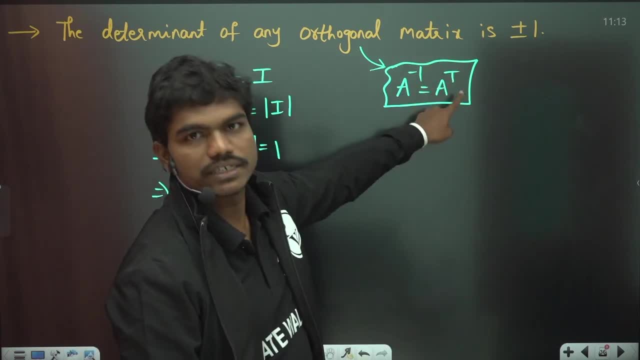 because transpose is nothing, but just because transpose is nothing but just interchanging rows and columns. so if a interchanging rows and columns, so if a interchanging rows and columns, so if a transpose is always present, a inverse is transpose is always present, a inverse is transpose is always present. a inverse is also always present, and you can clearly. 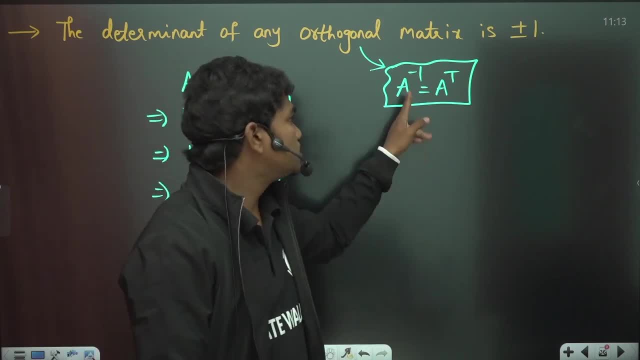 also always present and you can clearly also always present and you can clearly know from this: this determinant is never know from this. this determinant is never know from this. this determinant is never going to be zero. so there is no going to be zero. so there is no. 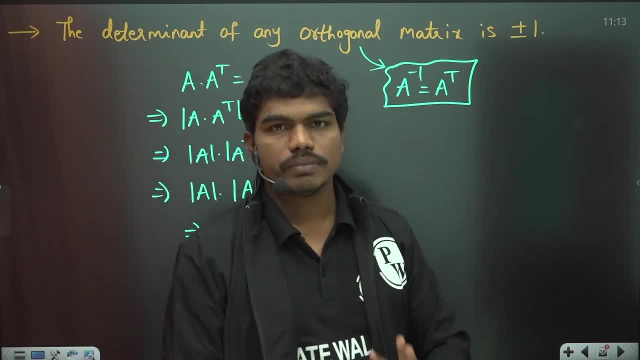 going to be zero. so there is no obstruction for the formation of this, a obstruction for the formation of this, a obstruction for the formation of this, a inverse clear, and basically I want to inverse clear and basically I want to inverse clear and basically I want to tell you one thing: what is orthogonal? 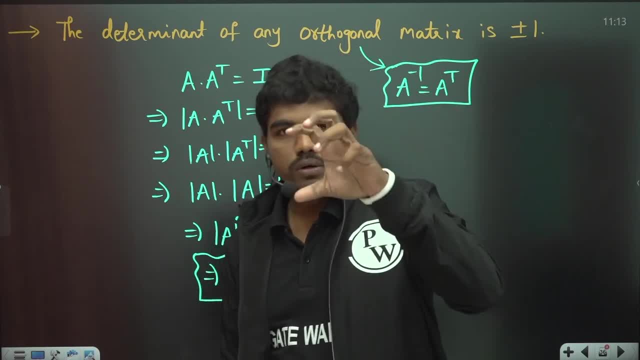 tell you one thing: what is orthogonal. tell you one thing, what is orthogonal. matrix also. I'll tell you basically so. matrix also, I'll tell you basically so. matrix also. I'll tell you basically so, if you take any two rows on any two, if you take any two rows on any two, 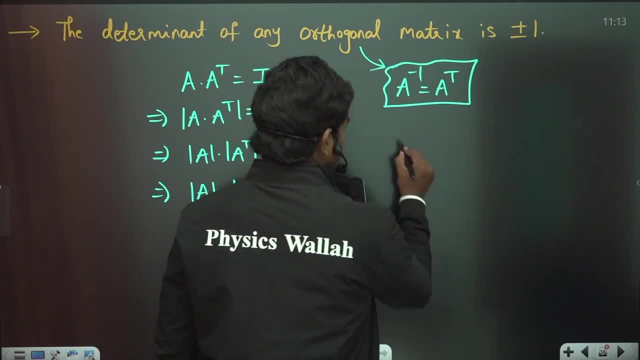 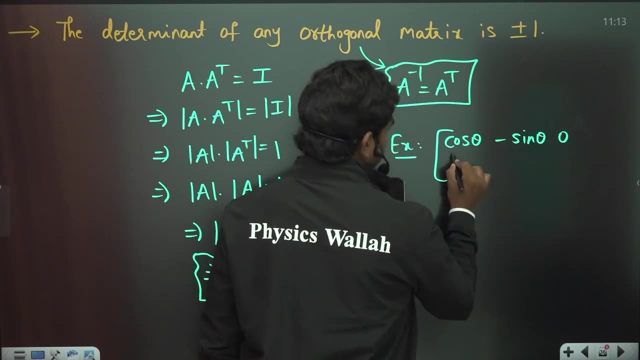 if you take any two rows on any two columns of any orthogonal matrix, for columns of any orthogonal matrix, for columns of any orthogonal matrix, for example, I have given you this matrix example. I have given you this matrix example. I have given you this matrix: cos theta minus sine theta, 0 sine theta. 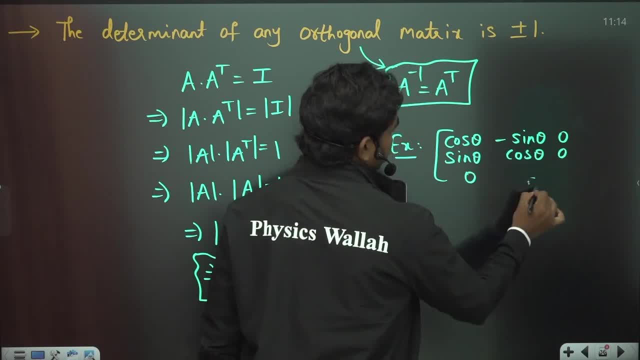 cos theta minus sine theta: 0 sine theta cos theta minus sine theta: 0 sine theta cos theta 0, 0, 0, 1. so basically, if you cos theta 0, 0, 0, 1, so basically, if you cos theta 0, 0, 0, 1, so basically, if you take any tools or two columns, then those 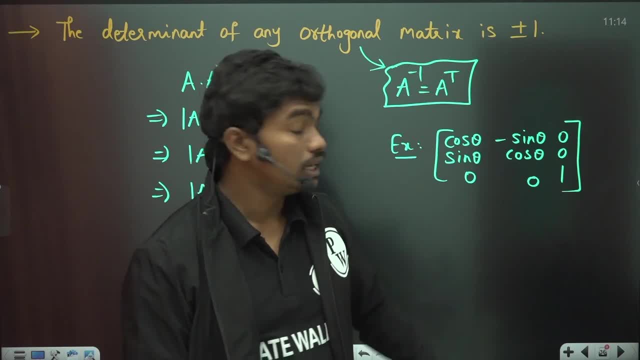 take any tools or two columns, then those take any tools or two columns, then those tools and two columns will be tools and two columns will be tools and two columns will be perpendicular to each other. what is the perpendicular to each other? what is the perpendicular to each other? what is the meaning of this? let us suppose, if I add: 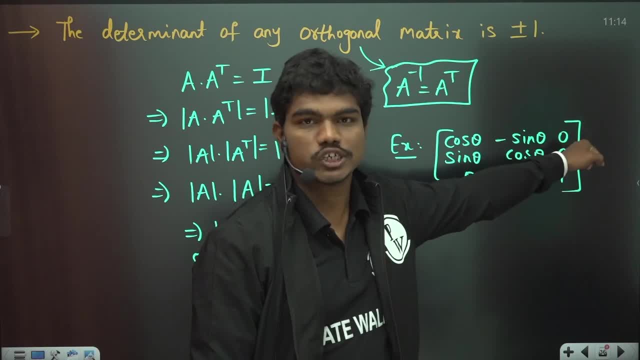 meaning of this. let us suppose if I add meaning of this. let us suppose if I add this: as cos theta i bar plus minus sine this, as cos theta i bar plus minus sine this, as cos theta i bar plus minus sine theta j bar plus 0 into k bar. similarly, 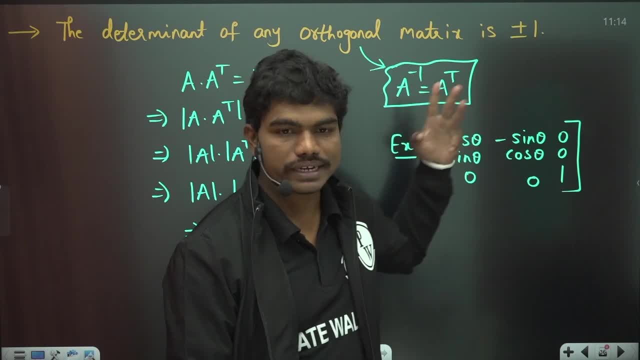 theta j bar plus 0 into k bar. similarly theta j bar plus 0 into k bar. similarly, sine theta i bar plus cos theta into j sine theta i bar plus cos theta into j sine theta i bar, plus cos theta into j bar plus 0 into k bar. means, if I take 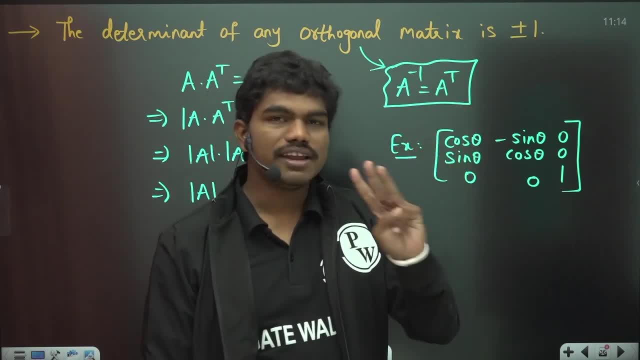 bar plus 0 into k bar. means if I take bar plus 0 into k bar, means if I take these three rows as three vectors for these three rows as three vectors for these three rows as three vectors, for example, then if I take any two vectors, 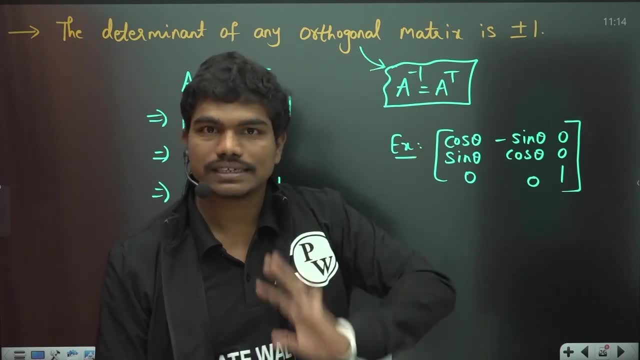 example, then if I take any two vectors example, then if I take any two vectors, then definitely the dot product of these, then definitely the dot product of these, then definitely the dot product of these two is going to be 0. you can tie if you two is going to be 0, you can tie if you. 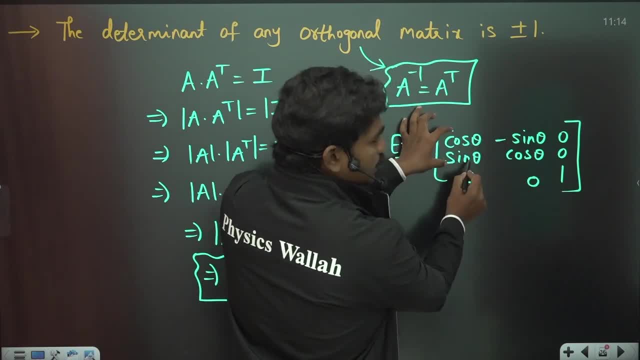 two is going to be 0. you can tie if you want. look if I multiply these two rows. want. look if I multiply these two rows. want. look if I multiply these two rows. for example, cos theta into sine theta. for example, cos theta into sine theta. for example, cos theta into sine theta, sine theta, cos theta plus minus, sine theta. 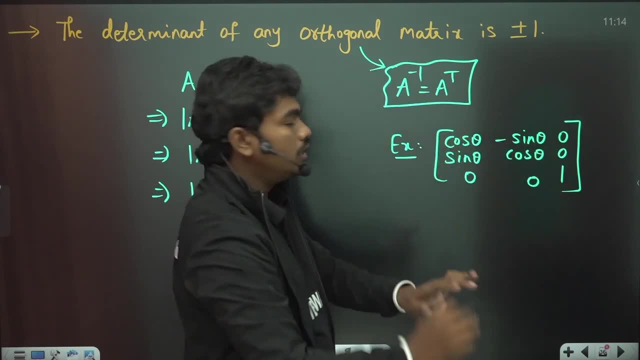 sine theta, cos theta plus minus sine theta. sine theta, cos theta plus minus sine theta into cos theta. this two gets cancelled into cos theta. this two gets cancelled into cos theta. this two gets cancelled: 0 into 0, 0 again. similarly, if you take 0 into 0, 0 again similarly, if you take: 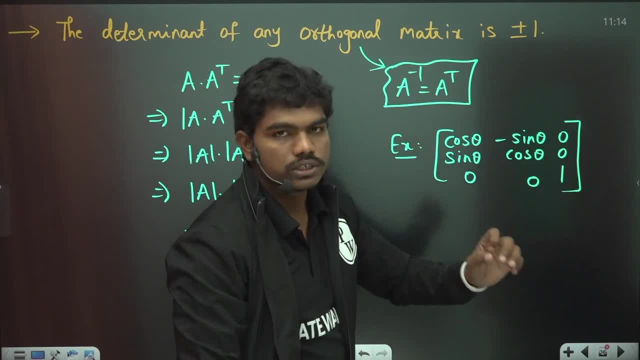 0 into 0, 0 again. similarly, if you take any two rows 0 into sine, theta, 0 into cos, any two rows 0 into sine, theta 0 into cos, any two rows 0 into sine theta, 0 into cos, theta 1 into 0, again, 0. so dot, product of. 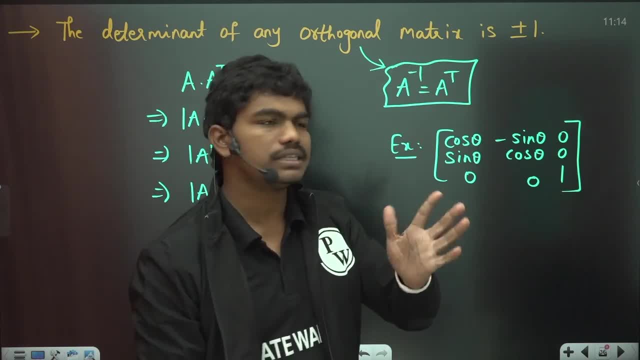 theta 1 into 0, again 0, so dot product of theta 1 into 0, again 0, so dot product of any two, any two, you know rose. if you any two, any two, you know rose. if you any two, any two, you know rose. if you take by general this or columns, also it. 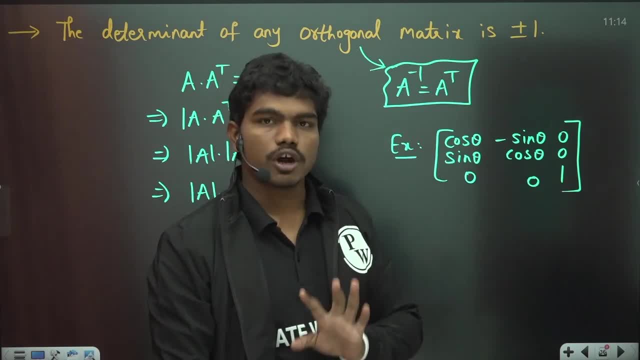 take by general this or columns also. it take by general this or columns also. it can be, for example, you can take first, can be, for example, you can take first, can be, for example, you can take first and last column, any two columns this dot and last column, any two columns, this dot. 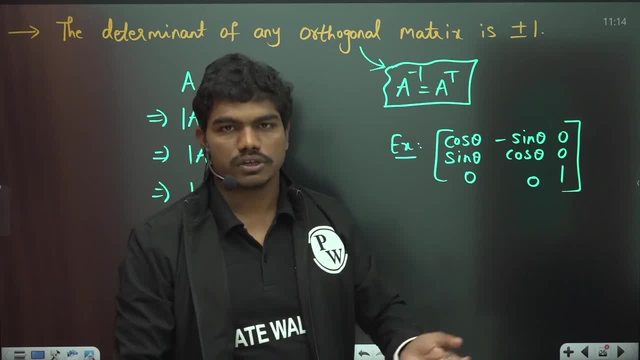 and last column, any two columns, this dot. product will always MN 0, which means product will always MN 0, which means product will always MN 0, which means- and that's the name why this matrix is, and that's the name why this matrix is, and that's the name why this matrix is also called orthogonal means. 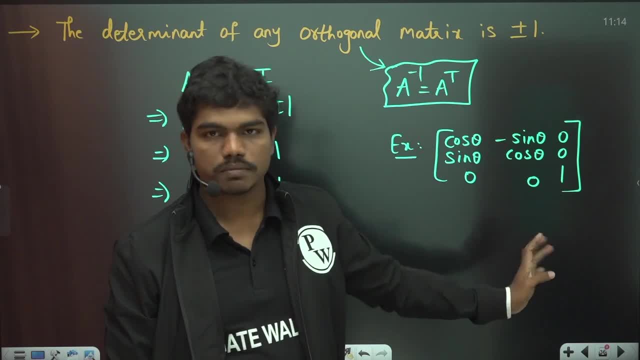 also called orthogonal means. also called orthogonal means perpendicularity. if you take any two perpendicularity, if you take any two perpendicularity, if you take any two rows or columns and if you do the dot rows or columns and if you do the dot rows or columns and if you do the dot product of these vectors, definitely will. 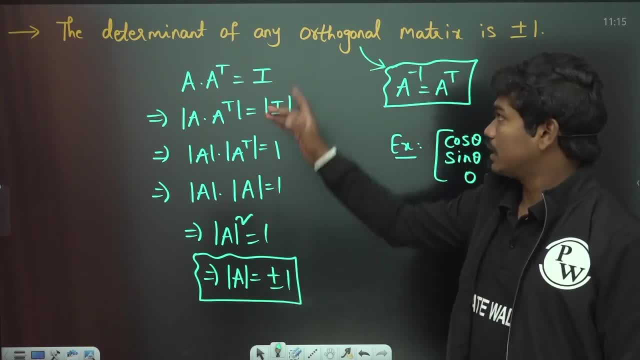 product of these vectors definitely will. product of these vectors definitely will get 0 here clear. so that's why this get 0 here clear. so that's why this get 0 here clear. so that's why this analysis and this matrix is one way: analysis and this matrix is one way. 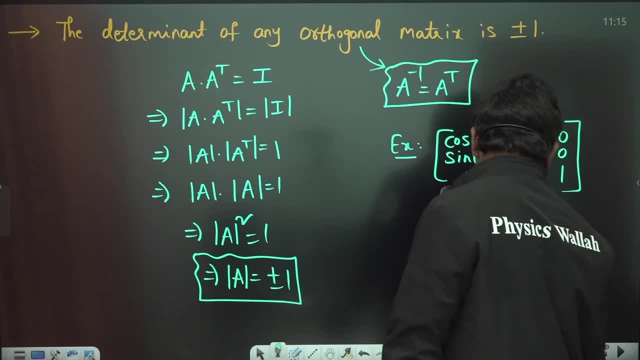 analysis. and this matrix is one way. special kind of matrix, actually clear. special kind of matrix, actually clear. special kind of matrix, actually clear. now let us go for some more properties now, let us go for some more properties. now let us go for some more properties. the determinant of 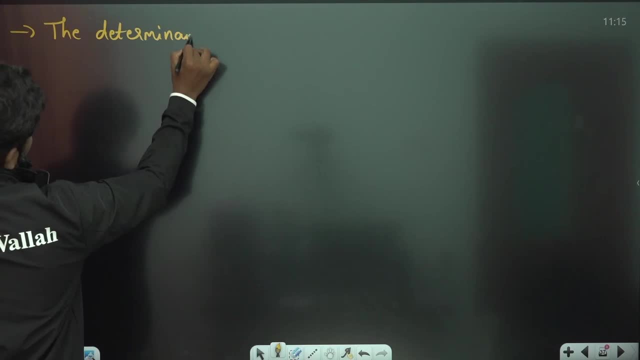 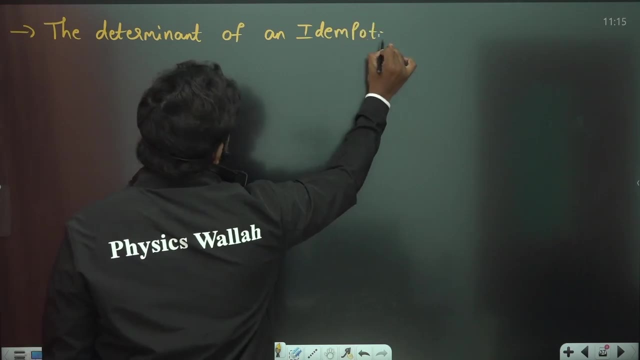 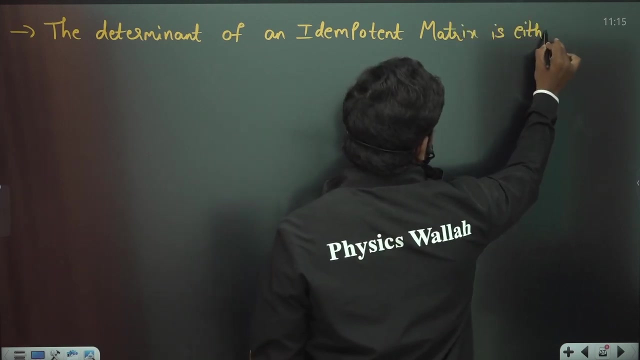 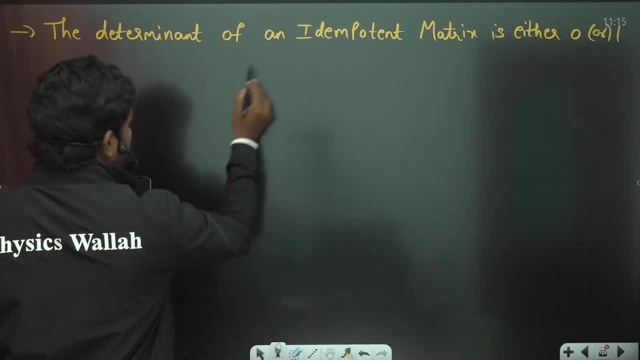 is either 0 or 1 is either 0 or 1 again. how you know this again. look, we have seen how you know this again. look, we have seen how you know this again. look, we have seen the definition of item potent matrix, so a. the definition of item potent matrix, so a. 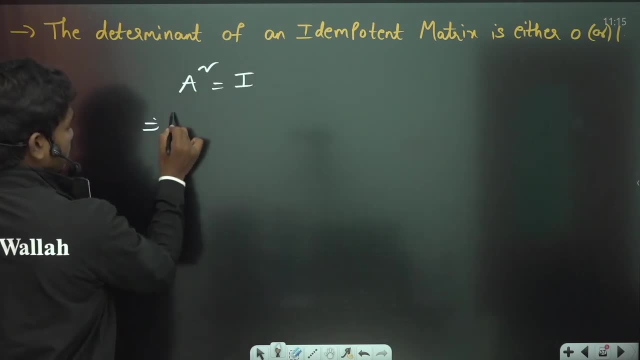 the definition of item: potent matrix. so a square is equal to I. so if you apply square is equal to I. so if you apply: square is equal to I. so if you apply determinant on both sides, that a whole determinant on both sides, that a whole determinant on both sides, that a whole square is equal to I and that I so this. 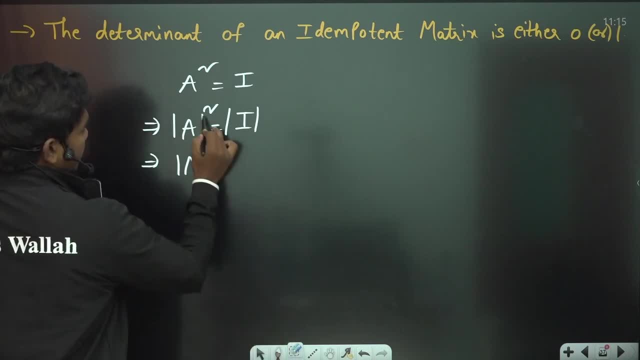 square is equal to I, and that I so this square is equal to I, and that I so this- that a whole square can be witness, or you that a whole square can be witness, or you that a whole square can be witness, or you can write that a square, this can be. 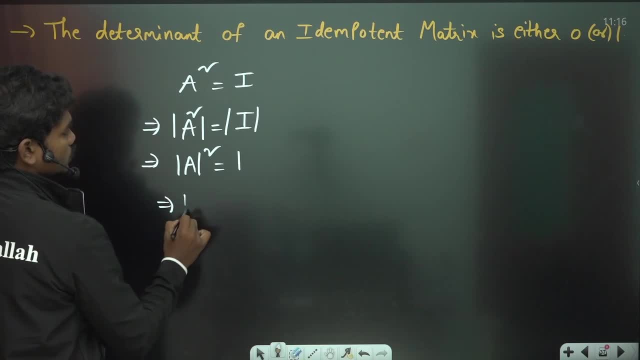 can write that a square this can be. can write that a square. this can be written as that: a whole square which is written as that. a whole square which is written as that. a whole square which is equal to 1, so that a is going to be I'm. 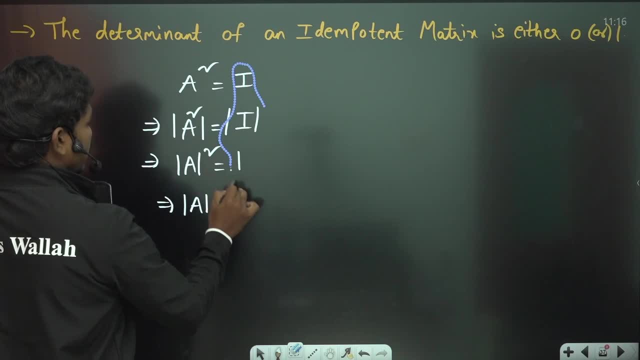 equal to 1, so that a is going to be I'm equal to 1, so that a is going to be I'm sorry, so we are talking about item. sorry so we are talking about item. sorry so we are talking about item. potent idea, then, this is not I, this is a. 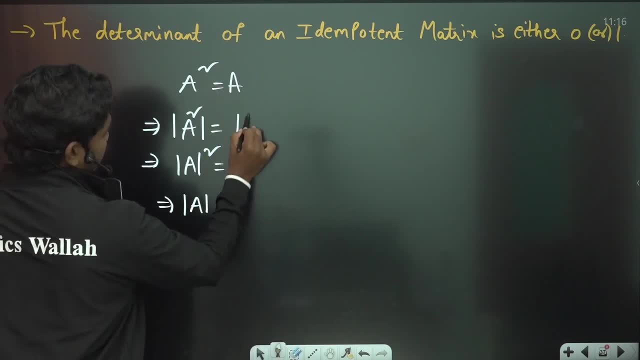 potent idea, then this is not I. this is a potent idea, then this is not I. this is a because item potent is a. so if you see, because item potent is a. so if you see, because item potent is a, so if you see, this is that a and this is that a. so if 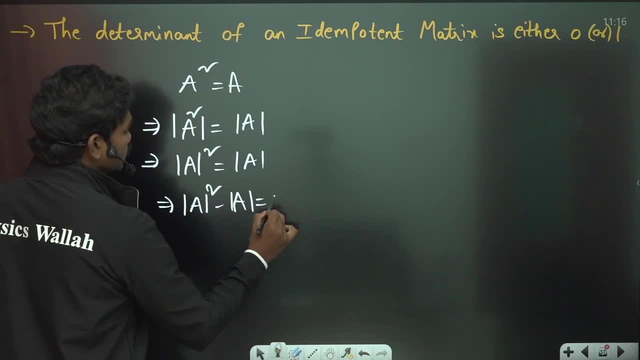 this is that a and this is that a. so if this is that a and this is that a, so if you bring this that a square minus that, you bring this that a square minus that, you bring this that a square minus, that a is equal to 0. so this implies, if you: 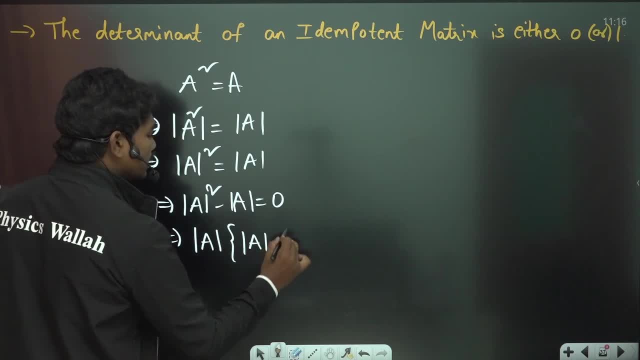 a is equal to 0. so this implies: if you a is equal to 0, so this implies: if you take that a common, then you have that a. take that a common, then you have that a. take that a common, then you have that a minus 1 is equal to 0. so this is a. 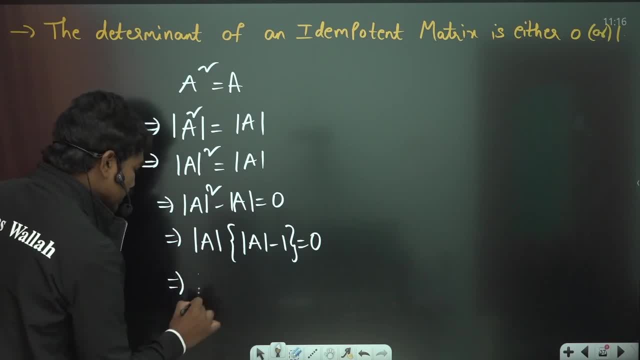 minus 1 is equal to 0. so this is a minus 1 is equal to 0, so this is a scalar multiplication. so definitely if scalar multiplication, so definitely if scalar multiplication, so definitely. if the term has to be 0, this implies either the term has to be 0, this implies either. 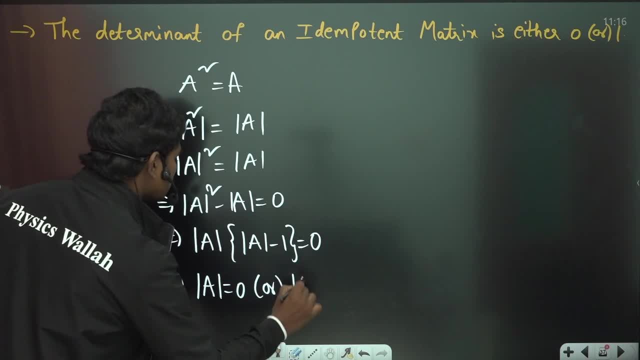 the term has to be 0. this implies either that a should be 0 or that a minus 1, that a should be 0 or that a minus 1, that a should be 0 or that a minus 1 should be 0, which means that a can take. 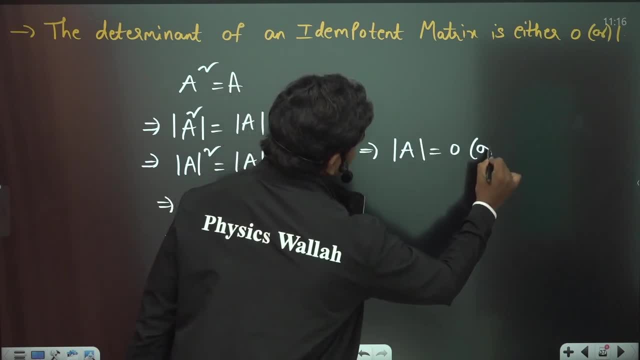 should be 0, which means that a can take. should be 0, which means that a can take two values which are nothing but either two values which are nothing but, either two values which are nothing but either 0 or 1, so it's not always guaranteed. 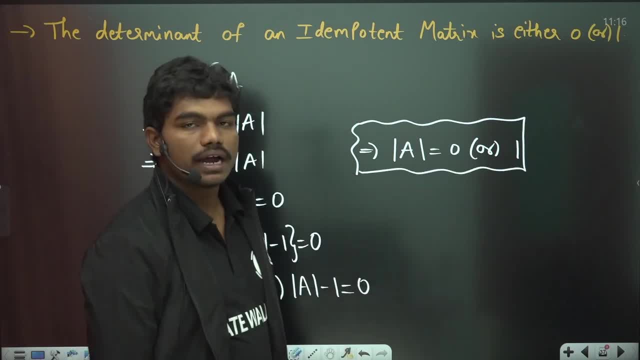 0 or 1, so it's not always guaranteed 0 or 1, so it's not always guaranteed that idempotent matrix have inverse, that idempotent matrix have inverse, that idempotent matrix have inverse, because probably the idempotent matrix, because probably the idempotent matrix. 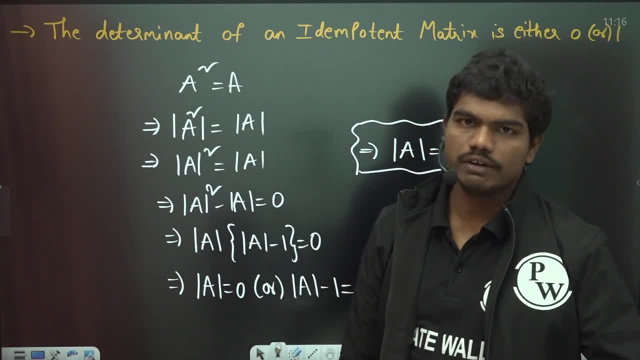 because probably the idempotent matrix can have a zero determinant and can have a zero determinant and can have a zero determinant and obviously may not find the you know. obviously may not find the you know, obviously may not find the you know inverse, sometimes. okay, so whereas in 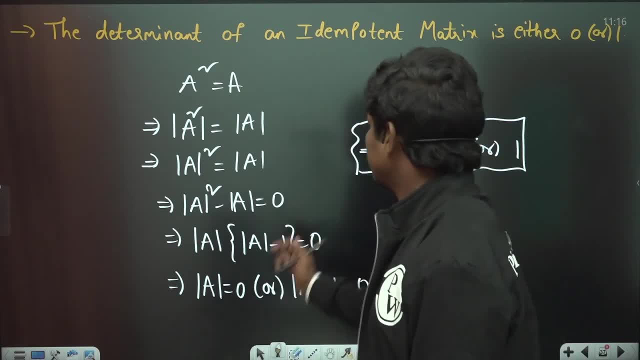 inverse sometimes okay, so, whereas in inverse, sometimes okay. so whereas in case of orthogonal you can always assure case of orthogonal, you can always assure case of orthogonal, you can always assure there is some inverse existing, okay. so there is some inverse existing, okay, so there is some inverse existing, okay. so anyhow, this is the case. now let's talk. 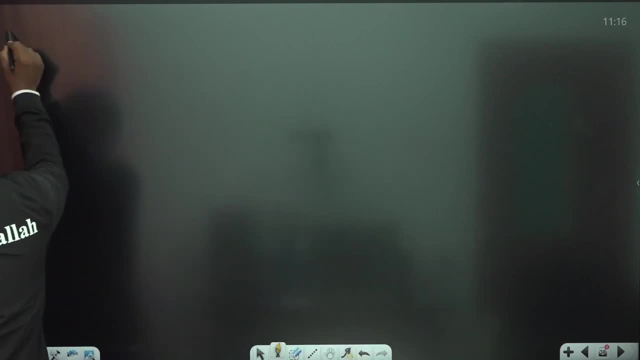 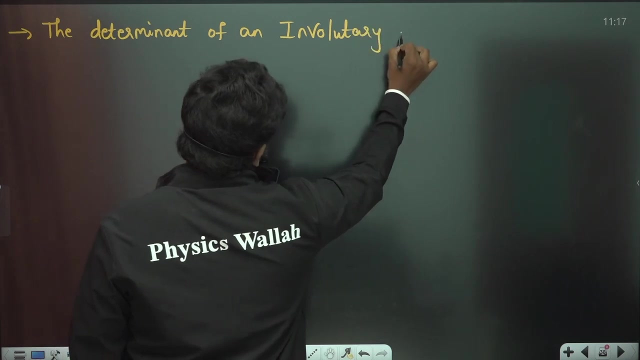 anyhow. this is the case now. let's talk anyhow. this is the case now. let's talk about invalidity also. the determinant of the determinant of an involute a matrix. an involute a matrix, an involute a matrix. the determinant of an involute a matrix. 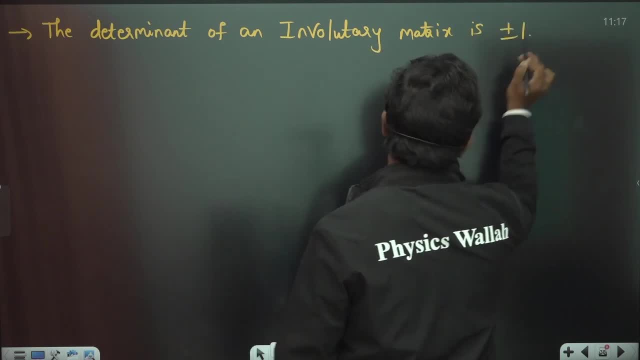 the determinant of an involute, a matrix. the determinant of an involute, a matrix is again plus or minus one. okay, as you is again plus or minus one. okay, as you is again plus or minus one. okay, as you have seen, have seen, have seen just now. so a square is equal to I, so this: 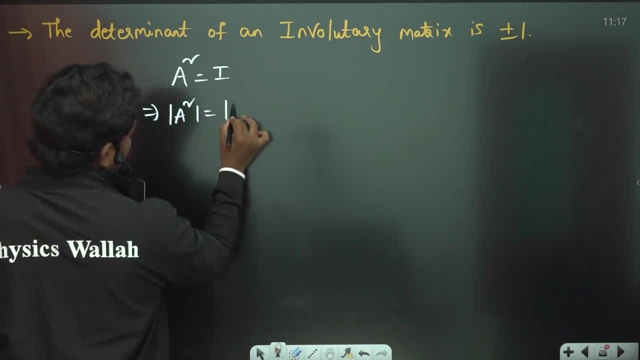 just now. so a square is equal to I. so this just now. so a square is equal to I. so this implies that of a square is equal to. implies that of a square is equal to. implies that of a square is equal to that of I. so this implies that a whole 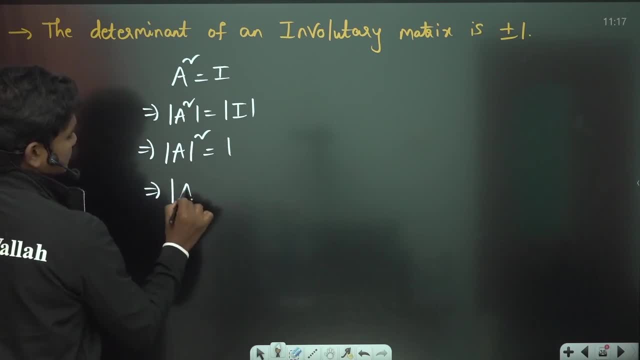 that of I. so this implies that a whole that of I. so this implies that a whole square is equal to this. one which means square is equal to this. one which means square is equal to this. one which means that a is equal to plus or minus one. so 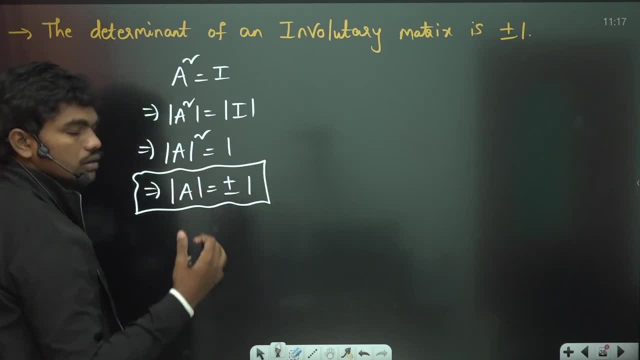 that a is equal to plus or minus one. so that a is equal to plus or minus one. so this is again one very important you. this is again one very important you. this is again one very important. you know result again okay, so sometimes they know. result again okay, so sometimes they. 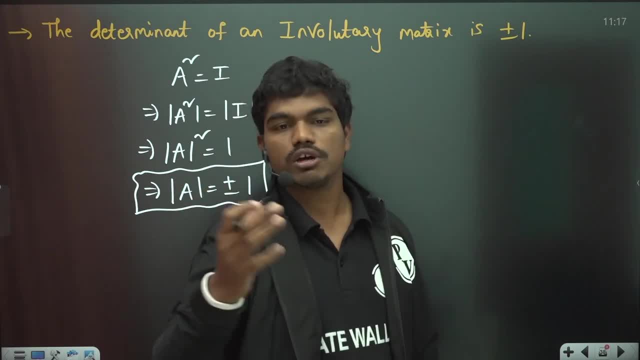 know. result again, okay. so sometimes they ask you in examination, they will give. ask you in examination, they will give. ask you in examination, they will give. you choose the wrong statement, the. you choose the wrong statement, the you choose the wrong statement. the determinant of an invalidity matrix is: 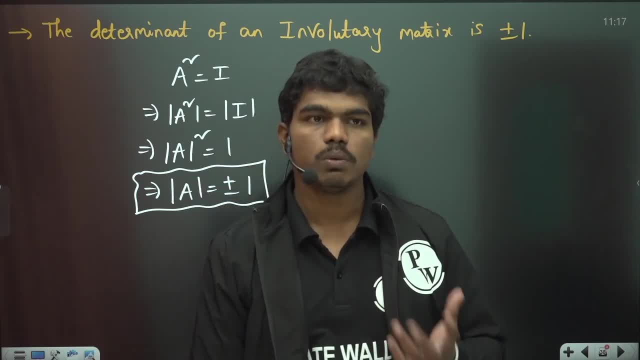 determinant of an invalidity matrix is determinant of an invalidity matrix is zero such sentences. they can give you zero such sentences. they can give you zero such sentences they can give you okay. so at that time you should know. okay, so at that time you should know. okay, so at that time you should know what is in value T, why these things are, what is in value T, why these things are, what is in value T, why these things are happening. but trust me, one thing: I'm happening. but trust me one thing: I'm. 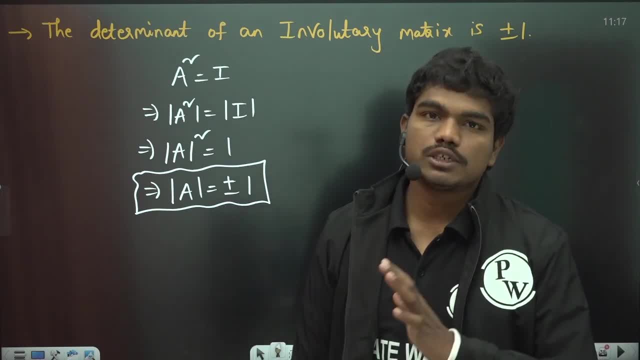 happening. but trust me, one thing I'm telling you your university exam, maths is telling you your university exam, maths is telling you your university exam: maths is much lengthier as compared to get maths. much lengthier as compared to get maths. much lengthier as compared to get maths and get maths is relatively very simple. 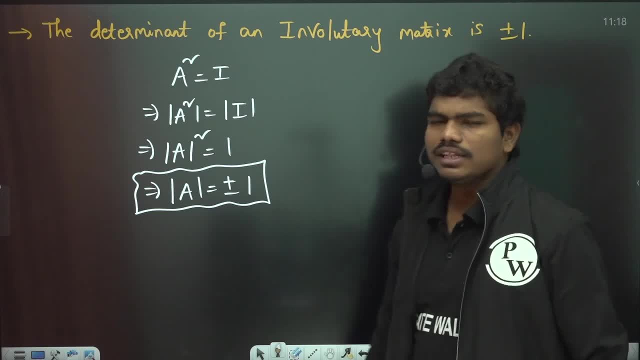 and get maths is relatively very simple and get maths is relatively very simple, clear. so now let us try to understand clear. so now let us try to understand clear. so now let us try to understand this fine, this formulas and all are fine. this fine, this formulas and all are fine. 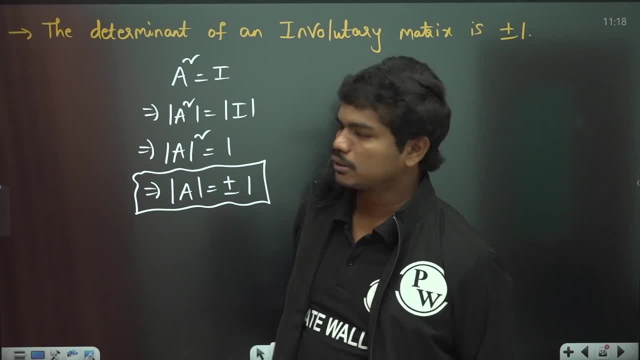 this fine, this formulas and all are fine. but let us suppose if you multiply two. but let us suppose if you multiply two. but let us suppose if you multiply two matters because next property I'm going matters, because next property I'm going matters, because next property I'm going to talk about some, something about. 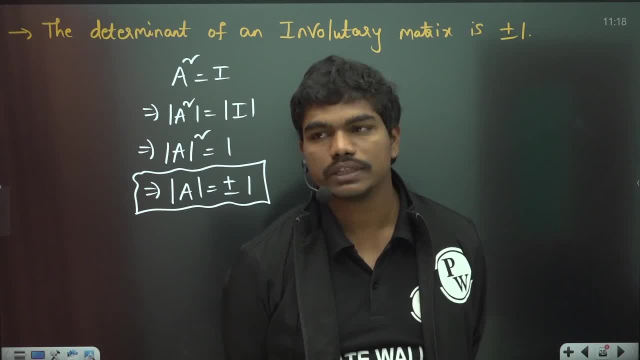 to talk about some. something about to talk about some. something about determinant of multiplication, something determinant of multiplication, something determinant of multiplication, something like that. now try to understand one like that. now try to understand one like that. now try to understand one thing. let us suppose you're actually 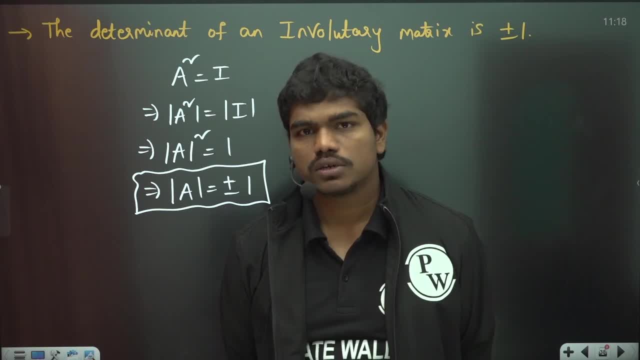 thing. let us suppose you're actually thing. let us suppose you're actually multiplying some matrices: okay, but for multiplying some matrices, okay, but for multiplying some matrices, okay, but for example two matrices, then what actually? example two matrices, then what actually example two matrices, then what actually you're doing? okay, this means okay. 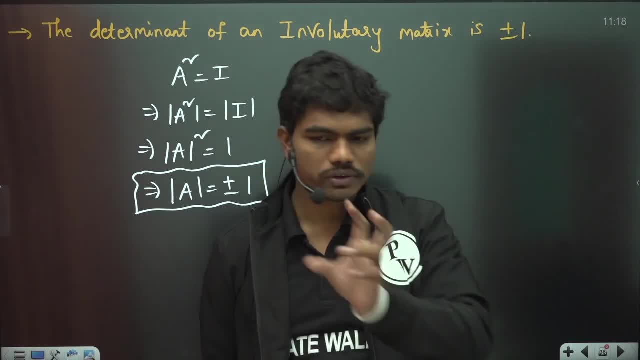 you're doing okay. this means okay. you're doing okay. this means okay. multiplication ways- you know this into multiplication ways. you know this into multiplication ways. you know this into this. you'll multiply additions this. you'll multiply additions this. you'll multiply additions everything. you'll get one matrix. but 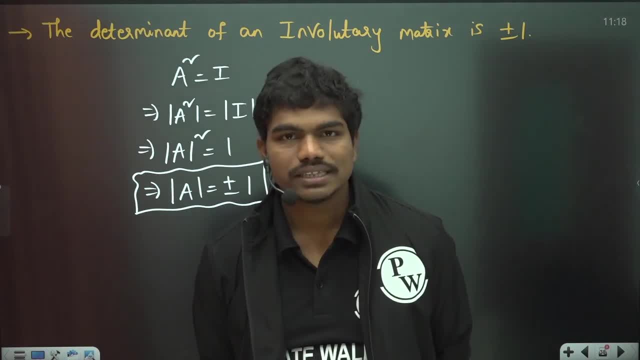 everything, you'll get one matrix. but everything, you'll get one matrix. but actually, what is that multiplication? do actually what is that multiplication? do actually what is that multiplication? do it okay. so basically, these are called it okay. so basically, these are called it okay. so basically, these are called transformation of matrices, or you can. 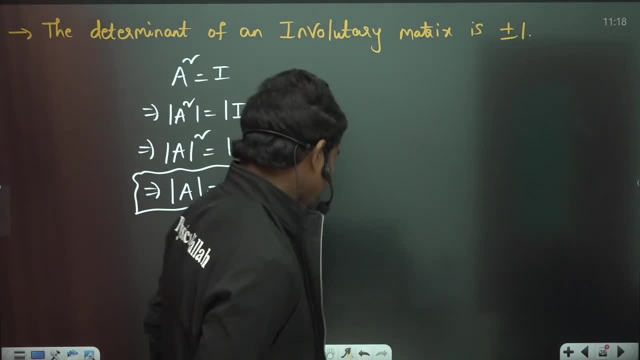 transformation of matrices. or you can transformation of matrices, or you can say this called transformation matrices, say this called transformation matrices, say this called transformation matrices, means. let us suppose if I have an means. let us suppose if I have an means. let us suppose if I have an example. I will give you one simple. 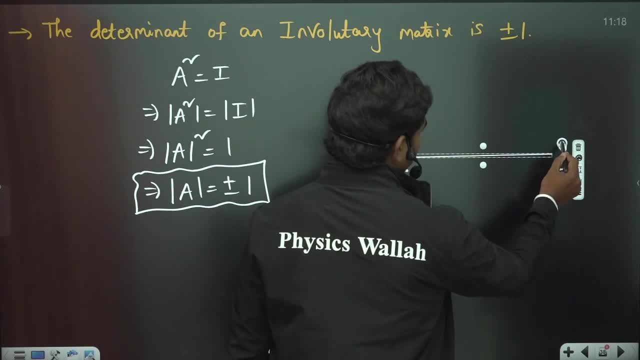 example. I will give you one simple example. I will give you one simple example. let us suppose you have some example. let us suppose you have some example. let us suppose you have some plane, for example. okay, so this is plane. plane, for example: okay, so this is plane. 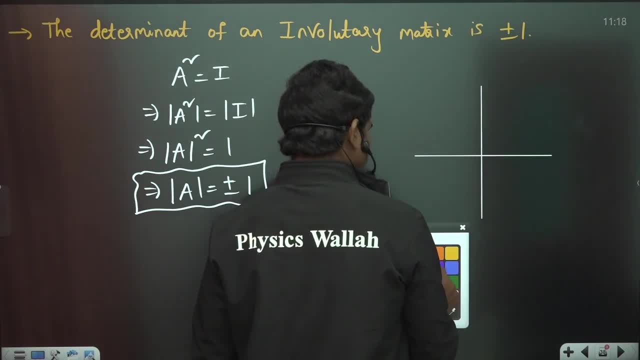 plane, for example. okay, so this is plane, this is plane now. let us suppose you this is plane now. let us suppose you this is plane now. let us suppose you have a line Y is equal to X, which is. have a line Y is equal to X, which is: 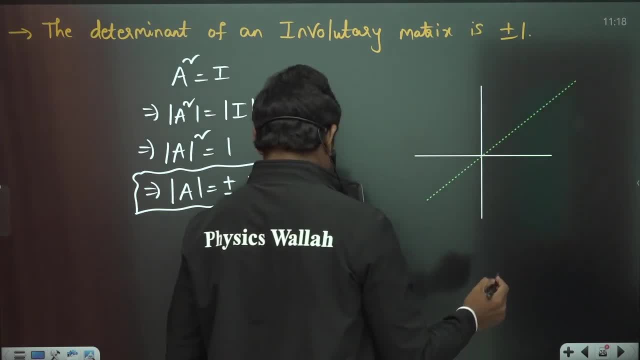 have a line- Y is equal to X- which is passing through the horizon. of course Y passing through the horizon, of course Y passing through the horizon. of course Y is equal to X. Y is equal to X. this is is equal to X. Y is equal to X. this is. 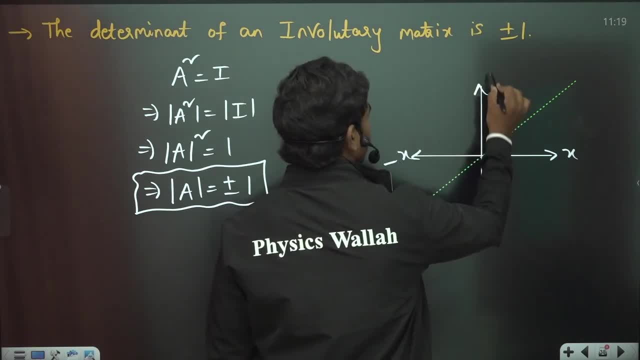 is equal to X. Y is equal to X. this is X axis. this is minus X. this is Y. this is X axis. this is minus X. this is Y. this is X axis. this is minus X. this is Y. this is minus Y. and let us suppose this is the. 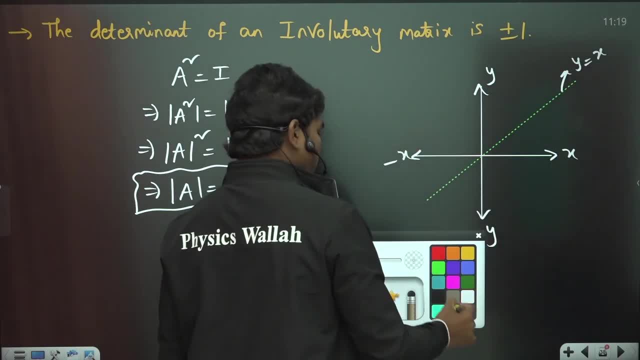 minus Y, and let us suppose this is the minus Y, and let us suppose this is the line. Y is equal to X. now, let us suppose line Y is equal to X. now, let us suppose line Y is equal to X. now, let us suppose you have taken a point a, comma B, for 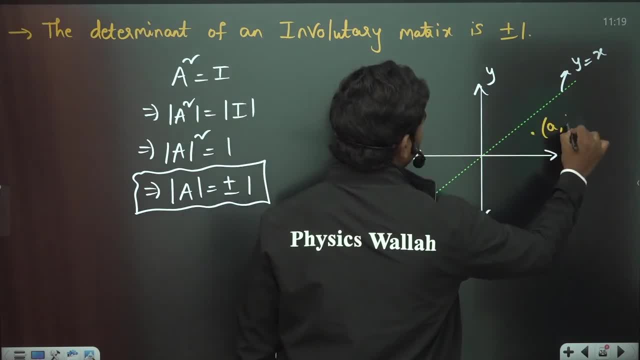 you have taken a point a, comma B. for you have taken a point a comma B, for example, here, a comma B. now, let us example here a comma B. now, let us suppose this point: if you, if this, you suppose this point. if you, if this, you suppose this point. if you, if this, you know coordinates, if you write as a: 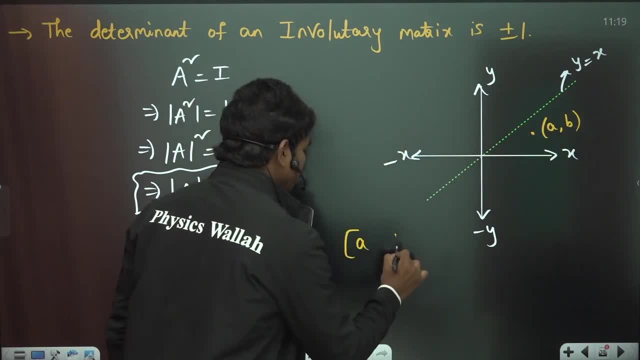 know coordinates if you write as a, know coordinates if you write as a matrix form- a, B, for example, a B. let us matrix form a, B, for example a B. let us matrix form a B, for example a B. let us suppose you have written like this now: 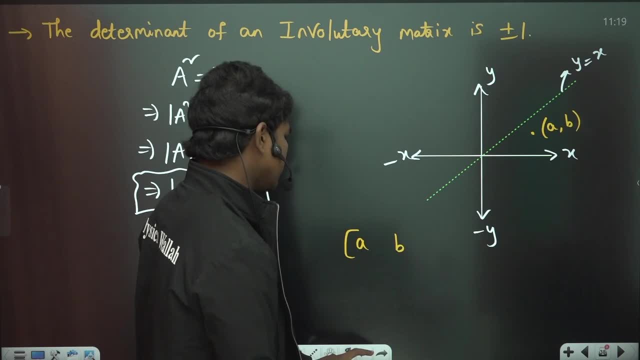 suppose you have written like this now. suppose you have written like this: now, try to understand one thing. or you write: try to understand one thing, or you write: try to understand one thing, or you write this as a B, for example, like this in the. this as a B, for example, like this in the. 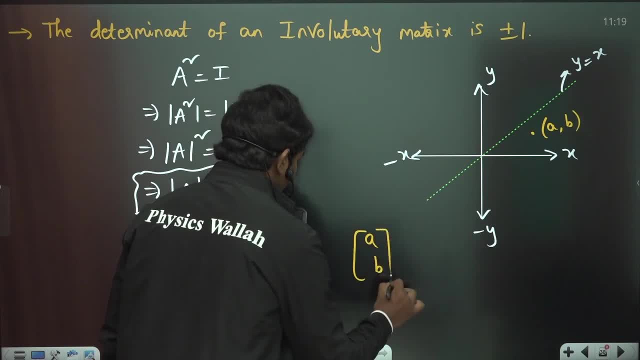 this as a B, for example, like this in the vertical space: a B like this. you at this vertical space. a B like this. you at this vertical space. a B like this. you at this point now. let us suppose if you want to point now. let us suppose if you want to. 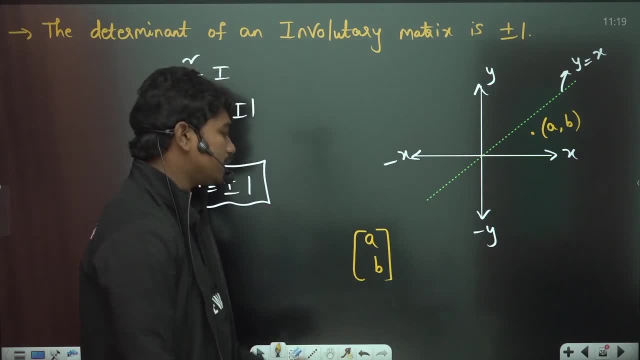 point. now, let us suppose, if you want to find a matrix which, when you multiply to find a matrix which, when you multiply to find a matrix which, when you multiply to this matrix, let us suppose there is some this matrix. let us suppose there is some this matrix. let us suppose there is some matrix here. for example, if you multiply, 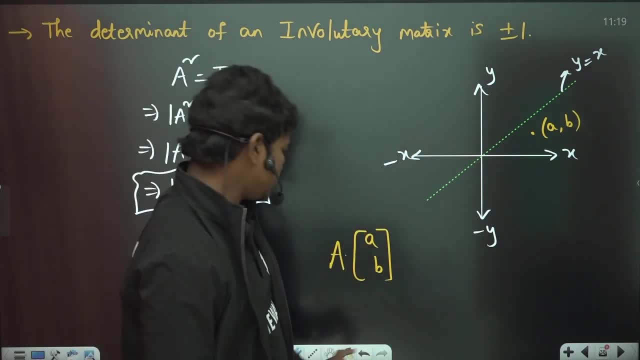 matrix here, for example, if you multiply matrix here, for example, if you multiply this matrix here to this matrix, let us this matrix here to this matrix, let us this matrix here to this matrix. let us suppose your intention is to find the. suppose your intention is to find the. 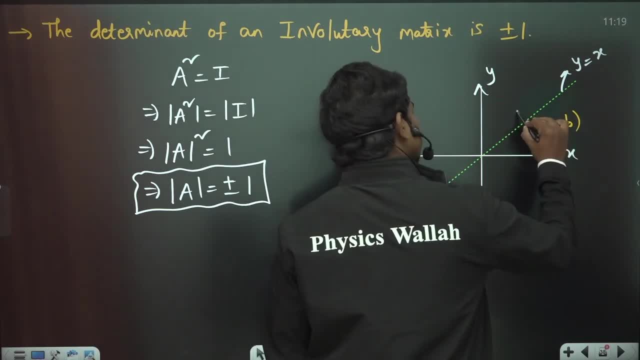 suppose your intention is to find the reflection of this point. to find the reflection of this point. to find the reflection of this point. to find the reflection about this. line Y is equal to reflection about this. line Y is equal to reflection about this. line Y is equal to X. okay, so you want to find this. 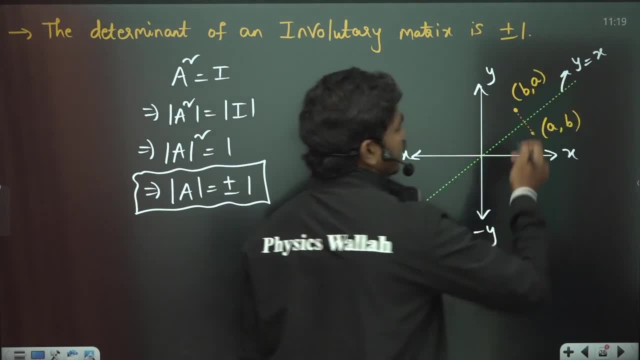 X. okay. so you want to find this X okay. so you want to find this reflection point and you know this reflection point and you know this reflection point and you know this reflection point is going to be become a reflection point, is going to be become a reflection point, is going to be become a example, because if take midpoint and all, 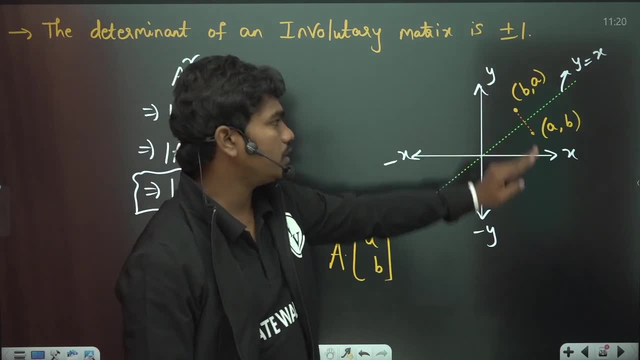 example, because if take midpoint and all example, because if take midpoint and all but you know product of slopes and all but you know product of slopes and all but you know product of slopes and all, you will get this point become a very. you will get this point become a very. 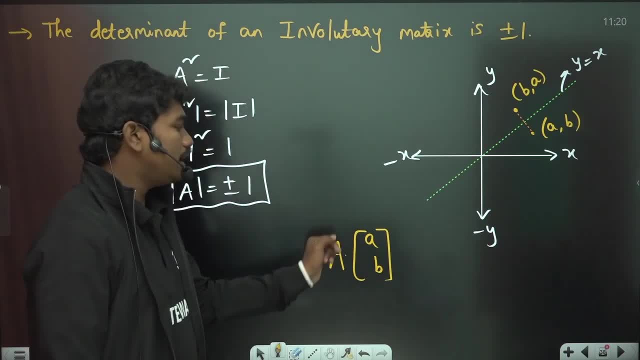 you will get this point become a very easily fine, okay now, what matrix a. when easily fine: okay now, what matrix a. when easily fine, okay now, what matrix a. when you multiply with this economy, will you multiply with this economy. will you multiply with this economy will transform this point as a reflection of 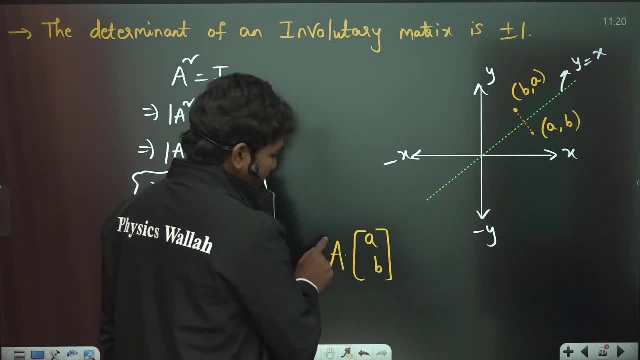 transform this point as a reflection of. transform this point as a reflection of this given point means basically, if you this given point means basically, if you this given point means basically, if you see if you multiply a matrix a to this, see if you multiply a matrix a to this. 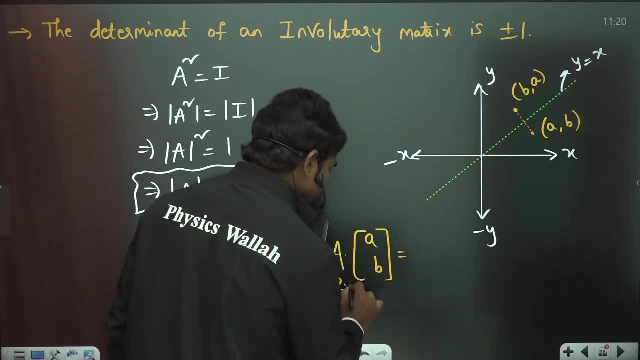 see, if you multiply a matrix a to this, you will definitely get. let us suppose you will definitely get. let us suppose you will definitely get. let us suppose this is size 2 by 2. this is size 2 by 1. this is size 2 by 2. this is size 2 by 1. 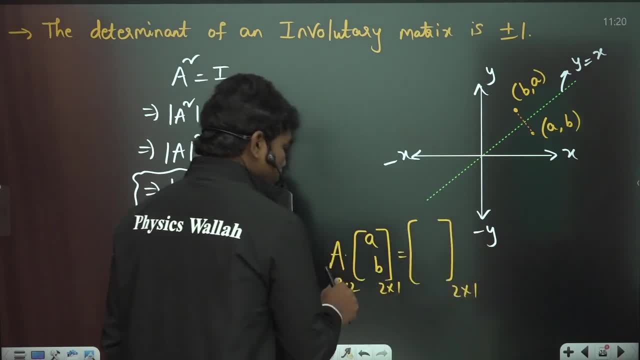 this is size 2 by 2. this is size 2 by 1. you will definitely get 2 by 1 matrix. you will definitely get 2 by 1 matrix. you will definitely get 2 by 1 matrix here. this much you know. but what matrix? 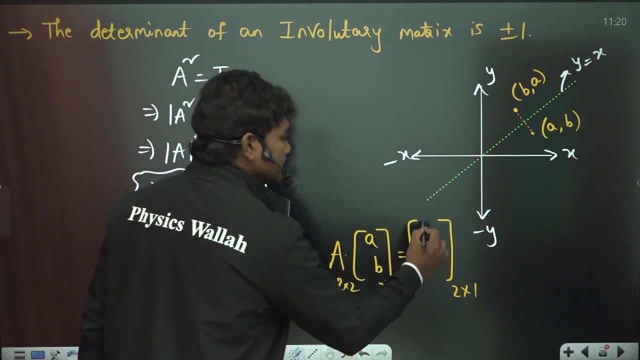 here, this much you know. but what matrix here, this much you know. but what matrix a can make this coordinates a comma B to here, this much you know. but what matrix a can make this coordinates a comma B. to get swapped means be a, so these. get swapped means be a, so these. 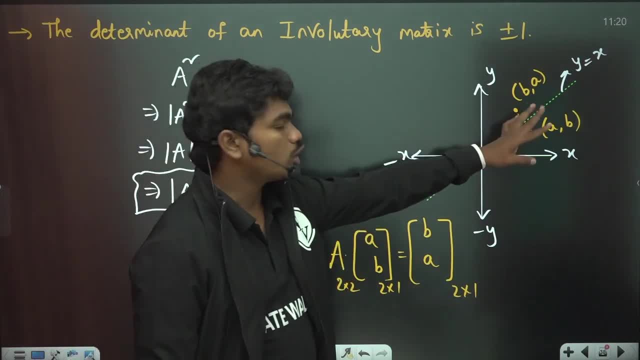 get swapped means be a. so these matrices, might this matrix multiplication matrices, might this matrix multiplication matrices, might this matrix multiplication is actually in geometric sense, what is actually in geometric sense, what is actually in geometric sense, what it's doing? it's basically reflecting the it's doing. it's basically reflecting the. 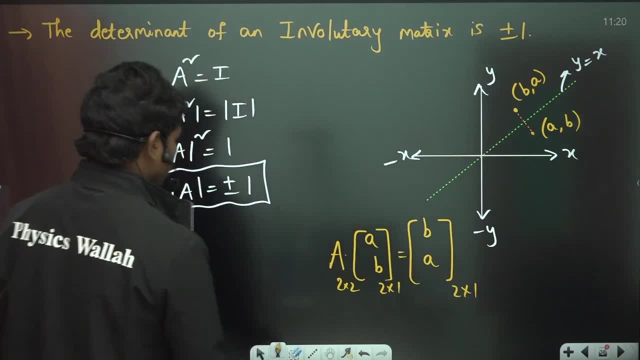 it's doing? it's basically reflecting the point now, what is this point? what is point now? what is this point? what is point now? what is this point? what is this matrix a? let us try to understand this matrix a. let us try to understand this matrix a. let us try to understand. okay, let a is equal to let a is equal. 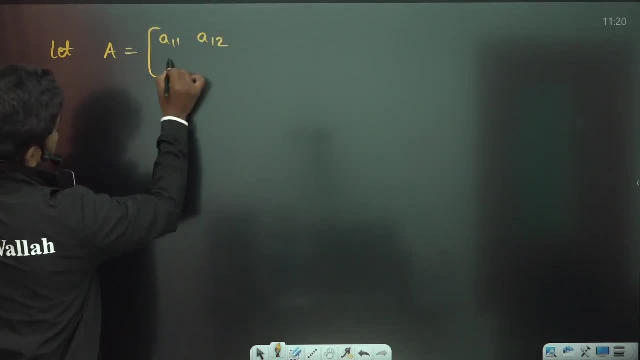 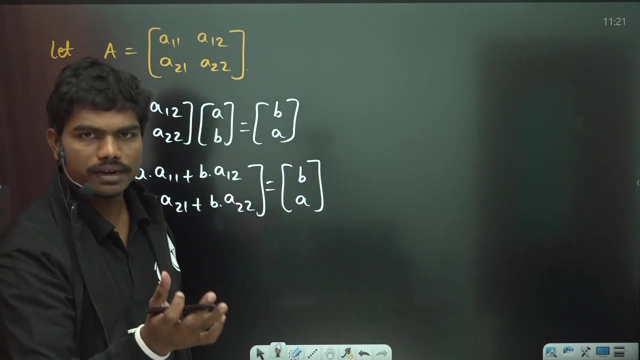 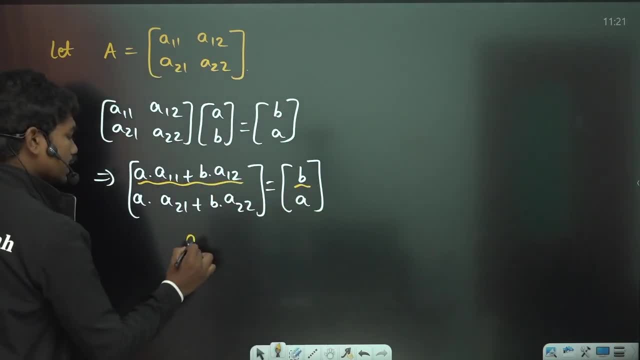 This first element. with this first element, you can easily understand: a 1- 1 value is 0 and a 1- 2 value is 1. Similarly, if you equate this element with this element, You will come to know a 2- 1 is equal to 1 and a 2- 2 is equal to 0. 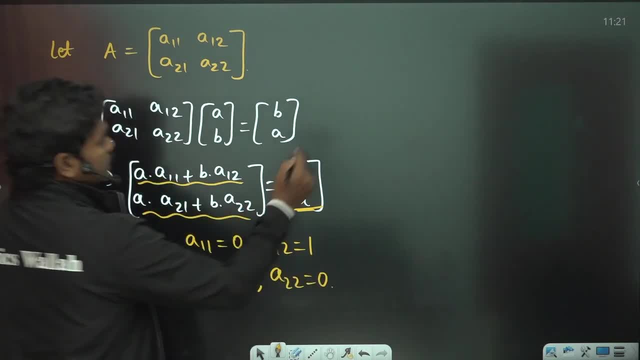 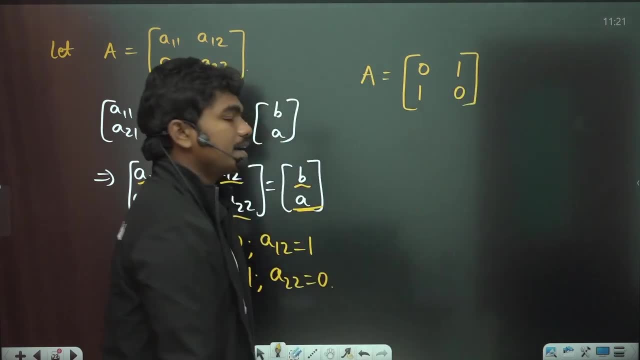 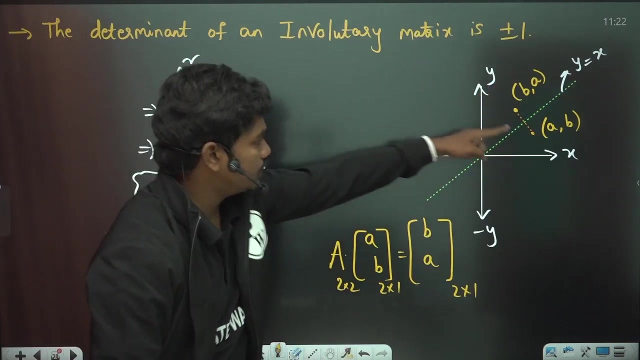 So if you form this, if you replace these values in this matrix, you will get a is equal to 0, 1, 1, 0. So basically, this is the matrix which can transform. this point. means you can see, this Point can be transformed as its reflection. if this coordinates are multiplied with this particular matrix, which is given by 0, 1, 1, 0, 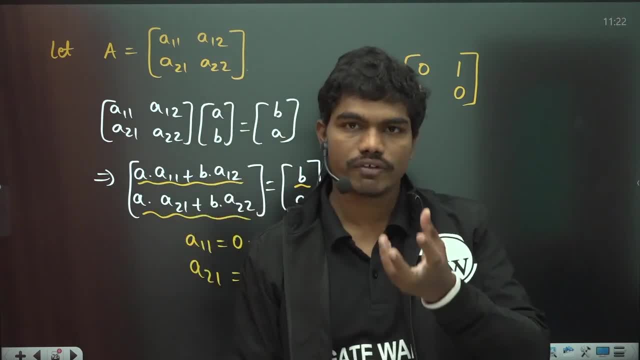 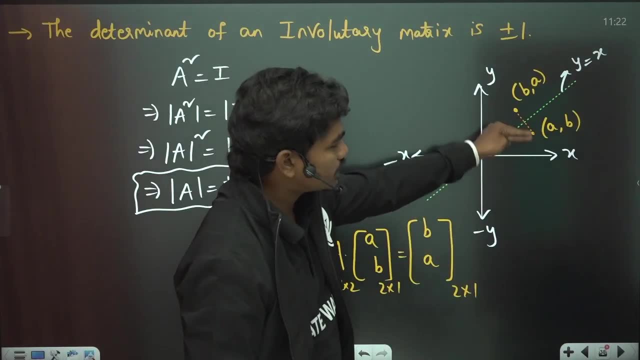 so this is how matrix multiplication is actually transformation of some given matrices with respect to the Your interest, your point of interest. you see, something I have, my I might have done is a reflection about x-axis or something like that, Or a reflection about y-axis. I would have done anything. 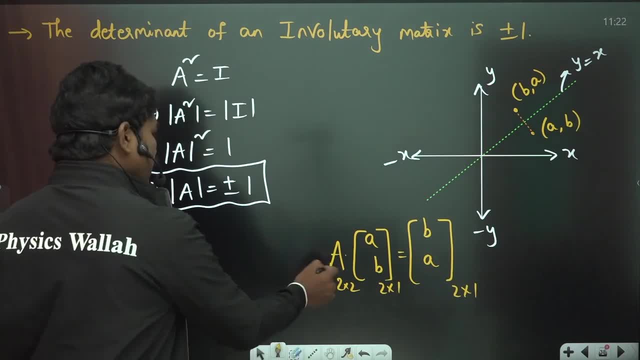 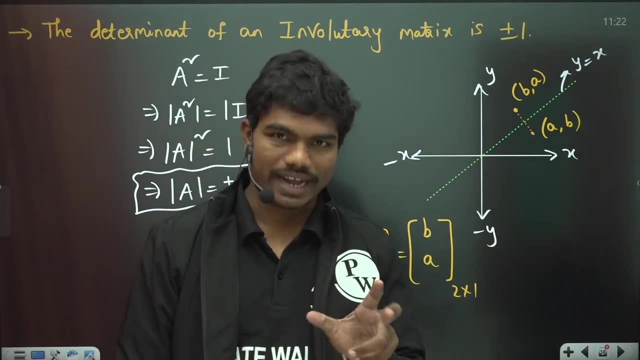 Okay, so these coordinates, this matrices, decide how these points gets transformed. similarly, have You know, in plus 1 or plus 2, You might have gone to something called transformation of axis. Okay, So, this cos theta, minus sine theta, sine theta, cos theta. if you see, if you multiply that matrix to a point, 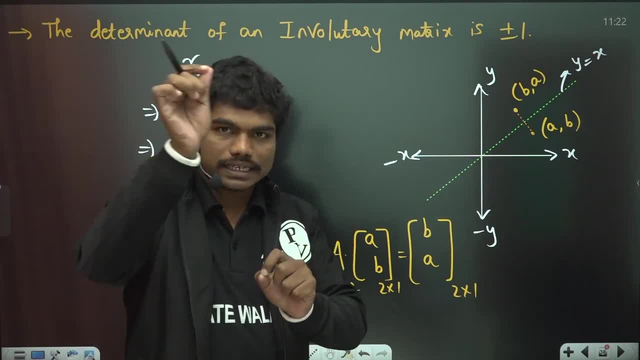 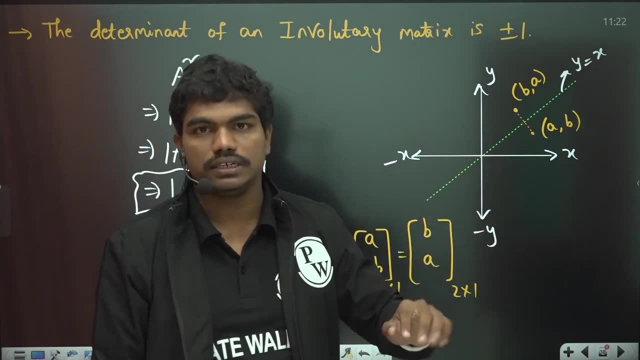 You will get some other values of x, comma, y. So if you evolve the axis by some theta degrees, then the new coordinates are given by this transformation matrix cos theta, minus sine theta, sine Theta, cos theta. you know, you have learned these things. This is the actual meaning of multiplications. now why I have talked about this. 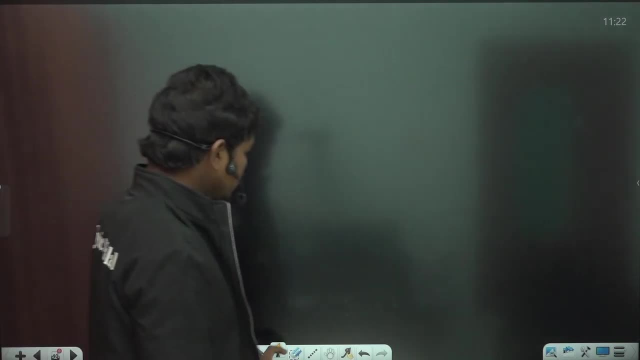 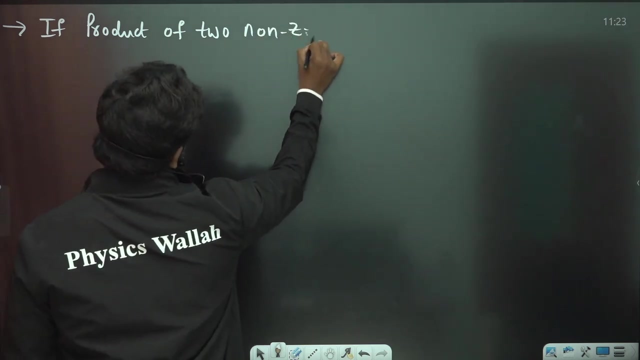 Because again next property, I am going to talk about this multiplication, masasa, gradient transformation. Make sure youeu've drawn someiter And make sure you have got all the. you know there are some addition and subtraction ubiquity in this Lipma of matrices. look if product of 2 non zero matrices. 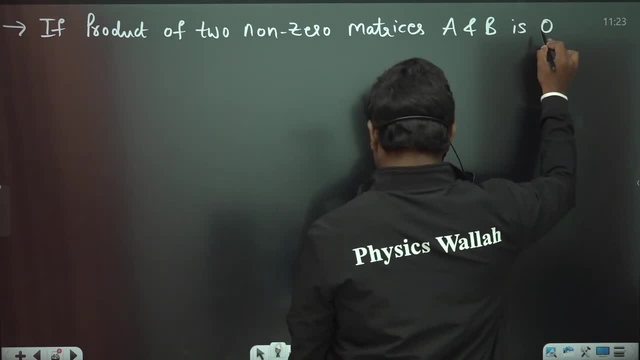 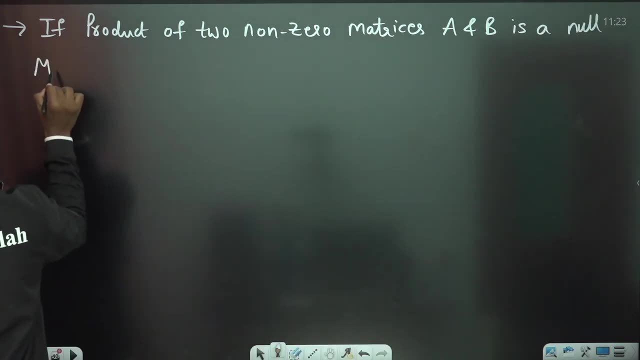 If product of To non-zero matrices, if product of two non-zero Matt is us a- a null matrix, if product of two non-zero matrices, a and b, is a null matrix, for example, then what happens? basically, that a is equal to zero and that b should also be equal to zero. look. 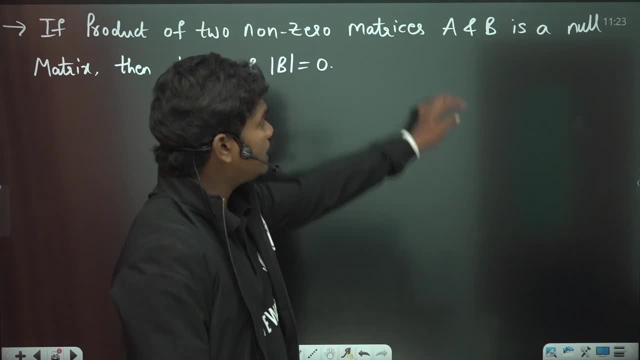 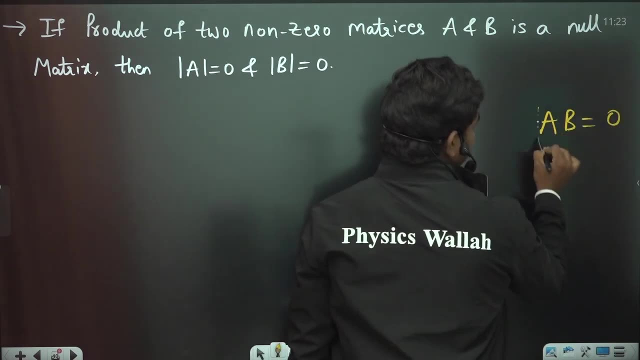 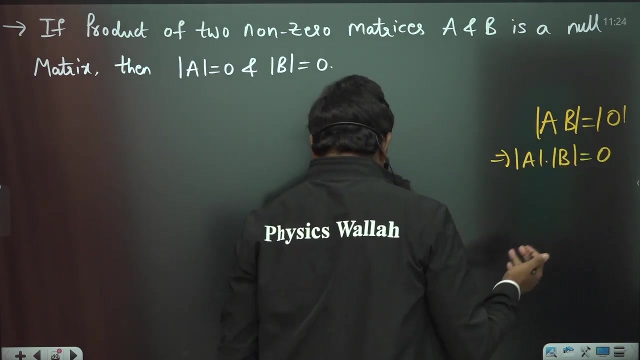 normally. i'll tell you one thing: many of you may feel that if a and b are non-zero matrices- but let us suppose if a, b is equal to zero, whenever a, b is equal to zero, if you apply determinant on both sides, you know that that a into that b is equal to zero. so by scalar equation you may feel. 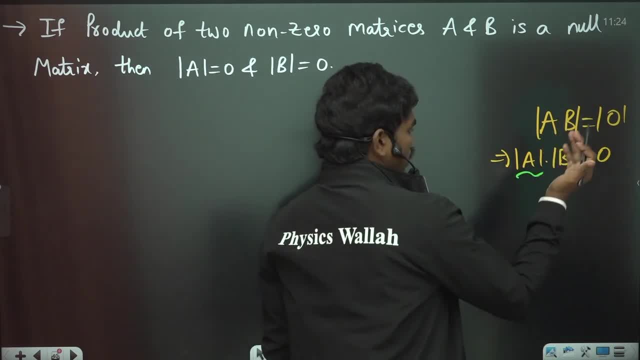 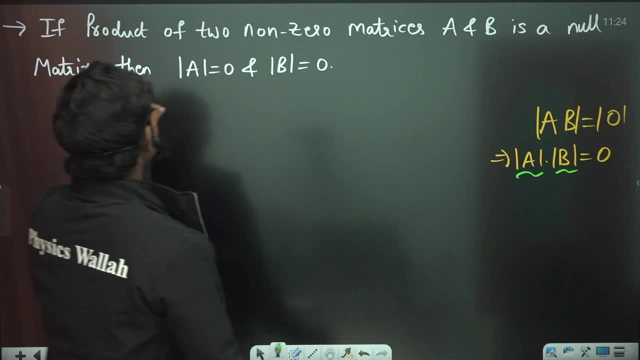 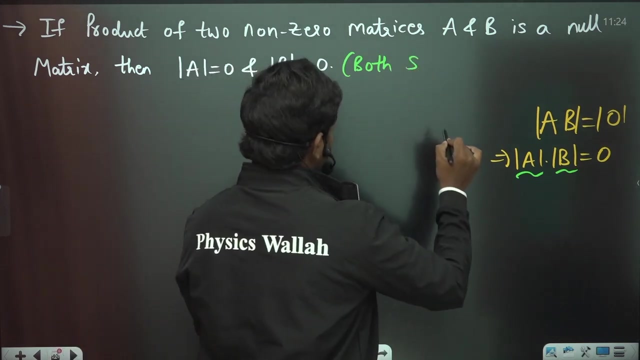 that if one of these two, if that a is zero or if that b is equal to zero, then this equation holds good. but actually if some case like this happens, then both you can write, then both should be singular matrices. both matrices should be singular. both matrices should be. 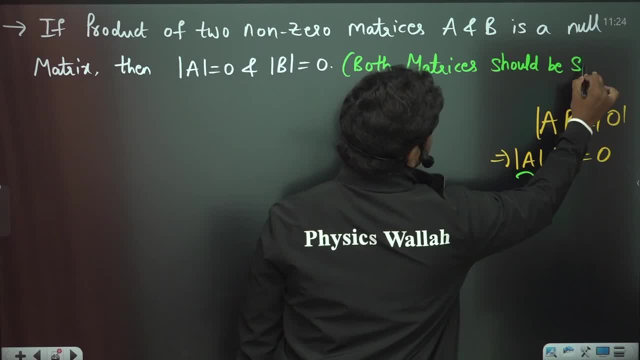 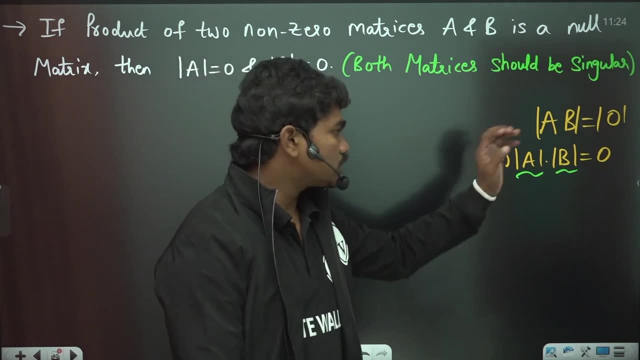 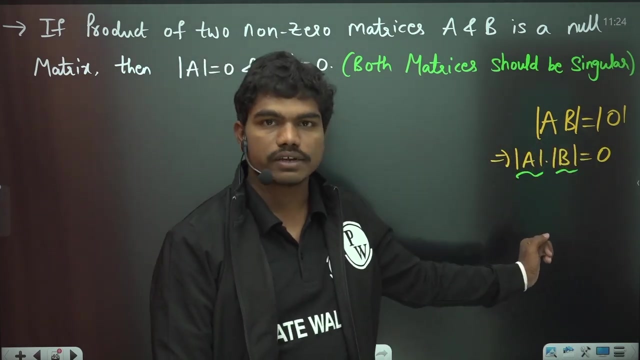 you both matrices should be singular, okay. so this is one very important point why i'll show you now: okay, because in we have a previous year gate question also like this: they'll give you that a equal to zero, that b not equal to zero, that a is not equal to zero, that b equal to zero. such options and our intuition: 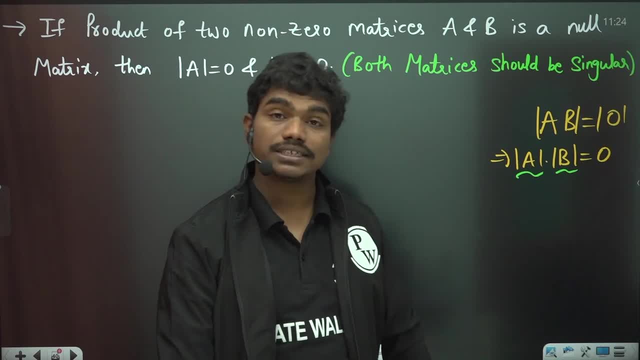 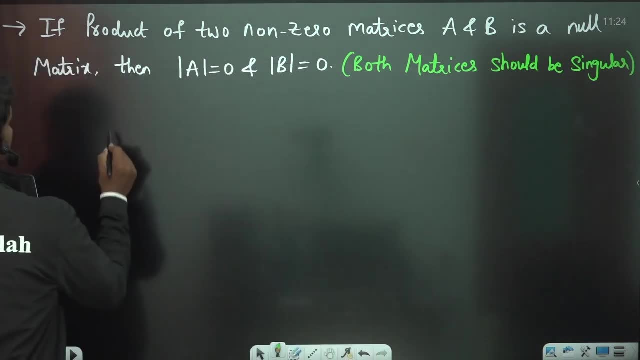 tells that, what if one of them is zero? that's good enough, but actually both has to be zero. why? i'll tell you now, look, we'll delete this. now see here why both has to be zero. look, let that a is equal to zero and that b not equal to zero, for example. okay, let us suppose this: 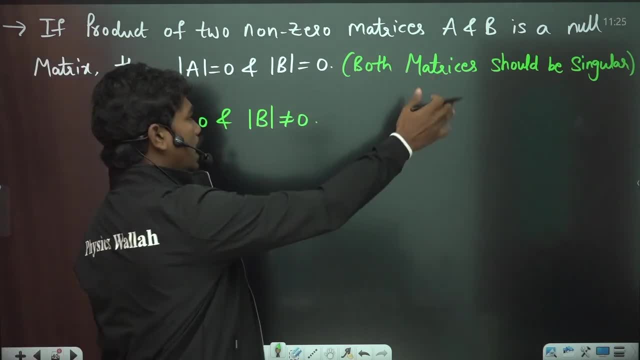 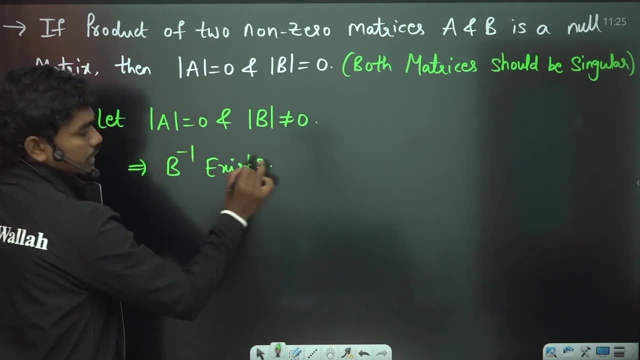 happened. one of this is zero. so that again a into b, you have zero. so this immediately tells you that b? inverse exist, b inverse exist. that means if that a is equal to zero and that b not equal to zero, then definitely you know b? inverse exist. so if you take this: a, b is equal to zero. and if you 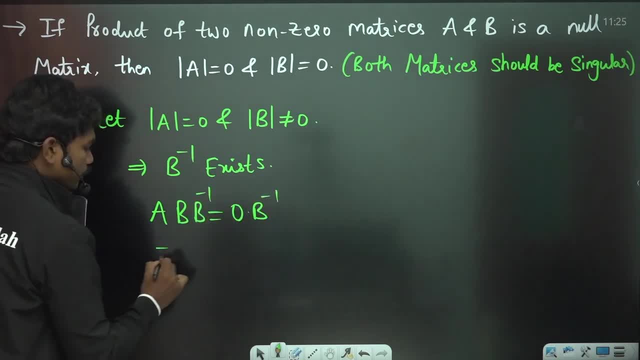 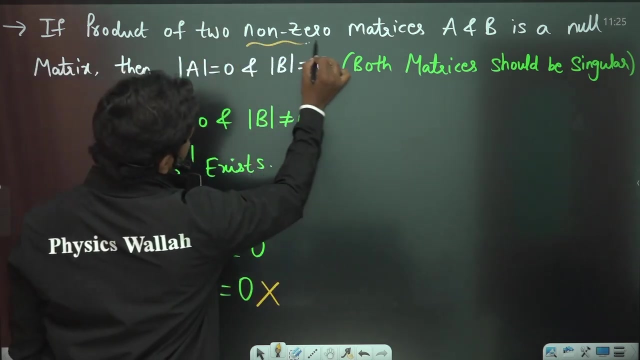 multiply with this b inverse, then you will get one thing: this b into b inverse is i. so a into i is equal to zero matrix, because zero into something, it is zero. this is given, which is a is equal to zero, which is actually wrong as per our assumption that two non-zero matrices, so a and b, should be. 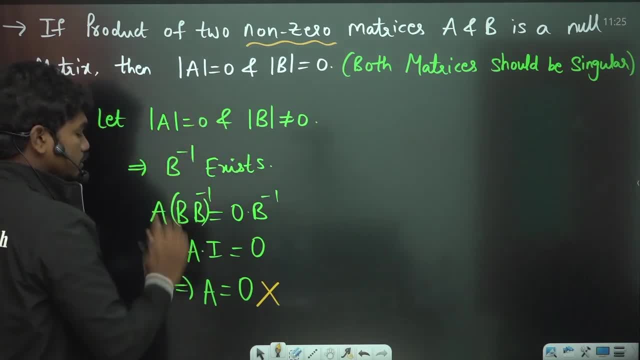 non-zero matrices. but if you feel that that b is not equal to zero, you are trying to understand that a is zero, which is actually contradiction to our take intake that both a and b are non-zero matrices. so that's why, similarly, if you take that a not equal to zero and that b equal to 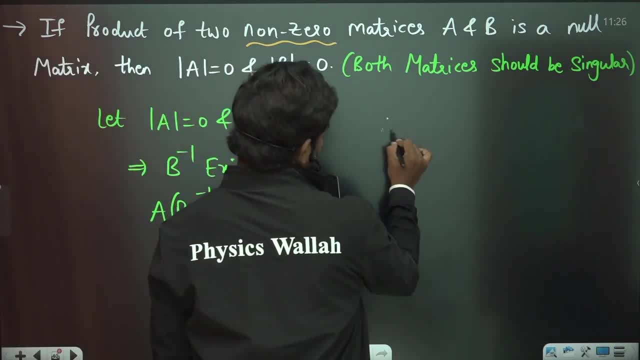 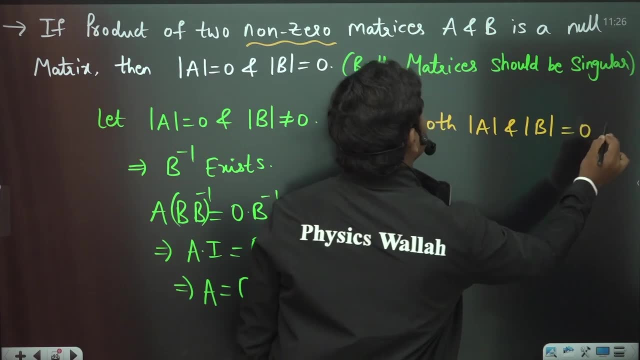 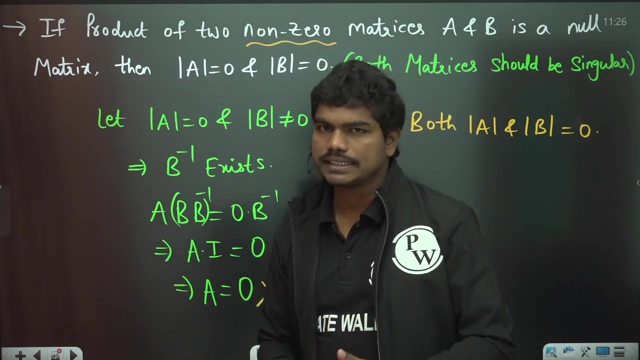 zero, you will find out b equal to zero, okay, so therefore, both that a and that b should be equal to zero, okay, so this is one very, very important property again in determinants, basically because many times they- you know, they- keep some questions around this for you, so that's the reason why it's. 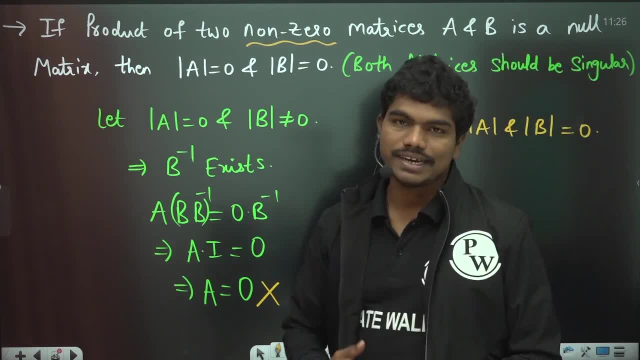 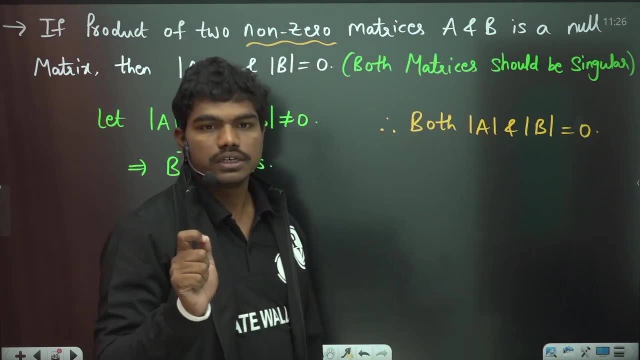 one very important property: the product of two non-zero matrices, a and b. if it's a zero matrix, then both the matrices should be definitely singular matrices. okay, both the determinant should be zero clear. so please make a note of these things very soon when we come to. 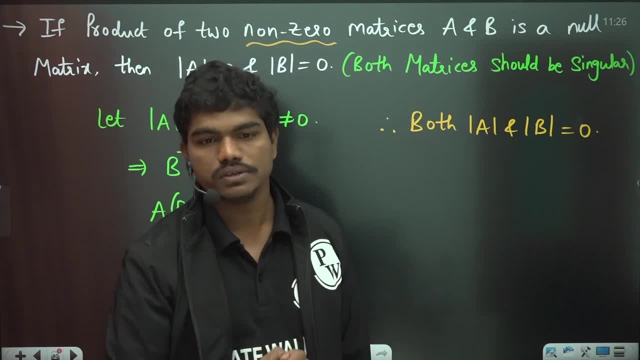 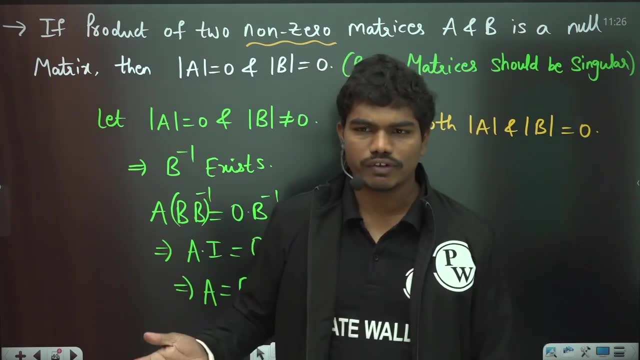 the practice questions session or something like that. it will be very helpful for you. okay so, and majority you can, you might be having some pyqs with you by this time. so once attending this lecture of four to five hours, almost, you can definitely solve almost some 95 percent of the. 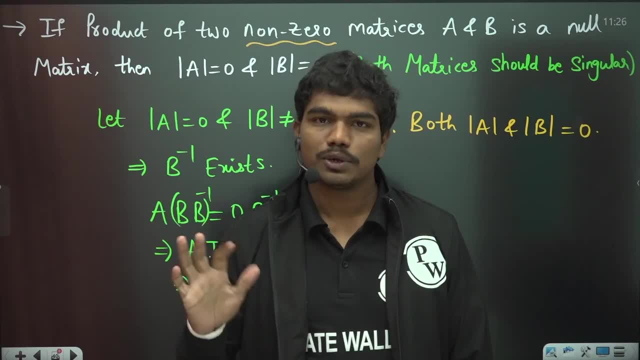 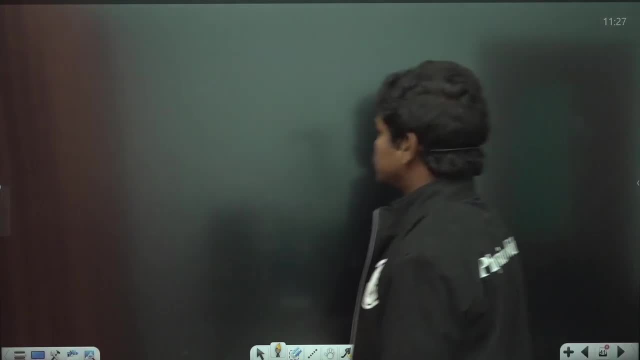 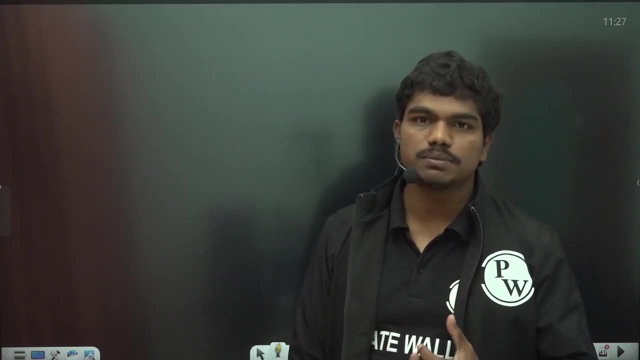 questions in engineering maths, i mean in linear algebra. okay, don't worry, remaining five percent of the questions are going to be very useful, okay, so let us continue. let us continue here. so i would like to talk about one very important uh, you know, uh, value, actually, value of one determinant at this. 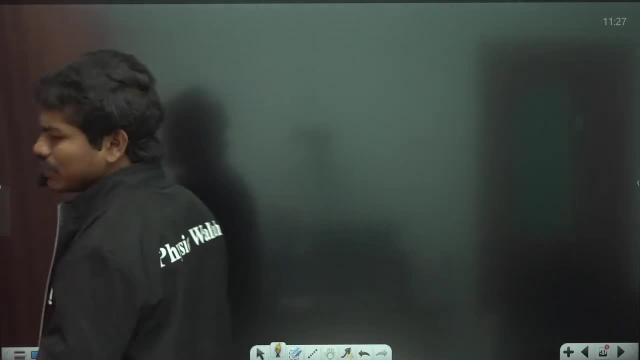 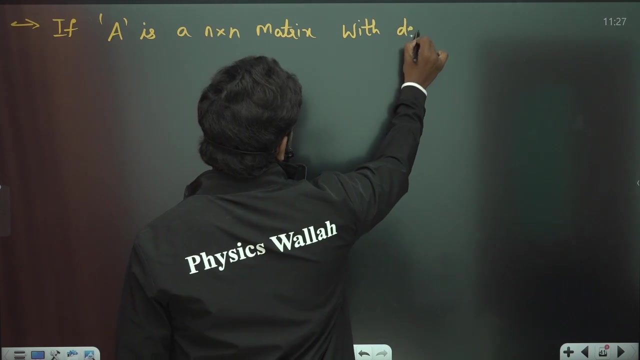 moment, moment, okay. so i'll also give you some technique, uh, for writing okay the things. if i any writing any three by three determinant easily, okay, look. so see here: let us suppose if a is a, n by n matrix, n by n matrix with determinant, with determinant as that, a with the determinant as 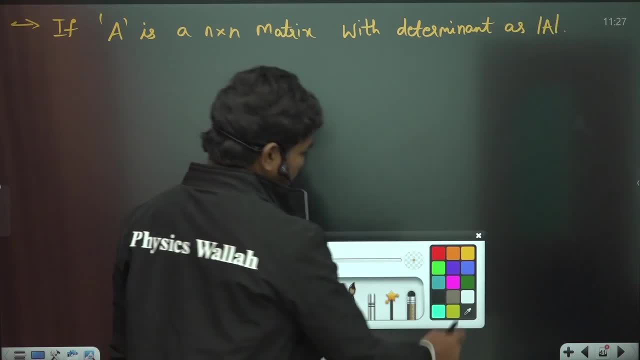 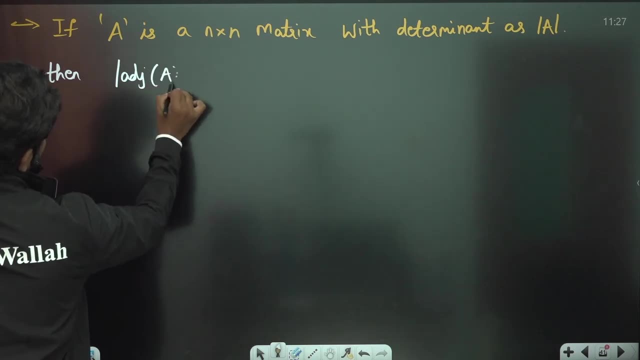 that a, for example. let us suppose: if this is that a, then that of adjoint of a is how much? so many times what they do? they don't give you the actual matrix. if they don't give you actual matrix, then you cannot calculate the adjoint. but they'll ask. 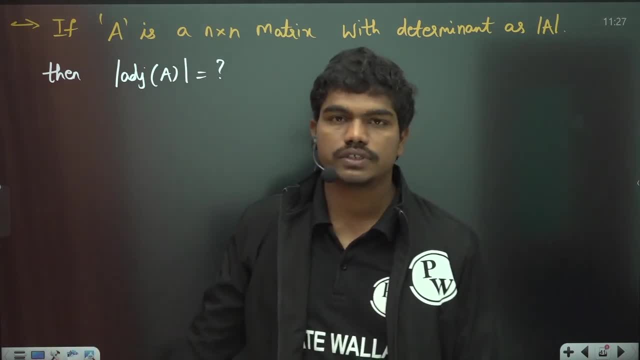 you about that of adjoint a, and this question is one very, very, very famous question in you know uh gate domain. so let us see here: if a is a, n by n matrix with determinant as that a, then what is the determinant of a joint of here? basically, 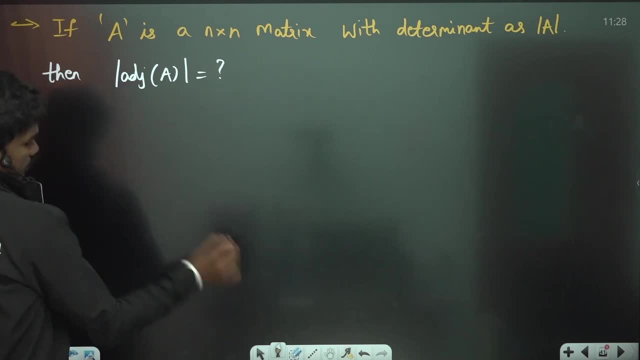 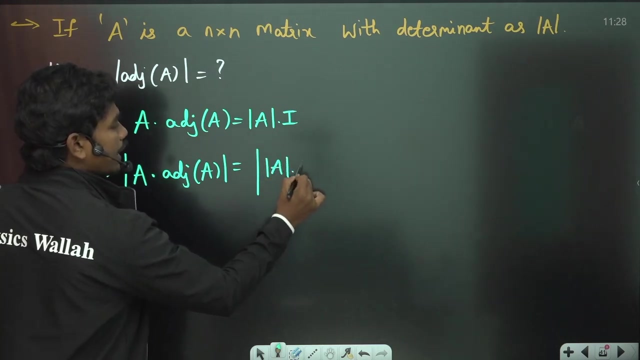 look, i'll tell you. we have this equation, that fundamental equation, that a into adjoint of a is equal to that a into. i correct. you have this equation now. if you apply determinant on both sides, that of a into adjoint of a is equal to that of that a times. i now try to understand one thing: this is product of. 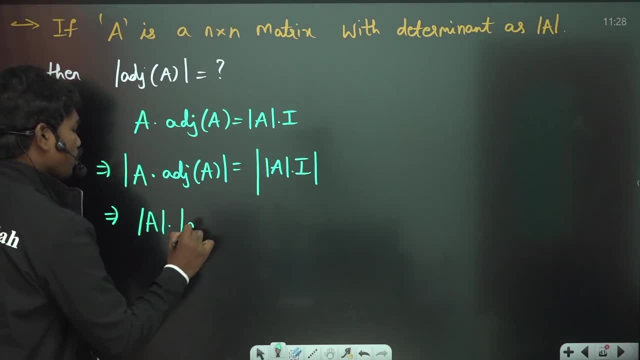 two matrices so i can split it- that a times that of adjoint a is equal to now this: that a is again some number. so and if a is of size n by n, this i is also of size n by n. so if you want to take this, that a out as a constant, out of this, 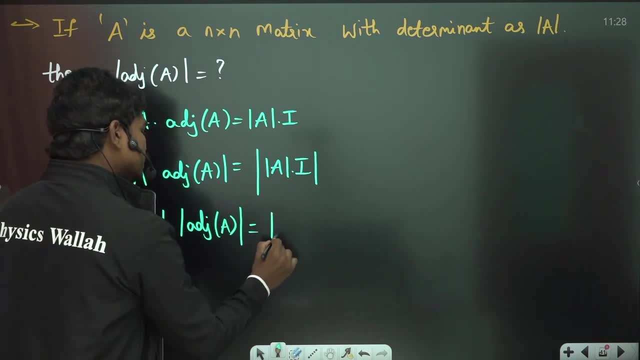 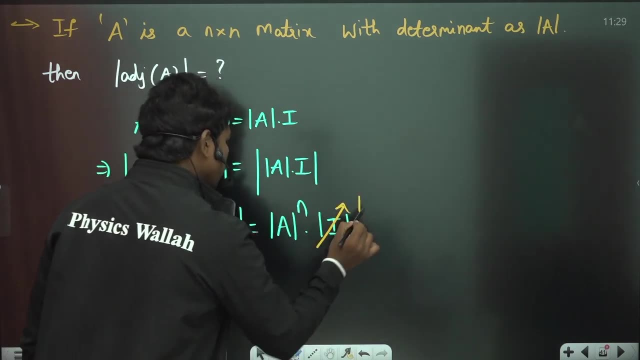 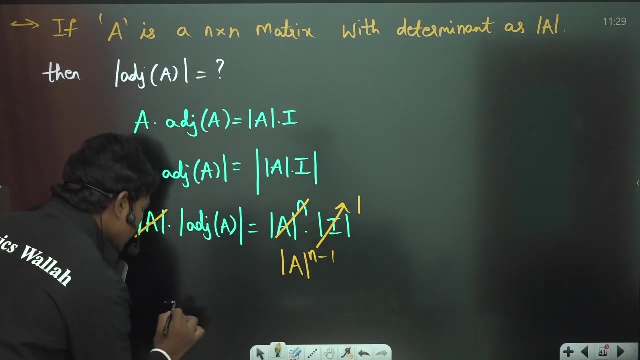 determinant, then you know, since this i is a n by n matrix, this turns out to be that a whole power i n times determinant of i. now you know one thing: this determinant of i value is actually one. so you can cancel that a some n minus one times, get a power n minus one. so therefore you can understand. 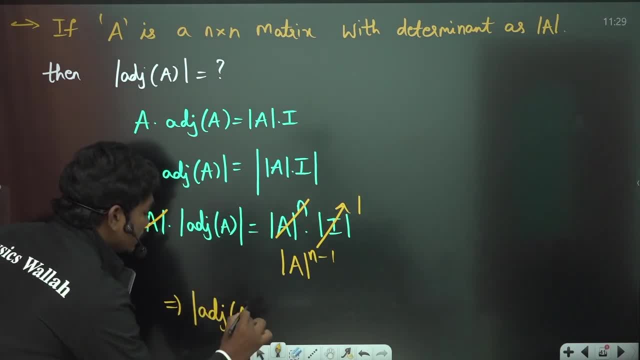 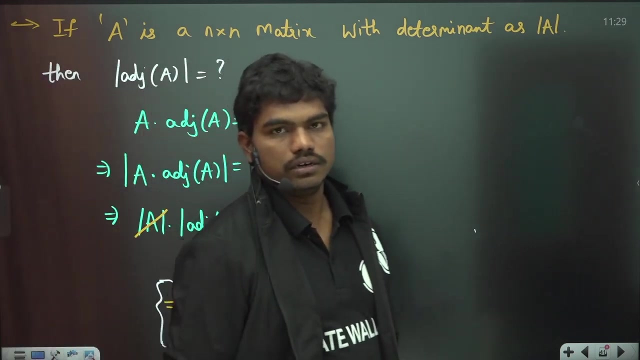 one thing, that of a joint a is how much that a whole power n minus one. so this result is one very, very important result for gate examination. okay, many times you see you could you'll find a from this uh, that you know, from this actual equation. okay, sometimes they go one step ahead. 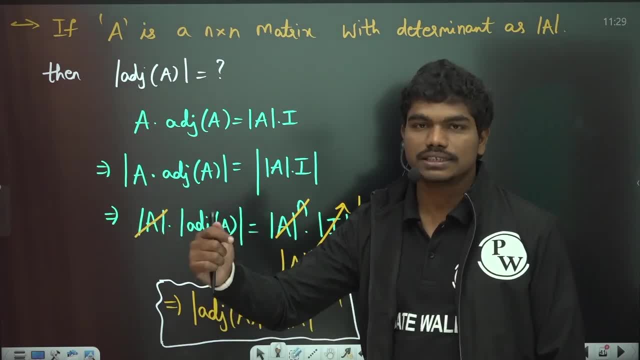 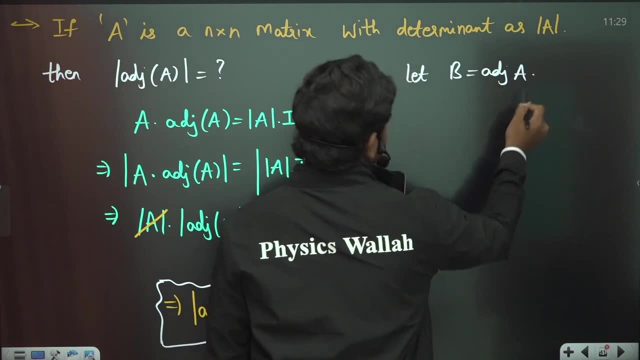 and they'll put one more adjoint here, adjoint of adjoint. here, they'll ask: let us see what is the case. let b is equal to adjoint a, for example. for example, there you have, you have a matrix a, you have calculated its adjoint, so let us consider that matrix as b now, since this b is also a matrix. 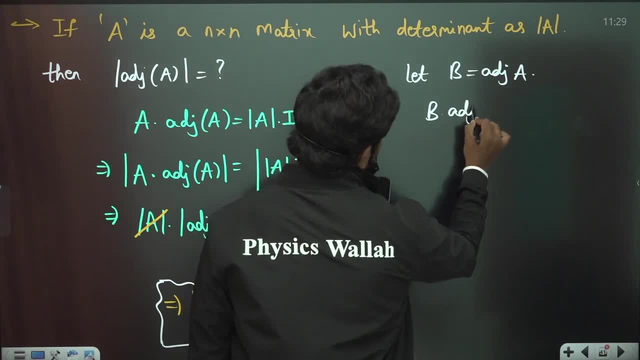 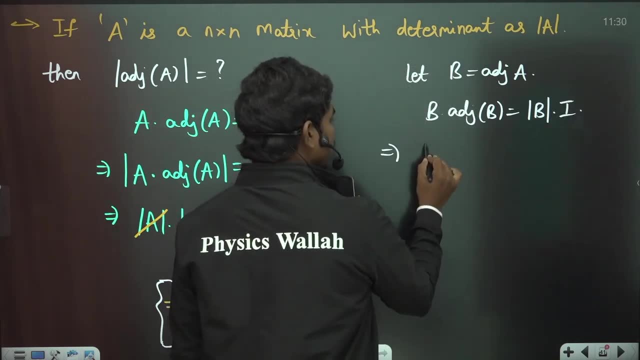 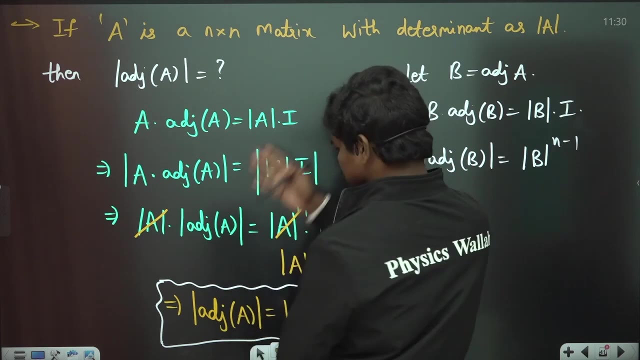 we can write b into adjoint b is nothing but debt b into i. you, i can write this correct. so if you again simplify, you will get: debt of adjoint b is equal to debt b whole power n minus 1. you will get again the same analysis. if you follow, you will get. 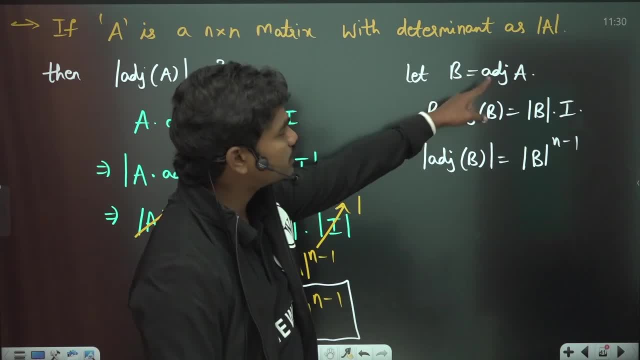 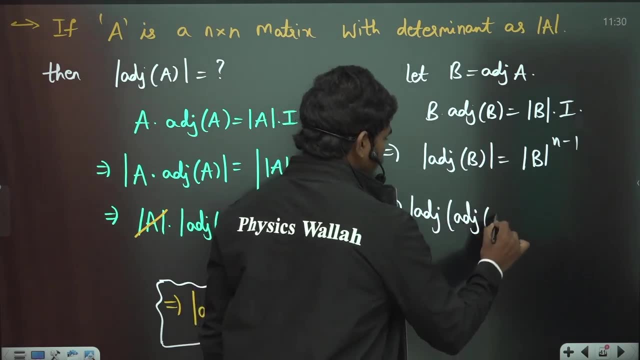 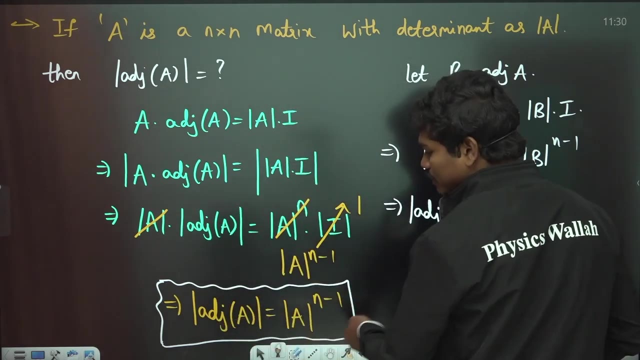 debt of adjoint b is that b whole power n minus 1. now, if you replace b as adjoint a, so this implies debt of adjoint of adjoint a. if you do this then you will get something like this: debt b is nothing but debt of adjoint a, which you have debt a whole power n minus 1 here. so debt a whole power n minus. 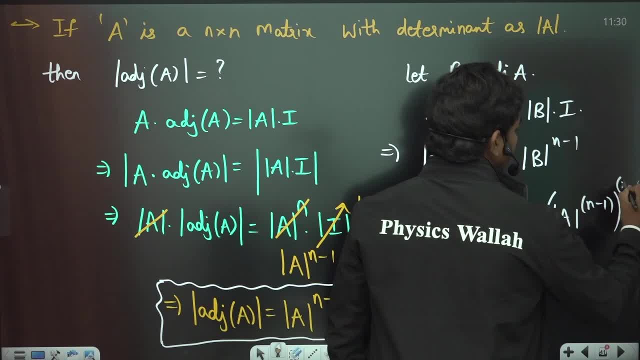 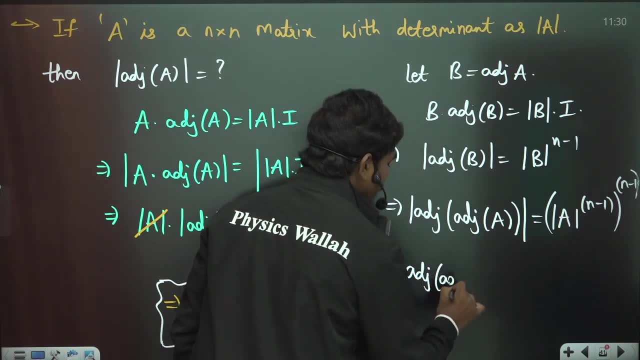 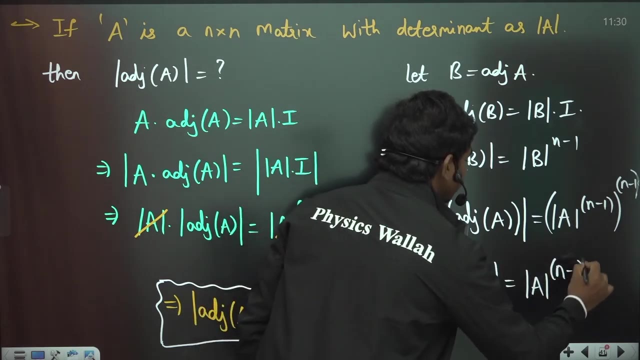 1, this whole power n minus 1. okay. so if you simplify this, you will end up with something like this: adjoint of adjoint a is equal to debt, a whole to the power n minus 1 whole square. okay, so this is how we have this. 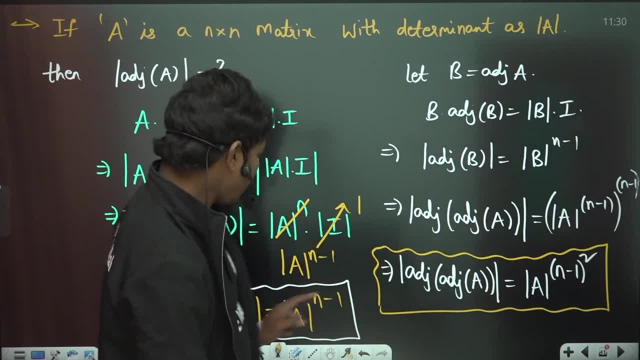 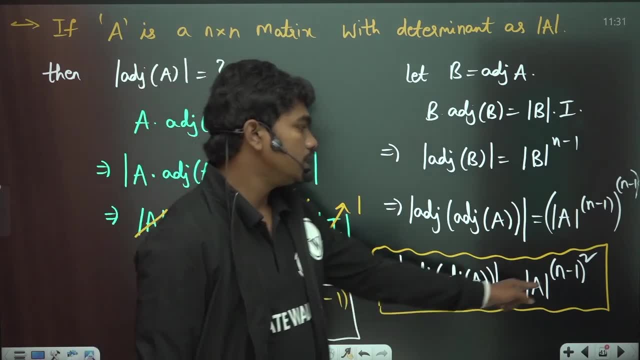 relation. now try to tell me one thing. let us suppose if you have taken one adjoint, you got n minus 1, n minus 1 whole to the power 1. for example you can say: when you took two adjoints, here there is two n minus 1 whole square. can now let us suppose if you put one more adjoint. 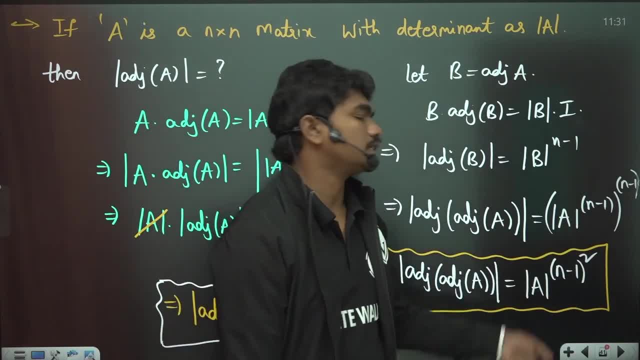 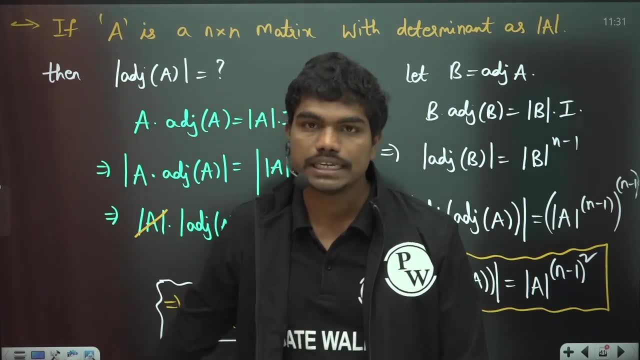 this turns out to be cube. it's a very simple analysis. again, like the same thing: if you follow so many times without giving the actual matrix, and even if they give actual matrix, it takes you so much time to calculate this adjoint a. okay, so that's the reason if you have this uh. 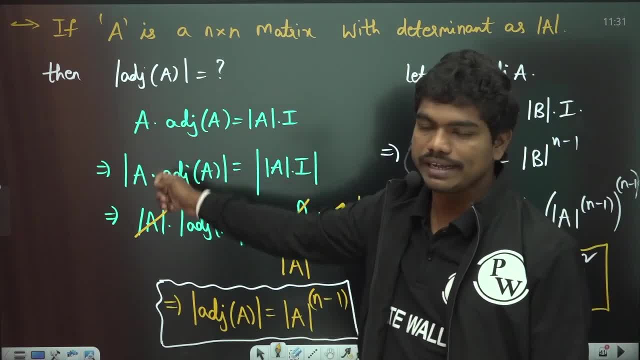 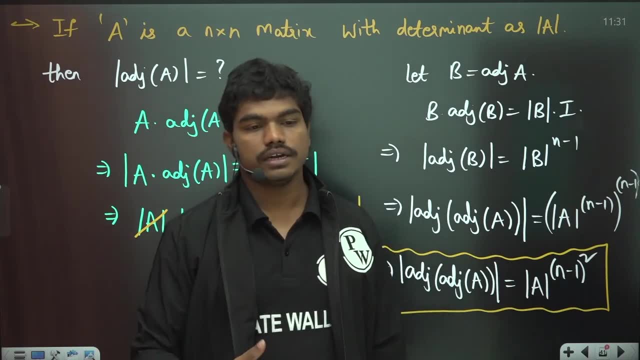 determination of the adjoint a. you can write this as a whole square, okay, so that's the reason you can easily tell. determinant of adjoint a: once you know the size of the matrix means basically: once you know the n value, you can- uh, you know- keep going ahead. for the determinants of the. 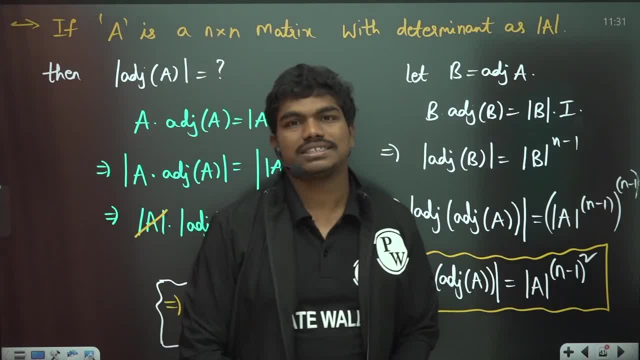 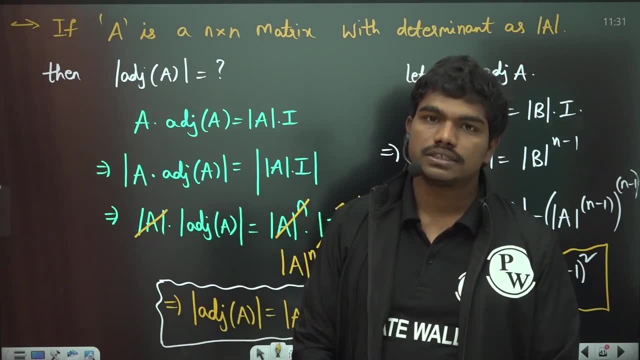 adjoints clear. so these are very much important properties in determinants that i want to talk about at this moment. okay, so i think i have discussed some 9 to 10 properties of determinants, which is again very- uh, you know, good thing. so this determinants are very important, uh, basically for 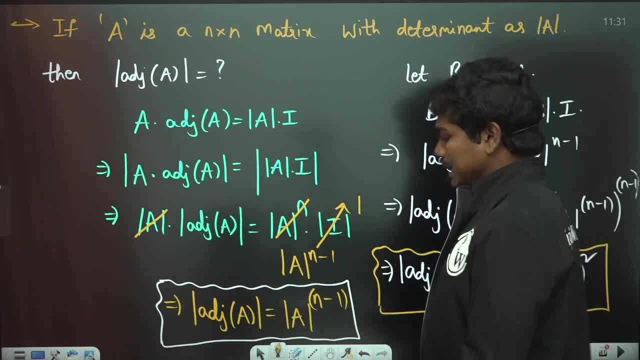 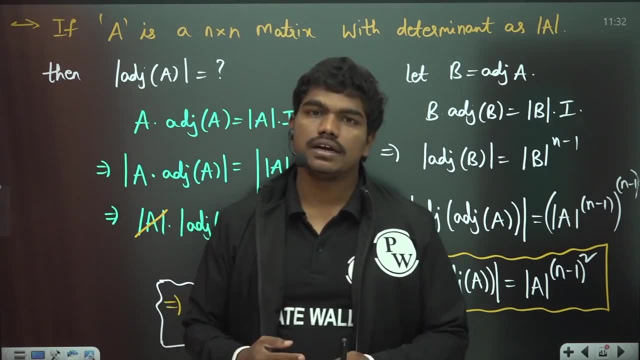 your understanding. okay, so we have seen the determinants of the adjoint a and we have seen all the types. basically here, clear now one thing, uh fine, so this is this. with this we close this second, uh, part of this video which is determinants. okay, so we have seen what is a determinant we have. 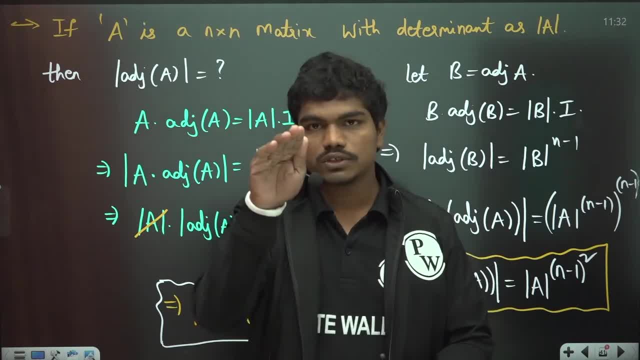 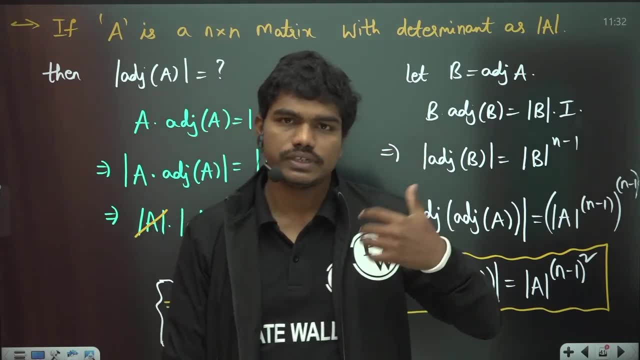 seen, determinant is nothing but the summation of product, of elements of a or column with the corresponding cofactors. okay, so we have seen that and we have seen certain properties of determinants which are very, you know, useful in general examples outside. now let us try to define. 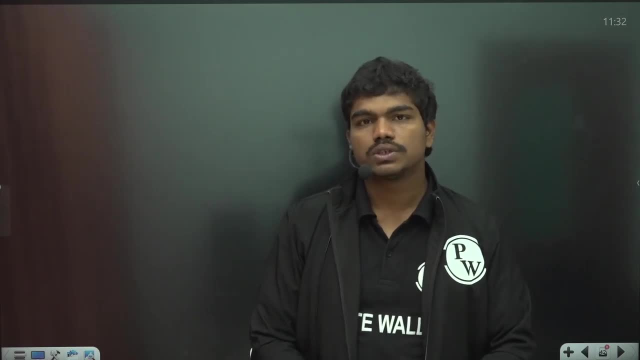 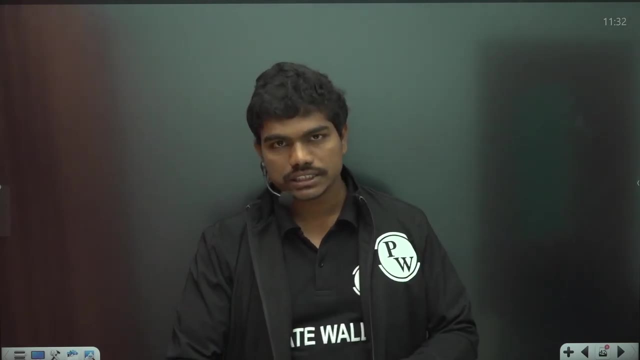 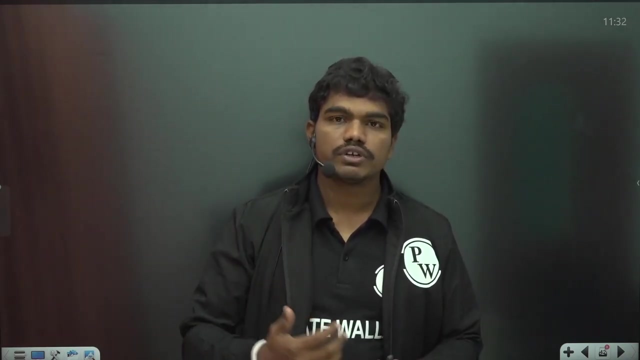 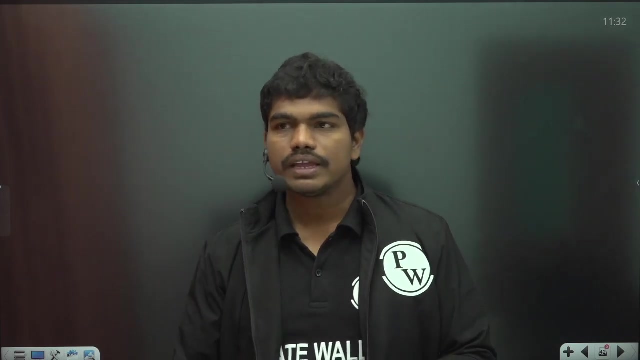 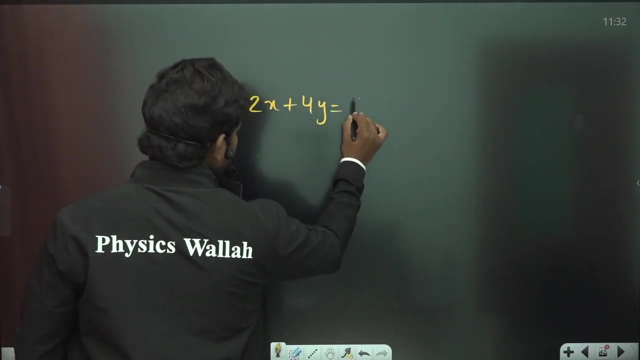 one, uh, the next part of the determinants. okay, so we have seen the determinants of the adjoint a and we have seen certain properties of this, uh, sweat grade here. okay, okay, so, un. so four in crushed X plus two Y is equal to nine. 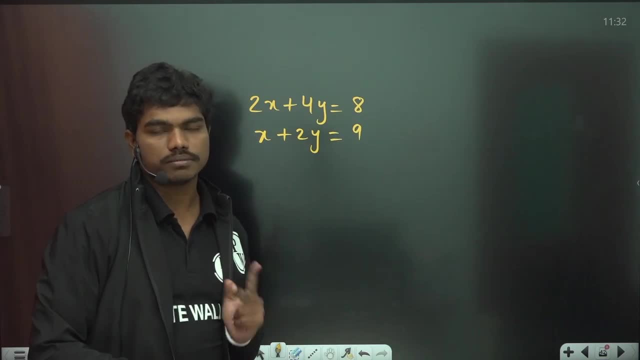 Let us suppose, if I give you these two equations, these are two equations for you, that's it. But actually, without solving, you can tell whether this equation- okay, if you try to solve you'll end up with these equations. don't have any solution. 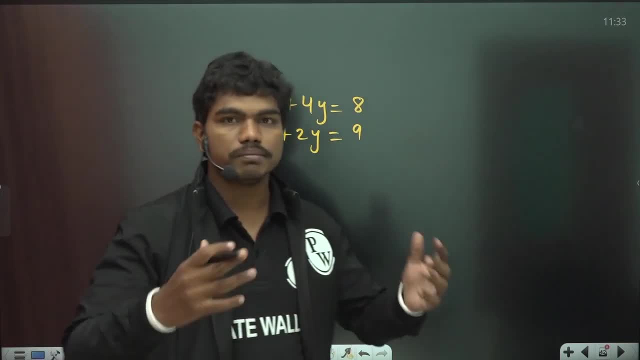 But normally it's a two by two case. it's a simple case. But let us suppose, if I give you some big case, four by four, five by five such cases, you should know some techniques, some mathematical checks to understand whether the given system 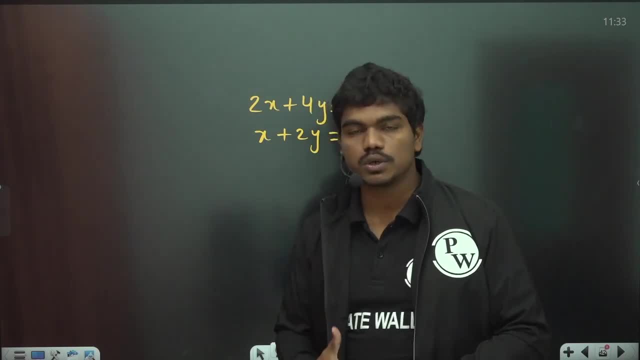 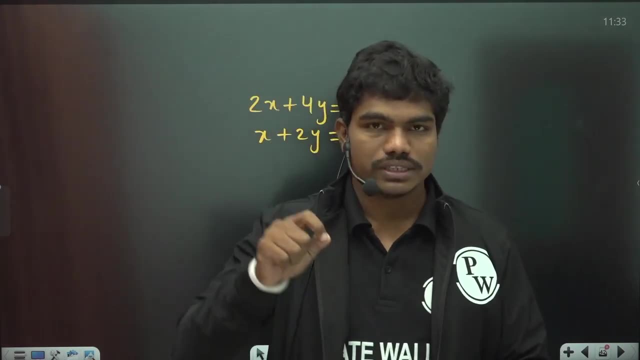 has a solution or not. okay, So that's how we check that. So, for checking that, we will be in need of one very, very important concept, which is called rank of a matrix. okay, So this rank of a matrix is one very important concept. 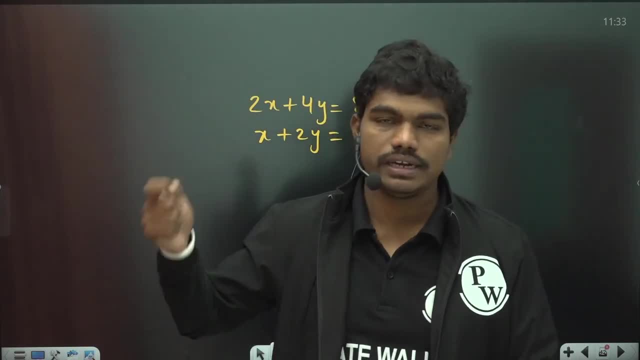 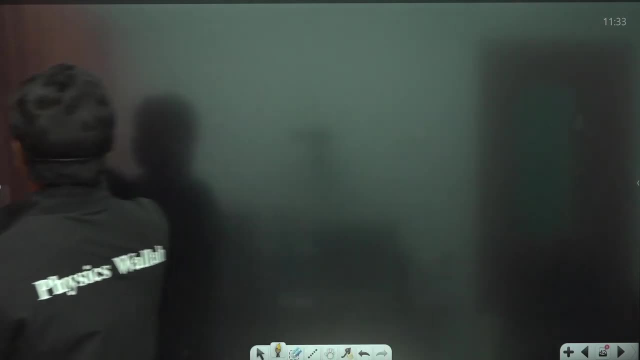 and we'll see the complete system of equations deals around with this rank of the matrix. okay, So let us see how we go ahead here. So let us put a heading rank of a matrix. Rank of a matrix. Rank of a matrix. 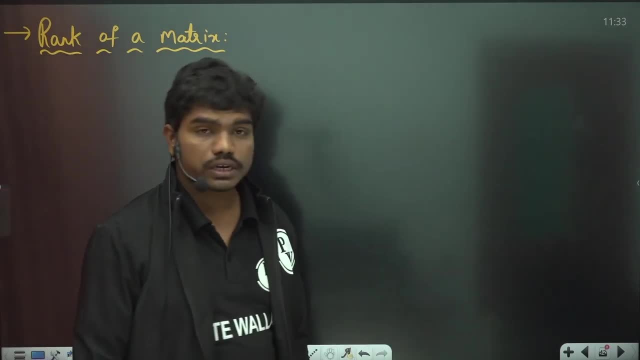 So what is this? rank of a matrix? okay, So this is one very important concept and we all should listen carefully here, okay, So for next 10 minutes, please don't, you know, look anywhere, be focused. So, rank of a matrix. 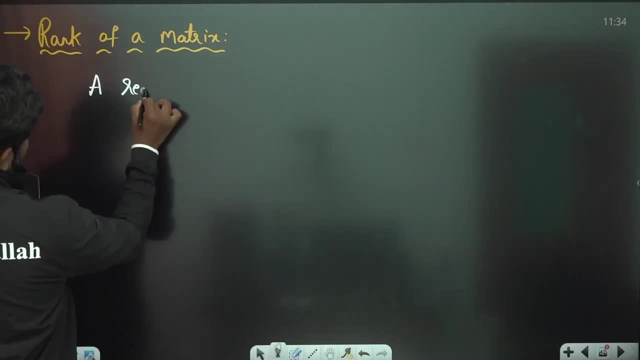 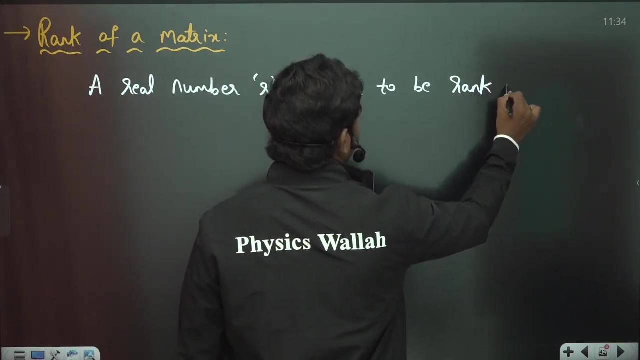 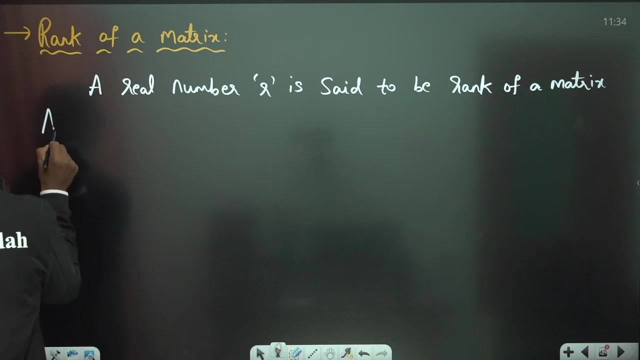 So a real number, a real positive number, you can say a real number in general. you can say: are is said to be rank of a matrix. Rank of a matrix a, m by n. okay, So this a real number. are smaller. you can say: 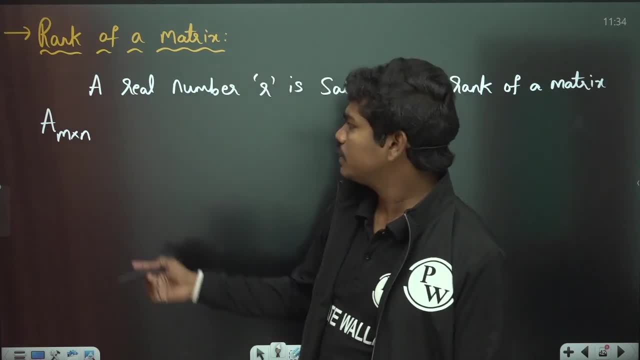 is said to be rank of a matrix: a, m by n. Here you need to observe one thing: this matrix need not be a square matrix. to talk about a rank, okay, For example, if you want to talk about determinants. 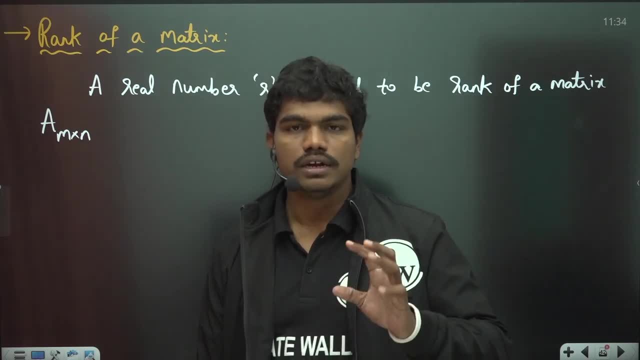 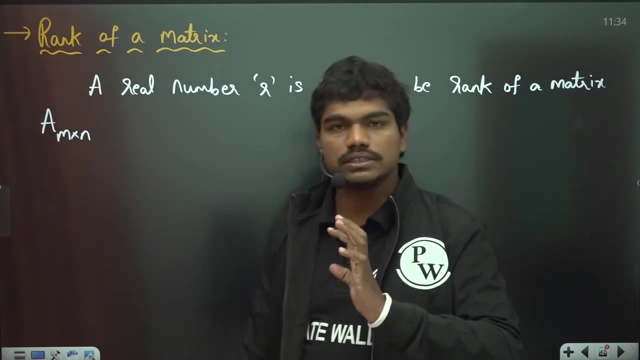 then definitely you should have a square matrix For rectangular matrices. you cannot talk about determinants, But if your idea is to talk about this- a m by n, I mean, if your idea is to talk about this rank of a matrix, then your matrix need not be a, you know. 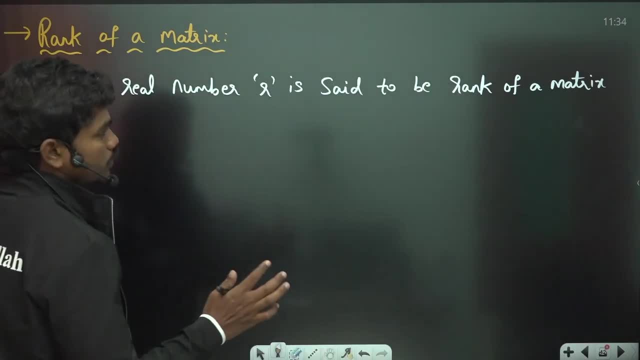 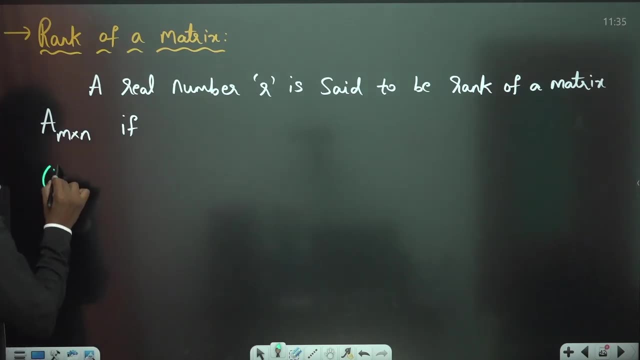 basically a square matrix. okay, So now see a real number. r is said to be rank of a matrix, a, m by n. if first point, first point, all the minus, all the minus of size, r plus one, by r plus one. 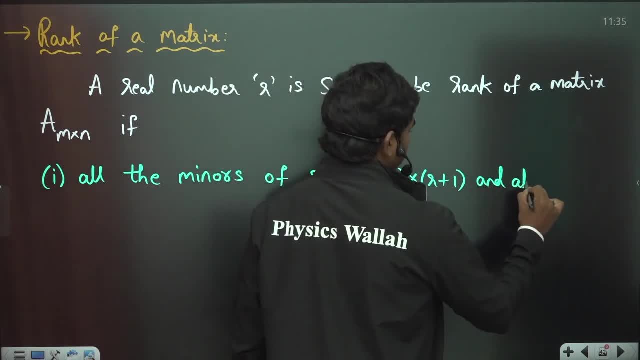 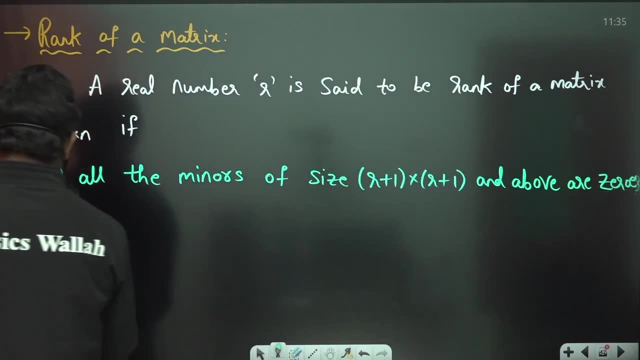 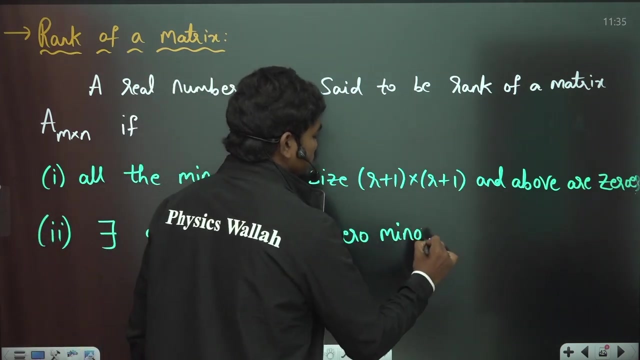 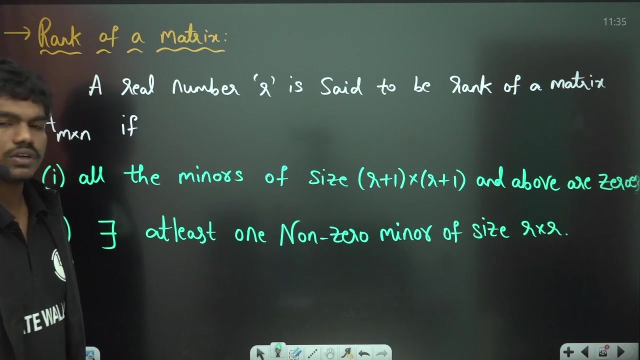 And above and above are zeros are zeros. Second, there exist at least one non-zero minor, non-zero minor of size r by r. okay, So what is the meaning of this? Okay, I have written two conditions here. So, first of all, all the minus of size more than r. 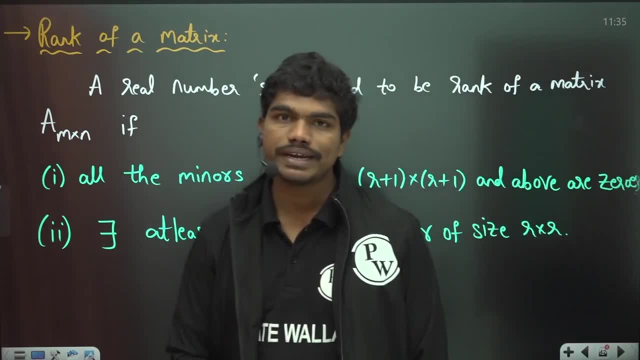 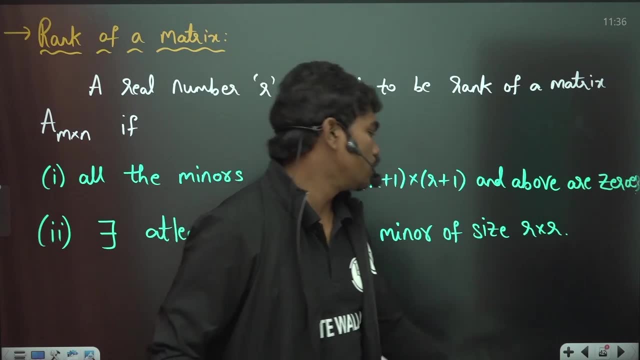 are definitely zeros And there exists at least one non-zero minor of this. you know matrix a, m by n. Now let us see how we practically do this. Look, let us suppose I have taken some example, because examples make you understand better. 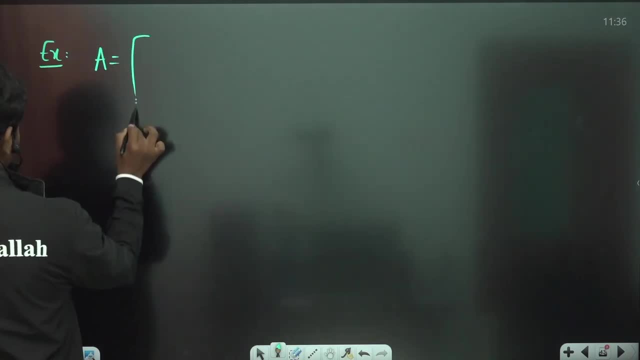 So let us suppose I have taken some example, So 1,, 2,, 3,, 4, let us suppose I have taken these elements two, four, six, eight. then, uh, say three, five, seven, nine. let us suppose i have taken. now try to. 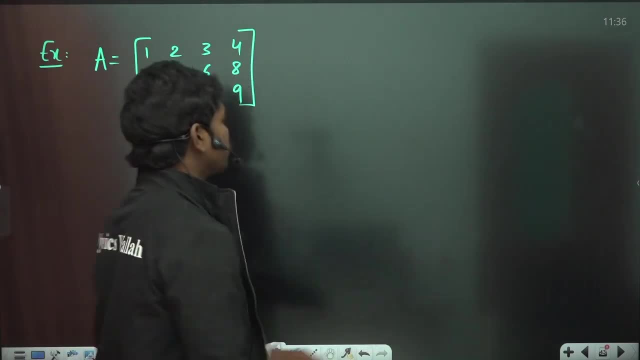 understand one thing: this is one matrix. this is of size three by four, for example. i have taken some random matrix. okay, so this is some uh, matrix, basically, and it's of size three by four. now how do i find the rank of the matrix? okay? so let us check here. let us check here. so if i want to find, 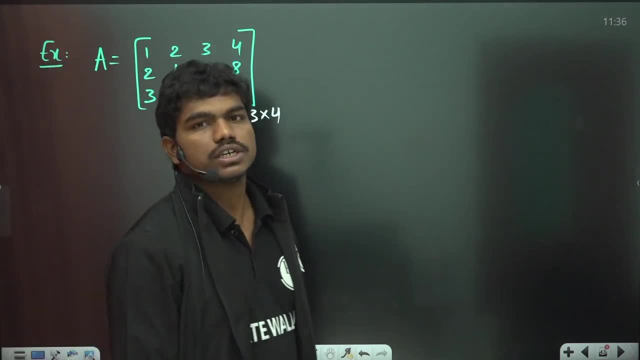 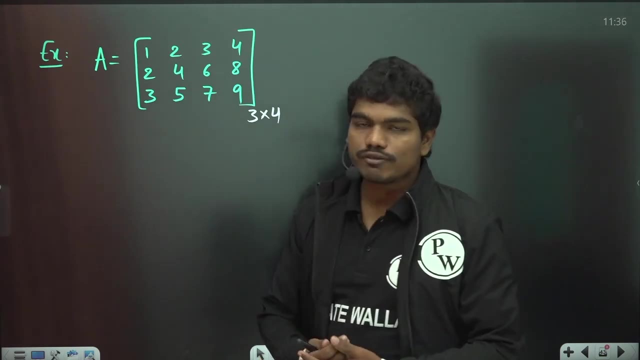 the rank of this matrix. first of all, i need to see what is the highest non-zero minor that is possible. so minor is basically some determinant, some part of the matrix, correct? so tell me, if this is a three by four matrix, what is the maximum size determinants i can take out of this matrix? 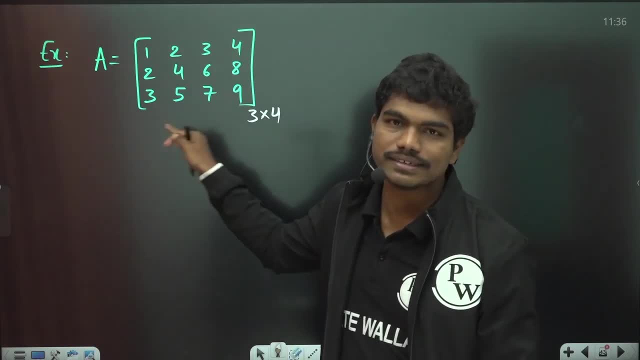 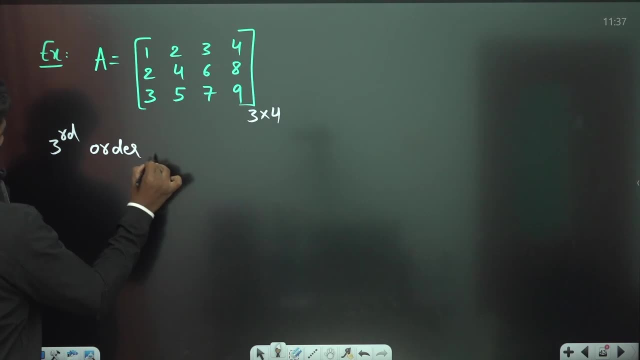 can i take four by four, because four is the highest? no, because there are only three o's in this matrix, so highest order that's possible is third order minus. third order minus. okay, we have seen this third order minus. so what are the third order minus that you can take out of this matrix? 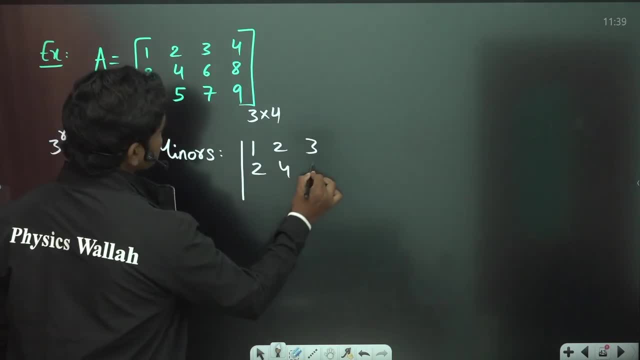 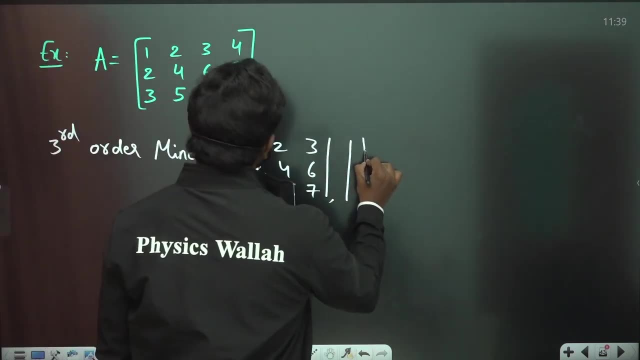 one, two, three, two, four, six, three, five, seven means basically i have deleted the fourth column. now i can take one more possible minor. what is that? let us suppose i am deleting the third column now. one, two, four, two, four, eight and three, five, nine. now let us suppose i have one more minor. if 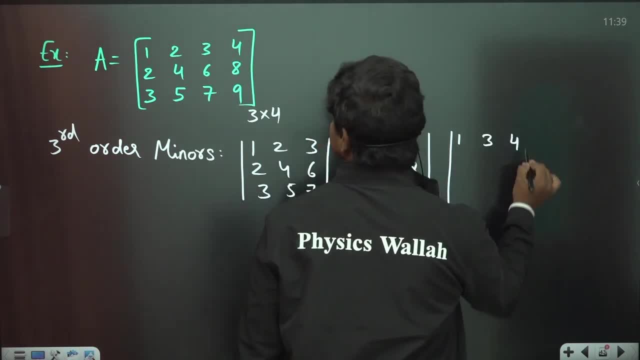 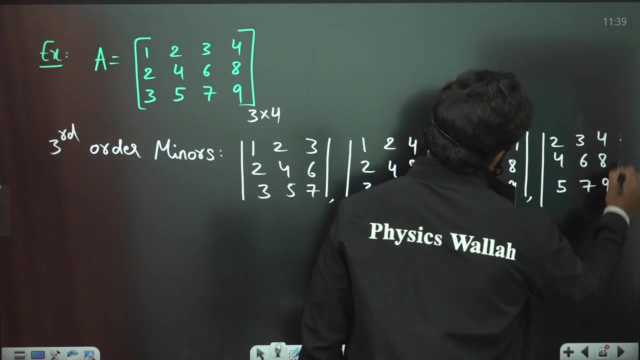 i delete the second row: one, three, four. i mean second column one, three, four, two, six, eight and, uh, three, seven, nine. and let us suppose i am deleting the first column: two, three, four, four, six, eight, five, seven, nine. so these are the four, three by three minors that 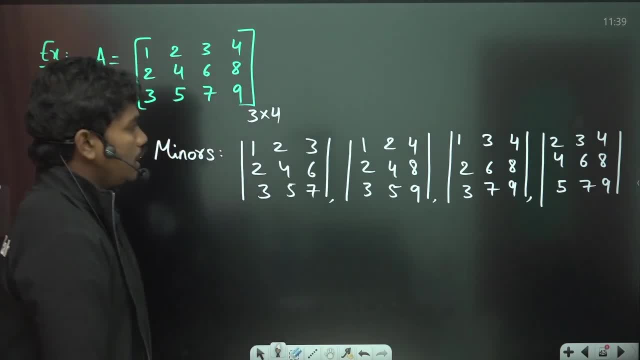 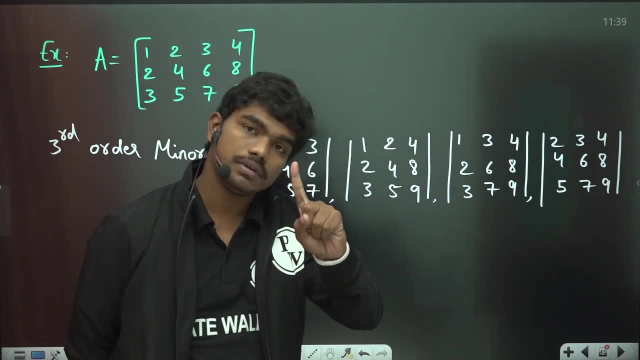 you can form using this three by four matrix, correct? now let us suppose if the, if one of these determinants is not equal to zero, for example, let us suppose even three are zero, but at least one determinant is non-zero, then we declare the rank of this matrix is three, because 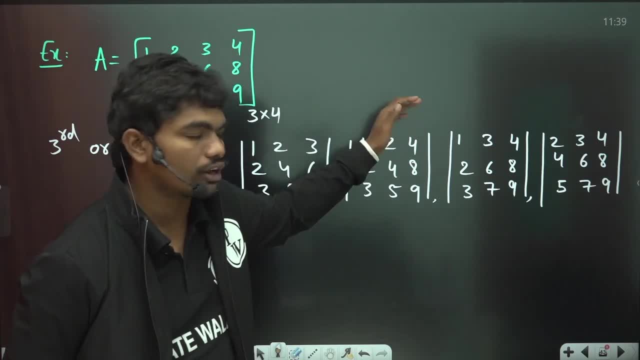 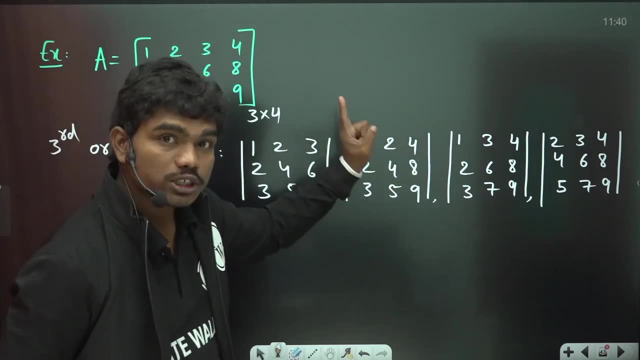 we cannot form four by four matrices or above. uh means we cannot form any four by four determinants or about determinants. and third order determinants are the highest order determinants that we can form and if you find at least one non-zero minor, then definitely you can declare rank of this. 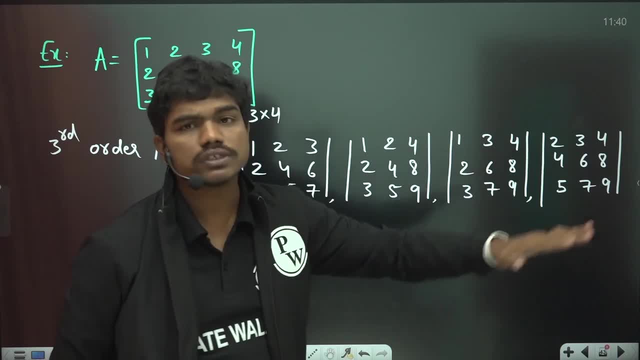 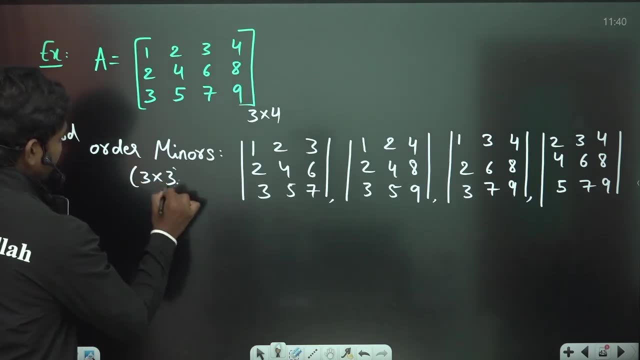 matrix is three. but let us suppose if all these four are zeros, now we need to go for next level. so third order, we have seen, means three by three. we have seen. now, if all these are zeros, then we'll go for second order minus. okay, so second order minus, second order minus. so basically two by two. 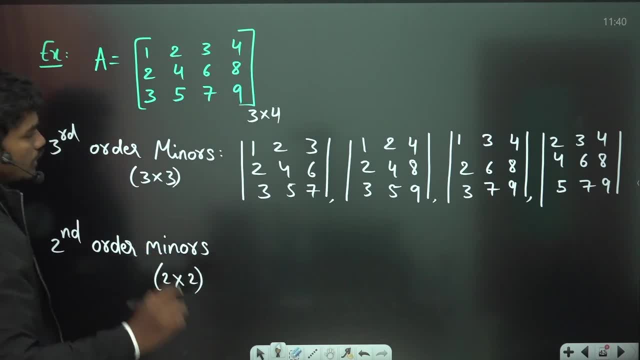 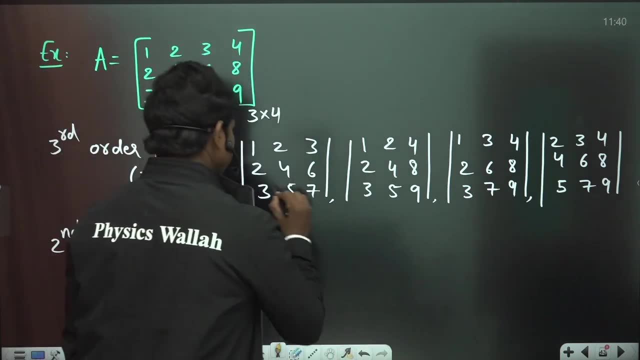 okay, so two by two. so now let us try to understand one thing: two by two minus. but first, before going to two by two, let us calculate these minus. so undoubtedly you can see, this determinant value is zero. why? because first row and second row are proportional to each other. that second row 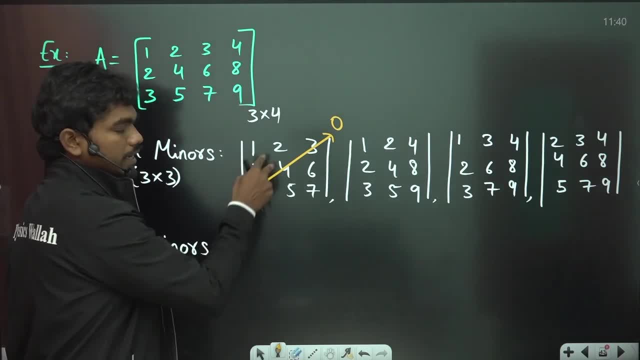 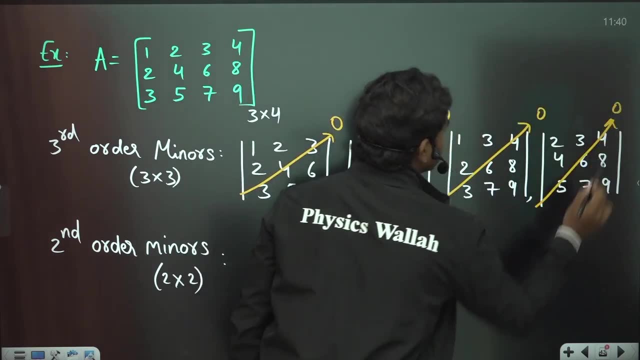 is just two times of the first row. so if you take one two out, first row and second row become identical. same is the case here, zero. same is the case here, also zero. and same is the case here, also zero. so basically, here all the four determinants. 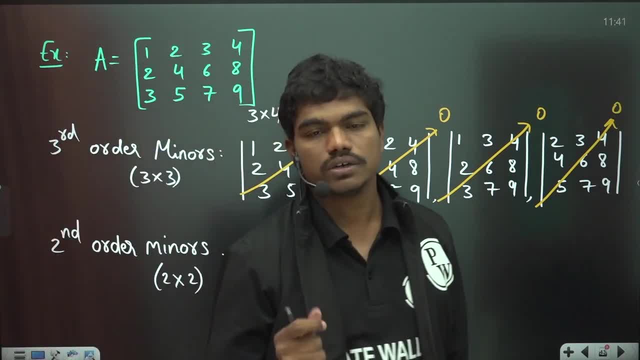 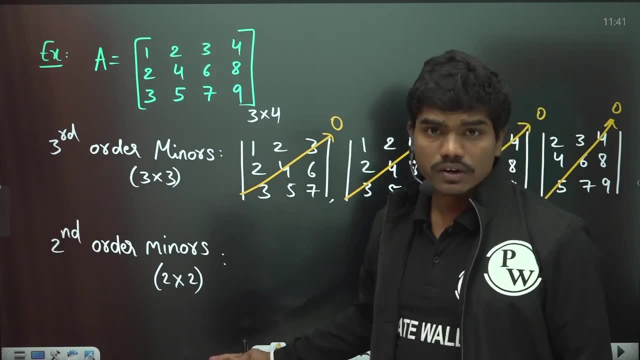 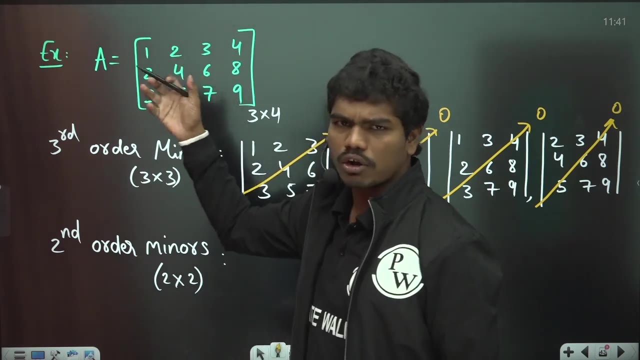 are zeros. so we cannot find any third order minor or this 3 by 3 size minor as non-zero. so then we need to go for second order minus again. if you want to write second order minus, you'll get lot of minus here. okay, you can take 1, 2, 2, 4, 2, 3, 4, 6, 1, 3, 4, 1, 3, 2, 6. again you can get a lot of minus. but 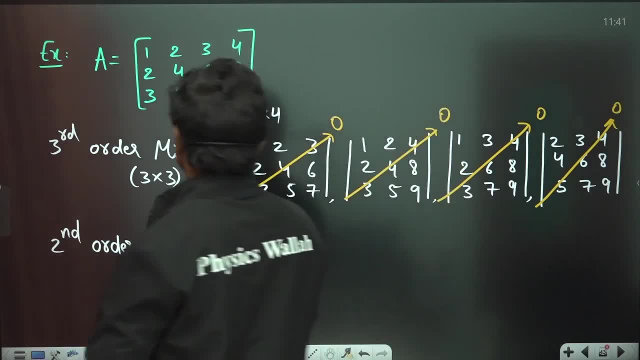 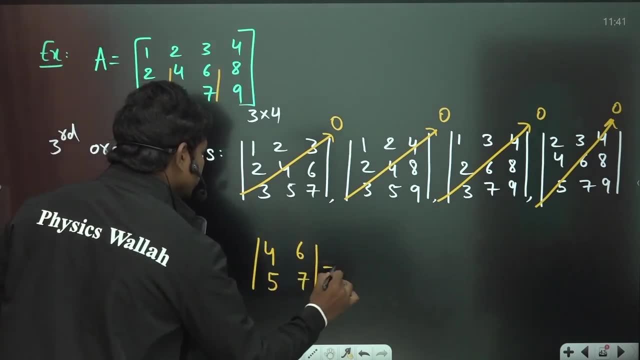 at least there should be one non-zero 2 by 2 minor. so let us let us suppose i'm taking this minor, for example, 4, 6, 5, 7, so if you see this value, this is not equal to 0, because 5, 6 is a. 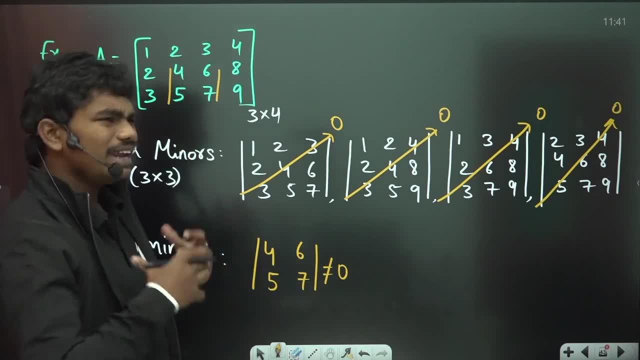 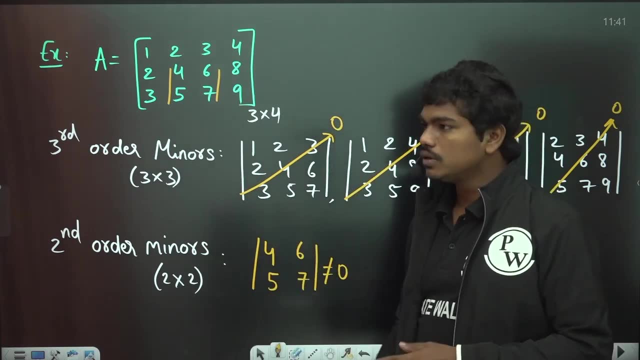 34, 7 is a 28. these two are not equal, so you can form any number of 2 by 2 minus, but at least you are pretty much sure that you have at least one non-zero minor of size 2 by 2. so now, if you want, 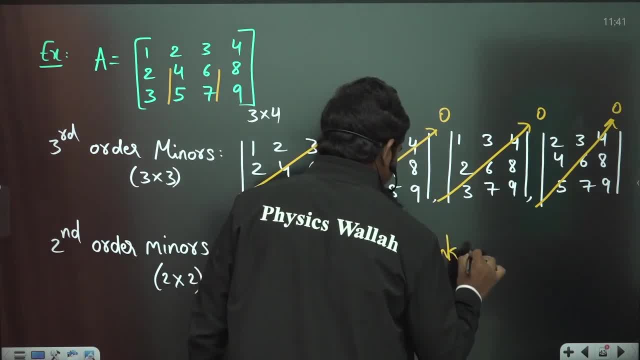 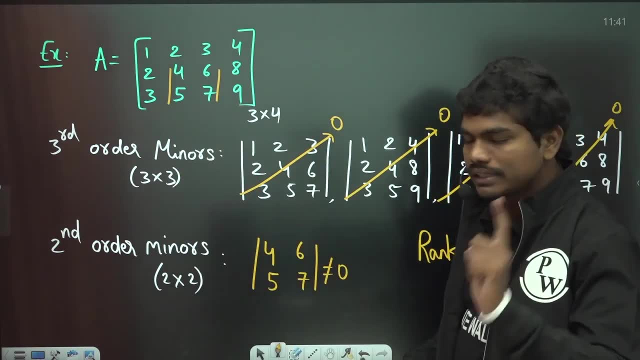 to declare a rank of this matrix. a rank of a is equal to 2. if you want to declare this, then you should make one sure, one thing very clear: that if you take size higher, minus means you know, if you want to declare this 2 as, 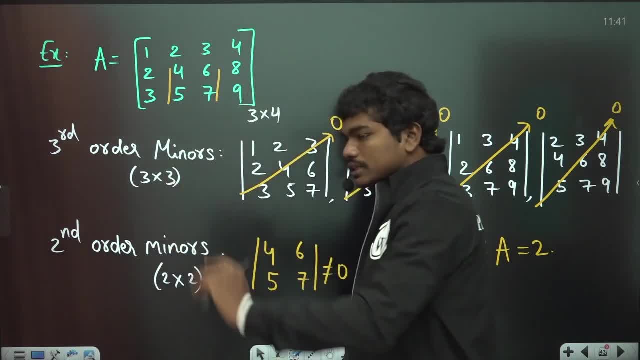 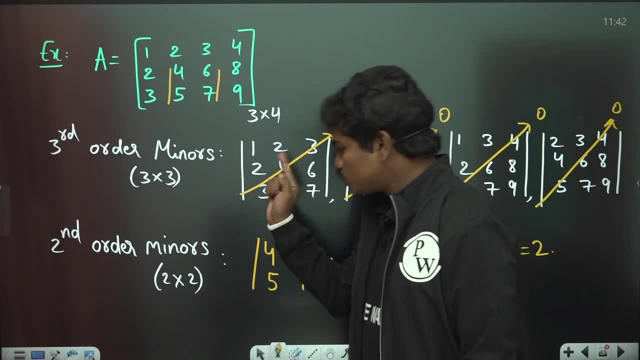 the rank of this matrix a, then you should pretty much sure that all 3 by 3, 4 by 4, 5 by 5 possible. of course all these things are zeros and definitely there exist at least one, 2 by 2 minor of non-zero. 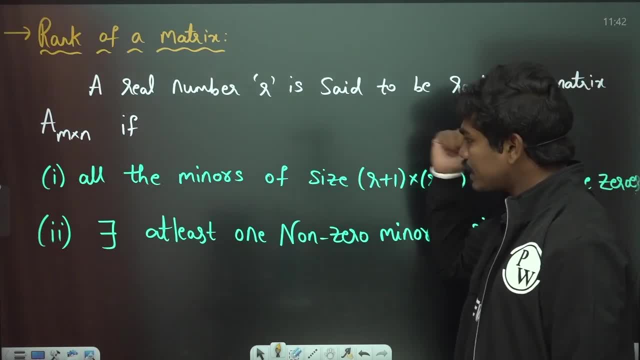 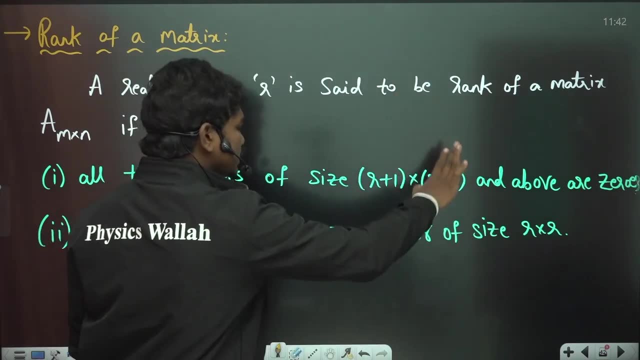 value. okay, this is what i have written actually here. so if you want to declare this number smaller as a rank of this matrix, all the minus of size r plus 1 by r plus 1 and above are definitely zeros and at least you have a rank of this matrix, a. so if you want to declare this number smaller as 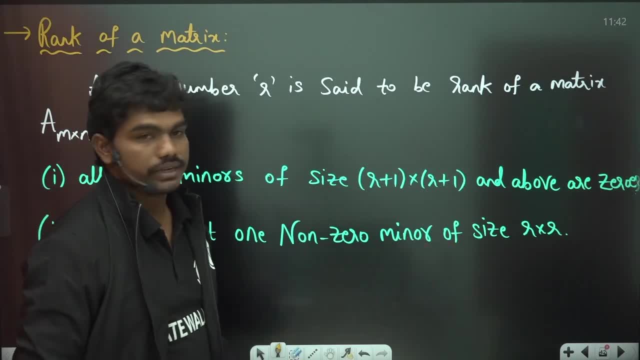 a rank of this matrix a, then you should pretty much sure that all 3 by 3, 4 by 4, 5 by 5 possible. at least you should have one non-zero minor of size, this r by r, if you do the r value with the. 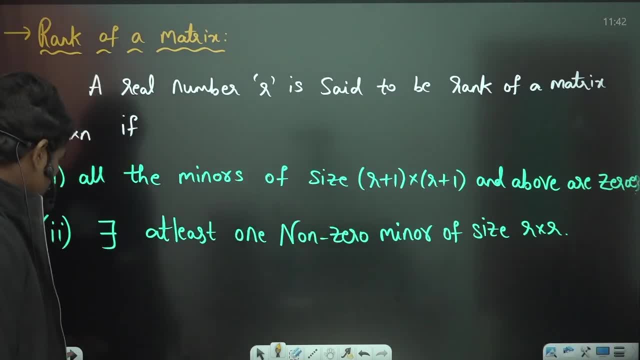 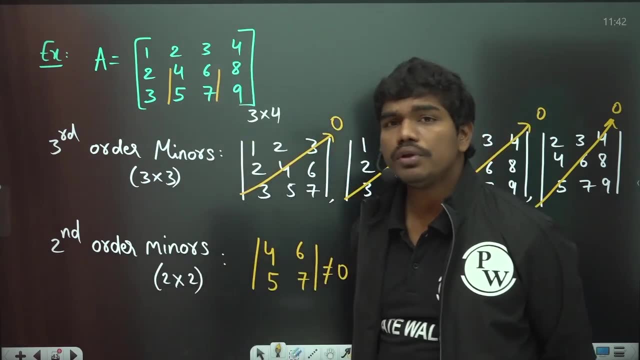 2. you will understand the next example. that's it okay now. so basically checking this, so if you understand one thing, many of you might have had this question by now: how do you know how many 2 by 2 minus you have and how do you know whether, in that 2 by 2 minus, you may have a 0 or not? look, 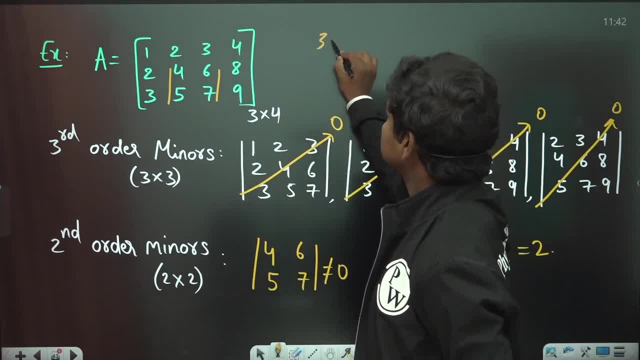 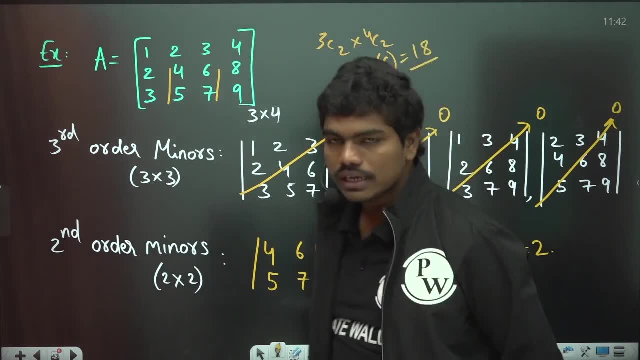 i'll tell you. if you want to form 2 by 2 minus, you will get 3 c 2 into 4 c 2, so this is basically 3 into 6. you will have 18, 2 by 2 minus, totally okay. so writing this 18, 2 by 2 minus and checking whether, 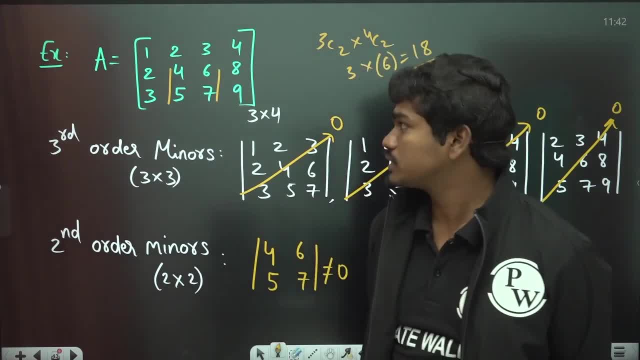 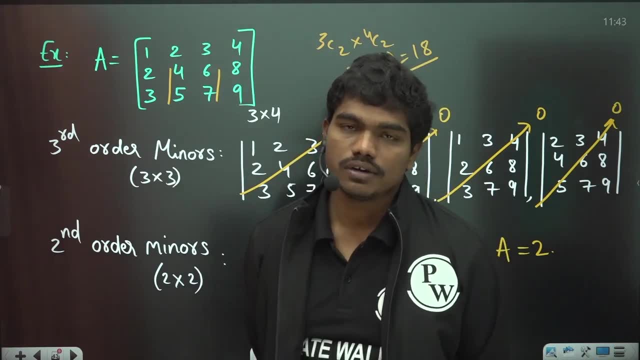 they are zeros or not is not very easy here right now. and of course, if the matrix size is of some 6 by 6, 7 by 7, of such kind, then forming 4 by 4 minus, 5 by 5 minus this is not very. uh, you know a very. 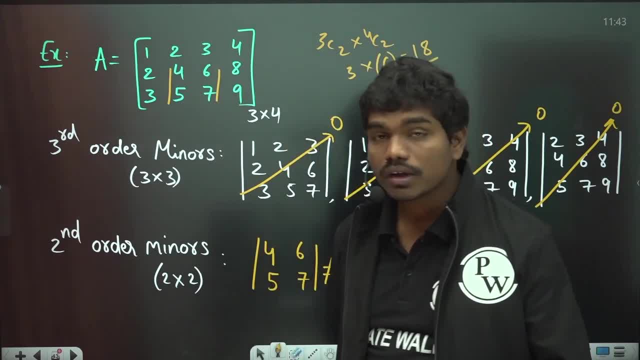 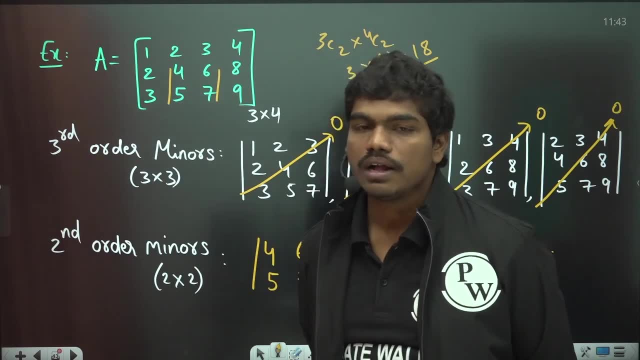 efficient way to check what is the rank of a matrix. so what we have done for this is: you definitely should have some easy procedure or some constructive way to decide what is the rank of a matrix. so now what we have done is: we have done a rank of a matrix, and we have done a rank of a matrix, and 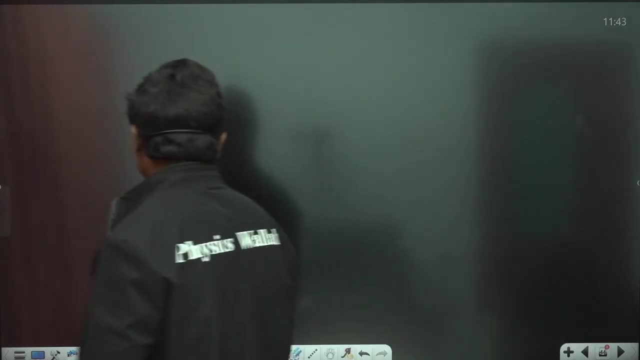 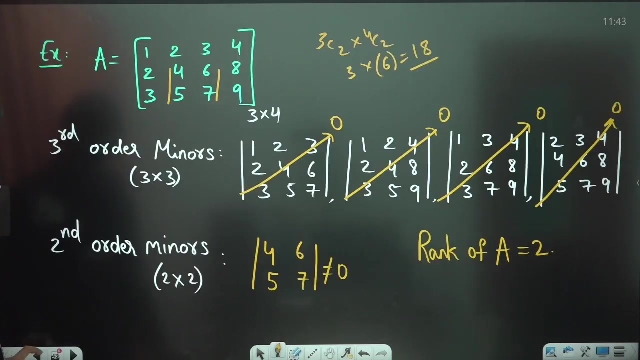 we talked about one thing which is called row echelon form of a matrix. this is one very, very important part: row echelon form of a matrix- matrix. now, before going for a clean form, i forgot to tell you one uh small thing here. look, what i want to tell you here is: it is denoted by: you can write. 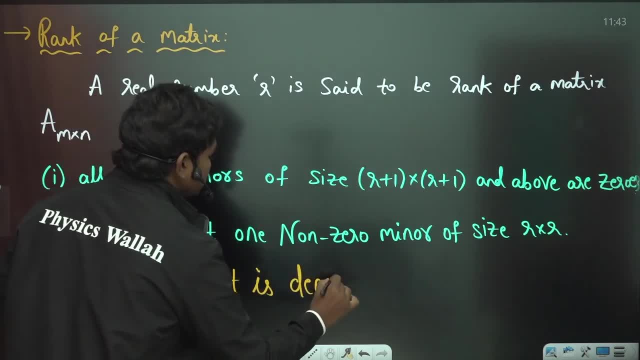 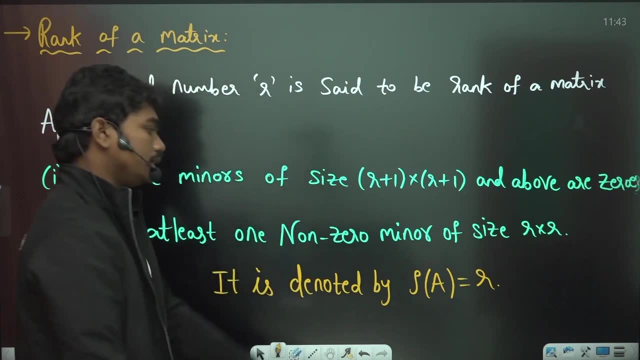 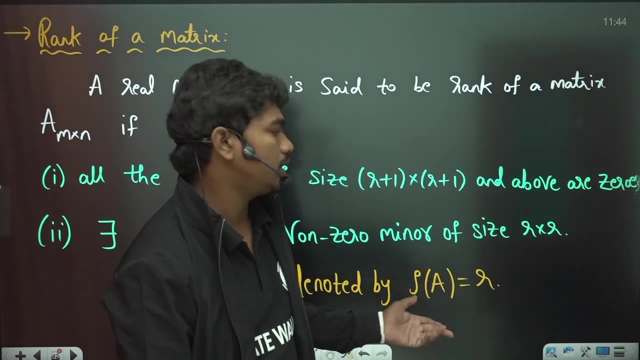 here it is denoted as it is denoted by. you can say: row of a is equal to r. okay, so this rank of a is actually denoted with this symbol, that common symbol you take for resistivity or density in mechanical on civil. so, if you see, this is the symbol that you uh denote for this uh rank. so rank of a is denoted with this. 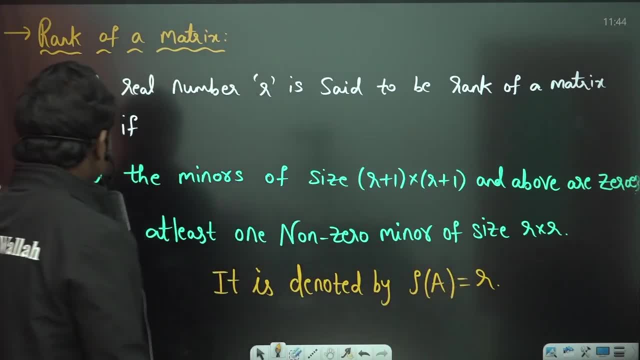 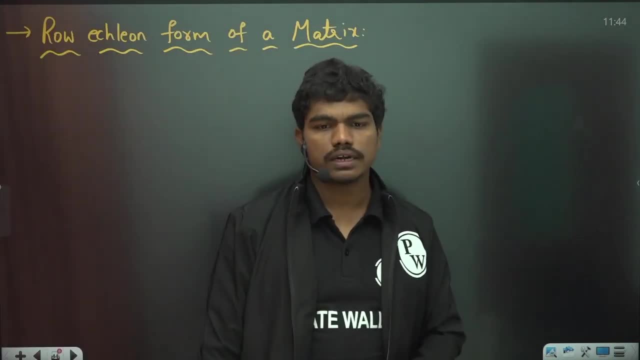 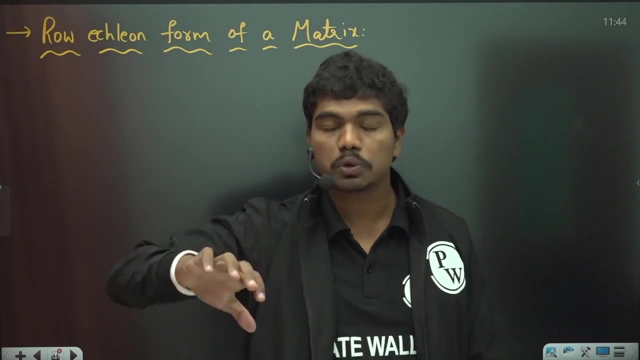 row of a is equal to r. okay, so now let us come to this row- echelon form. okay, so let us come to this form of a matrix. How do we know that? basically, what is this Euclidian form? Let us see. Then we'll see if a matrix is in the Euclidian form or not. We'll also see how to convert. 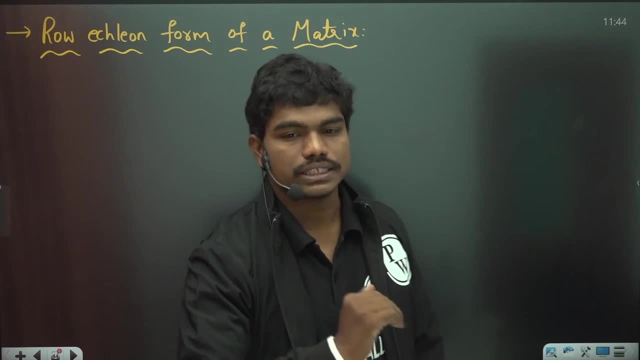 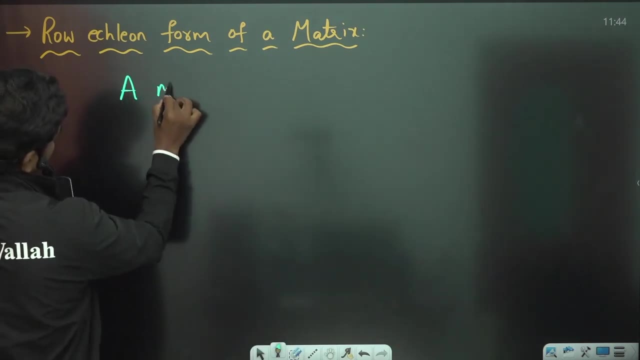 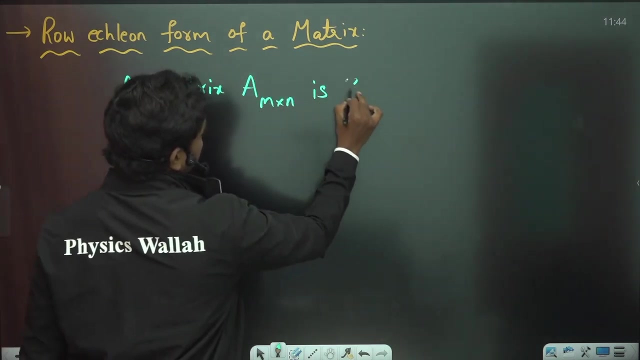 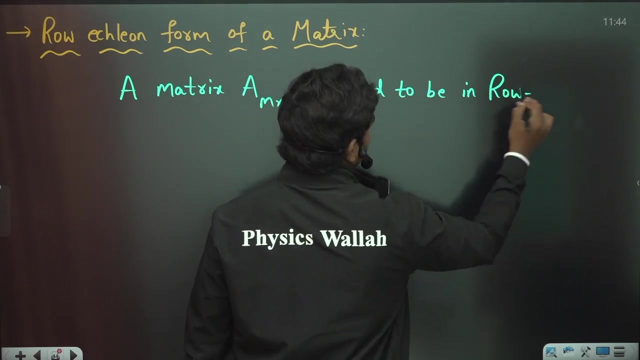 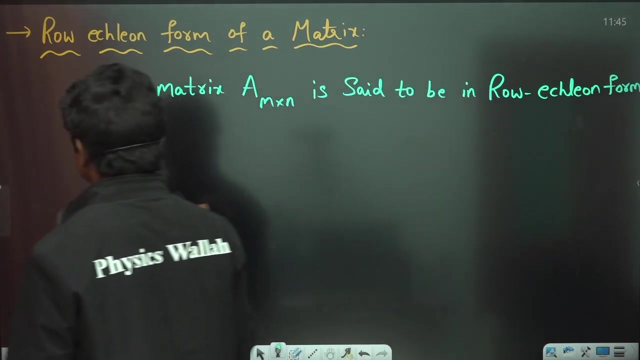 any given matrix into Euclidian form. Okay, we'll see these things. Look a matrix. let me change the color. A matrix. a matrix A M by N is said to be in a row. Euclidian form Is said to be in a row. Euclidian form if, again, there are two conditions here. If a 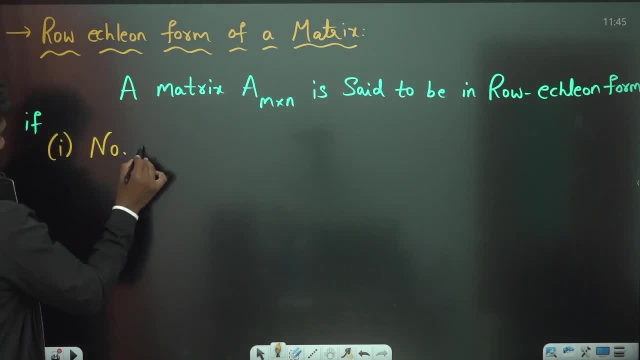 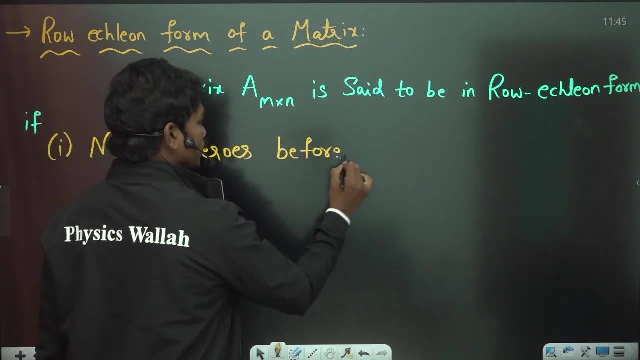 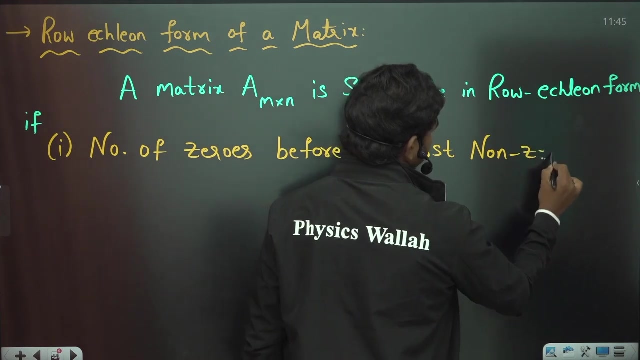 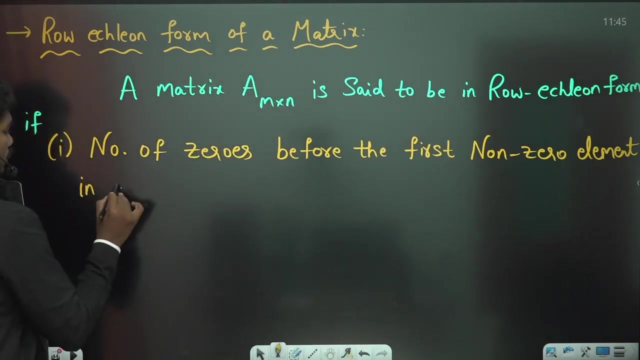 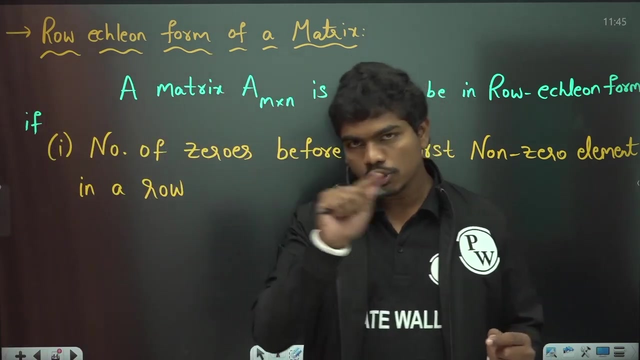 first condition: number of zeros before the first non-zero element. before the first non-zero element: before the first non-zero element in a row. before the first non-zero element in a row. basically so, if you have taken ematics, for example, then in a row, if you take 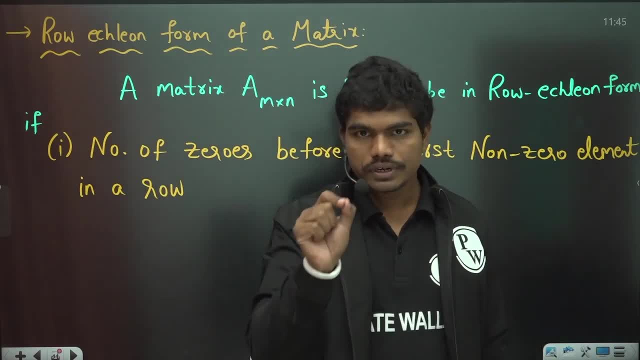 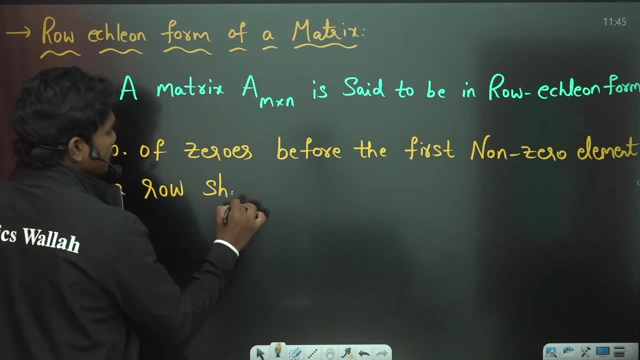 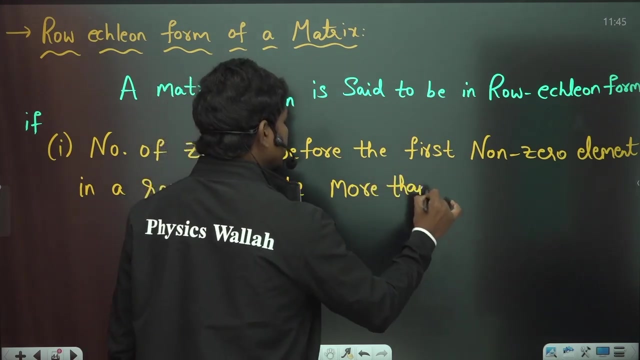 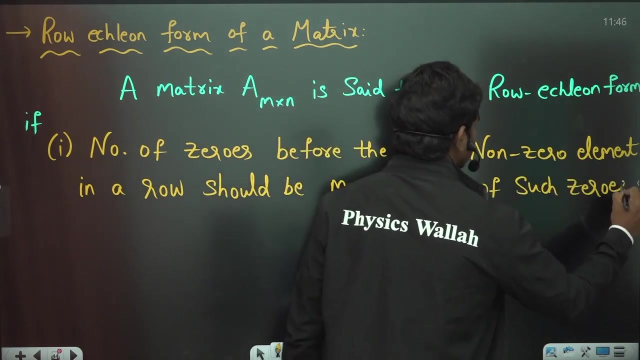 definitely some elements can be zeros and some can be non-zeros. so if you take the first non-zero element that's coming if you count the number of zeros before that, so this should be, should be more than should be more than number of such zeros. such zeros in its preceding row. preceding means one above that in its preceding row. 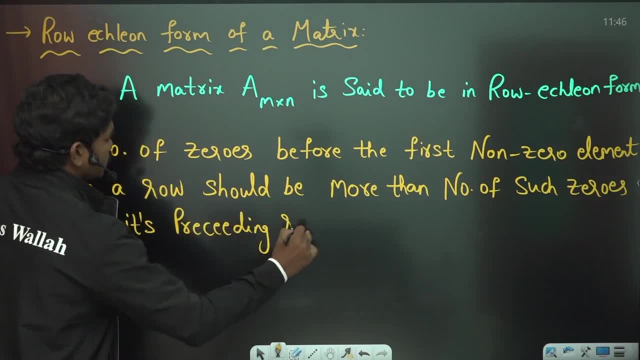 preceding row and second thing. second thing: number of zeros before the first non-zero element in a row should be more than number of such zeros in its preceding row. and, importantly, we can have second thing as zero rows, if any means. let us suppose during some transformation, if you get any zero rows, for example, then should like at bottom of the matrix should lie. 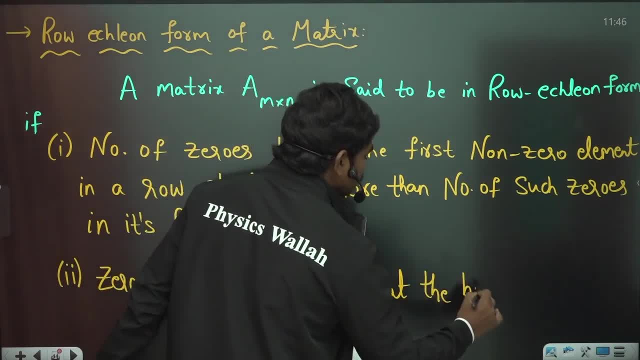 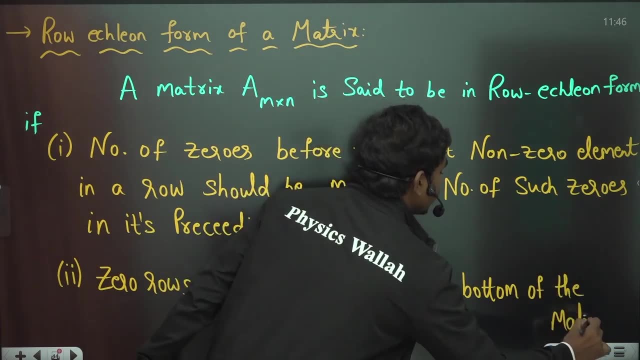 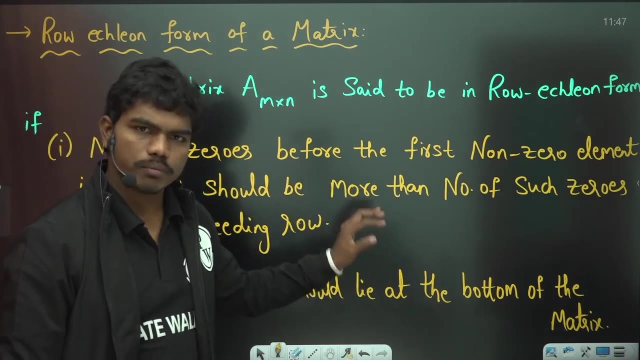 at the bottom of the matrix, should lie at the bottom of the matrix. should lie at the bottom of the matrix means basically, let us let me show you one example in row echelon form. we will understand as the Це– live condition and take of it like this: will be ok, so if we take, and it will be. 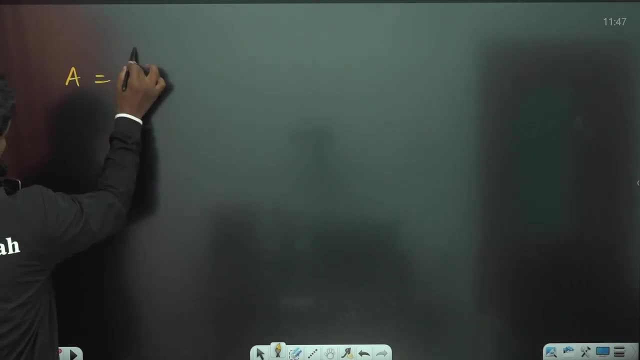 understand that. okay. so let us suppose, if you take this matrix which is in this form, for example one, two, three, four, five, six, seven, eight, all zeros, for example, let us suppose you have taken it need not be square matrix, also, it can be some other matrix as well, no, 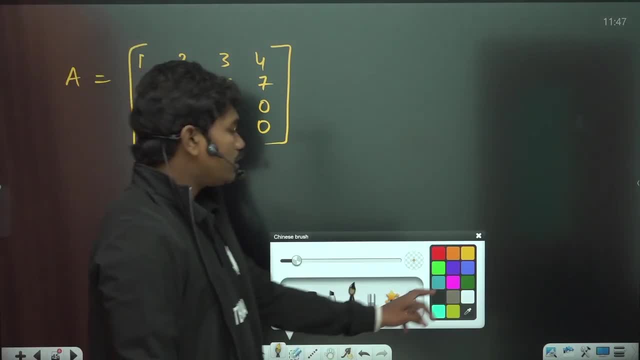 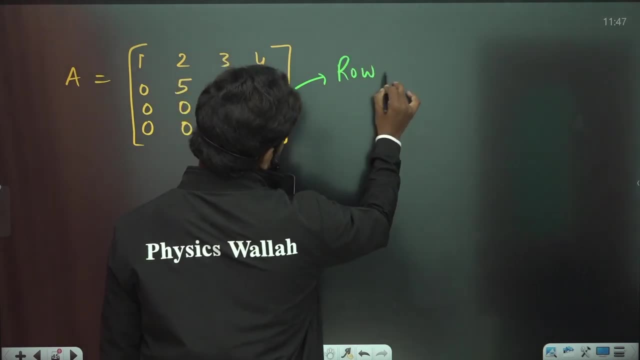 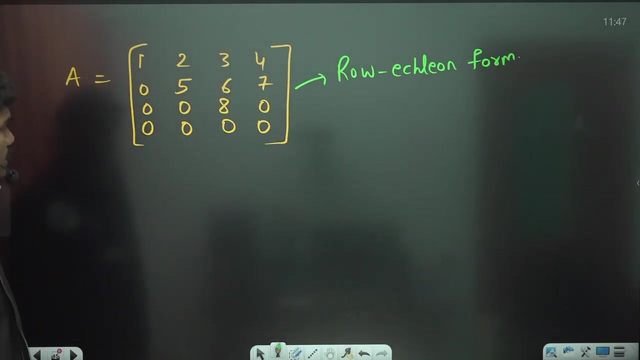 issue. now, what is the meaning of the first statement that i have written here? this matrix is actually in row echelon form. this is in row echelon form how. i will tell you: row echelon form. row echelon form now. how. actually this, uh, this two points will actually in line with: 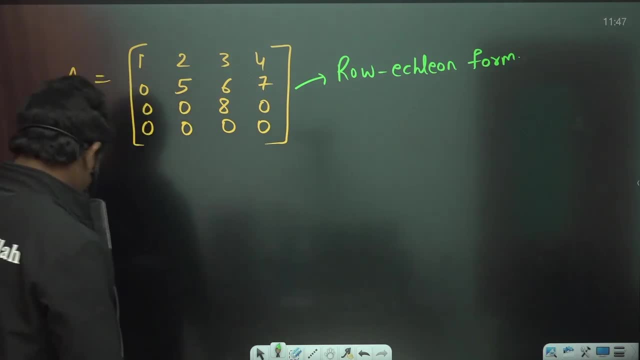 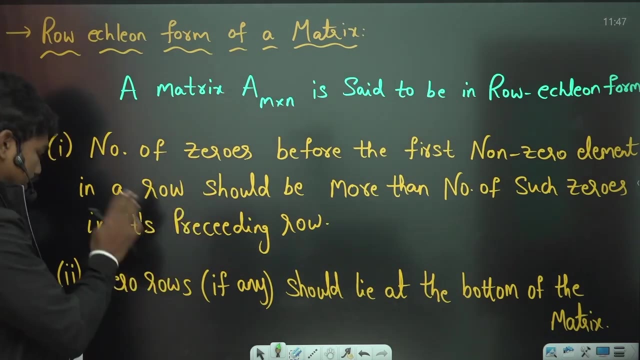 this example that i have given you here. let us check. so. first statement: number of zeros before the first non-zero element in a row should be more than number of such zeros in its preceding row. look, what is the meaning of this. let us suppose i have taken the first. 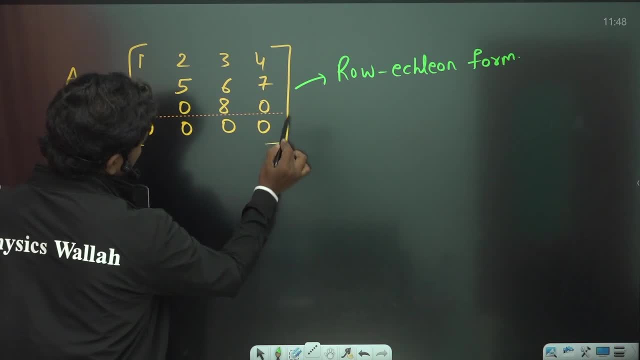 third row. for example, if i take this third row, if i take this third row, then this is the first non-zero element in this row, correct? so this is the first non-zero element, and number of zeros before the first non-zero element are two in this case. now this number. 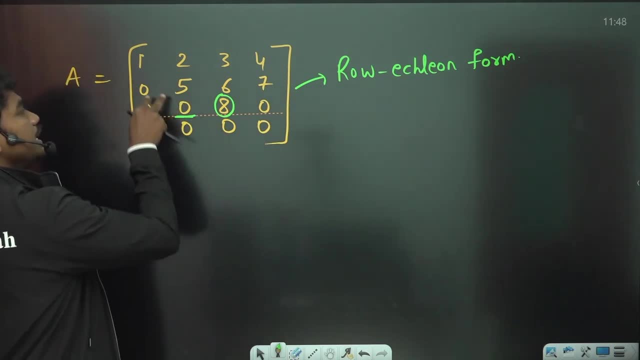 of zeros before the first non-zero element is two. so definitely in its preceding row you should have one either or zero elements. so basically, here you can see one why i have intentionally kept one here, because if you take the second row, this is the first row before the first non-zero element. so here, if you have one zero here there should be. 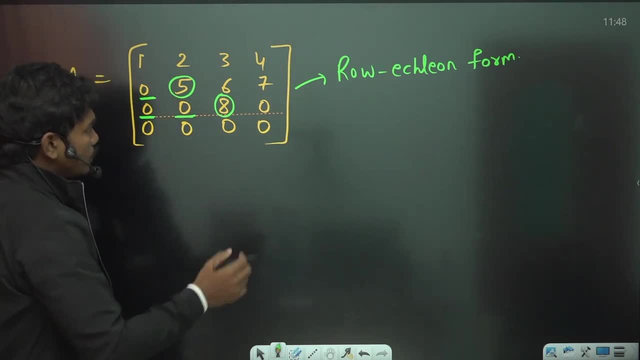 no zero. that's the reason why i have taken like this. so if you take any particular row, then the number of zeros before the first non-zero element should be definitely more than number of such zeros. such means again, if you take this second row, this is the first. 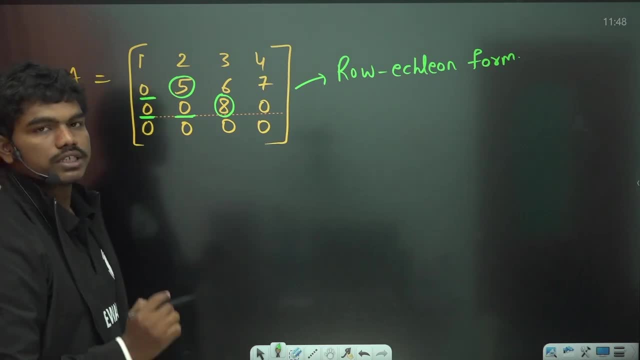 non-zero element and these are the zeros before this first non-zero element. so, if you see, this number of zeros before the first non-zero element should be definitely more than number of such zeros in its preceding. so for third row, number of zeros should be more than the. 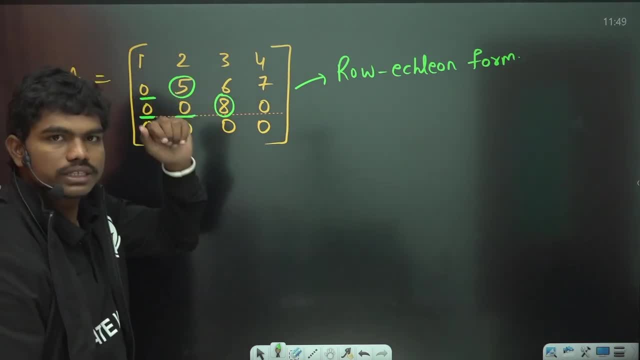 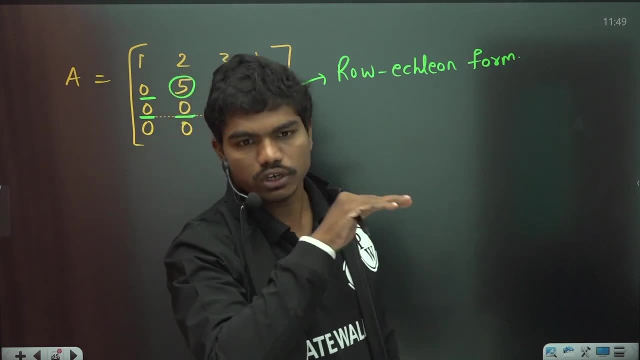 first row. for second row, number of zeros should be more than the first row, like this. okay, so this is what i mean. second point: it's a easy point you can understand. zeros means basically, if there is some any row which is in which all the elements are zeros, they should. 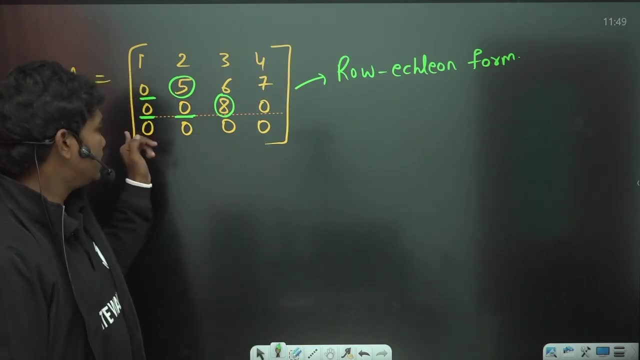 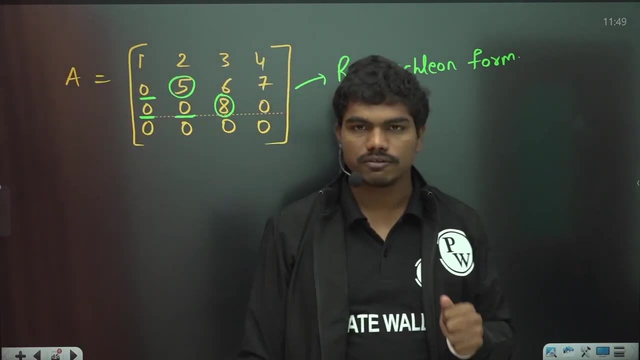 lie at the bottom of the matrix, basically. so, if you see there is one zero which is completely zero, so this should lie at the bottom of the matrix. actually clear. so that's how you know. uh, this matrix is in row echelon form. okay, now, basically. okay, i have given one direct. 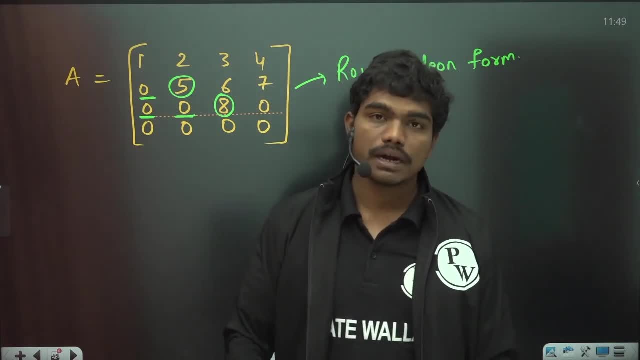 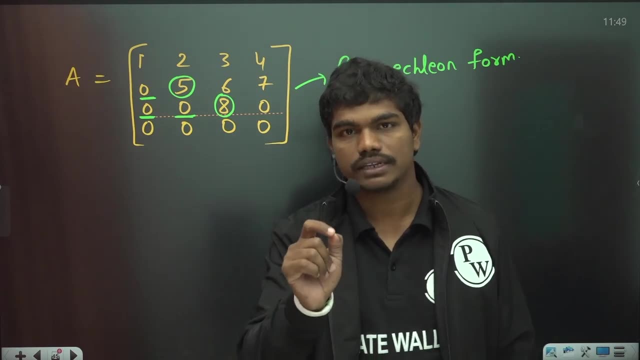 exist and i made you understand how a form of matrix look likes. but let us suppose, if i actually give you one matrix, then how you convert that matrix into a weight uniform. that's the very important thing. okay, so that is what next? i am going to discuss that. 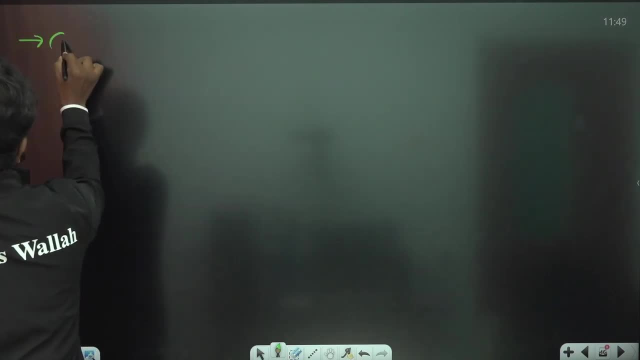 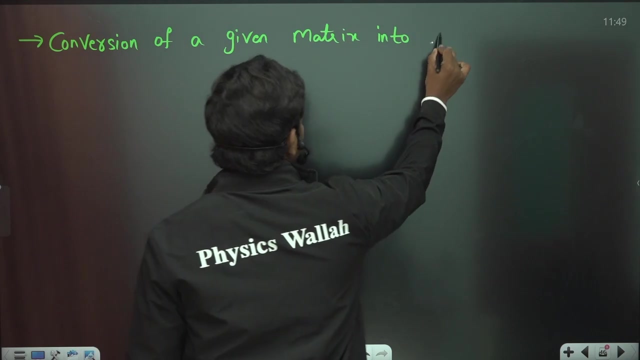 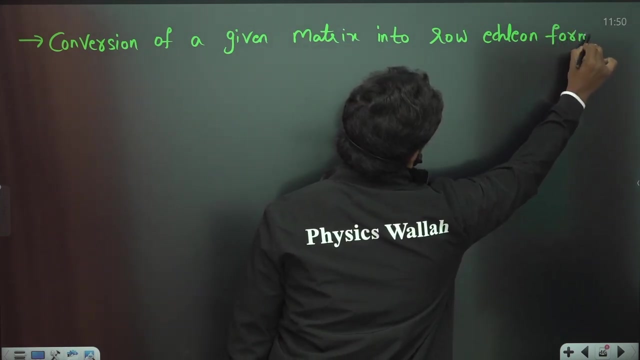 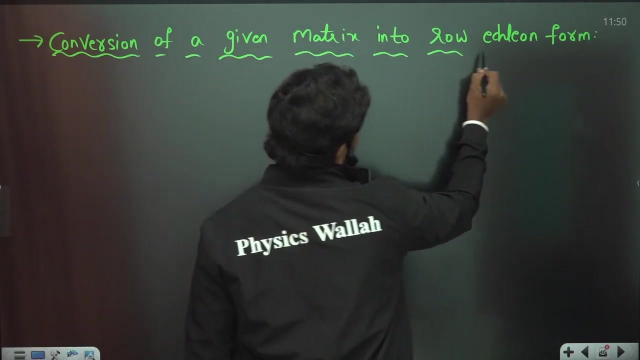 fuerzaJask puzzling can version of you que les voulez � kız matrix into row echelon form this is one very important part that you should know basically here okay so conversion of a given matrix into conversion of a given matrix into row echelon form so how 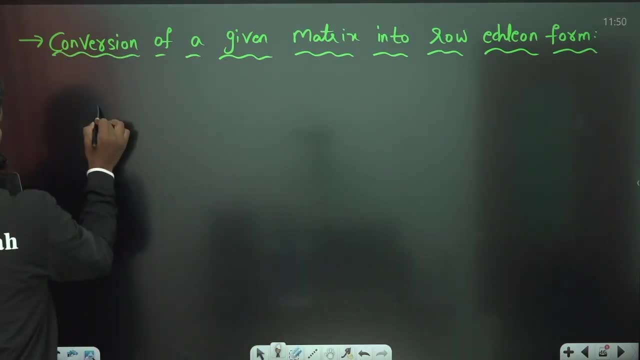 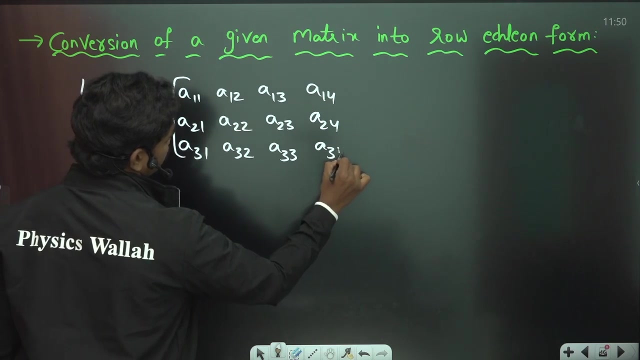 we'll convert. look, let us suppose i have given you one matrix. let a is equal to a 1, 1 a 1, 2 a 1, 3 a 1, 4. let us take 3 by 4: a 2, 1 a 2, 2 a 2, 3 a 2, 4 a 3, 1 a 3, 2, a double 3 and a 3, 4, for example. 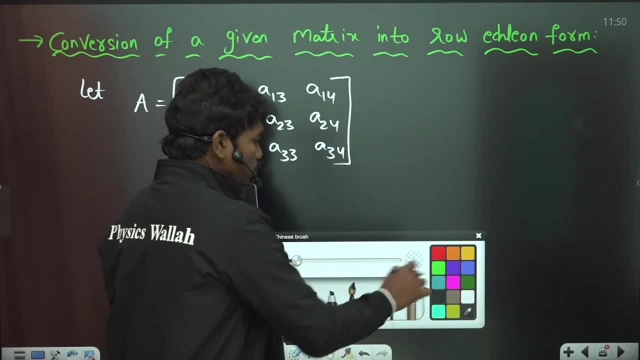 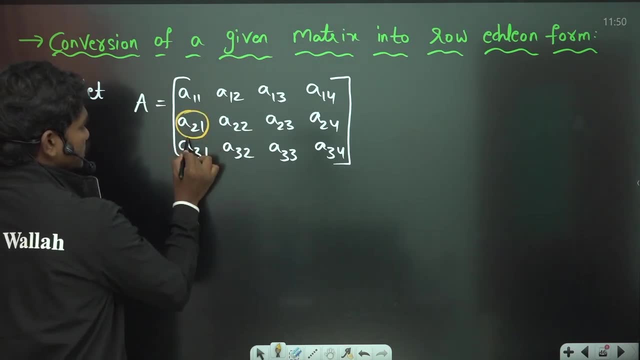 so let us suppose this is the matrix. now, how to make this element, make this matrix a, you know, into a echelon form, let us see. first of all, try to make these two elements zeros. first of all try to make these two elements zeros, okay, you? so when you try to make what are the transformations, you'll apply r 2 changes to r 2 minus r 2 minus. 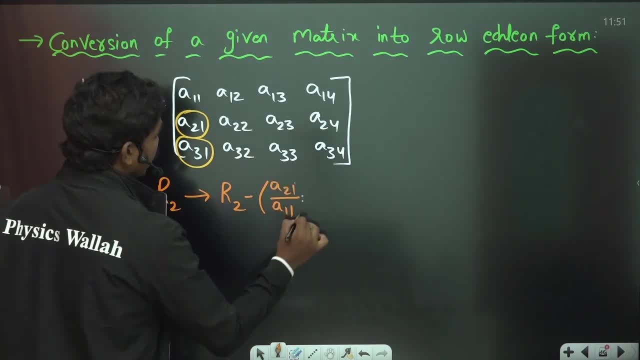 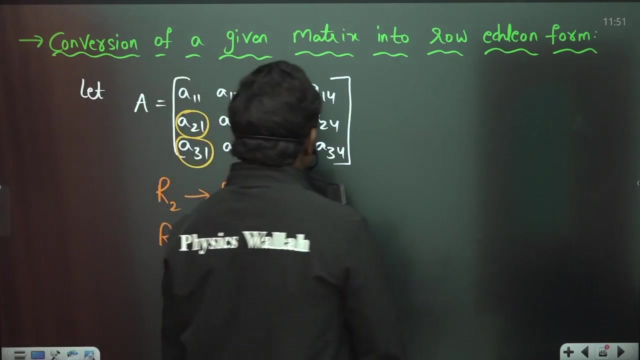 a 2, 1 by a 1, 1 into r 1, and r 3 changes to r 3 minus a 3, 1 by a 1, 1 times r 1. so let us suppose this is the transformation you have to apply now. if you apply this transformation, then undoubtedly. 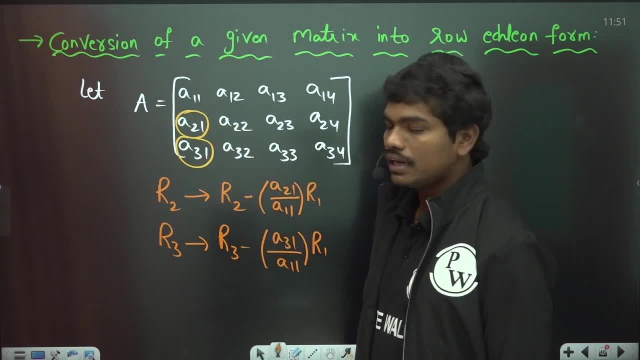 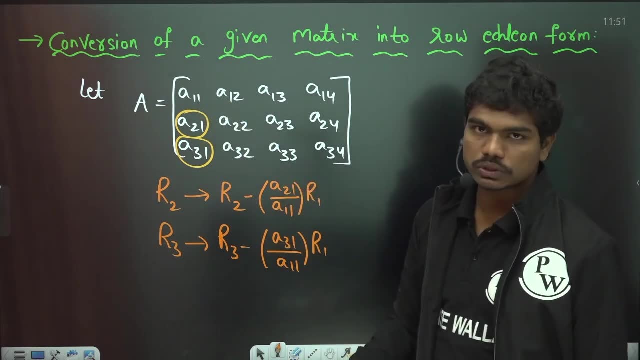 these two elements will become 0 and all the six elements will change. okay, now here you can have one question. okay, so we'll do this. but let us suppose if a 1- 1 is 0 and these two are not zeros, okay, if this element is 0, but 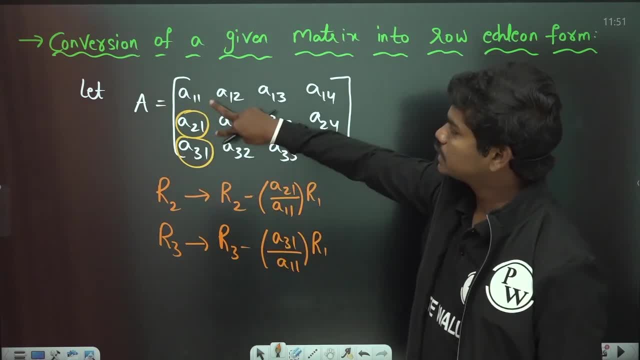 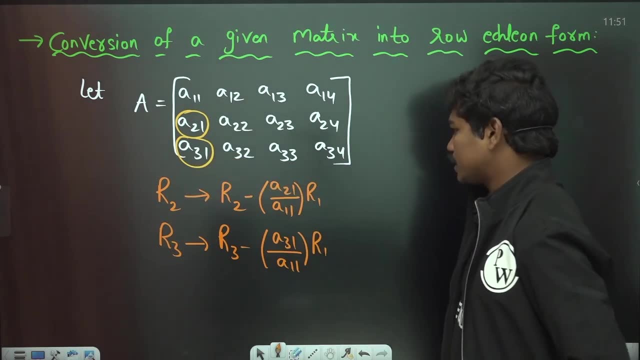 these two are non zeros. then how to do this look simple. you can swap those then. okay. so when you swap here, you'll get a non-zero and maybe one zero you will get in some cases. okay. so that's how you actually perform this transformation. then this matrix gets equivalent to first row, doesn't? 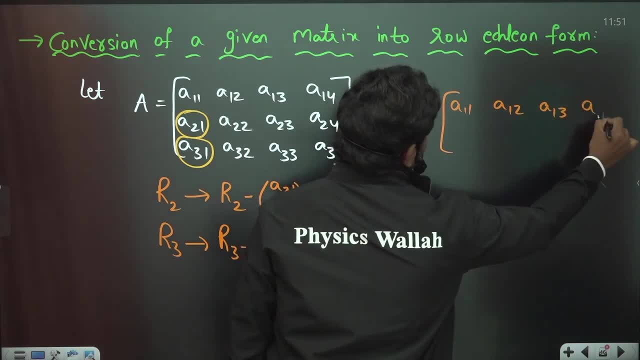 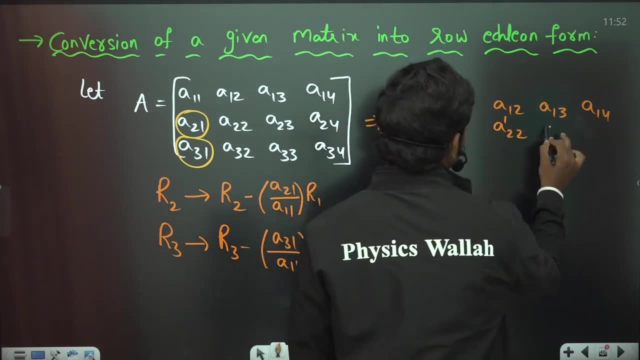 change a 1- 2, a 1 3, a 1- 4. these two turns out to be zeros. then you have a 2- 2 dash, because this value changes after this transformation. a 2- 3 dash. a 2- 4 dash. similarly, a 3- 2 dash, a 3- 3 dash and a 3- 4 dash. this 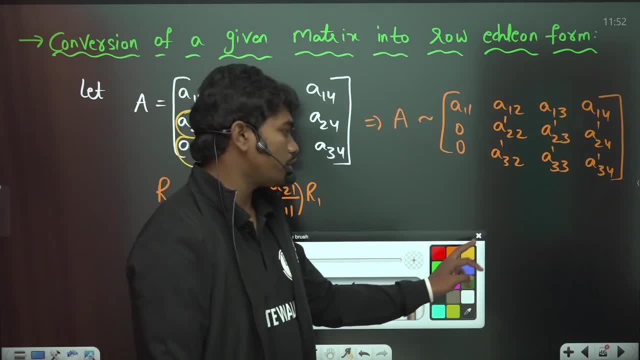 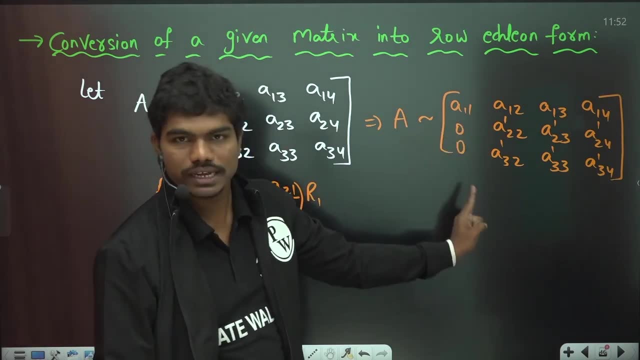 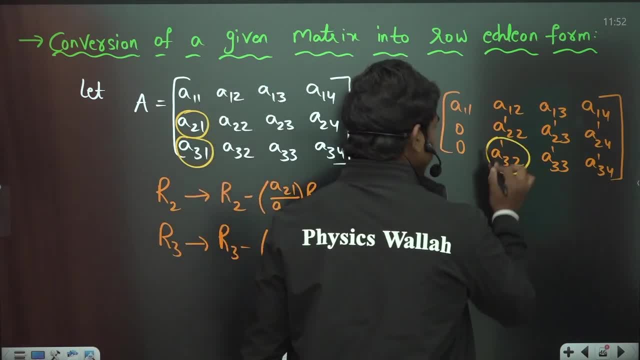 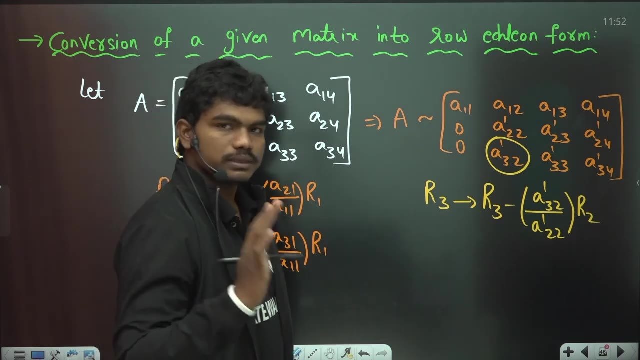 only one zero. so that's the reason we will make this element again zero. how will you make that again? one more transformation: r3 changes to r3 minus a dash 3, 2 by a dash 2, 2 times r2. this is what you can apply. so if you apply this transformation, first and second row remain as it is. 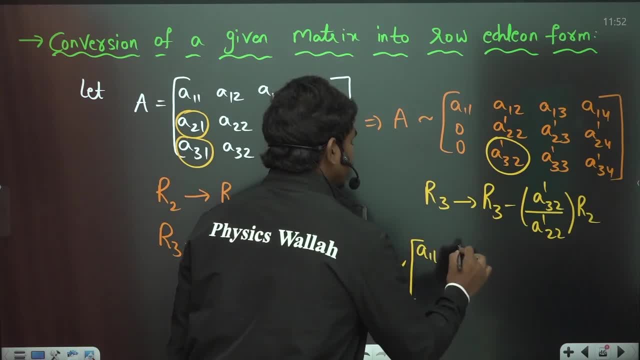 so first and second row remain as it is a 1, 1 a 1, 2 a, 1, 3 a 1, 4. then again you can have 0: 0. second row remains as it is a 1, 1 a 1, 2 a 1, 3 a 1, 4. then again you can have 0: 0. second row remains as it is. 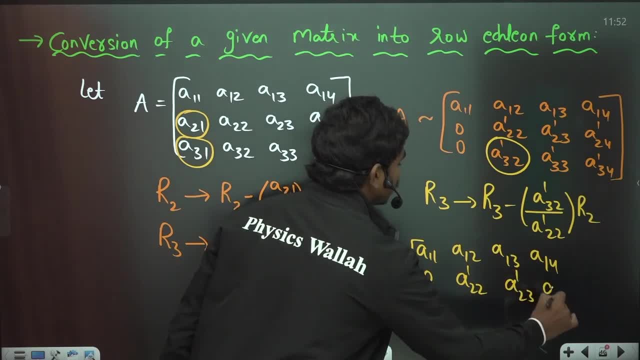 a 2 2 dash, a 2, 3 dash, a 2, 4 dash. and this third. oh, it changes this 0 minus something into 0. this will be 0, so this is also one more 0 here and again, these two elements will change a double. 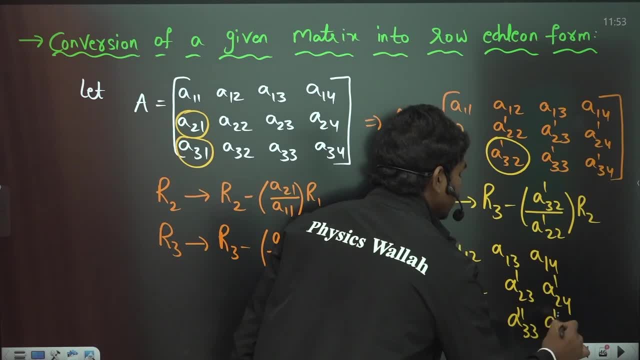 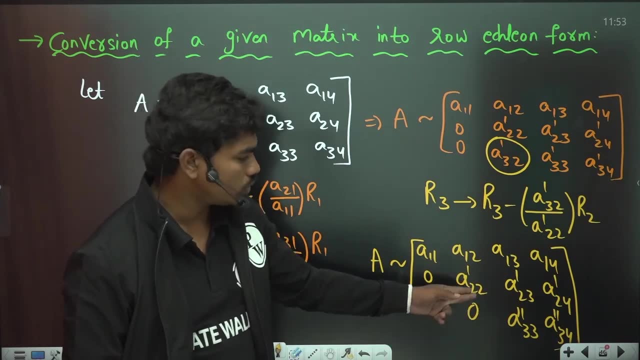 3 double dash, a 3, 4 double dash again. so this is how you have a basically o a cleon form. now, if you see in this matrix there are no zeros, so there is no nothing at the bottom. but here you can see, before the first non-zero element there is no 0. before the first non-zero element there is at. 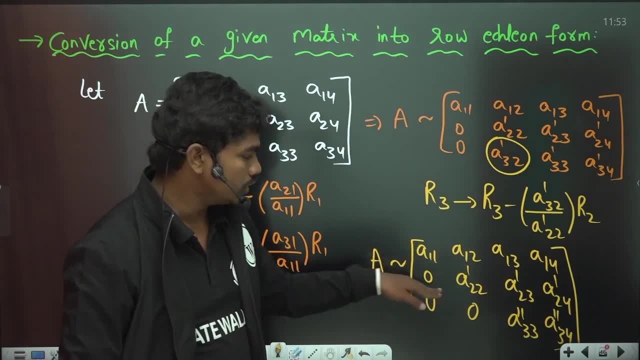 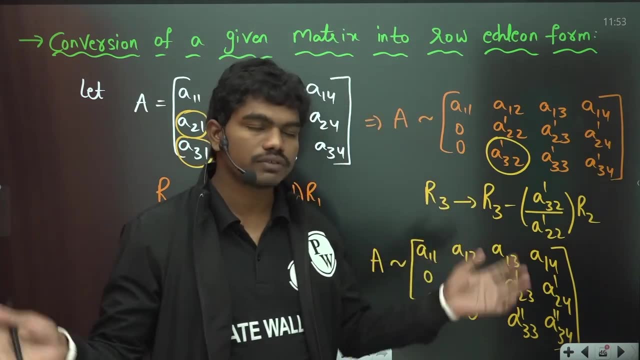 least one. 0 it should be definitely, because here it's 0, it should be more than 0. similarly, here they are 2. so this is how you convert any given matrix into row, a cleon form actually. so now, if it's of size 3 by 5 or 5 by 5, whatever it is, you can always have this conversion, and anywhere if 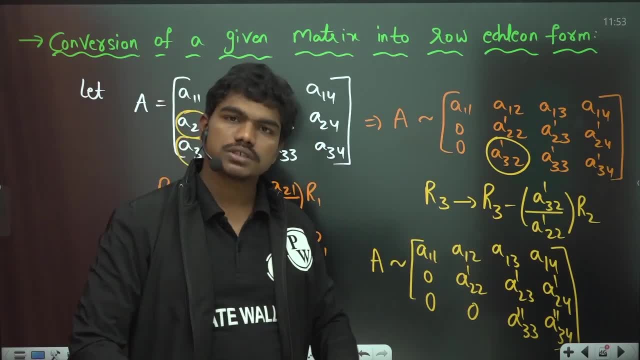 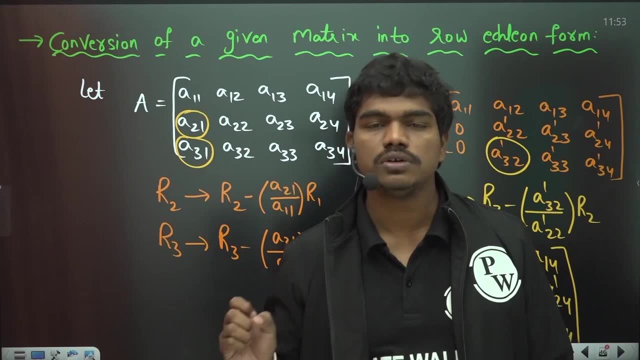 you are getting this denominator elements as zeros, then just swap those and try to avoid the zero division. that's it, okay. so now why we have taken so much pain in converting a given matrix into row, a cleon form. what is the relation between this row, a cleon form and rank of a matrix? 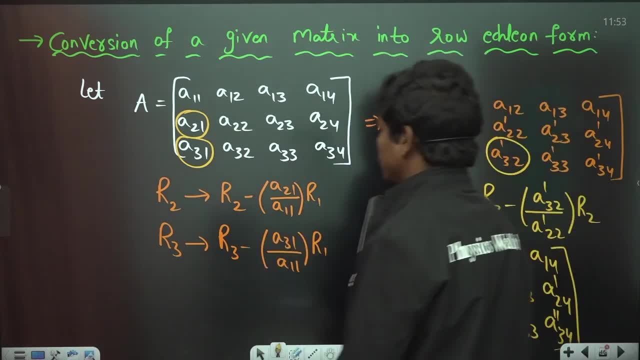 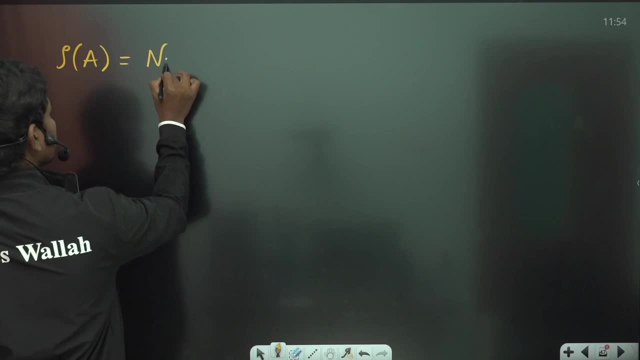 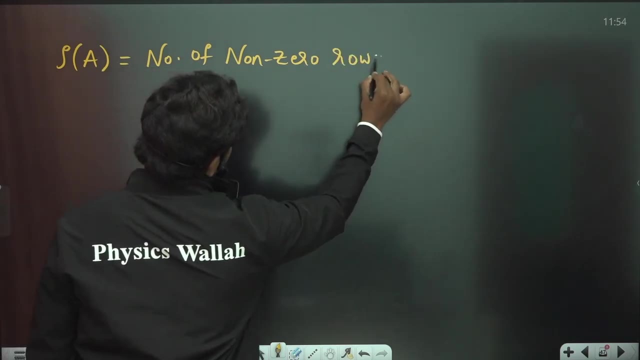 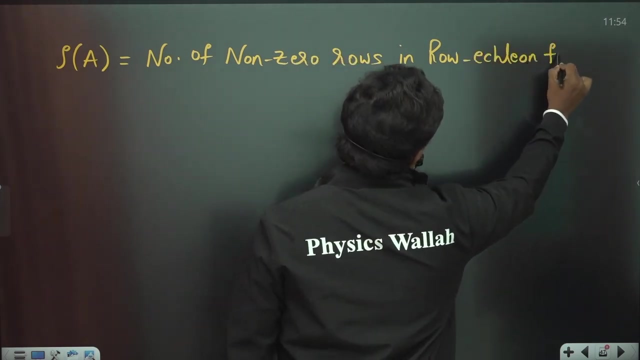 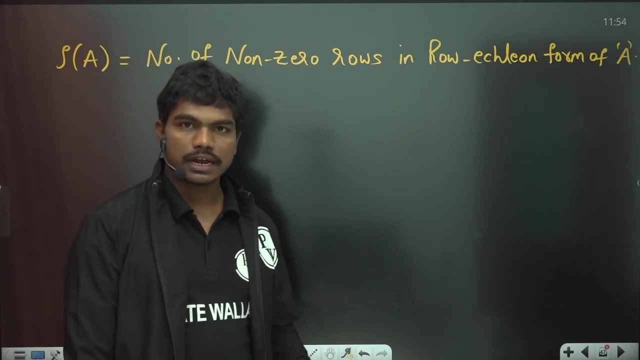 so, if you want to understand this, you will get this connection with this formula. rank of a matrix a is equal to number of non-zero rows: number of non-zero rows in row, a cleon form of a row, a cleon form of a, basically here. okay, so if you take a rank of a, that is basically equal to. 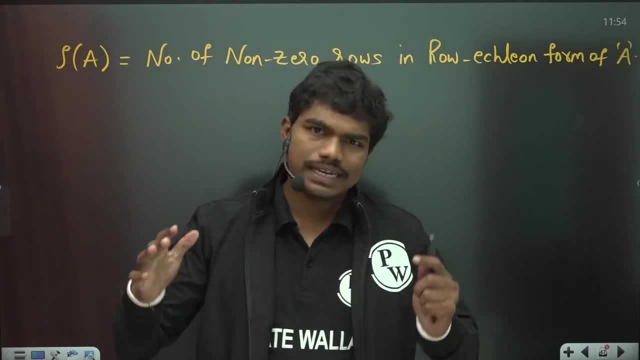 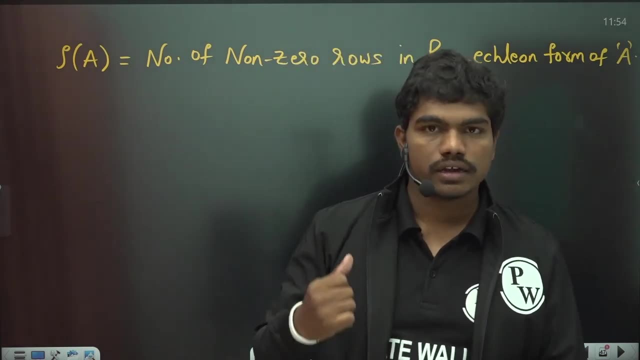 number of non-zero rows. okay. so once, independent of the size of the given matrix, if you can convert the matrix into, you know, a row, a cleon form, then definitely you can identify rank of the matrix very easily. clear, so that's one common thing again. so that's why we have taken so much. 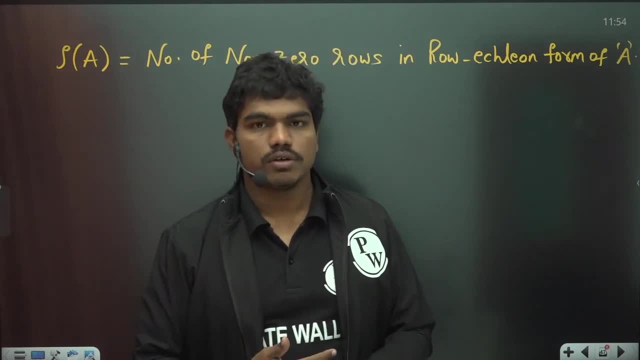 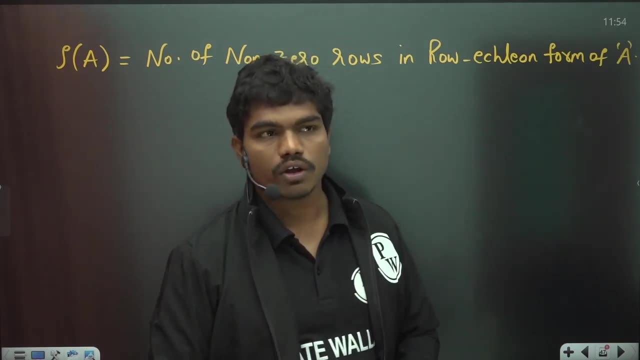 of pain in converting the rank of the matrix to you know, by knowing it's a row, a cleon form. now, one thing that i would like to tell here, why we have learned this concept of rank. as i told you to talk about system of equations, okay, so let us, without doing any time, okay, before going for that, 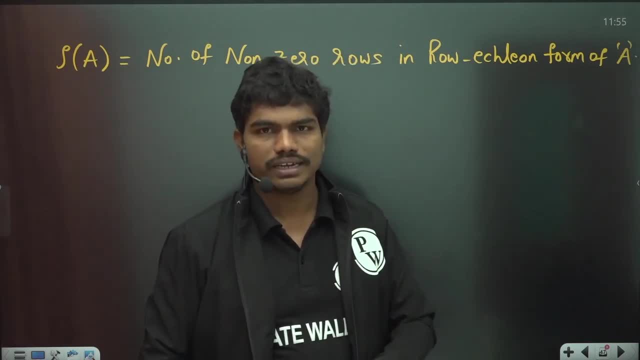 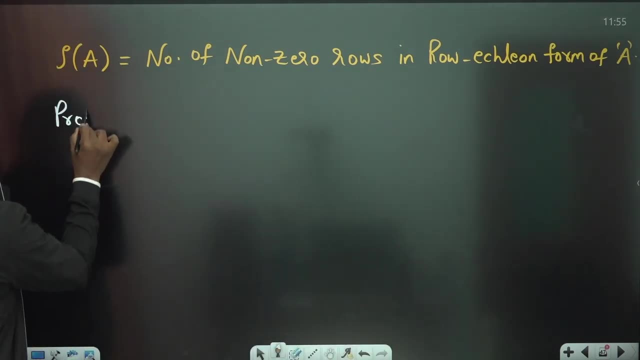 i would like to give you some properties of this rank of the matrix which could be, you know, helpful for you. so, first property, or i can say properties of properties of rank, you can write some two, three properties which are good. so, first, rank of a, m by n will be definitely less than or equal to minimum of m by n, m, comma n. 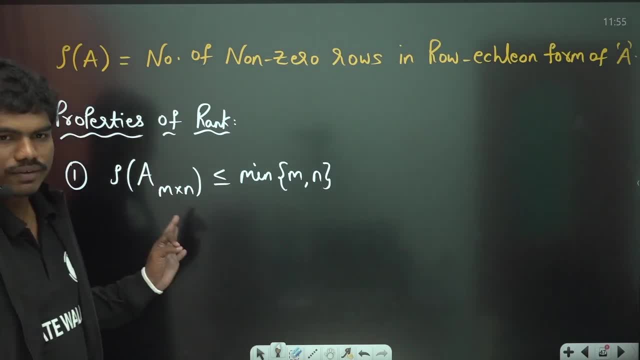 correct. so basically, we have seen, if it's a three by four matrix, at maximum rank can be three or maybe less than that, depending upon the minus being zeros or not. okay, so out of these two, which is minimum, the rank of this can be at maximum, equal to that or it can be less than that. 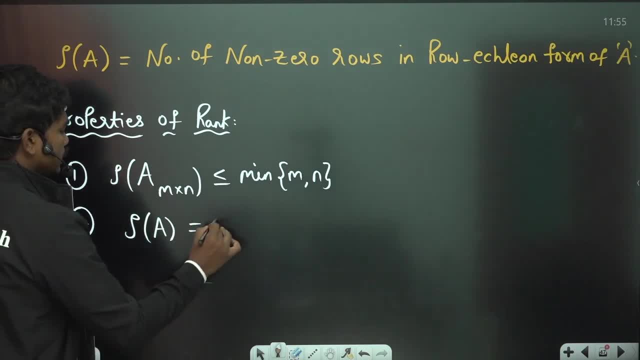 and similarly, you know, rank of a is always equal to rank of a transpose, because if you take transpose of them, okay. so that's the reason. and third, one very good property i would like to give you: rank of a into b will be less than or equal to minimum of rank of a comma. rank of this. 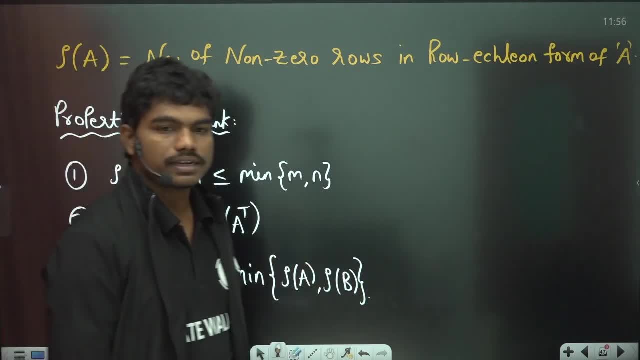 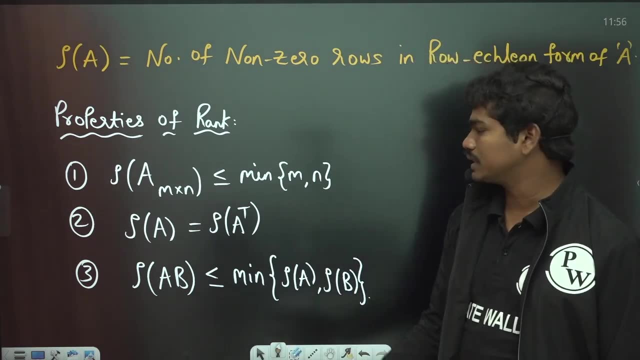 matrix b here. okay, so that's how. if you do the product of two matrices, rank of a multiplied with b, then this is less than or equal to minimum of rank of a comma. you know rank of b. so this, basically, are some good, important properties of rank of a and rank of b. so that's the reason why i 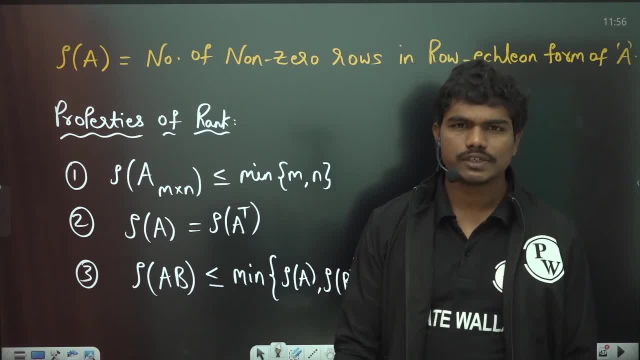 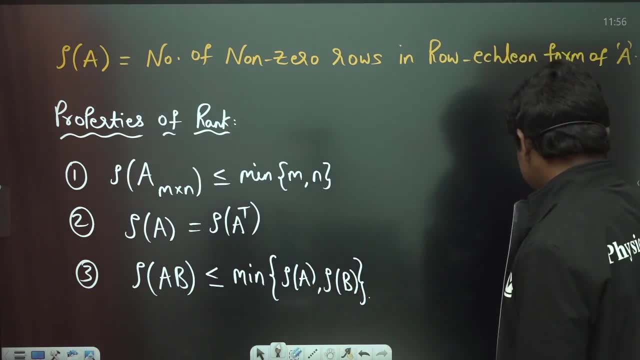 have given you the three properties, and especially the third property is somewhat, you know, uh, not very frequent, but sometimes it's good to know in gate examination when you're going for matrices. okay, so that's how we have this. the matrices now are three properties. now let 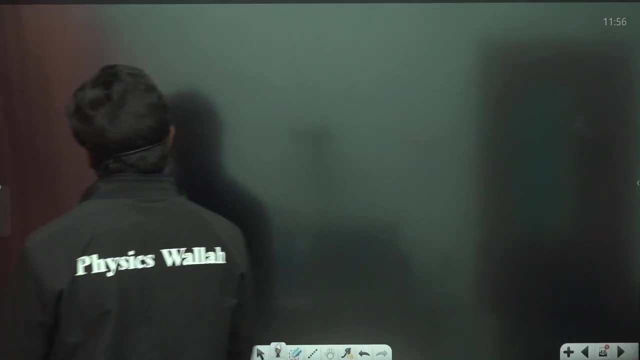 us go to one very important part of this linear algebra, the main core of this system of equations. system of equations, so almost i'm going to spend some 30 minutes of duration on this system of equations, so this is a very important portion that you all should actually- uh, you know- put some interest in. okay, so, system of equations, let us. 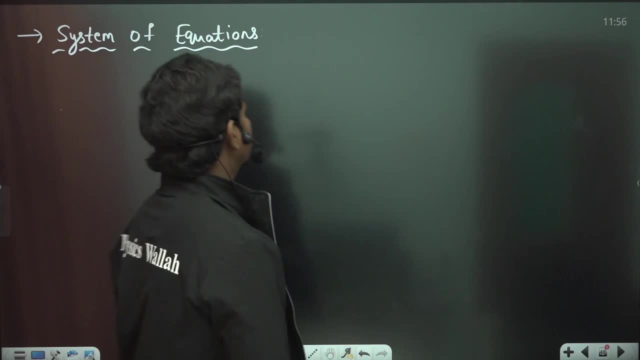 see what is this system of equations and how it actually helps you out. okay, so let us deal with the case of t by t, the equations with the unknowns. let us start because t by t is generally some not very easy, not very difficult also to deal with. okay, so let 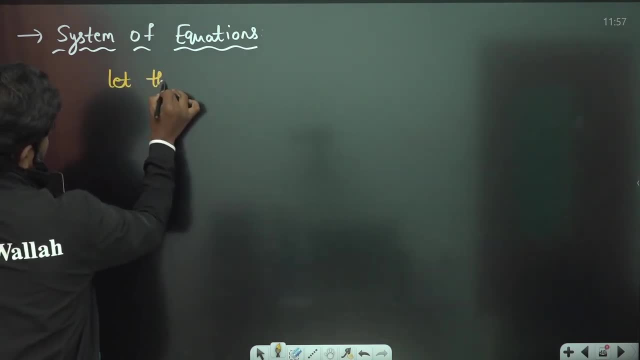 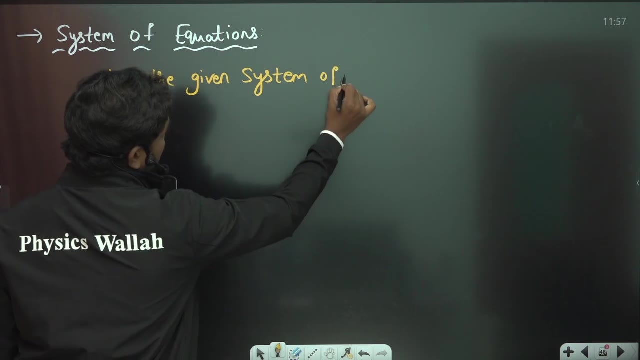 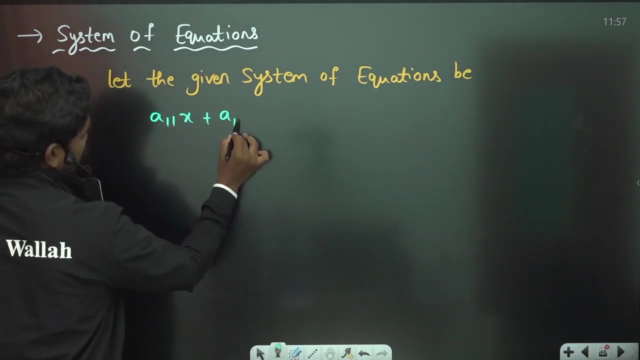 the given system of equations, let the given system of equations b. let us suppose you have three equations with the unknowns, so let me add them: a one one into x plus a one two into y, plus a one three times of z is equal to b1 a 21 times of x. 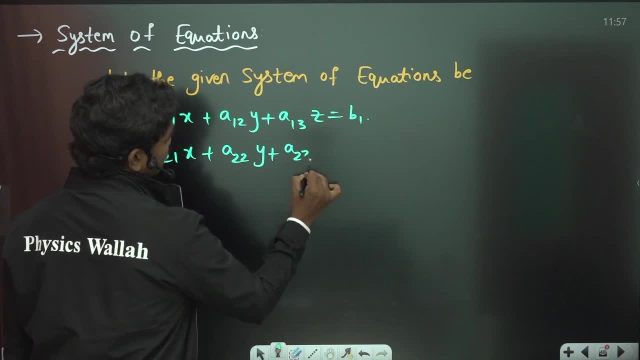 plus a 22 times of y plus a 2, 3 times of z is equal to b to a 31 times of x plus a a32 times of y plus a33 times of z is equal to b3. okay, so let us suppose these are the three. 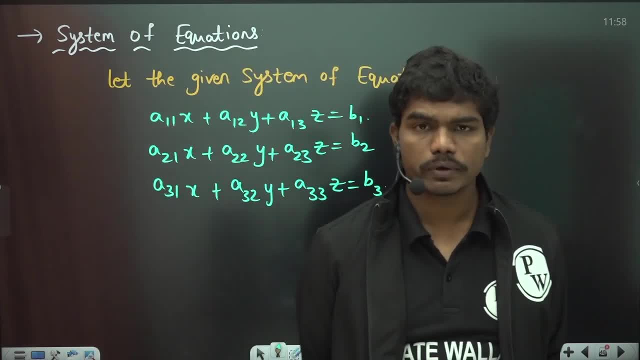 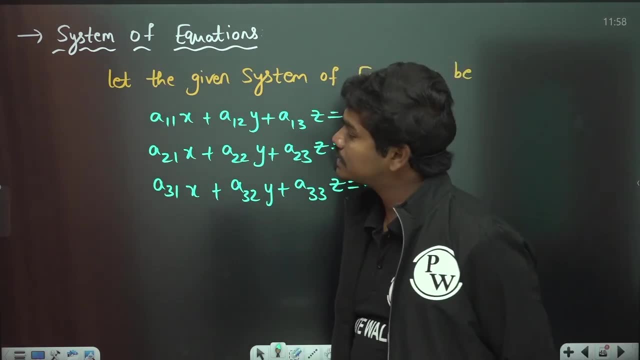 equations with the unknowns. now your job is rather than solving. okay, you have the techniques to solve. we have many methods, like gauss, elimination, all these things. but right now, let us suppose if you want to know whether this system of equations has a solution or not, okay, so means if you try to solve. 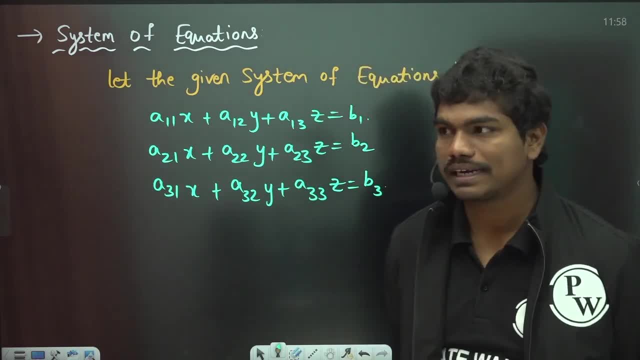 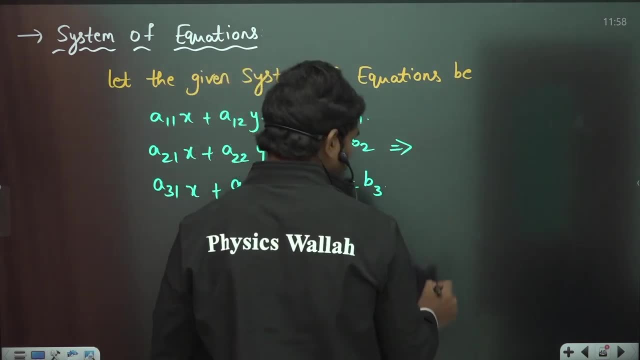 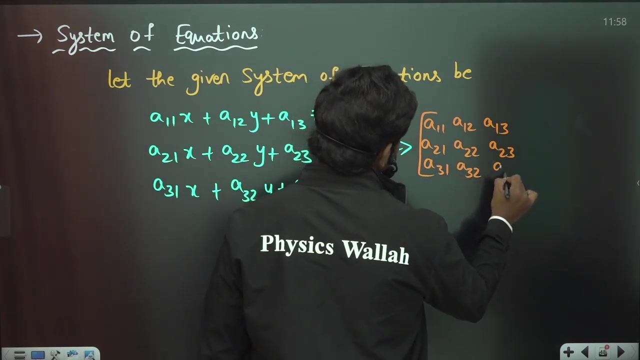 this equation. so will you get a solution? this is what you are interested to know right now. so, if you see, this same system of equations can be written as matrices like this, how come i can write this matrix: a11, a12, a13. this is a23, a32, a33. this if you multiply with this matrix. 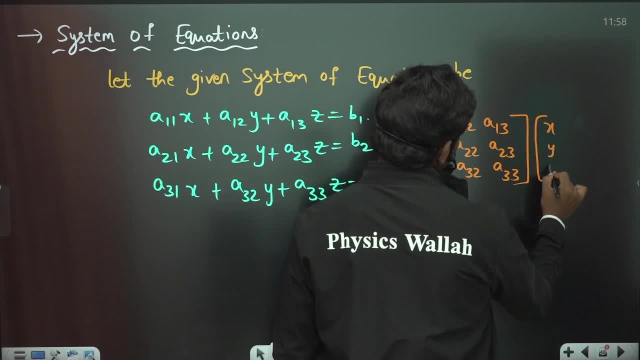 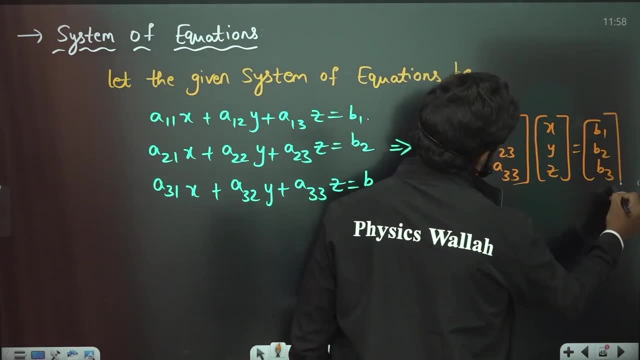 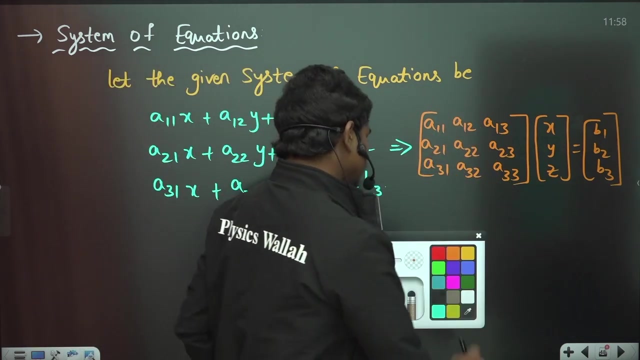 x, y, z is equal to b1, b2, b3. so this is how you can actually write this system of equations into this matrices. how come? because, if you see, this is a size 3 by 3. this is of size 3 by 1, so obviously. 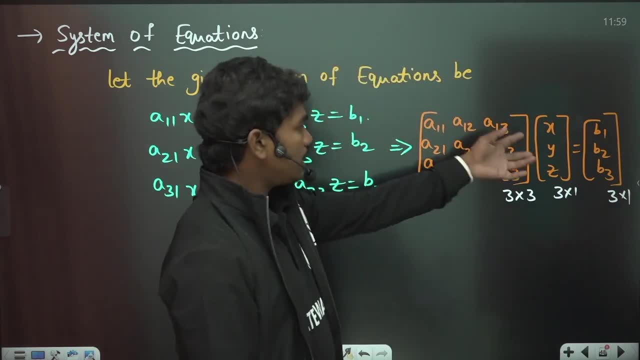 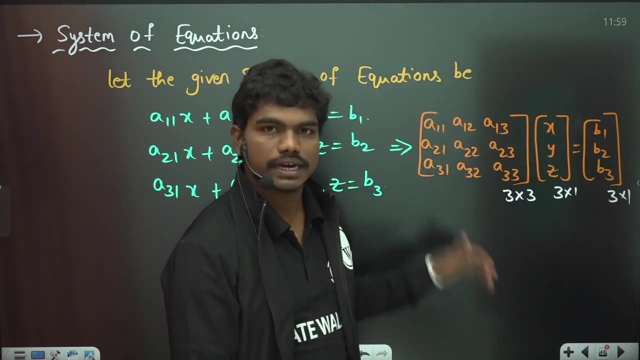 this product is of size 3 by 1. now if you check this, if you multiply these two matrices on the left hand side, a11 into x plus a12 into y plus a13 into z, this is what you will get as the first element, first element second, of a21 into x plus a22 into y plus a23 into 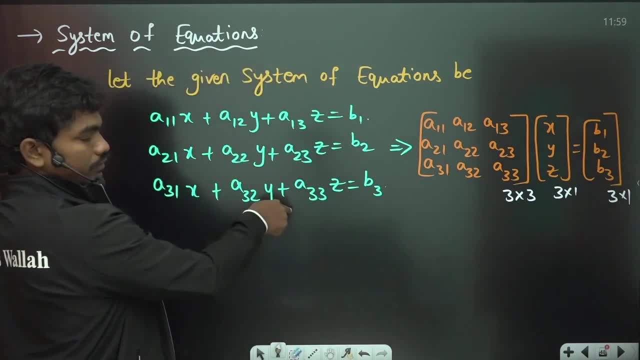 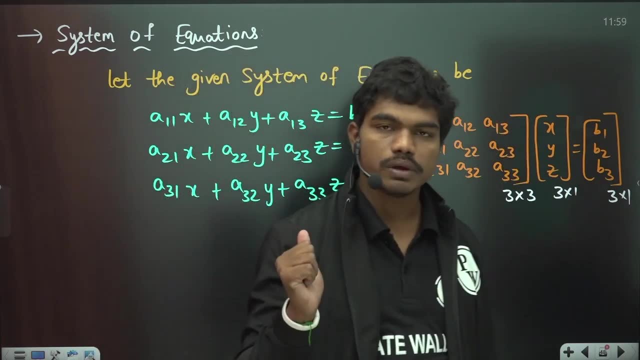 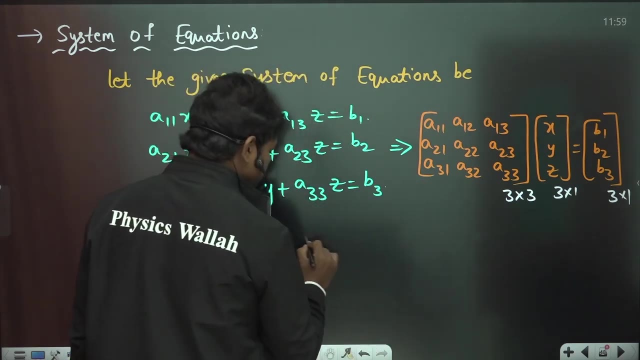 z. similarly, third one. so if you see, these left hand sides of the equations are nothing but the elements in the matrix, multiplication of these two matrices. okay, so that's how this given system of equations can be, you know, converted as a product of basically some matrices. okay, so this can be written as: a into x is equal to b, so this system of equations can. 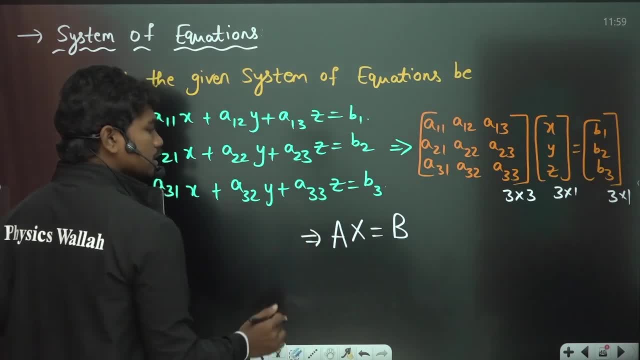 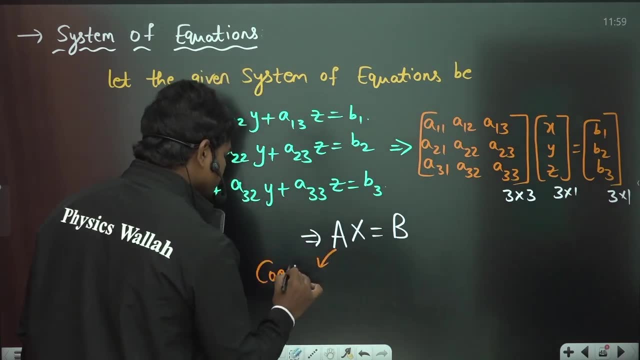 be written in terms of some matrices. okay, so this can be written as: a into x is equal to b. where a is called this capital, a is called coefficient matrix, coefficient matrix. so why it's called coefficient matrix? because you see, clearly, this is basically your a and 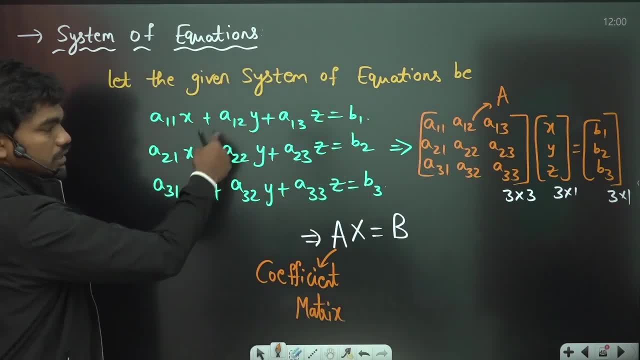 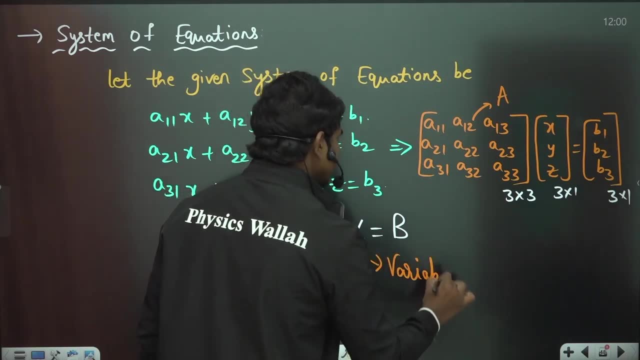 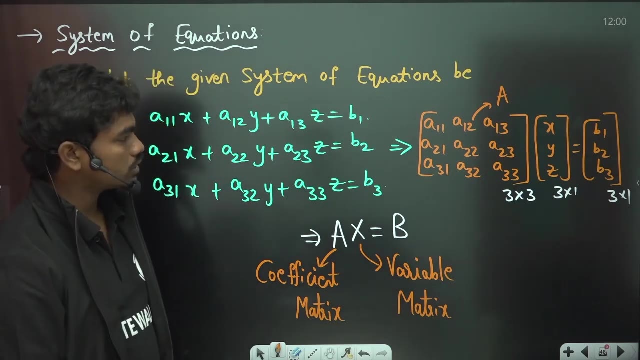 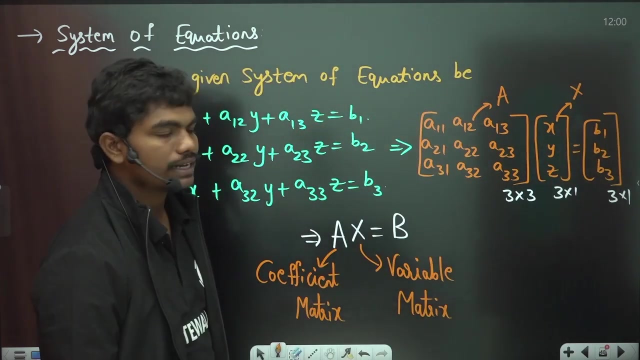 this matrix is formed by the coefficients of the variables in this equations. next, this x is called a variable matrix. variable matrix, okay, so variable matrix, because that this x capital x. i am denoting this, this capital x is basically here. uh, you know, the matrix containing all the variables involved. 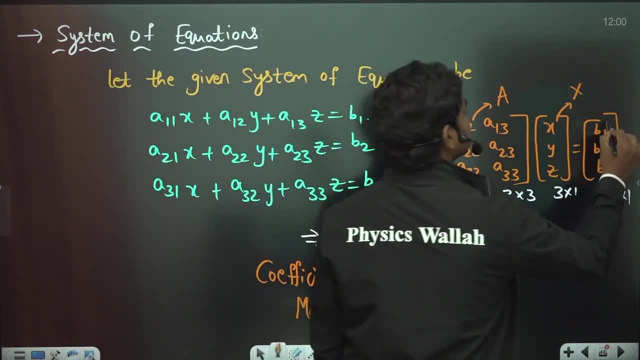 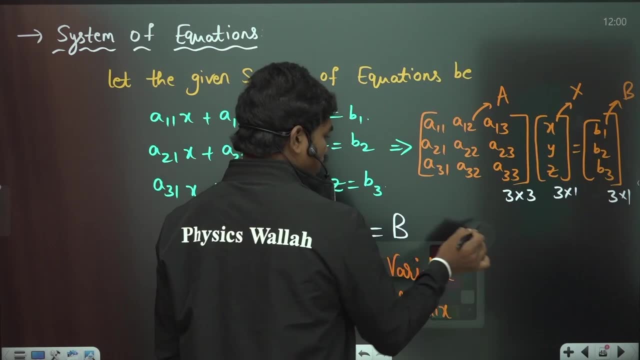 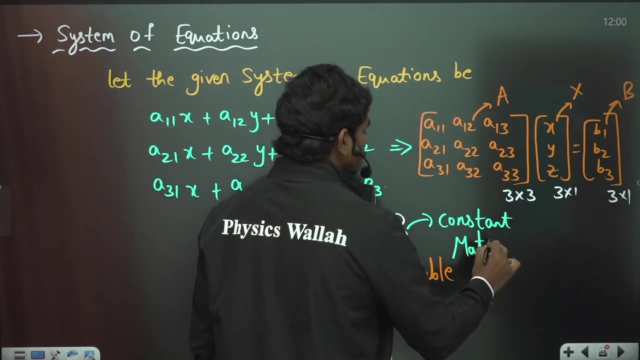 in the equations. so this is variable matrix. similarly, this is b. so if you see this, b is basically a constant matrix. these are the constants on the right hand side. so this is is called constant matrix, which many of you have seen cut. so now people will tell. if you want x. 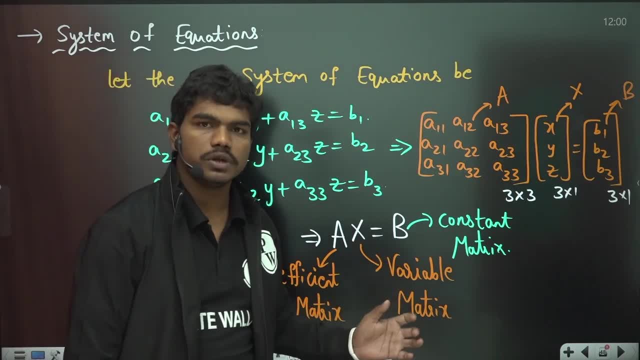 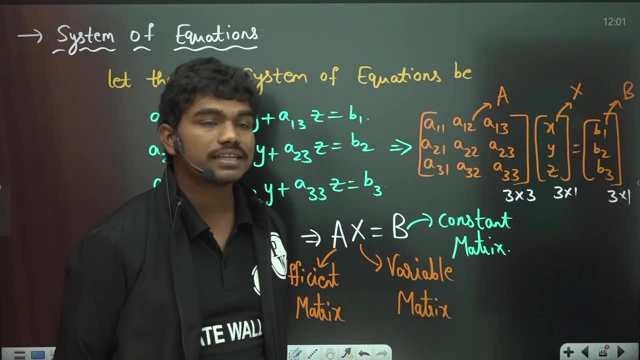 then x is equal to a inverse into b. you have one method, you have karma. so you have gosh, jordan, goss, elimination. they have n number of methods. okay, but my job here right now is not to find the solution, but to know whether these equations have a solution or not. okay, 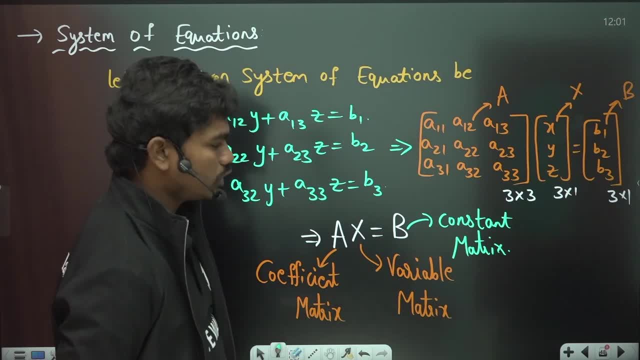 so let us see what, how we can do this. so ax is equal to b. now a system and you can see carefully. here these equations are non homogeneous equations. y it's as it has been programmed here. yeah, you can see that a and y is equal to b. now the system and you can see carefully. 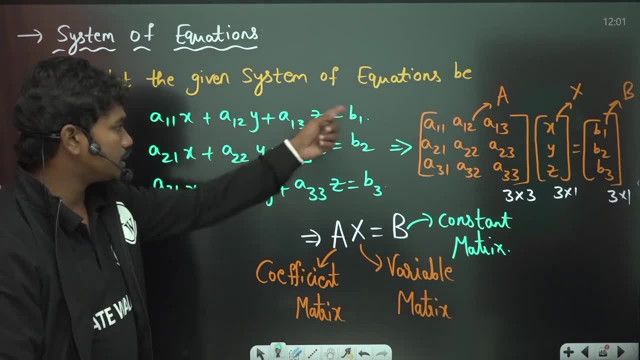 here these equations are non homogenous, equations y, it's not non homogenous and you can see it is equations. why, if you take this equation, this is first degree equation, because first degree term, because here you have a power one, here also you have a power one, here also you have a power one. 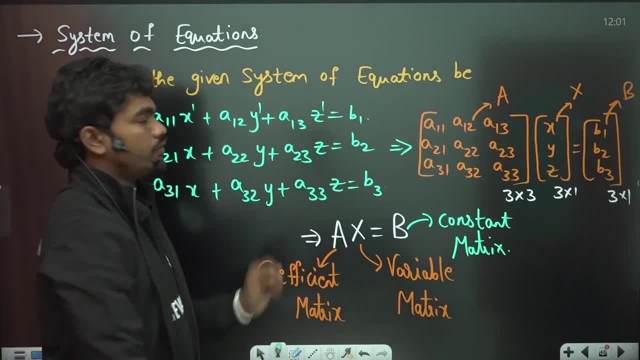 so all these three have power one, but here the power is not equal to one. for example, if you write this: z power zero, or x power zero, anything the degree is zero. so all the four terms of this equation don't have a same degree. so that's why this is called non-homogeneous equations, okay. 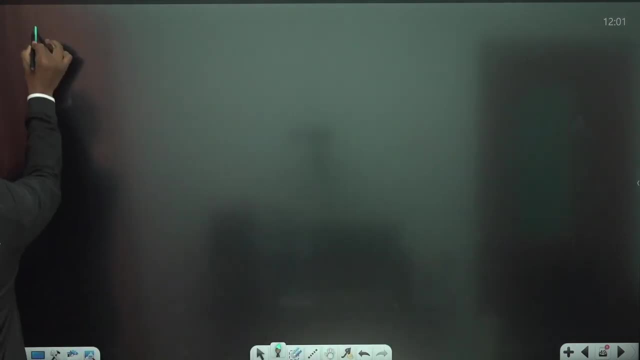 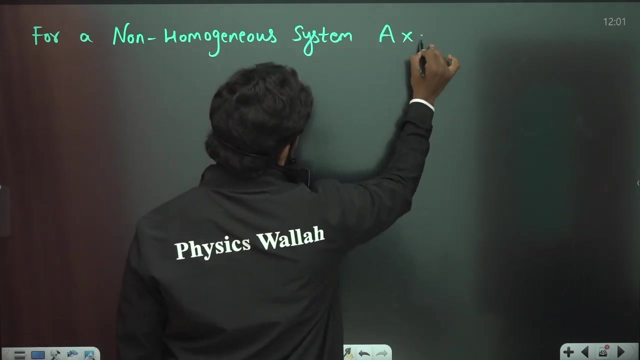 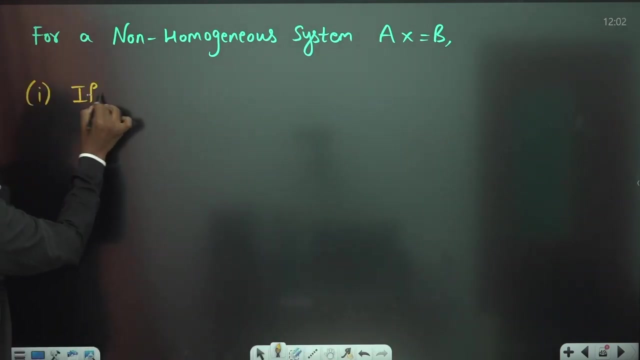 so let us write for a non-homogeneous system. for a non-homogeneous system, ax is equal to b, ax is equal to b. first case: if rank of a is equal to rank of a slash b, we'll see what is this a slash b. this a slash b is called the augmented matrix. okay means basically: 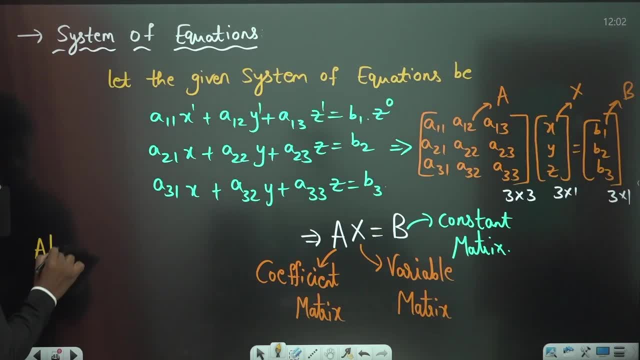 if you write a slash, b, augmentation means addition, okay, so a 1, 1, a, 1, 2 a, 1, 3 a 2, 1 a 2, 2 a, 2, 3, b. i mean, sorry, a 3, 1, a, 3, 2 and a 3, 3, for example. so if you take this, then b. 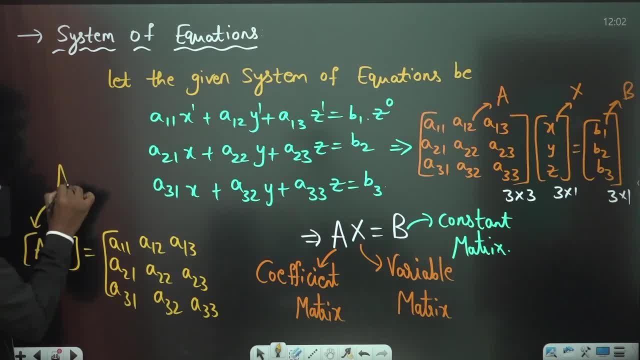 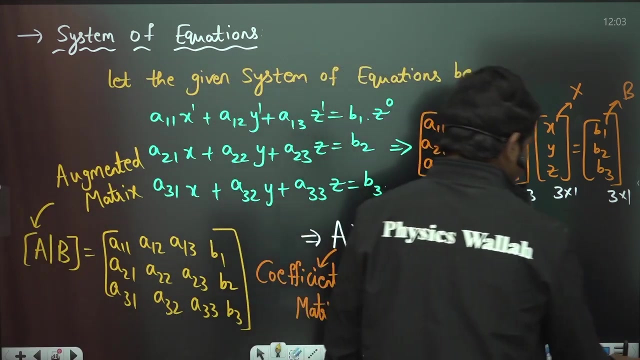 augmentation, augmentation. this is called basically augmented matrix, augmented matrix, augmented matrix, for example. so augmentation means addition, means you will add the column b to this matrix. so b 1, b 2, b, 3, this is how you will have your augmented matrix, basically 3 by 4 in this case. okay, so this is the augmented matrix. so now if 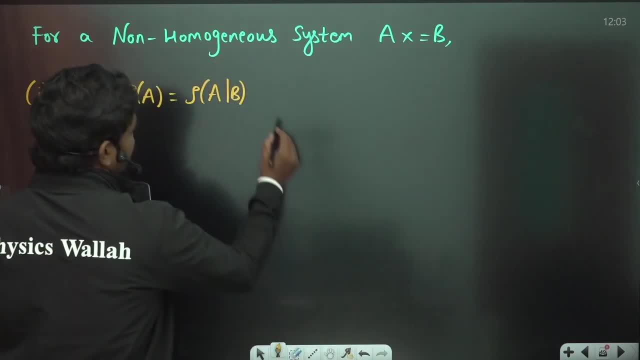 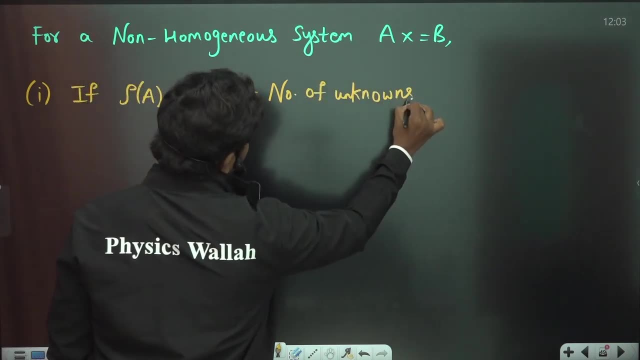 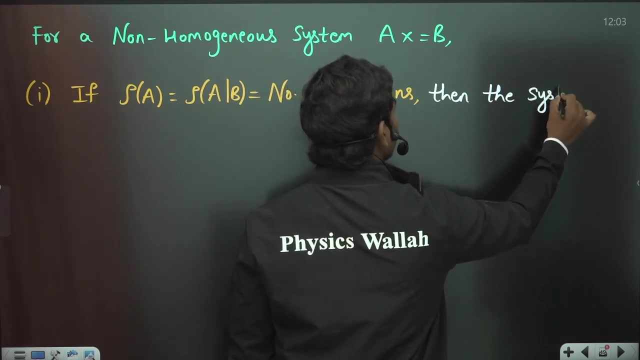 you see, if this rank of a is equal to rank of a, augmented b is equal to number of unknowns. in the equations here you have three unknowns, basically, so number of unknowns. if this happens, then the system has unique solution, means it will have only one solution then. 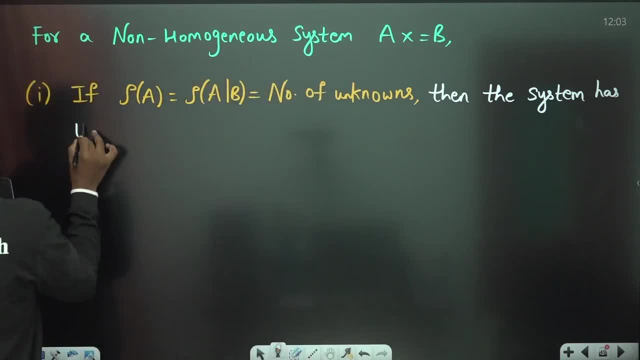 the system have other than system has unique solution. unique means only one solution. unique basically one solution. unique means basically one solution. now, it could be possible in that case if a rank of a is equal to rank of a augmented b, but this time both these values are less than number. 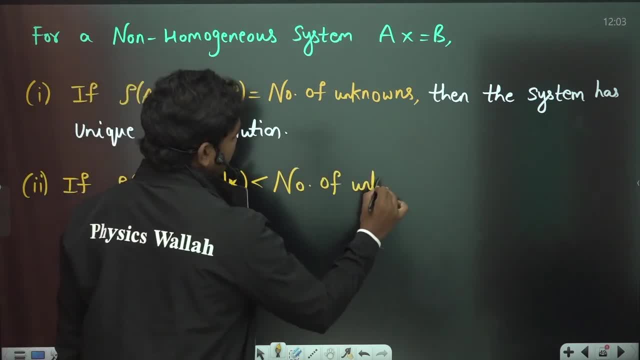 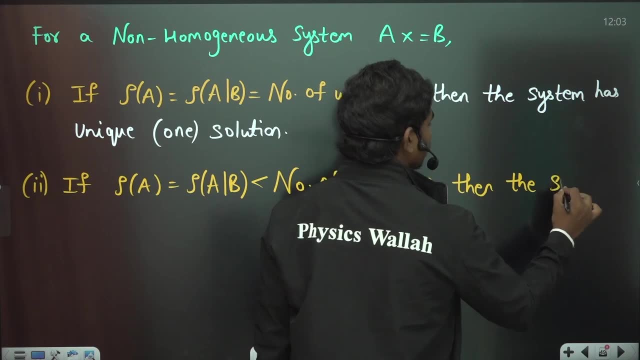 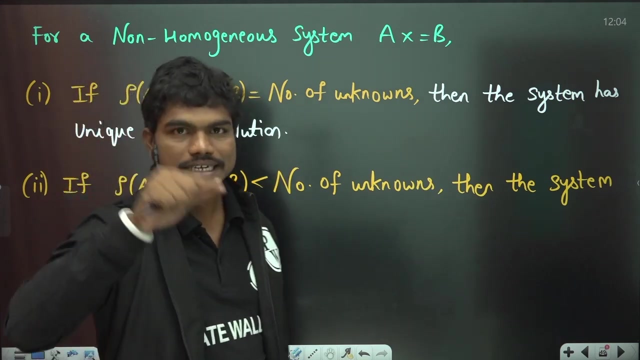 of unknowns, less than number of unknowns, then the system has. i'll take examples of each. these three cases total. there are three cases. i will take examples. i'll show you geometrically what is happening when you, when these conditions gets hold. okay, so then the system has. 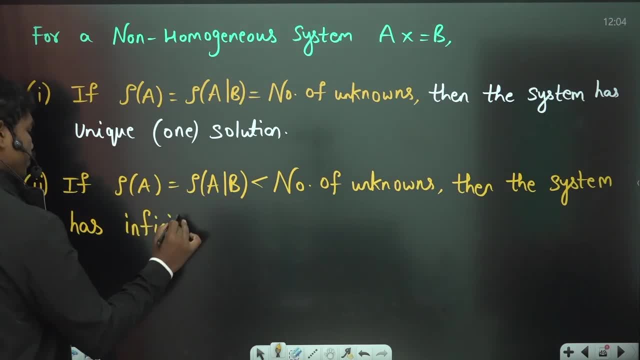 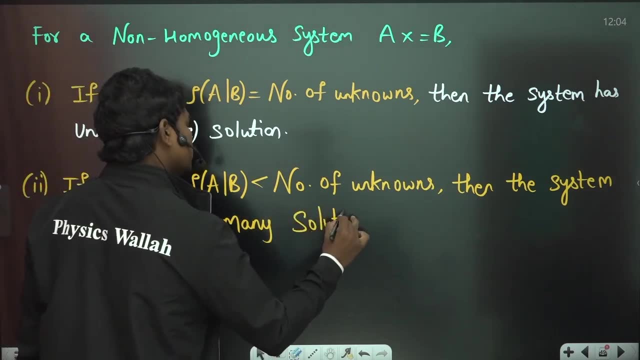 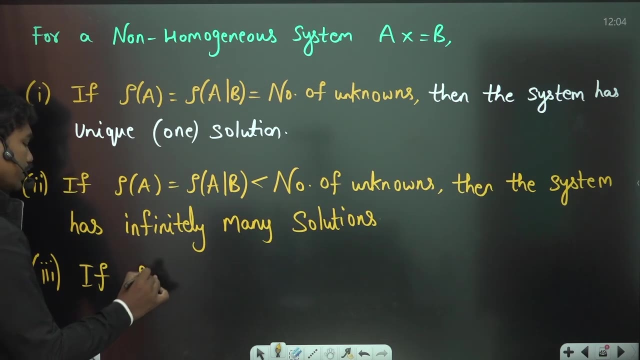 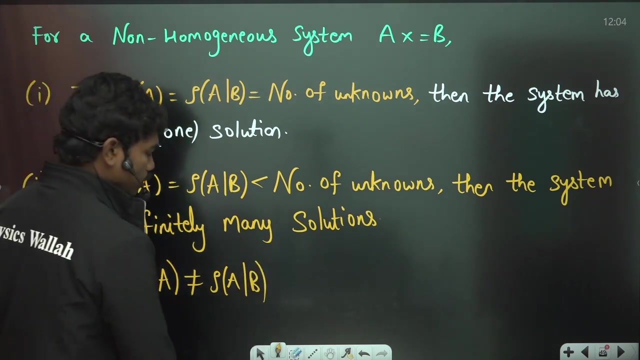 infinitely many solutions, infinitely many, infinitely many solutions. and third, if rank of a is not equal to rank of a augmented b, i'll show you how these three cases can come. so if rank of a is not equal to rank of a augmented b, then the system has no solution. then, 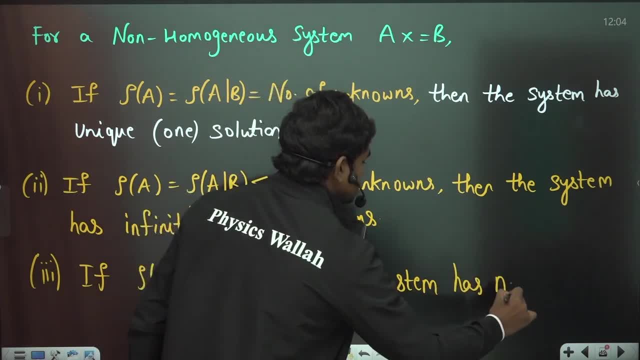 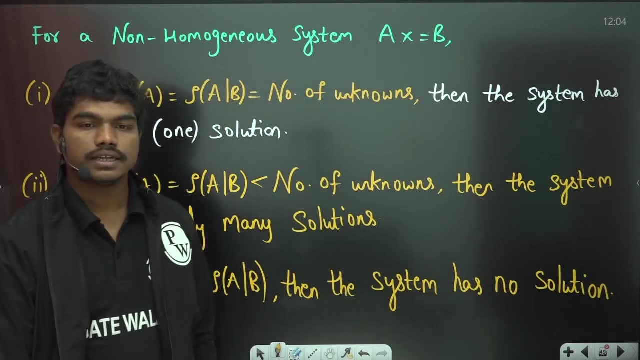 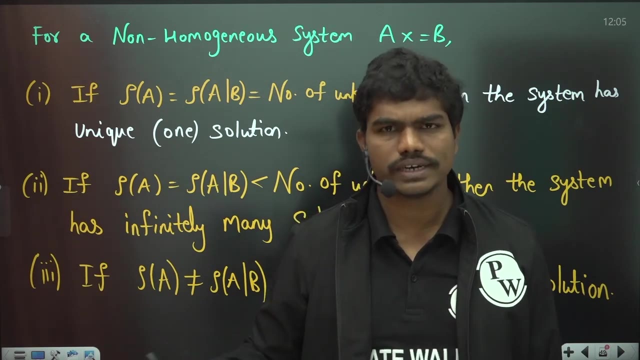 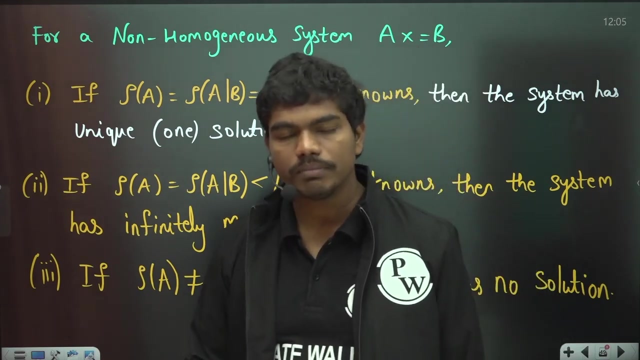 the system has no solution, basically here. okay, then the system has no solution. how we can have this kind of systems? basically, when you have a system with only one solution, normally when you solve two equations you will get some solution. how a system can have infinitely many solutions? how a system can have zero solution? let us see the cases of each of them. 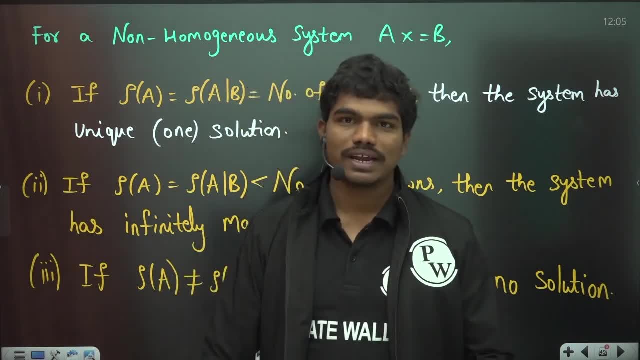 and let us try to understand. i hope this is a very long video, so i expect you to be patient and let us try to understand. i hope this is a very long video, so i expect you to be patient, because obviously it's a, you know, very short time and uh, forget 2023. so definitely you. 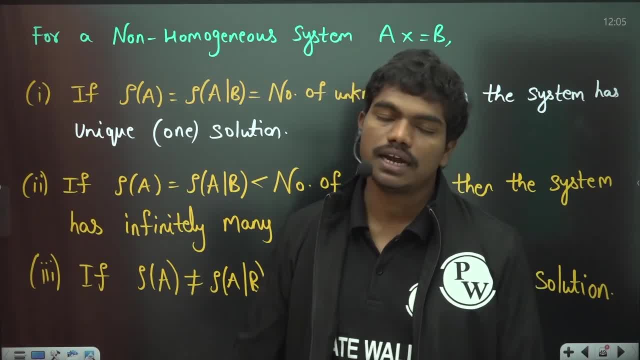 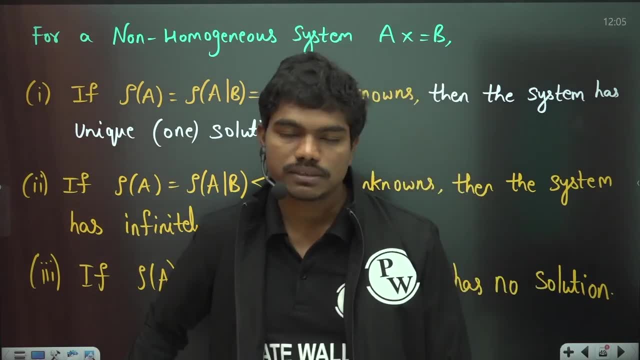 need to, uh, spend some good time on this mathematics, because started with 13 marks and unknowingly or indirectly you can say many other marks will be coming from this engineering math subject. i have taken this first video to be on linear algebra because you will feel little. 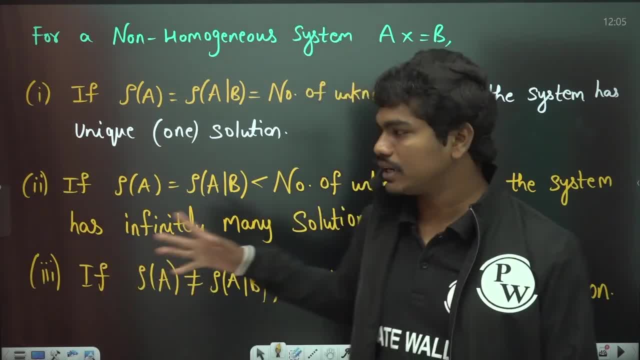 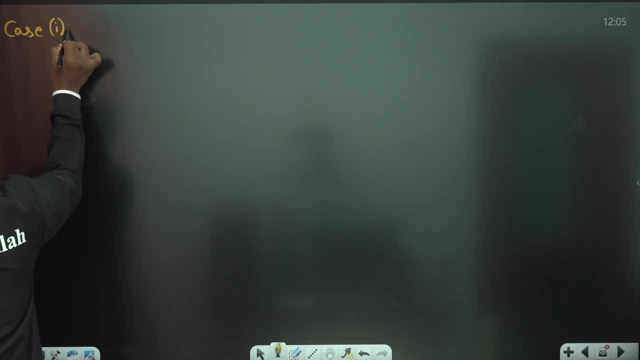 comfortable, and next video we are going to make on basic calculus. okay, so anyhow, let us see here continue. so case one: let us suppose i give you two equations. this one, let us suppose i will give you two equations. this one justice, this hypothesis, this rules, weather conditions or other condition of the 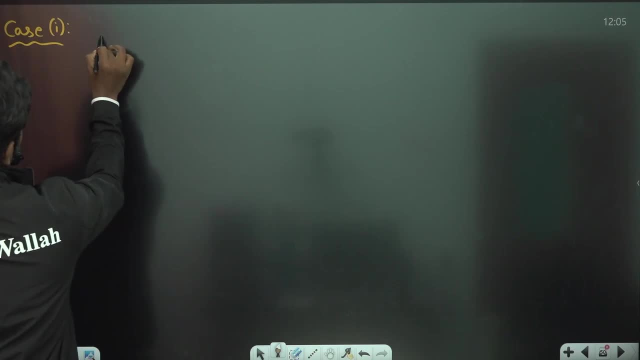 Let us suppose I have given you two equations. for example, 2x minus y is equal to some 7, let us say: and for example some another equation: 3x plus 2y. let us say so 3x plus 2y is let. 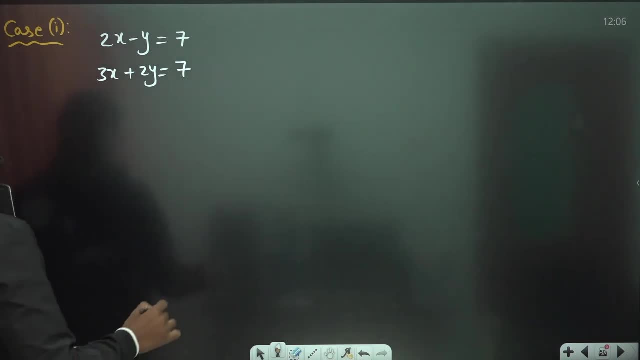 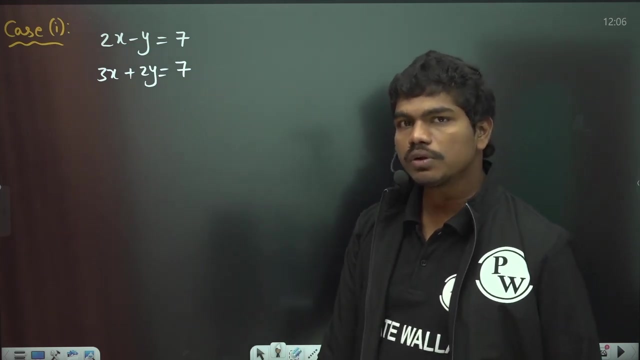 us suppose again it is 7. okay, so if you take for example, let me calculate this. okay, fine, so let us suppose 2x minus y is equal to 7 and 3x plus 2y is equal to 7. okay, it need not be 7 and 7 here in this case. it got happened, okay, now, definitely, you know one thing: if 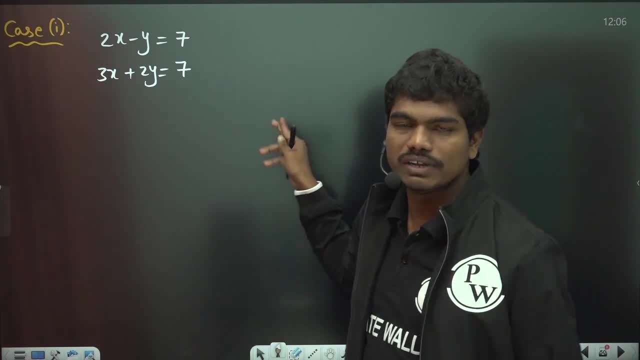 you form this. I am dealing with 2 by 2 because I want to show geometrically. also, if I want to take 3 by 3, then I will need to talk with planes and all. so it will be little complicated. so right now I am explaining with 2 by 2 so you all will understand. now let us suppose 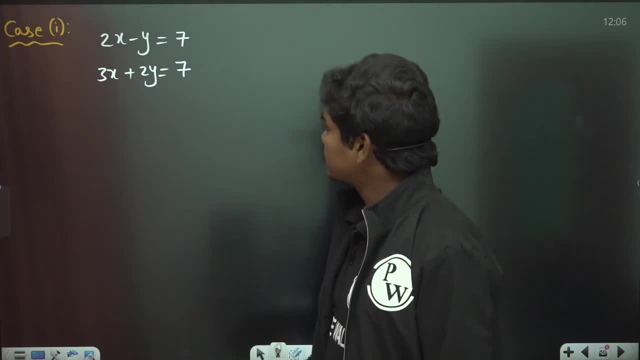 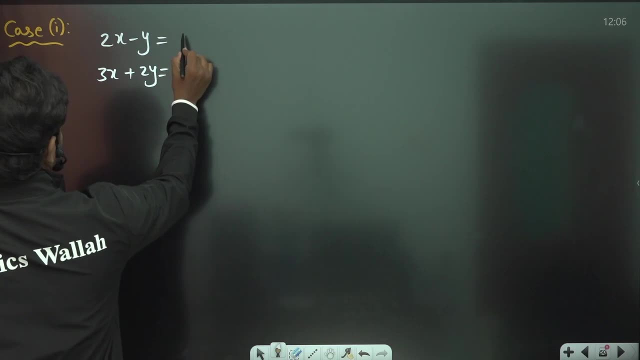 if you want to. you know, like this, basically, shall we make the equation simple a bit. let us make this constant 2 by 2.. and simple a bit. so this is 3, this is 8, let us take, for example. okay, so we, I just want. 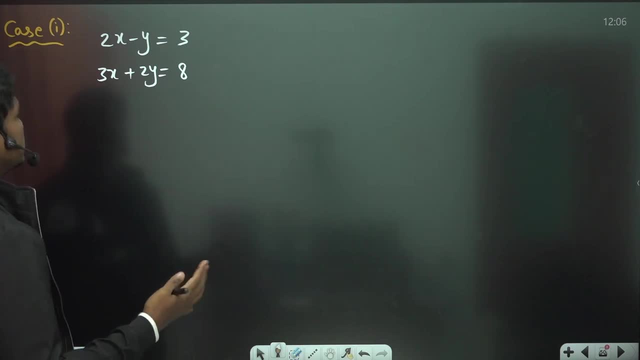 to make the equation slightly simple. so, yeah, this is fine now. so if you see this equations, now let us try to convert this equations into matrices. okay, so if you see, a is equal to coefficient matrix, basically, what is the coefficient matrix? 2 minus 1, 3, 2, b is 3, 8 and, of course, 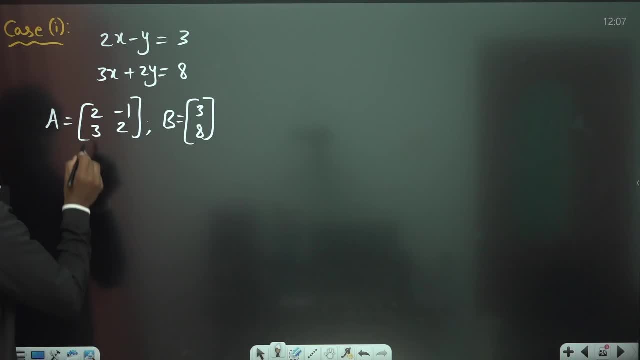 capital X is equal to 2 minus 1, 3, 2. b is equal to 3, 8 and, of course, capital X is equal to x, is x, y. now, if you calculate determinant of a, that a is equal to 4 minus of minus. 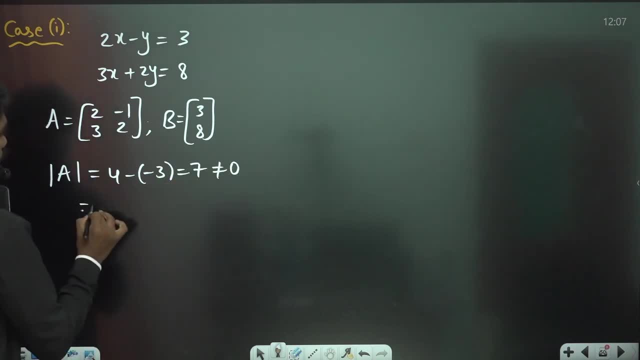 3, which is 7, so which is not equal to 0. so therefore, rank of a is equal to 2. that is clear. now a augmented b is how much? a augmented b is 2 minus 1, 3, 2, 3, 8. so definitely this. 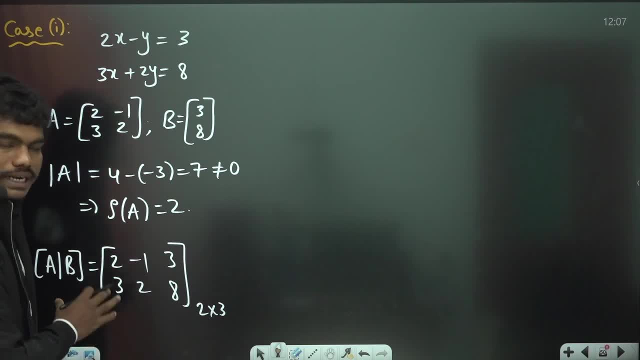 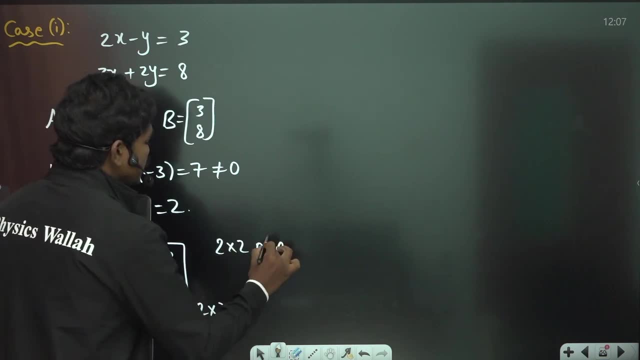 is a 2 by 3 matrix, so the maximum second order miner you can take out of this matrix is 2, this second order. so if you write 2 by 2 minus 2 by 2 minus direct claim writing, so if you write 2 by 2 minus the first minor will be 2 minus 1, 3 minus 2, so which is, oh sorry, 3 plus 2, okay. 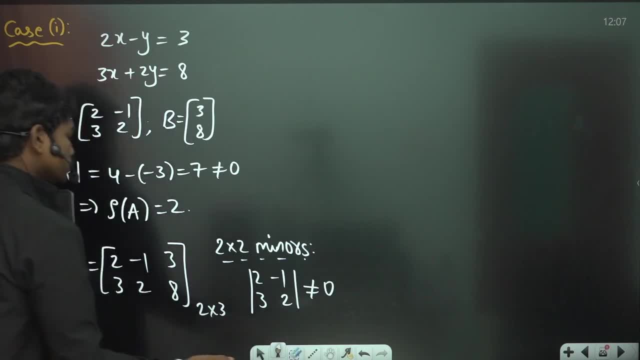 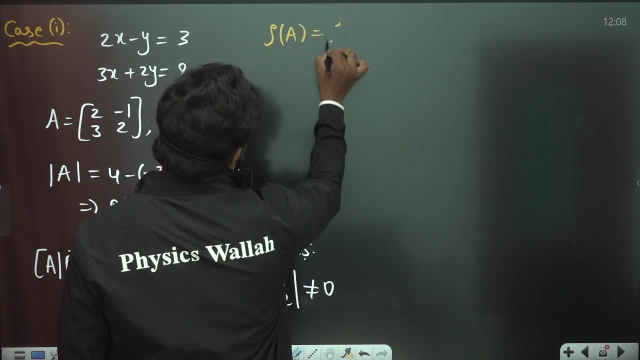 so this is plus 2 and obviously you know this is not equal to 0. so because that's same as the determinant of a, which means one thing you got here is very clear: rank of a is same as a rank of a augmented b and of course this is equal to 2, and here 2 is nothing but number of unknowns in. 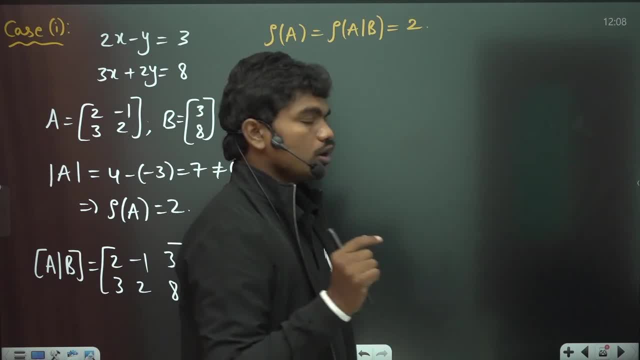 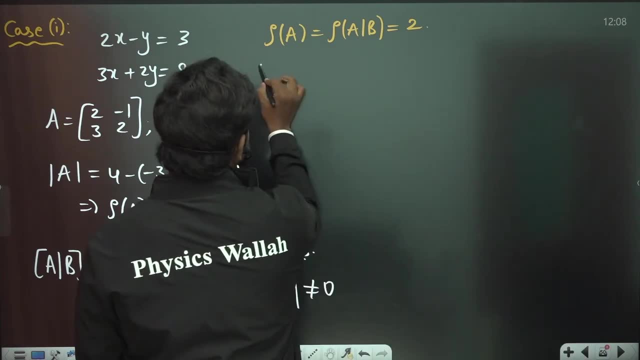 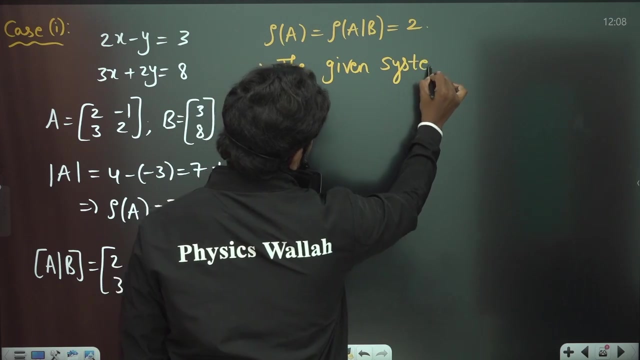 this equation correct. so now, if you see rank of a and rank of a augmented b, both are same and of course, these two are equal to the number of unknowns in this equation. so therefore, the given system has a unique solution. the given system has unique solution. 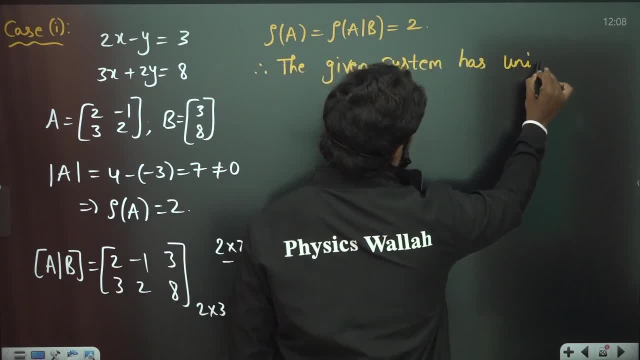 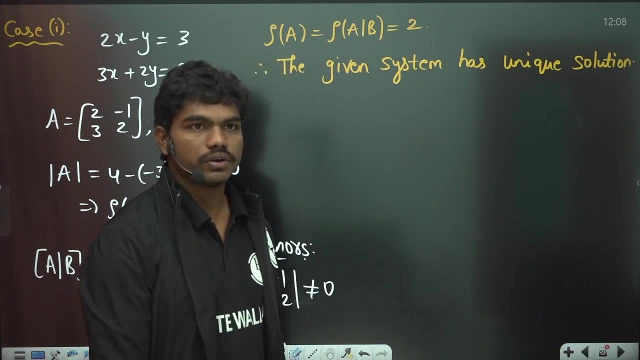 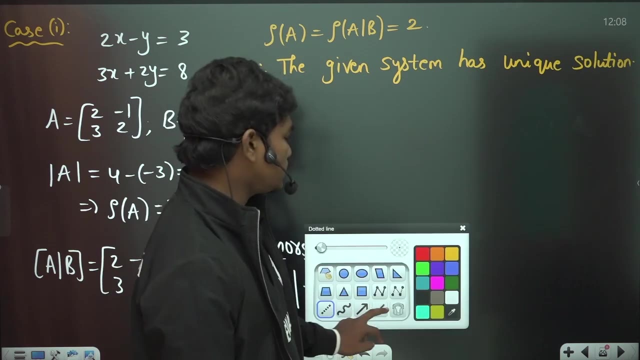 the given system has unique. the given system has unique solution. okay, so the given system has a unique solution. basically, here now try to understand one thing: number given unique solution, now how do i know that it has unique solution? so, basically, if you see geometrically i told you i'll talk about. so these two are the equations, are two linear. 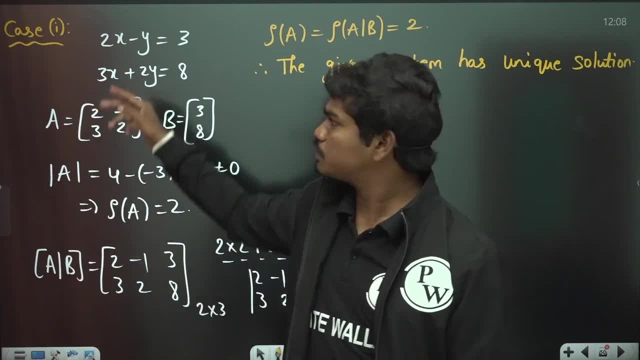 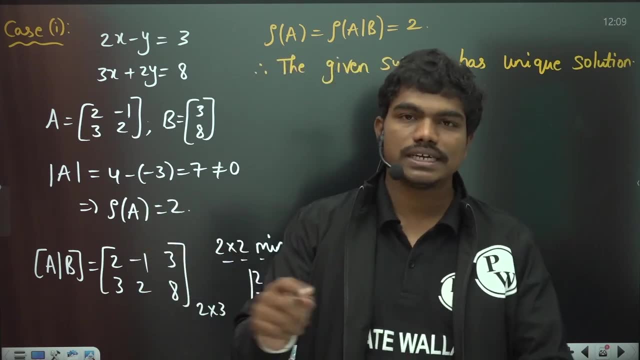 equations. so if you try to plot them you'll get straight lines, correct? let us try to plot these straight lines and let us find at how many points they are intersecting. okay, so, because solution mathematically means geometrically the point where the two lines meet each other, correct, or? 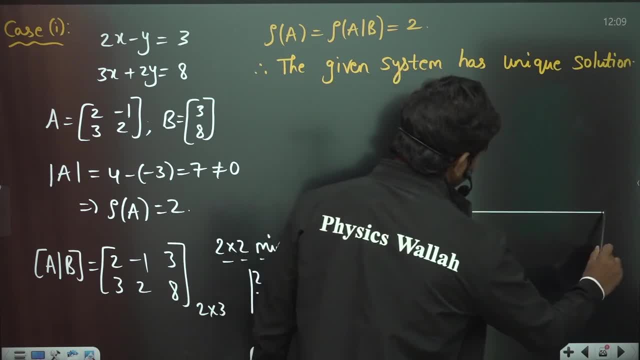 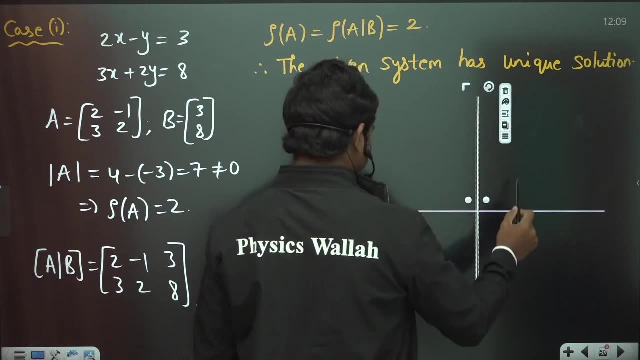 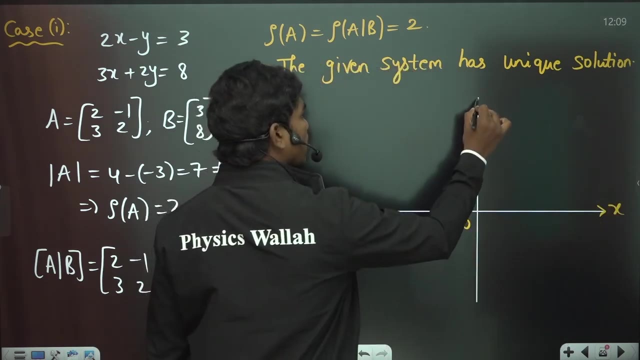 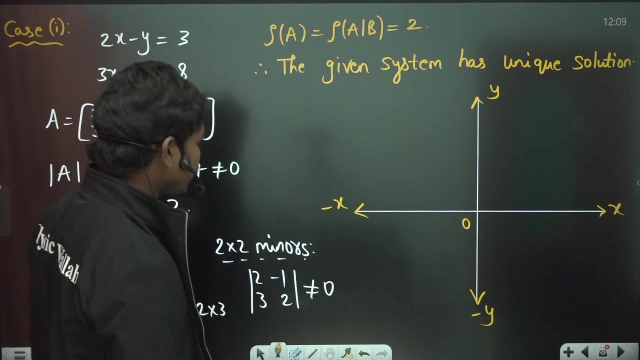 they cut each other. so now, if you try to plot these points, this is x and let us suppose this is y, for example. okay, so this is your y, or is it x minus x, y and minus y? now try to form this line: 2 x minus y is equal to 3. so if you write this: 2 x minus y equal to 3, this equation can be written as y equal to 2x minus y and x. casa of x as a sum. this equation can be written as y equal to 2x and x as a sum. 때� to form this line: two x minus y is equal to 3. so if you write this: 2 X minus y equal to 3, this equation and witness: y equal to x minus y, A and A. 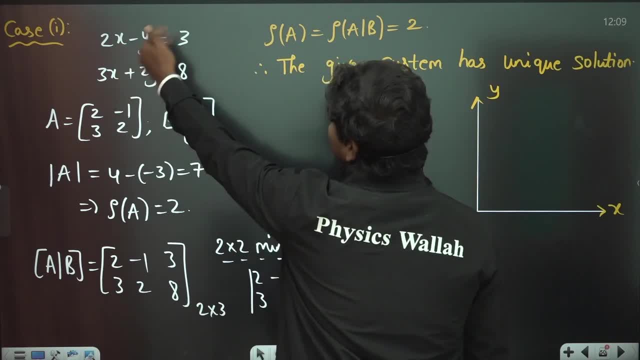 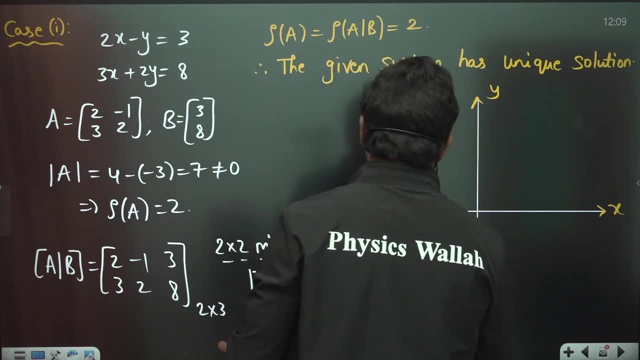 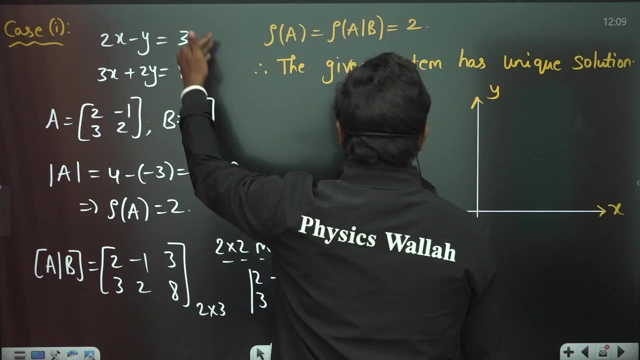 start, this equation can be written as y equal to 2x plus 3, correct? so if you see, basically, if you want to plot that line, so let us find the x coordinate. so if you want the point on, you know x axis, if you put y equal to 0, x equal to 3 by 2, so this is the one point, this is one. 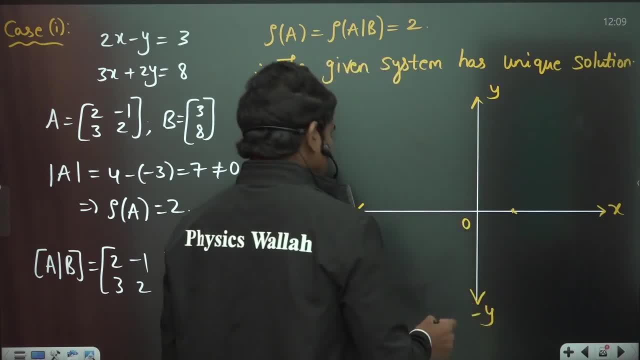 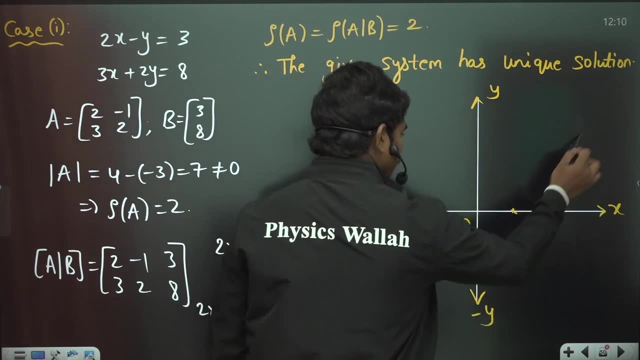 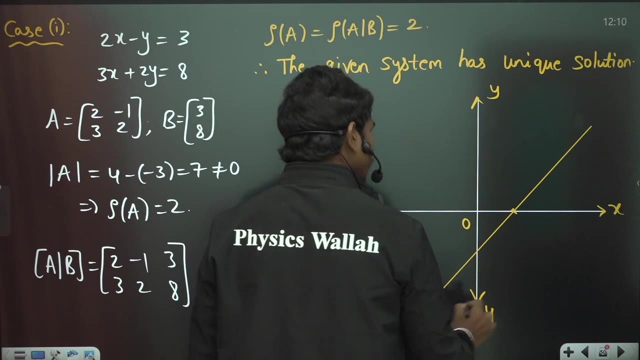 point. and if you put x equal to 0, y equal to minus 3, so the line is something like this: so, okay, let me change the ink so you can understand better. so this is one line where- okay, fine, so this is the equation of the line: 2x minus y is equal to 3. 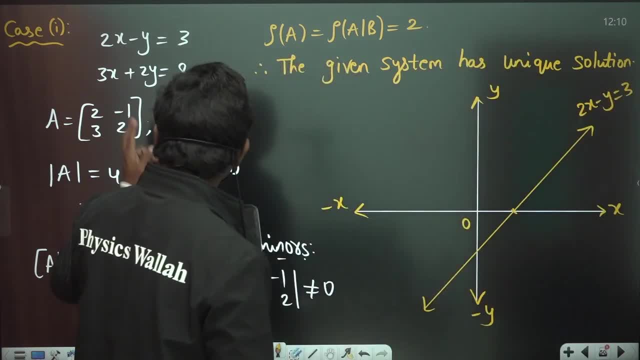 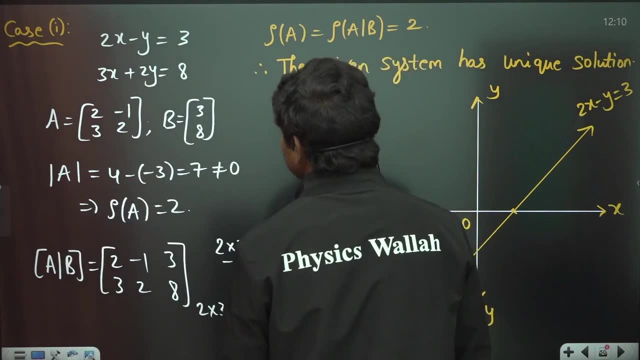 and next, if you want to plot the other line, 3x plus 2y is equal to 8, so y is equal to 4. generally, when you do this, and x is equal to x is equal to 8 by 3, so x equal to 8 by 3 and y is equal to 4. 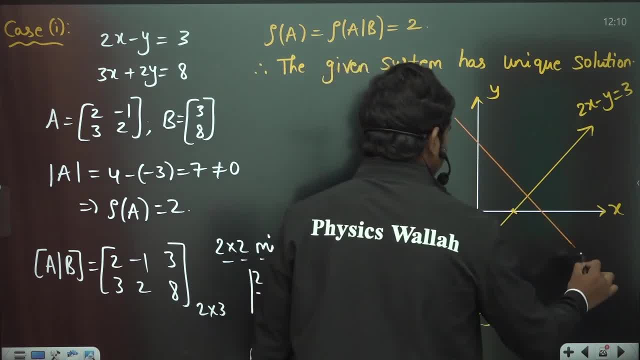 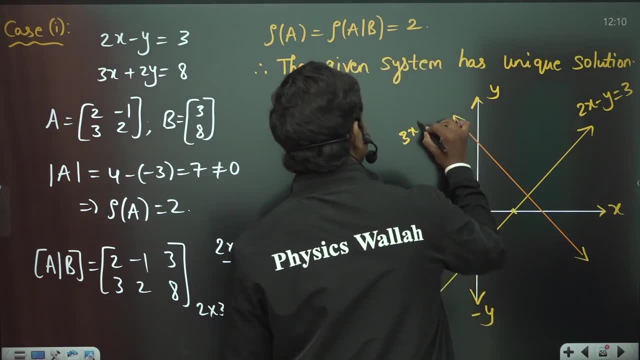 means if you take this line, it turns out something like this. so it comes something like this here. so if you see these two lines, these are the equations of 3x plus 2y is equal to 8, and you can clearly find from this matrix analysis, you found that this: 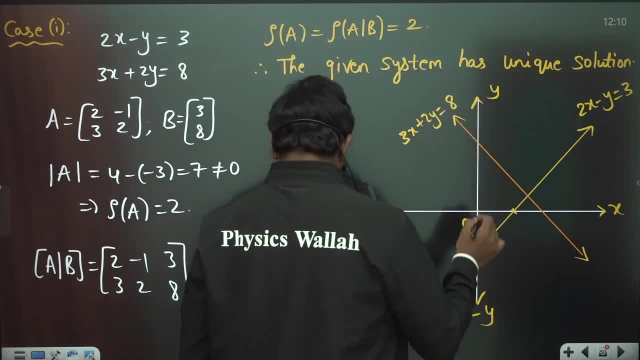 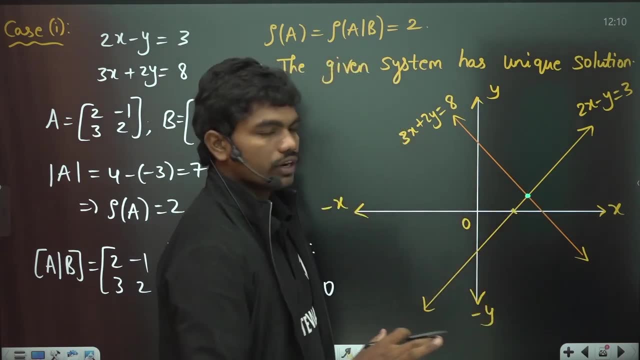 system of equations will have a unique solution, correct? and, of course, if you see the number of points this lines touch or cut each other is only one point. so that's how we have a unique solution. we don't know what is the value of that, but right now, your job is to identify whether a given system 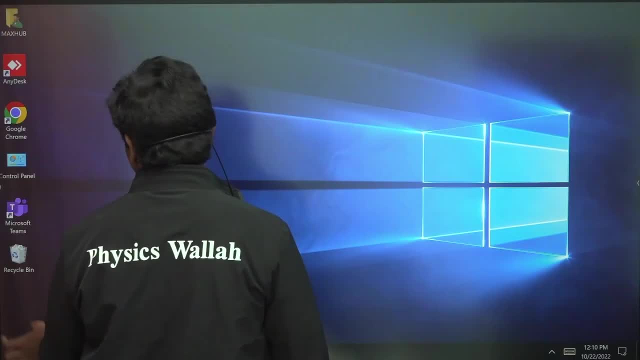 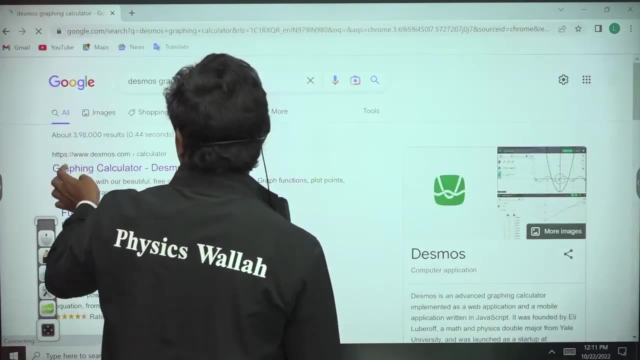 has a solution, or not? if you want me to be more colorful, i have a tool. i generally use this in my. i've used this for the first time in my research, but right now i can show you this graphing calculator by desmos. this is one very good graphing calculator, so let us see the equations. 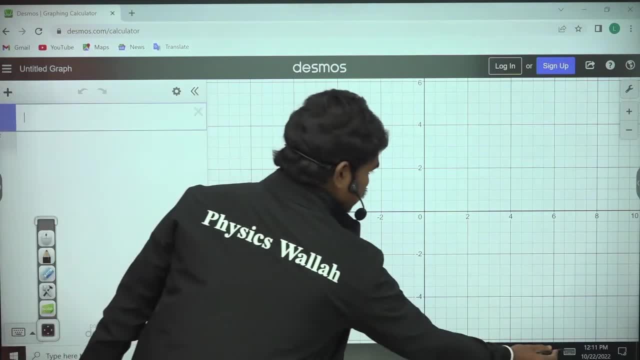 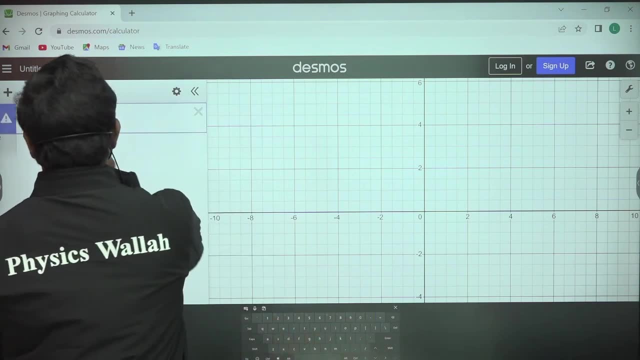 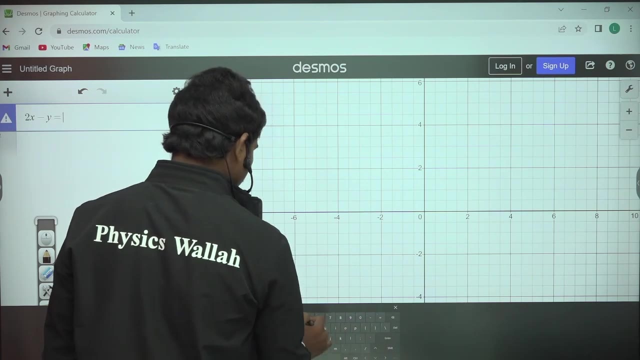 2x minus y is equal to 3. so let us see: yeah, 2x minus y is equal to 3, okay, oh, i think i have written something. so 2x minus y is equal to 3. so this is first equation. you see, as i have done the first line, this line. 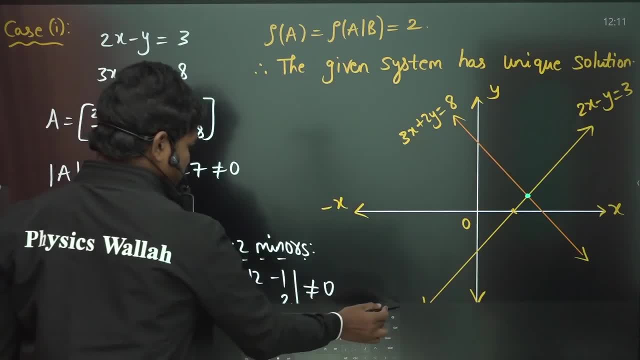 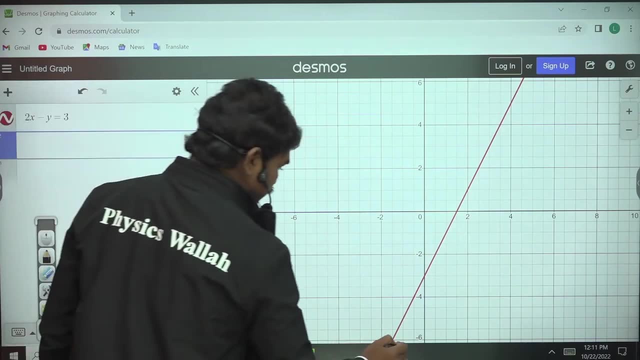 yellow line i have done. you can see that yellow line here also. like: 2x minus y is equal to 3. so what about the other equation? 3x plus 2y equal to 8. so let us see: 3x plus 2y is equal to 8, 3x. 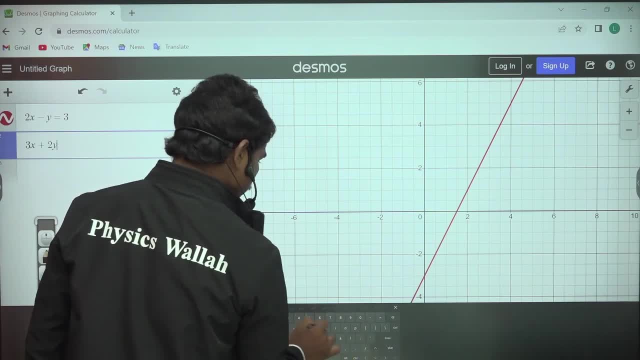 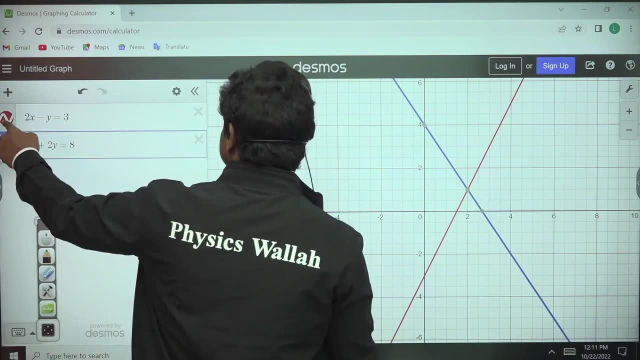 plus 2y is equal to 8. okay, so 3x plus 2y is equal to 8. you have seen some other line coming like this: the blue line- you can see the colors. a red line is for 2x minus y, equal to 3. 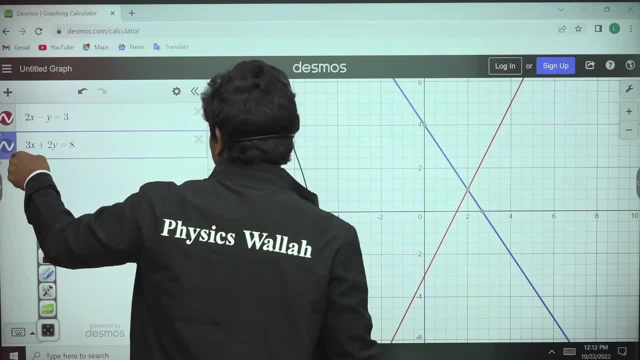 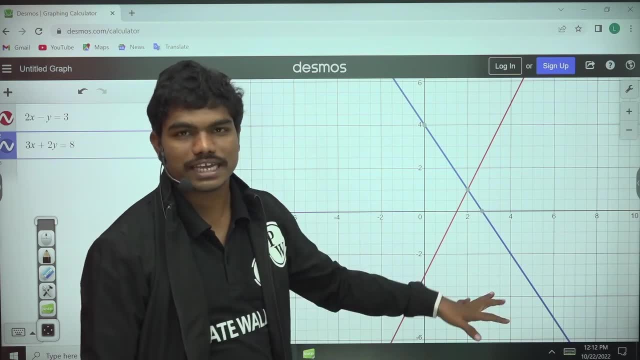 the line that is a red in color, blue line is for means this blue color is basically for this blue line. 3x plus 2y is equal to 8. so if you see these two are intersecting at this point and of course using this calculator you can just know the solution. also, if you dot this point 2, comma 1. 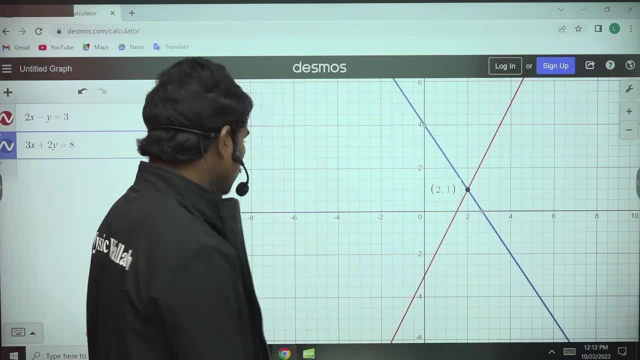 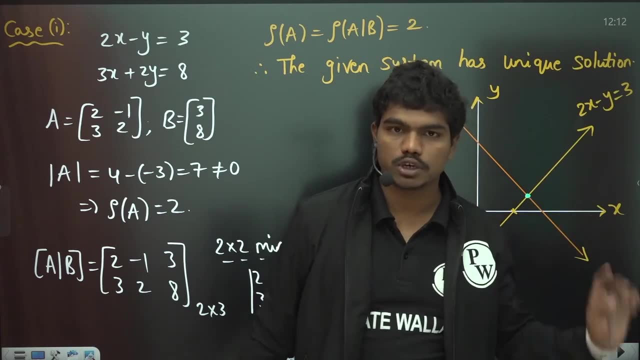 is the solution of this equations? okay, but right now we are not interested in solving, we are just interested to find. how many solutions does this equation have? this is from the geometry and this is from the. i mean, this is from the geometry and this is from this. you know matrix analysis. okay, so that's how you can have some system of. 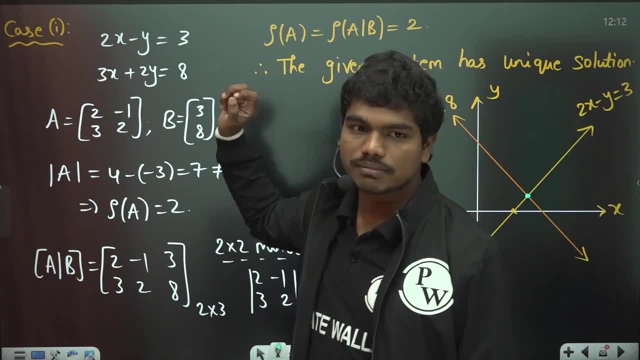 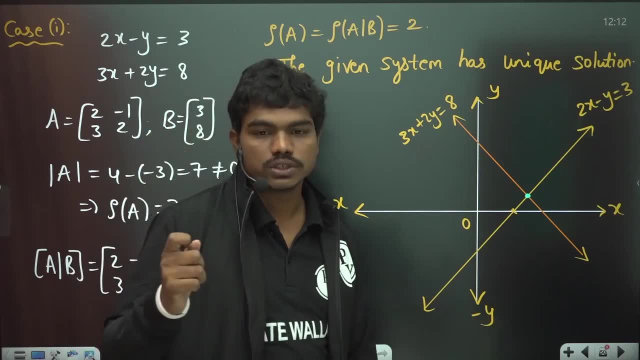 equations where you actually have the rank of this coefficient matrix is equal to rank of augmented matrix and that total value is equal to, you know- number of unknowns. so in such cases you will have only one solution and if you try to solve this equation, you will get only one solution, which is: 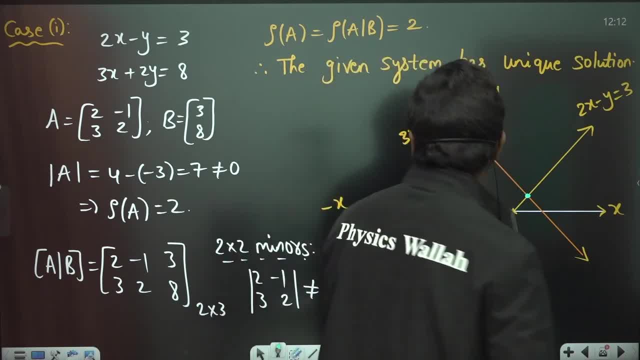 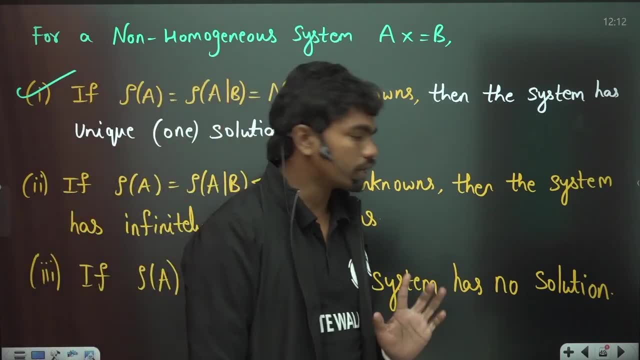 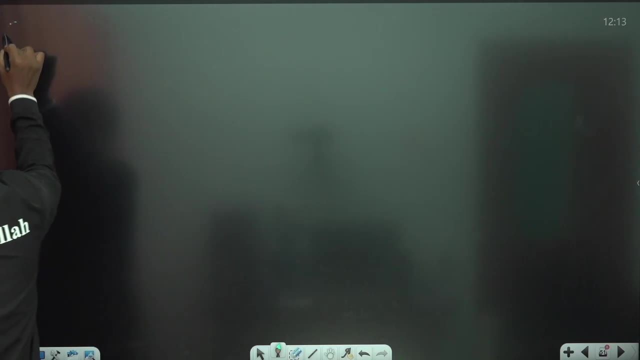 x equal to 2 and y equal to 1. so this is the first statement that i'm talking about. if this is the case, then the system has unique or one solution. okay, now let us come about the second case, case two. let us talk about case two. case two, let us suppose i have given you these equations: x plus 2y is equal to 4. 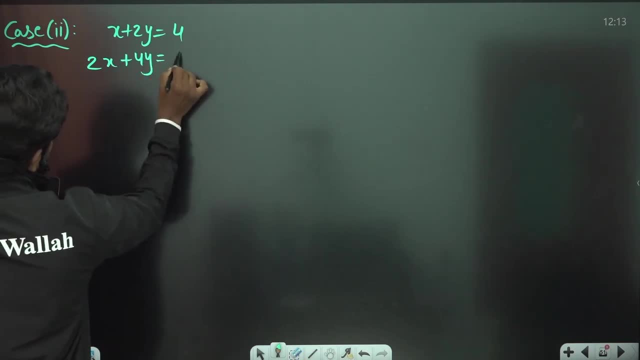 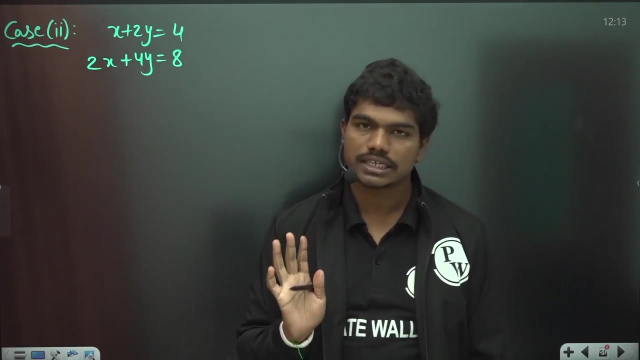 and 2x plus 4y is equal to 8.. so let us suppose these are the two equations, for example. okay and practically you can understand one thing right by looking at the equations itself. you can understand one thing: because it's 2 by d, you can. 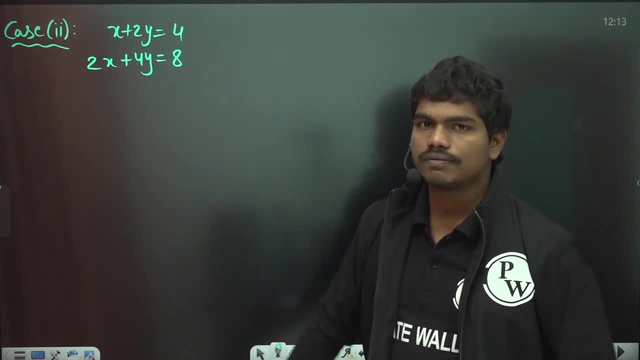 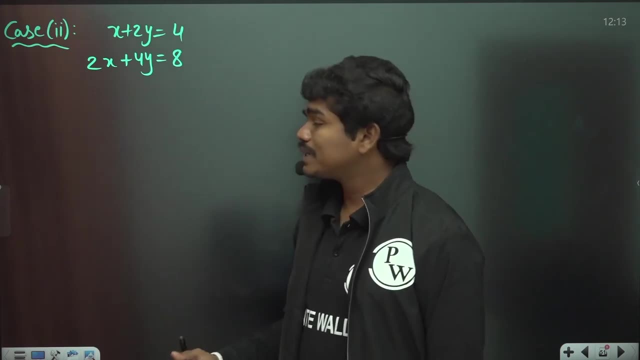 because it's 2 by 2. you can just tell them by looking, but for some high systems it's not very possible, okay? so let us see here: x plus 2y is equal to 4, and 2x plus 4y is equal to 8.. so let 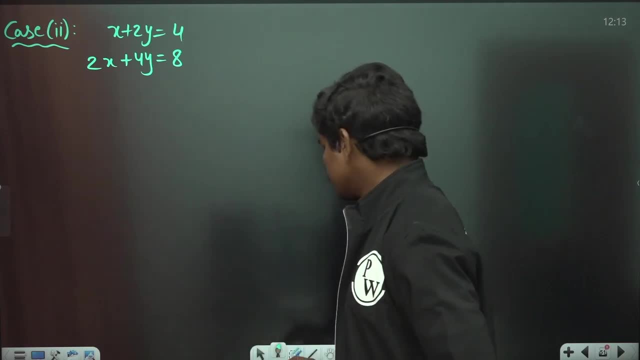 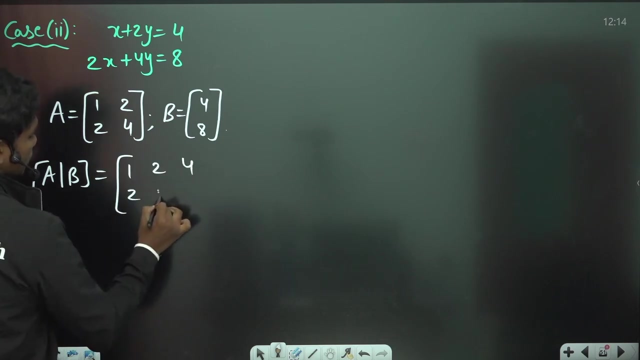 us suppose if you try to- uh, you know, solve this using the matrices. so let us write these equations so you know, a coefficient matrix is basically 1, 2, 2, 4. what about this b constant matrix, 4, 8.. so a augmented b is how much? a augmented b is equal to 1, 2, 4, 2, 4, 8.. now let us try to understand. 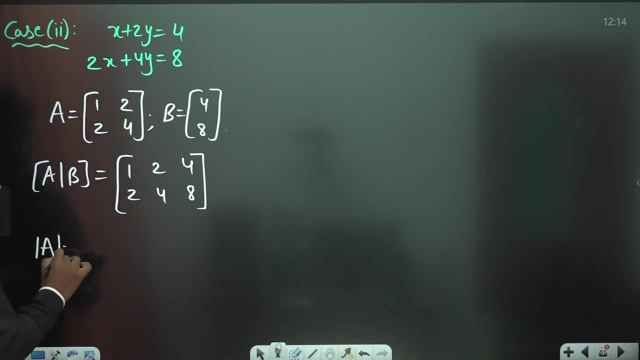 one thing. first of all, let us calculate that a. if you calculate that a, 4 minus 4, which is 0.. so this, that a is actually 0.. so 2 by 2 minor of this, a becomes 0.. now you should go for 1 by. 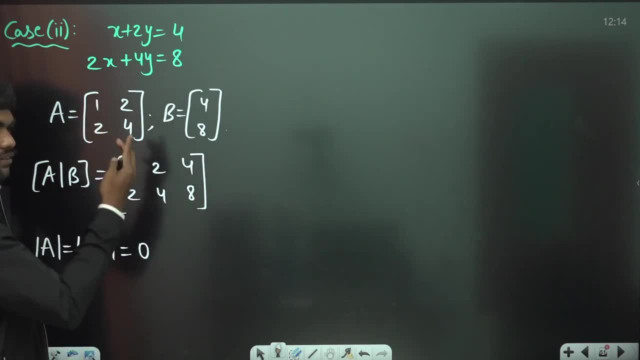 1 minus. okay. so if you go for 1 by 1 minus what are the 1 by 1 minus total, you have 4. 1 by 1 values here: 1, 2, 2, 4 and obviously all these are non-zeros, so you can say rank of a is equal to 1.. 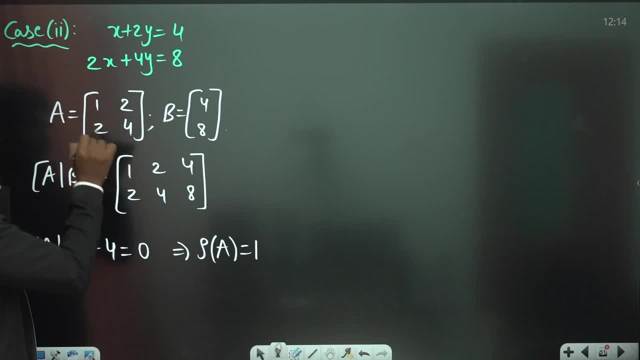 how you know that rank of a is equal to 1, because second order minor is coming out to be 0, so and you cannot have any third order, fourth order, so the only possible is first order. if you take any of these four elements, at least you have one of these four elements as non-zeros. so that's why 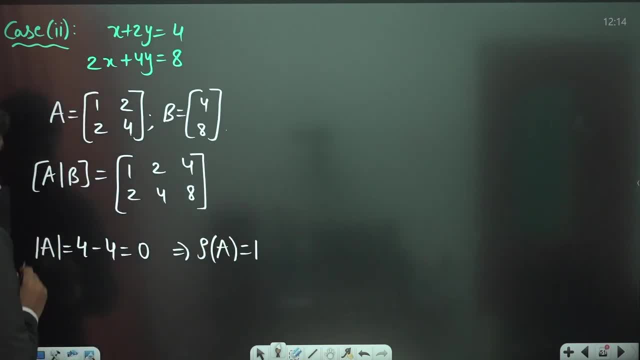 rank of a is equal to 1.. now coming to the rank of a augmented b. rank of a augmented b. so let us suppose if you take this is of size 2 by 3, so maximum you can take 2 by 2 minus. so if you take 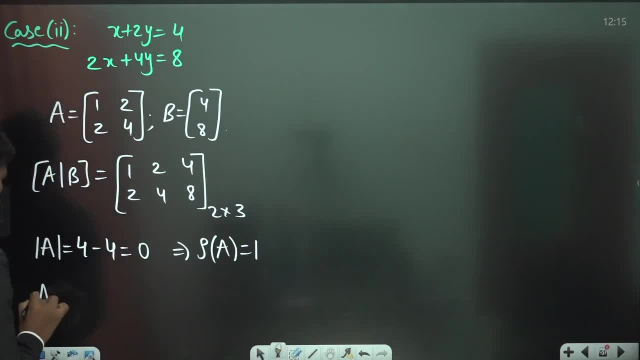 2 by 2 minus of a augmented b, a augmented b. if you take this matrix and if you take 2 by 2 minus, okay, so 2 by 2 minus. so if you take this 2 by 2 minus, then we have 3, 2 by 2 minus. what are they? 1, 2, 2. 4 means deleted the third column, deleted the second. 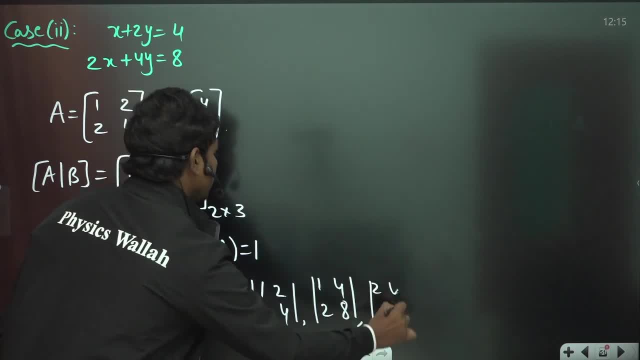 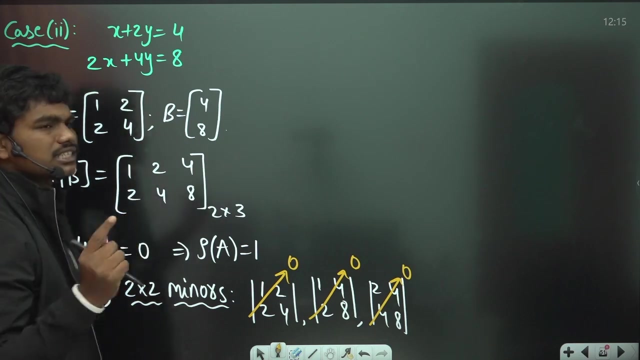 column and deleted the first column. so you will find by strange that all these values are zeros, because 4 minus 4, 8 minus 8, 16 minus 16, all these are zeros. so definitely you should go for 1 by 1 minus, followed by: and you see, in this six elements there is at least one element which is non-zero. so 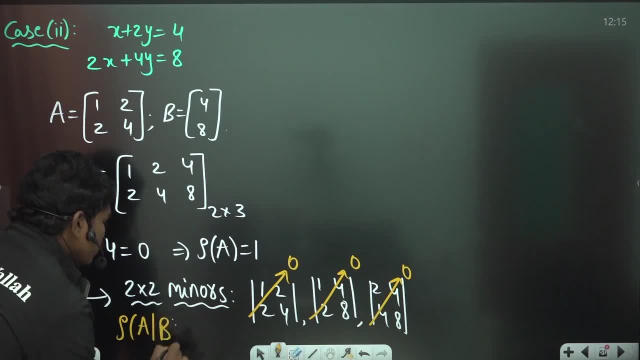 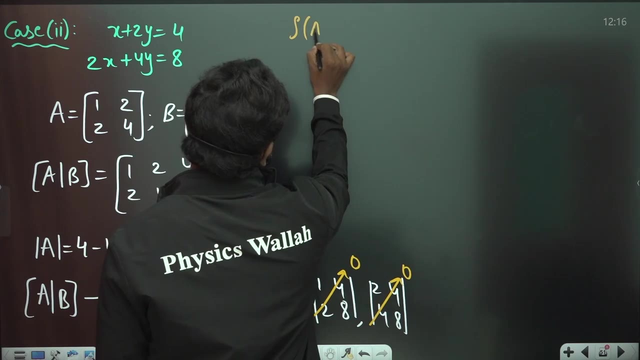 rank of a augmented b is equal to 1.. so here you understood one thing: rank of a is 1, rank of a augmented b is also 1, but these two are not equal to the number of unknowns in this equation, correct? so if you simplify this, i means if you write it in a organized way, rank of a is equal to rank of. 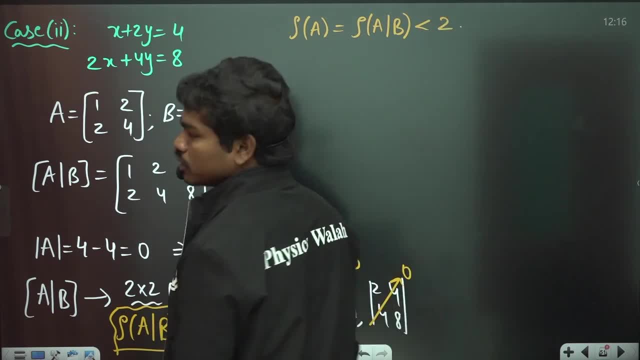 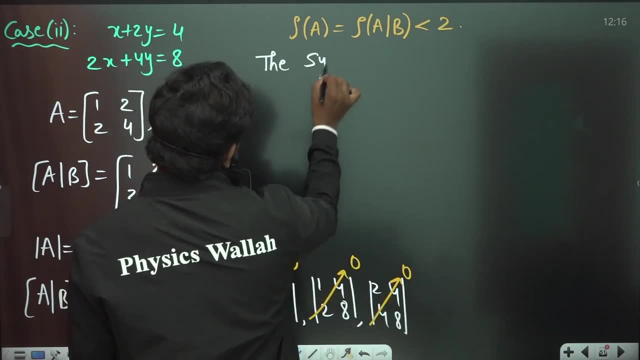 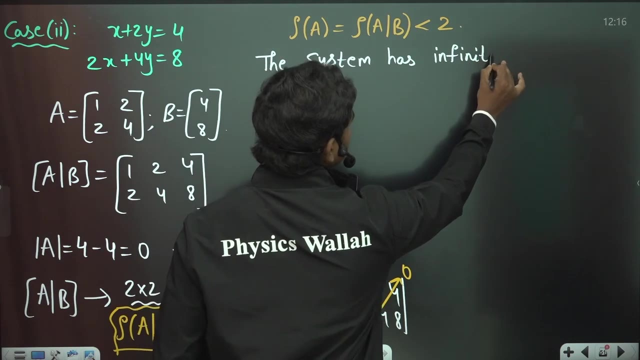 a augmented b, but this is less than 2 because number of unknowns is 2.. so, as per our understanding, the system has infinitely many solutions. the system has infinitely many solutions and, of course, i am explaining you for a 2 by 2 case, because john 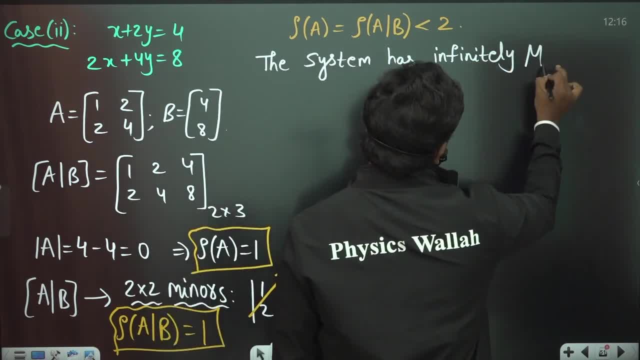 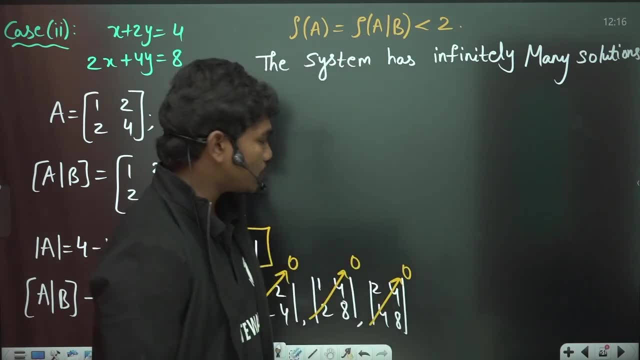 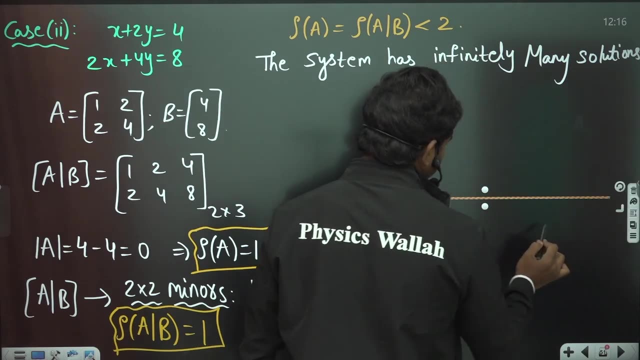 medically. i can draw some lines and explain you. the system has infinitely many solutions. okay, so the system has infinitely many solutions. now try to understand carefully here. if i plot them again. this is your x axis, this is your x axis and this is your y axis. for example, 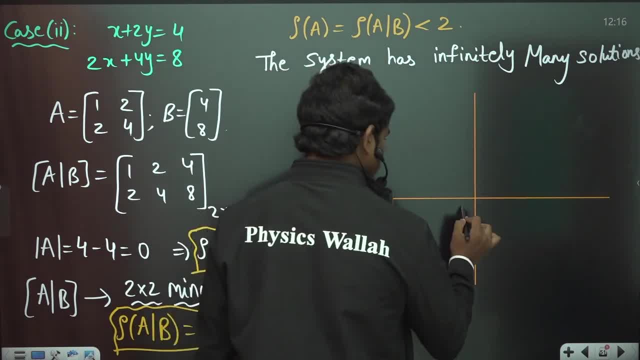 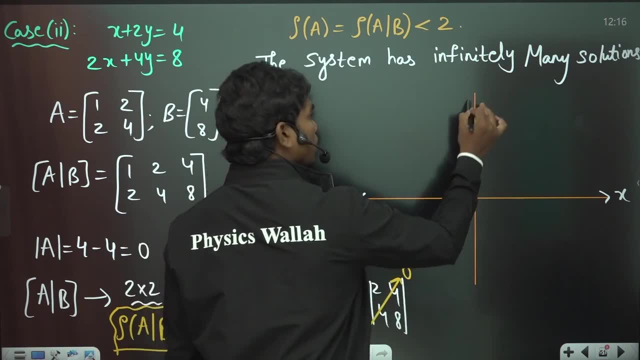 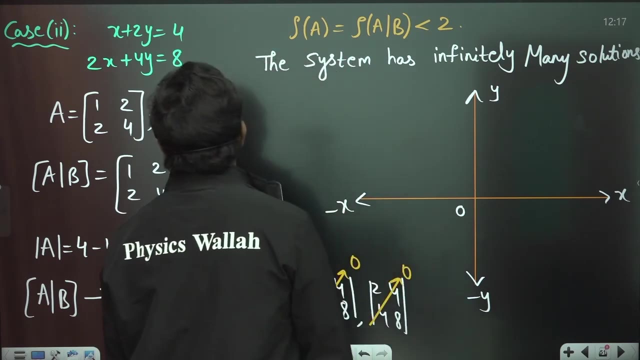 this is your y axis. so horizon, horizon, oh, i'm sorry, yeah, horizon- x minus x, y and minus y. so if you take this equation, so the first equation, x plus 2y is equal to 4.. so if you plot that point basically, so at x equal to 0, y is equal to 2, 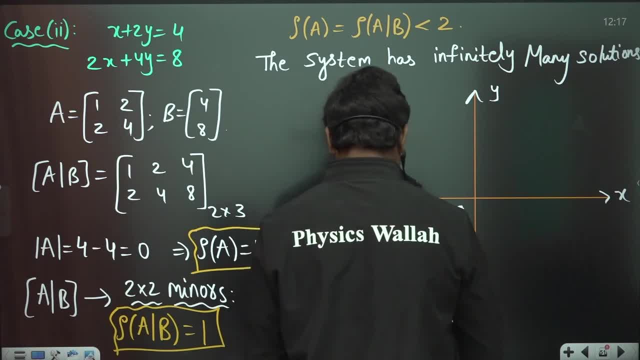 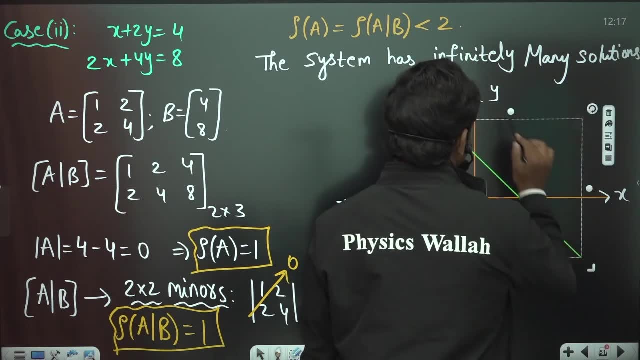 and that y equal to 0, x equal to 4, so which means the line looks something like this: this is the line, so x value should be little high. so let us suppose i am putting some line like this. okay, so x is more compatible. so this is the. 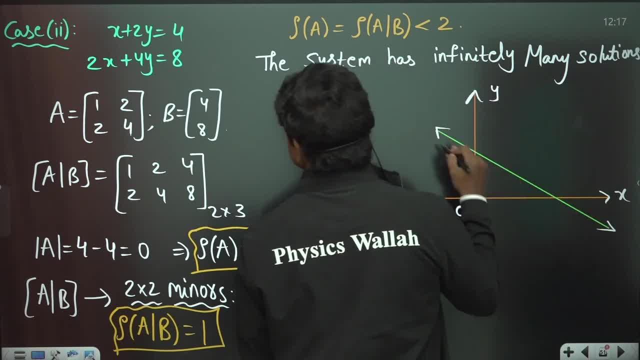 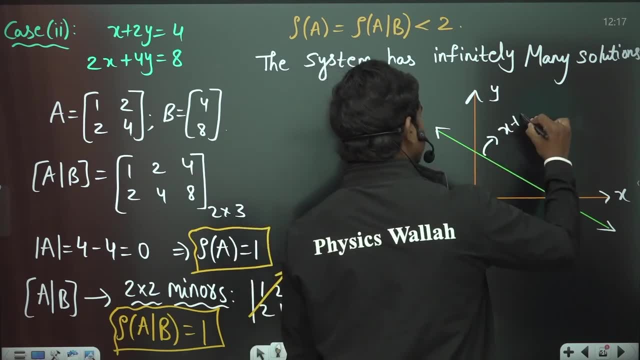 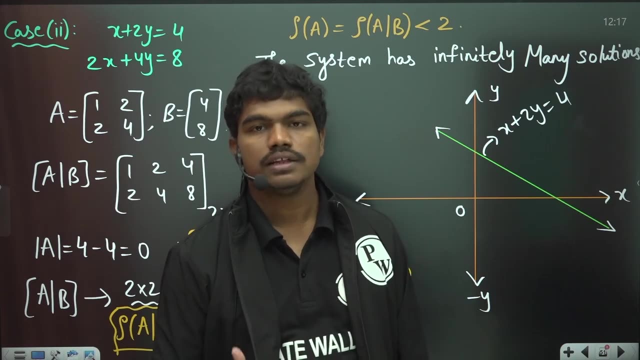 equation of the line, or this is the representation of this line: x plus 2y is equal to x plus 2y is equal to 4.. now, mathematically, okay, you got infinitely many solutions. but physically, how can you have infinite points of intersection? this is possible when the two lines 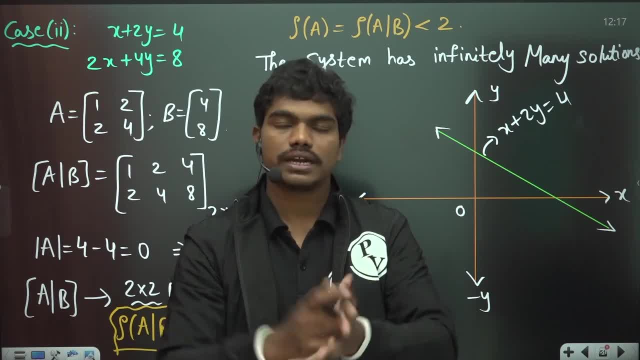 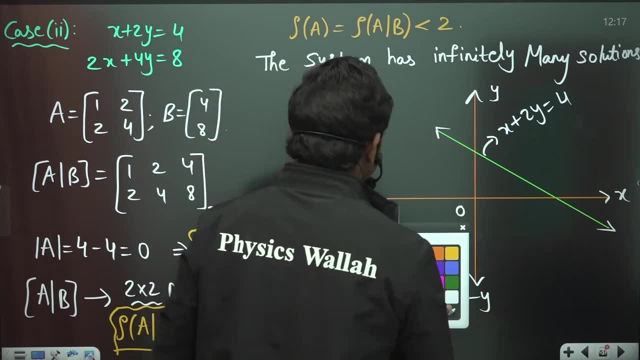 overlap each other. correct. when two lines are overlapping each other, you can understand that at each and every point both these lines touch each other, so they have infinitely many solutions. so if you plot this, 2x plus 4y is equal to 8. again you will get along the same line. 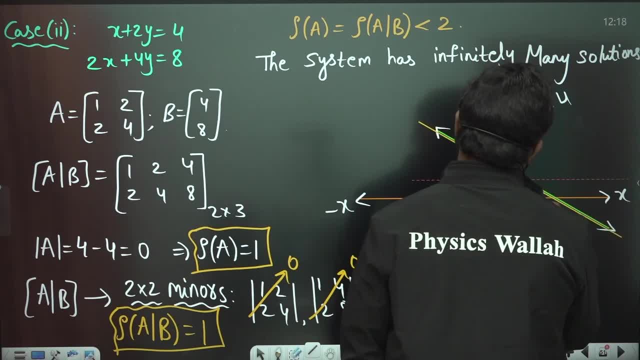 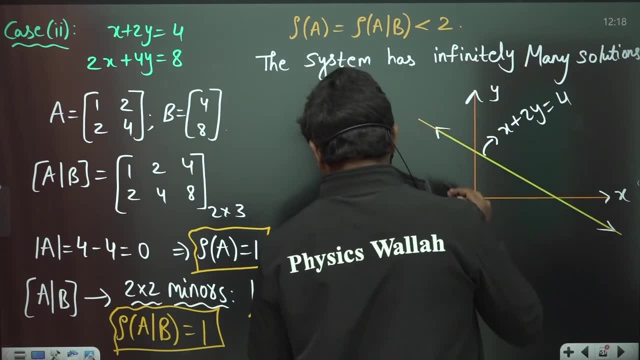 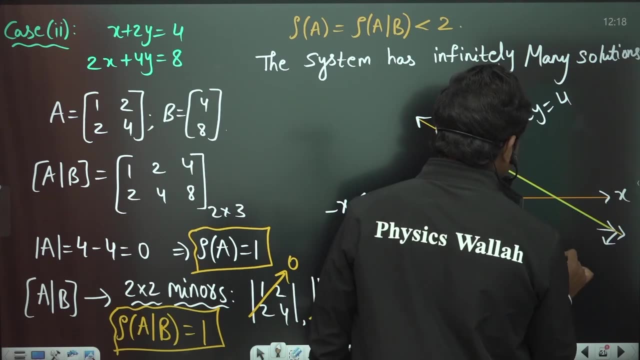 you will get along the same line, okay, okay, so i am trying to overlap it slowly, fine, so, if you see, i have just shown some difference, at least so that you can understand that this equation is 4x or sorry, 2x plus 4y is equal to 8, and if you see, all these points are: 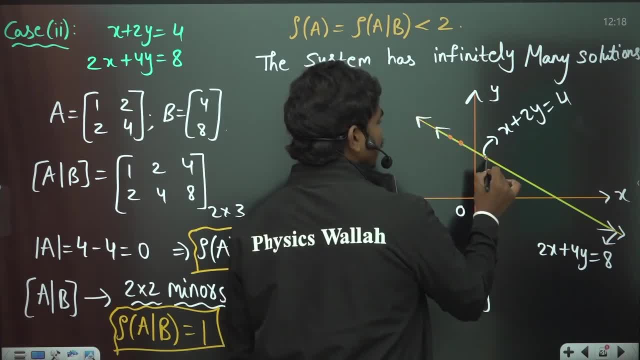 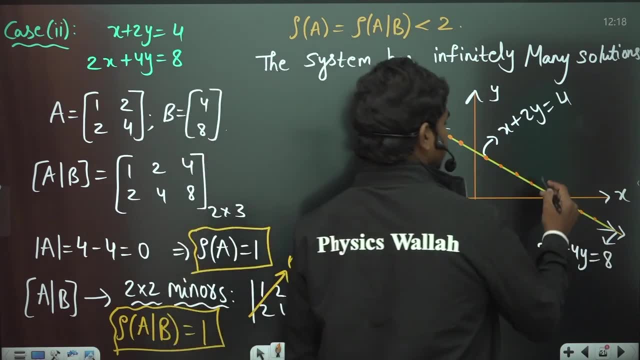 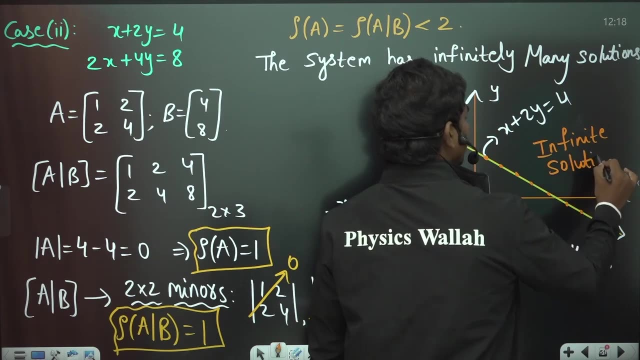 nothing but points of intersection here, this point, this point. so you have lot of infinitely many points. obviously on a line. you have infinitely many points, so all these are infinitely. you know solutions basically. so infinite solutions, infinite solutions. okay, you know, basically, if i give you a equation of a line, how to draw the line, okay, so, if you want, if you identify this point and these, 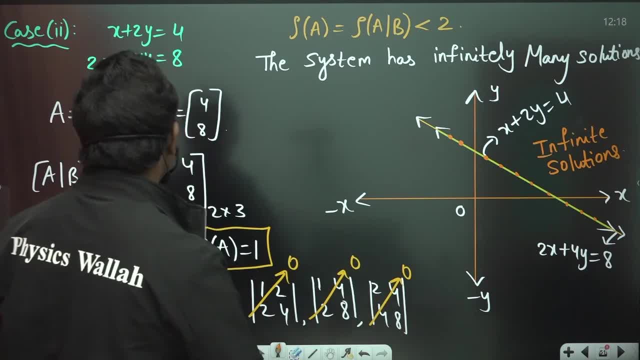 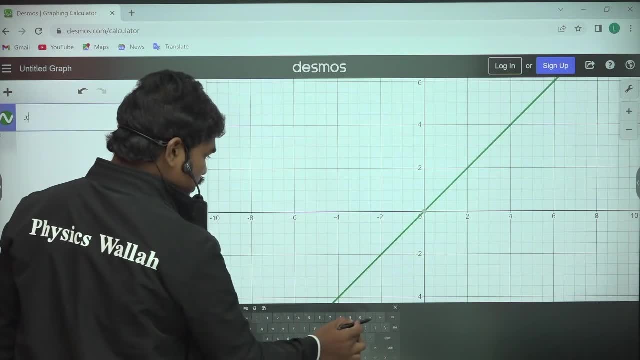 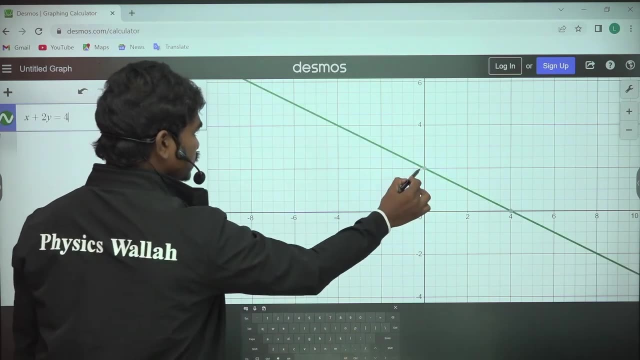 two points. you can draw a line connecting those two points. okay, anyhow, i'll show you. on desmos also, x plus 2y is equal to 4. so the first equation, so the first equation: x plus 2 y is equal to 4. so x plus 2y is equal to 4. this is the line. you can see the green line here. and what about the next? 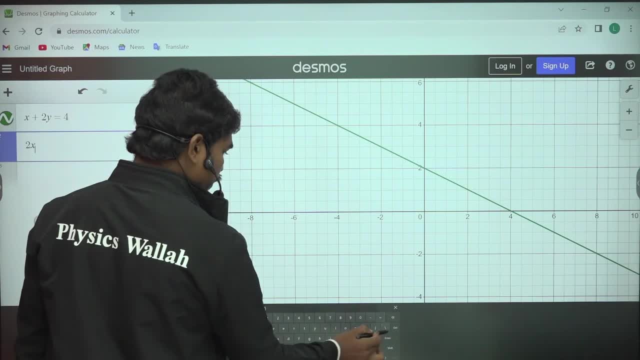 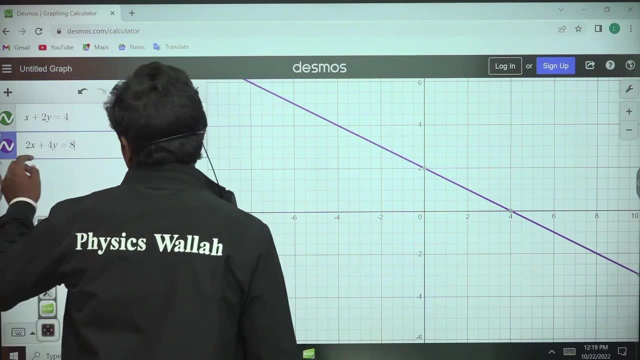 equation: 2x plus 4y equal to 8. 2x, oh sorry, 2x plus 4y is equal to 8. so 2x plus 4y is equal to 8. so this is in purple color. okay, one is in green, one is in purple, but right now we cannot see the game. 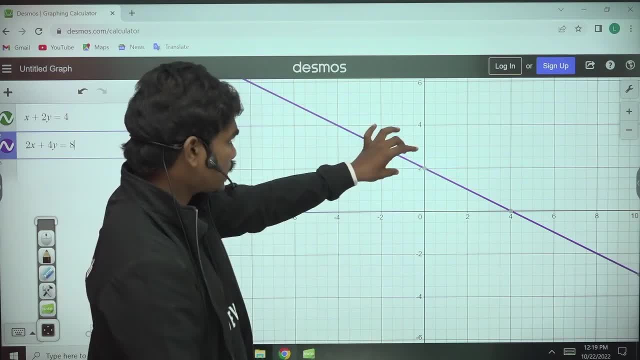 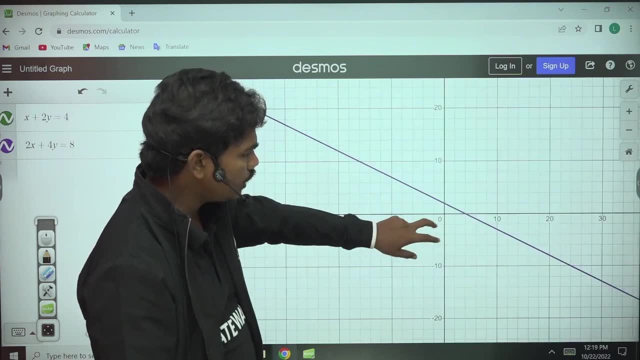 the purple has overlapped this green one. okay, so right now you cannot see, you can see this as only one line, but actually there are two lines which are involved here. okay, so that's the reason why, if you see this, they have infinitely many points of intersection, always, okay, so. 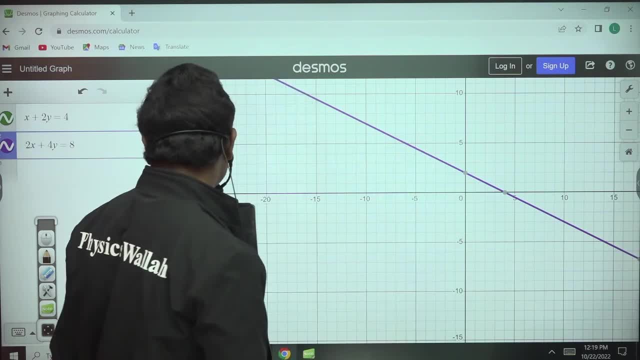 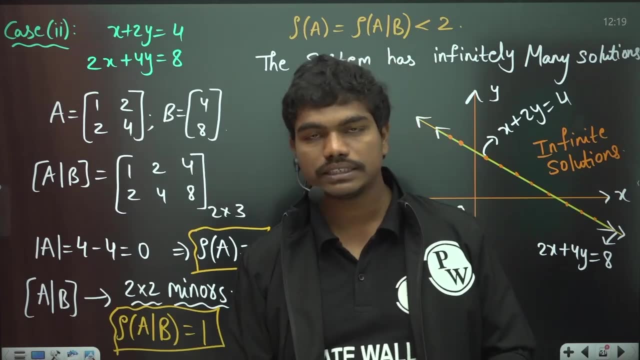 you can see all this. at every point there is a point of intersection, clear. so that's how this system of equations can have infinitely many solutions. when this condition holds good means, rank of the coefficient matrix is same as a rank of this. what do you say adjoint? 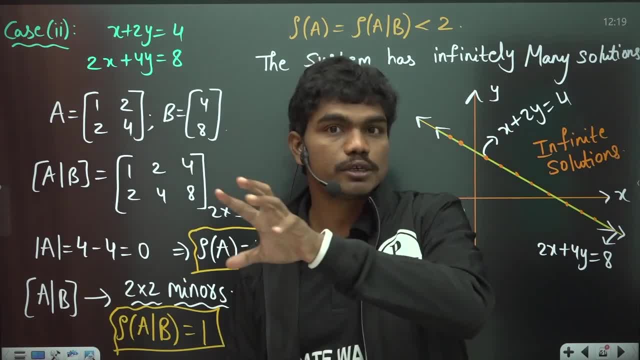 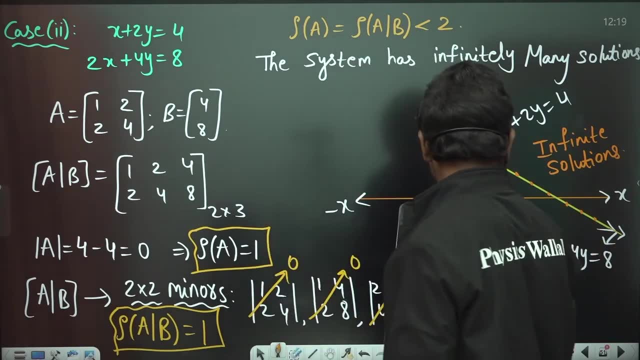 matrix, but at the same time, both of them together are less than the number of unknowns in that equations. okay, so this is one very, very important step that you need to make a note of. now let us go for the last case. so basically, that's the third case that we are talking about this. 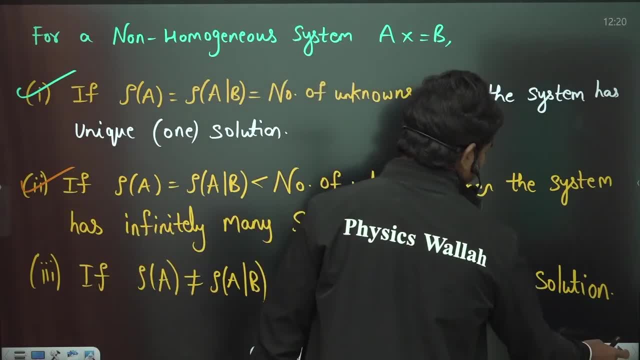 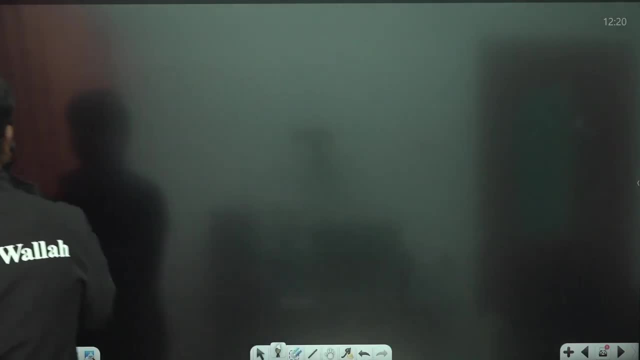 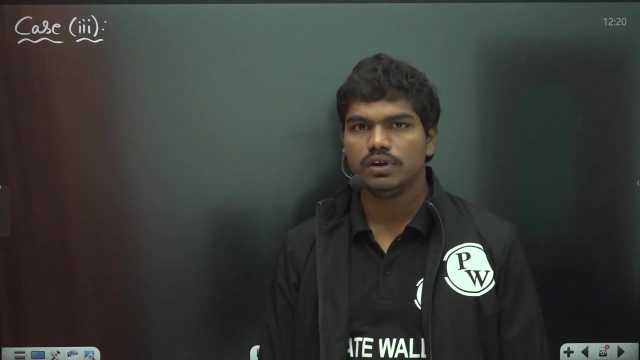 is the second case we have discussed. let us come to the third case. no solution case, no solution case. okay. so let us see case three. also okay, case three. let us see. what is this case three? now try to understand one thing: sometimes equations can have no solution. also, how look? let me again take one example and let us show again. so x plus. 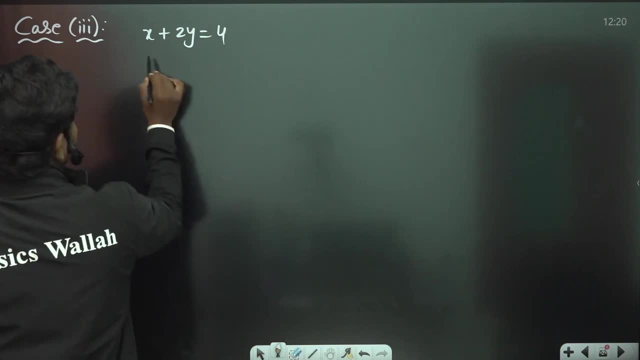 2y or x plus 2y is equal to 4. for example- and let us suppose i have taken the equation, same equation with some different constant- 2x plus 4y is equal to 9. let us say, instead of 8 i have. 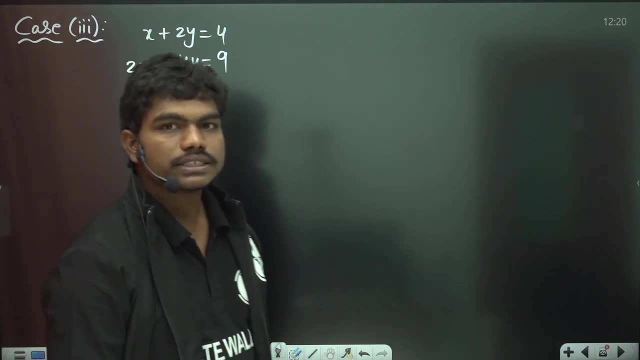 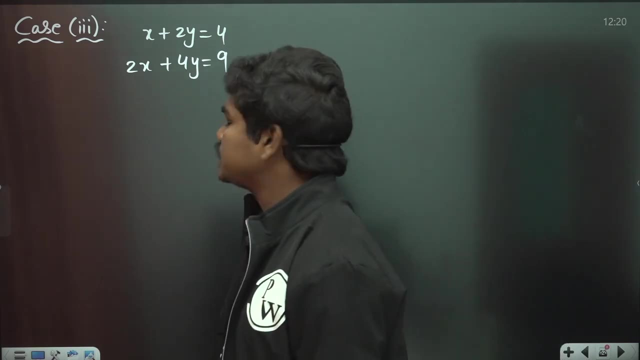 taken 9. now you can understand one thing: if both lines do not have any solution, you can another prediction. that means, practically speaking, they are parallel to each other. okay, if you check the slopes, minus x coefficient by y coefficient, then minus of x coefficient by y coefficient is same for these two lines. so that's why you can have these two lines. 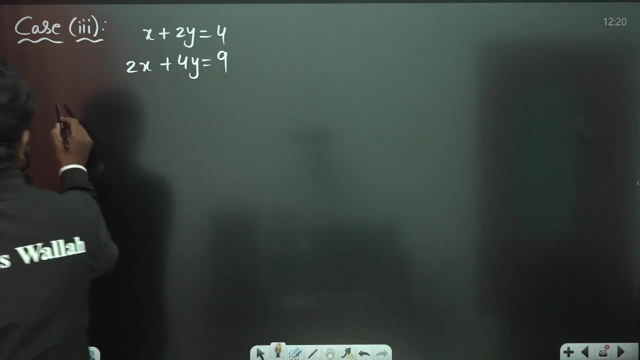 as parallel lines. anyhow, let us check the matrix conditions. so a is equal to 1, 2, 2, 4. so a augmented b, a augmented b is equal to 1, 2, 4, 2, 4, 2, 4, 9. so you can calculate one thing easily: if you take a rank of this matrix, if you take determinant, 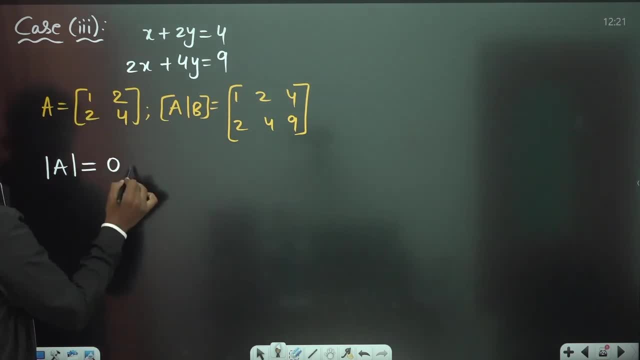 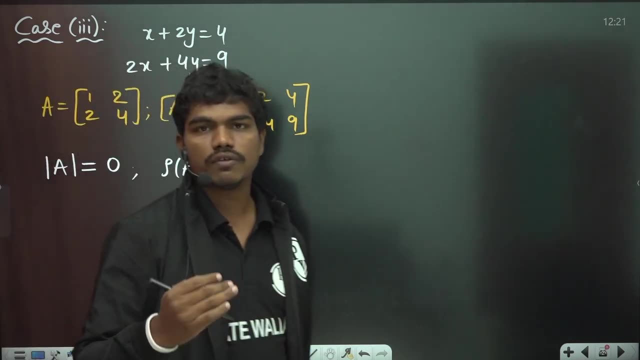 of a. this is equal to 0 straight away. 4 minus 4, 0. so rank of a is equal to 1. definitely clear, because if you 2 by 2 minus are 0s, then you will go for the first order minus and obviously out of. 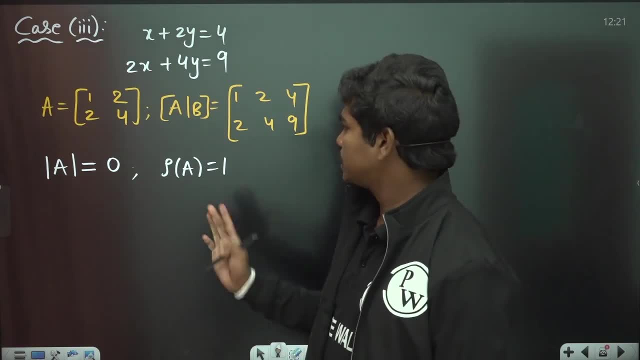 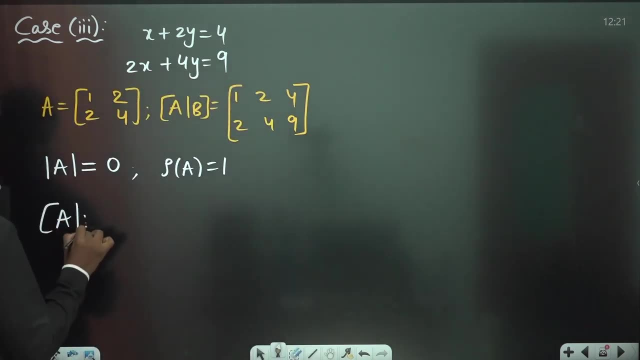 all these four elements, you can see at least there is one element which is non-zero. so rank of a is 1. now what about the rank of a augmented b? let us consider so a augmented b. if you consider 2 by 2 minus of this, 2 by 2 minus, because they are the highest order minus, you can consider so 1, 2, 2, 4. 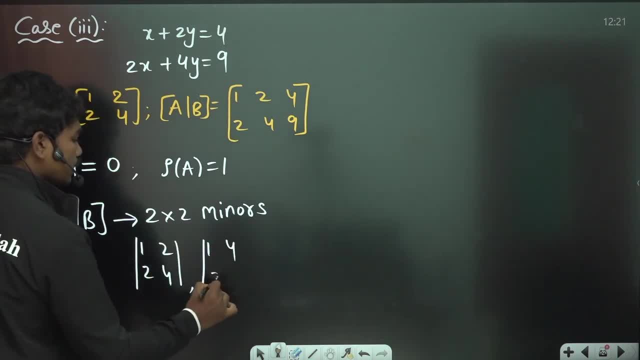 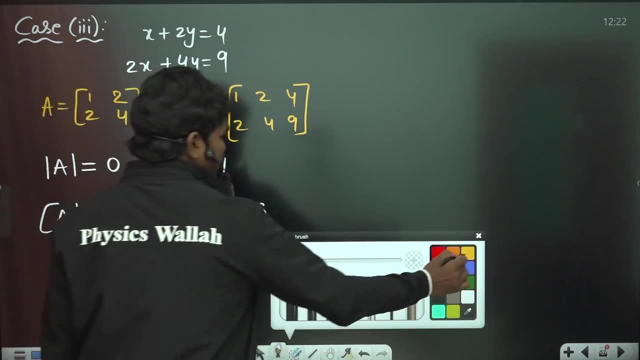 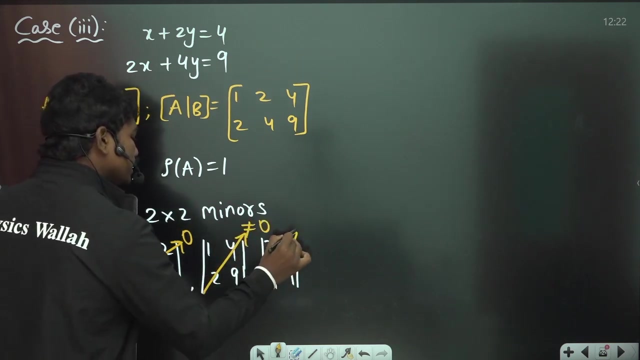 this is 1 minor. 1, 4, 2, 9- this is one more minor. and 2, 4, 4, 9- this is one more minor. now you can understand this thing: that this determinant is 0, but this determinant is not equal to 0. similarly, this determinant is also not equal to 0. so, out of this, 3, 2 by 2 minus you. 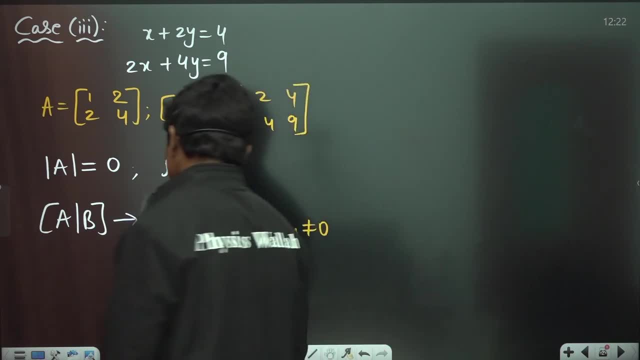 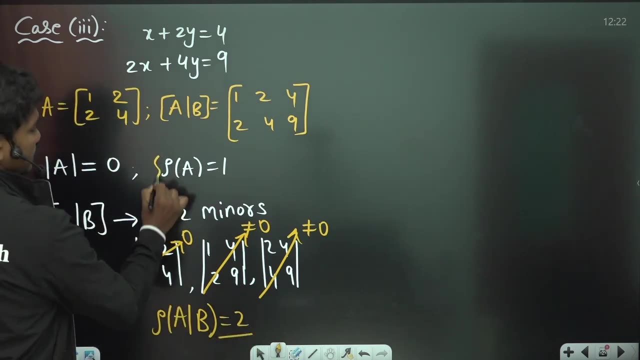 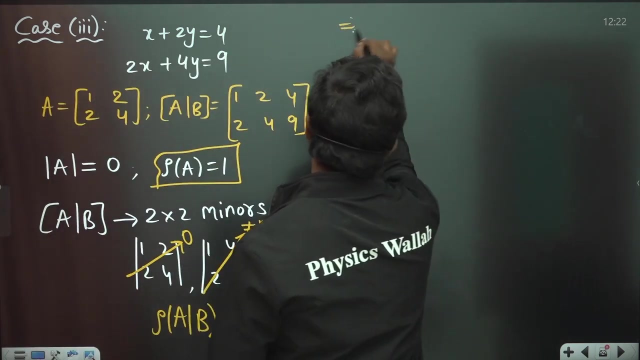 have at least one minor which is not equal to 0. so therefore, rank of a augmented b is basically 2 in this case, whereas rank of a is only 1 in this case. okay, so that's how rank of a and rank of a augmented b- both are not equal in this case. so this implies rank of a is not equal to rank of. 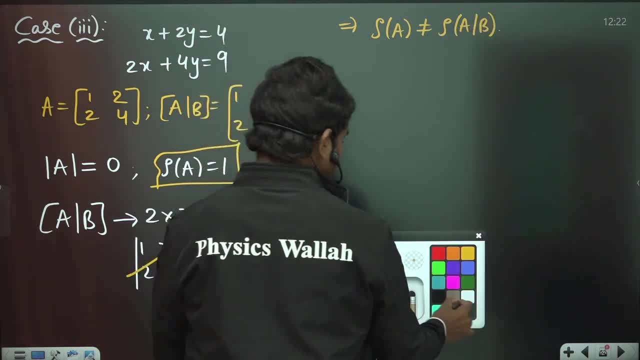 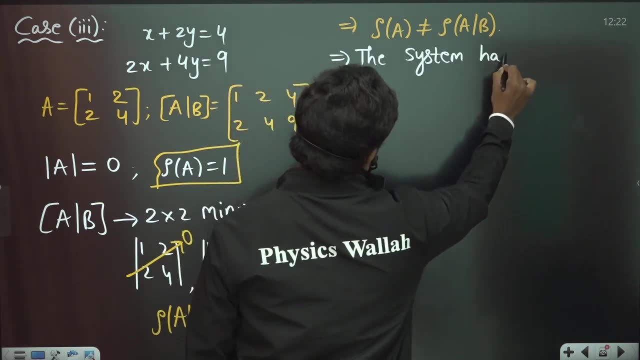 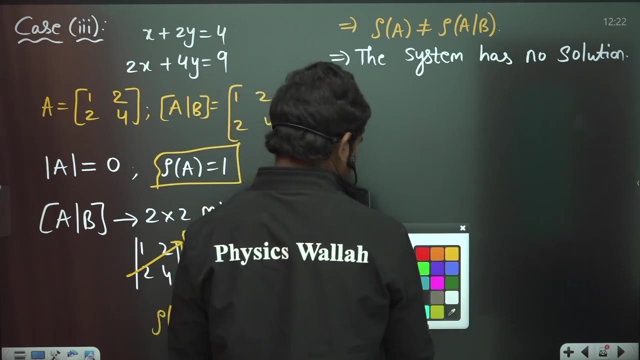 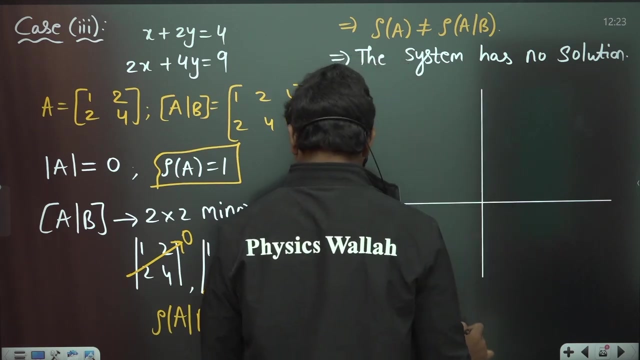 a augmented b. so this implies the system has no solution, the system has no solution generally. so what is the meaning of no solution? both these lines will look parallel actually if you draw them. so if you take x axis and if you take y axis. so horizon x minus x y. 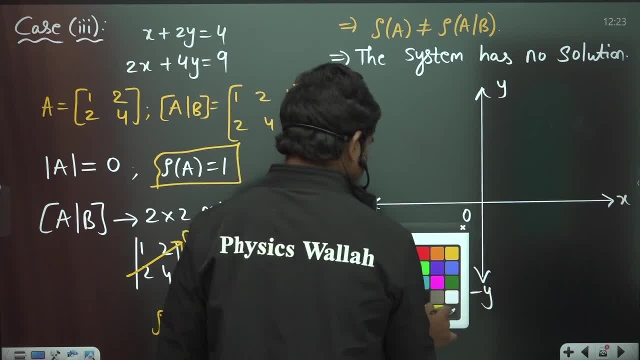 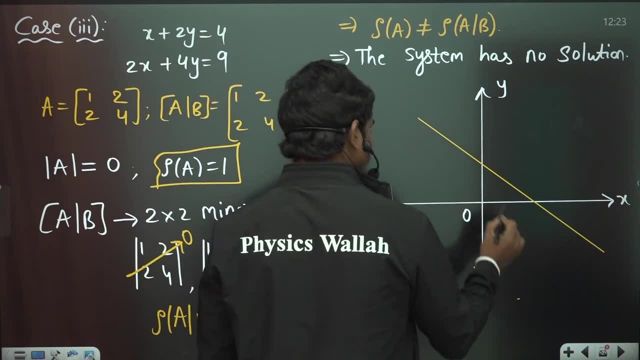 minus y. so now, if you see this, 2x, x plus 2 y- we have seen previously- the line looks something like this. so this is: x plus 2 y is equal to 4. this is the equation of the line: x plus 2 y is equal to 4. 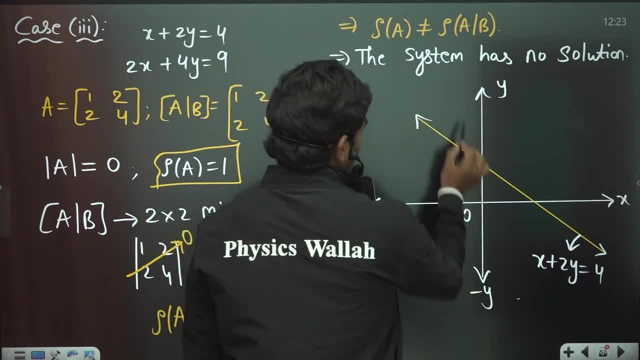 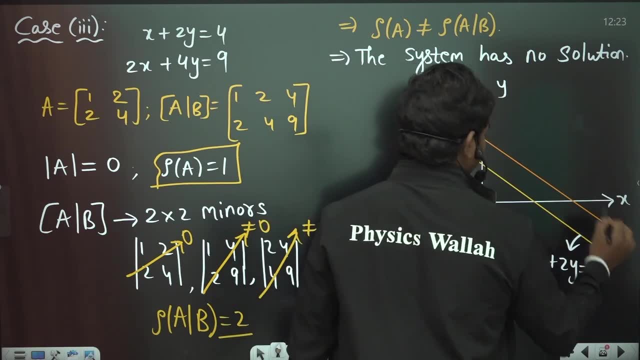 and similarly, if you take some other line of 2x plus 4 y is equal to 9, will be something like this: so 2x plus 4 y is equal to 9, so 2x plus 4 y is equal to 9. and if you see, 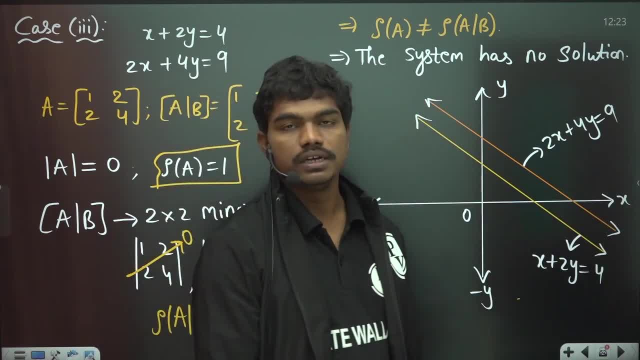 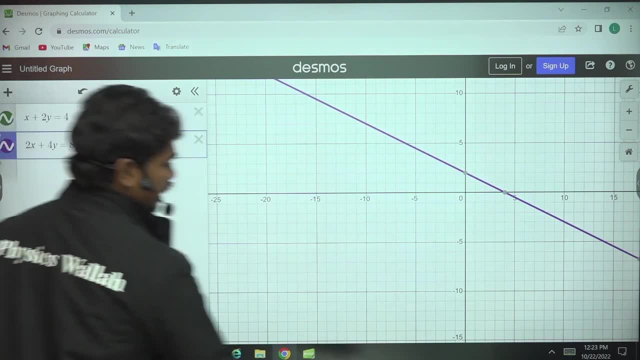 These two lines are parallel and you cannot find any point of intersection between them, So, mathematically speaking, you don't have any solution. Okay, Anyhow, I'll show these lines on this plot. The only difference is I made this 8 as 9.. Okay, so let us see. 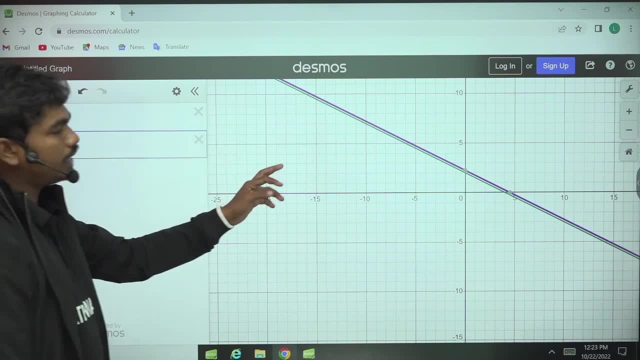 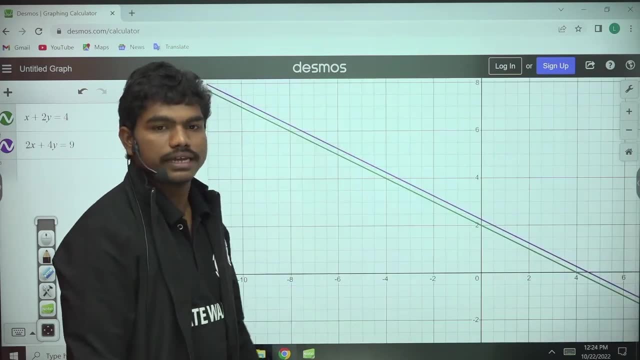 So now, if you see when I made this 8 as 9, you can find the two lines, and these two lines are parallel And section. you cannot find any point of intersection at any point because these are parallel lines. Okay, so that's how it. it's clear that whenever and of course this is a 2 by 2 case, 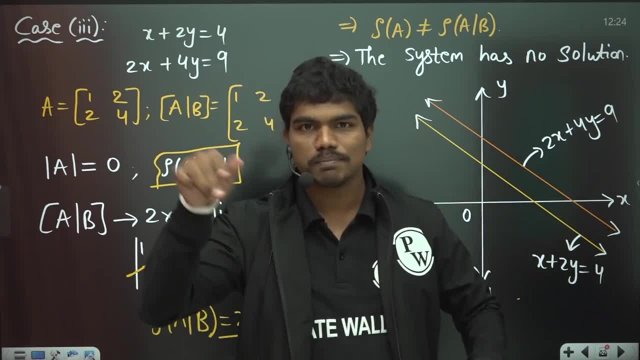 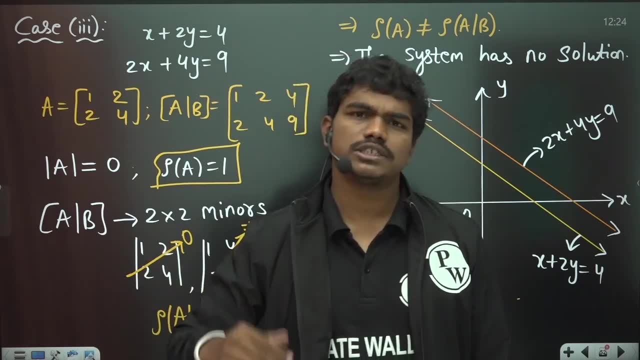 So I have explained you with straight lines. if I go for 3 by 3, I need to draw some planes and also it looks A little clumsy so I haven't taken. but the same case holds good for any size matrix, The equations with the unknowns, the equations with four unknowns, anything basically okay. So now. 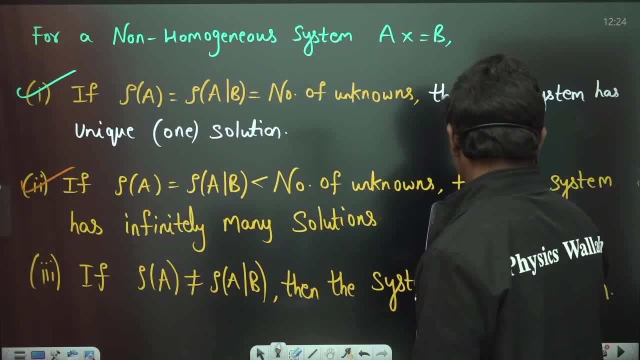 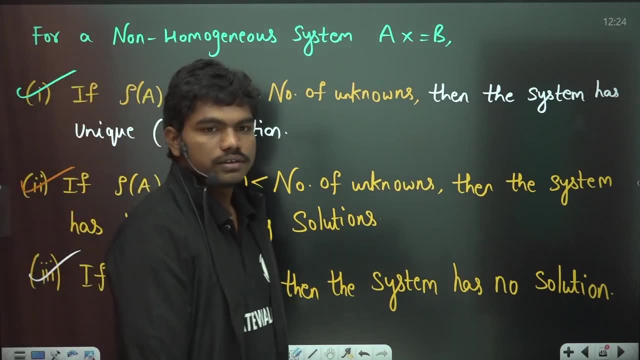 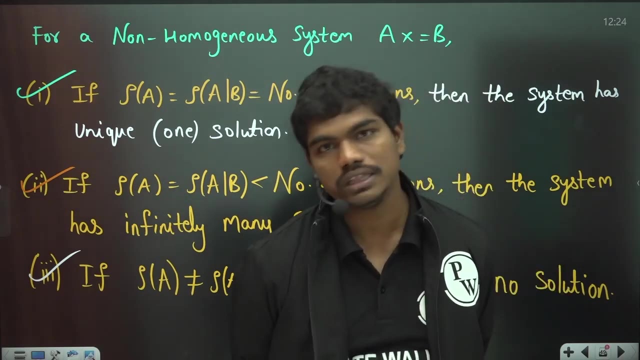 That's how we have cleared this. third point, also third point. Okay, So basically this point and basically this is: this system is a non homogeneous system. cut, This is a non homogeneous system. Now, let us suppose you have a homogeneous system means you are all Constants: B 1, B 2, B 3- all these are zeros. then let us see what is the case. 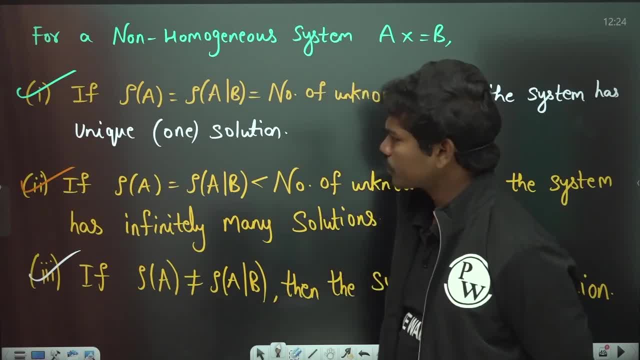 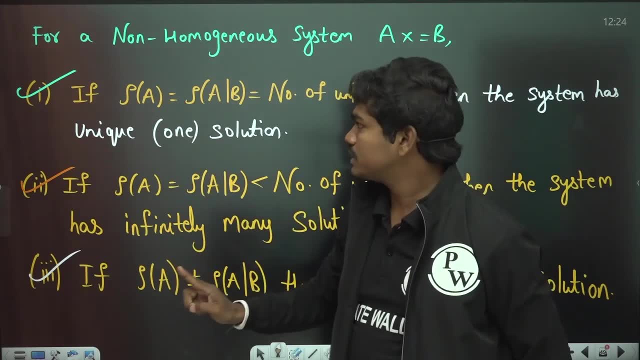 Okay, and before going for that, I'll tell you one thing. look, Try to understand one thing. in this case, You got that T and not equal to 0, correct? So try to remember this thing whenever. if the determinant of the coefficient matrix is non-zero, 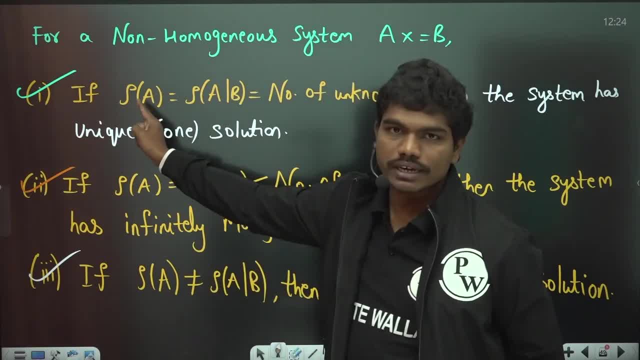 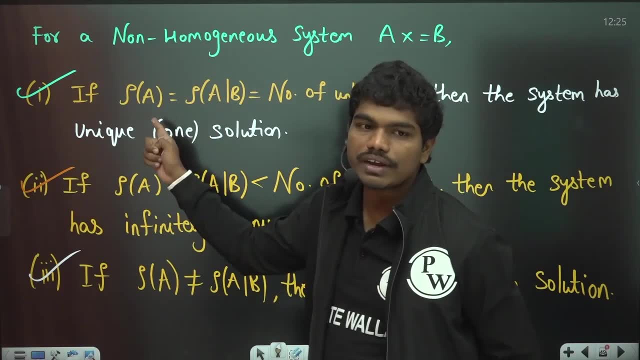 You always have a unique solution, because if that T is not equal to 0, here also you will get one minor Which is equal to that Okay. So that's why these two will be definitely equal. if that is non, Okay. so if that A is not equal to 0, then system will have single or unique solution. 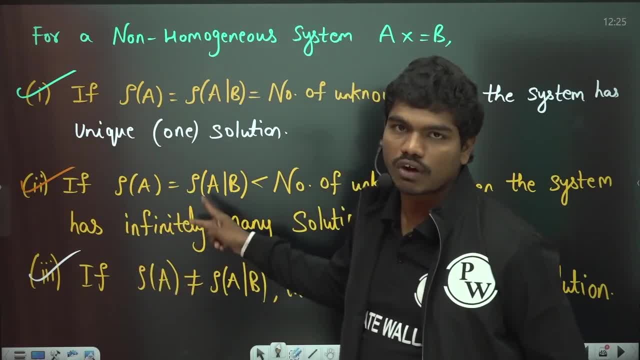 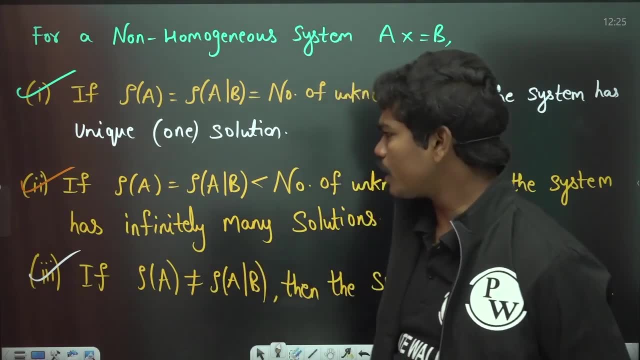 Okay, but if that A is equal to 0, then the case falls into one of these two things. Okay, then the system may have infinitely many solutions, or the system may have no solution. Also, It depends on the you know for the Analysis. but if that A is not equal to 0, the system will definitely have a unique solution. 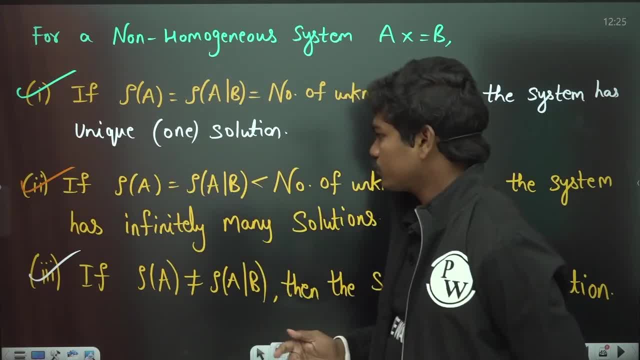 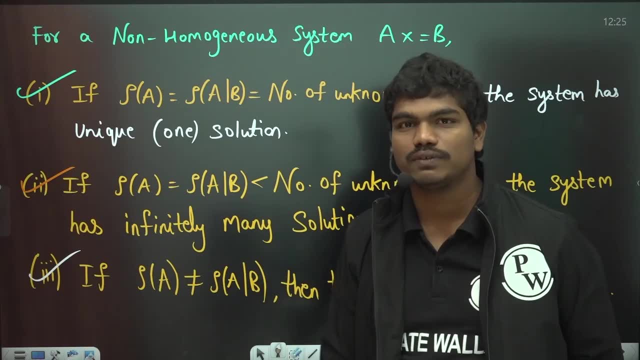 This point has to be very clear in your mind. Okay Now, and obviously you know, if that A is not equal to 0, your equation Is equal to a inverse B. You can calculate directly. you will get X value. Okay, single solution, You can directly calculate. 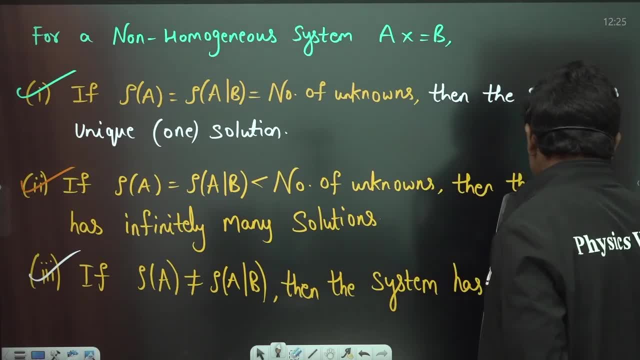 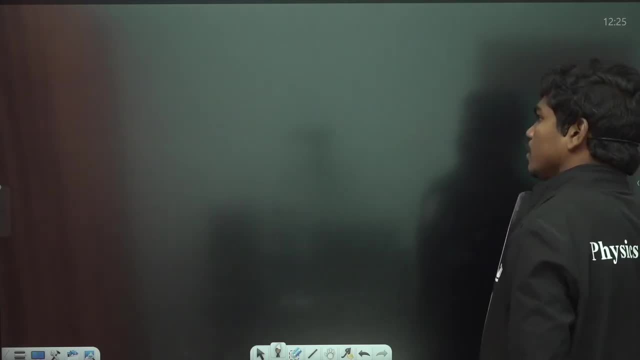 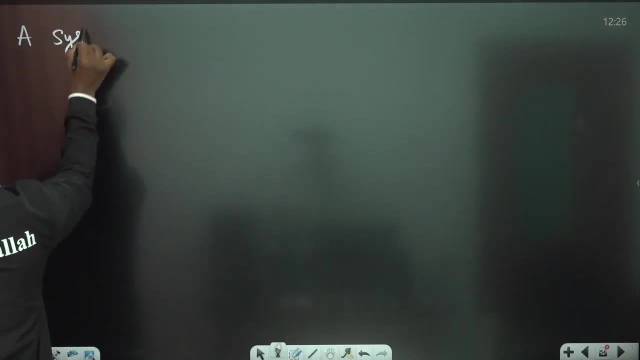 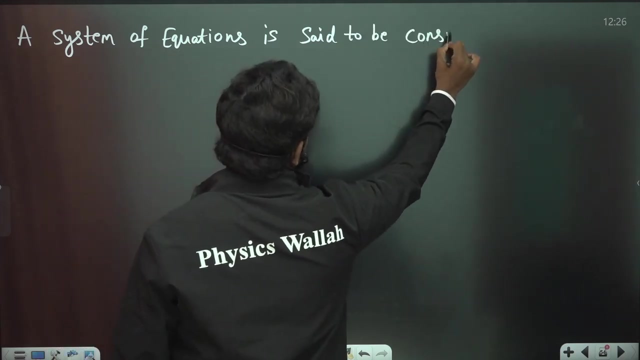 This is what it happens. now I'll Write one thing, one word here, which is actually, you know, Yes, Fine, So a system is said to be consistent or a system Of equations. A system of equations Is said to be consistent. a System of equations is said to be. 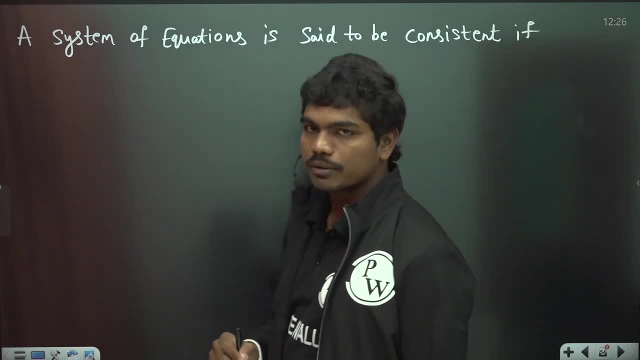 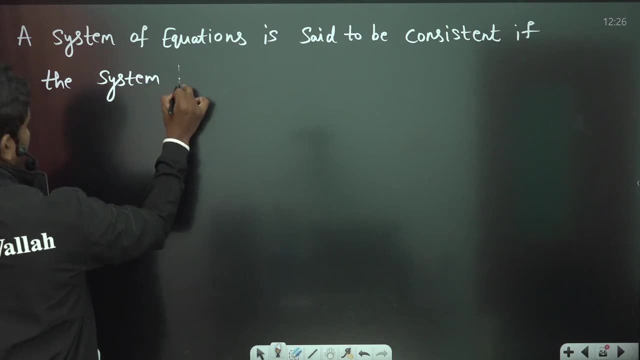 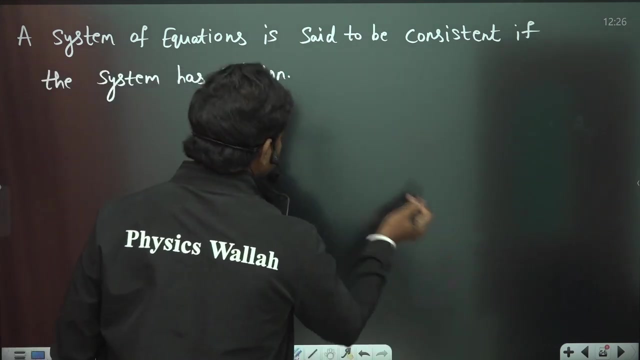 consistent. if a system of equations is said to be consistent, if The system has a solution, This is if the system has Solution, the system has Solution. So, basically, what's the meaning of this? this? solutions can be unique or infinitely mean, it doesn't matter. but as 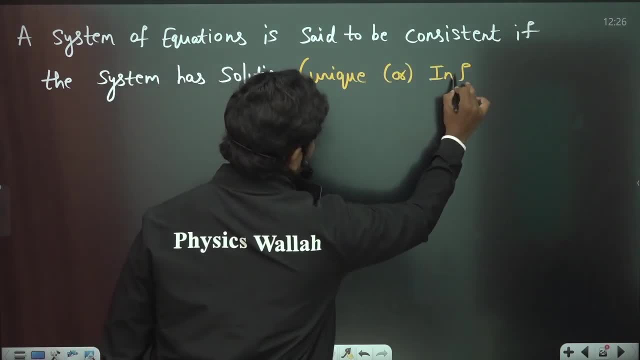 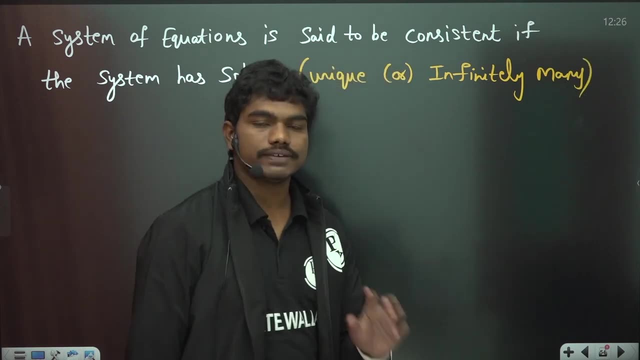 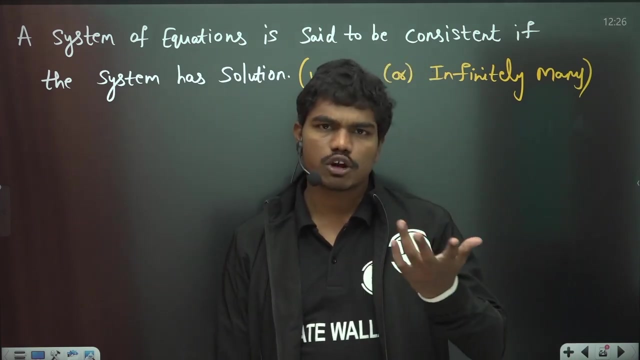 Long as the system has a solution, it's called consistent system. It can be unique solution or it can be infinitely many solutions, But as long as the given system has a solution, We call that system as a consistent system. and for the system to be consistent, that you can be 0 or it cannot be equal to. 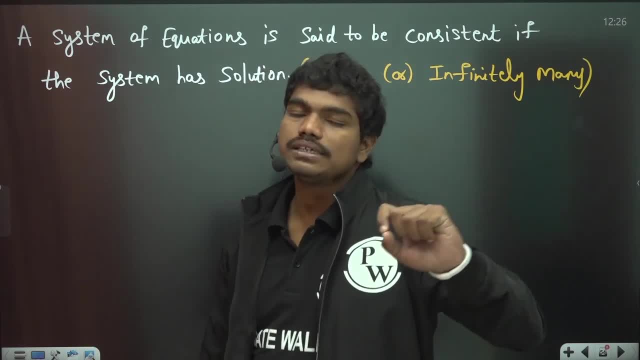 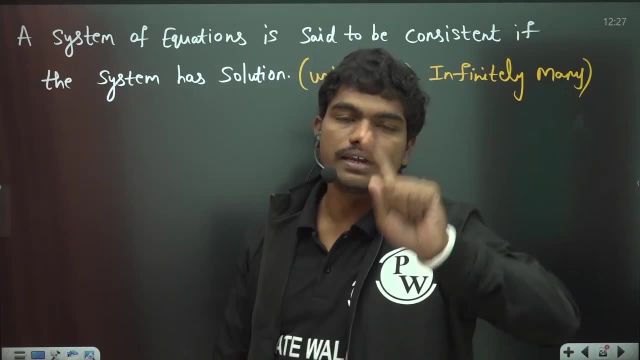 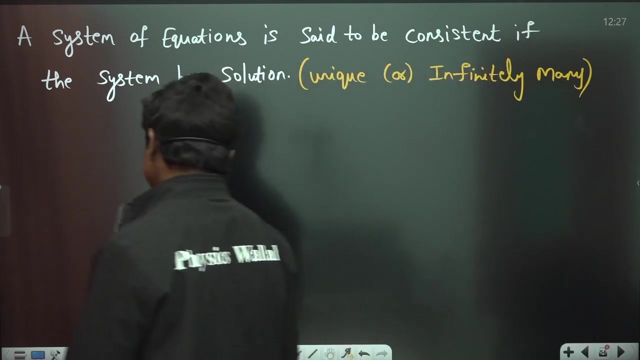 0 also like this, depending on these cases. but one thing is very clear: as long as your determinant of a is, it is not equal to 0. the system always and always has a inverse and that system will have A unique solution. clear. now let us talk about homogeneous system of equations. Okay, so for homogeneous system of equations. 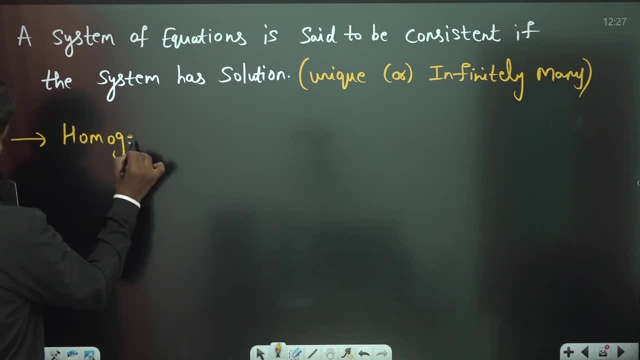 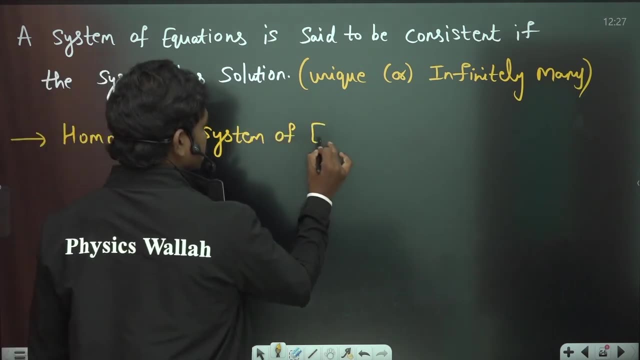 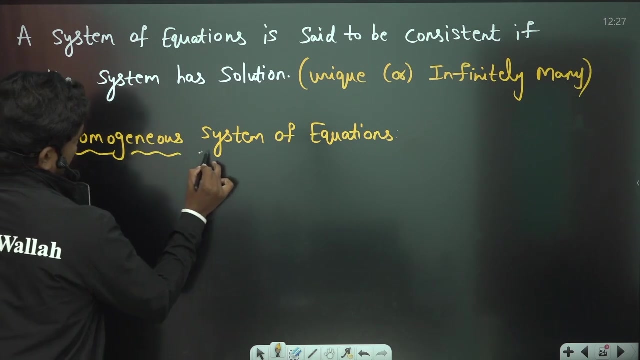 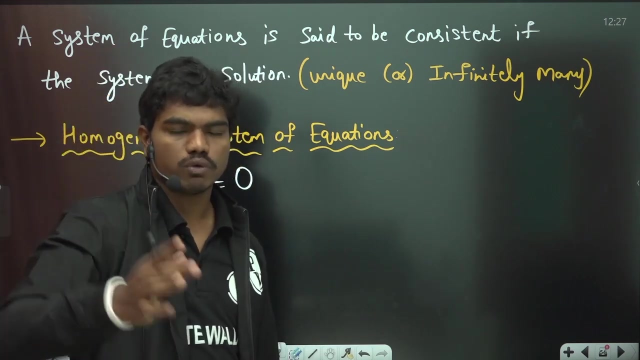 You can write homogeneous, Homogeneous System of equations. Homogeneous system of equations means basically you have right-handed term. this B matrix is actually a null matrix- 0. okay. so whenever the right hand sides of the equations are 0, you can write 0 into x power 1, 0 into y, power 1, whatever you want, and all the four terms. 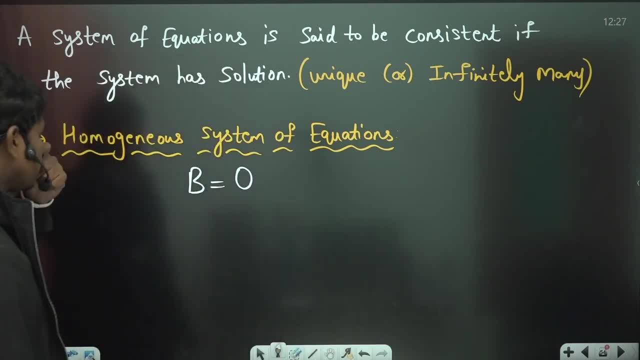 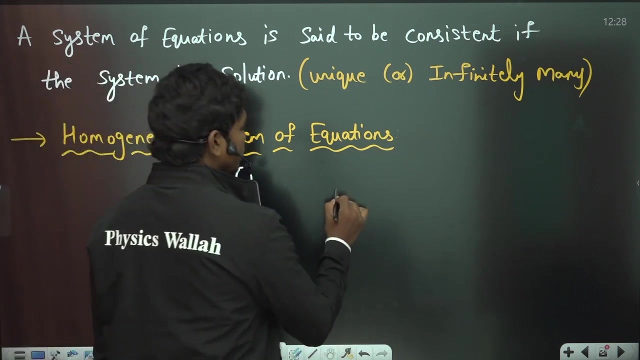 of the equation was single degree, so that's why this system is called homogeneous system. whenever this coefficient matrix is- i mean this constant matrix- is 0, this implies a into x is equal to 0. is the system? now try to tell me one thing. let us suppose if your a is like this: a 1, 1 a 1 2 a 1, 3. 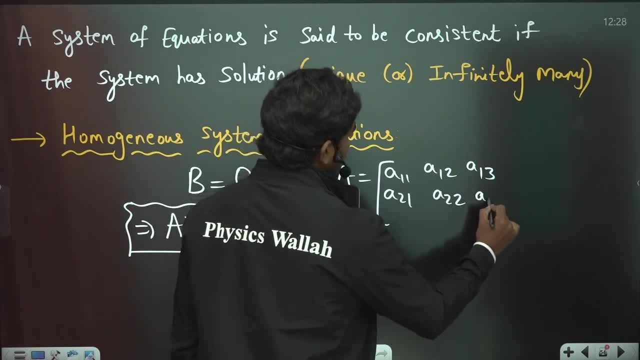 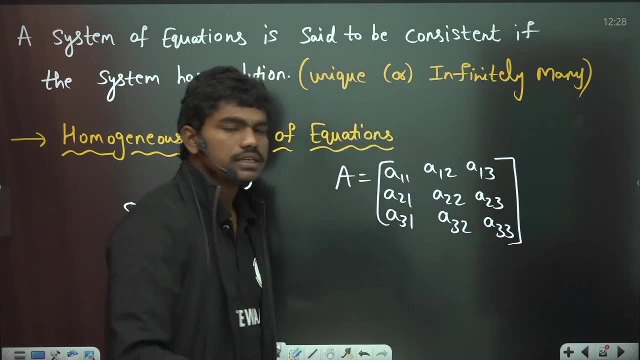 a 2, 1 a 2, 2 a 2, 3, a 3, 1 a 3, 2 and a 3, 3. why the equations are: a 1, 1 x plus a 1, 2 y plus a 1, 3. 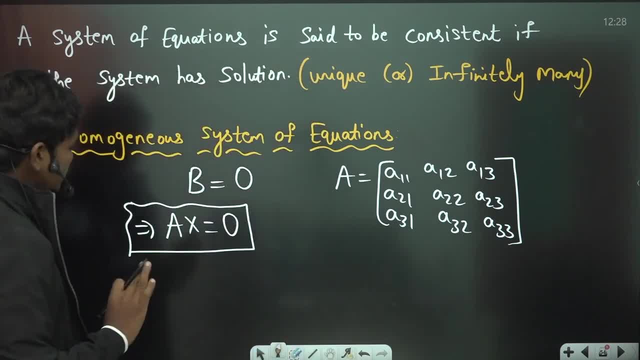 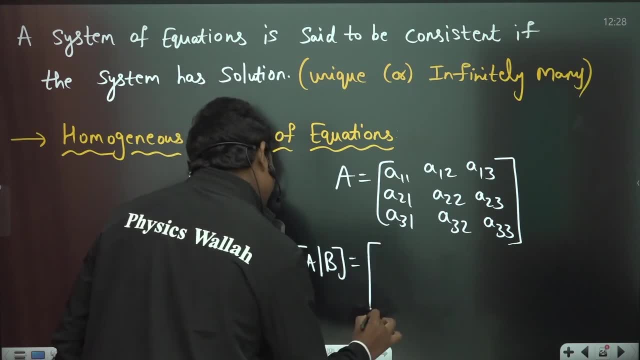 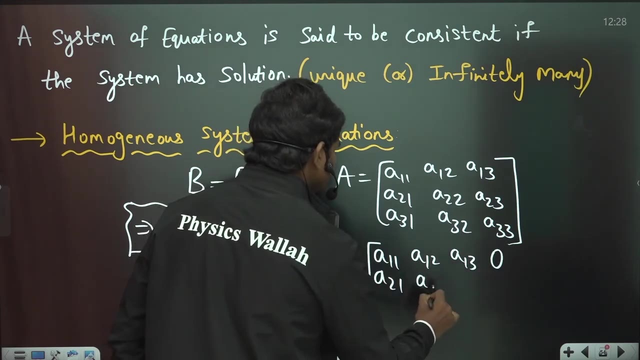 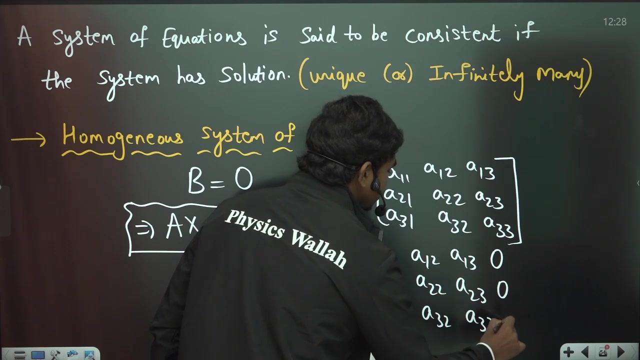 into z is equal to 0. similarly, the other two equations. now, if this is a consistent system, now try to tell me one thing: a augmenting augmented b, a augmented b will be a: 1, 1 a 1, 2 a. 1, 3, 0 a. 2, 1 a 2, 2 a 2, 3, 0 a 3, 1 a 3, 2 a double 3, 0. 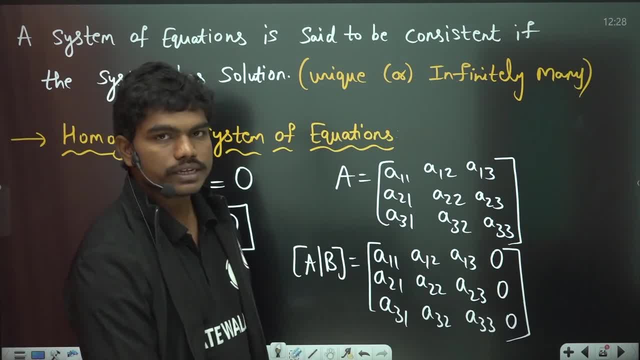 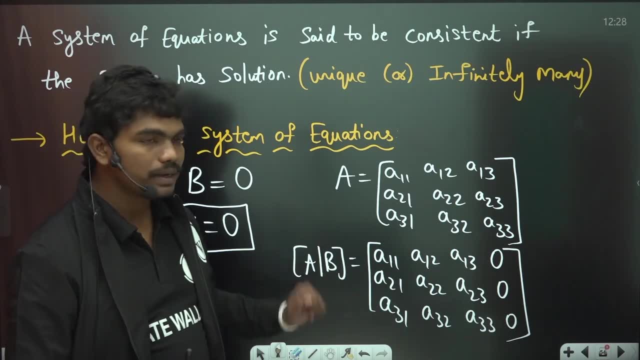 okay, so you will have this system. now try to tell me one thing: if you are interested to calculate a rank of a- okay, it's a 3 by 3 matrix- you will calculate. if you want to calculate a rank of this augmented matrix, how we will calculate. 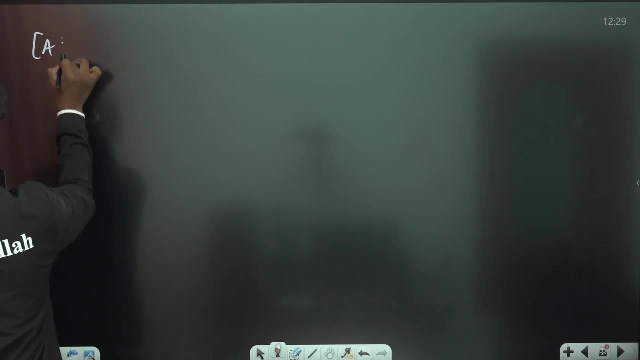 look, a augmented b is a 3 by 4 matrix, correct. a augmented b is a 3 by 4 matrix. so basically: a 1, 1 a, 1, 2 a. 1, 3, 0 a 2, 1 a 2, 2 a, 2, 3, 0 a 3, 1 a 3, 2 a double 3. this is again 0 now, if you see this. 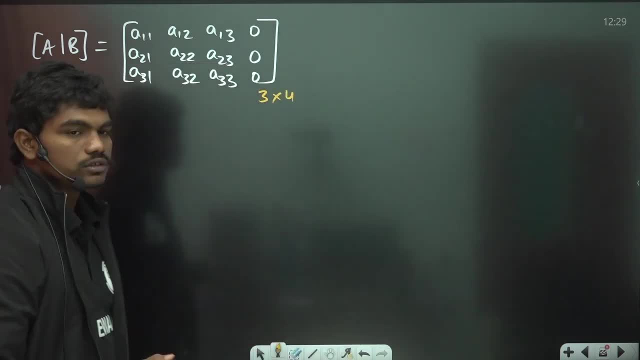 is of size 3 by 4. if this is of size 3 by 4, the maximum size minus that you can take out of this is of size 3 by 4. so you will have this 3 by 3, third order correct. so if you take 3 by 3, 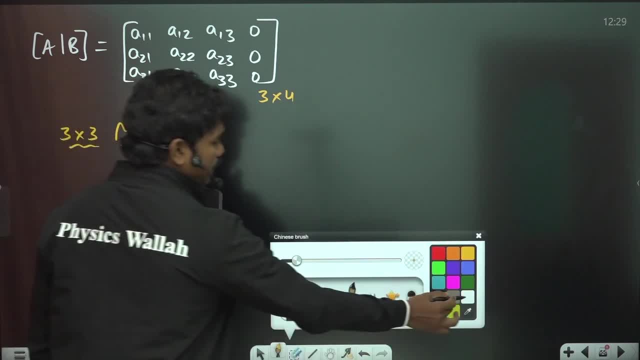 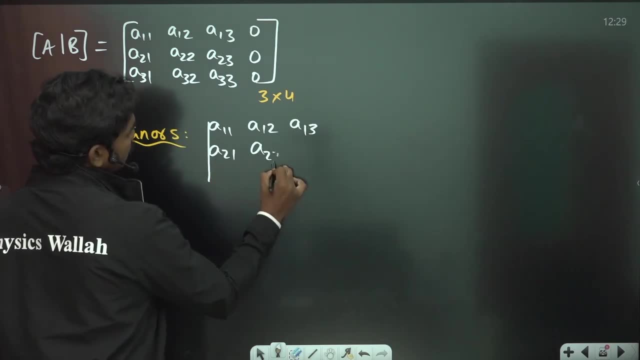 3 by 3 of size 0. I will tell you one thing here, one very important point I want to reveal here. so if you want to take 3 by 3 minus, what are the matrices, the, what are the determinants? you can have a 1, 1 a 1, 2 a 1, 3- I have deleted the fourth column, so a 2, 1 a 2, 2 a 2, 3 a 3, 1. a 3, 2 and a double 3, so this is one determinant. okay, now, if you delete the third column, then you have 1, 1 a 1, 2, 0 a 2, 3, 0 is equal to 0. so this is 2 by 3 minus delta integral a 1我觉得. CAS良 regional. a 1, 1 a1. tool a1: THEY have deleted the fourth column, so a 2, 1 a, 2, 2 a, 2, P a A entre a 3 and a double 3, so this is one determinant. okay, nhım now, if youvan. 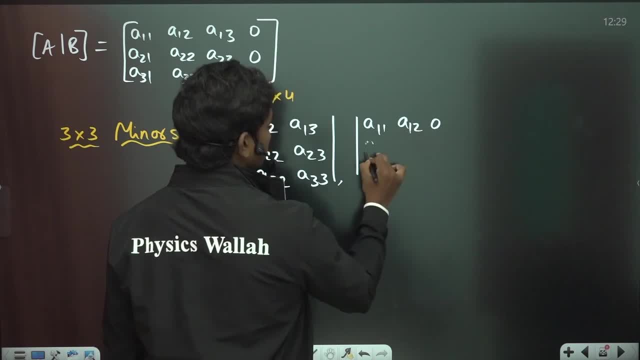 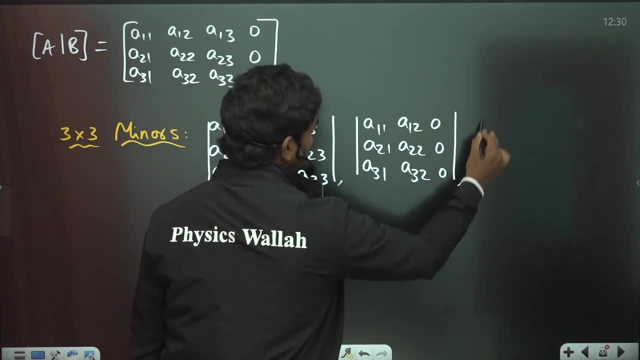 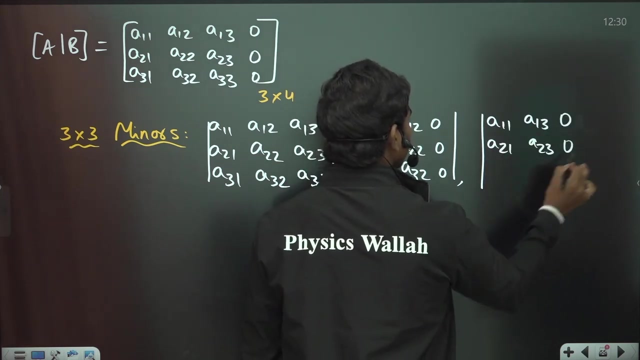 column, then you have a 1, 1 a 1, 2, 0 a 2, 1 a 2, 2, 0, a 3, 1 a 3, 2, 0. you have deleted the third column. next, if you delete the second column: a 1, 1 a 1, 3, 0 a 2, 1 a 2, 3, 0, a 3, 1, double 3, 0. this is one minor. 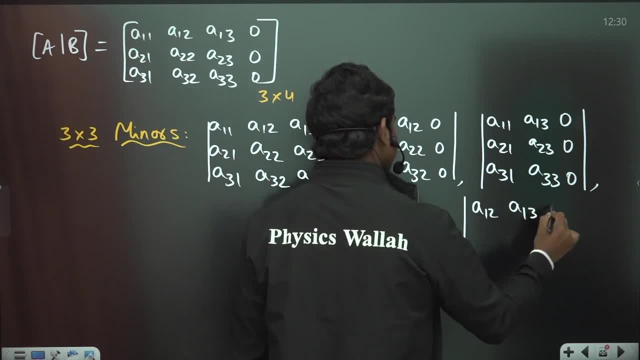 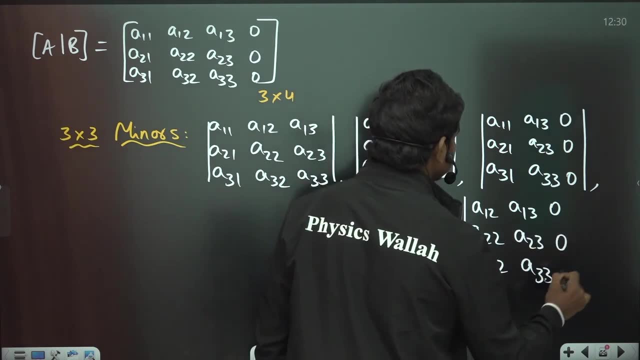 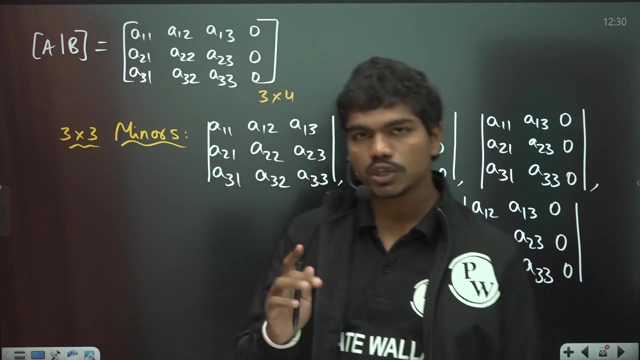 and the last minor, if you delete the first column: a 1, 2 a. 1, 3 0 a. 2, 2 a, 2, 3 0. a. 3, 2 a, 3, 3, 0. so these are the four 3 by 3 minors now, the rank being 3 or less than that depends on only one determinant. 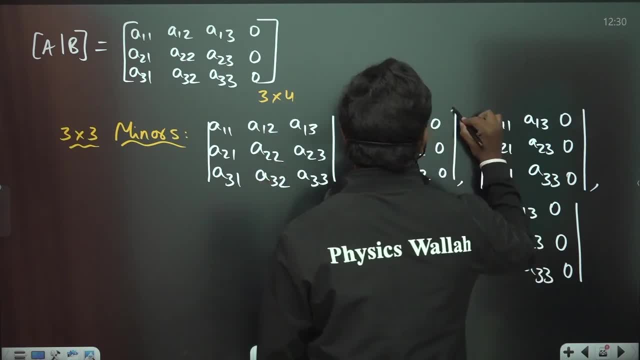 which is nothing but this determinant. why? because this determinant value is 0. you have a complete 0 column. okay, you have one complete column of zeros, so this determinant is 0, this determinant is also 0, 0, 0 and this determinant is also 0. so your rank being 3 or less than 3 depends upon this. 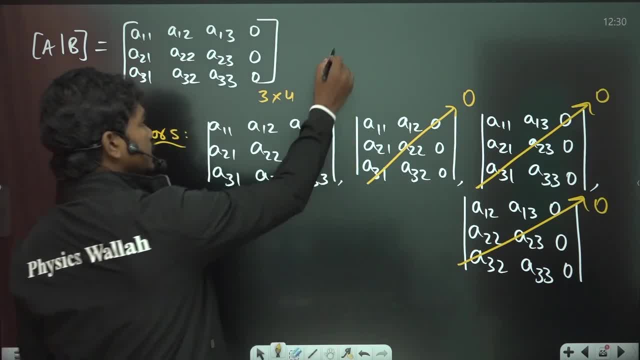 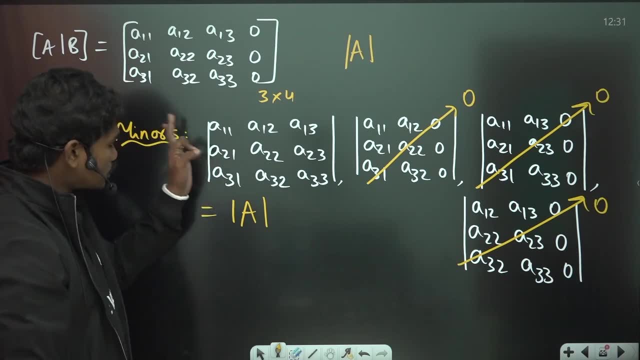 that a correct. now try to observe one thing: if you take this matrix a, if that a is equal to 0, then this, all third order minors, will also be 0, because the rank of this augmented matrix depends only and only on this determinant, because all these, they are zeros by default. now tell me one thing, can i? 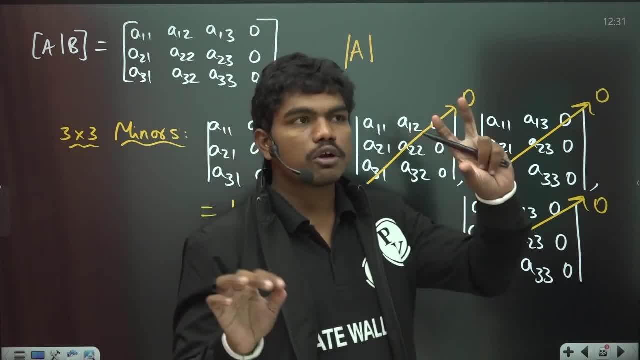 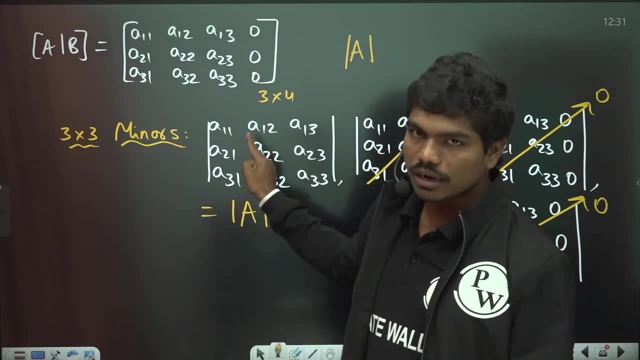 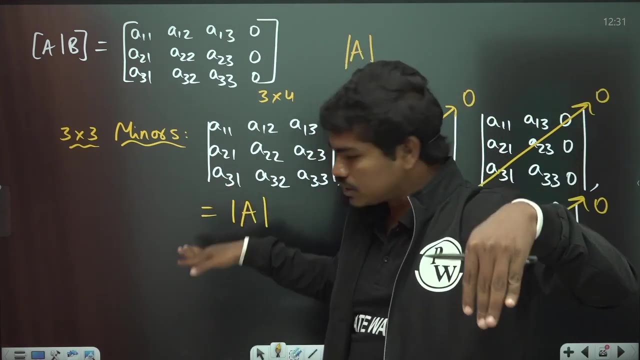 say one thing here: we don't get any case like rank of a not equal to rank of a augmented b correct. why? because this rank of a augmented b depends upon this determinant, which is again depending on that a. so if that a is 0, then rank of a will be something less than 3. here also, this will be. 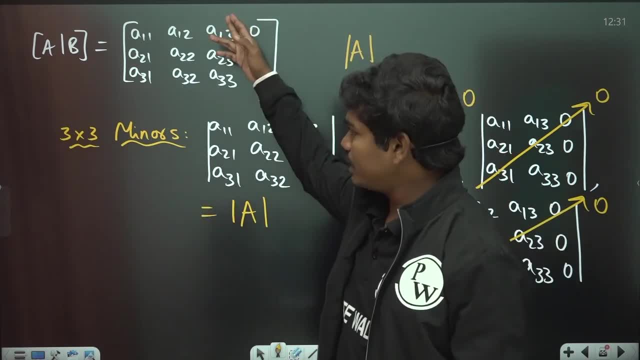 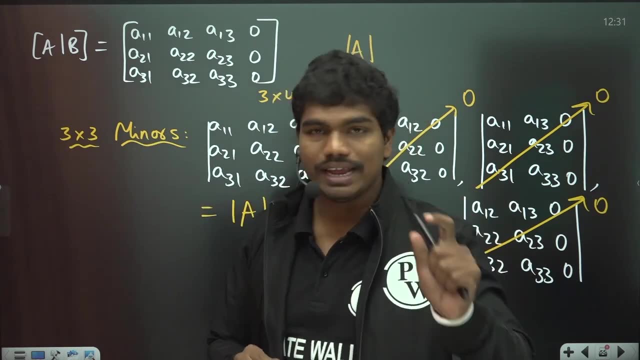 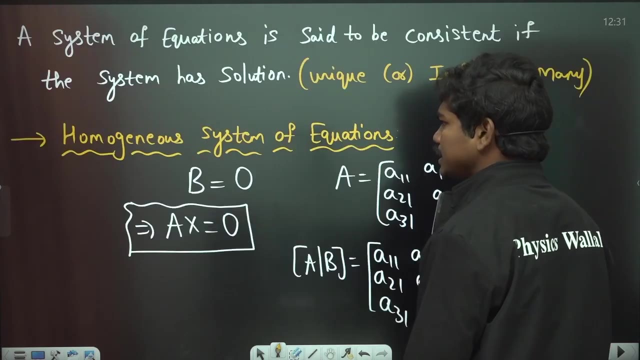 something less than 3. if that a is not 0, then rank of a is 3. this is also not 0, like a augmented b is also 3. so here we don't have any case like rank of a is not equal to rank of a augmented b. now, if you see this condition, if you see this condition, this case, 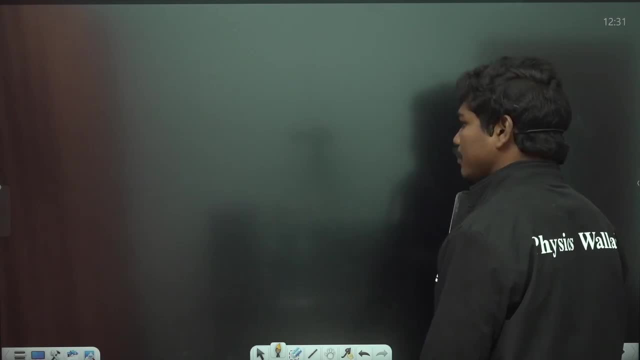 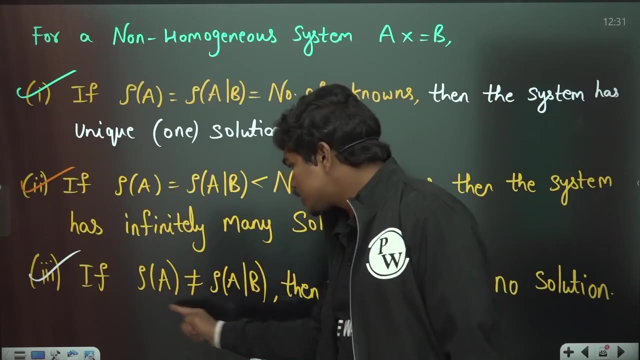 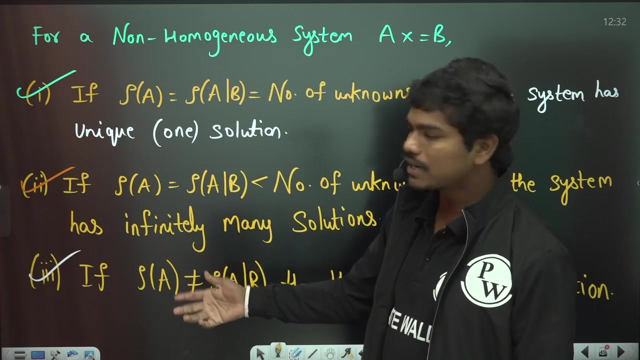 is ruled out. yes or no means. oh, i think something happened. okay, fine. so if you see one thing carefully, in this case of homogeneous system of equations, this third case is not anymore value getting valid means. these two will be always same, but it depends depending upon the debt value it. 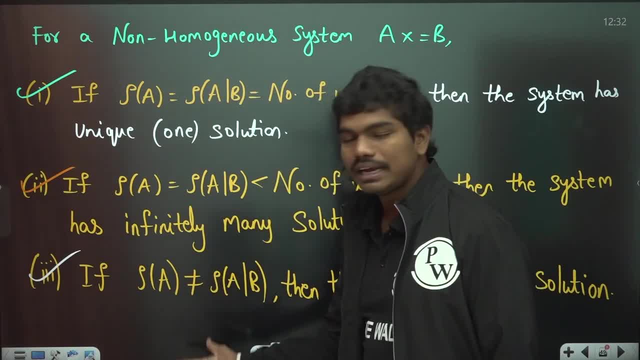 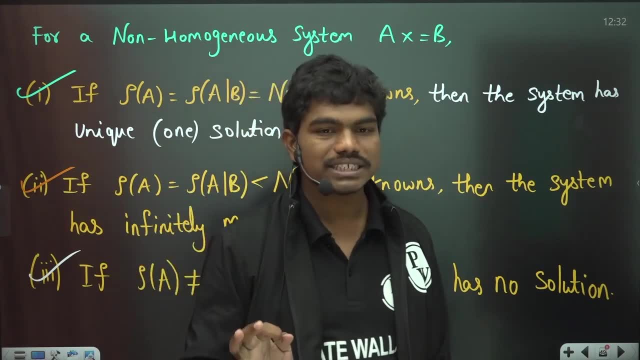 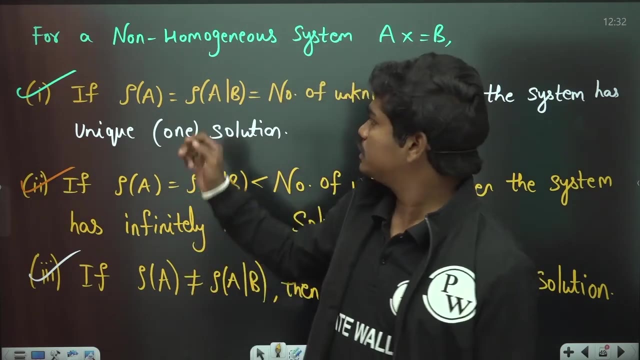 has unique or infinitely many, but this case cannot happen in case of a homogeneous systems. what is the meaning of that? the system always has solution, yes or no. so homogeneous systems always has a solution, and the solution is nothing but x equal to 0, y equal to 0 and z equal to 0. if you replace 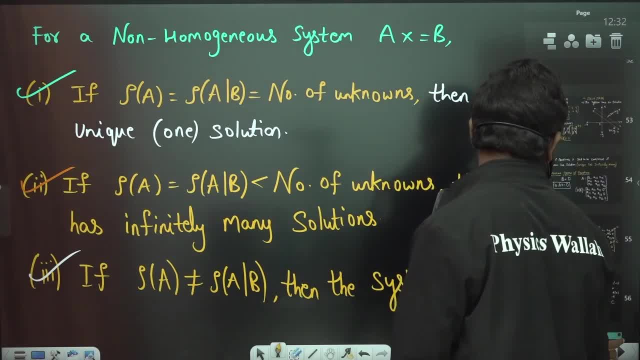 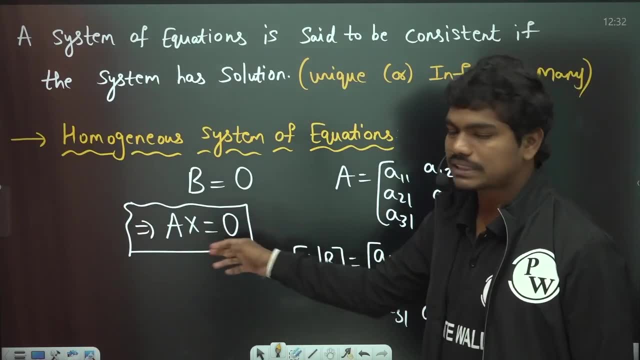 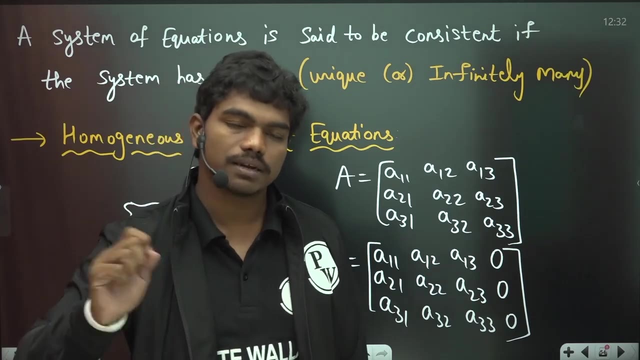 all these coefficients to be zeros. yeah, so if you see this equation, if you replace all this x, y, z values with the zeros, then definitely this equations get satisfied. so in case of homogeneous systems, it's never a case like the system don't have a solution. the system always has a solution and the solution is x equal to 0, y equal to 0 and z is equal to 0. 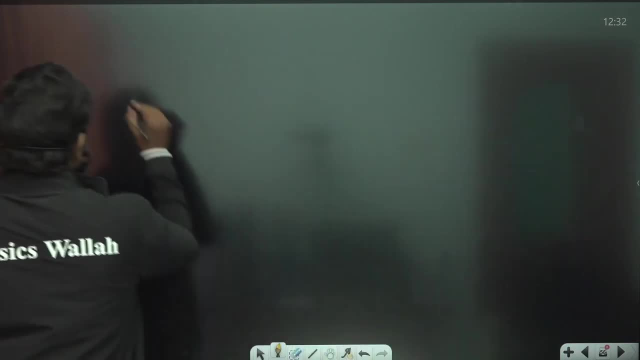 okay. so here you can see, rank of a will be always equal to rank of a augmented be. that's why- which means you can it always rank of a is equal to a rank of a augmented be, which means the system always has a solution. the homogeneous system. you can write better: the homogeneous system. 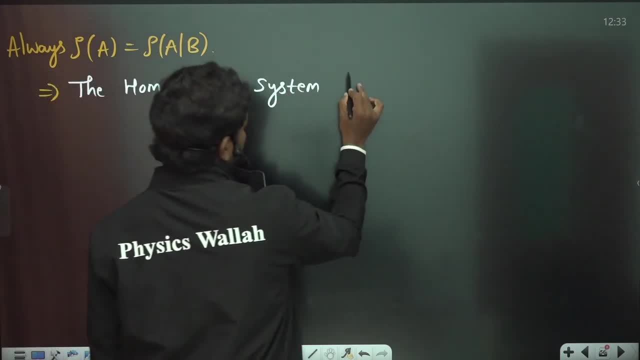 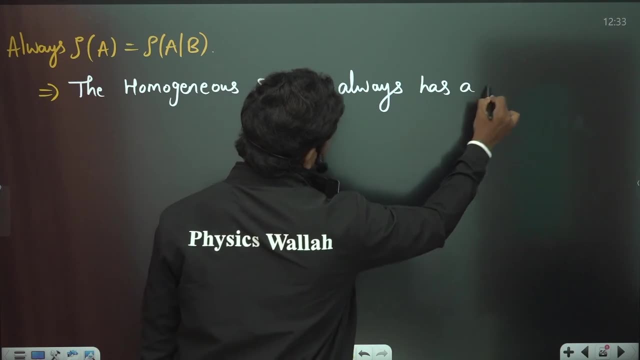 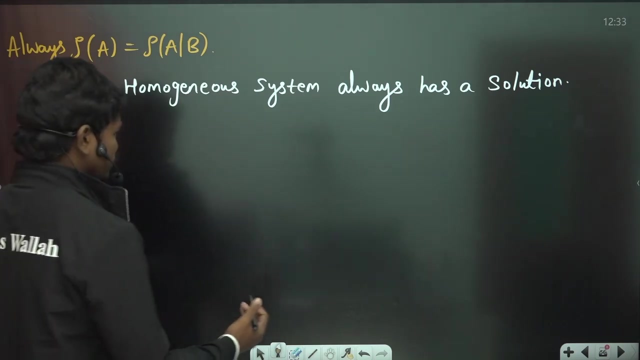 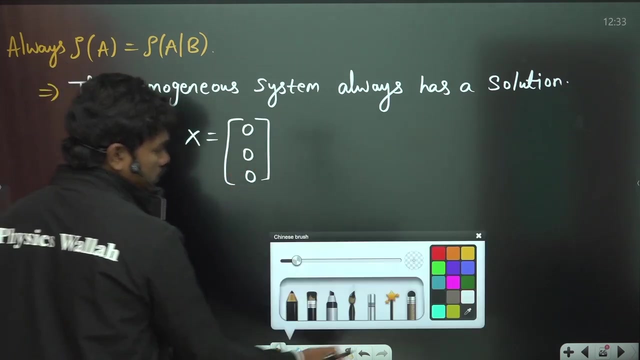 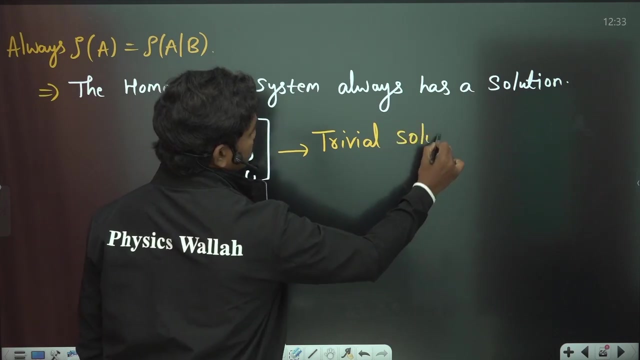 you homogeneous system has, you know, always has a. the homogeneous system always has a solution, always has a solution. okay, so now if you see this, what is that? solution x is equal to 0 0, 0 and this solution is called trivial solution. trivial solution: what is the meaning of trivial independent? it is solution always by default. 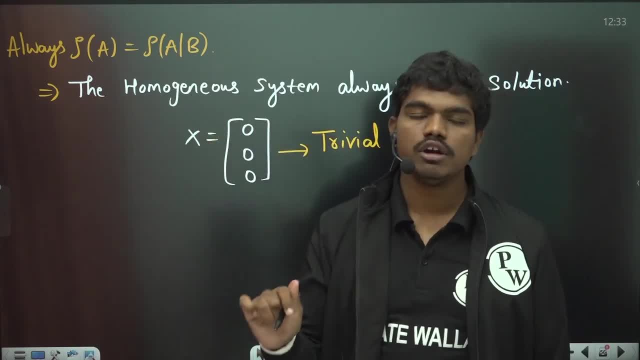 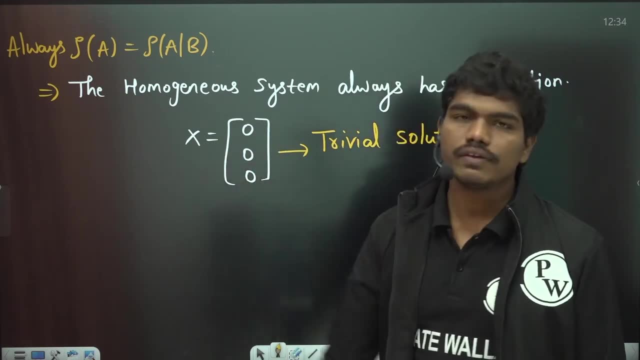 for when you put x equal to 0, y equal to 0 and z is equal to 0, you need not bother about what are the nine coefficient values correct? so this solution always acts as a solution for the given homogeneous system of matrices. okay, and this solution is called trivial solution. now let us 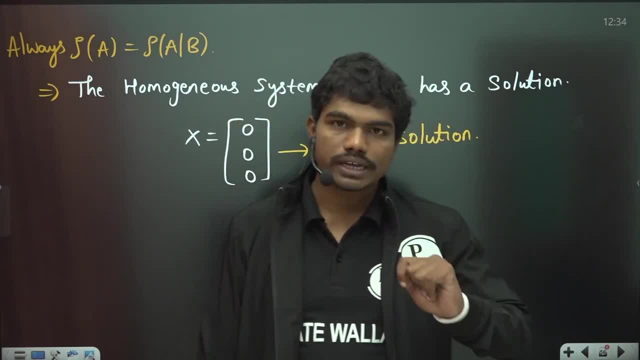 suppose, if that a is not equal to 0, for example, if that a is not equal to 0, then what happens? a rank of a will be equal to 0. if that a is not equal to 0, then what happens? rank of a will be. equal to 0. if that a is not equal to 0, then what happens? rank of a will be equal to 0 if that a is not equal to 0, if that a is not equal to 0, if that a is not equal to rank of a augmented b. 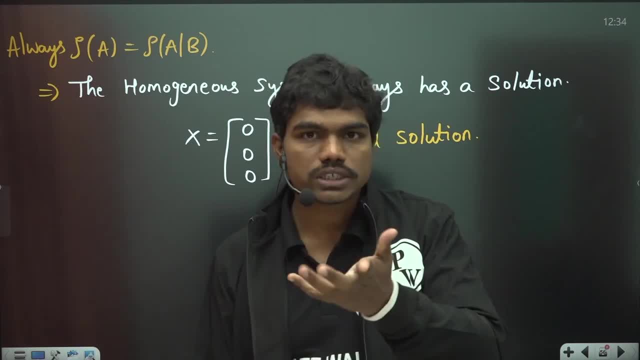 rank of a augmented b, and that is equal to number of unknowns, then the system will have, and that is equal to number of unknowns, then the system will have unique solution, obviously unique solution, obviously, so that unique solution is nothing but this solution. now, if the homogeneous 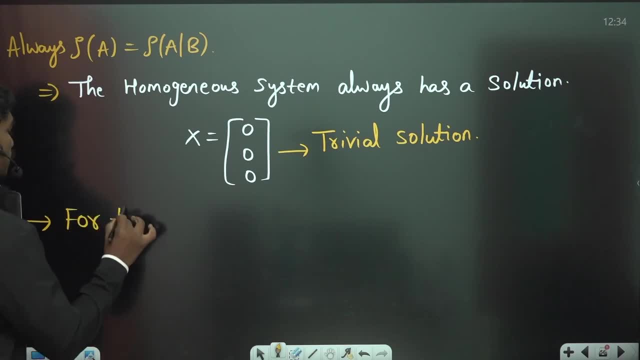 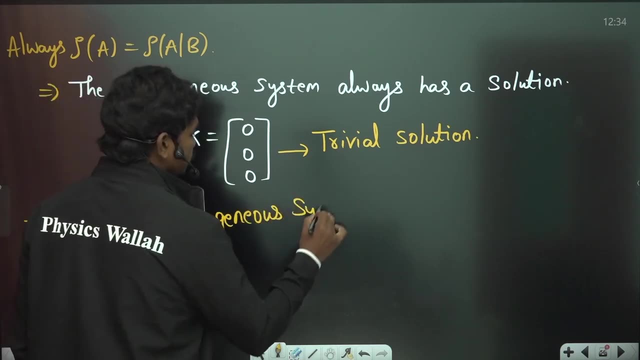 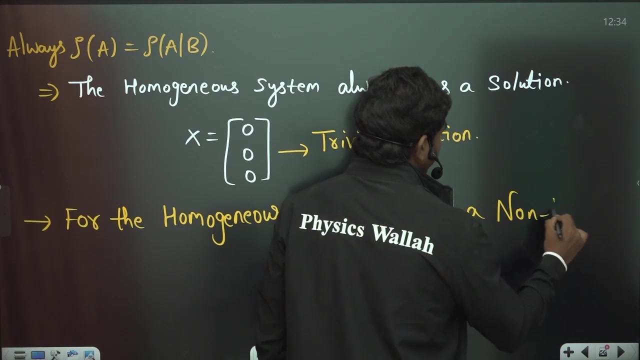 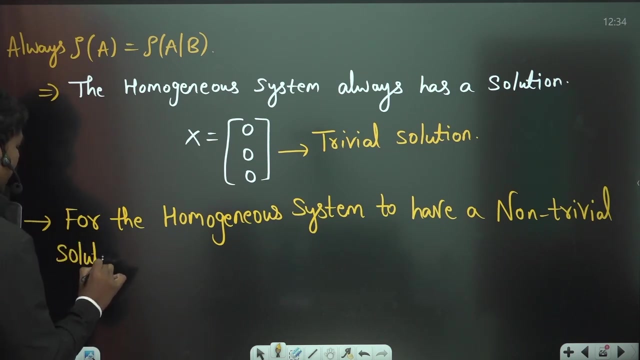 so that unique solution is nothing but this solution. now, if the homogeneous system for the homogeneous system, for the homogeneous system, to have a non-trivial solution, to have a non-trivial, to have a non-trivial solution, to have a non-trivial solution means, apart from 0 comma, 0 if 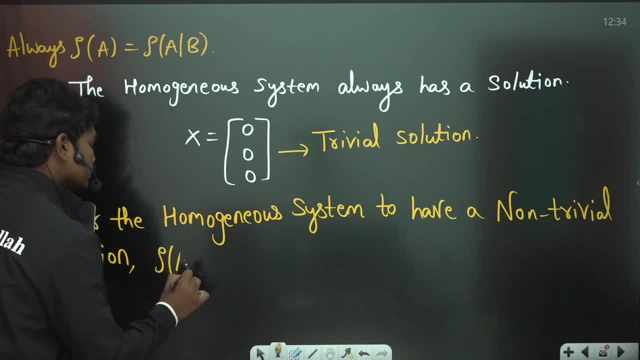 non-trivial solution means, apart from 0 comma 0. if it want to have some other solution, then you know it want to have some other solution, then you know definitely. rank of a less than n- n is basically definitely. rank of a less than n. n is basically number of equa unknowns. if you see, this implies 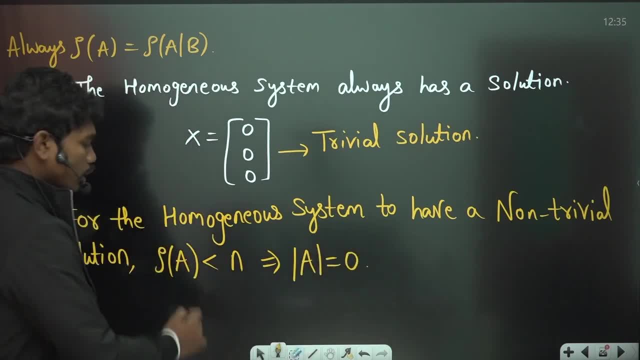 number of equa unknowns. if you see, this implies determinant of a should be definitely zero, correct. determinant of a should be definitely zero, correct because a is a n by n matrix. if a is n by n matrix, because a is a n by n matrix, if a is n by n matrix and if rank of a has to be less than n, then 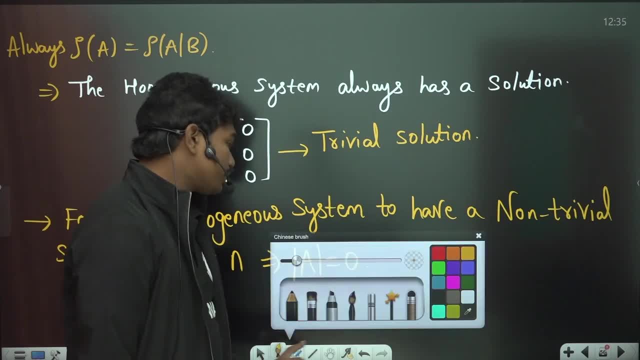 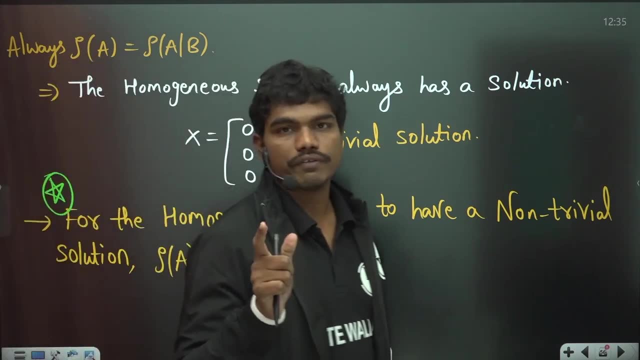 and if rank of a has to be less than n, then definitely this determinant has to be zero. and this point is very, very important point for get examination- that for the homogeneous system to have a non-trivial solution, the determinant of the coefficient matrix should be zero. why this is important? because 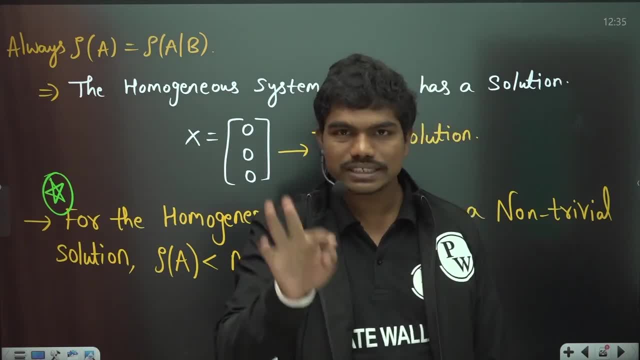 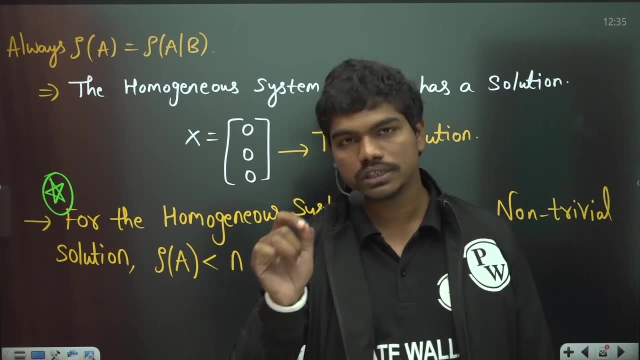 they give you a question like this, they'll give you three homogeneous equations and out of these nine coefficients, they don't give one coefficient value and they'll ask you for the given system to have a non-trivial solution. what is the code constant or the unknown value? so basically what? 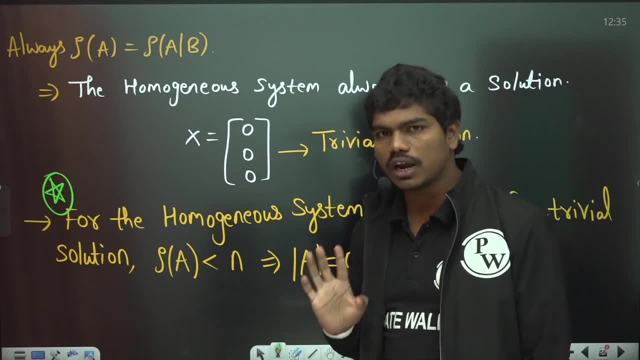 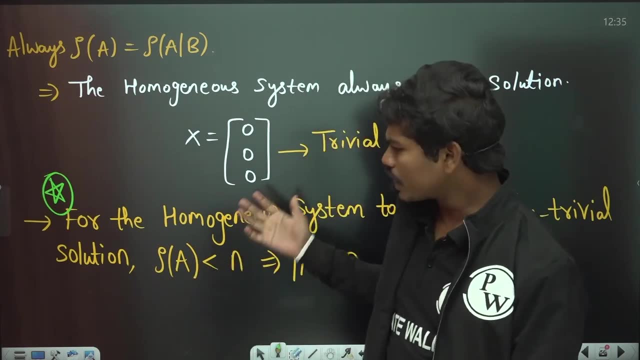 you will do, you liquid the determinant to zero, so you'll have one equation with one unknown and you will, you know, uh, write the solution of this clear. so this is clear. so this is how we decide whether the system has you know, whether the system has a solution or you don't. 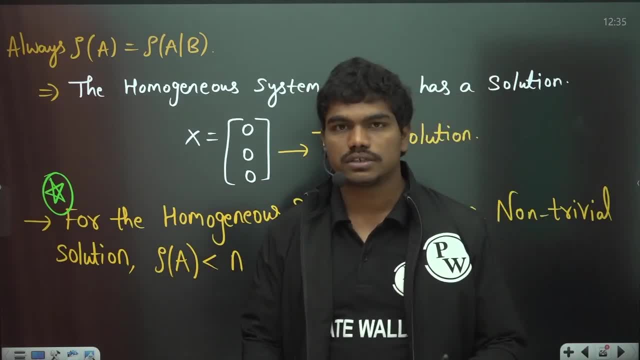 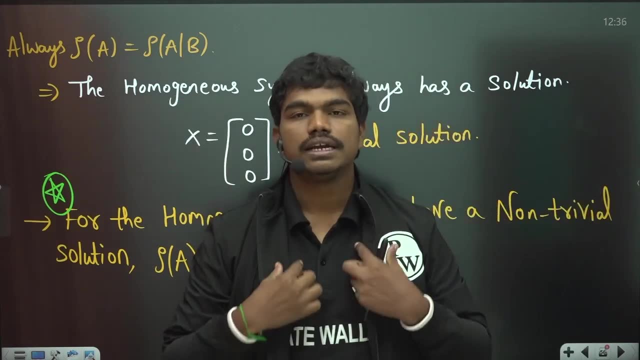 have a solution generally clear. so this is basically the talk about system of equations. almost half now we have discussed on system of equations. so normally if you take non-homogeneous systems, depending upon the ranks of a and a augmented b, you decide how many solutions does. 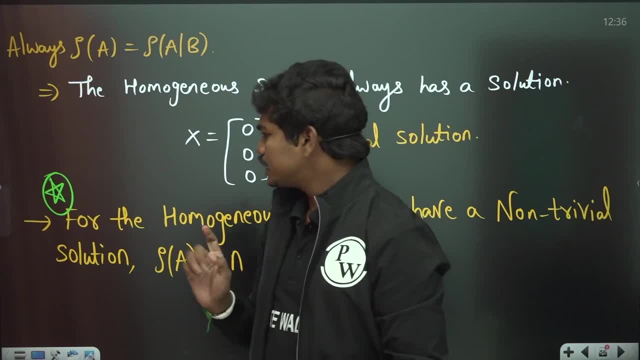 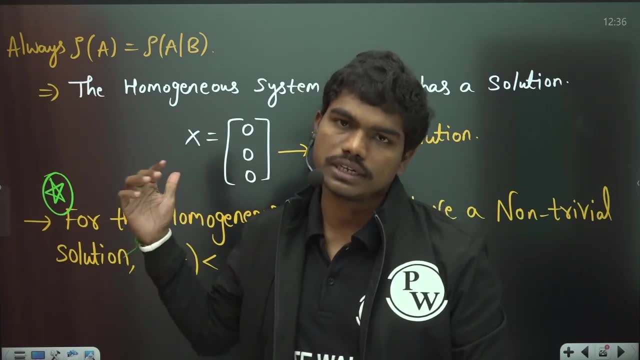 the set of equations have actually clear. so this is one very important part of this linear algebra and the main crux of this linear algebra is talking about this. vectors, or you can say this: equations, basically here clear. i hope you understood this. so with this we close this part. 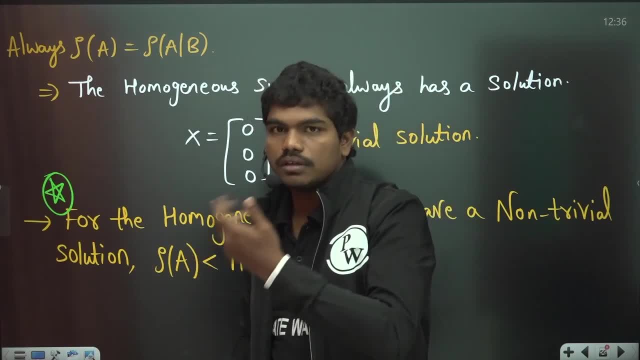 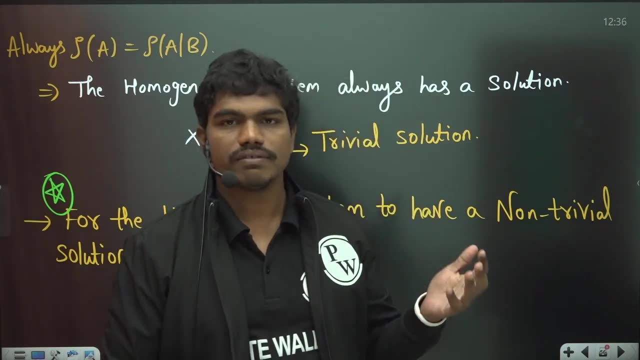 three, which is system of equations and you know, basically this ranks of the matrices. okay, now i would like to talk. okay, before going for one last part, which is eigenvalues and eigenvectors, i would like to talk something on linear dependent vectors and linearly independent vectors, basically, okay. 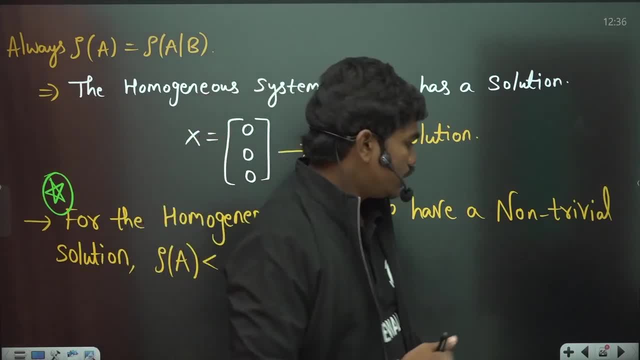 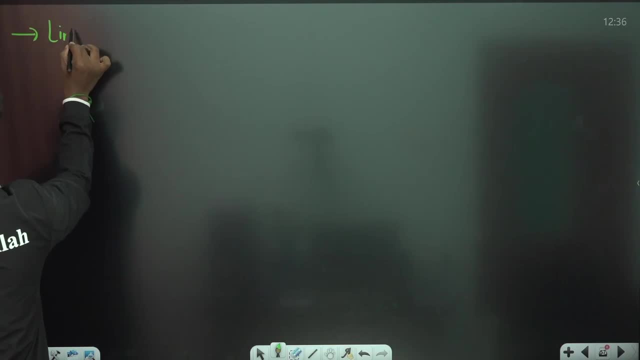 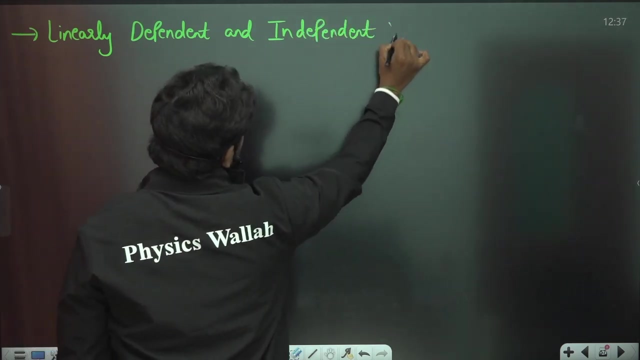 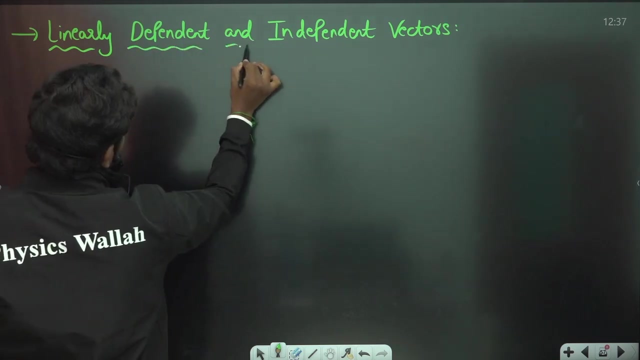 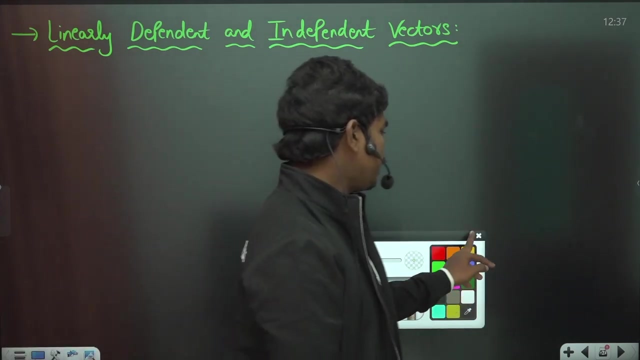 so let us talk about that for a while. okay, now see carefully. here i'll talk about linearly dependent and independent vectors. linearly dependent and linearly dependent and independent vectors. let us see. what are this? linearly dependent and independent vectors? why i'm calling vectors? because 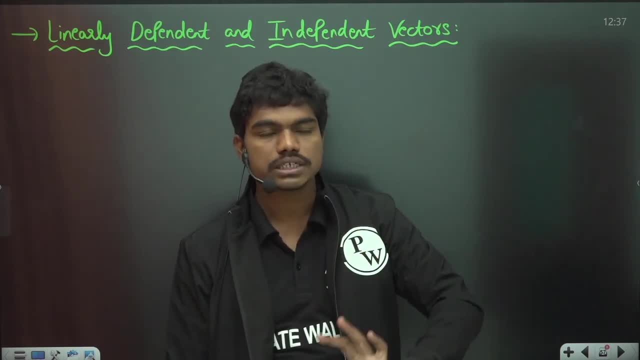 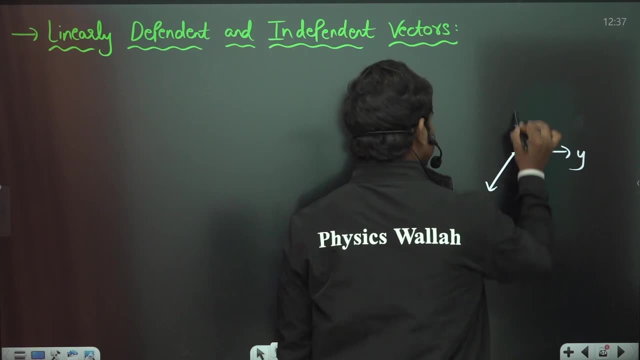 normally, if you take 3d space, for example, if you are talking in three dimensional space, if you want to draw a position vector, for example, let us suppose x, y and z. let us take in this direction a right-handed coordinate system. so let us suppose, if you want to take a point in space, 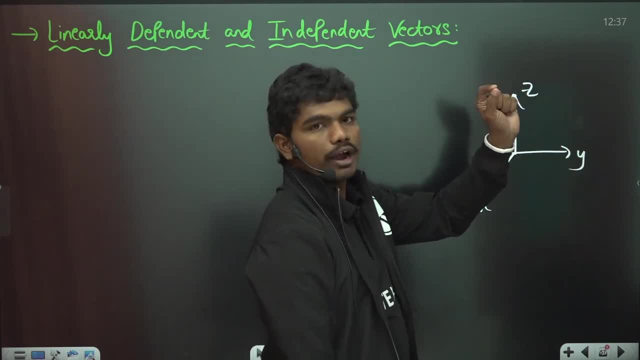 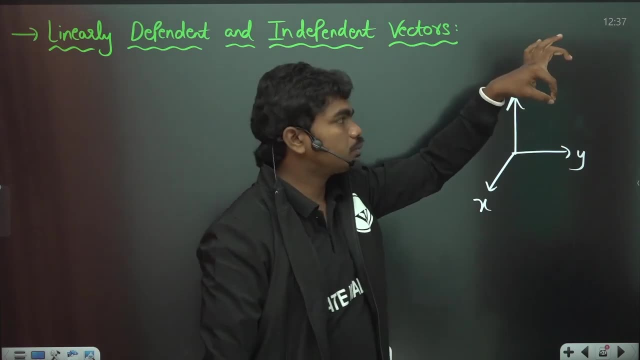 let us suppose this: my finger tip is a point in space which i want to talk about, then if i can connect this horizon to this fingertip, to a vector, then definitely this point has some coordinates in space: a, b, c, correct? so for three coordinates: x coordinate, y coordinate and z coordinate. now, 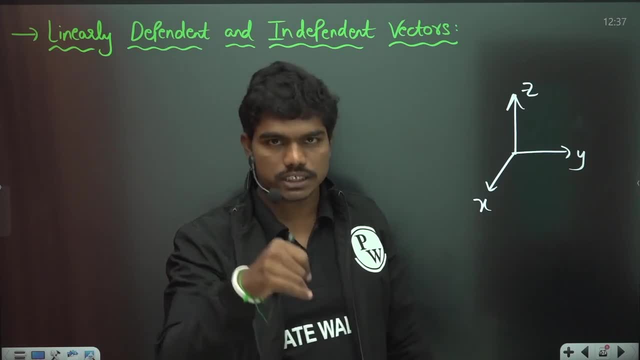 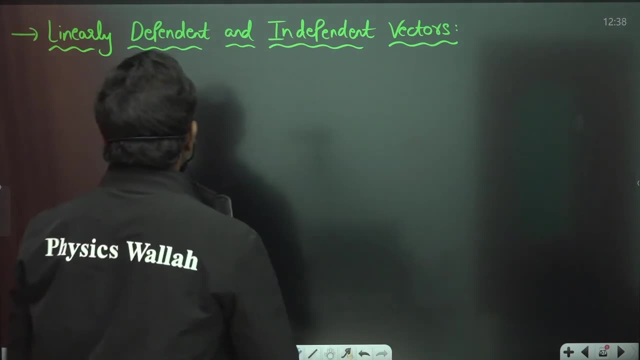 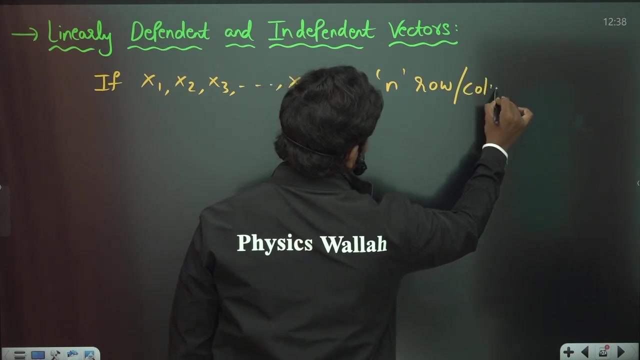 these three coordinates can be represented as a matrix: x, y, z. that's why we deal generally vectors in matrices. okay, so now, if you see, anyhow, if x, 1, x 2, x 3 and so on, x, n are n, row or column vectors, what is column vectors basically? 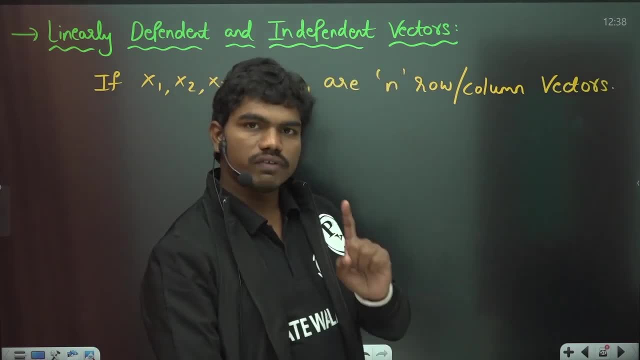 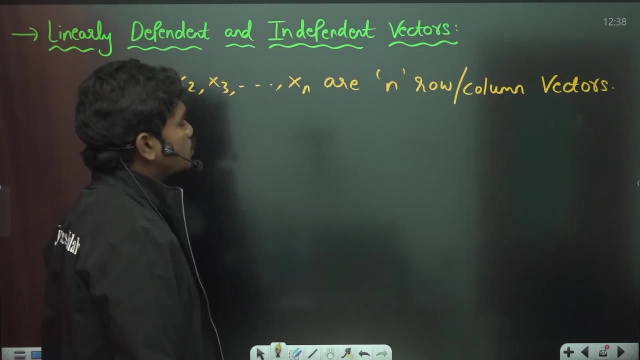 these are column matrices. if a matrix has only one column, it's called a column matrix. if a matrix has only one row, it's called a row matrix, basically okay. so now if x, 1, x, 2, x3 and so on, xn are in row or column vectors, vectors and and k1, k2, k3 and so on, xn by zero. okay, so x, n, two, xn, A and A is column vectors. at 1 x two is column matrix. so if we take 1 x 2 and x, 2 and xn is column vectors. 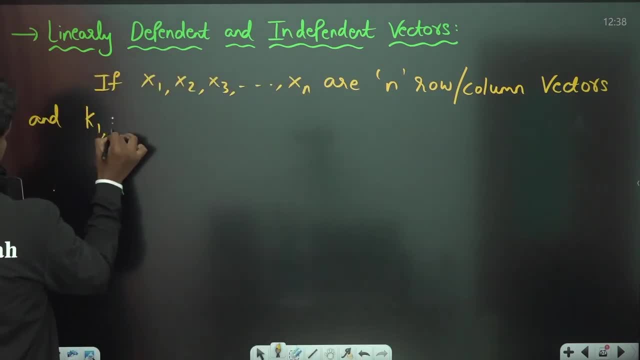 but let us like, assum A is column from R and this is a column matrix, and up here we have 1, x2 x, n, so this is a column vulnerability accessory. so let us think, helps us know if we think about column vectors and, and in fact this, we need toelly catch them from mfc as well. so but we asked point 3 and M, f1 and Fransi, they should create an算s sets. 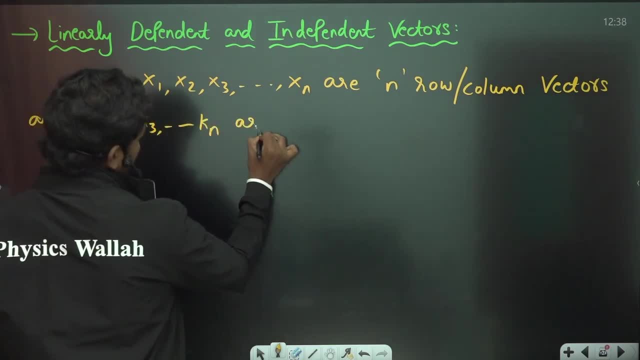 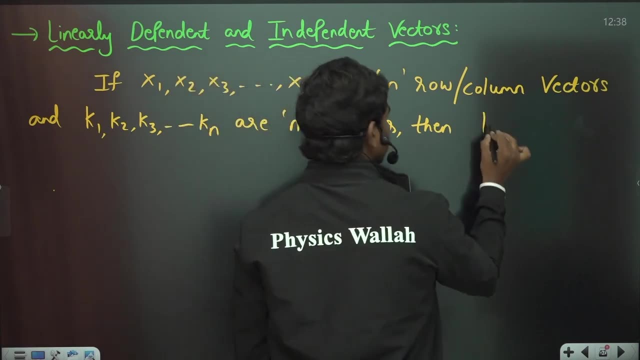 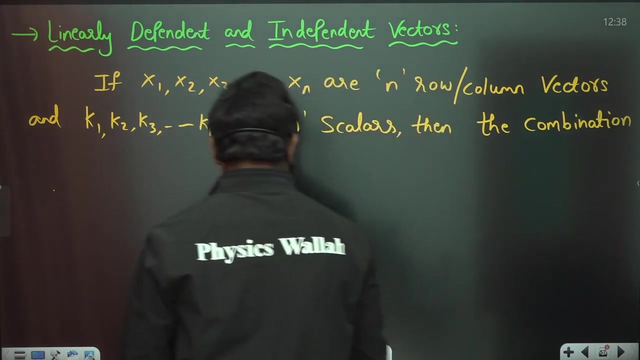 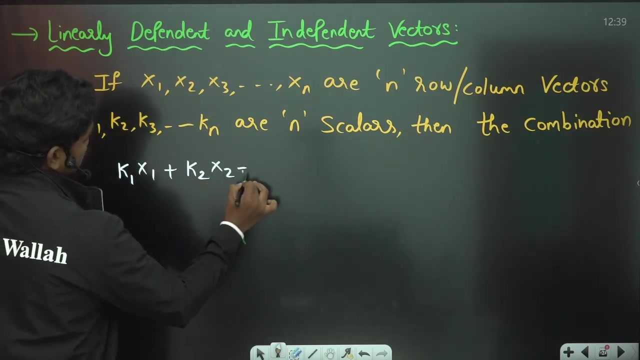 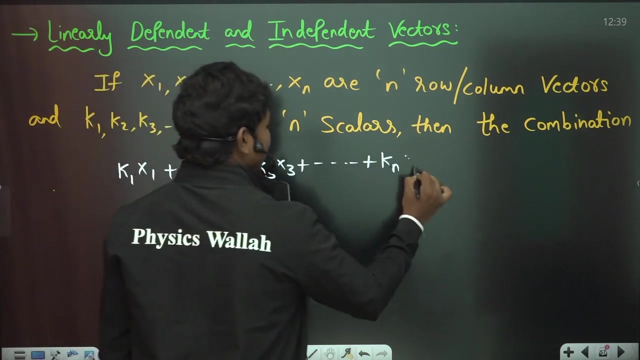 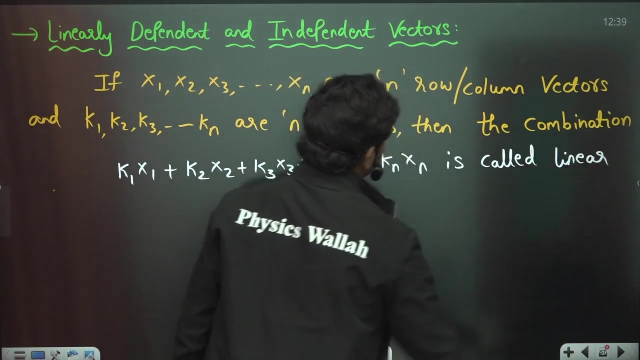 and so on. kn are n scalars, are n scalars, then the combination, then the combination, then the combination: k1, x1, k1, x1 plus k2, x2 plus k3, x3, and so on. kn, xn, xn is called linear combination of these vectors, linear combination of vectors. 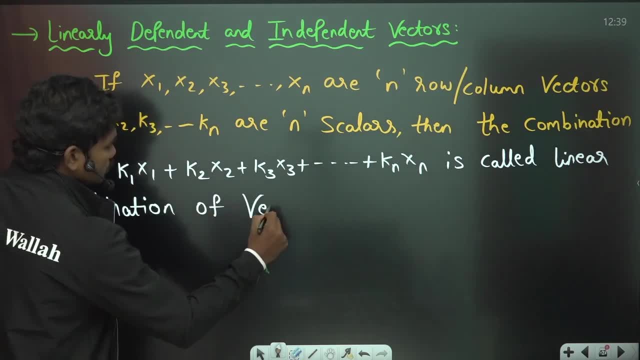 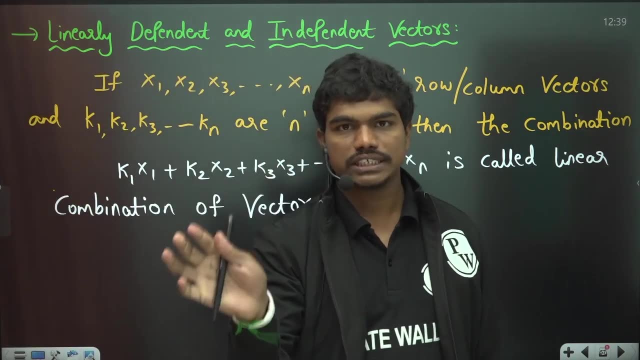 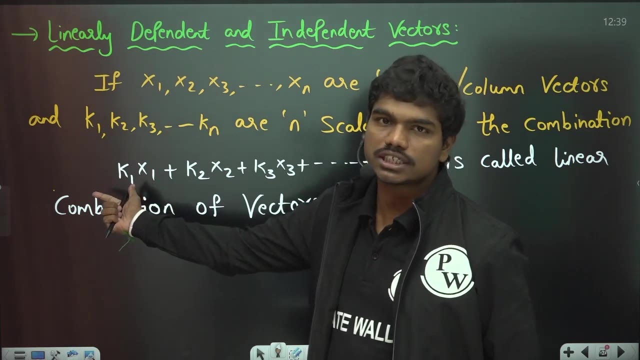 these are called linear combination of vectors. okay, now you can understand one thing, basically. what is linear? just, we are changing the size, we are not changing any direction. so if you see, this vector is multiplied with this scalar k1 so that the magnitude of this vector changes, but the direction doesn't change, correct? let us suppose, if i take this: 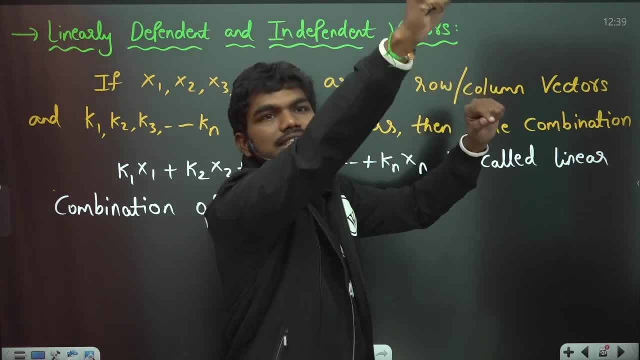 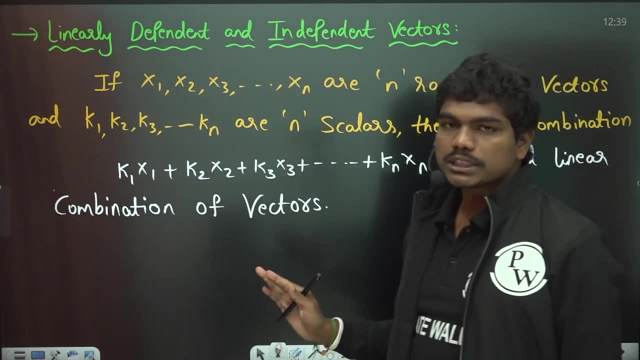 fingertip this vector. let us suppose, if i two times of this vector, the length changes, but the magnitude, i mean the direction of the vector, doesn't change. okay, so that's what i'm telling you. this is called linear combination of vectors. now this combination is said to be linearly. 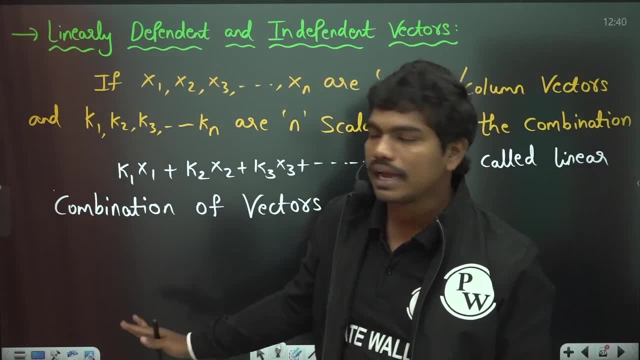 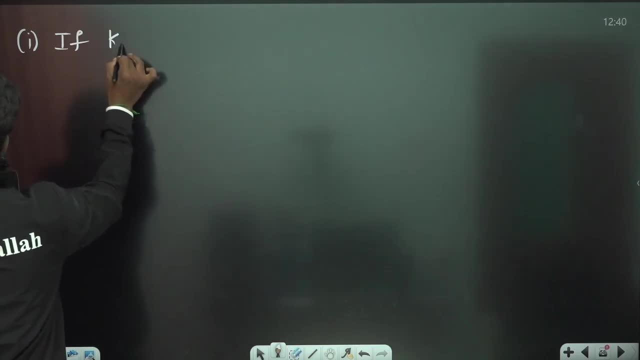 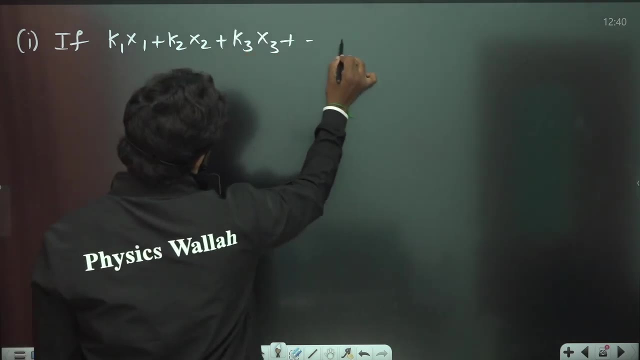 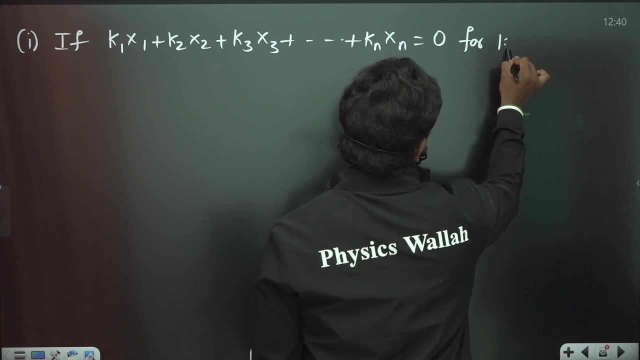 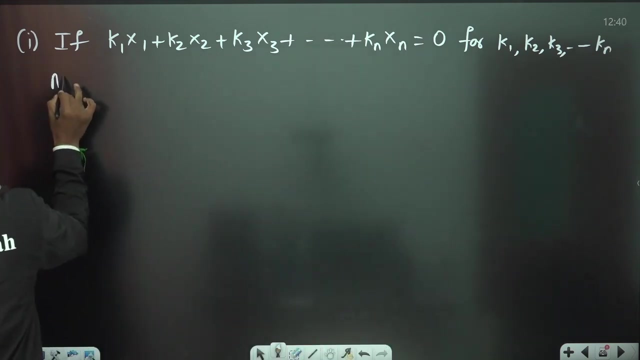 dependent or independent, depending on a particular equation. i will show you now. okay, if, if k1 x1 plus k2, x3 plus k3, x3 and so on, kn xn is equal to zero for k1, k2, k3 and so on, kn not all zeros simultaneously. 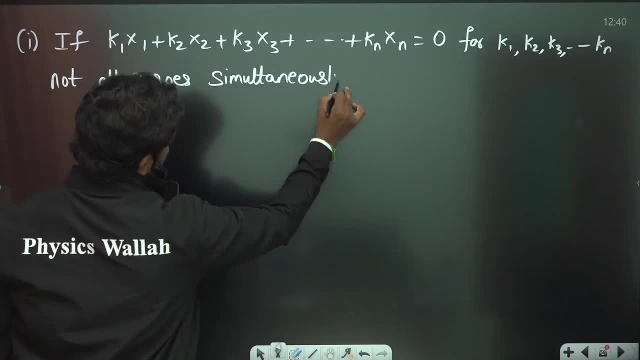 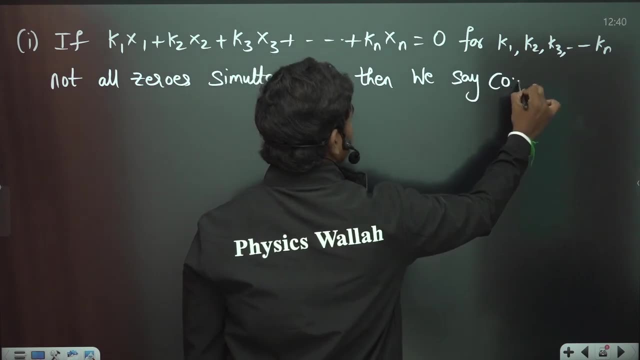 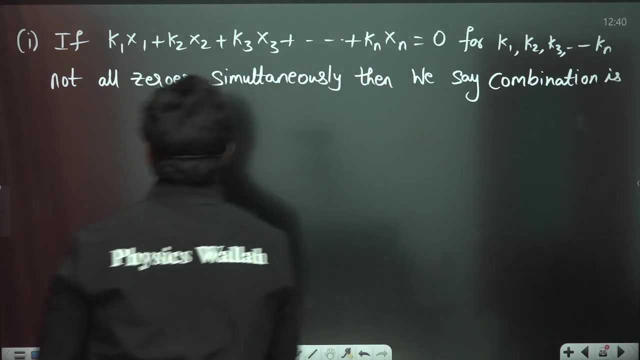 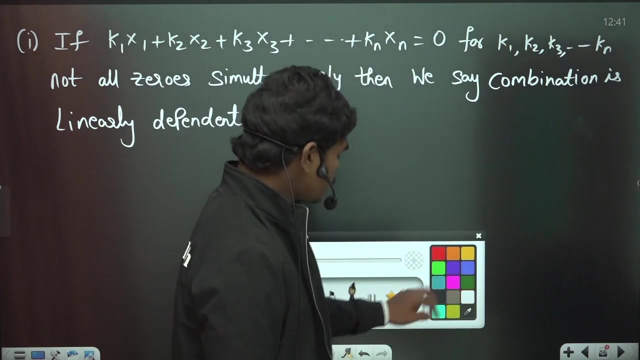 not all zeros simultaneously. than we say combination is linearly dependent, we say combination, combination is. combination is linearly dependent. combination is linearly dependent. look, let me explain you with the help of example. you will understand. for example. okay, so now let us suppose i have taken k1 plus k2, x3 and so on. k2- x2 is equal to zero. 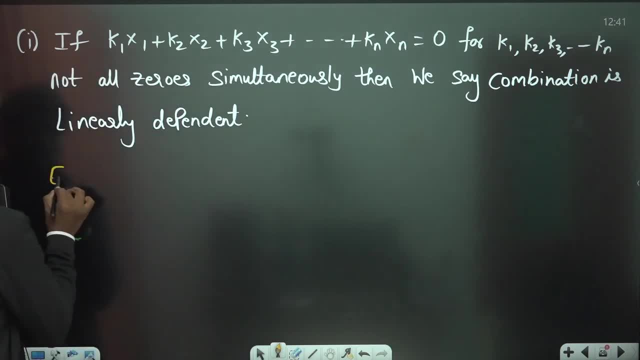 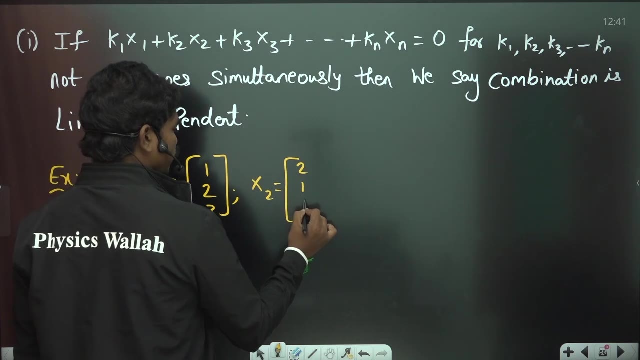 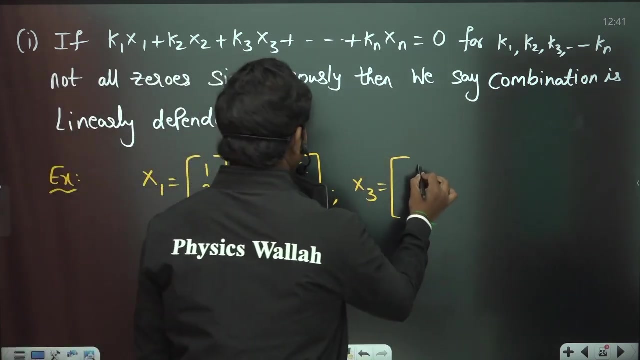 taken three vectors example. let us suppose I can take three vectors. x1 is equal to say 1, 2, 3, for example. x2 is equal to some something: 2, 1, 4, something like this, anything x3, for example. let us take x3 is 1 minus 1, 1, for example, something like this. okay, now try to. 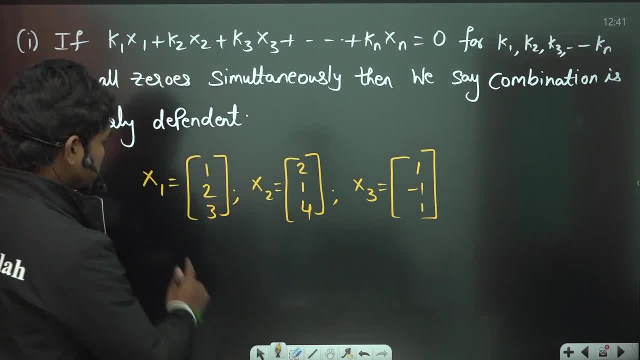 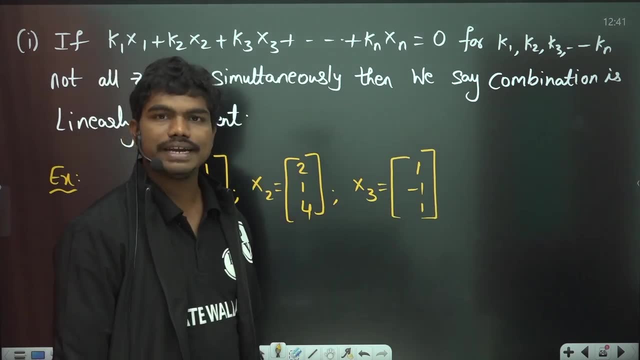 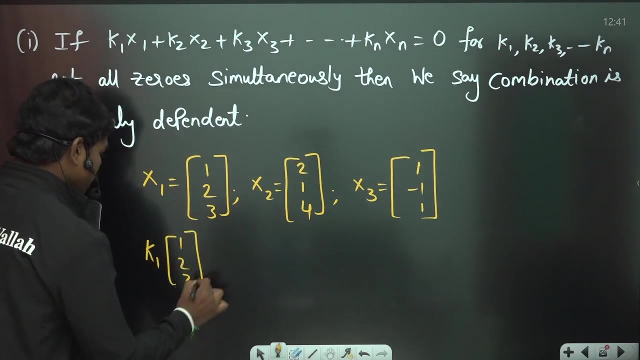 understand one thing. let us suppose, if we hear the linear combination some constant into this plus some constant to this plus some constant into this, then k1, x1 plus k2, x2 plus k3, x3 will become linear combination. now let us suppose k1 into x1 plus k2 into. 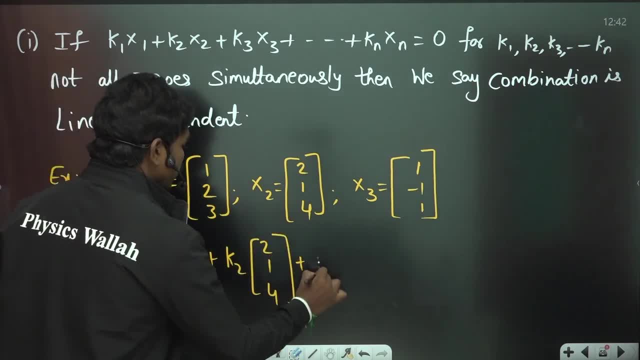 x2 less k3 into this is equal to 0.. Let us suppose ofcing for saying one right now like this: Let us suppose a time limit, x0 is equal to a total of 0. so let us suppose if I write this, y19, then k1 is equal to 0. cause a time limit, x2 is equal to zero. so 1 plus 12 surprised. 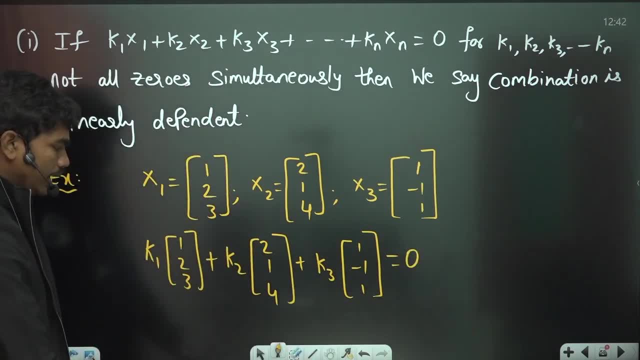 writing this equation. so these are some constants which are to be multiplied, and these are three, by one matrices. now, when all these are not zeros, when all these things are not zeros, if this equation is getting satisfied, then we say that the that these vectors are depending on each other. 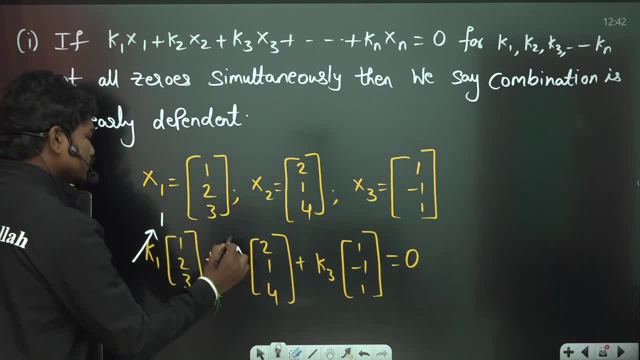 how come look, let us suppose if i keep one, if i keep this value minus one, and if i keep this value minus one, okay, for example, if i keep this value or plus one, let us suppose i am keeping plus one, plus one, then when k1, k2, k3- these are all not zeros, but still this equation is holding good. 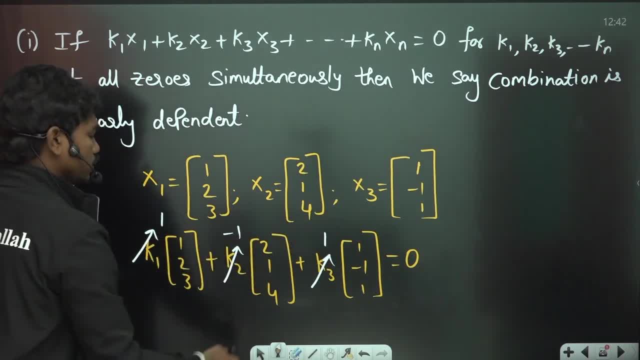 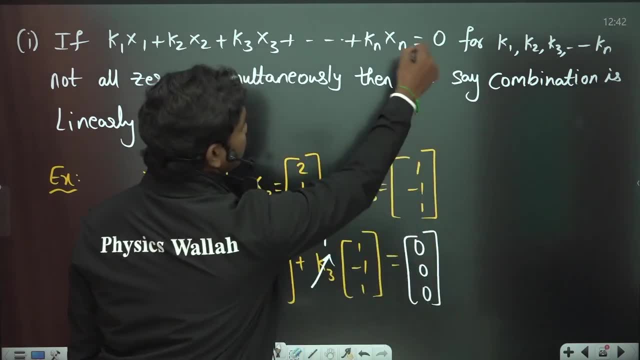 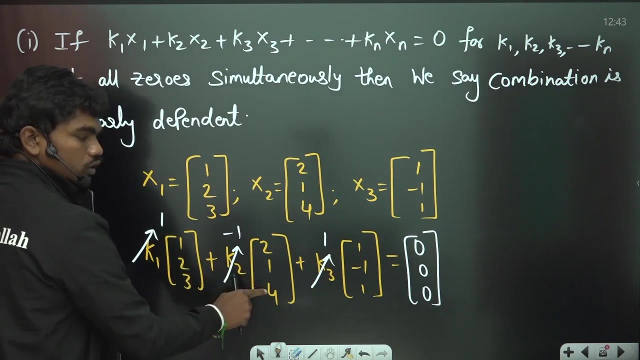 yes or no. one minus two minus one minus one plus one, zero means basically here: i mean, this is the matrix, actually the null matrix: zero, zero, zero. okay, i have written capital o. that's why, if you see so, this is zeros. similarly, if you take two minus one, one minus one zero, three minus four, 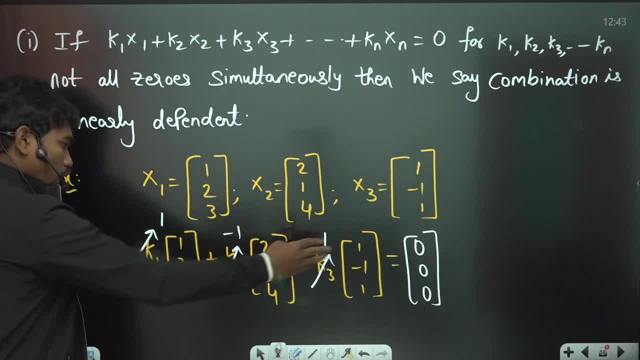 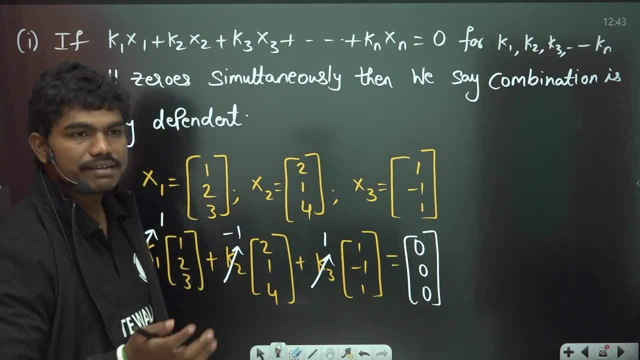 minus one plus one zero. so here, if you see, this combination is getting satisfied. but if you take two minus one, one minus one zero, you can see that the matrix is still holding good when k1, k2, k3 are non-zeros, actually clear. so such combinations are called linearly dependent. 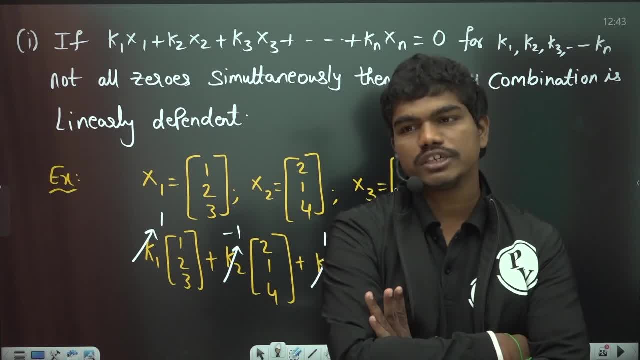 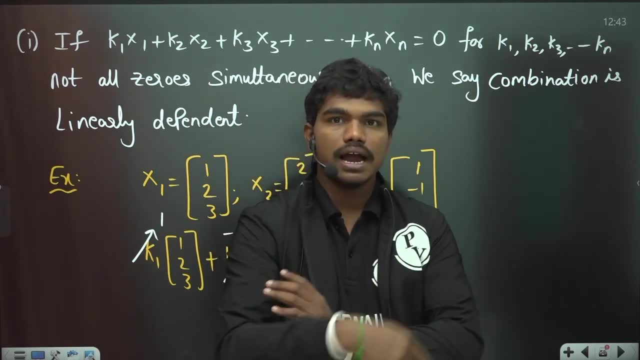 you know this word dependent very often. let us suppose, if i give you some equation, y is equal to some function in terms of x, then you say that y is depending on x, correct? so that's basically dependency, and here the vectors are linearly multiplied. so that's why this combination is. 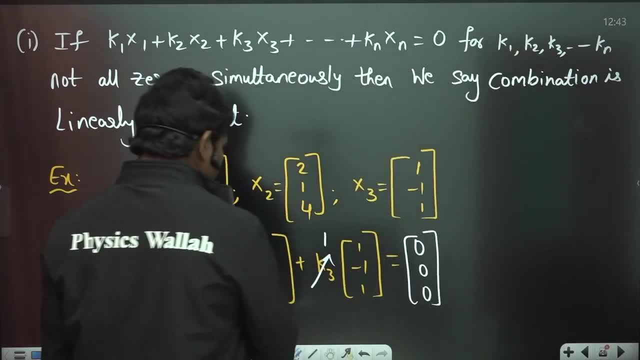 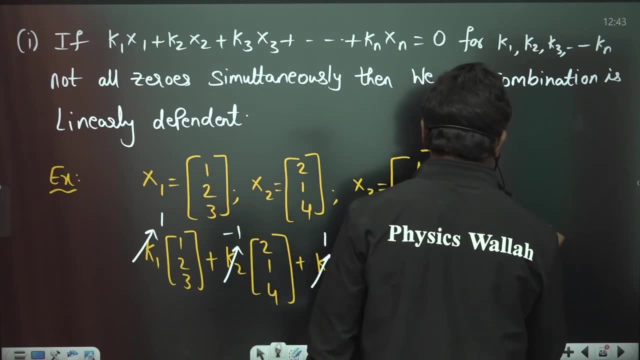 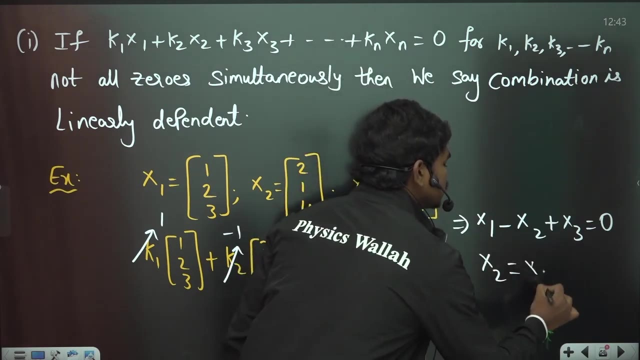 called linear combination and here, if you see, i can write this equation as: look, can i write this equation as: 1 into x1, x1 minus 1 into x2 minus x2 plus x3 is equal to 0. so which means, for example, if i write expression for x2, i can write this as x2 is equal to x1 plus x3. similarly, if i want to, 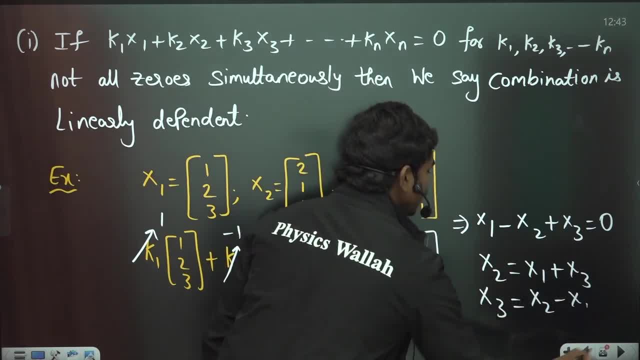 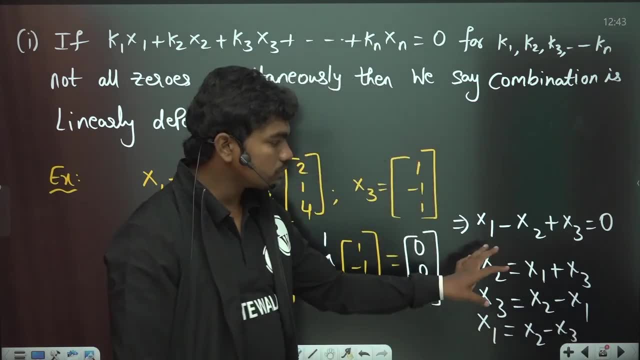 write x3, i will write this as x2 minus x1. similarly, i can write expression for x1 also, as you know, x2 minus x3, like this. so here, if you see you can write these vectors as depending on some other vectors. okay, this can happen only. 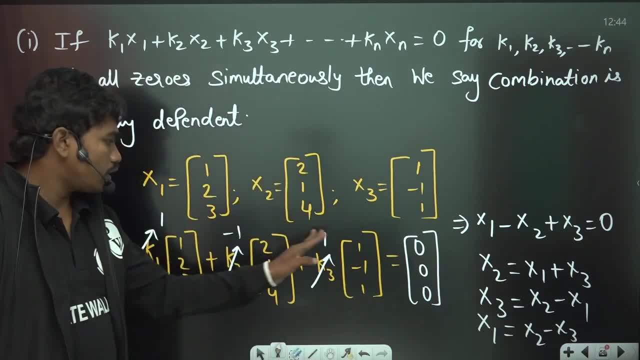 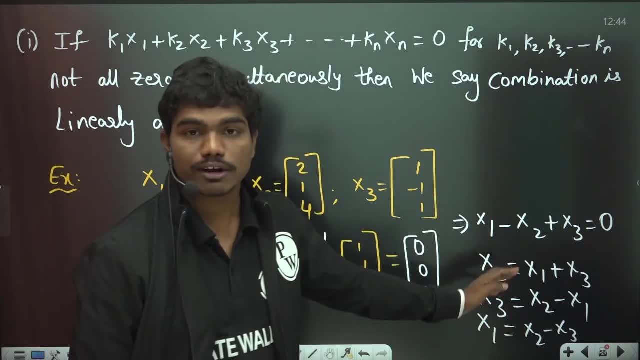 if these constants are non-zeros. look, let us suppose if all these constants are zeros- k1, k2, k3, all are zeros- then definitely this equation will get satisfied. but you cannot write any relation like this. you cannot show any dependency of vectors on the other vectors. so that's why 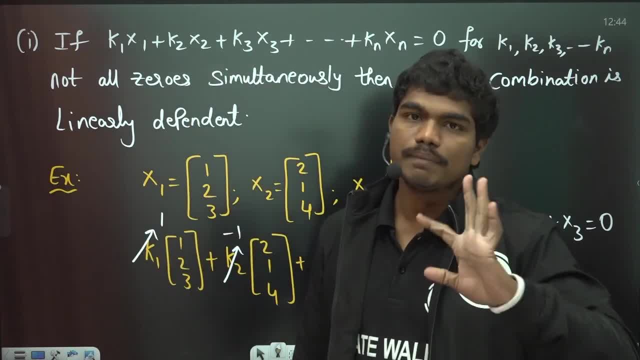 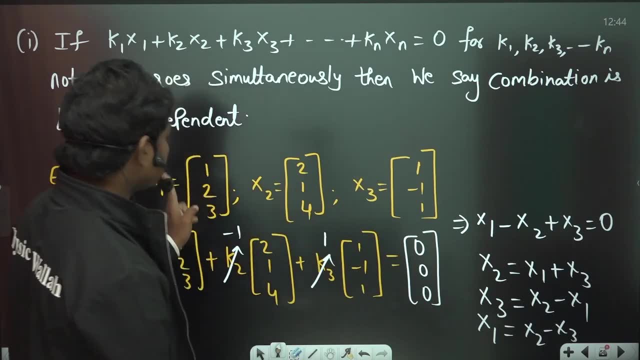 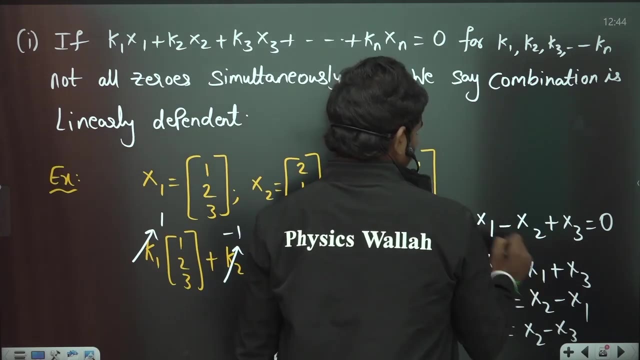 this combination is called linear combination with linear dependent vectors. now i'll ask you one thing you can understand easily. look, when i write these vectors, if i take these vectors x1, x2, x3, determinant, let us suppose, if i take the determinant x1, x2, x3 means basically my 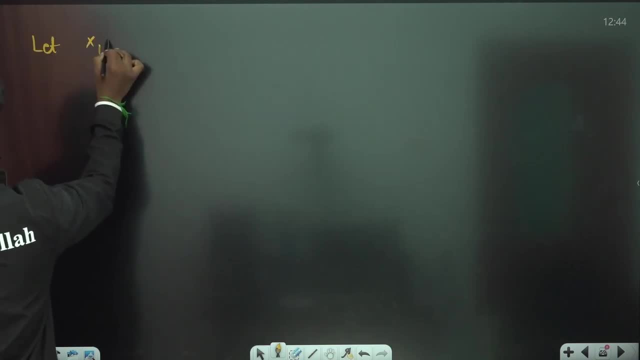 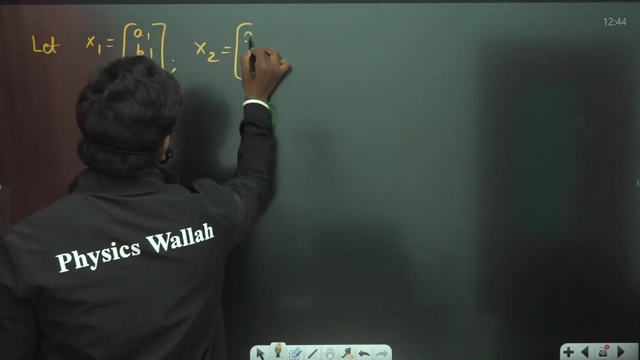 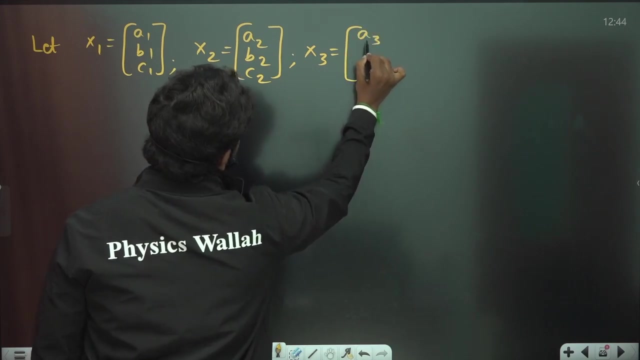 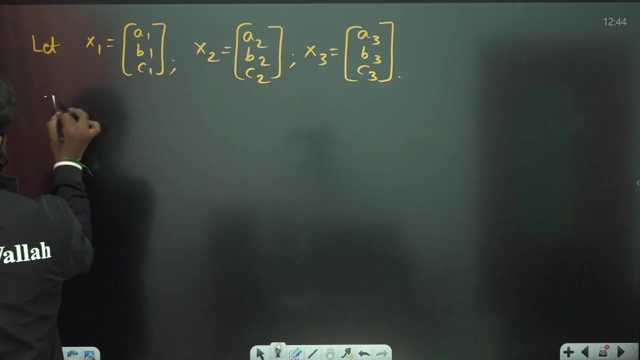 intention is to tell you that let x1 is equal to a1, b1, c1, x2 is equal to a2, b2, c2, x3 is equal to a3, b3 and c3. let us suppose these are the vectors not dependent. if x1, x2, x3 are dependent, are linearly dependent, you can say are linearly. 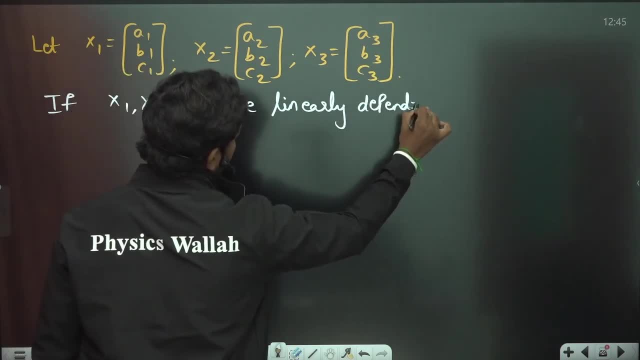 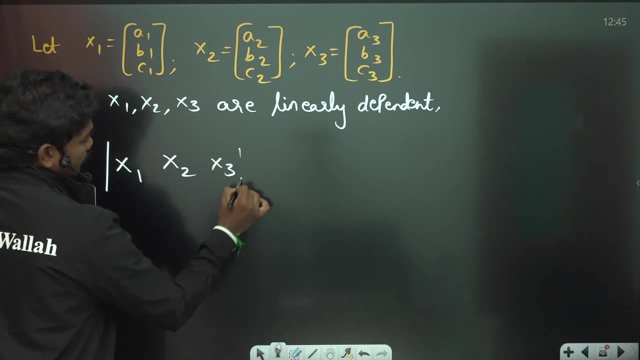 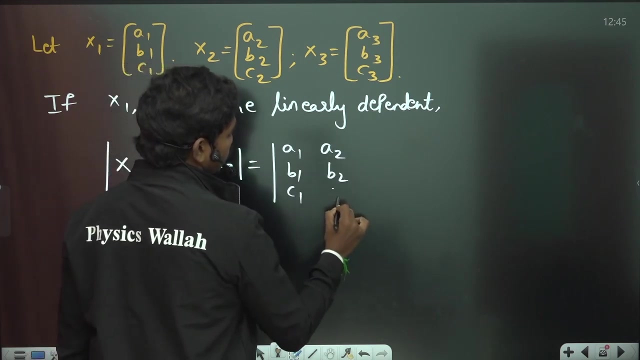 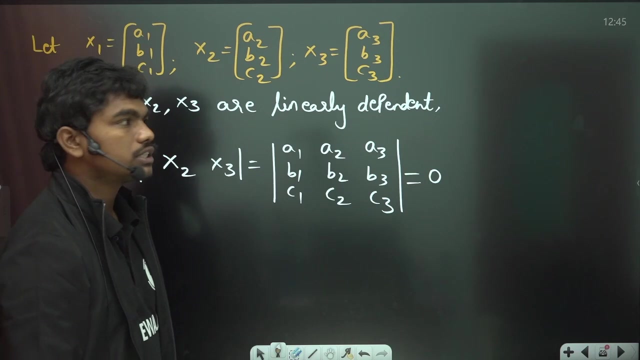 dependent, dependent. now tell me one thing. first determinant of this: x1, x2, x3 means basically: x1 is one column vector: a1, b1, c1. this is another column vector: a2, b2, c2. this is a3, b3 and c3. this determinant should be definitely equal to zero. why it should be equal to zero? 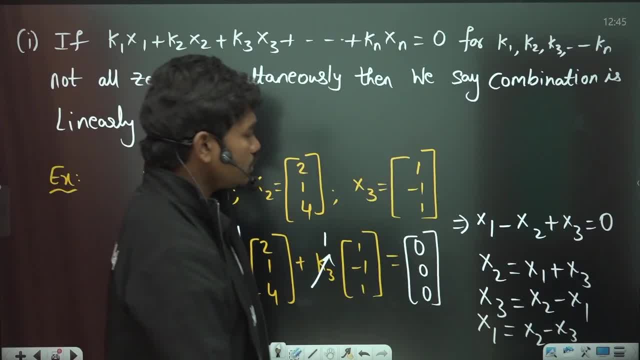 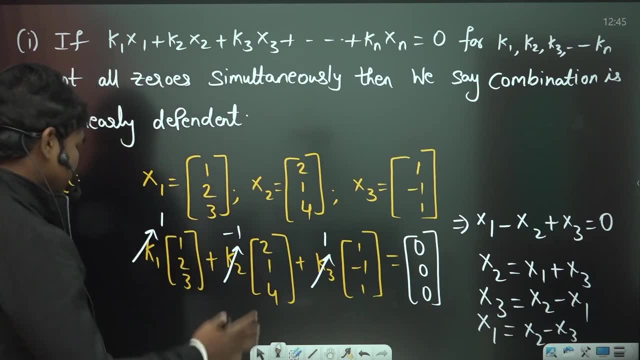 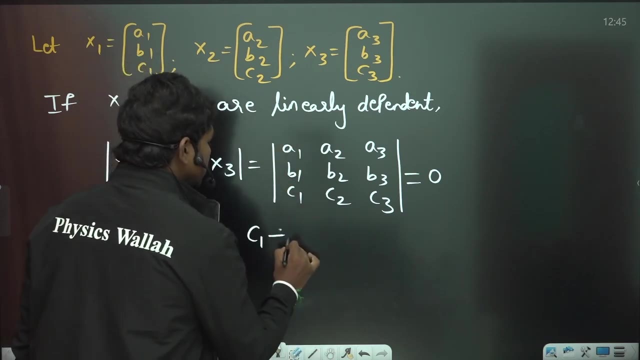 because you know that this x2 is nothing but some combination of x1 and x3. similarly, if you see, if, for example, if i write this transformation, column 1 changes to column 1 minus column 2 plus column 3, for example, if i write this combination: c1 changes to c1 minus c2 plus c3, then what you 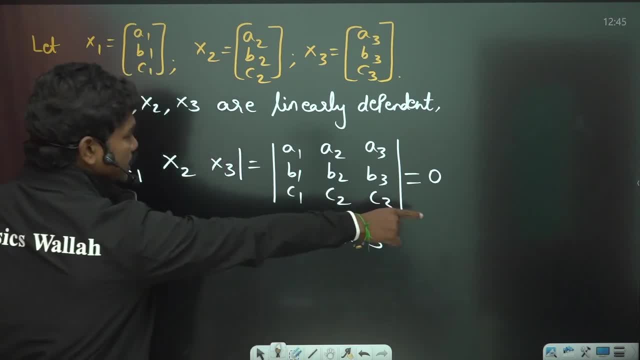 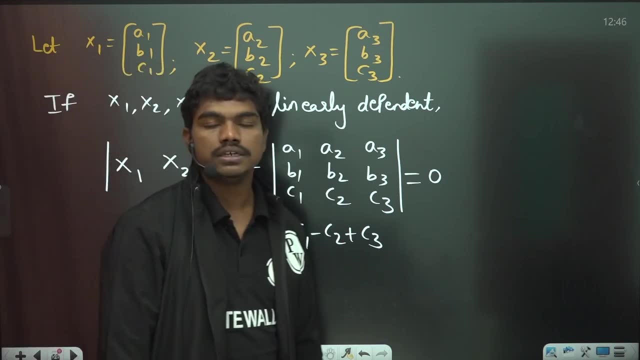 will get here x1 minus x2 plus x3, which is actually zero in this case. okay, so the first column, if you apply this transformation to this determinant, the first column will be zero. so definitely, this determinant is zero. so, whenever these vectors- i have taken the three by three. 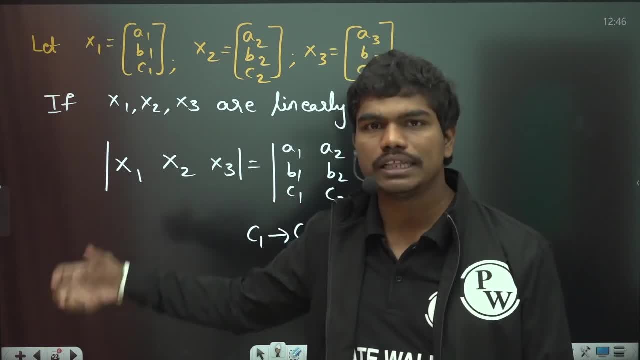 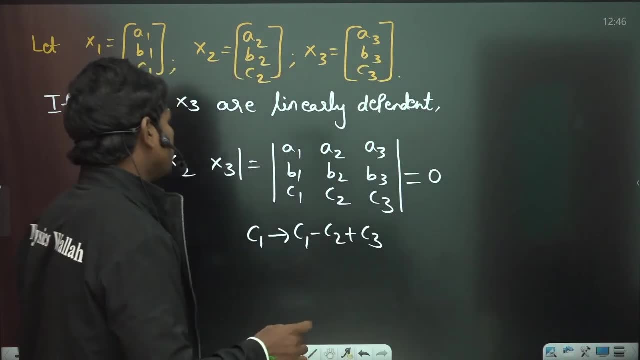 case, simply. similarly, same thing holds good for four by four, five by five, all these things actually okay. so if you see carefully, if certain vectors are linearly dependent, then you have to do make sure that this determinant is always zero. and why this determinant is zero? because you can see this: 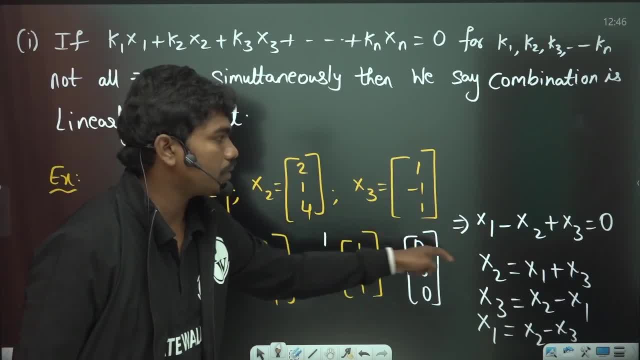 vector is always zero and this determinant is always zero. because, you can see, this vector is always zero and whenever things are depending linearly, we get such equations and if you apply the corresponding transformation, means if you apply this, c1 changes to c1 minus c2 plus c3. 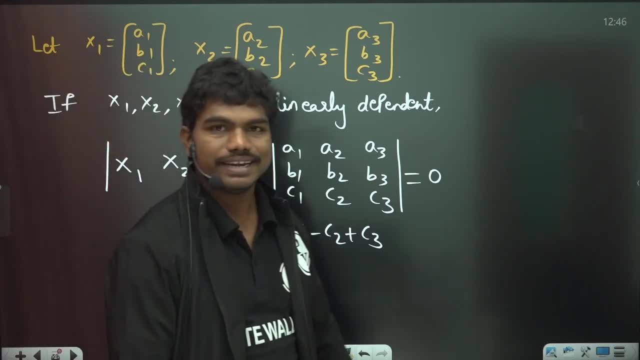 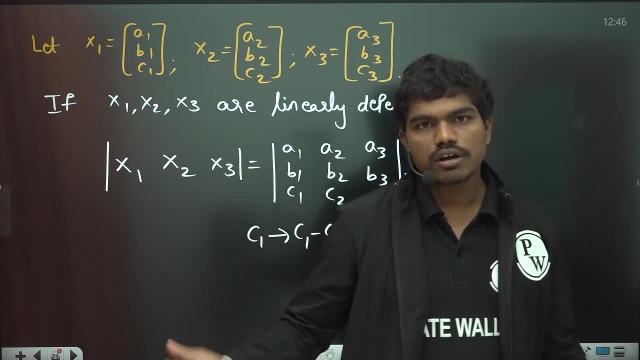 this first column gets out to be zero. so that's called linear combination of vectors and this case is said to be linearly dependent. okay, and obviously, if we cannot write any such dependency, we'll call the case as linearly independent. okay, so linearly independent if you write. 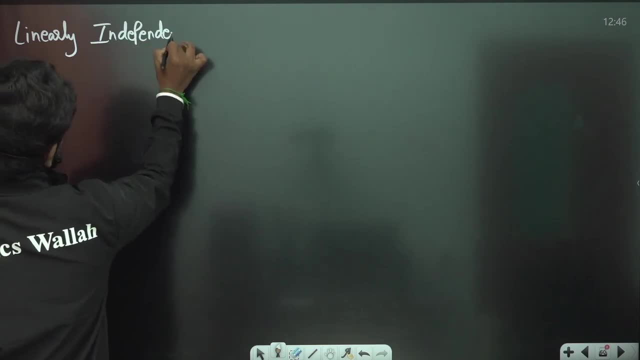 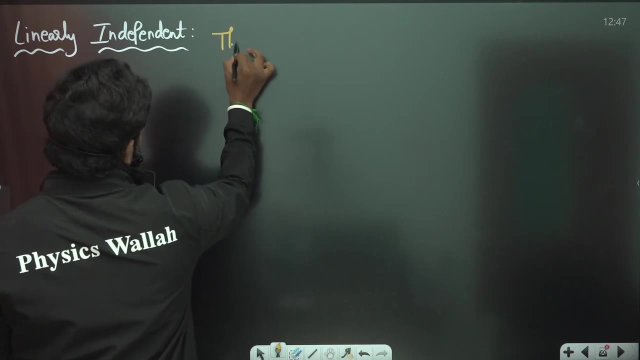 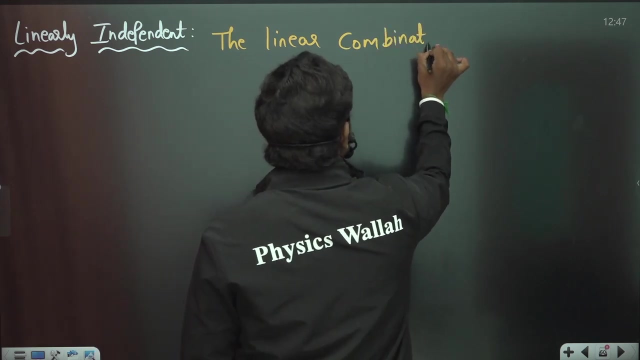 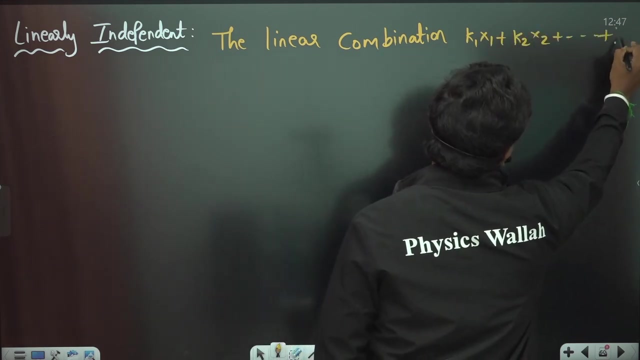 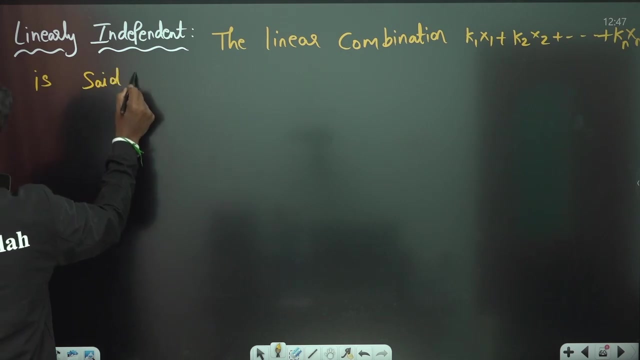 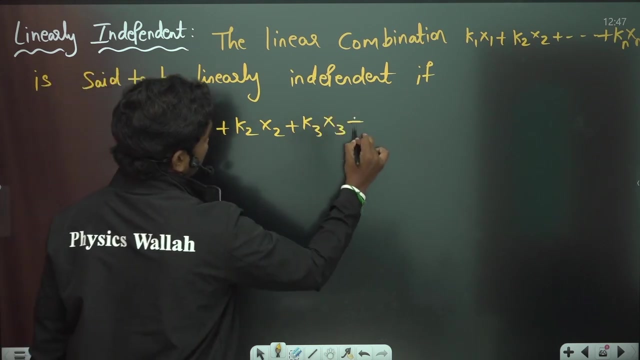 this a combination, the linear combination, the linear combination- k1 x1 plus k2, x2, and so on, plus kn xn is said to be, is said to be linearly independent. linearly independent if, if k1 x1 plus k2 x2 plus k3, x3, and so on, plus kn xn is equal to zero. when 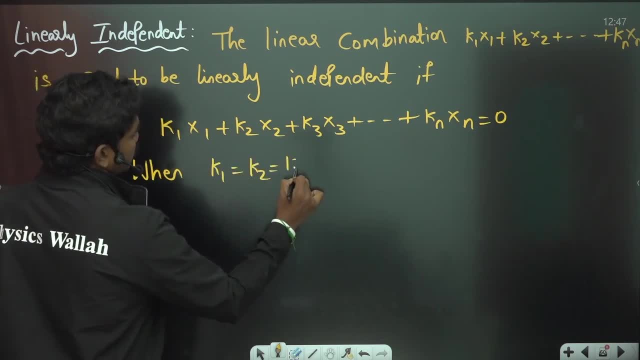 if k1 x1 plus k2 x2 plus k3 x3 and so on, minus kn xn is equal to zero. when so on, plus kn x1 plus k2 x2 plus k3 x3 and so on, plus knxn is equal to zero. so whenever. 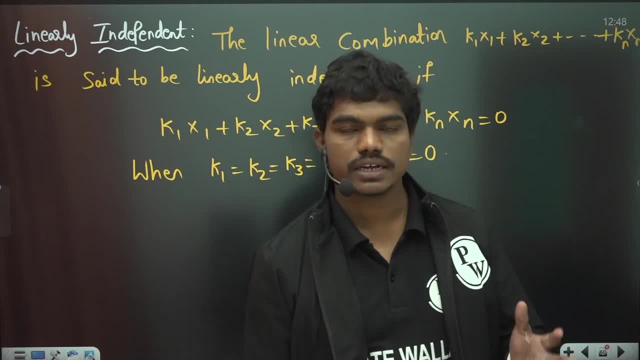 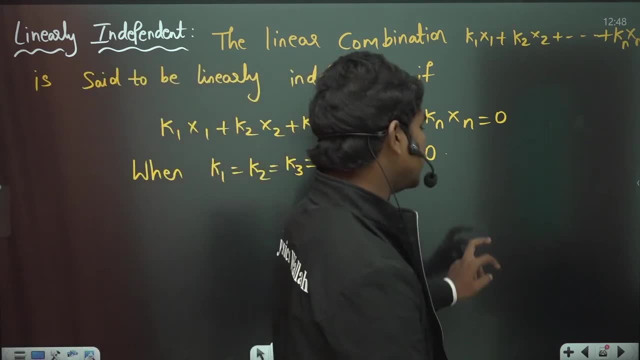 all these constants are zero's. you cannot write any linear dependency of a vector on other vectors. for example, you cannot say that x3 is equal to x1 minus x2, anything like that. okay, and why. i have told this about linear independency. my, i want to give one minute point here. 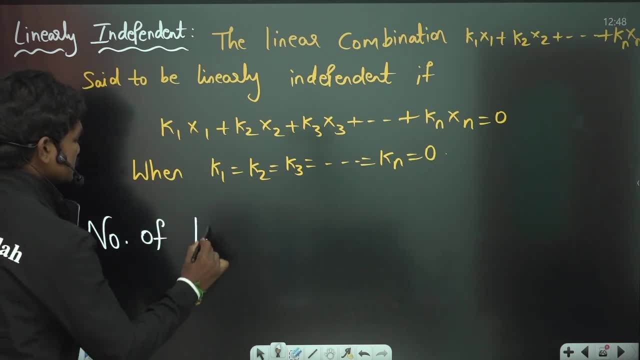 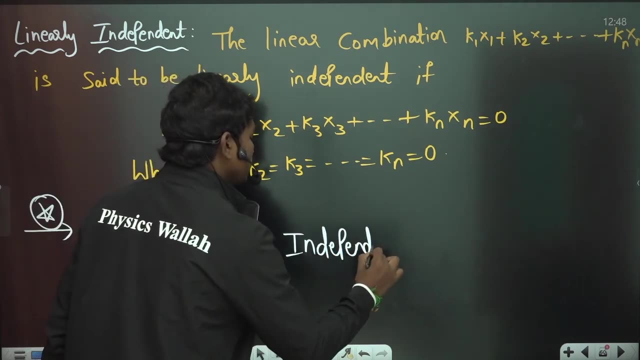 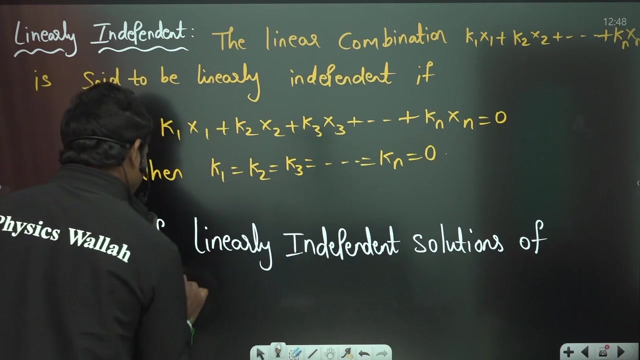 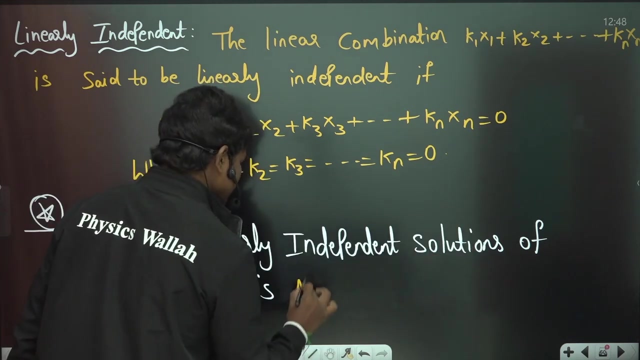 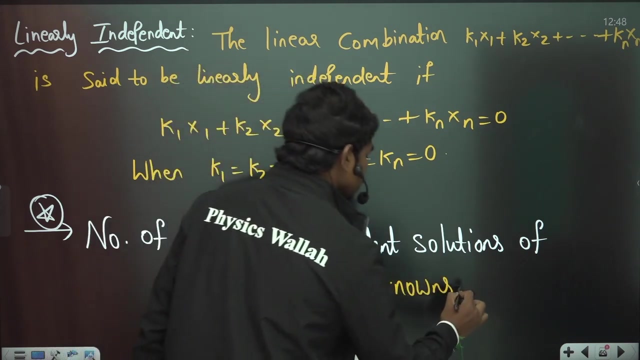 number of linearly independent solutions. number of linearly independent solutions, uni solutions bags. thus things end up getting linearly independent solutions. number of linearly independent solutions of AX is equal to B is number of unknowns minus number of unknowns. unknowns minus rank of A. basically here, okay. so this point is very important. 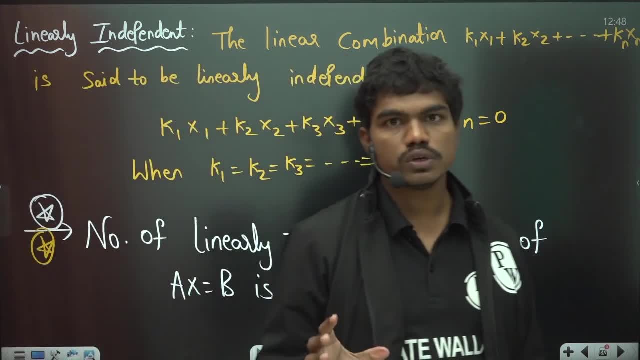 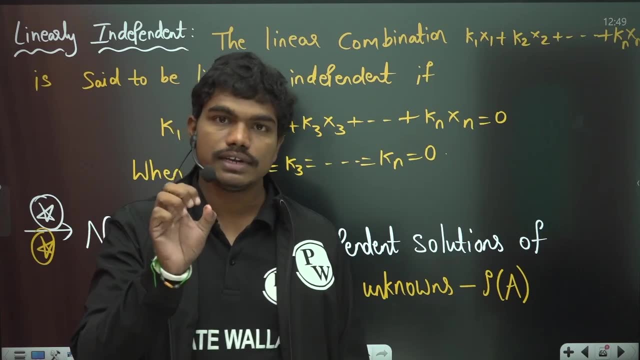 basically what happens when you get infinitely many solutions, then few solutions will be linearly depending on each other and a few will not be depending on each other. okay, so if you want to find out what are the number of linearly independent solutions, you have a simple formula for that number of. 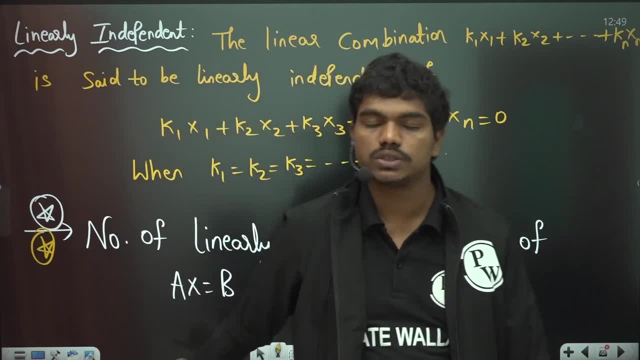 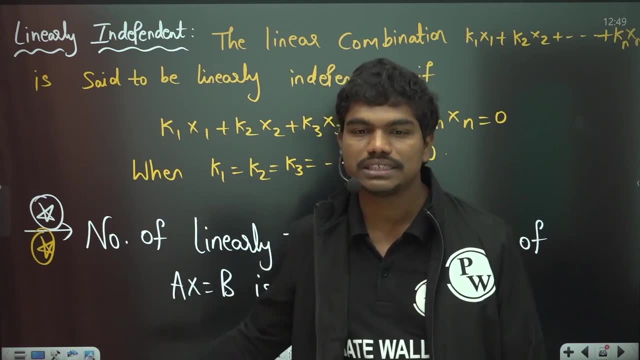 unknowns, minus a rank of A. I just want to give you this formulation. so it's necessary for me to make you understand what is linearly dependent and what is linearly independent. so I have talked about this linear dependency and independency a bit, for example. okay, so now we'll go for this last module of. 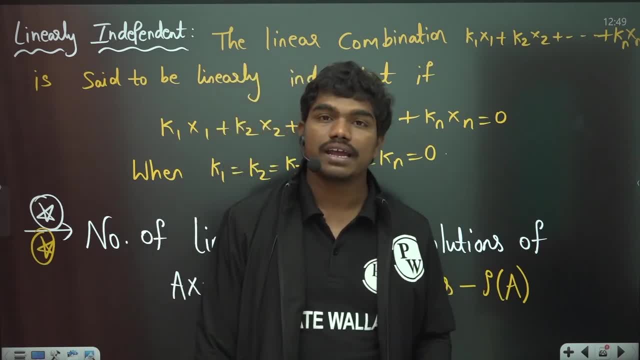 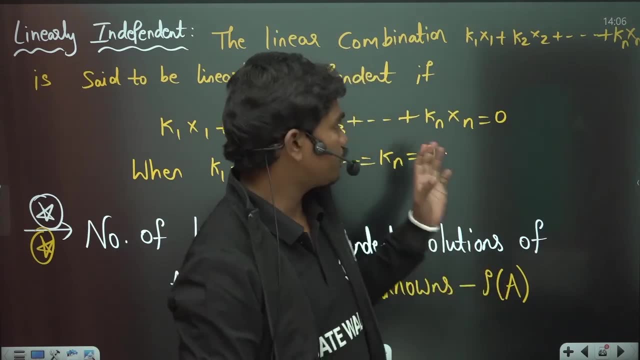 this or the last part of this video, which is eigenvalues and eigenvectors, which is again one way most questions asked region in linear algebra. okay, so we have discussed about this linear dependent and linear independent combinations of vectors. now let us go to one next and the last, most important. 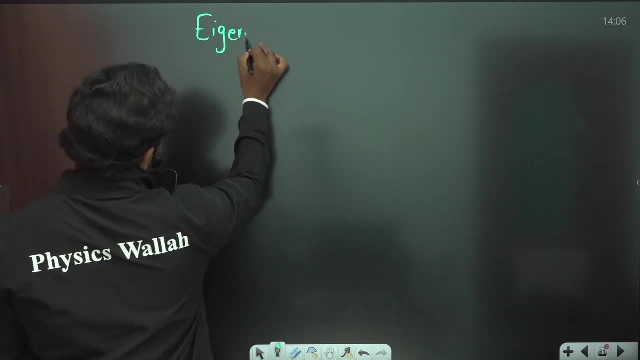 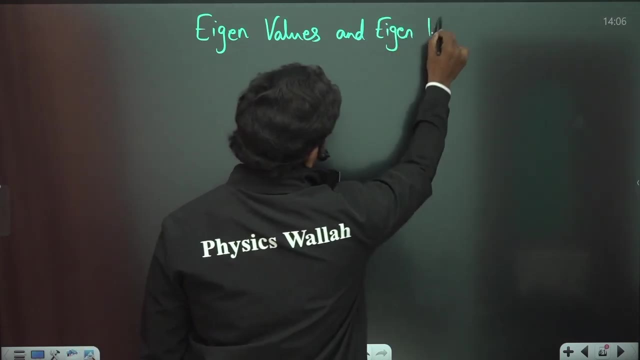 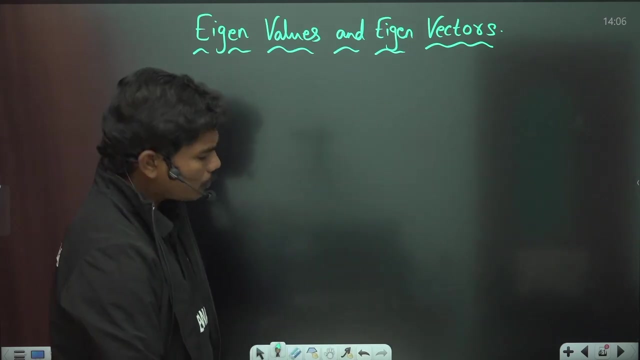 part which is eigenvalues and eigenvectors. eigenvalues and eigen vectors. eigenvalues and eigenvectors. so let us see what are this eigenvalues and eigenvectors? these are practically very important vectors actually. now, what are these betters actually? look, let us try to understand. so normally see the 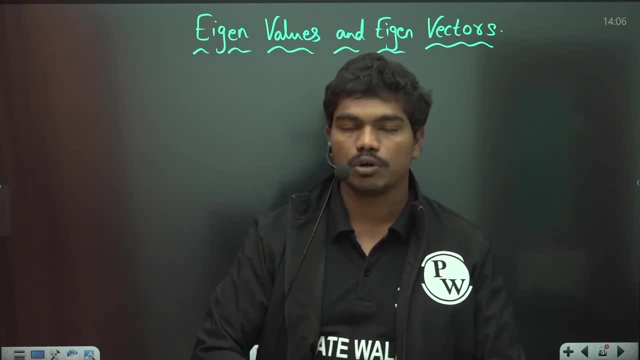 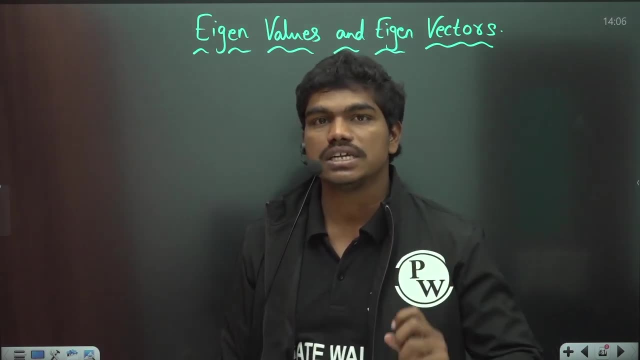 definition, that of a minus lambda, is equal to all these things. that's characteristic polynomial. but why this, Alberto? A minus lambda? I should be all to see how. this is what that Knight� separate시간. So this is what you need to understand. means how the characteristic equation is coming. 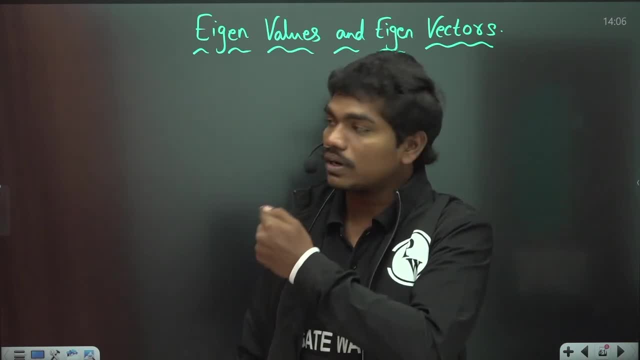 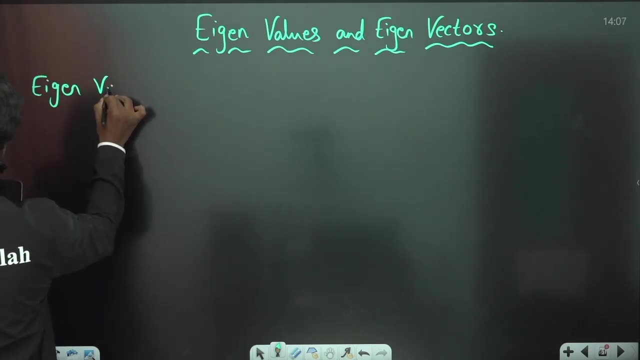 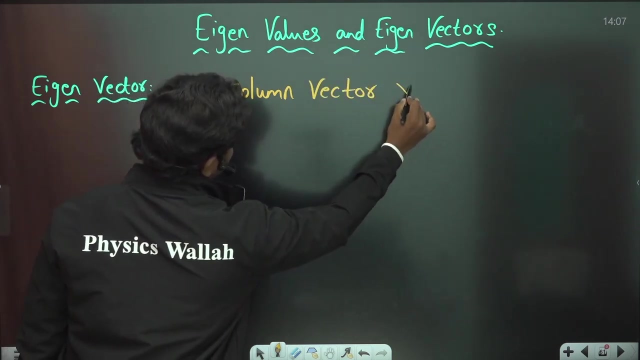 out. Okay, so for writing that you should first of all know what. what is the definition of an eigenvector? Okay, so let us write eigenvector, eigenvector. So the definition of this eigenvector is basically any column vector, any column vector x, basically. 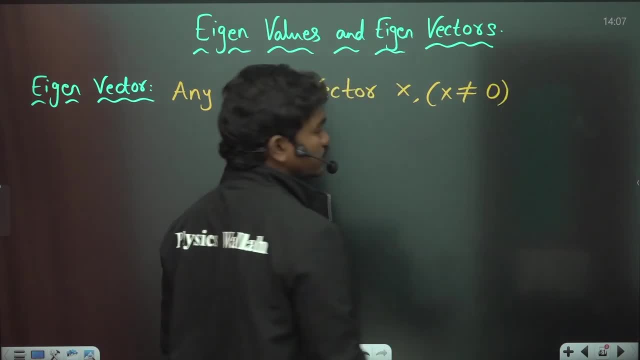 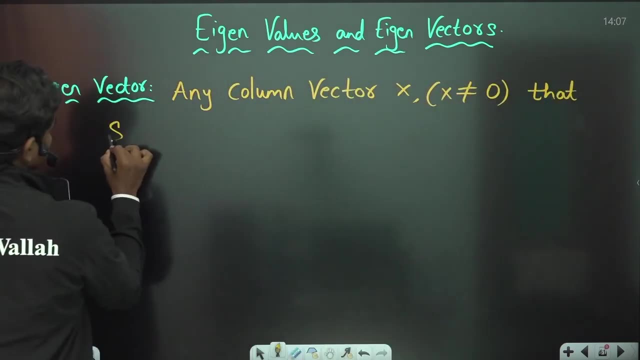 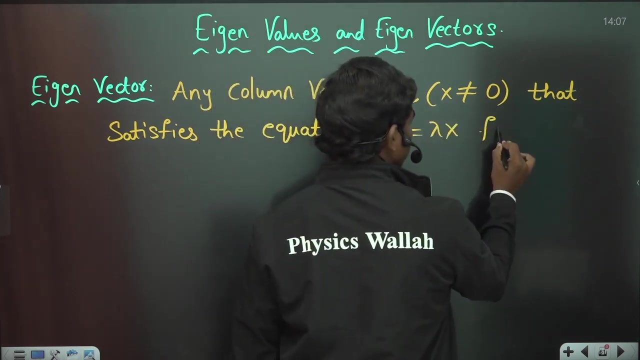 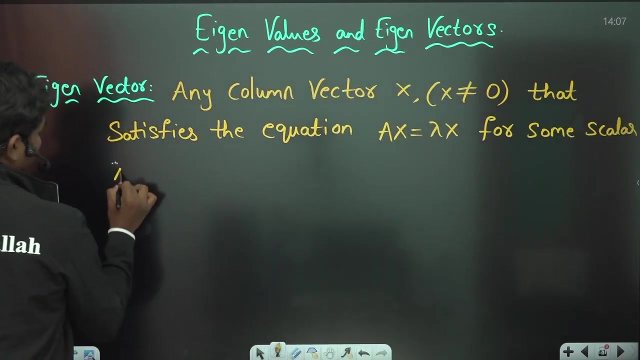 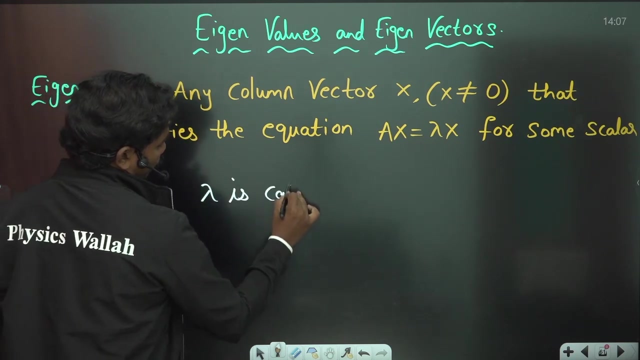 this x is not equal to 0 means basically it is not a 0 column vector. So any column vector that satisfies the equation, that satisfies the equation that satisfies the equation Ax, is equal to lambda x for some scalar lambda, for some scalar lambda, And basically this lambda is called eigen value. of this x lambda is called eigen value. 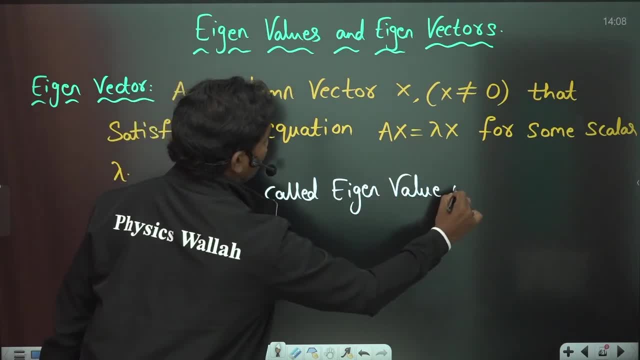 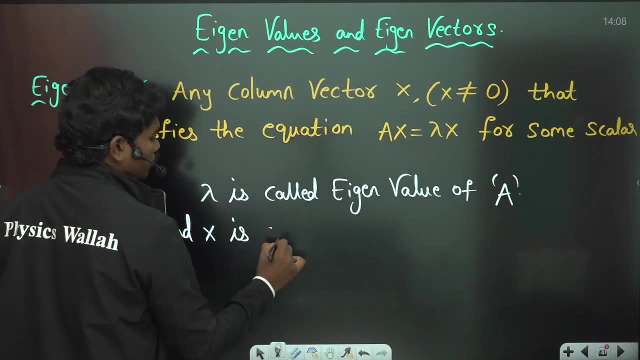 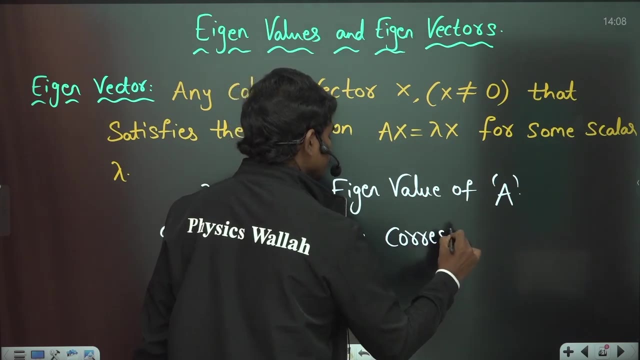 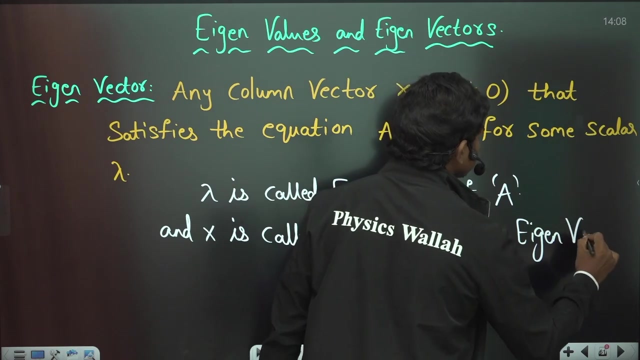 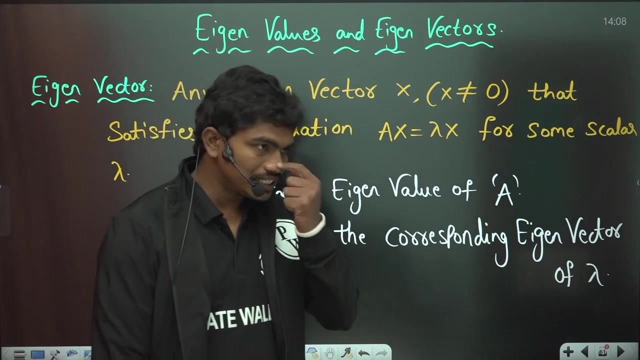 of a eigen value of a and x is called. x is called the corresponding eigenvector, the corresponding, the corresponding eigenvector of lambda. eigenvector of lambda. okay, so this is eigenvector of lambda. Now, basically, if you see, this matrix x is basically one matrix, it is a column matrix. 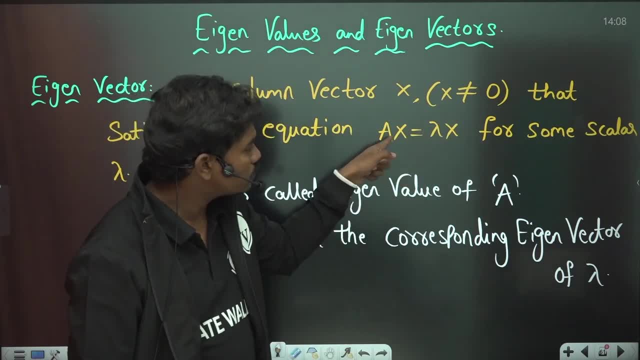 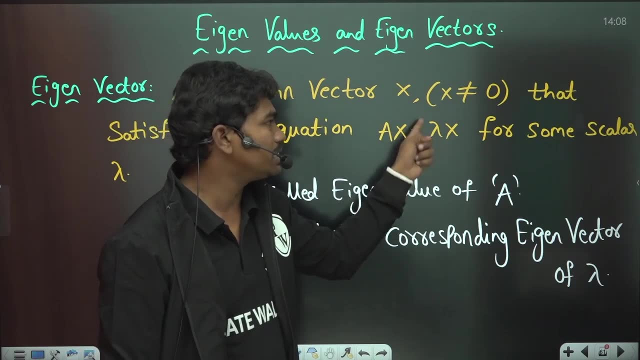 Now what is happening? if you take any matrix and if you transpose on, this means, if you are multiplying these two matrices, If you are applying this, a transformation on this x, you see the outcome is again x, correct. So if you write this in vector form, like this, for example, you will understand it better. 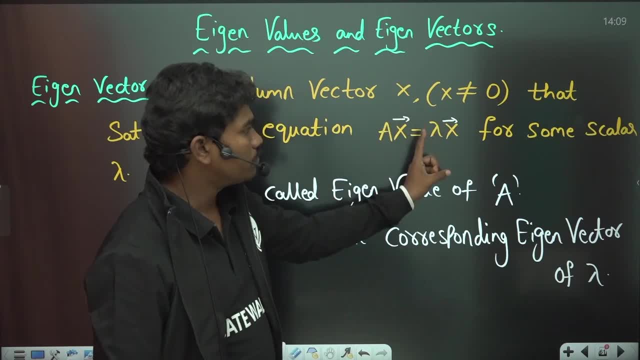 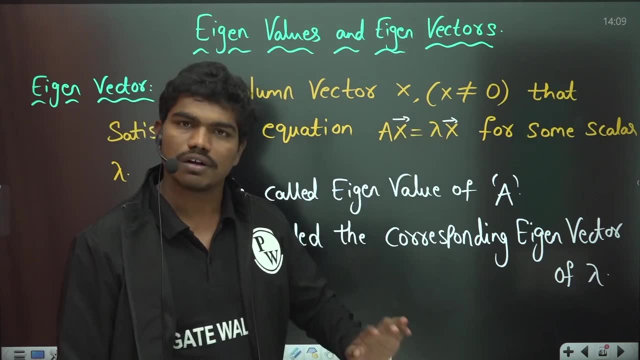 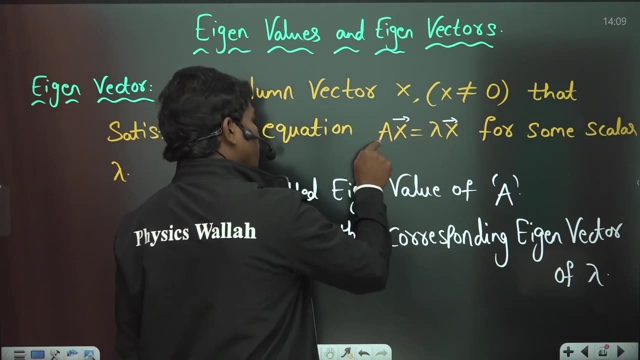 whenever you are applying any transformation on a vector, the outcome is in the same direction, but magnitude is changing because depending on the lambda. lambda is a scalar, So scalar multiplication of a vector will always keep the direction same, correct. So, if you see, these x vectors are such special vectors such that when you apply transformation, 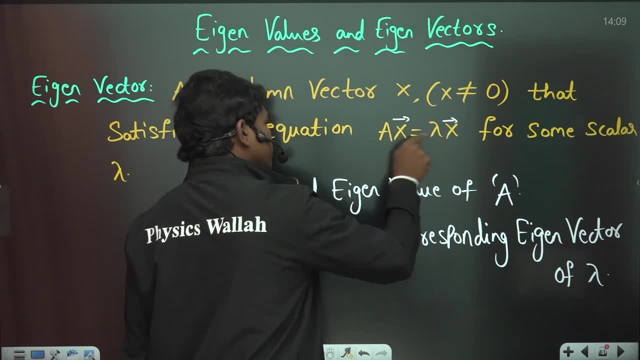 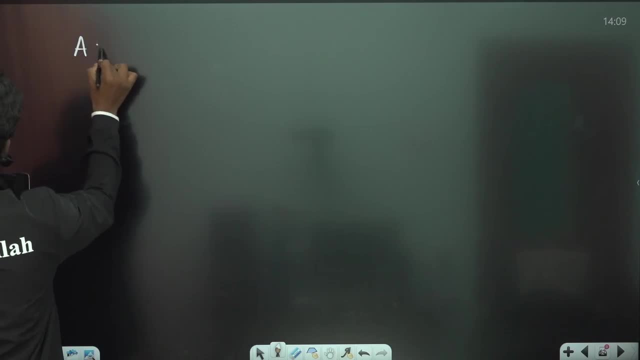 of this a on this vector, Then the direction of the vector remains same, but only the magnitude changes. Now try to understand one thing. we have this equation: a, x is equal to lambda x, correct? So if you simplify this equation, a minus lambda times of i into x is equal to 0 here, correct? 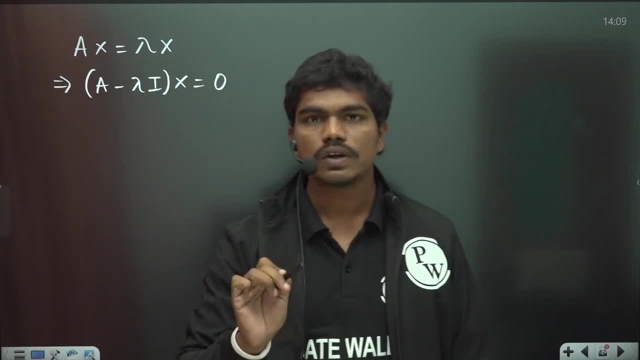 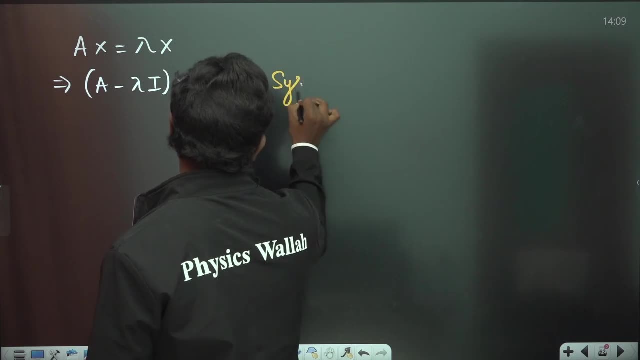 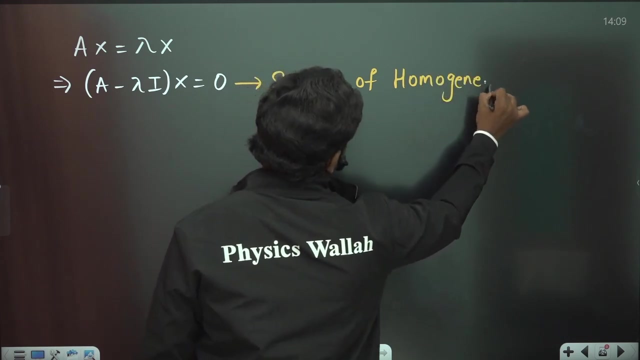 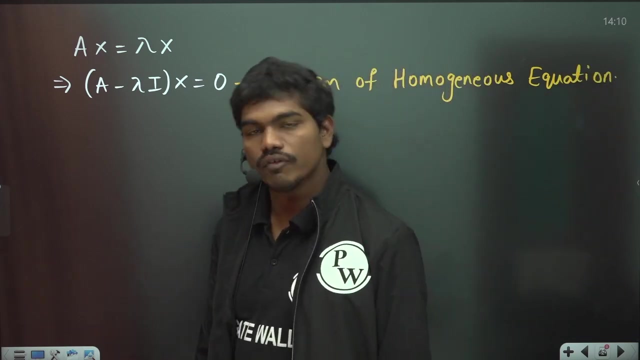 So a minus lambda times of i into x is equal to 0.. Now tell me one thing: this equation, or this, is basically system of homogeneous equations, correct? So this is a System of homogeneous system of homogeneous equation? okay, So this is system of homogeneous equation. now try to understand one thing: if this system 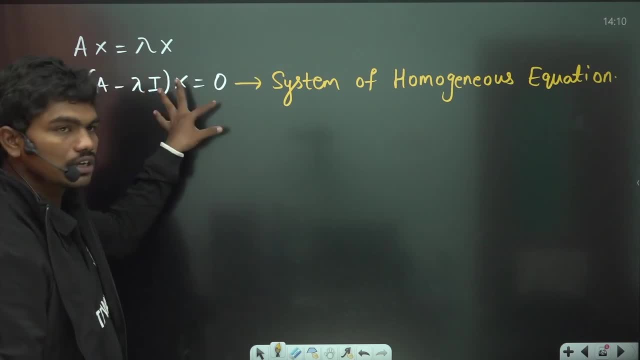 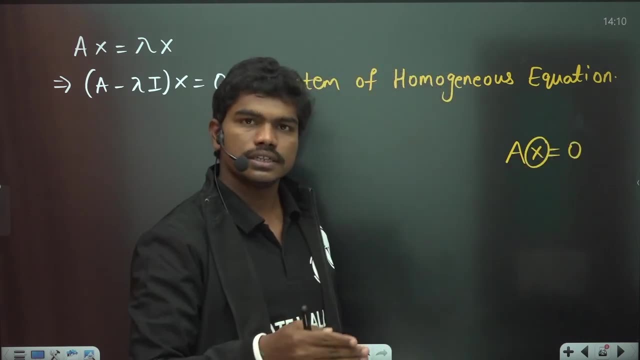 has to have a non-trivial solution. of course, when x is 0, then this equation automatically get satisfied. you have seen in previous case, when a x is equal to 0, whenever this vector is basically 0 vector, Then this equations get satisfied automatically. 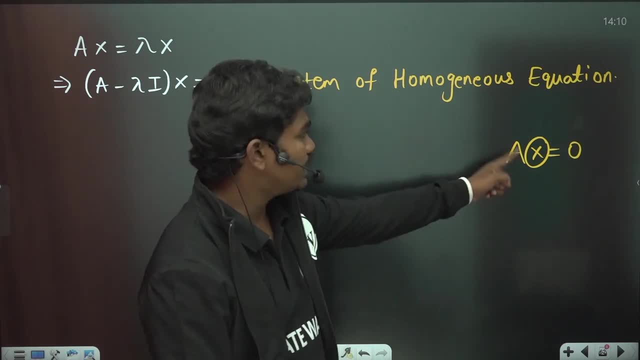 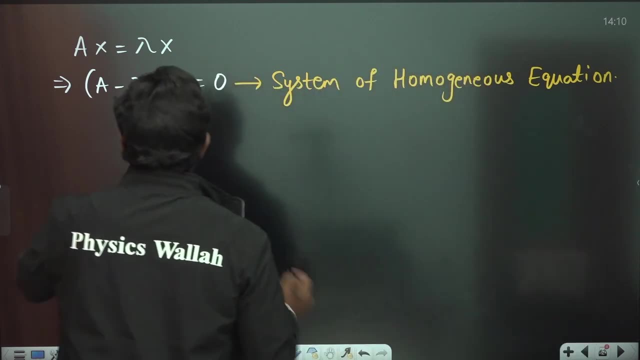 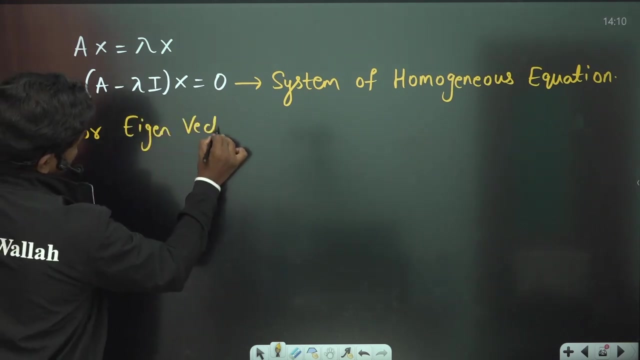 That's called a trivial solution. but we have clearly defined that this x is non-zero. if this x is non-zero, that means what do I mean? if this x is non-zero, this implies for eigenvectors to exist, for eigenvectors to exist, for eigenvectors to exist. this system should have non-trivial 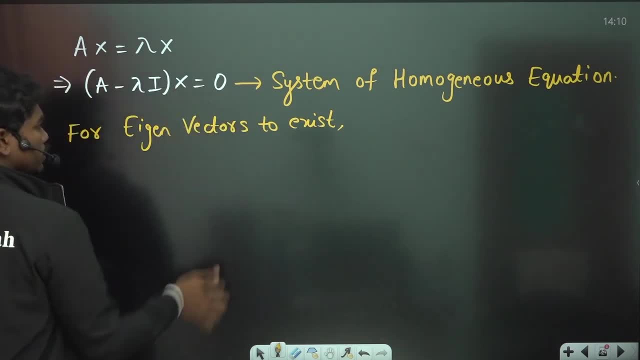 solution, yes or no? And you know, for a homogeneous system, to have a non-trivial solution, Determinant solution, Determinant of the coefficient matrix, which means this here in this case: so that of lambda a, this determinant of this matrix should be definitely equal to 0, and this is how you. 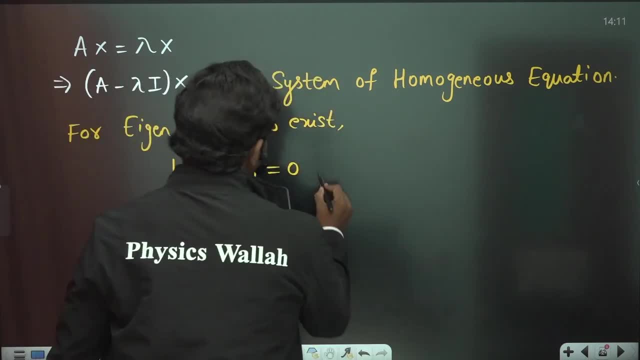 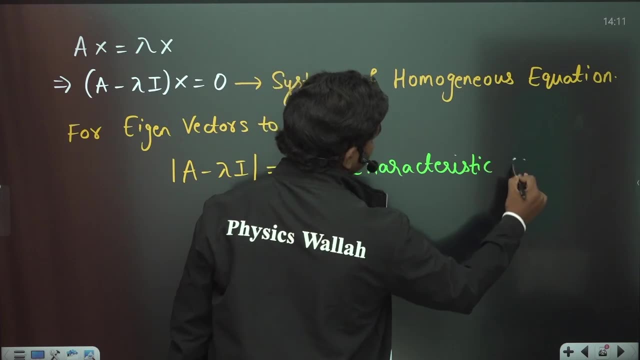 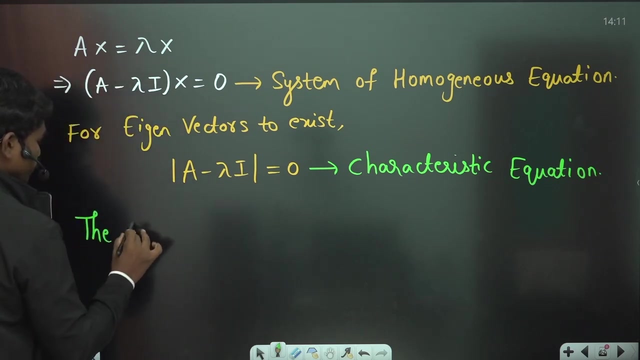 get the characteristic equation and this equation is called basically characteristic equation, characteristic equation, characteristic equation and the roots of the characteristic equation, the roots of The Roots Of the characteristic equation. so basically, if you see, this is a polynomial in terms of lambda, so if you solve you'll get the values of lambda, so the roots of the characteristic. 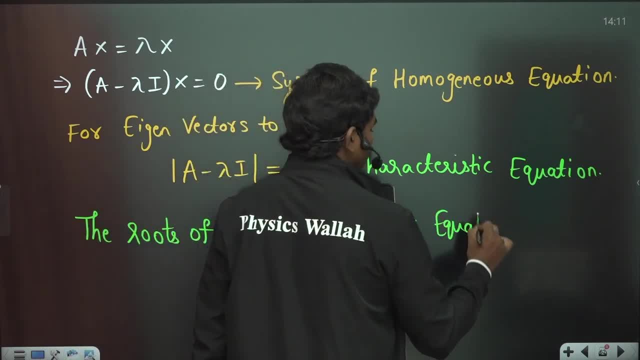 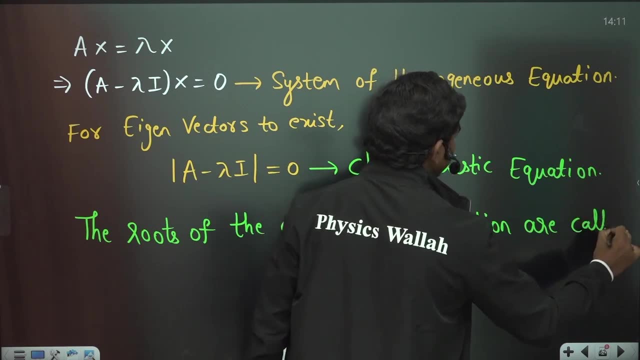 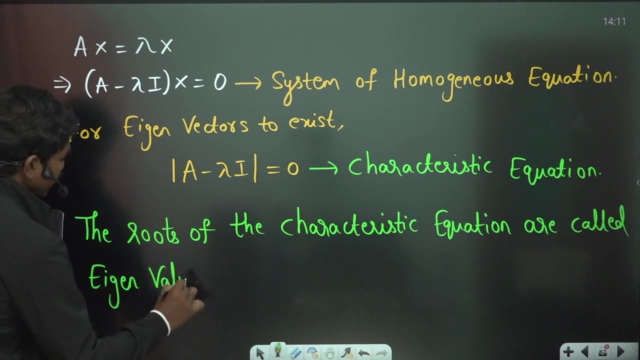 characteristic equation is called roots of the characteristic equation are called eigenvalues are called are called eigenvalues basically. okay, so these are called eigenvalues. so basically, how you will calculate the eigenvalues of any matrix. you know You will equate this determinant to 0. but why that determinant is 0? because this system. 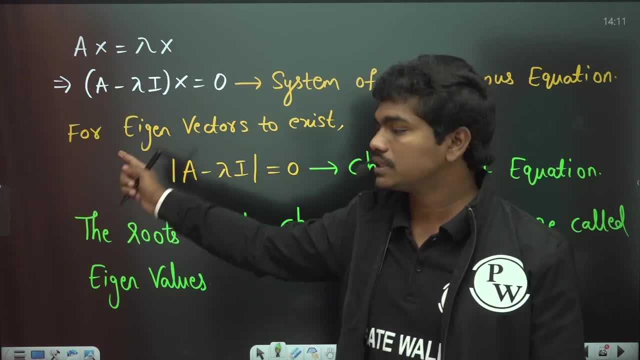 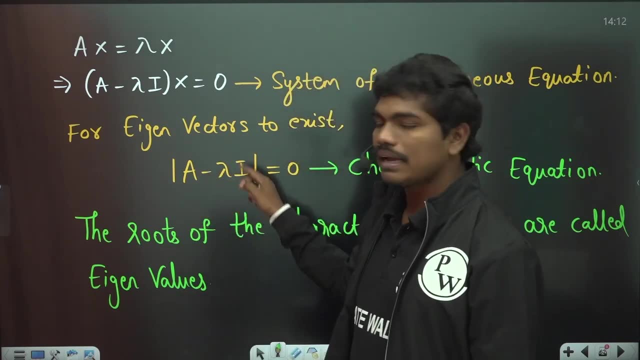 of equations should have a non-trivial solution understood. so that's the reason why this determinant should be equal to 0.. So obviously, once I give you the square matrix, then what you can do, you can write a minus lambda times of i, you can get the determinant, you equate it to 0, then you will get some. 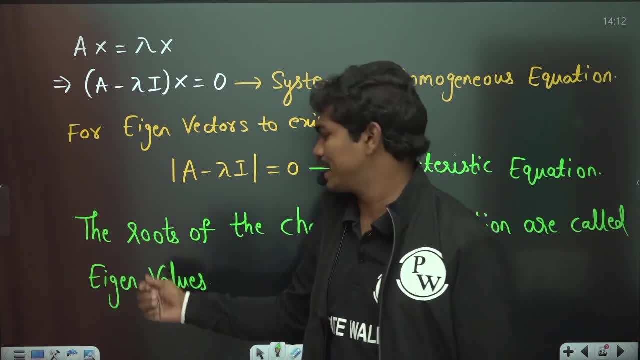 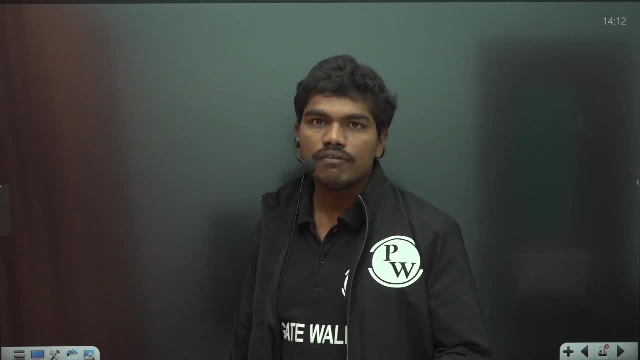 polynomial in terms of lambdas and once you solve that polynomial, you will be getting the values for this. you know eigenvalues, okay, so basically, this is how you calculate the eigenvalues And how, basically, we will discuss some properties, some important properties of eigenvalues here. 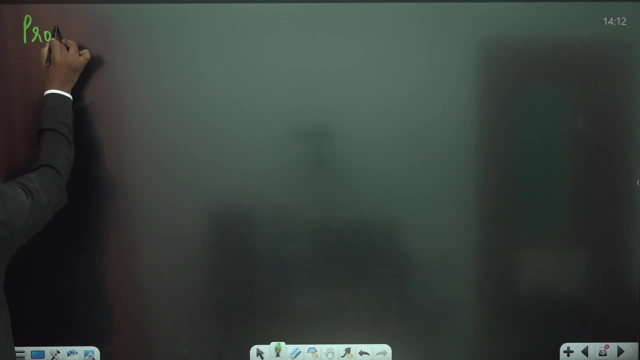 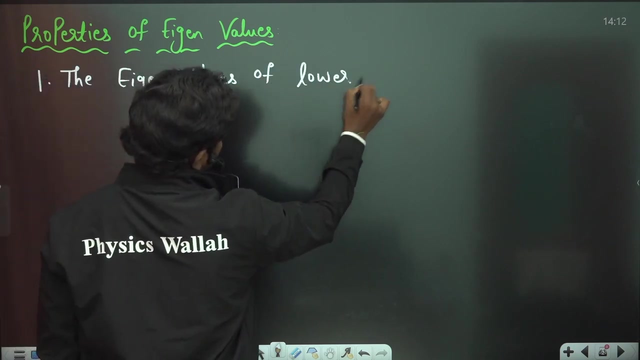 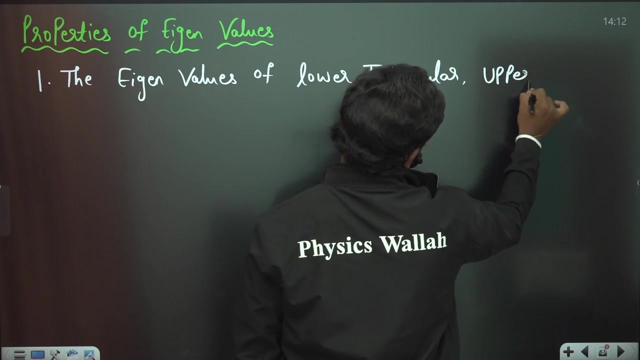 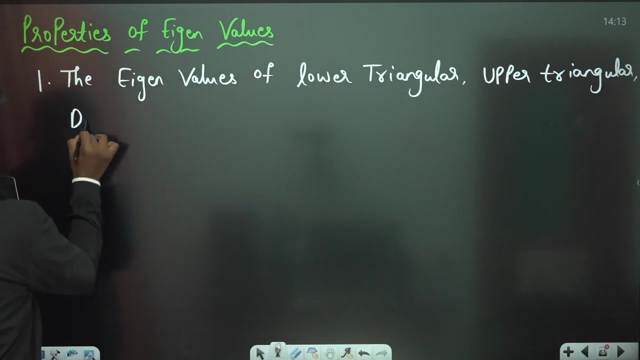 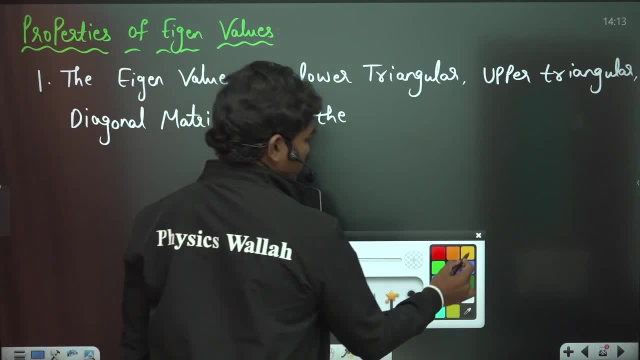 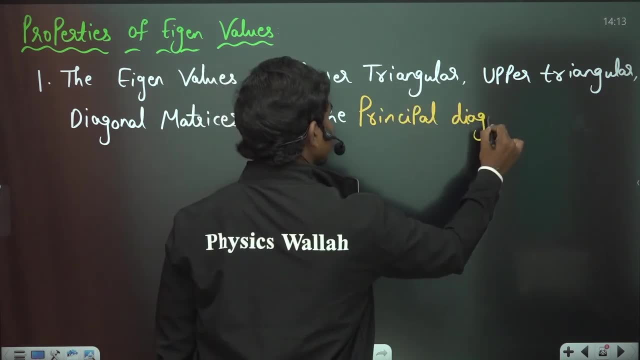 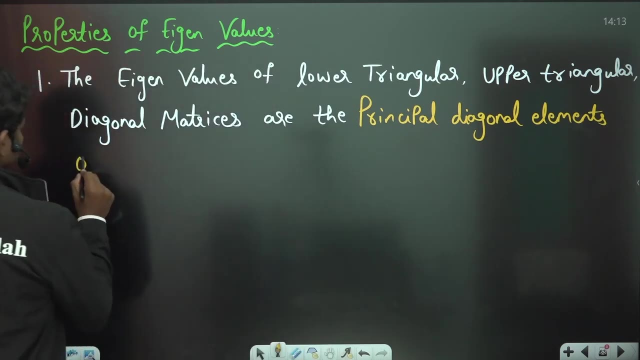 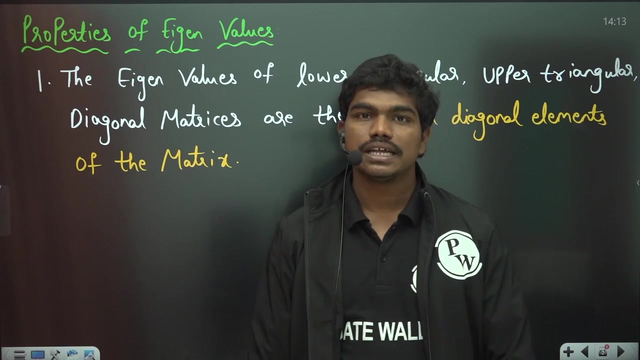 Okay, Okay, Okay. So this is how we have the result, because obviously it's way. you might know this very well- because if a is upper triangular or lower triangular matrix, then a minus lambda i will also be upper triangular or lower triangular, because this lambda i subtraction will only make. 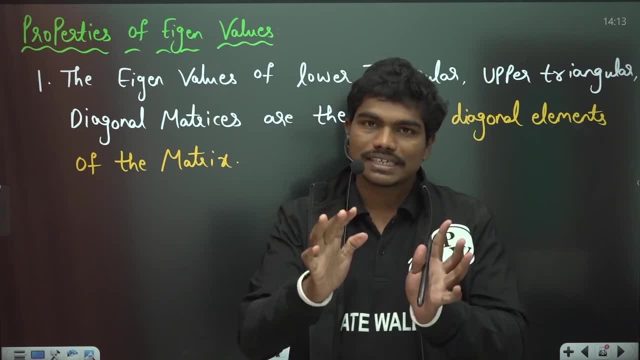 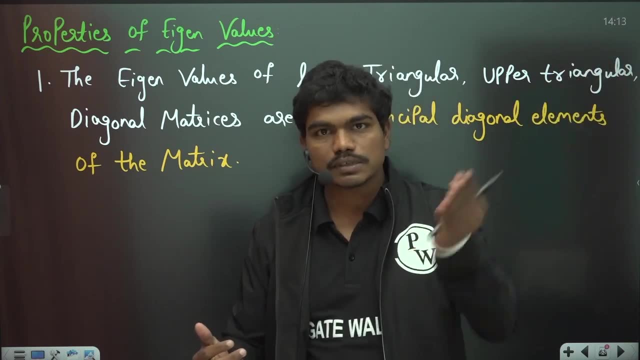 changes to the principal diagonal elements, correct. so if the matrix is by default upper triangular or lower triangular, a minus lambda, i will also be upper and lower triangles. so the debt is nothing but product of the principal diagonal elements. basically means- if i want to explain you for 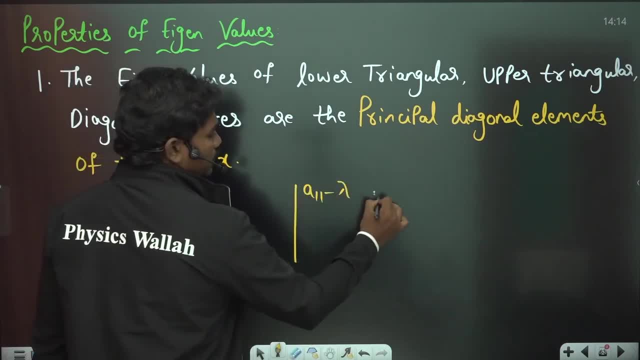 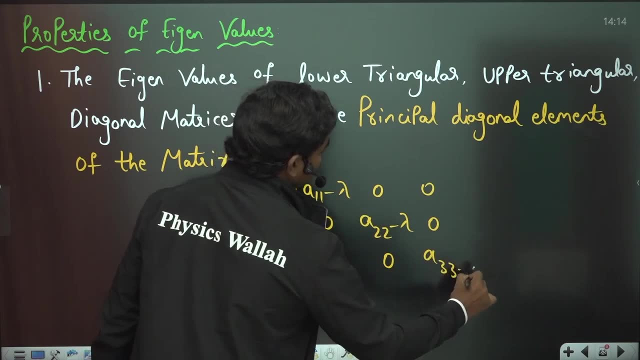 example, if i take a diagonal matrix, a minus lambda, i will be like this: 5, 2 by 2. i'm talking about so 0, 0, 0. a 3, 3 minus lambda is equal to 0. correct example? i'm talking about one example here. so if 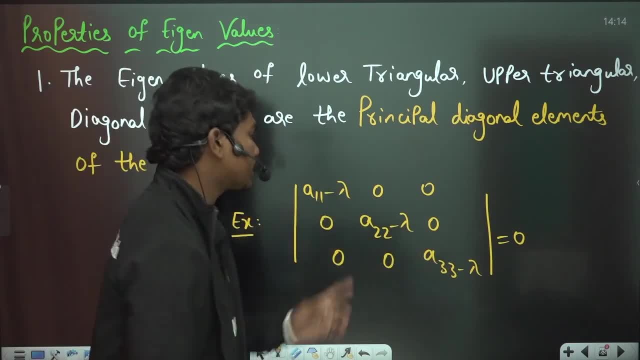 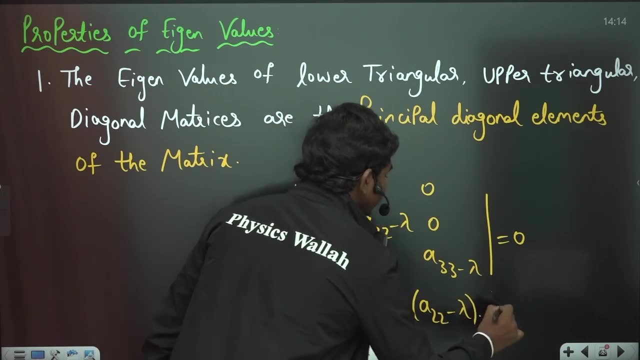 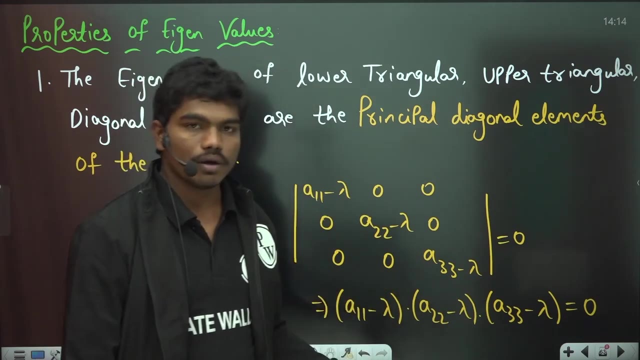 you see, if you want to calculate the determinant of this matrix, again the product. so this implies a 1, 1 minus lambda into a 2, 2 minus lambda, into a 3, 3 minus lambda, this is equal to 0, basically here. okay, so if that is equal to 0, then obviously you know this is already in factorized form. so if 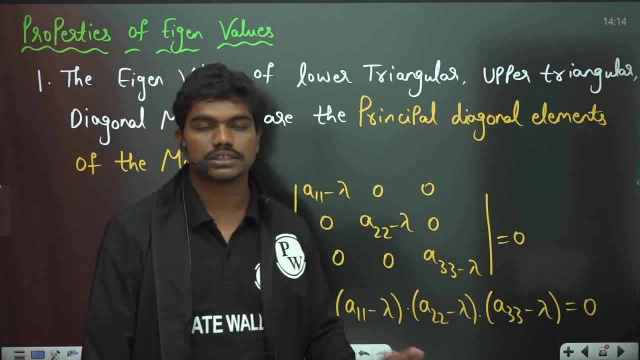 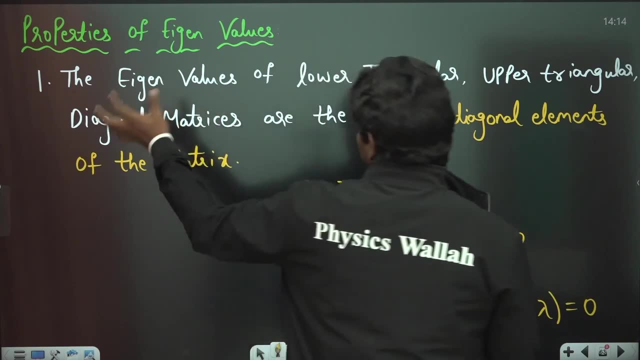 this has to be 0. lambda can be a 1, 1 or a 2, 2 or a 3, 3. so basically, these are the things which we have, you know, principal diagonal elements of the given matrix. okay, so this is one very, very important property and this property you 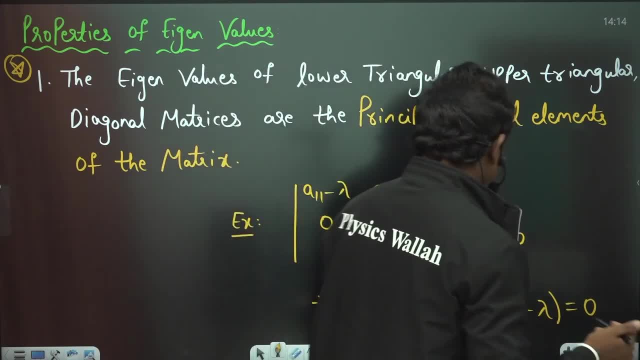 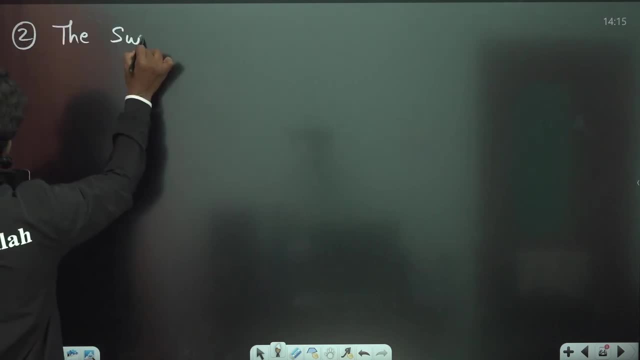 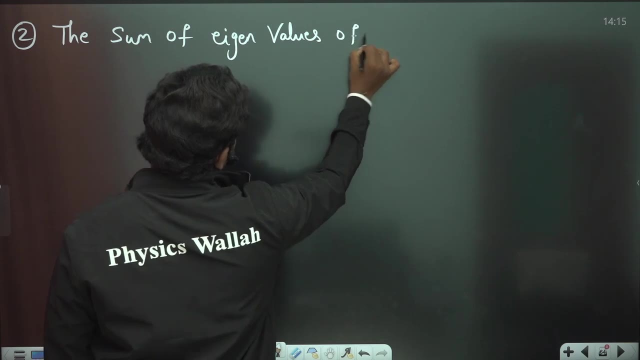 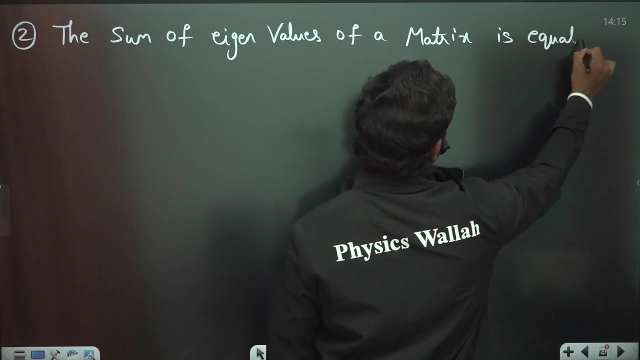 know generally many times you will be using that in examinations. okay, and second, i would like to give you second property: the sum of eigenvalues of a matrix. the sum of eigenvalues of a matrix, the sum of eigenvalues of a matrix is equal to, is equal to trace of the matrix, trace of matrix. so 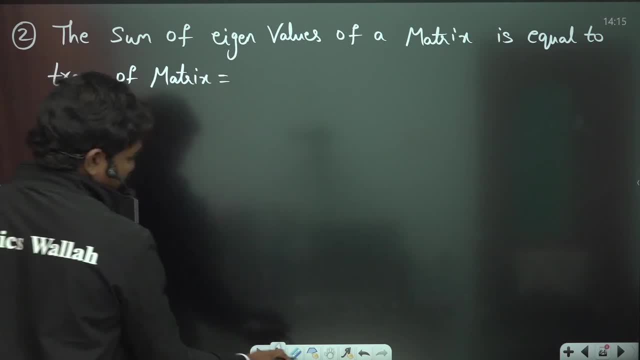 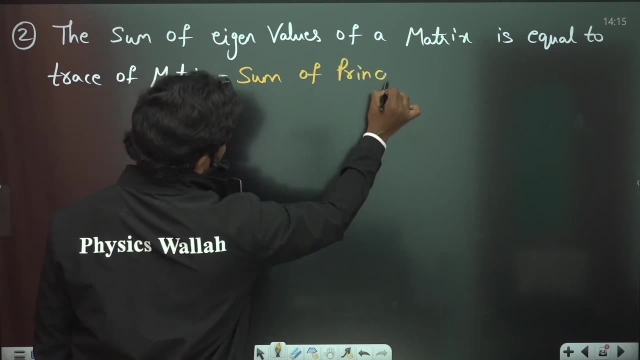 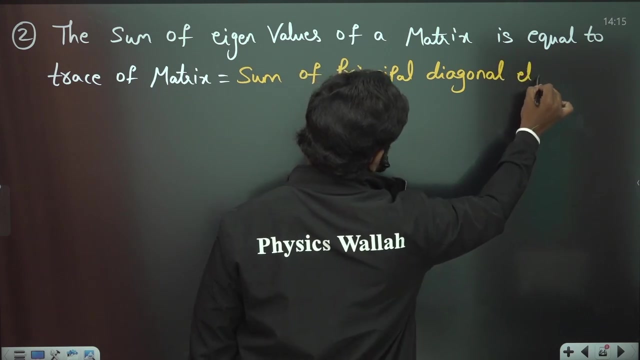 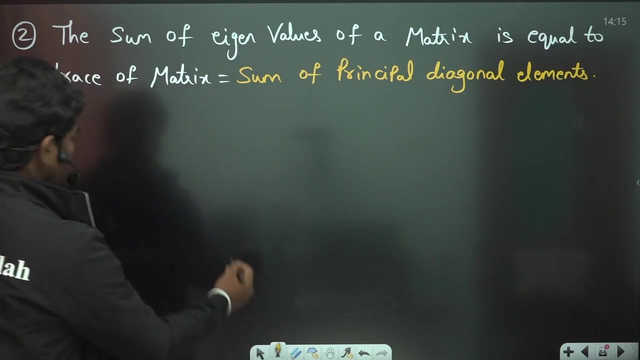 basically, what is trace of a matrix? this is equal to sum of principal diagonal elements. sum of principal diagonal elements, sum of principal diagonal elements basically here. okay, so this is equal to sum of the principal diagonal elements. means basically, if you want to mention this sigma i is equal to 1. 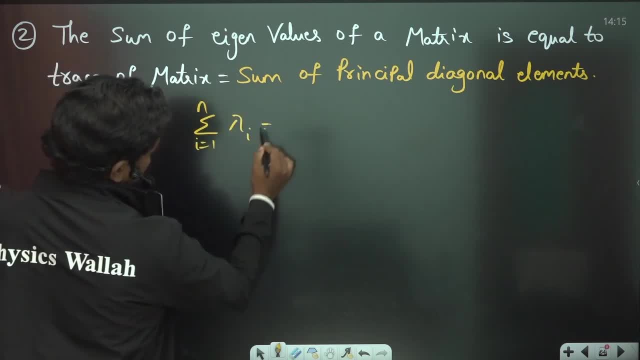 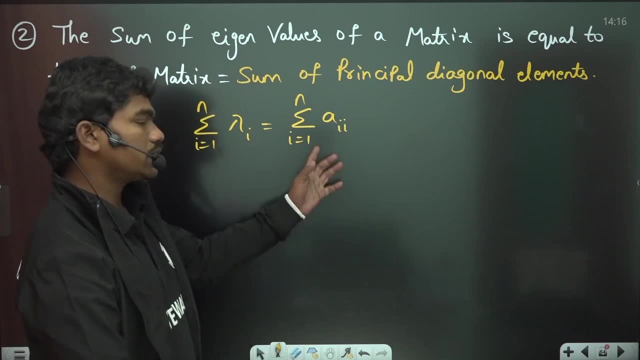 to n. let us suppose if you have n by n matrix, then you will have n eigenvalues. so this is equal to sigma i, is equal to 1 to n a i, i, that's it okay. so a 1, 1 plus a, 2, 2 plus a, 3, 3, and so on. a n, n, okay. 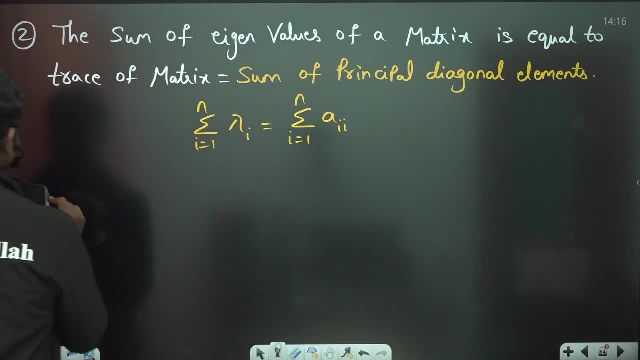 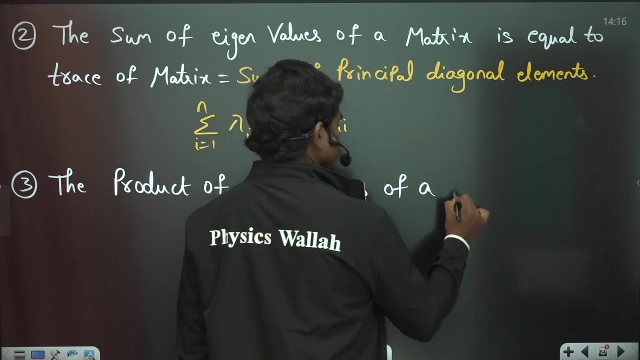 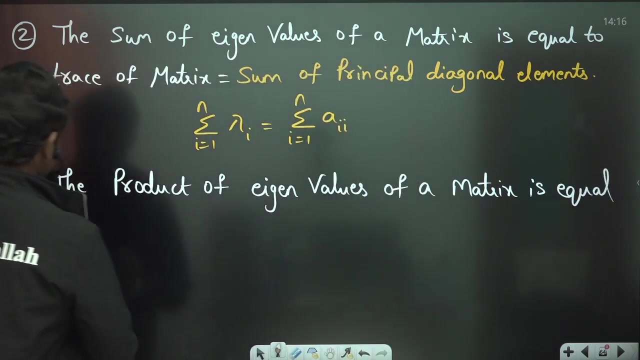 now coming to the third very important property: the product of eigenvalues. the product of eigenvalues of a matrix, of a matrix, is equal to- again, it's very important and very simple property, of course, is equal to the determinant of the matrix, is equal to the determinant of a matrix, is equal to the determinant of a matrix. 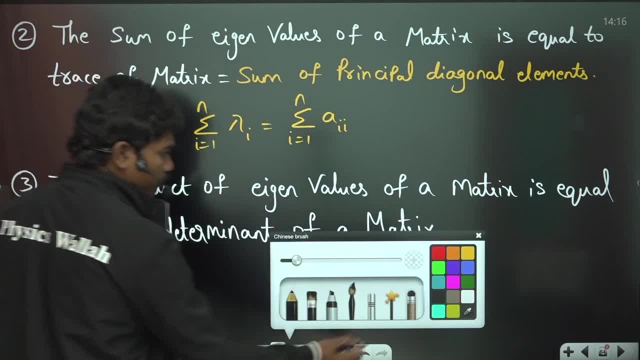 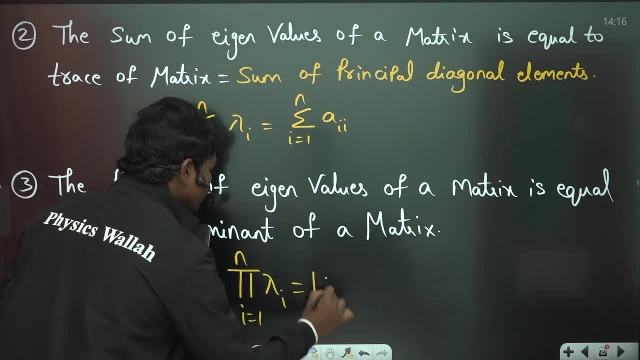 is equal to the determinant of a matrix. okay means basically, if you take the product, if you take the product, notation, product i is equal to 1 to n lambda i. if you take this, this is nothing but determinant of a actually here. okay, so these two properties are very much important. 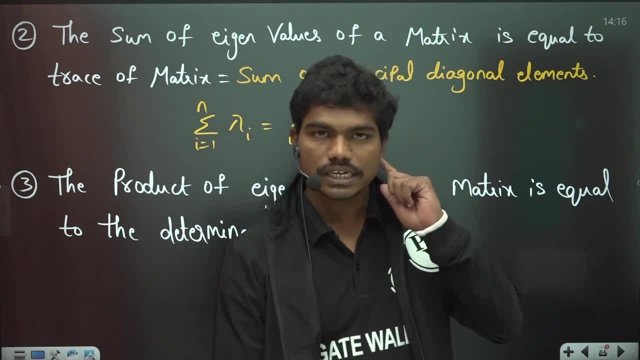 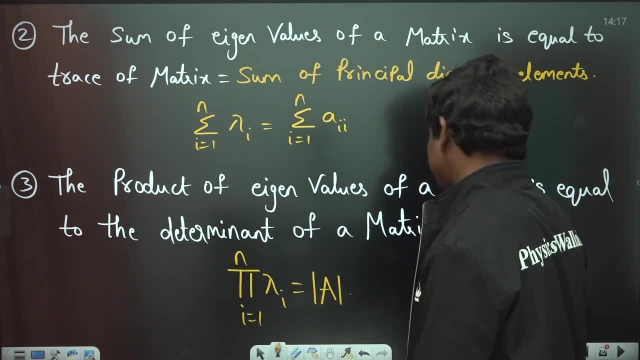 and many times you can expect a question from this- that sum of the eigenvalues is actually equal to the sum of the principal diagonal elements, and product of the eigenvalues is equal to the- you know- determinant of that particular matrix. okay, now i'd like to give. 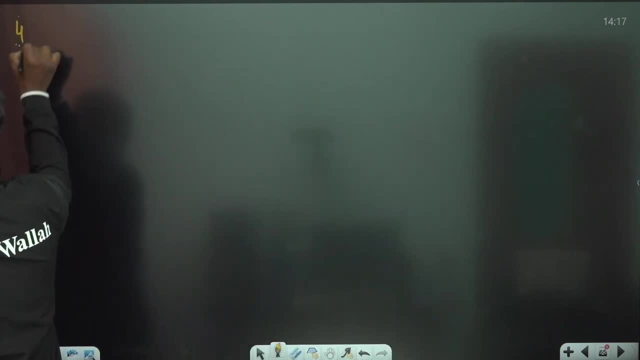 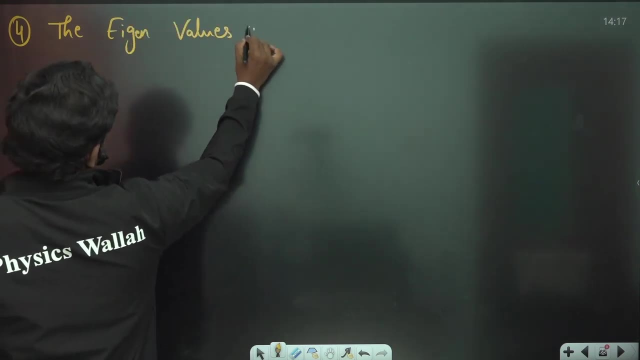 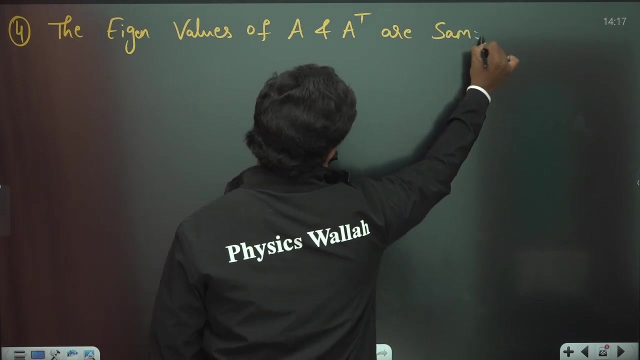 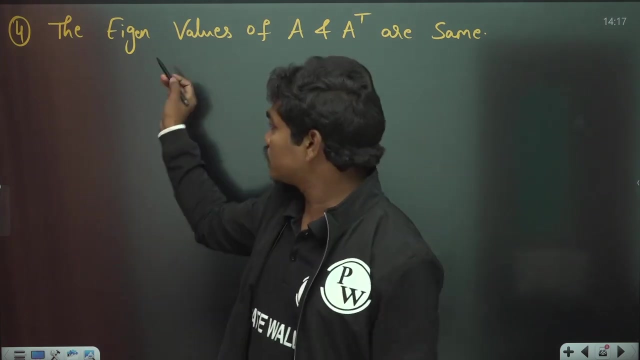 you some more, uh, good information. the eigenvalues of the eigenvalues of a and a transpose. a and a transpose are same because, you see, this means basically, if you take this eigenvalues of a and a transpose, if you see, the diagonal elements remain the same and, of course, the determinant, basically determinant of a minus lambda or a transpose. 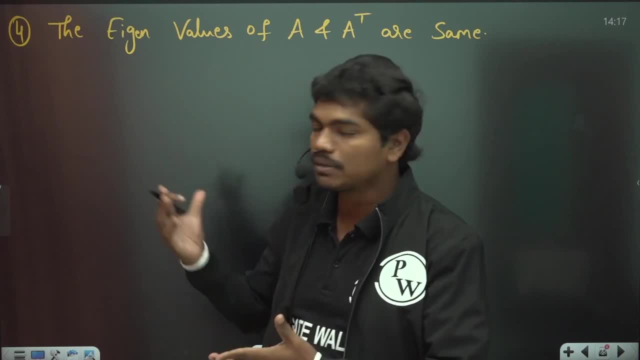 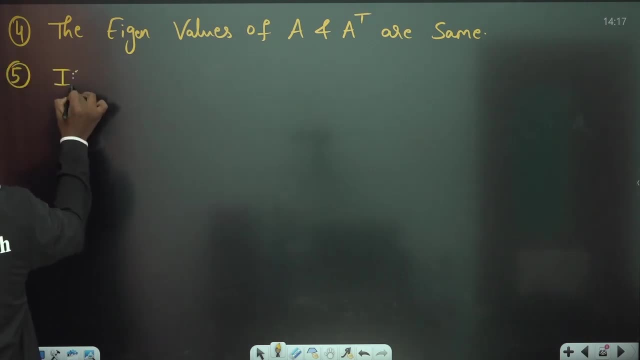 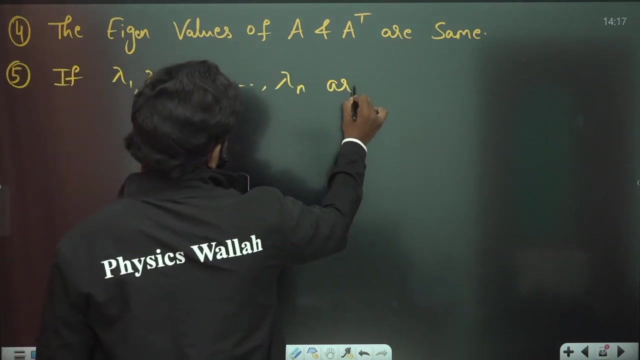 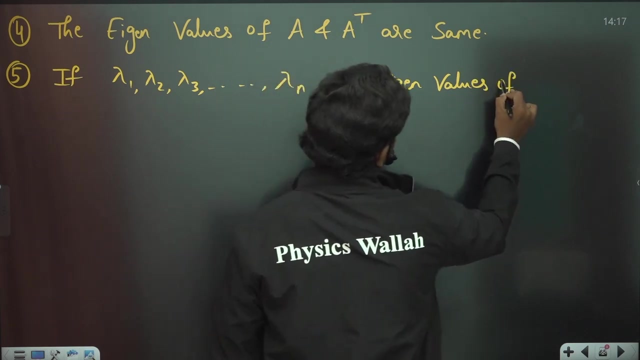 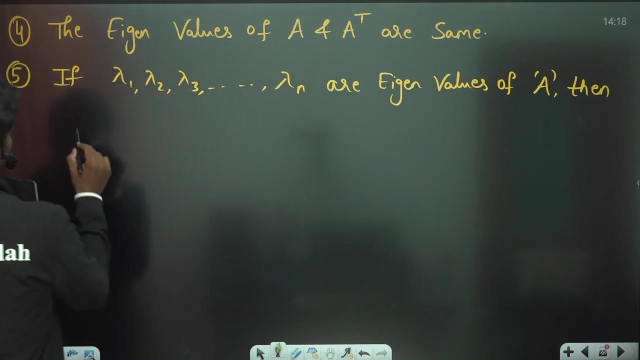 minus lambda i, that remains the same. okay, so that's how. the characteristic polynomial is same and eigenvalues will also be same. okay, now five: if lambda 1, lambda 2, lambda 3 and so on, lambda n are eigenvalues of a, eigenvalues of a, eigenvalues of a, then first point: you have certain points here. 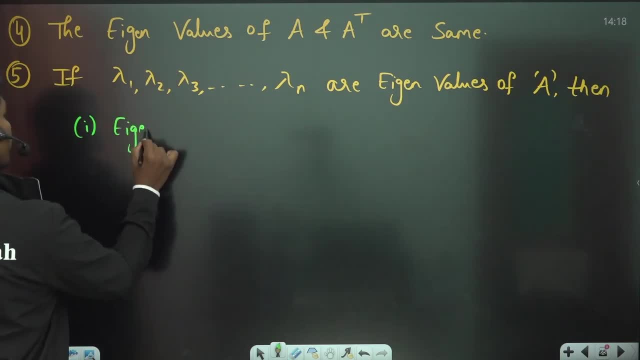 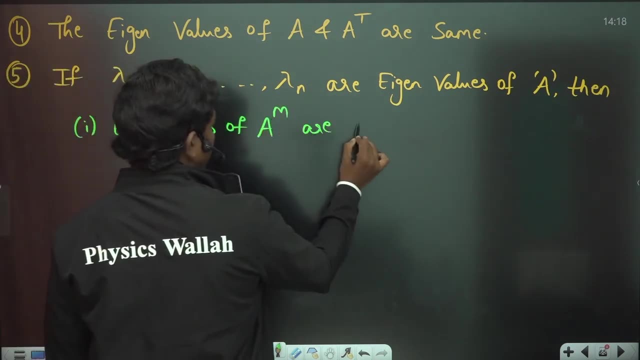 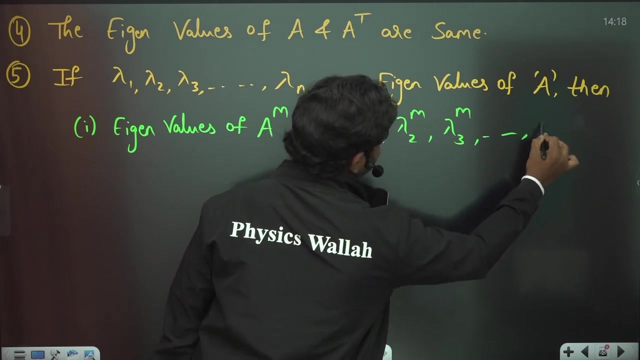 so first point: you have certain points here. so first point: you have certain points here. so the eigenvalues of eigenvalues of a power m are lambda 1 power m. lambda 2 power m. lambda 3 power m and so on, lambda n power, and so on. this result will basically go on. 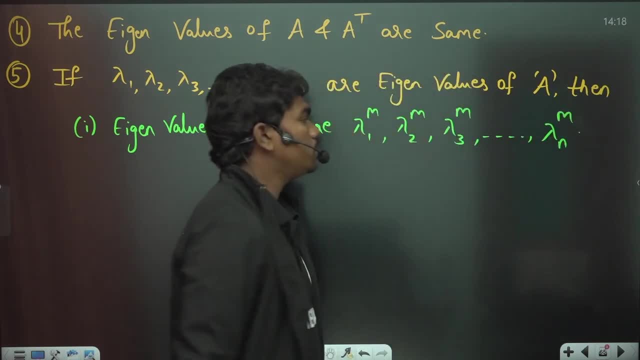 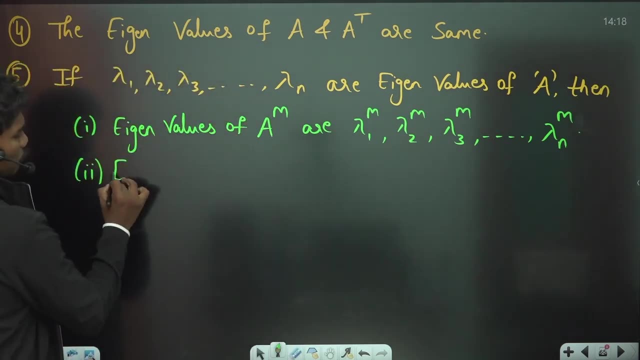 and so on. lambda n power m okay. so when you raise the power of a matrix, then automatically the eigenvalues also raise their power. and second, so when m value is equal to minus one, one special. and third time ich we understand that beta isantes have an eigenvalue of zero in the 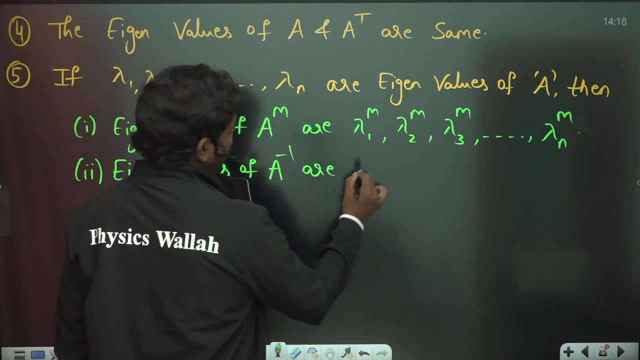 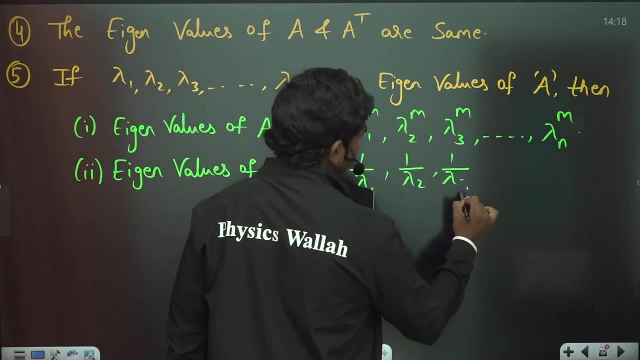 case of a inverse. when eigenvalues of a inverse are 1 by lambda 1, because lambda 1- whole power minus 1, gives you 1 by lambda 1 by lambda 2, by lambda 3 and so on, this goes onto 1 by 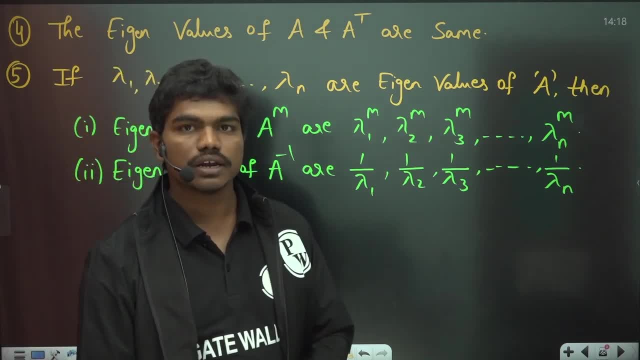 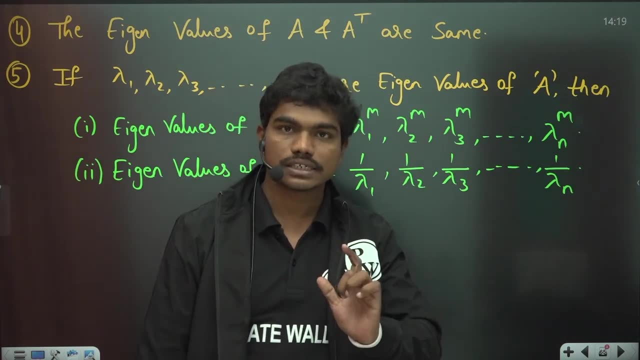 lambda n. okay, so here you can observe one thing. let us suppose if matrix is singular means. let us suppose if the determinant doesn't exist. if matrix is singular, that means definitely at least one and value will have been definitely zero. correct, because you see, determinant is Key, finding, is integral to lambda n, is because in danger of perdition. 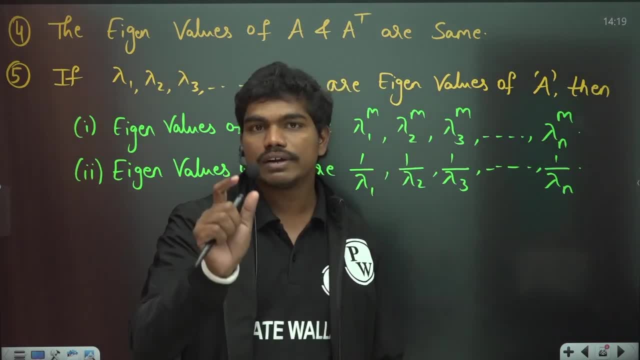 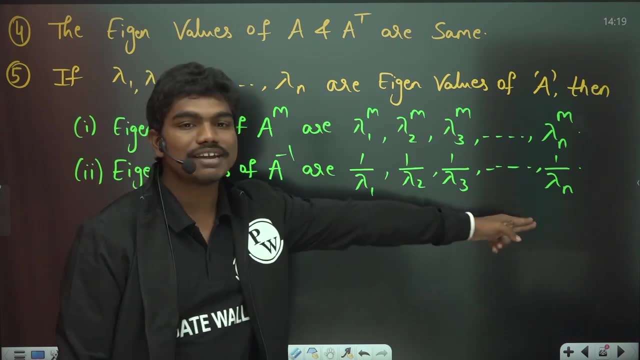 is nothing but product of the eigenvalues. so if determinant is zero, definitely one of the eigenvalues should be definitely zero. so that's how, here, if you are writing a inverse, that means you are very much sure that no eigenvalue is zero. so they all are in the denominators. okay, so no. 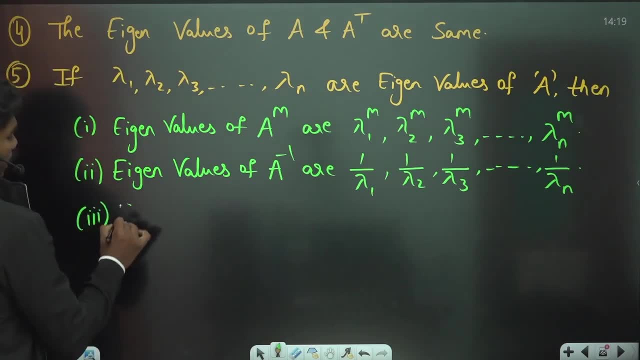 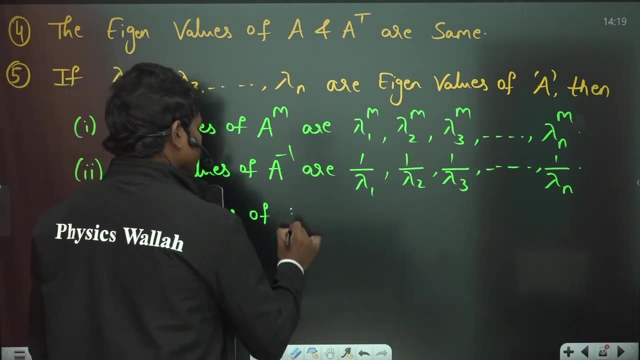 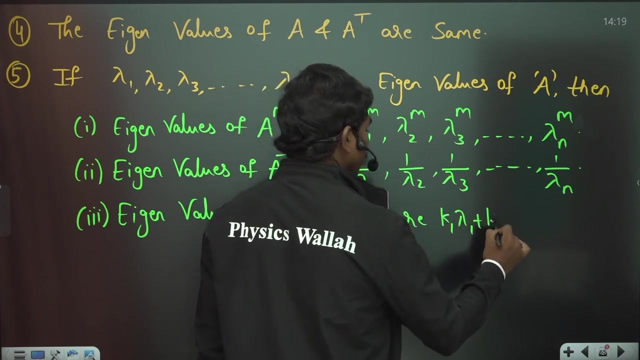 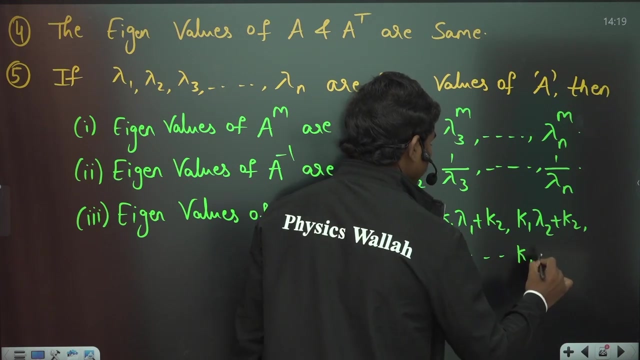 issues. next: third: eigenvalues of eigenvalues of some constant k1 into a plus some b, some k2 into i. let us say: let us suppose, if you have some combination, k1 into a and k2 into i are k1 times of lambda 1 plus k2 comma, k1 times of lambda 2 plus k2 comma, and so on, k1 lambda n plus k2. this 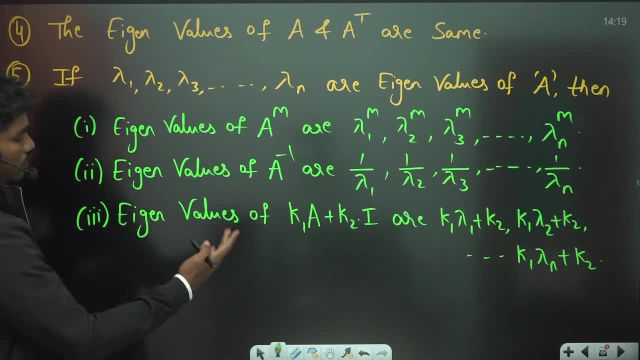 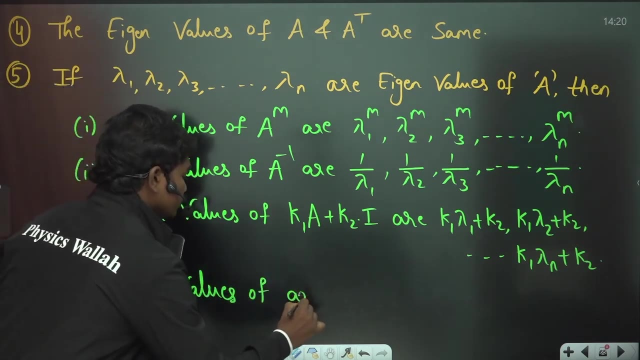 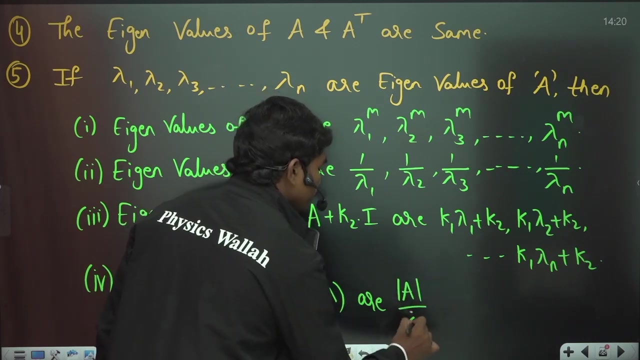 is how we have the eigenvalues of some, uh, advanced, you know terms basically here, okay, and a and a transpose has the same eigenvalues, of course, okay. next fourth one: eigenvalues of adjoint a. eigenvalues of adjoint a. are that a by lambda 1? this property is very important, okay, sometimes. 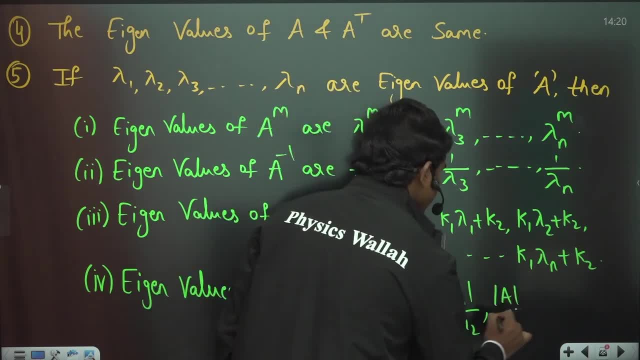 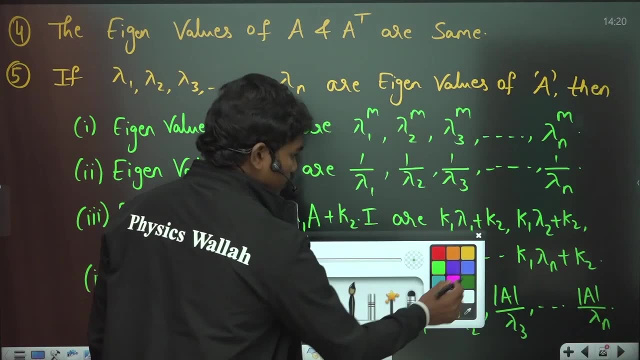 they ask you this lambda 2, that a by lambda 3 and so on, that a by lambda n. okay, so this property is again- uh, you know, very much important property generally. many times they try to frame a question on this property. so this property is again- uh, you know, very much important property generally. 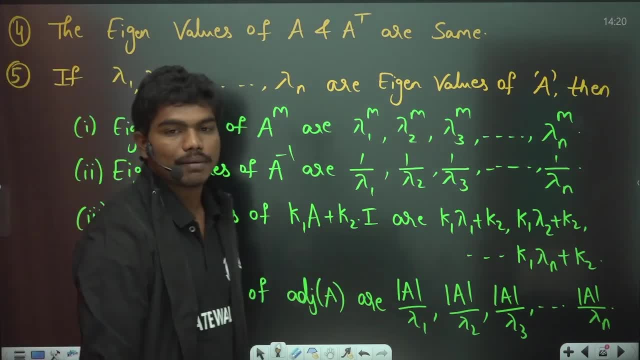 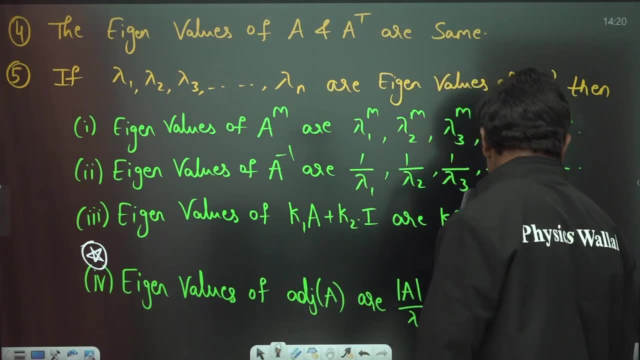 many times they try to frame a question on this. so eigenvalues of this adjoint a are of this form: that a by lambda 1, that a by lambda 2, and so on. basically, they exist like that. okay, and so, generally, these are the things which could be available for you, and now i would like to go for. 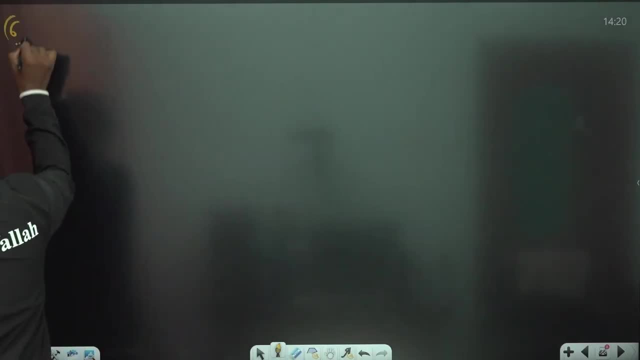 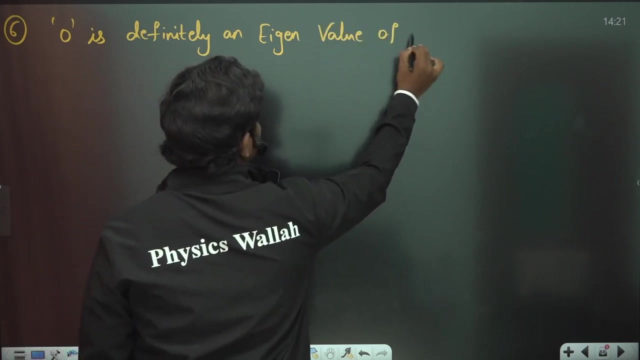 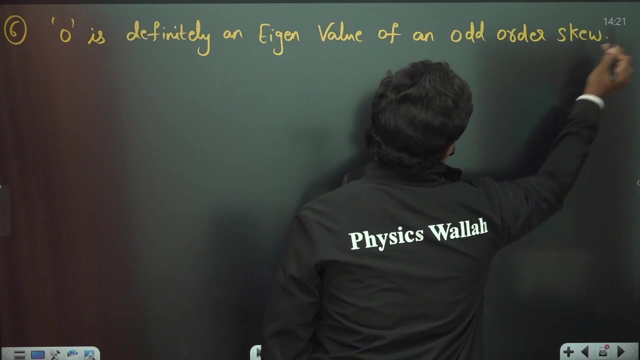 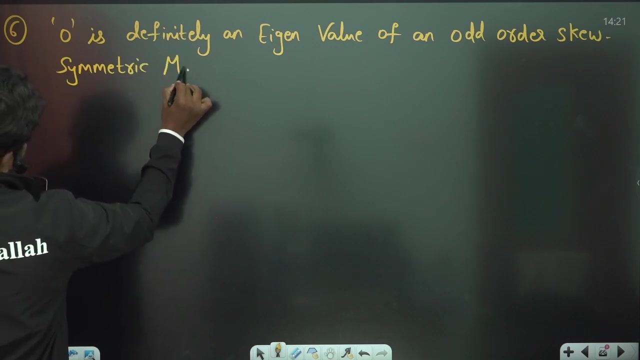 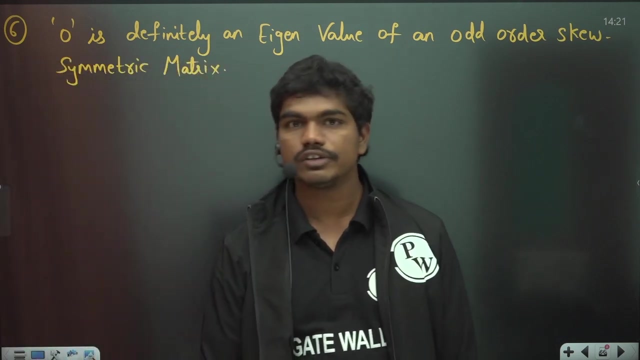 a sixth property, which is again some good property: 0 is definitely an eigenvalue. 0 is definitely an eigenvalue of an odd order skew, symmetric matrix. an odd order skew, symmetric matrix, basically okay. so zero is definitely an eigenvalue of odd order skew. symmetric matrix means basically: if you see you, 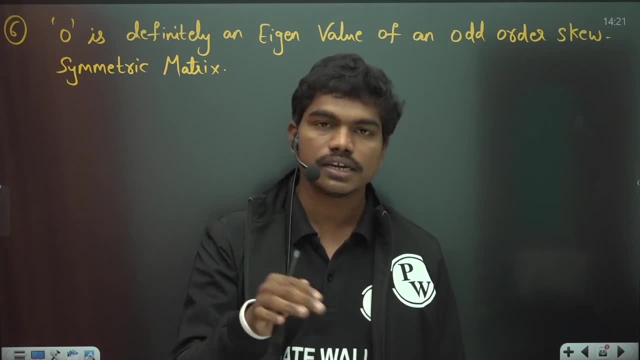 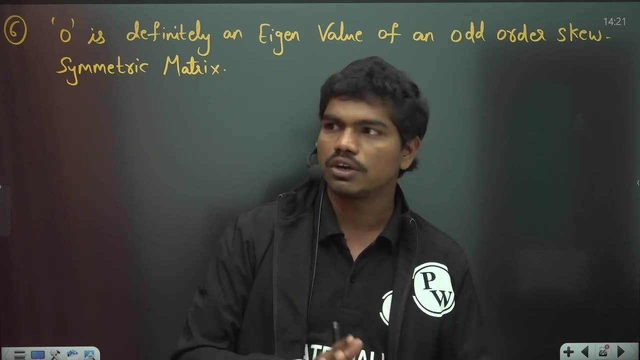 know that every skew symmetric matrix of odd order has zero determinant. so if that is zero, definitely one of the eigenvalues should be zero. okay, so this is one very good statement, because now you know logics of all these things. it's not like you buy hard something or you just take it. 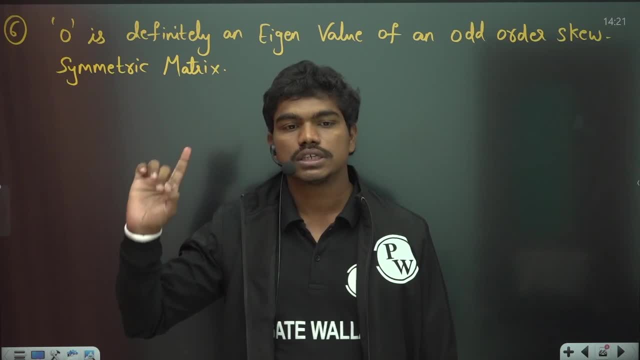 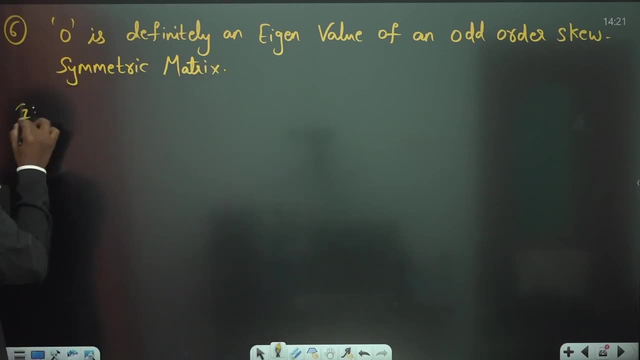 for granted. you know why zero is definitely an eigenvalue? because for every odd order skew symmetric matrix- your determinant should be zero. clear, now let us continue. seven eigenvalues of skew symmetric matrix. or you can write eigenvalues of real symmetric matrix, symmetric matrices: if you take symmetric matrix normally, ml. real symmetric matrix. 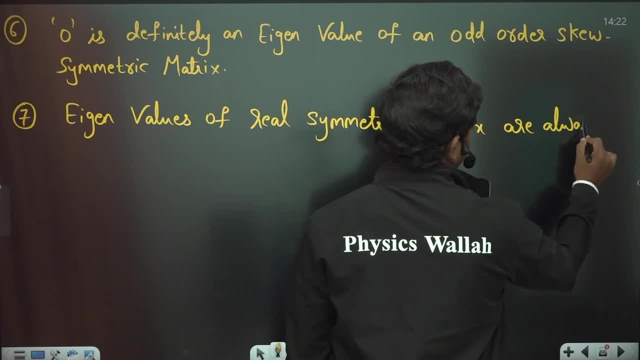 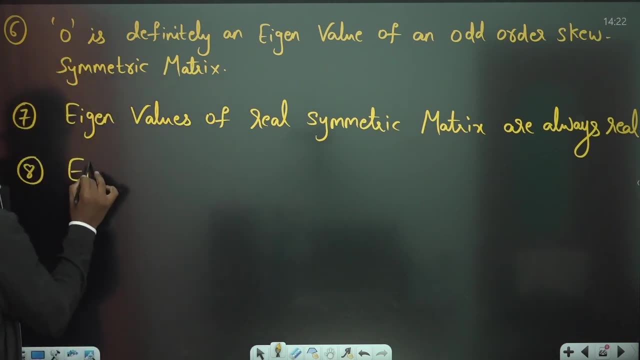 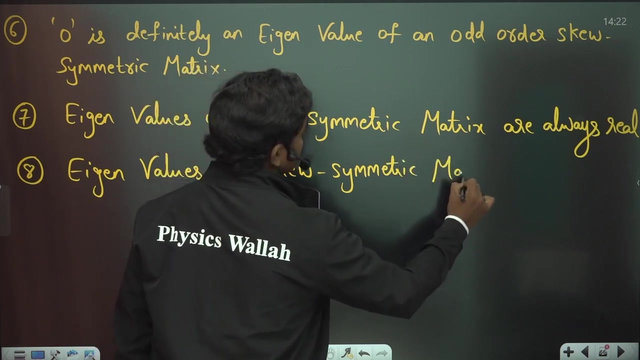 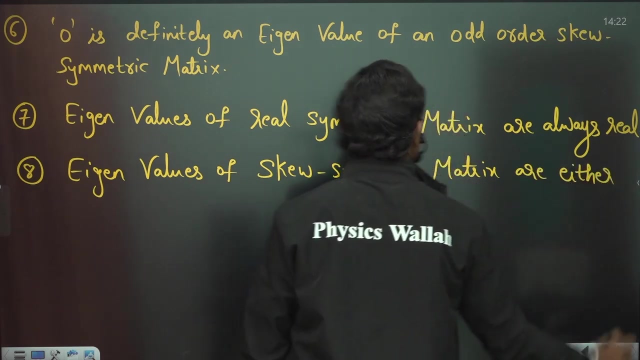 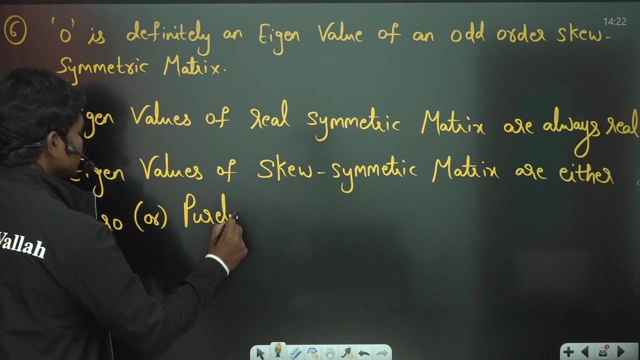 are always real, are always real. okay, next eighth property: i could give you something like eigenvalues of eigenvalues of, uh, you know, eigenvalues of skew symmetric matrices. if you talk about skew symmetric, eigenvalues of skew symmetric matrix are either zero- either they'll be zeros in case of odd order- or purely imaginary. what is the meaning of purely? 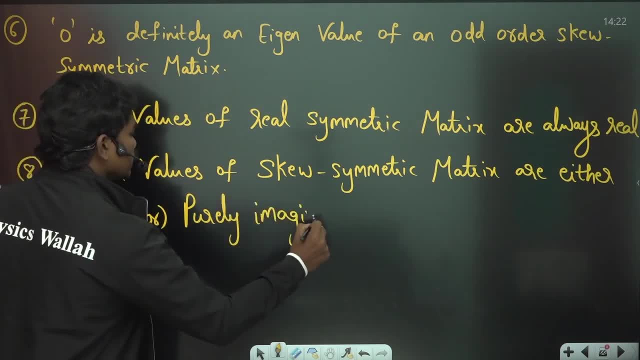 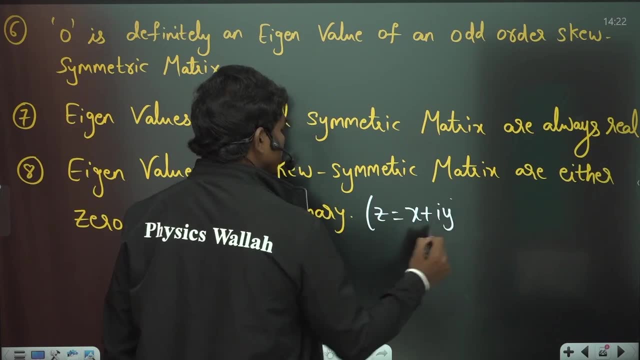 imaginary. if you take any complex number, you know basically, uh, complex numbers have of this form: z is equal to x plus i, y. if you take this as the complex number, then you know x is called the real part, y is called the imaginary part. so here, in these cases, this x value will be zero. okay, you'll. 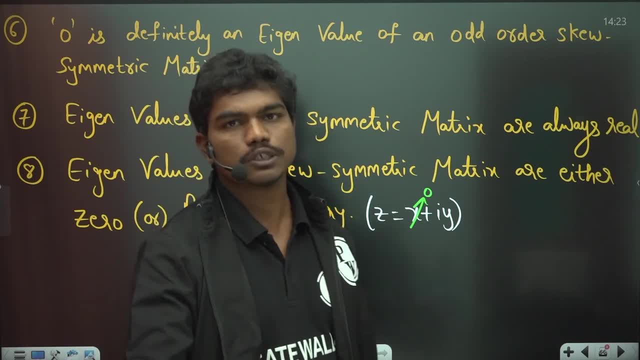 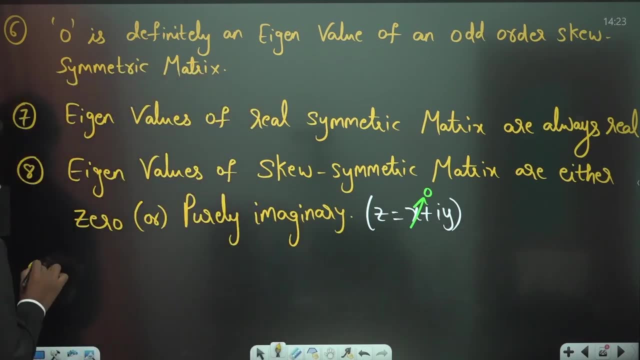 have only the y part, so your complex numbers come out in the form like i, into some constant, basically. so that's how you have this: eigenvalues of skew symmetric matrix, one important property. i give you here nine eigenvalues of eigenvalues of eigenvalues of- uh, you say eigenvalues. 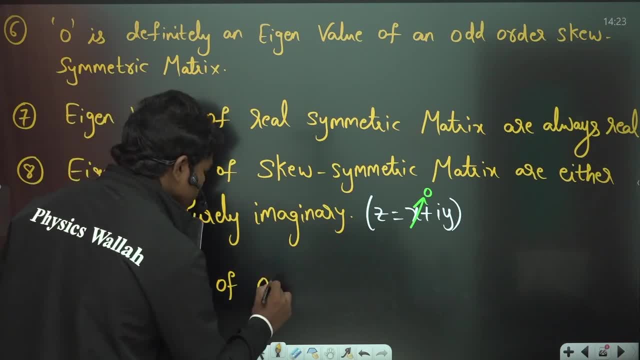 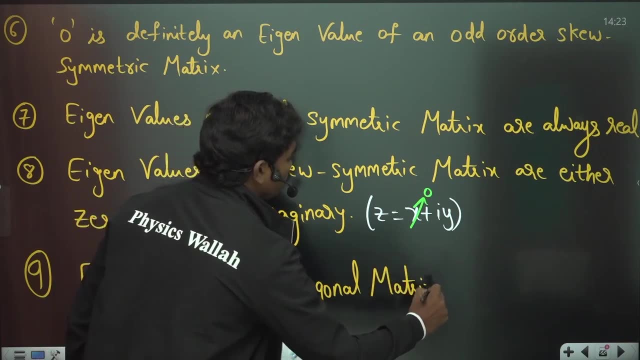 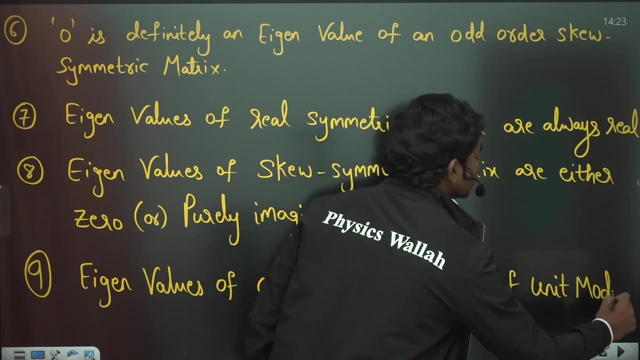 of uh, for example. uh, we can talk about orthogonal matrix. eigenvalues of orthogonal matrix matrix are of unit modulus. are of unit modulus means basically: what's the meaning of that? if they are real numbers, they'll be either plus or minus one. if they are complex numbers, then they turn out to be some complex numbers. 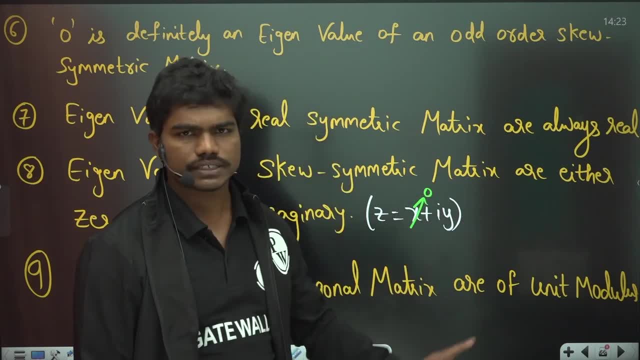 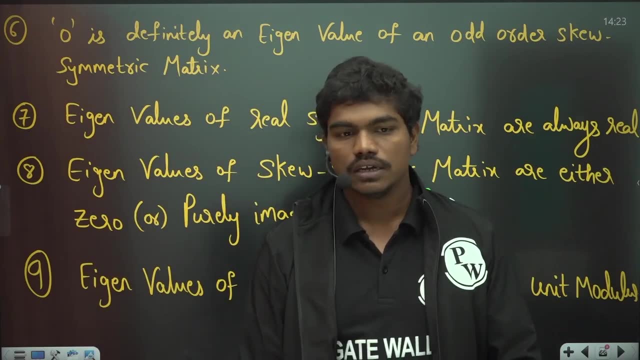 of magnitude one. okay means basically, if you calculate root of x square plus y square, that x square plus y square will be one actually here. okay, now there are many more properties actually, but at the gate level, uh, this are properties which they generally ask you. but coming to some advanced, 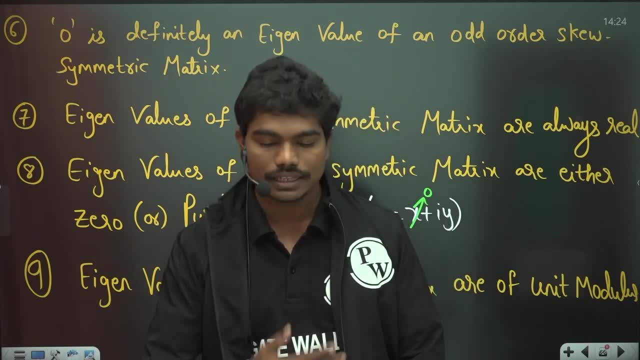 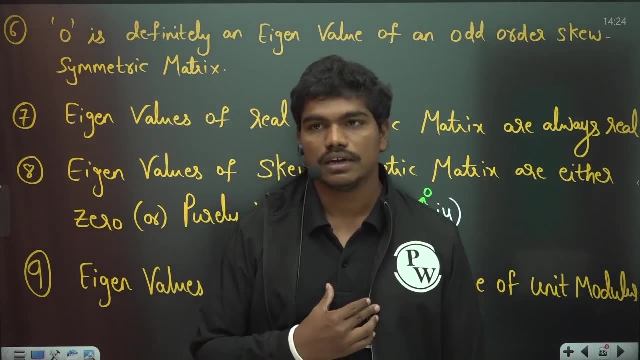 levels. linear algebra is a fantastic subject and i would like to give and thank actually one person right now, because you know, uh, by this time you might have passed already. they asked, or the end of hours of video, but uh, all this knowledge, what i've got is from one person. 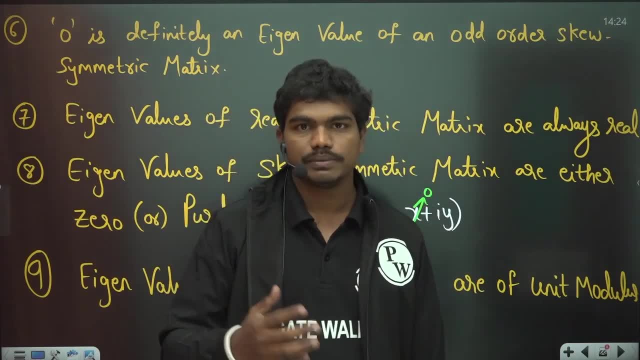 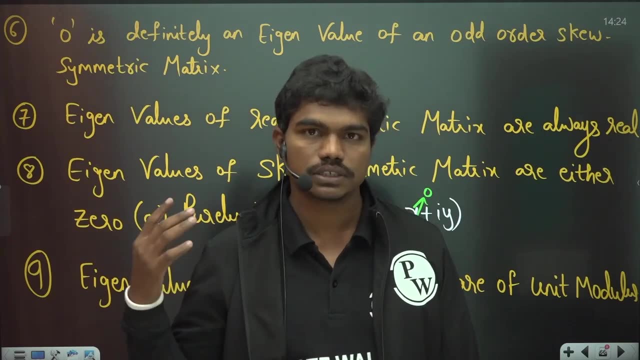 gilbert strang. he has a very good book on linear algebra- linear algebra by gilbert strang. he is basically from mity and you know he is fantastic professor across the uh. he is known for his works in linear algebra across the world. okay, so you can also find him on some youtube or somewhere. in m separating. 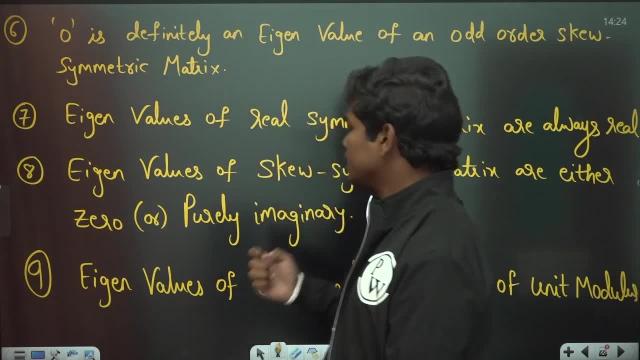 web courses anywhere. so he is really a fantastic guy. okay, so eigenvalues of orthogonal matrix are of unit modulus basically, and yeah, this is the maxim eigenlijk value i can get it equal to 1.5 and you can take the problem here to knees. as to the point, is d and 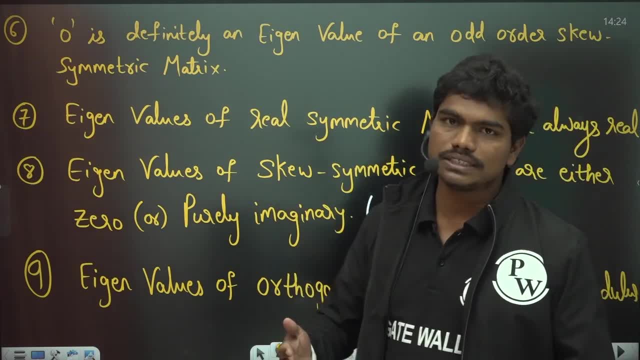 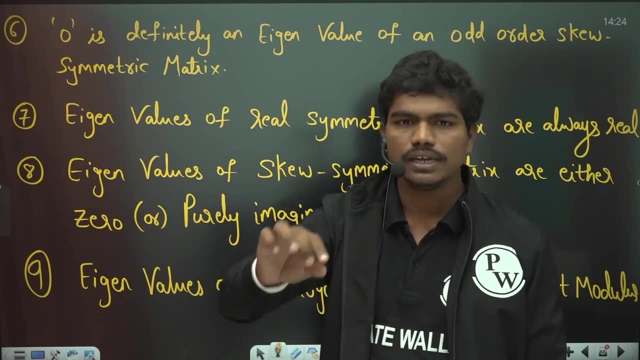 yeah, if you keep on, there are certain many other things like, for example, every eigenvalue lies within the cycle of certain radius, of where the radius is defined by some sum of two other elements. okay, we have certain things like that very importantly, but right now, coming to the gate, 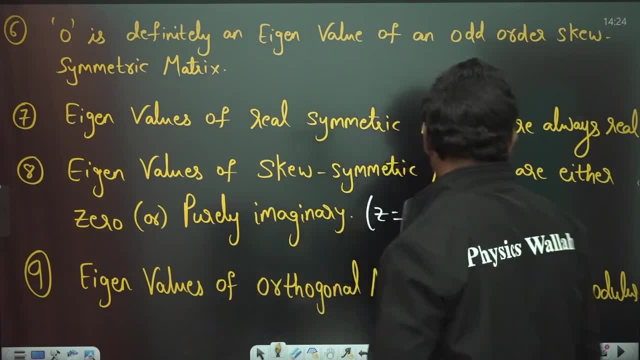 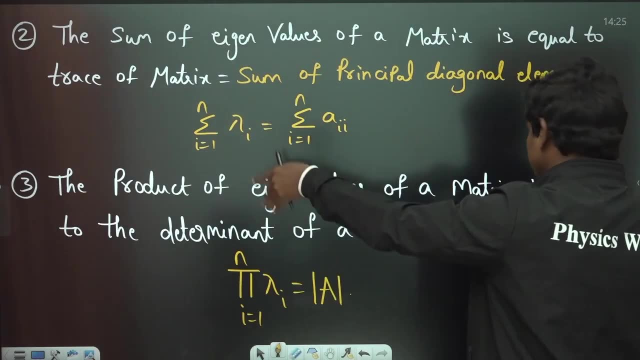 you know examination level. all these points could be definitely helpful for you. these four or five points, what i've given here, then these points and finally these two points, are definitely a lot. many questions in eigenvalues comes from these two and of course, the first one is a direct thing that you 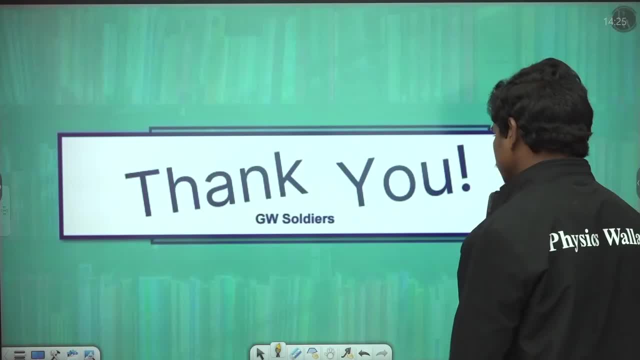 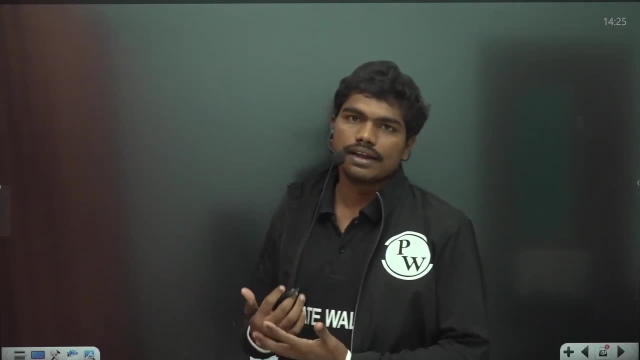 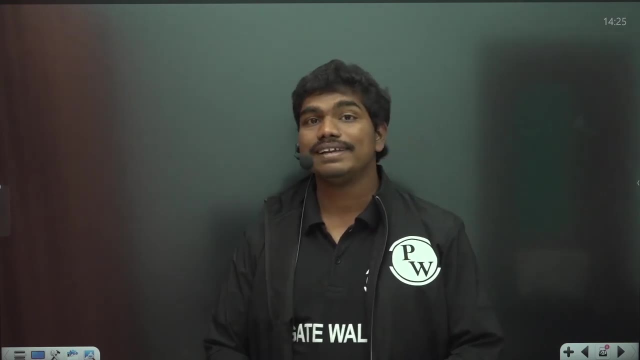 can talk of. okay, so yes, so generally, these are the things that that they come off. so 10th: okay, so fine, i think we had a lot of enough eigenvalues and how to calculate this, eigenvectors. okay, so how to calculate this eigenvectors, i will show you shortly, because we will deal with one very 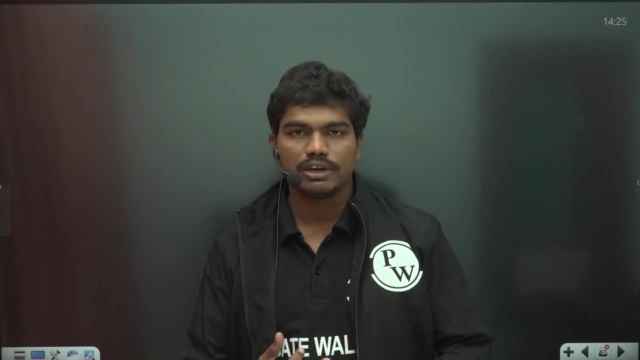 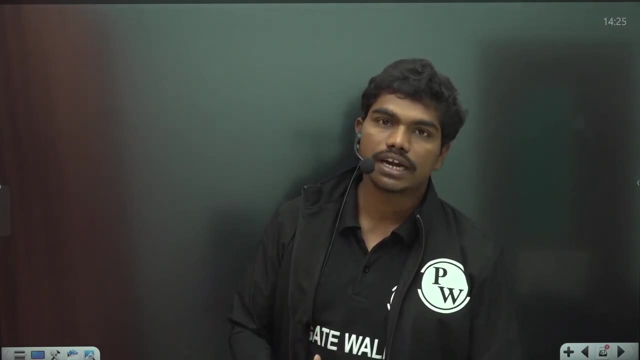 important concept which is called diagonalization of matrices. okay, because many of you might be writing engineering sciences paper as well. so this diagonalization is one very important concept in matrices. okay, we'll see what is this diagonalization. okay, look you so eigenvectors. so if you write properties of eigenvectors, 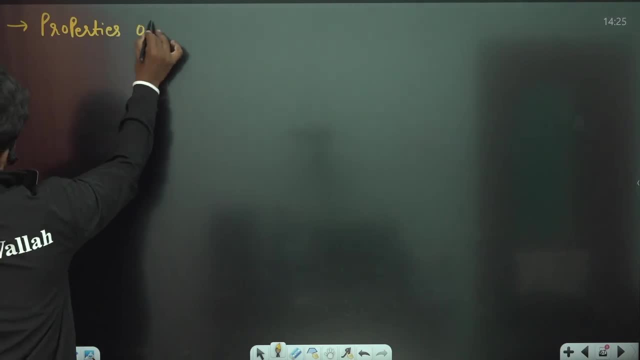 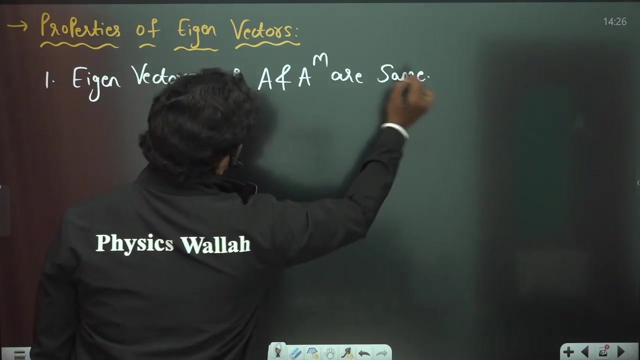 properties of eigenvectors. properties of eigenvectors. okay, so properties of eigenvectors. so if you see, we'll write one thing: eigenvectors of of a and a power y of a and a power y of a and a power y are same, because what is the difference between them? look, i'll tell. i'll make you understand one. 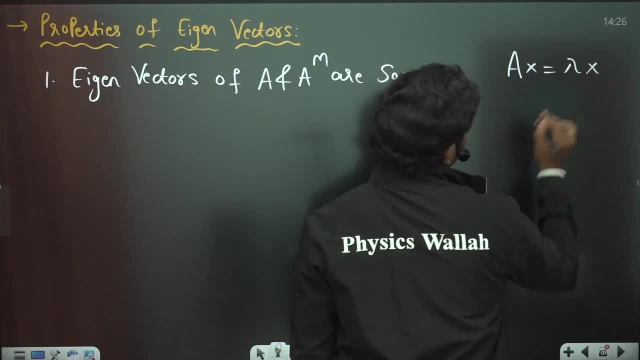 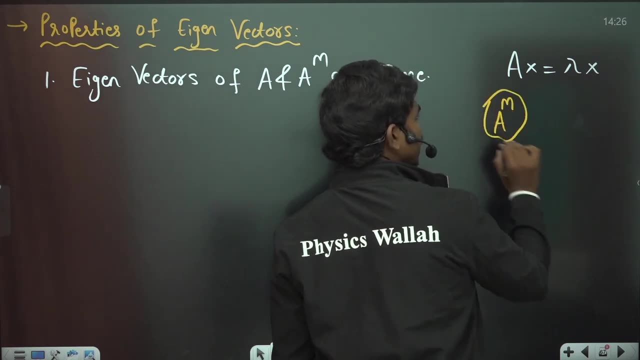 thing. normally eigenvector means ax is equal to lambda x, correct? now let us suppose if you make this power m, then what happens? let us suppose if you have a power m, then the eigenvectors corresponding to this, a power m, will be just lambda power m, times of this x. so on, look this. 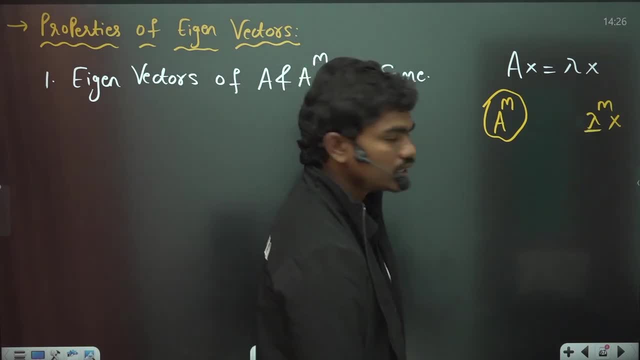 lambda. power m is just a scalar and it don't actually- uh, you know- change the things. so that's why this a power m. if you apply transpose on this, this will again match each other. so that's how you actually have the eigenvectors of a and a power. 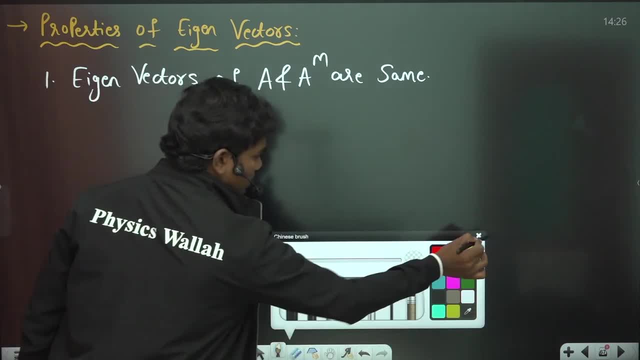 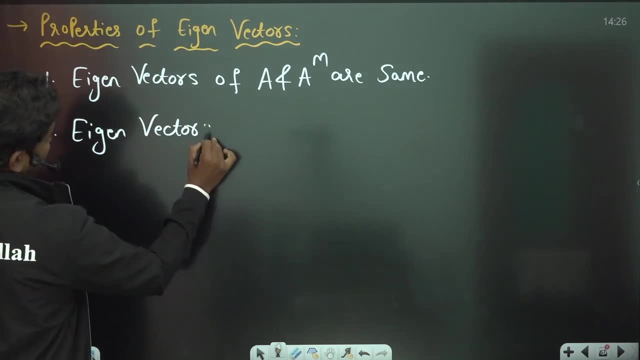 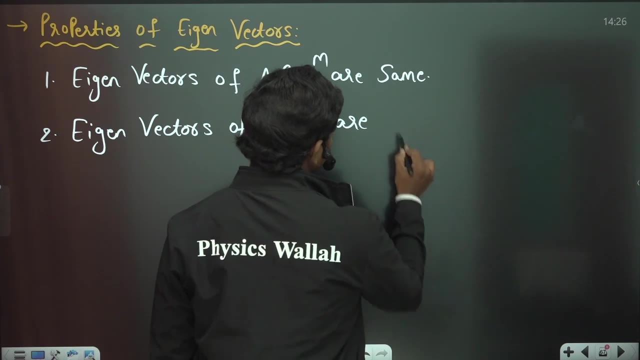 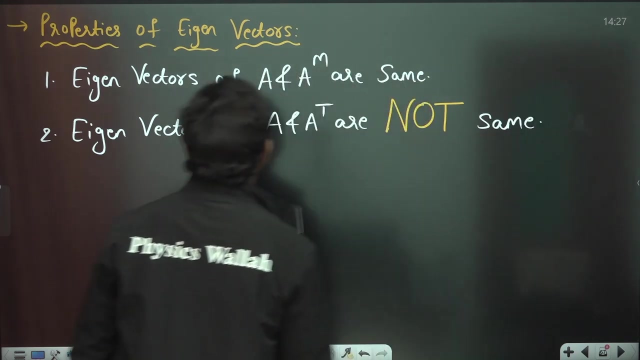 m, both same. second, i would like to give you this. so, second is, eigenvectors of a and a transpose are. i would like to change the color because this is important- not same, okay, are not same actually here. and one very good property i would like to give off. 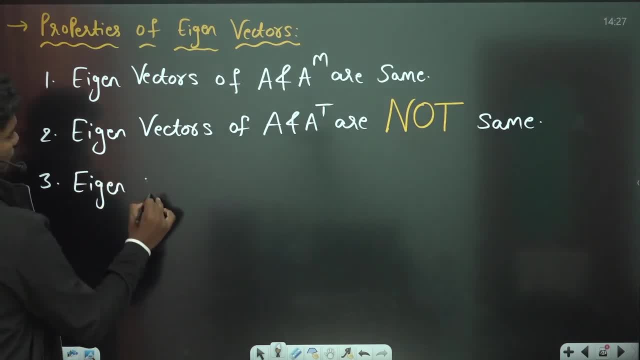 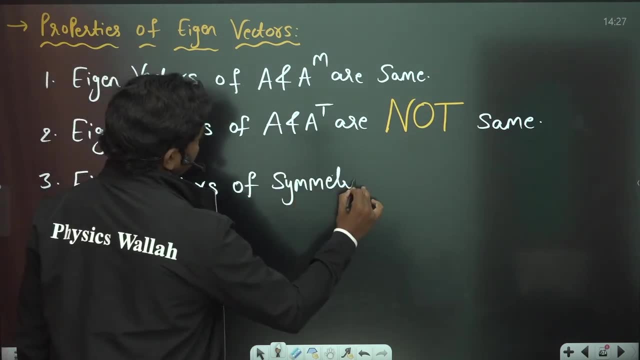 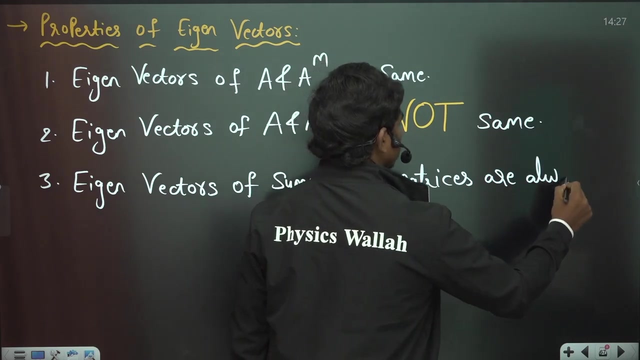 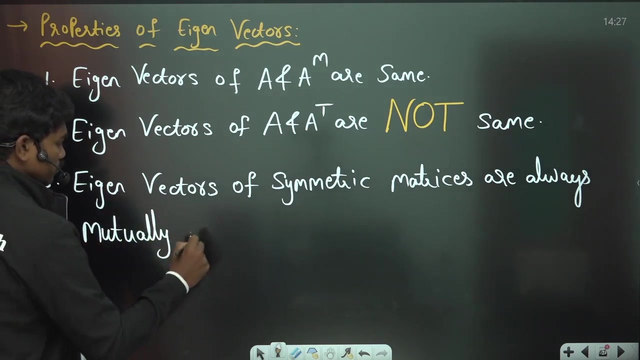 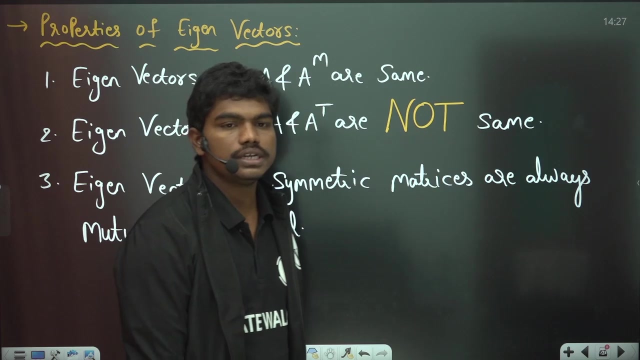 symmetric matrices, eigenvectors of symmetric matrices, eigenvectors of symmetric matrices are always orthogonal, are always mutually orthogonal, are always mutually orthogonal. okay, so these matrices are basically mutually orthogonal. actually okay, and means basically: let us suppose for 3 by 3 matrix you will have, for any given 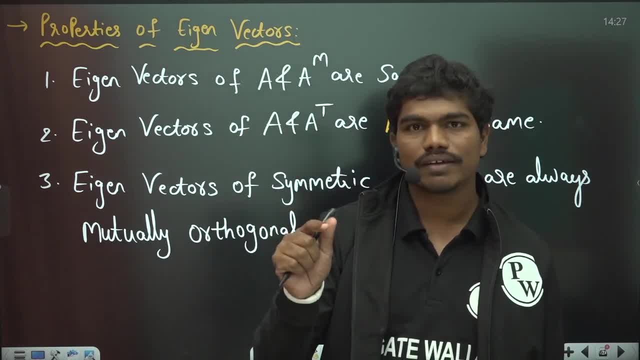 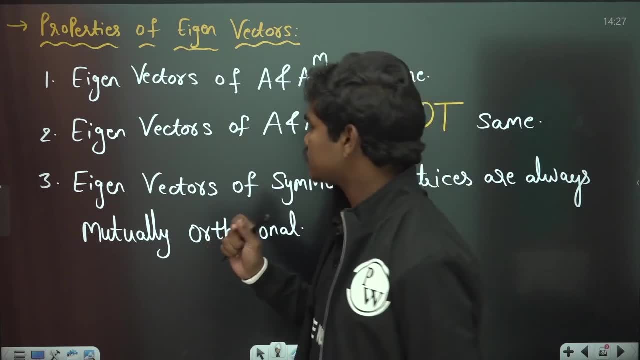 eigenvalue. you can have any number of eigenvectors, but if you take any two eigenvectors corresponding to two different values of lambda, then definitely this dot product is going to be zero. okay, so now let us try to understand this this: eigenvectors of symmetric matrices are always mutually